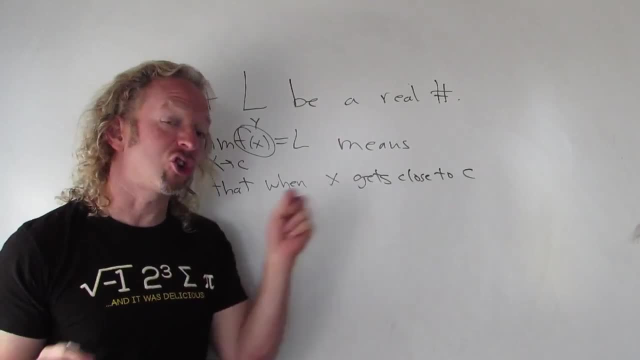 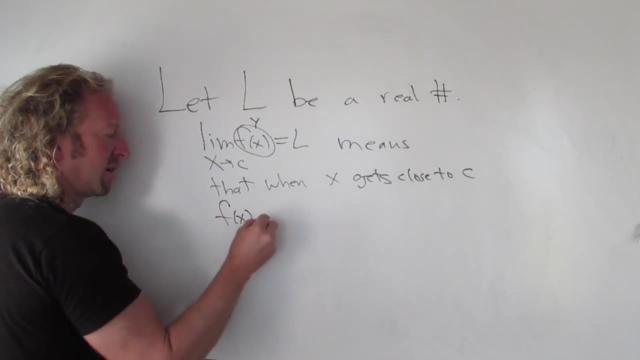 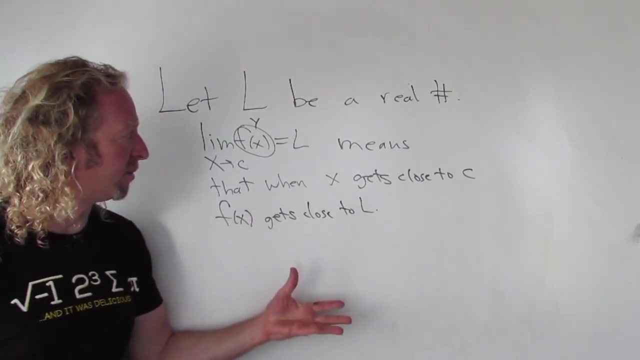 you might say: what does close mean? Ah, so how close? As close as you like, right, You can literally get as close as you like. So when x gets close to c, f of x gets close to L, Maybe now we should do a simple example of a limit So you can see what. 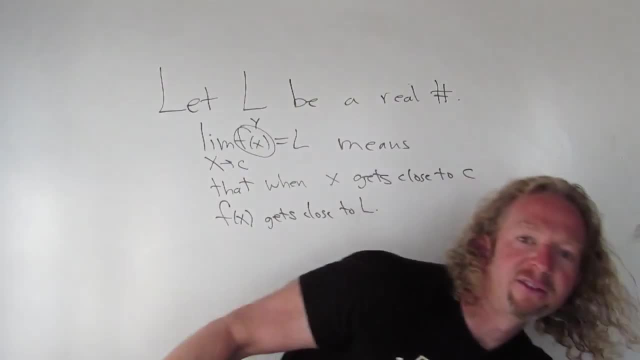 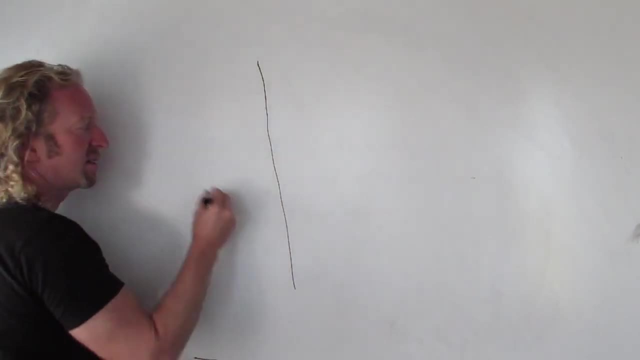 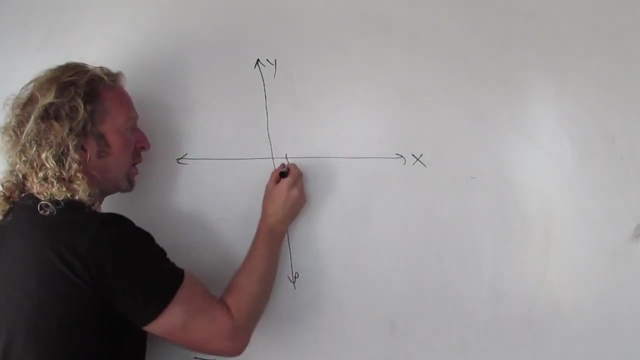 it means intuitively, and so you can see what it means graphically. I think I have something here to erase, so let's do it. So let's draw a quick graph. Say we have the y-axis, and say we have the x-axis, So x, y- And let's make up some numbers. Let's see So like 1,, 2,, 3,, 1.. And I'll 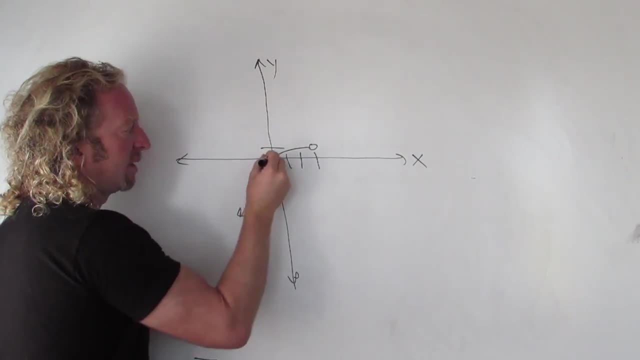 put a little hole here, And I'll put a little hole here And I'll put a little hole here And I'll come down here and go through 0. And come up here at 1,, 2,, 3, 4.. Just use different numbers. 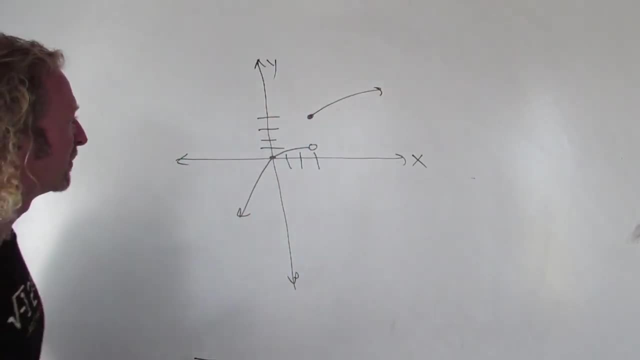 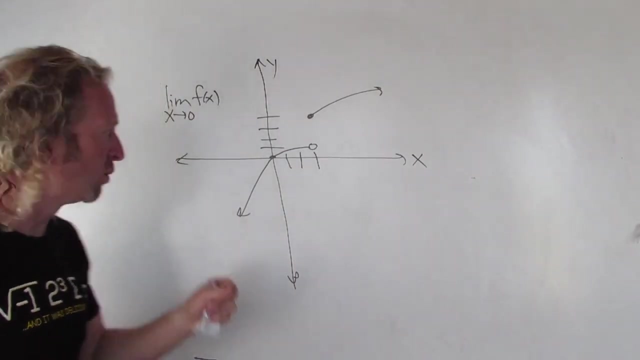 And that's good. So let's compute some limits. Let's do it. So first let's find the limit as x approaches 0 of f, of x. So this is asking what happens to the y value when x gets close to 0? So the idea is this: You want to approach 0 from both directions: from the left: 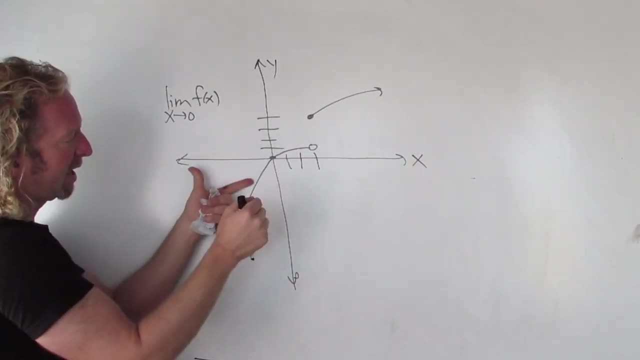 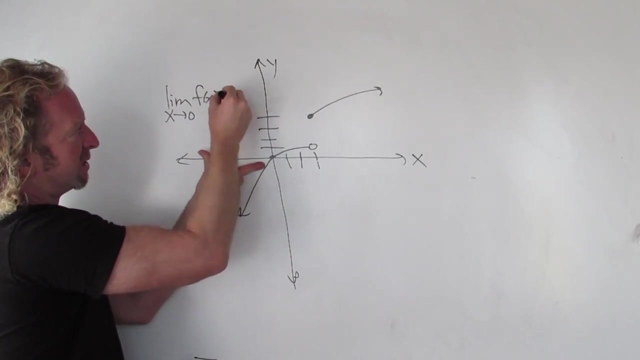 and from the right. So when x gets close to 0 from the left, the y value is 0.. When x gets close to 0 from the right, the y value is 0. Therefore, the limit is 0.. So you have to be able to approach. 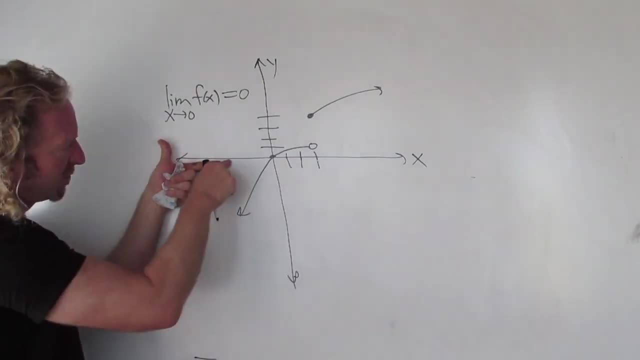 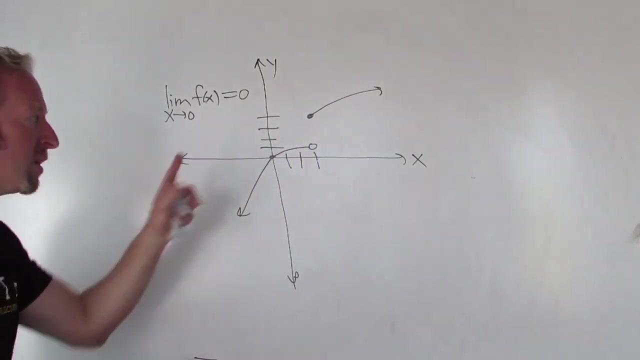 from both directions to get an answer. So, as x approaches 0 from the left, the y value approaches 0.. As x approaches 0 from the right, the y value approaches 0.. Therefore, the limit is 0.. Let's look at approaching 3.. Let's approach 3.. However, 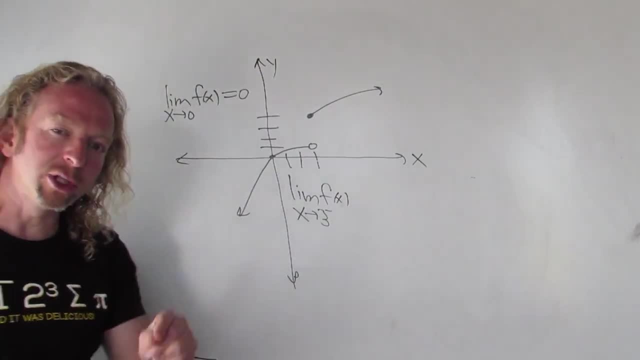 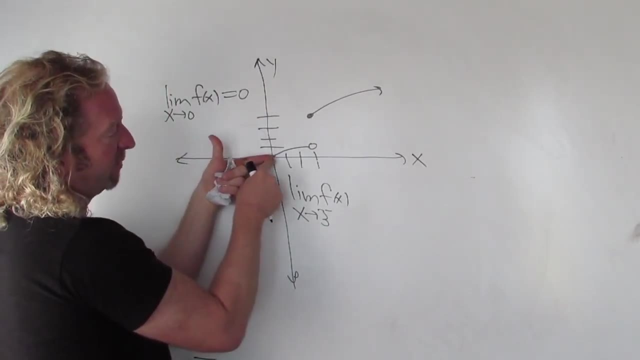 I'm going to put a little negative sign here. So this negative sign means we're approaching only from the left. If you put a plus sign, it means you're approaching from the right. So we're approaching 3 from the left. So as the x value approaches 3 from the left, 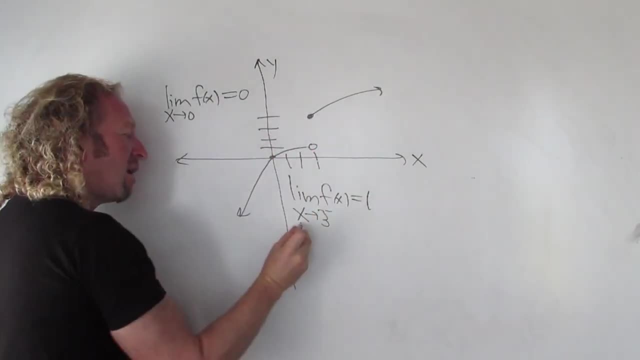 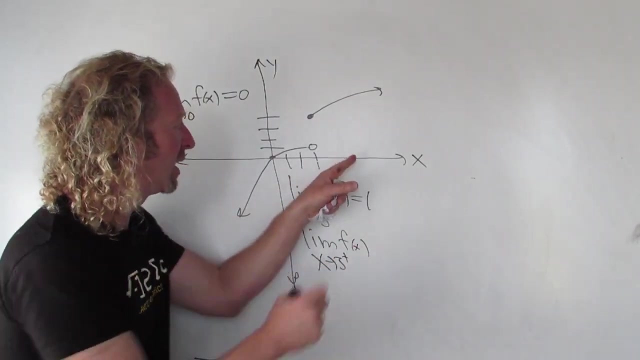 looks like the y value is 1.. But now let's approach 3 from the right, So we'll use the plus sign for that. So as x approaches 3 from the right, let's see what happens. So here's x. 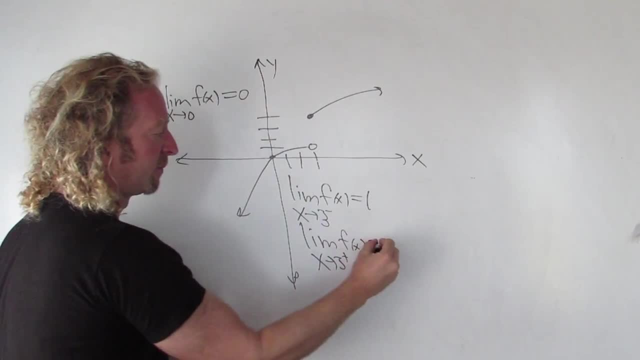 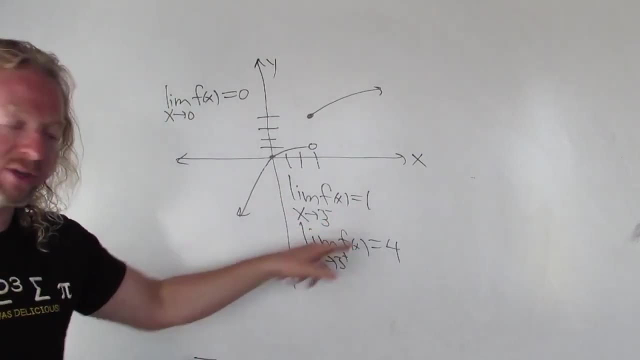 It's approaching 3.. So the y value gets close to 1,, 2,, 3,, 4.. So when you approach 3 from the left, the x value gets really really close to 3.. The y value gets close to 1.. So we say the limit. 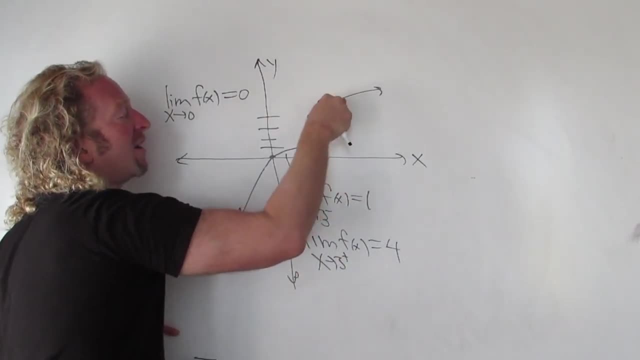 is 1.. As x approaches 3 from the right, the y value gets really, really, really, really, really close to 4.. So we say the limit is 4.. So what would that mean in terms of the limit? Well, 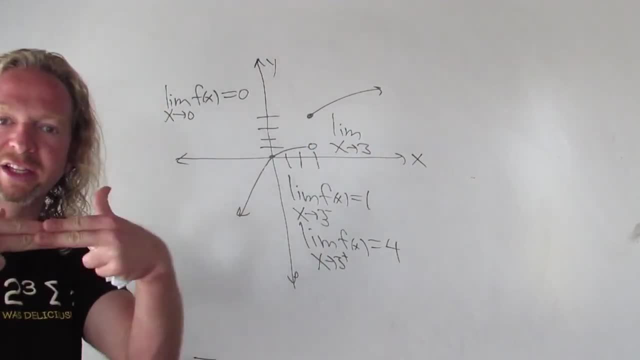 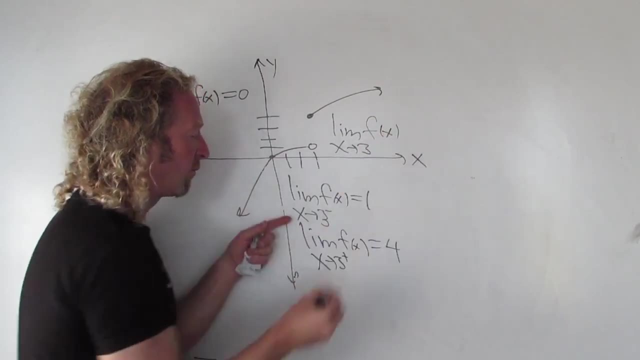 that means that the regular limit- you can think of this as a two-sided limit. These are called one-sided limits. The regular limit means from both directions. So as x approaches 3,, well, from the left we get 1.. From the right, we get 4.. Therefore, we get no answer when we approach. 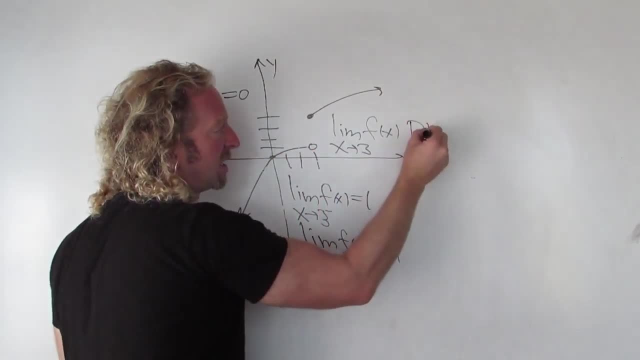 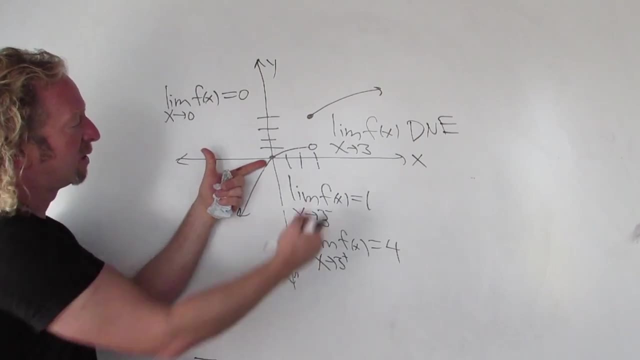 from both directions. So in this case you would say the limit d and e, And that means it does not exist In this example. here I didn't use one-sided limits. I just showed you: from the left you get 0.. From the right you get 0.. Therefore, the limit is 0.. If you wanted to write it, 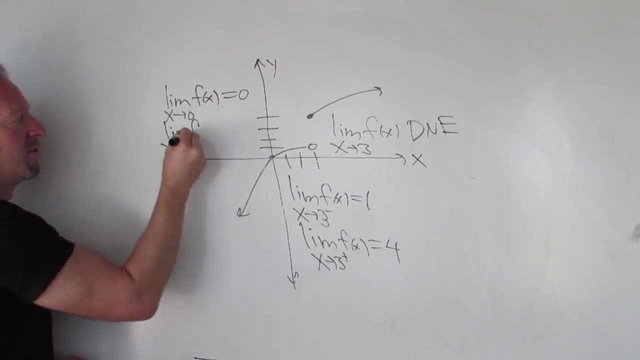 formally you'd write the limit as x approaches 0 from the left Or from the left. we know we get 0. Then you can do it from the right. So the limit as x approaches 0 from the right, Well, from the right we get 0. So whenever you get the same answer from the left and from the 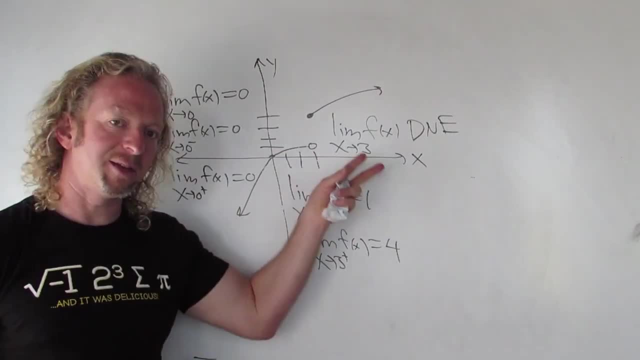 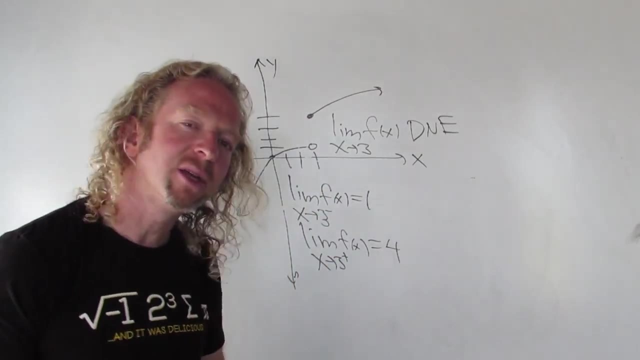 right, that's the value of the limit. If you get different values, then the limit does not exist. You'll notice there was a hole here. also, You might say: why is the value 1 if there's a hole? Well, when we're talking about limits, we only care about getting really, really, really, really. 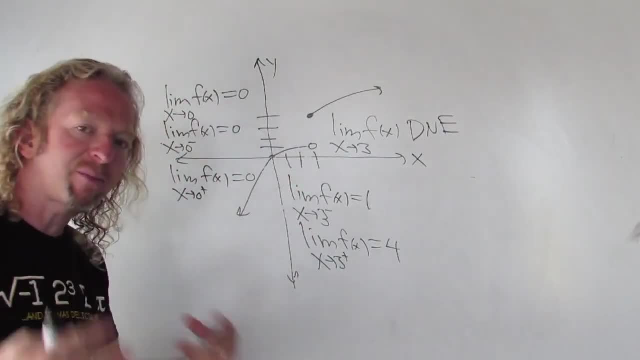 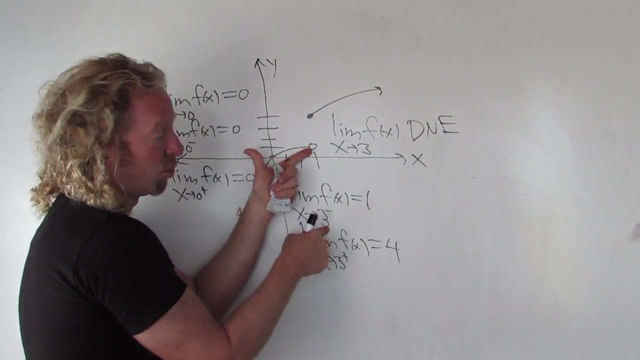 close to 3 from the left, We actually don't care what happens at 3.. We don't care. So when x gets close to 3 from the left, the y value gets really, really, really close to 1.. It never actually gets. 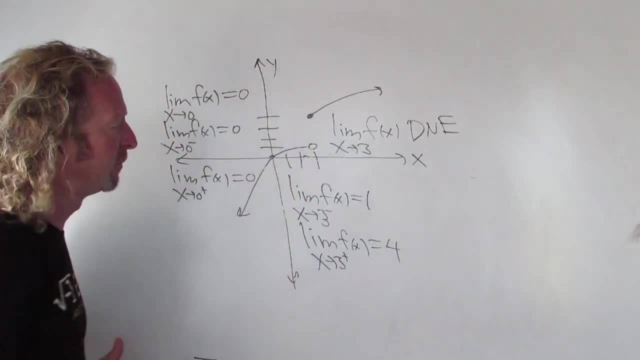 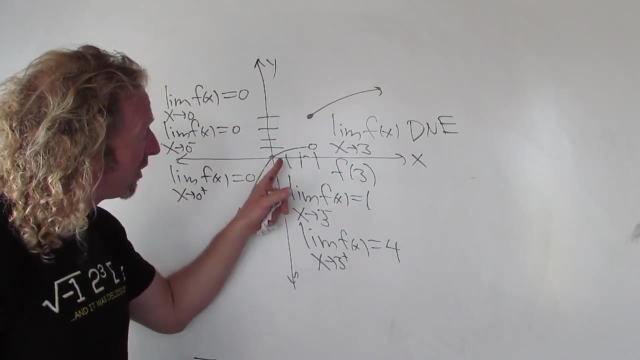 to 1.. It just gets really close. There's an open circle there. 1, right. If you were to say: evaluate f of 3, let's talk about that. What is the y value of 3?? Well, the y value of x equals 3, is 1, 2,, 3, 4.. So that would be 4.. So the y value of 3 is 4,. 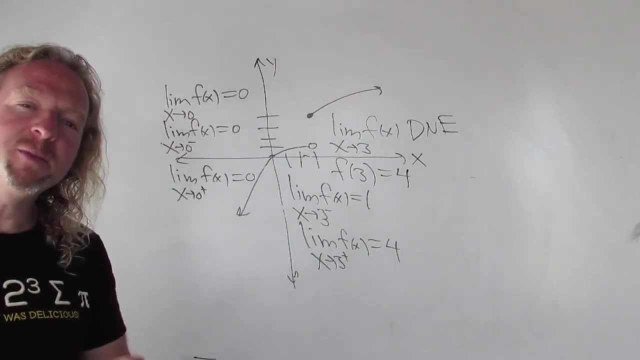 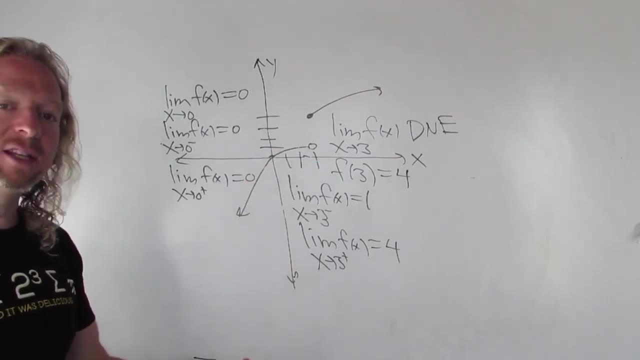 but the limit as you approach 3 from the left is 1.. And again why? It's because we only care about getting really, really, really, really close to 3, not actually being at 3.. So the main idea behind 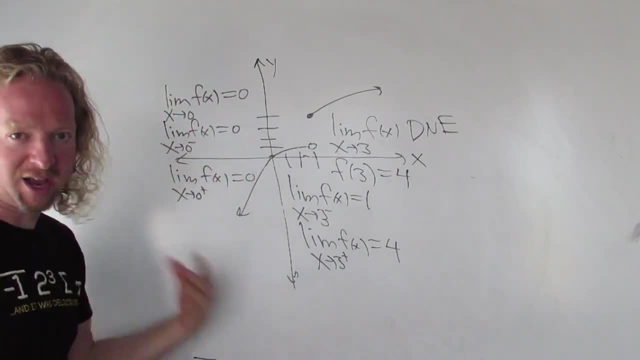 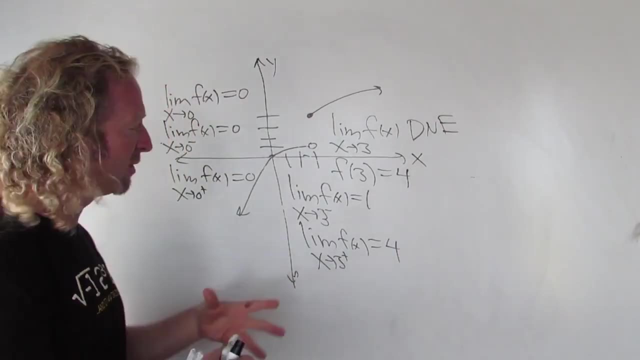 limits is what happens to the y value when x gets close to some x value. What are limits for? Limits are used to define derivatives. A derivative is a rate of change. It's studied later on in calculus. So limits are central and necessary for all of calculus, right for all of calculus, And that's. 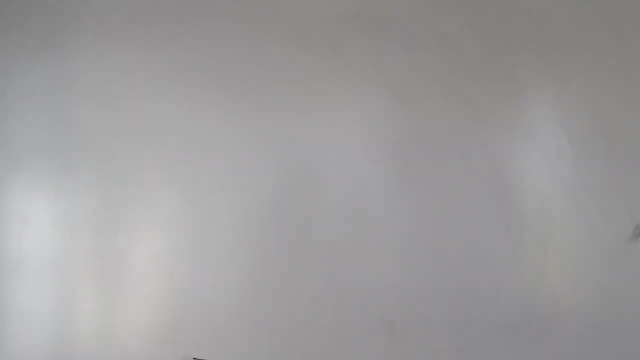 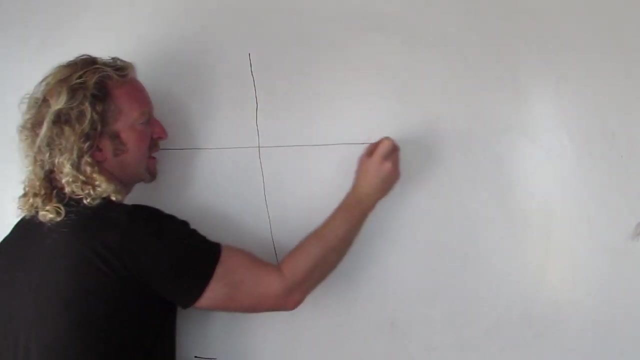 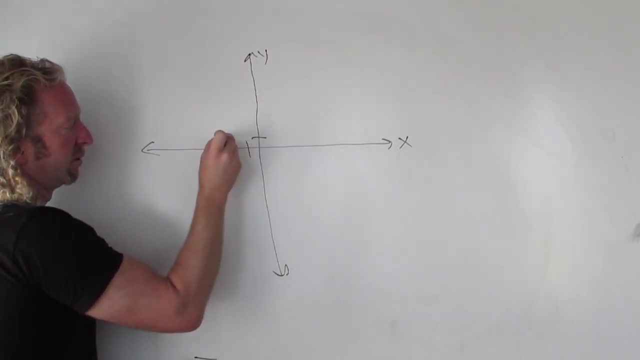 why we usually study them at the beginning of a course. Hey, YouTube, In this video we're going to compute some limits from a graph, So let's do it. So we have the y-axis, We have the x-axis, There's x, There's y, And let's do this. Let's take 1,, 2,, 1, put a little dot here. 1,, 2,, 3,. 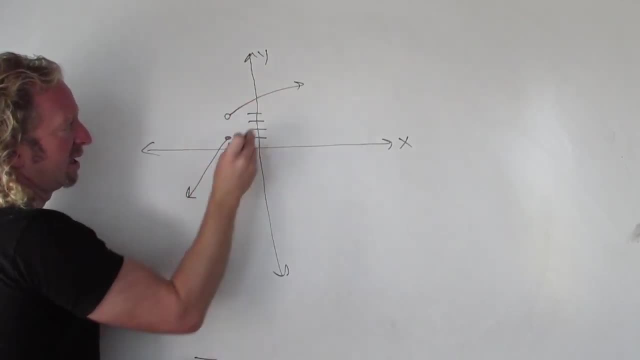 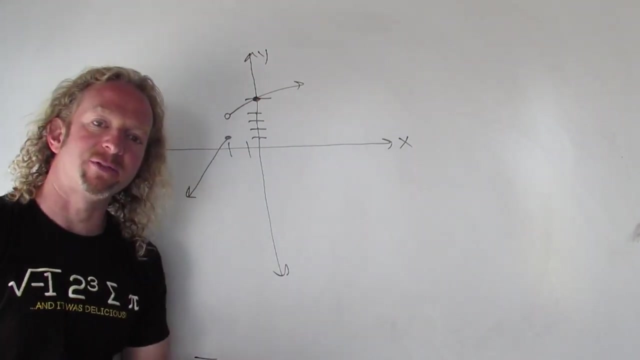 put a little hole here, Do this and this. And here let's put 1,, 2,, 3,, 4.. Let's do 5.. That's good, OK. now from this graph we can just compute some limits for practice. Let's start by finding the limit. 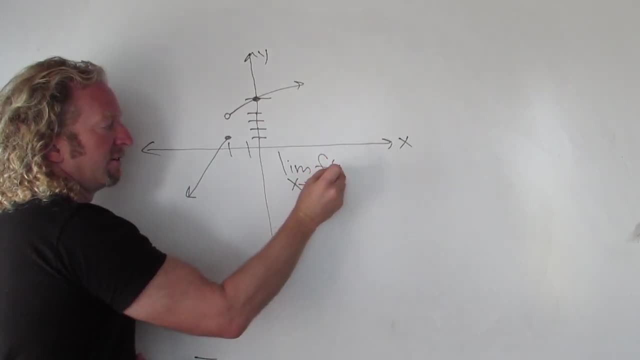 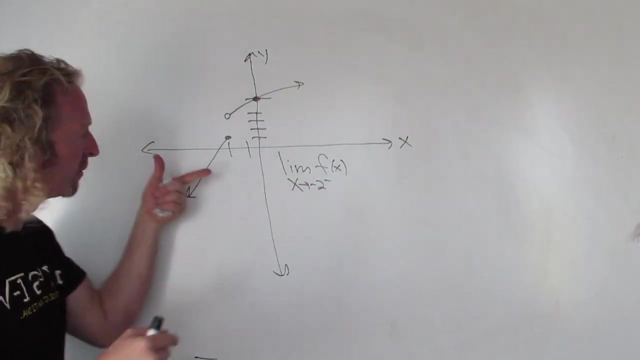 as x approaches negative 2 from the left of f of x. OK, so the question is, what happens to the y value when x gets really, really, really close to negative 2 from the left? So here is negative 2.. So x is getting close to negative 2, right. So the y value is getting really. 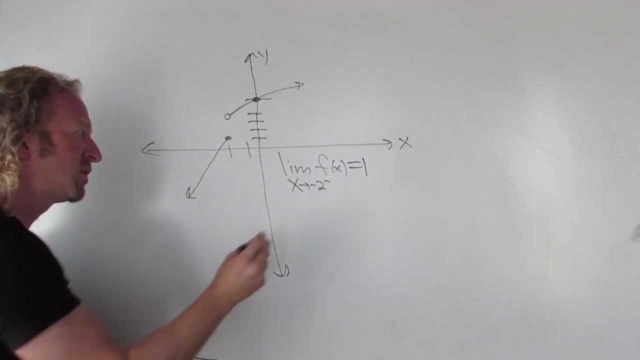 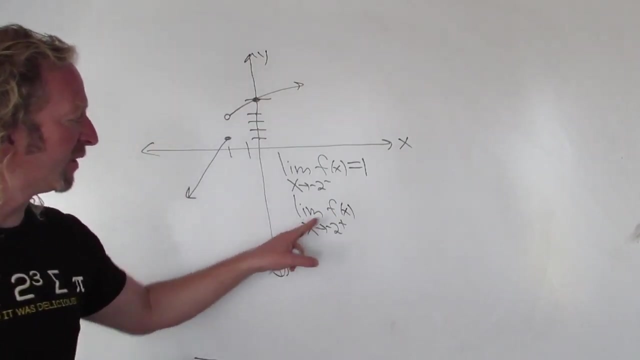 really close to 1.. So the answer is 1. Let's do the same thing. Let's approach negative 2 from the right. So this is the limit of f of x, as x approaches negative 2 from the right. So now we're approaching negative 2 from this direction. So as you approach from this direction, 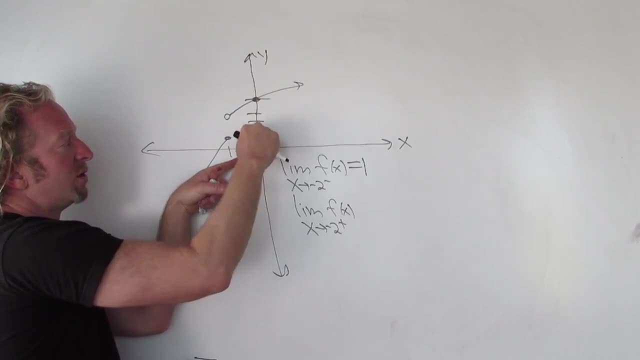 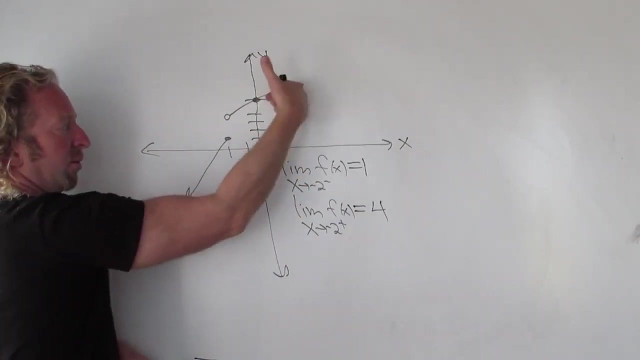 right, the y value gets really close to this little hole here. So 1,, 2,, 3,, 4.. So, boom, 4.. So from the left we get 1.. From the right we get 4.. Therefore the regular limit does not exist. 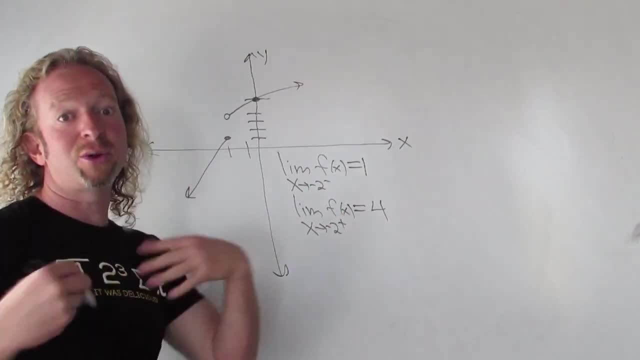 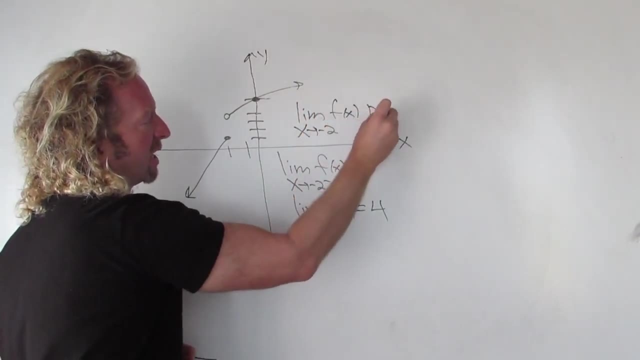 These numbers have to be the same. If they're the same, then that is also the value of the regular limit. Let's go ahead and write that down. So the limit as x approaches negative 2 of f of x does not exist. Remember, for a limit to exist it has to be equal to a number, first of all. 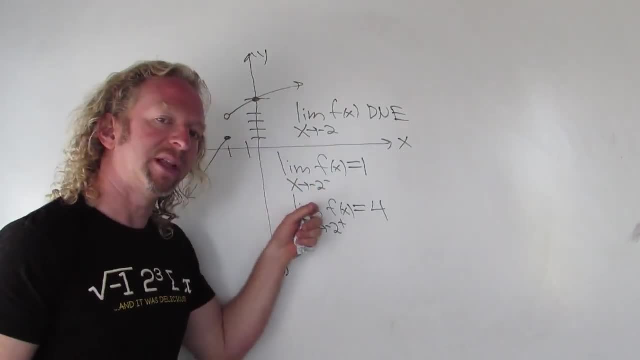 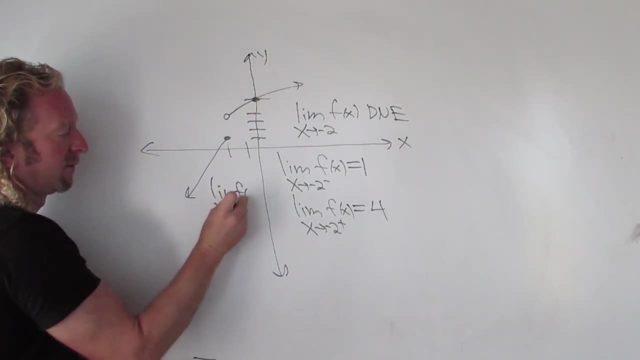 And it has to be the same number from both sides, right from the left and from the right. Let's see the limit as x approaches 0 from the left. So as x approaches 0 from the left, it looks like the y. 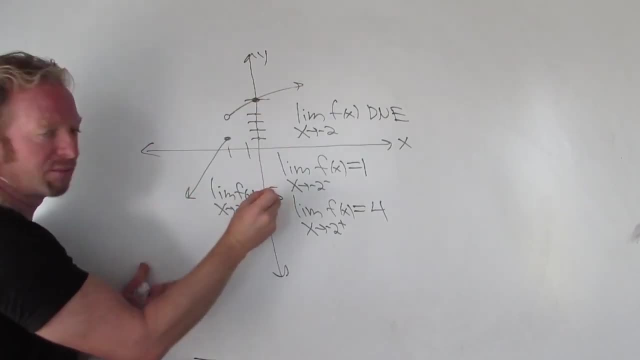 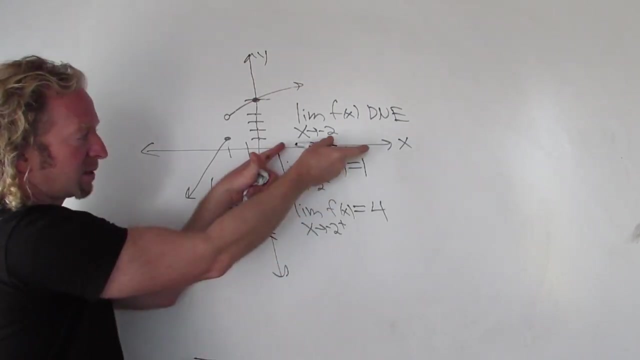 value is getting close to 1,, 2,, 3,, 4,, 5.. So the answer is 5.. Pretty simple. Let's approach from the right As x approaches 0 from the right, f of x So as x approaches 0 from the right. 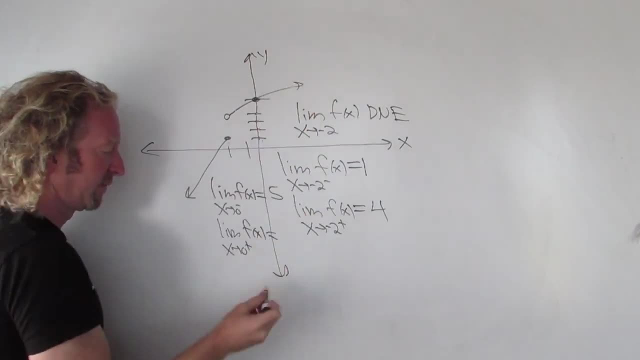 it looks like the y value is getting close to 1,, 2,, 3,, 4,, 5.. So 5.. So from the left you get 5.. From the right you get 5.. Therefore, the limit is 5.. So if you take the regular limit, 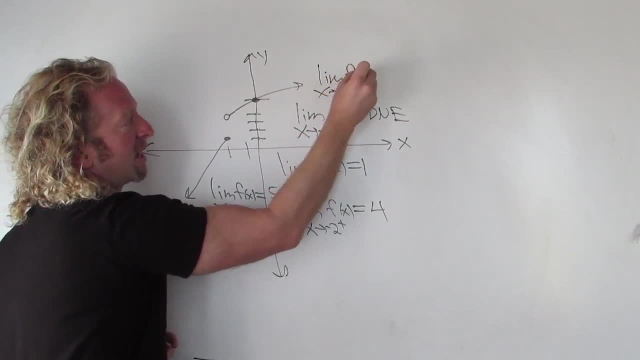 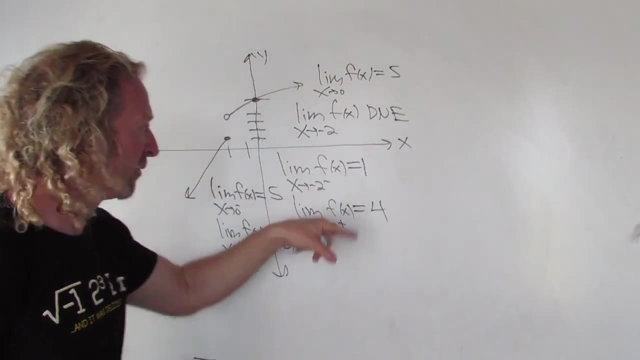 I'll write it up here, running out of room. as x approaches 0,, you get 5, right? so both one-sided limits have to be the same. therefore the limit is also the same. if they're different, then we say: 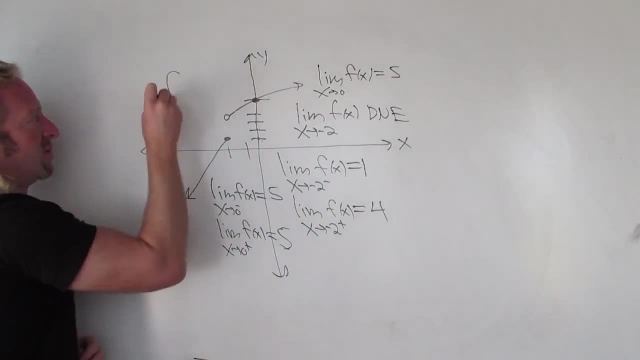 the limit does not exist. just for fun, let's compute some function values, just to make sure you got all this down. let's compute f of negative 2, so f of negative 2 is asking: what is the y value when x is negative 2,? well, when x is negative 2, the y value is 1, right, because there's a solid. 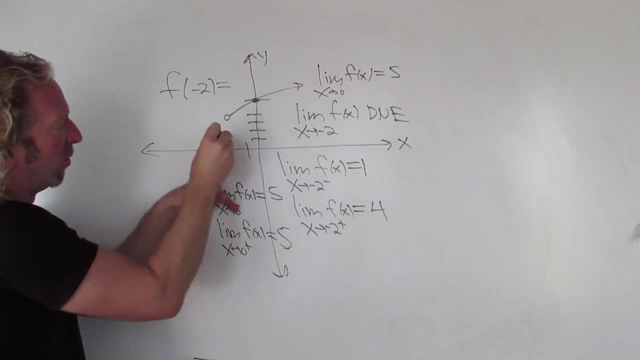 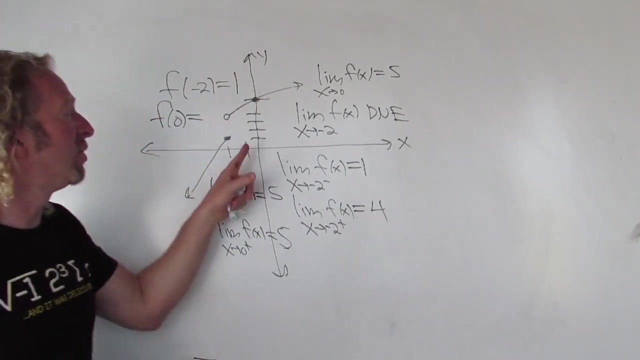 dot there the hole means you don't go there, right, no way. so avoid the hole. so right there. so 1, boom, let's find f of 0, this is asking: what is the y value when x is 0,? so 1,, 2,, 3,, 4,, 5, so 5,. 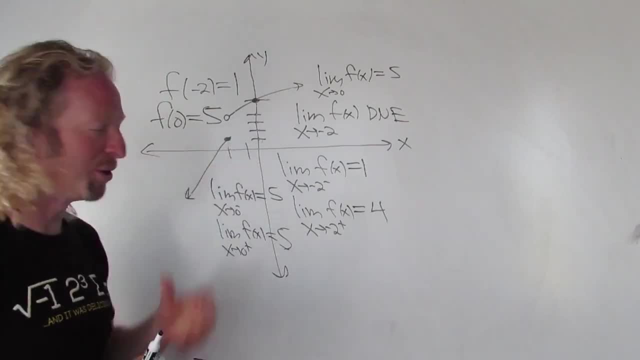 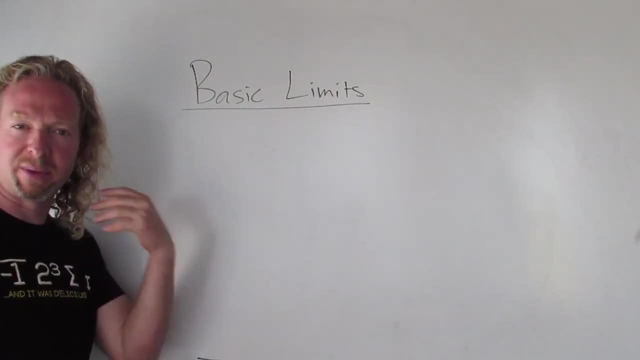 that's it. I hope this video has helped you with whatever you're working on. that's it. hey, everyone, in this video we're going to evaluate some really, really basic limits. so let's do an example. so let's take a limit. 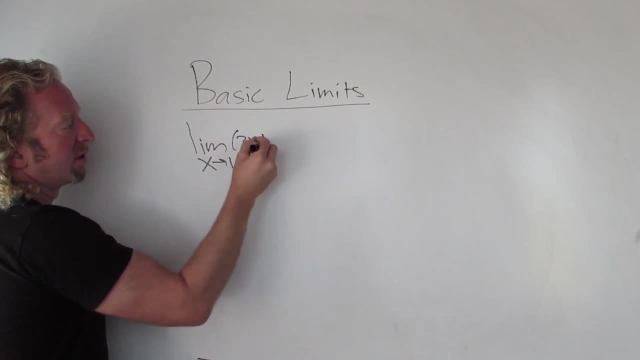 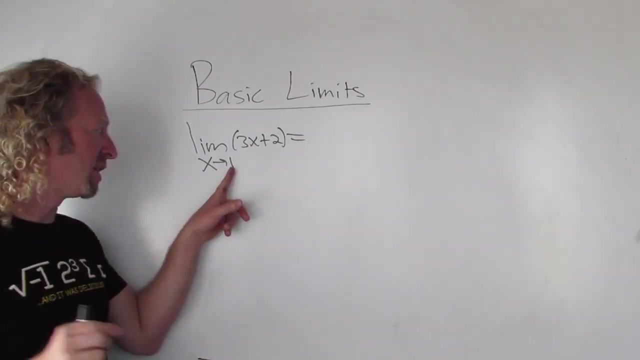 as x approaches 1, 3x plus 2, so we're trying to find this limit algebraically. so here's the number one rule: if you can take this number and you plug it in and you get an answer, like you. 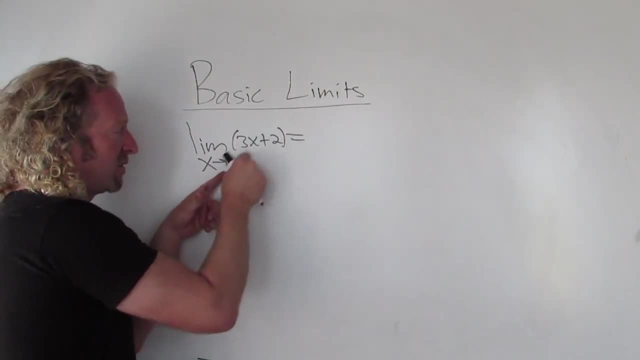 get a number, you're done. that's the answer. but if you try to do this and you try to plug it in and you don't get an answer, then you have to do something else. what else do you do? well? 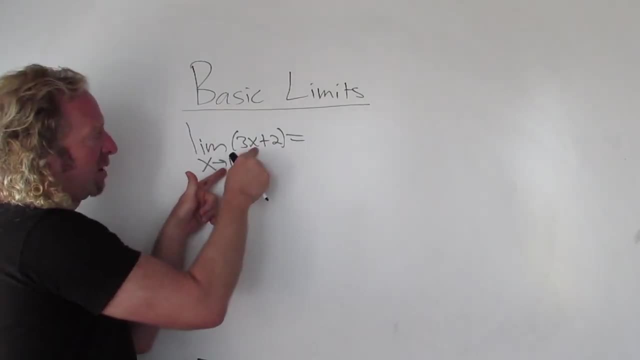 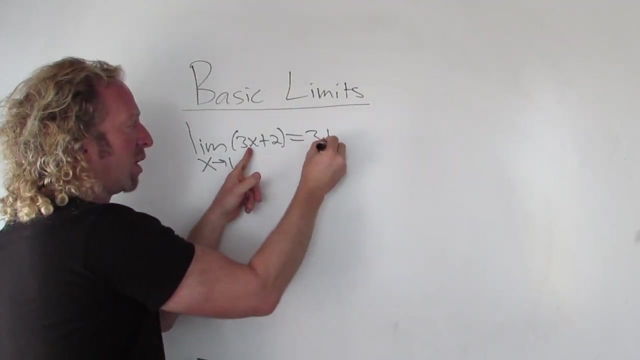 that's calculus right, so let's try it. so can we plug the number in? yes, we can right, because you would get 3 plus 2, which is 5, so then you just do it, so you get 3 times 1 plus 2, the answer is 5,. 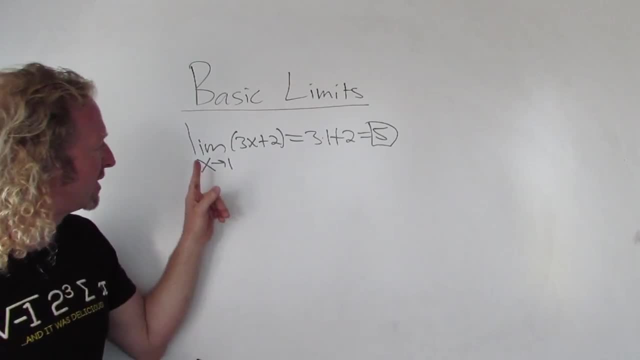 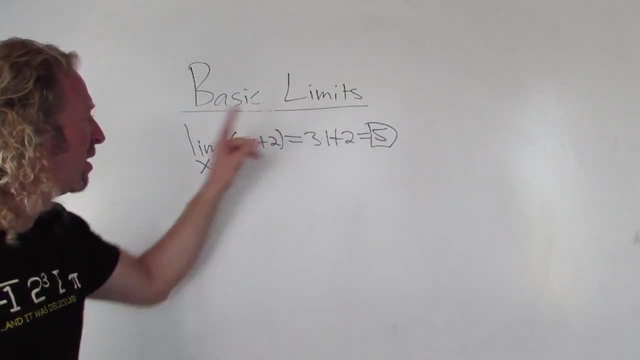 so the answer to this question is 5,. right, so the limit as x approaches 1, of 3x plus 2 is equal to 5, that means that this function gets really, really, really really close to 5, when x gets. 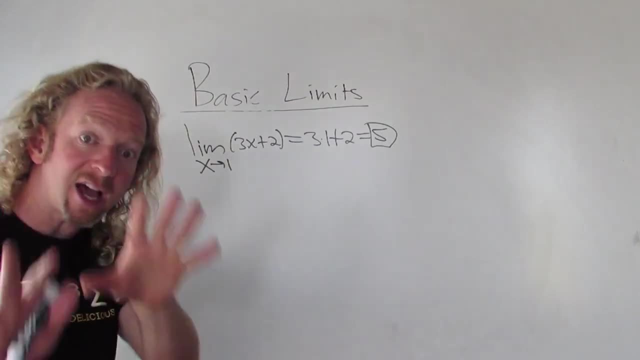 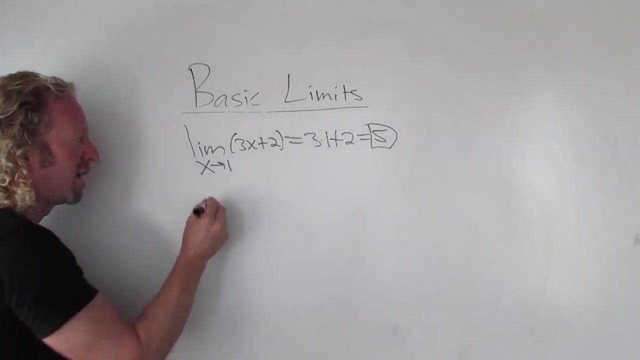 really, really, really, really close to 1,. so can you always do this? yes, absolutely right, you can always do this as long as you get an answer, like if you get like division by 0, game over, for example. 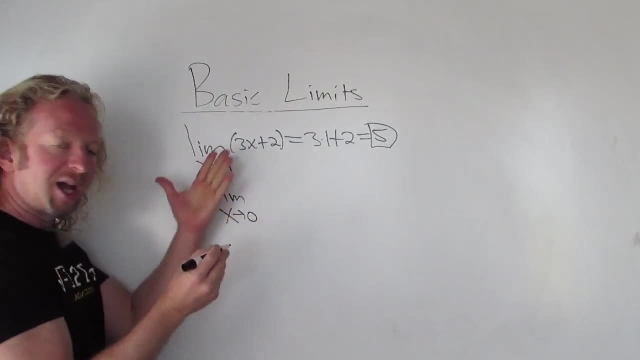 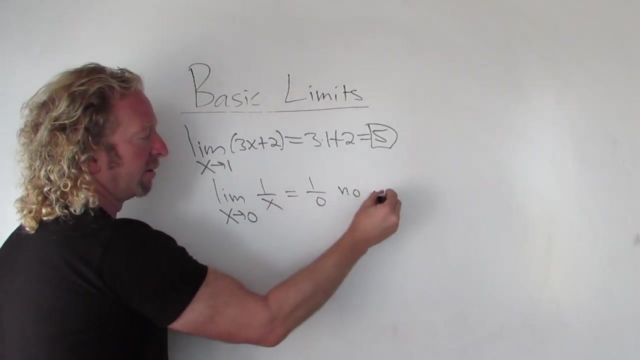 say you try to do it in this example here: limit as x approaches 0, of 1 over x. in this case, when you plug in 0, you would get 1 over 0, so no good right fail, huge fail. 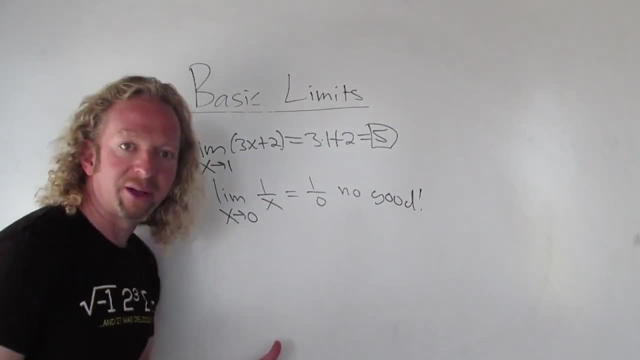 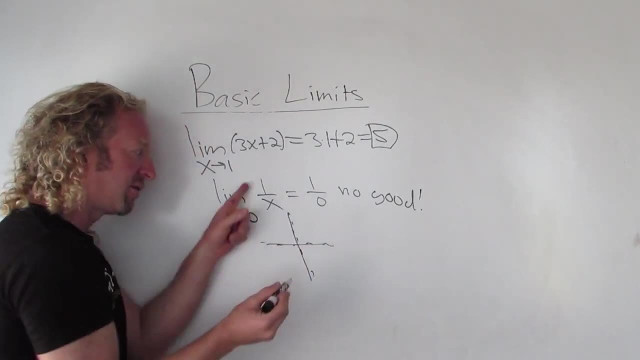 right, terrible right. so what do you do? well, you do something else right. later on we'll learn how to evaluate limits like this. I'll show you how to do it. you can do it graphically. if you graph this function, 1 over x, it looks like this: as you approach 0 from the left, 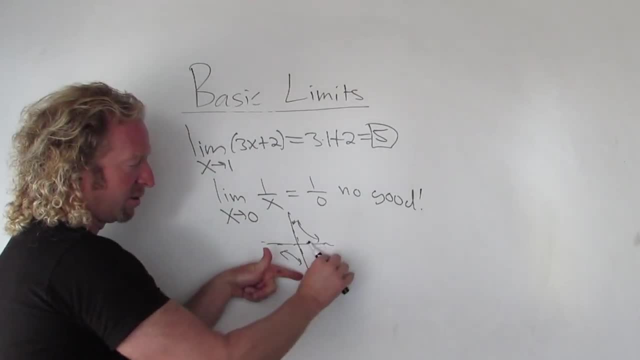 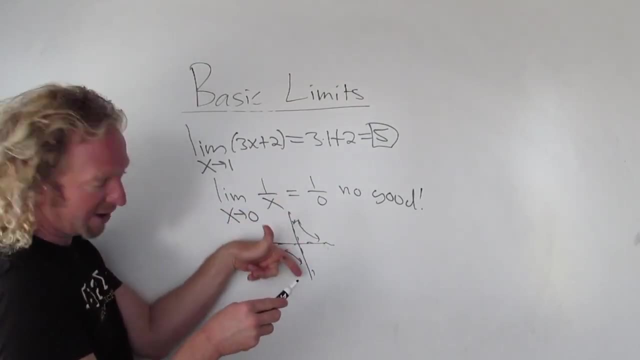 you get negative infinity. as you approach 0 from the right, it goes off to infinity. therefore, you get different values, so the limit does not exist again. as you approach 0 from the left, it goes down forever. so you get negative infinity. as you approach 0 from the right, it goes up forever. so you get. 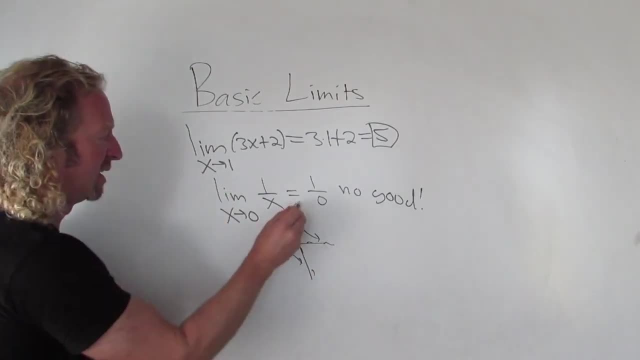 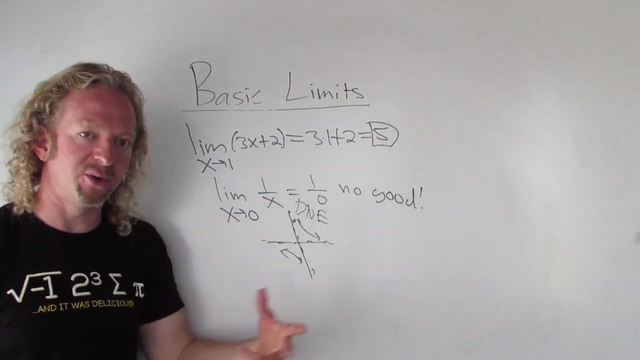 infinity. infinity is not equal to negative infinity, so this limit is dnE. there's not really a nice algebraic way to do this limit, so the moral is, if you can plug in the number and you get an answer, you do it. if you don't get an answer, then you try something else. 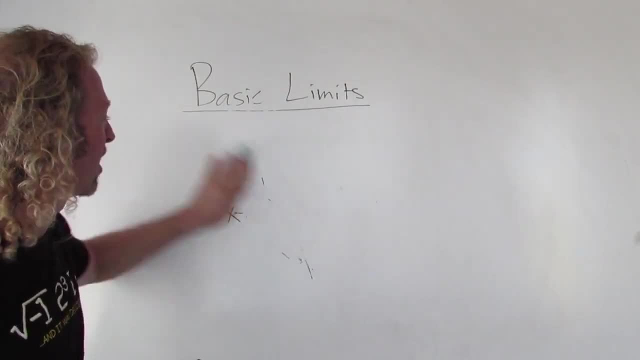 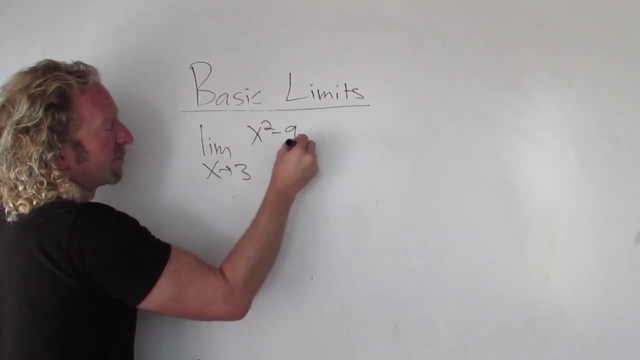 let's do another example, just so you see what I mean. let's try this one. take the limit as x approaches 3 of x squared minus 9 over x minus 3, so in this case, here, if you plug in 3, you would get 0 over 0, right. 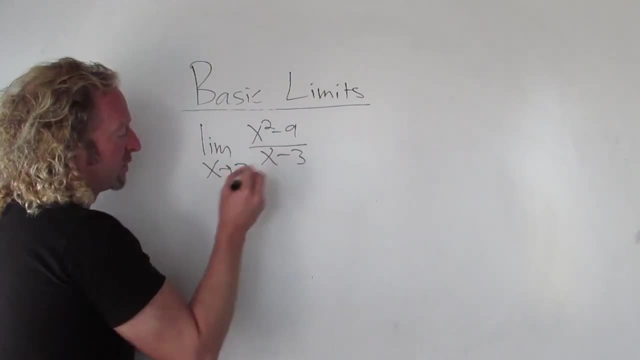 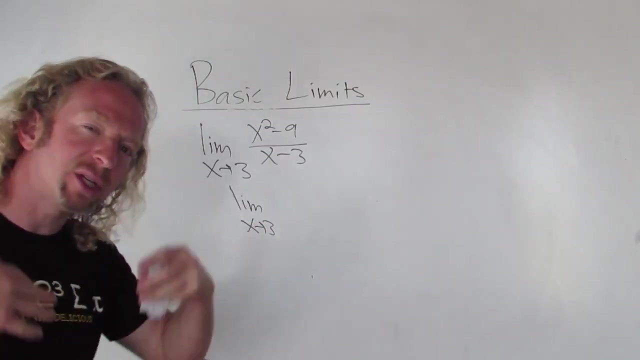 so that's no good right. so what do you do? well, it looks like you can factor right. so at the limit sign. again. now it's really important to always write the limit sign until you actually take the limit. okay, by taking the limit I mean like using a formula. 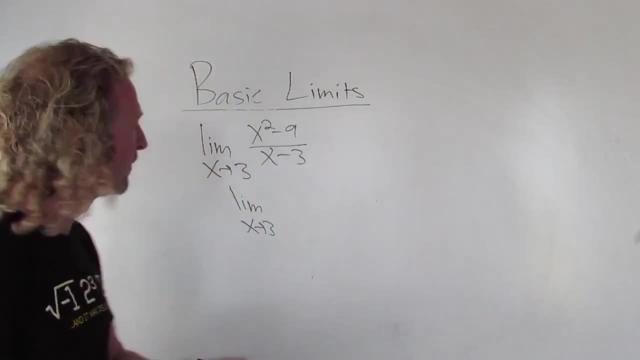 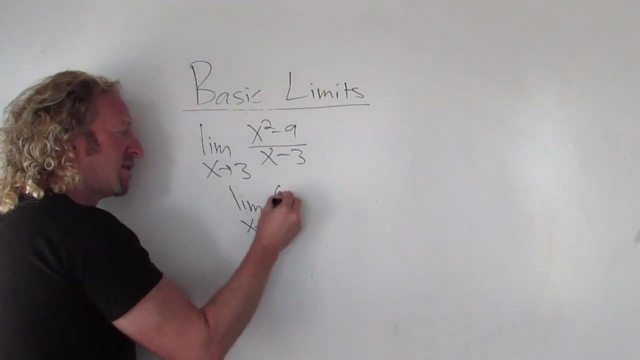 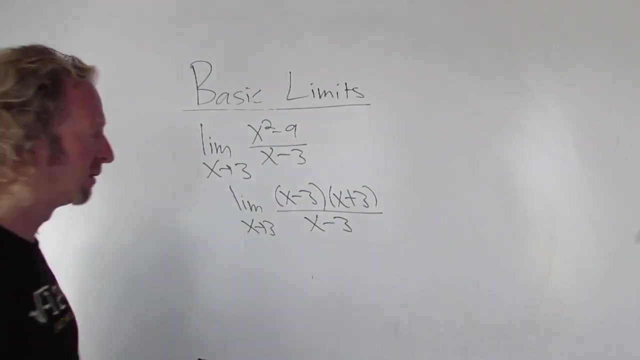 plugging in a number or using you know some technique that gives you the result. in this case, we're not plugging in the number, yet we're going to factor this right. this is the difference of squares, so it'll be x minus 3, x plus 3, all over, x minus 3,. okay, now you just cancel, we're. 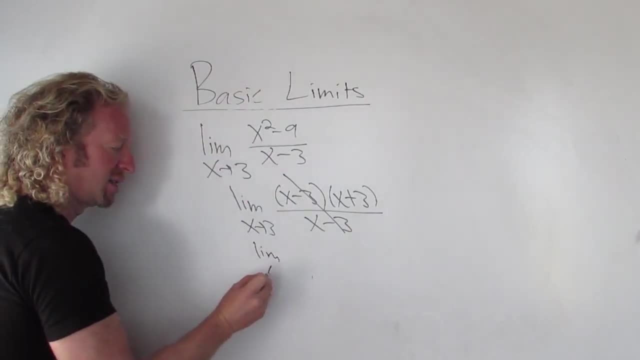 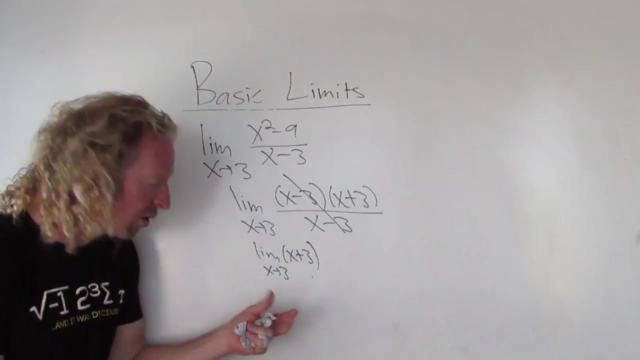 not going to plug in the number yet, so I'll rewrite it one more time. this is the limit as x approaches 3 of x plus 3, so you always write the limit sign right, no matter what, until you take the limit. whatever that may be right, in this case taking the limit is plugging. 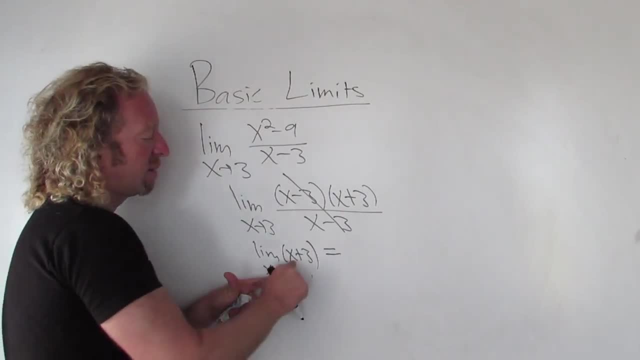 in the number. so we're going to take this 3 and put it there. when you plug in the number, that's when you stop writing the limit sign super important, right? so 3 plus 3, which is 6,. 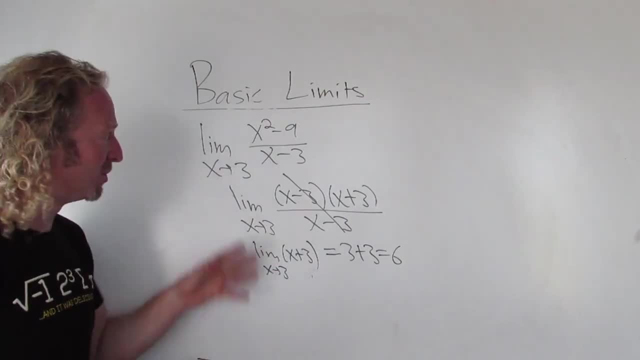 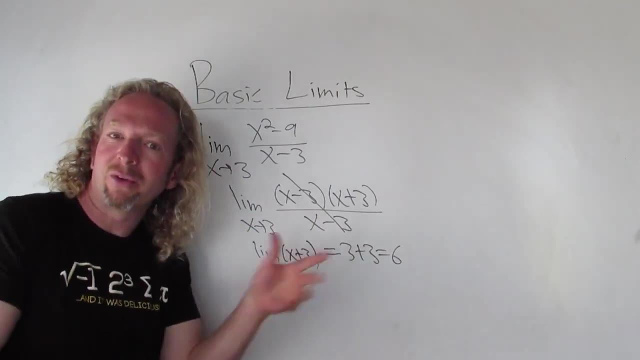 one of the most common pitfalls. one word to use in calculus is: people will drop the limit sign or they'll put it where it's not necessary, like if you put the limit sign here, that would be wrong. you've already taken the limit. so a lot of it is about structure in calculus. 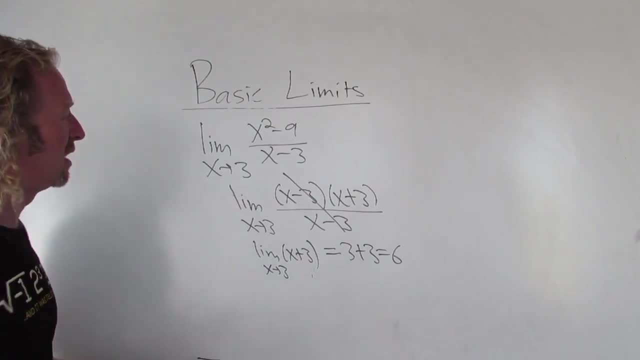 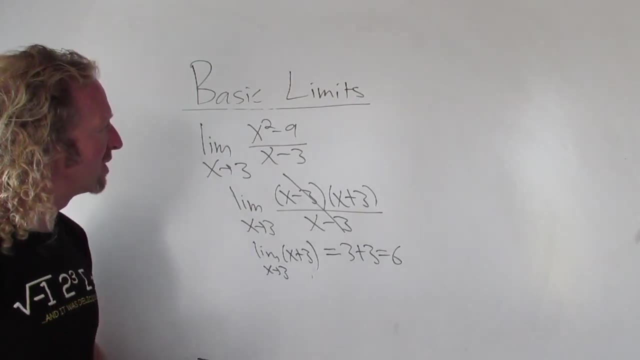 and in all of mathematics. so again, the main rule in limits is: if you can plug in the number and you get an answer, do it. if you can't do something else, and what is that something else? well, that's the rest of the course. so hope this video made sense in the videos that follow. 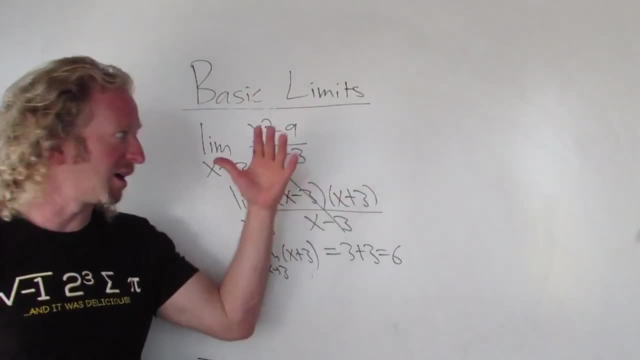 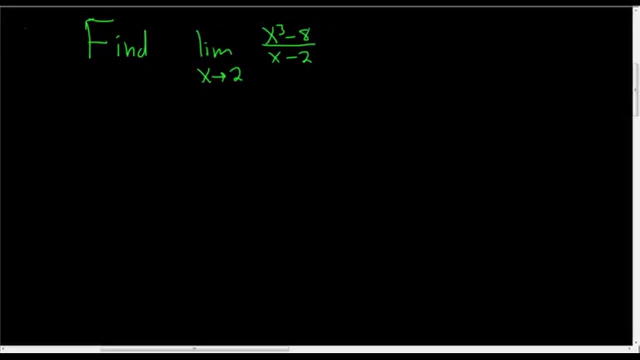 you'll see more examples of limits. thanks for visiting my YouTube channel. that's it. In this problem, we're being asked to find the limit, as x approaches 2, of x cubed minus 8 over x minus 2.. So the problem is we're going to have to find the limit, as x approaches 2, of x cubed minus 8 over x. 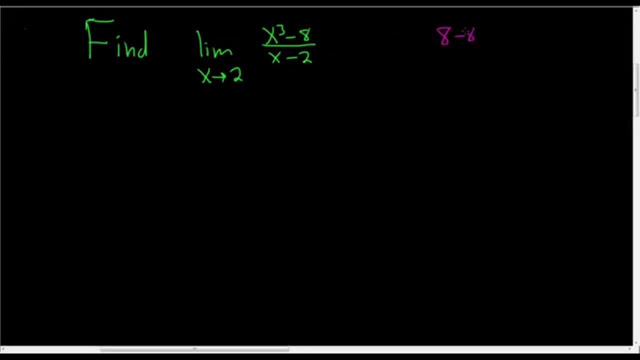 minus 2.. So the problem is, if we plug in 2 right away, we end up with 8 over 8, 8 minus 8,, rather over 2 minus 2, which is 0 over 0, and that's undefined. 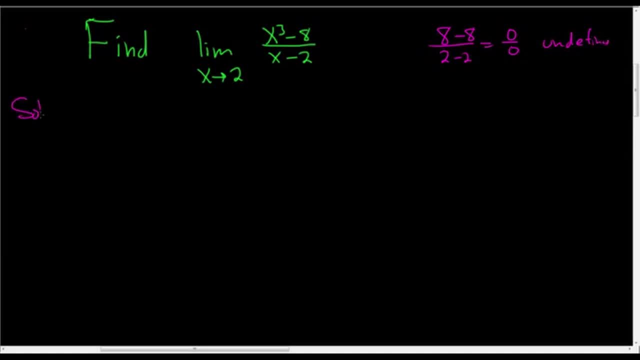 So the trick is to recall a formula from algebra. If you have a cubed minus b cubed, and the way I memorize this formula is: it's a and then you keep the sign so minus b, and then you have a squared and then you switch the sign. so we have a minus, so we put a plus. 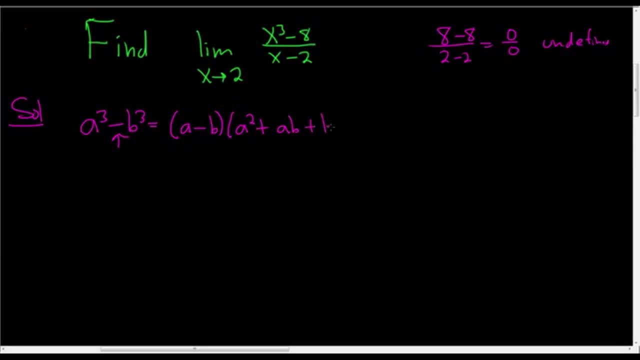 and then it's a, b and it's always plus here, no matter what. so b squared. So in this case we can rewrite our limit as follows: This is the limit as x approaches 2,. well, let's see x cubed minus 8.. 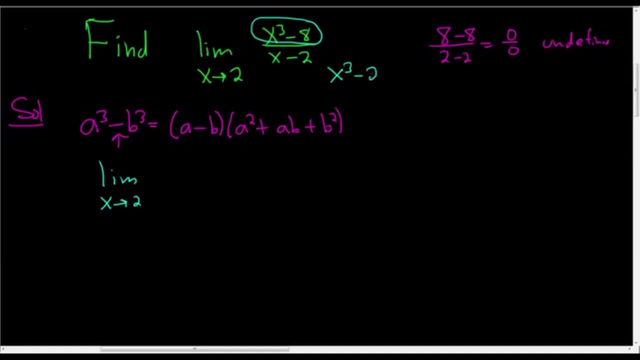 So in this case it's x cubed minus 2 cubed. So a is x and b is 2, so it's going to be x minus 2, and then parentheses, and then x squared plus and then a- b. so in this case it's simply 2x. boom, there it is. 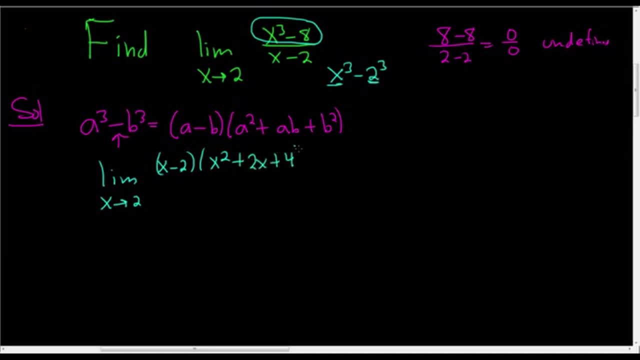 and then plus b squared, which is 4, beautiful stuff all divided by x minus 2.. And so you see now that these guys cancel, and so we end up with the limit as x approaches, 2 of the quantity x squared plus 2x plus 4.. 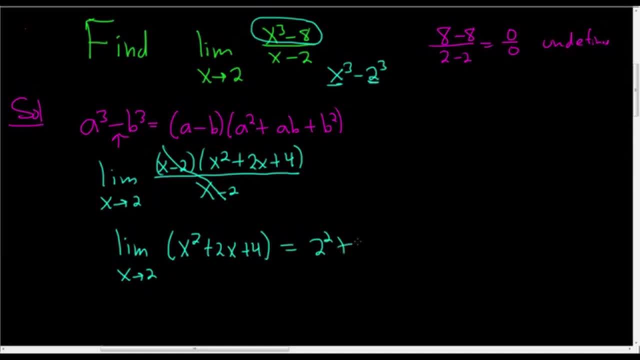 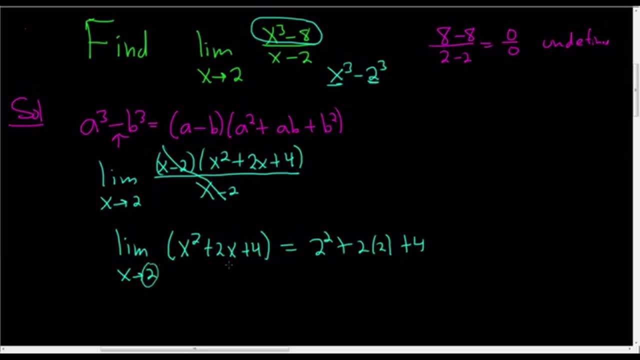 Remember when you're taking limits, if you can plug in the number and it makes sense, go for it. And this is 4 plus 4 plus 4, which is 12.. And that is the limit as x approaches 2 of the quantity x cubed minus 8, all divided by x minus 2.. 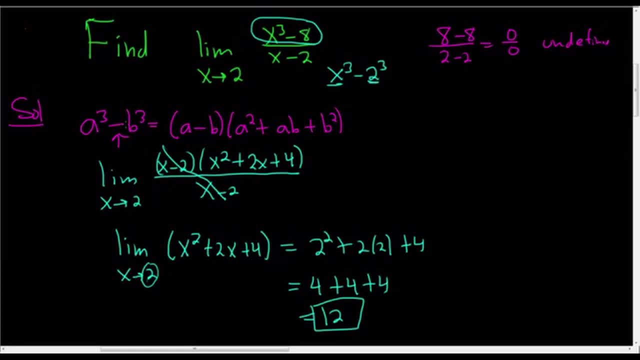 Super easy. Problems like this aren't about being smart or being witty. It's all about recognizing that there is a limit, that you have the difference of cubes, and just knowing this formula. If you know this formula, you can do this problem every single time. So I hope that. 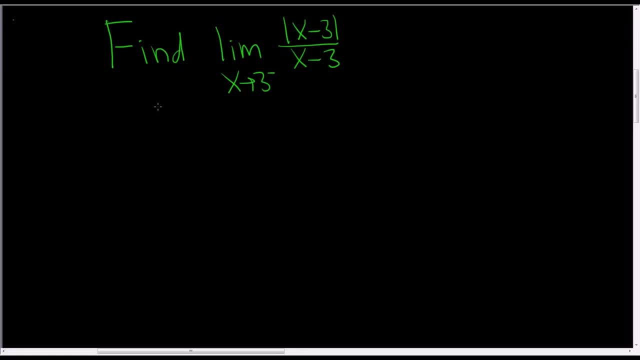 helps. So we have to find the limit, as X approaches 3 from the left, of the absolute value of X minus 3 over X minus 3.. So solution: So before we start the problem, it's important to remember the definition of absolute value, So the. 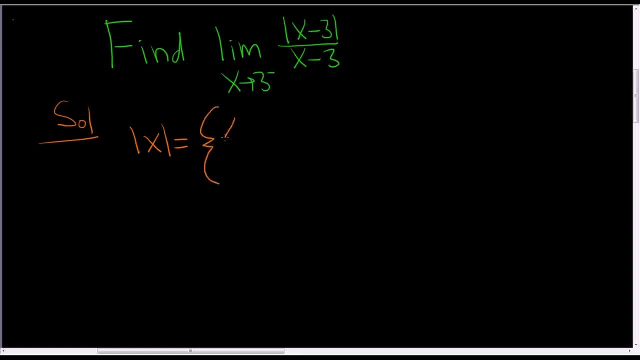 absolute value of X. it is, in fact, a piecewise function. It's equal to X if X is greater than or equal to 0, and it's equal to the opposite of X if X is less than 0.. So, in our case, all we have to do is think about what's going on and we 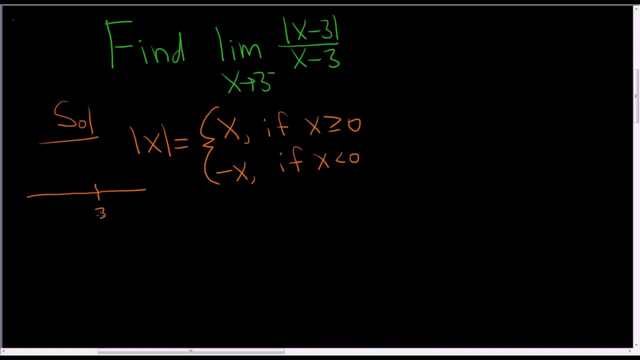 should be able to figure it out. So here's 3.. The negative sign here- a little minus, not really a negative sign- indicates that we're approaching from the left. That means that X must be less than 3. So X minus 3 must be less than 0. That. 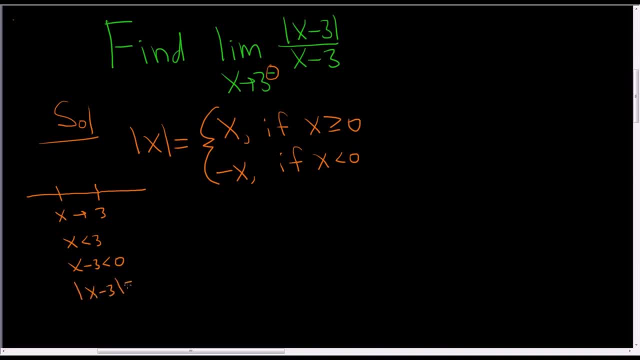 means the absolute value of X minus 3,. well, according to the definition, since X minus 3 is less than 0, we use this piece. So then we end up with minus X minus 3.. So now we have a formula for the absolute value of X minus 3 that we can. 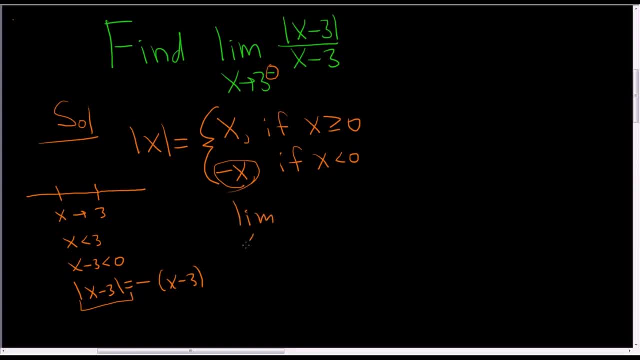 use in our problem. So finally, the limit as X approaches 3 from the left. now we're going to replace this with this, So this becomes negative X minus 3, all over X minus 3.. These cancel. you get the limit as X approaches 3 from the left. 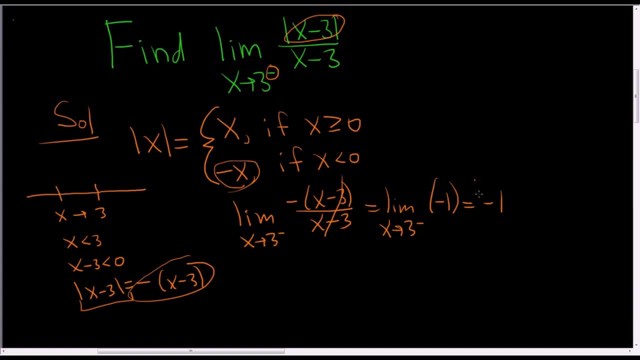 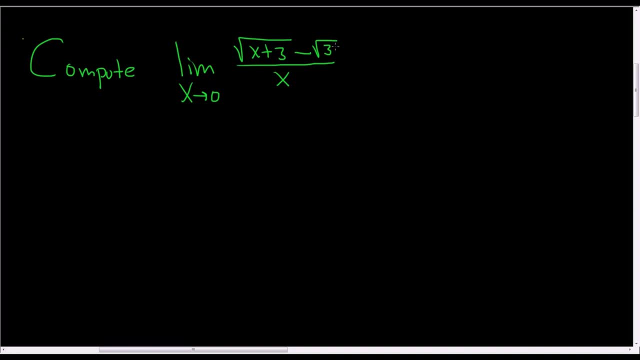 of negative 1, and that's just negative 1, and that's the answer. So we're being asked to compute the limit as X approaches 0 of this quantity here. So the first thing you should do whenever you have a limit is: take the number and 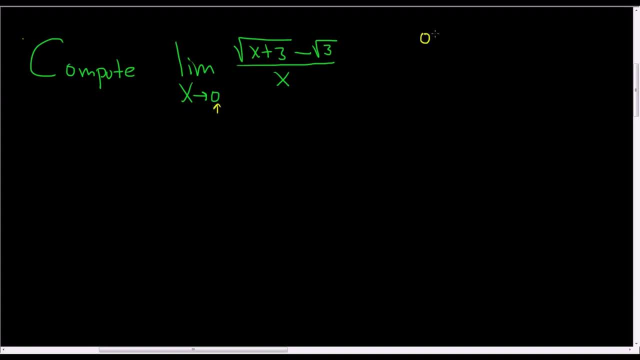 plug it in and see what happens. so if we do that, we get 0 plus 3, we have a square root minus the square root of 3, over 0. So that's 0 over 0 and that's undefined. so that's no good. So we have to take a different approach. so the 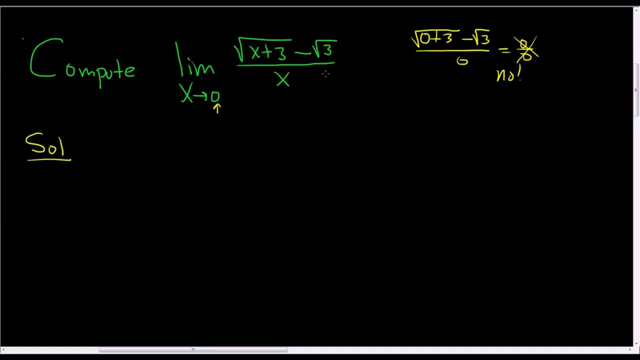 approach that kind of jumps out at you after you do a couple of these is to rationalize the numerator Whenever you have like a square root minus something else. rationalizing the numerator is usually a good first bet, so let's go ahead and rewrite the whole thing one more time, so x plus 3 minus the square root of 3, and then here we have x. 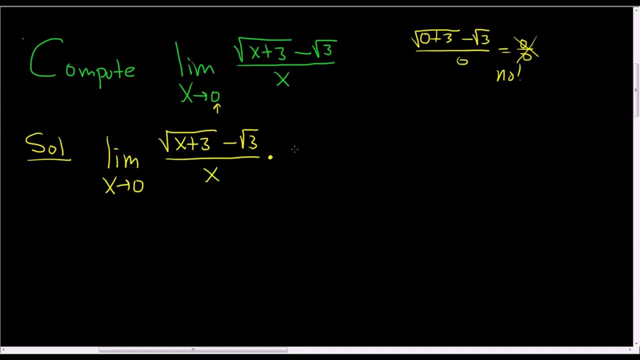 okay. so to rationalize the numerator, we'll multiply by the so-called conjugate. so we multiply by the square root of x plus 3 plus the square root of 3, and then we divide by the exact same thing. so square root x plus 3 plus the square root of 3, and this is really equal. 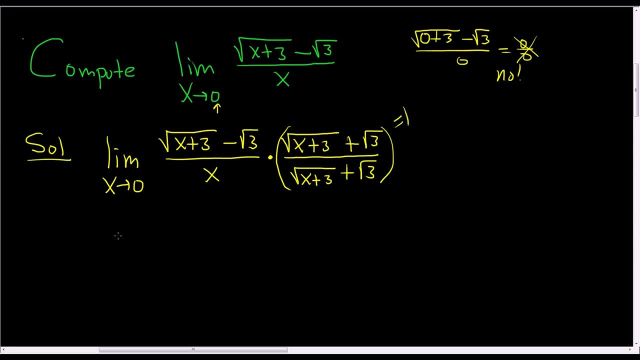 to 1, right, so everything here is good. we're not doing anything bad. so this is the limit as x approaches 0. and now we're going to use a formula from the past, right? so if you have a minus b times a plus b, this is the difference of squares formula. this is a squared minus b squared, so in 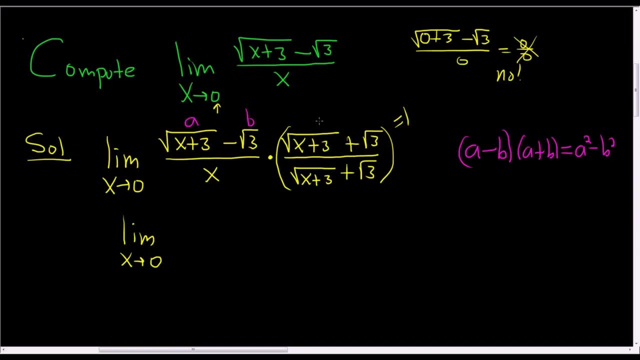 this problem: this here is our a and this is our b. this is our a, this is our b. so it's just going to be a squared, so we square this guy. so we just get x plus 3 minus, and then we square the b so we just get 3, and in the 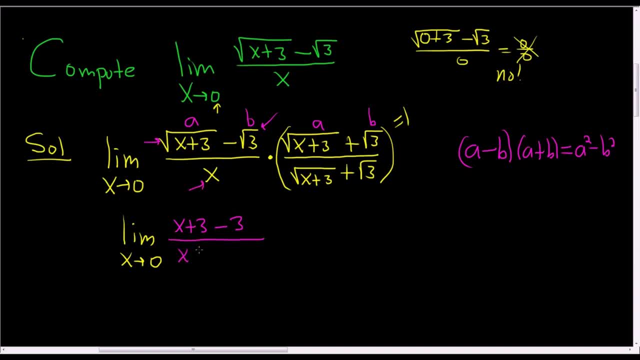 denominator, we still have our x, and then it's really easy to forget this piece as well. this is being multiplied by the denominator, so we have parentheses- square root x plus 3 plus the square root of 3. let's see what happens here. the 3 is cancelled, so we have the limit. 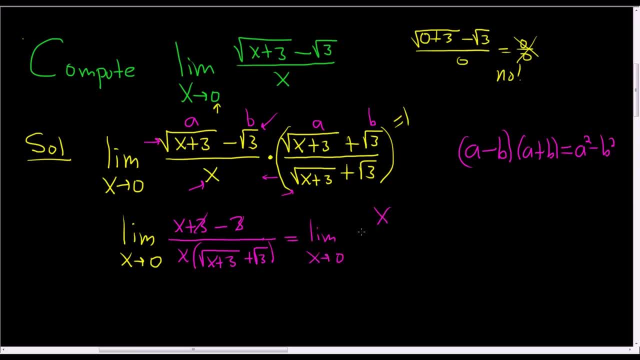 as x approaches 0 of x divided by x, and then parentheses, square root x plus 3 plus the square root of 3. now the x is cancelled. let's go ahead and write it one more time. so limit x approaches 0 and we have 1 over the square root of x plus 3 plus the square root of 3. 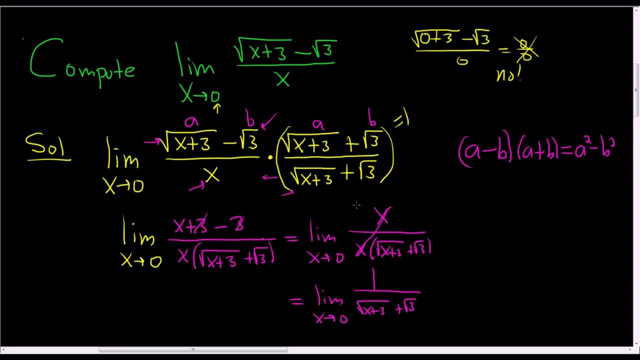 And at this point we can finally plug in 0, right? We tried to do that at the beginning of the problem and it didn't work, So now we can do it. So now we stop writing the limit sign. So it's 1 over. 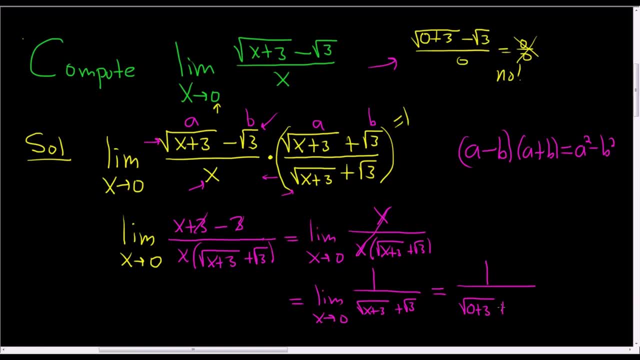 We're taking the limit right. So 0 plus 3 plus the square root of 3.. That's simply 1 over the square root of 3 plus the square root of 3.. And we have two of them. So this is 1 over 2 square root of 3.. 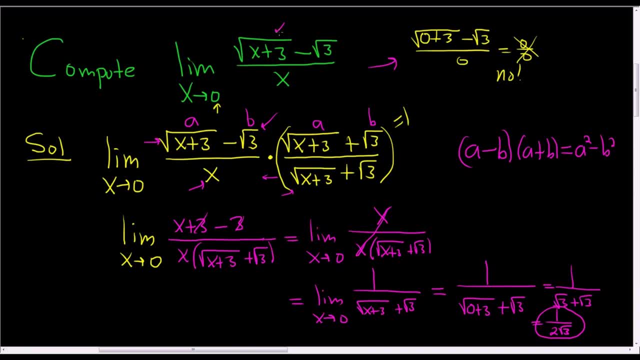 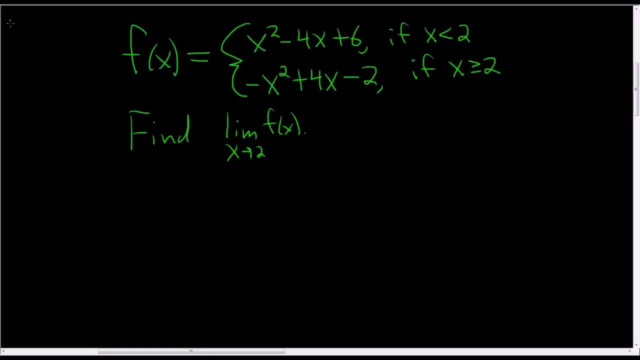 So how do you know to do this? Well, whenever you have, like, a square root minus another square root or something that remotely looks like this, it's a good attempt, a good thing to try, That's it. All right, we have to find the limit of this piecewise function. 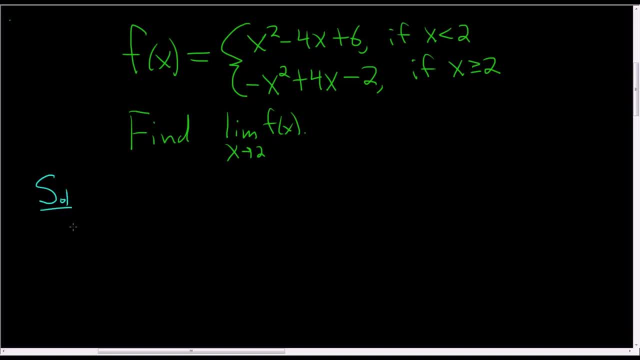 So let's work it out. Solution. So it's a piecewise function and it looks like: for x less than 2, we're using this function And for x greater than or equal to 2, f of x is actually this function. 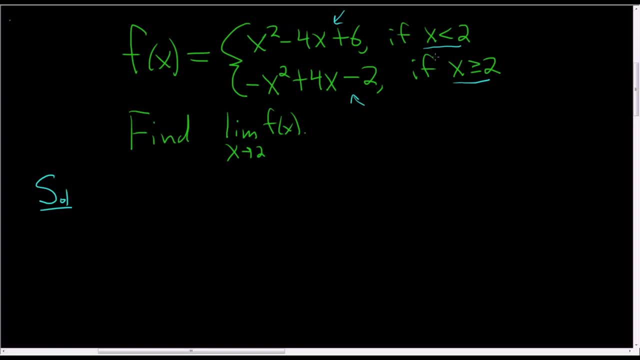 So what we'll do is we'll take one-sided limits as x approaches 2.. That way we can actually compute the limit. So let's look at the limit. Let's look at the limit as x approaches 2 from the left. Let's think here: 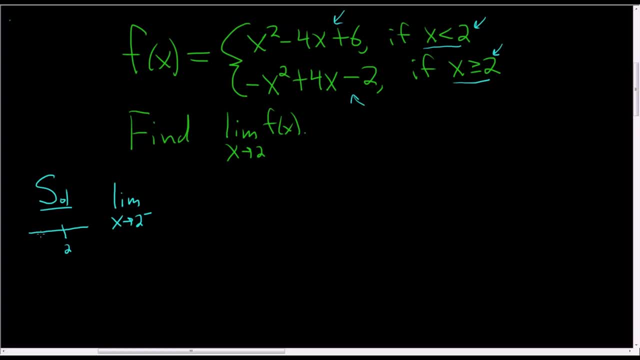 So here's a little picture. Here's 2.. We're approaching 2 from the left. So here's x Right, we're approaching from the left. That means x is less than 2.. That means we're going to use the first piece right here. 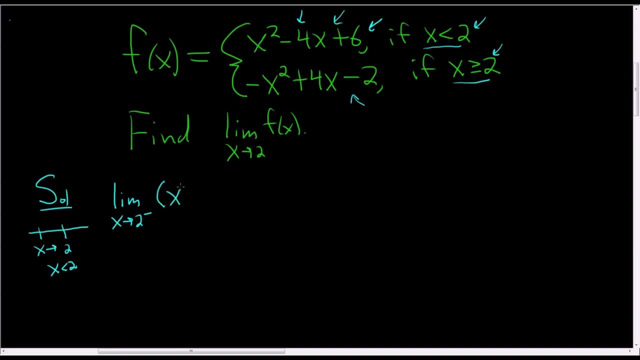 So in this case f of x is x squared minus 4x plus 6.. This is a polynomial, so we can just plug in 2. So we get 2 squared Minus 4 times 2, plus 6.. 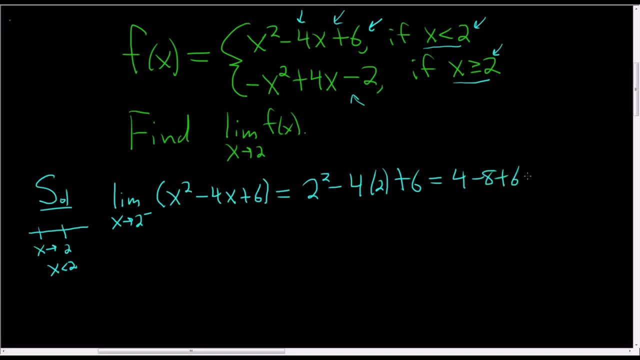 So this is 4 minus 8, plus 6.. Here's where it gets tricky: Negative 4, and then this is a 6, so we just get 2.. Right, so now we have to compute the limit from the right. 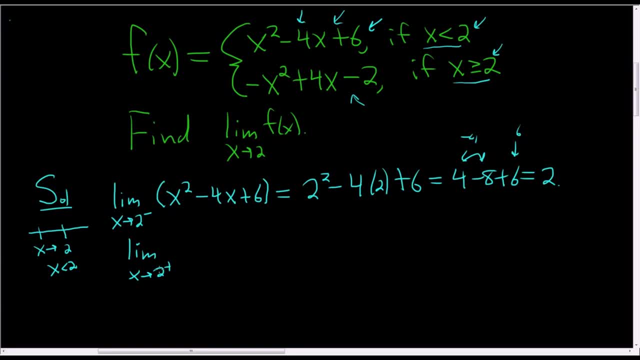 So, as x approaches 2 from the right, Now if x is approaching 2 from the right, x is bigger than 2.. So here we have negative x squared plus 4x minus 2.. Right, We're using this piece here, right. 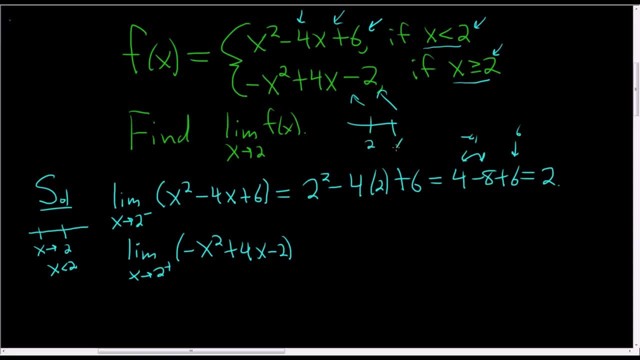 Because here's 2.. We're approaching 2 from the right, So x is bigger than 2.. Right, x is bigger than 2.. That tells us to use this piece here. All right, at this point we can just plug in the 2 again. 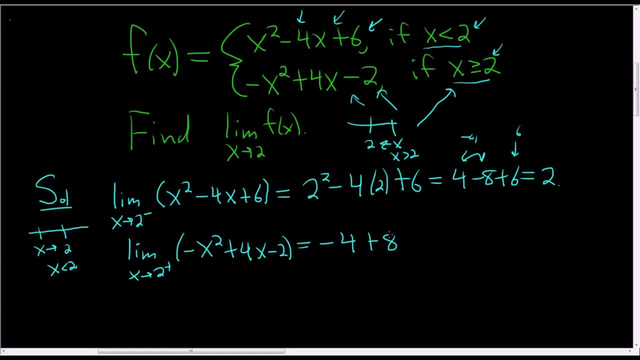 So we get negative 4 plus 8.. 4 times 2 is 8, minus 2.. So negative 6 plus 8 is equal to 2.. So the limit from the left is equal to 2.. The limit from the right is equal to 2.. 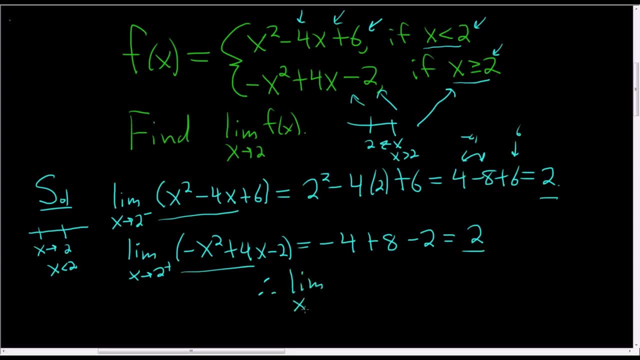 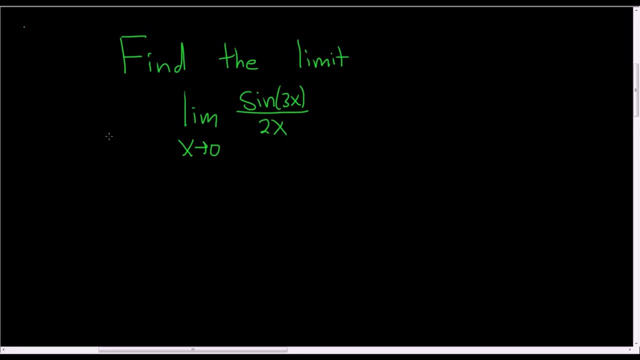 So therefore, The limit as x approaches 2 from any direction is also equal to 2.. Now, if we had gotten different answers here, then the limit would not exist. Find the limit as x approaches 0 of sine 3x over 2x. 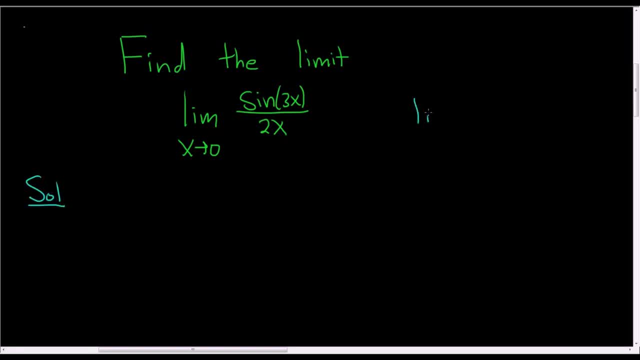 Solution. So the goal is to write it in a way that lets us use this limit here. The limit as x approaches 0 of sine x over x is equal to 1.. So we want to rewrite What we have in this form here. 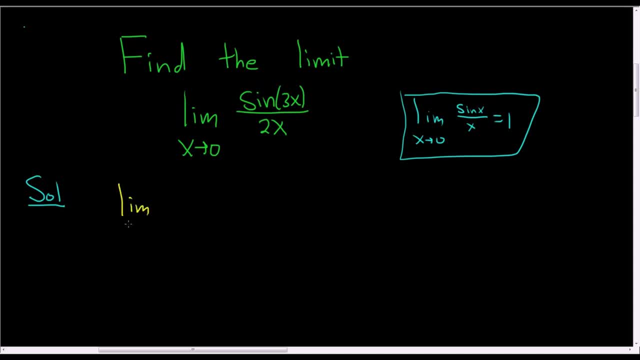 So let's go ahead and carefully do that. So this is the limit as x approaches 0.. Well, we have sine of 3x, So sine of 3x, And it would be nice if we could make the 3x match down here. 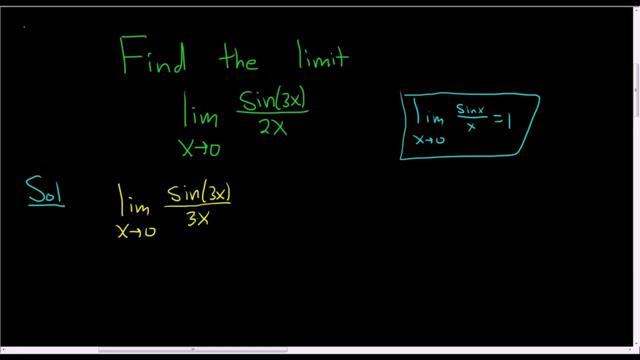 So let's go ahead and put it there. But we can't really do that, We can't really just put a 3x here. Well, first of all we have to deal with the 2.. Well, we can pull the 2 out. 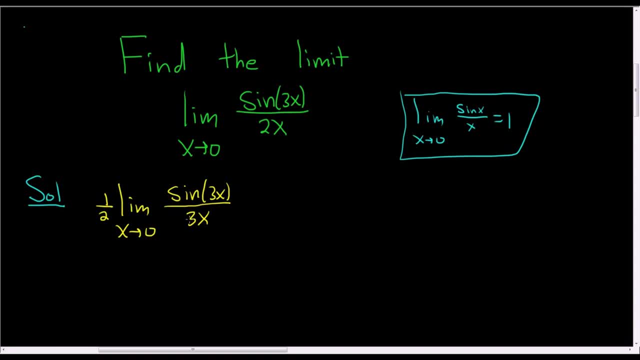 That's really 1 half, And then, in order to get rid of the 3,, we can multiply by 3.. So we end up with 3 halves, And this limit here is 1.. So 3 halves, And that's it. 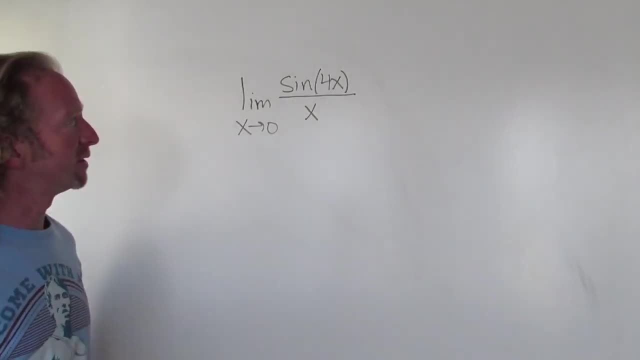 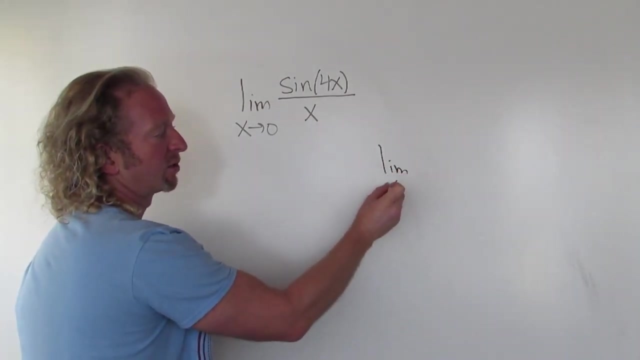 Hey everyone, In this video we're going to find this limit. So in order to find this limit we have to use another limit. So recall that the limit, as x approaches 0 of sine x over x, that is equal to 1.. 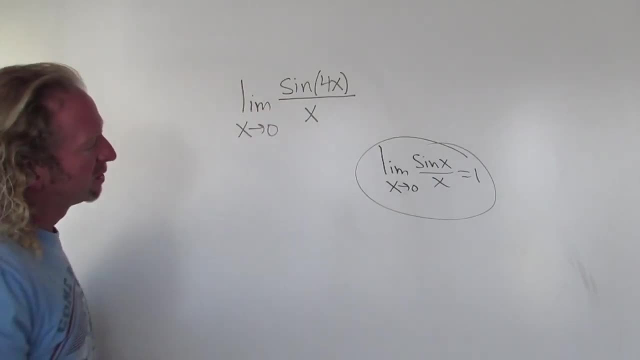 So we're going to use this limit to figure out this one. So the idea here is to make the numbers match. So here we have a 4x, So we should have a 4x here as well. So we're going to rewrite this as limit x approaches 0, sine 4x. 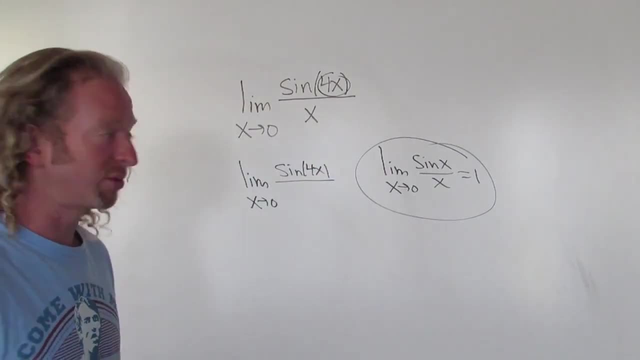 And so on the bottom, we want a 4x. Right, We have an x here. So what we do is we just put it there. So we just put it there. You say, whoa, you can't just put stuff there. 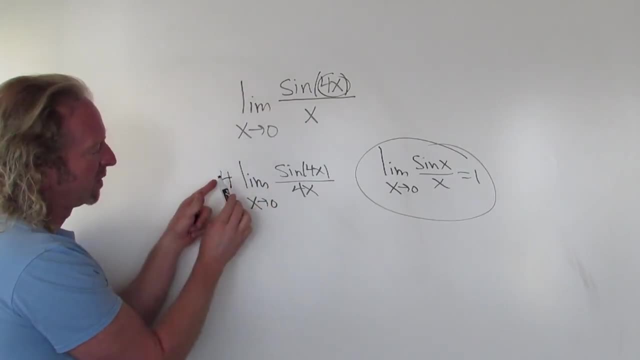 Yes, we can. Right, Because what you can do is you can put a 4 outside, Because when you do that, you're going to get a 4. When you distribute, you would do 4. And then these 4s would cancel and you'd get back what's up top. 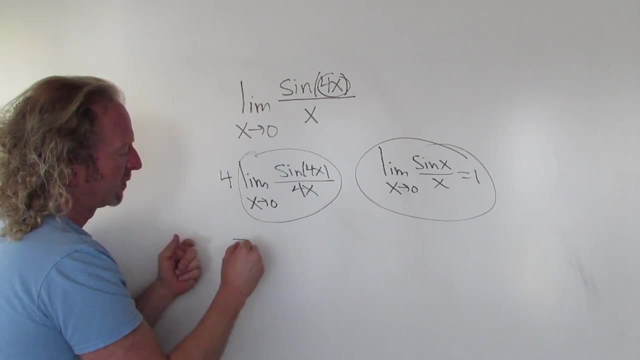 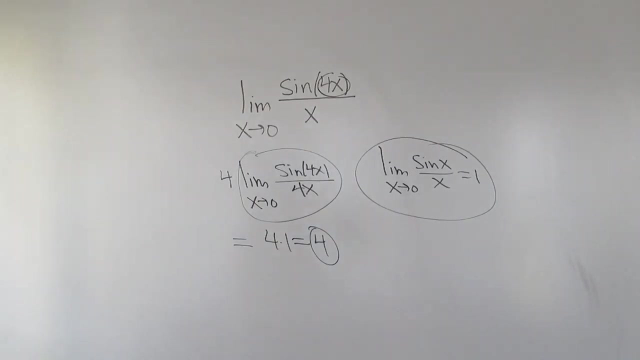 So now that these numbers match, this whole thing here is equal to 1.. So it's 4 times 1., And so the answer is 4.. That's it, This problem. we have to compute a limit as x approaches 0.. 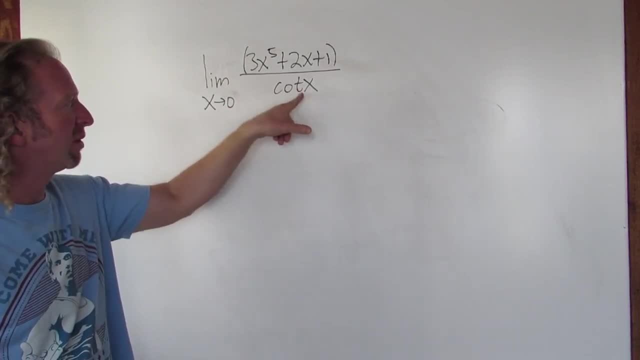 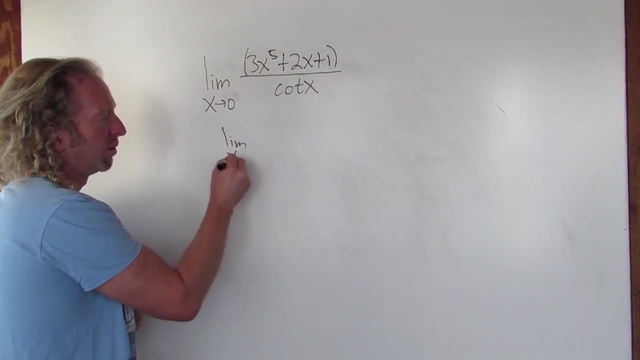 So we have a polynomial over cotangent. So if you plug in 0, cotangent of 0 is not going to work Right. And the reason is: if you're not sure, if you're not sure what to do, then a good first step. 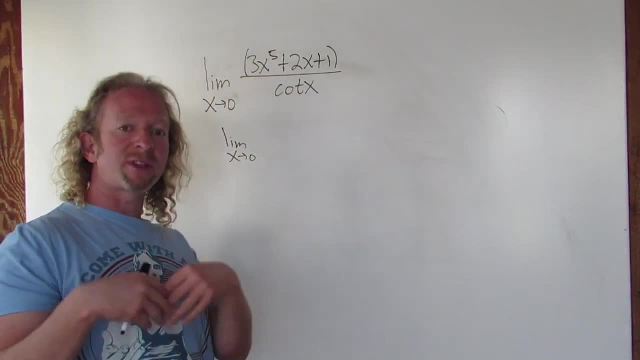 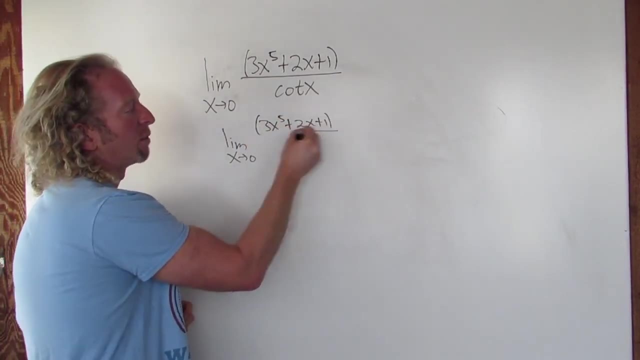 even before you plug in 0, is write cotangent in terms of something that you're more familiar with. So the numerator stays the same. So it's 3x to the 5th plus 2x plus 1.. But cotangent is cosine over sine. 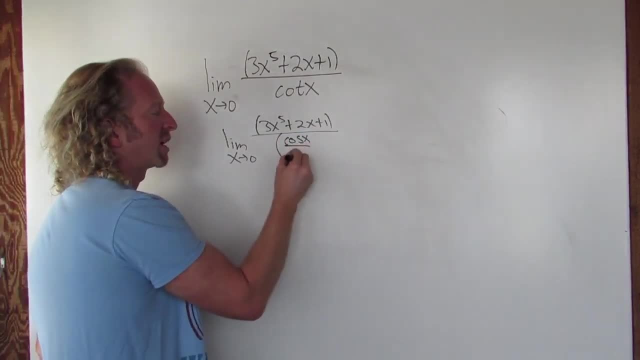 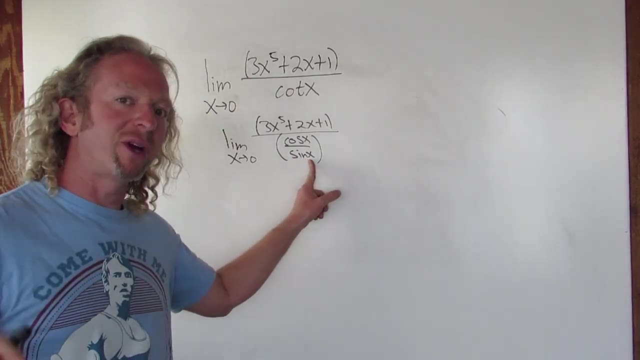 Right, So this is cosine of x over sine x. And now you see, if you plug in 0, it does not work, because then you get the sine of 0, and sine of 0 is 0, and you cannot divide it by 0. 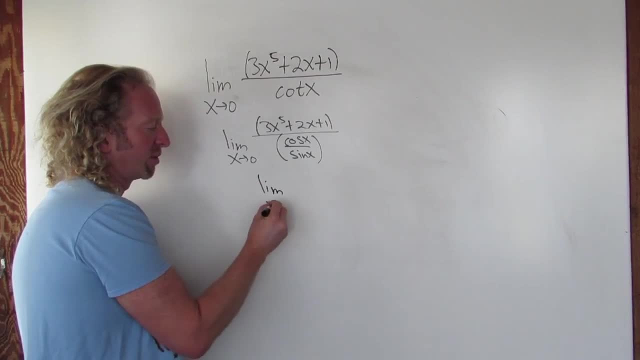 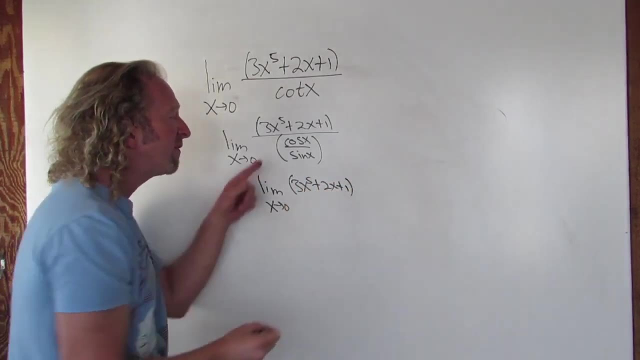 So what you do next is you just do some algebra. So this is the limit as x approaches 0, and we still have this piece here. So 3x to the 5th plus 2x plus 1.. We're dividing by cosine over sine. 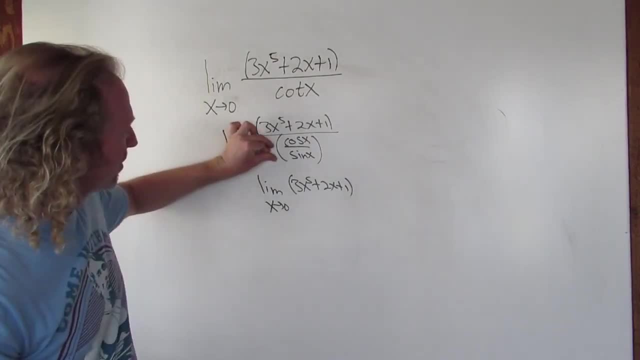 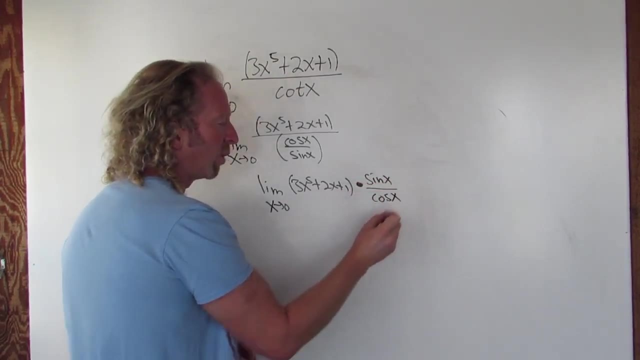 So when you do that, you multiply by the reciprocal Right. So the reciprocal of cosine over sine is sine over cosine. So it's times sine over cosine. And now we're in a position where we can actually plug in 0. Because if you plug in 0 here on the bottom, the cosine of 0 is 1.. 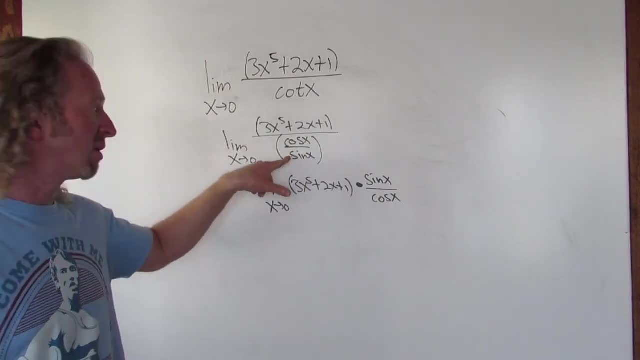 See, we couldn't do it over here, Right? So when you do it here, sine of 0 is 0, so you get a number over 0. You can't have 0 on the bottom, But now we can do it here. 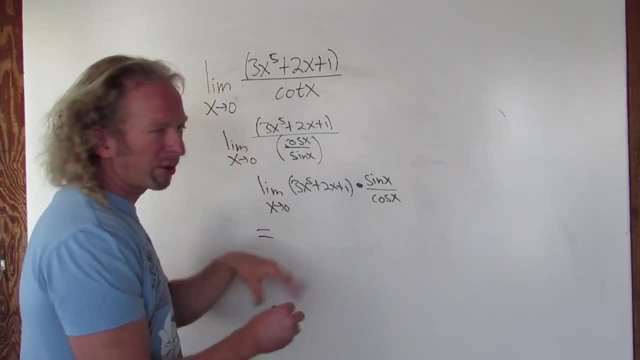 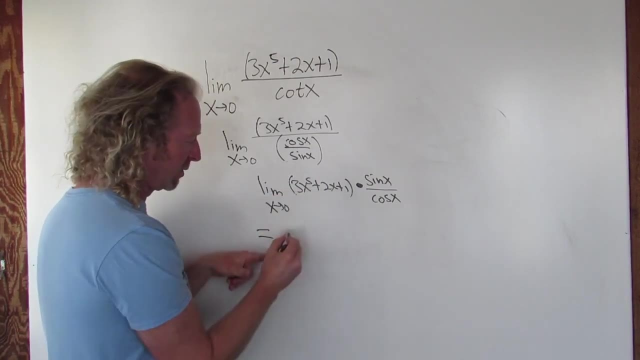 So now you just replace all of your x's with 0's. This is the part where you drop the limit sign. Whenever you evaluate the limit, that's when you drop your limit sign. Okay, So this is going to be 3 times 0 to the 5th, so just 0 plus 0 plus 1.. 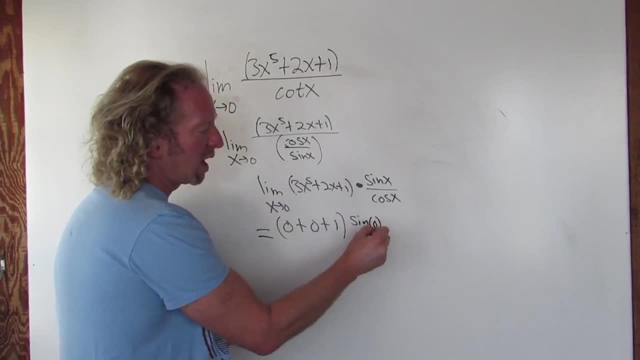 Sine of 0,, which is- I'll write it- sine of 0, and then cosine of 0.. Good stuff, This is just 1.. Sine of 0 is 0,, cosine of 0 is 1, you just get 1 times 0, so the answer ends up being: 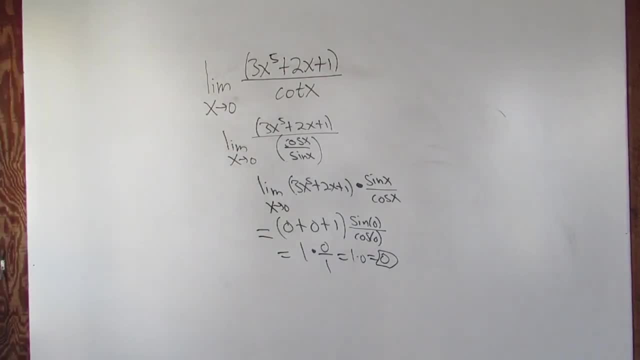 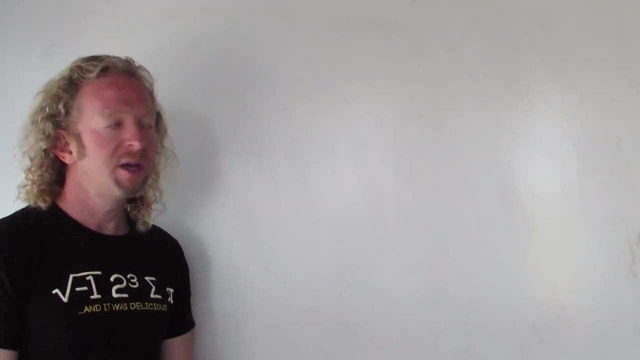 0.. That's it, Hey, YouTube. In this video, we're going to talk about what it means for a function to be continuous. So intuitively, a function is continuous if you can draw it without picking up your pen or pencil. 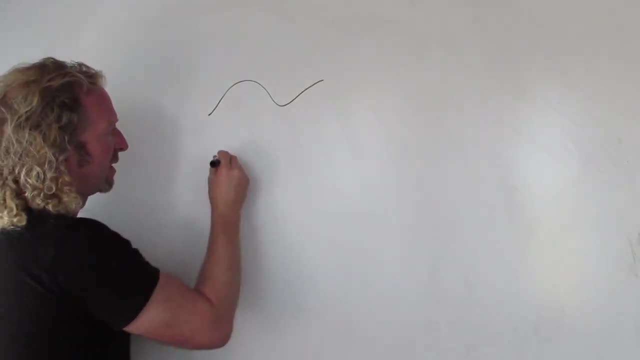 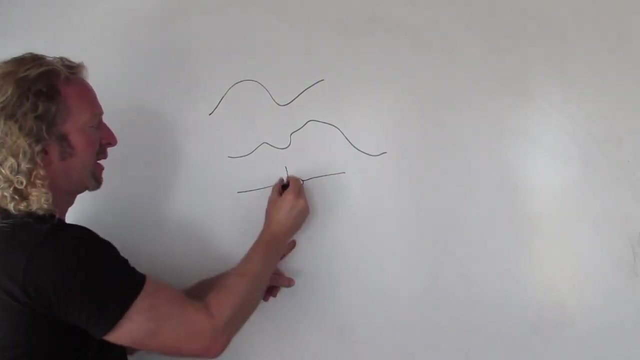 So something like this would be continuous, Something like this would be continuous, Something like this would not be continuous, Something like this would be continuous at this particular x value, So like, for example, if this was 3,, we would say: the function is not continuous at 3, or. 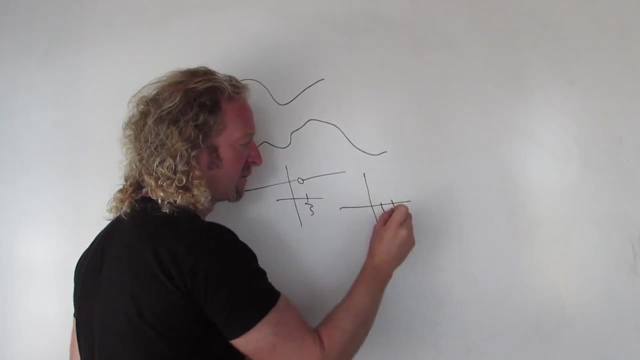 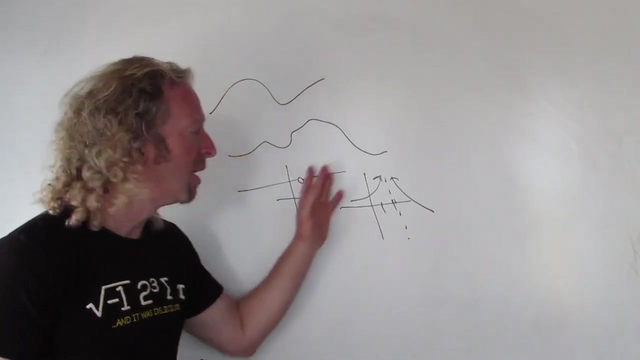 discontinuous. Another example would be something like this: You have a vertical asymptote that gives you a break, So this function would not be continuous at x equals 2, but it would be continuous everywhere else. Okay, It would be continuous everywhere else. 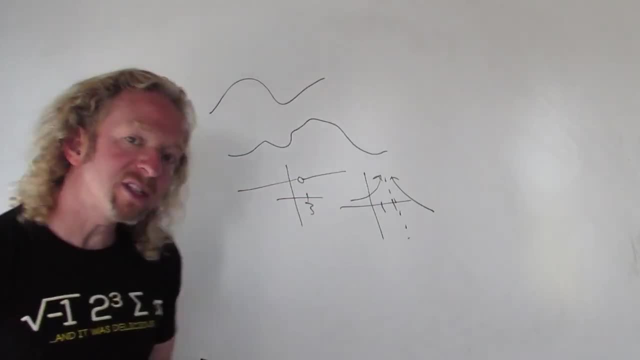 So intuitively. a function is continuous. if you can draw it without picking up your pen or pencil, What does it mean for a function to be continuous at a point? That's how we define continuous. Okay, That's how we define continuity. 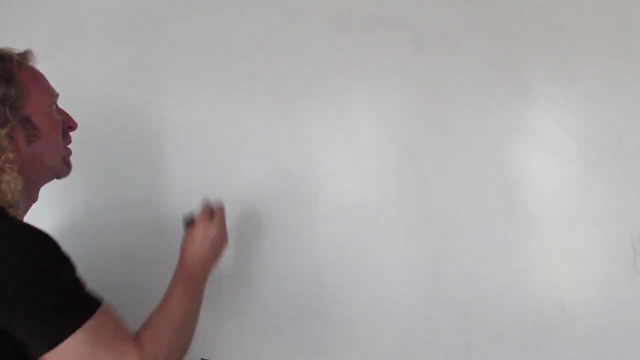 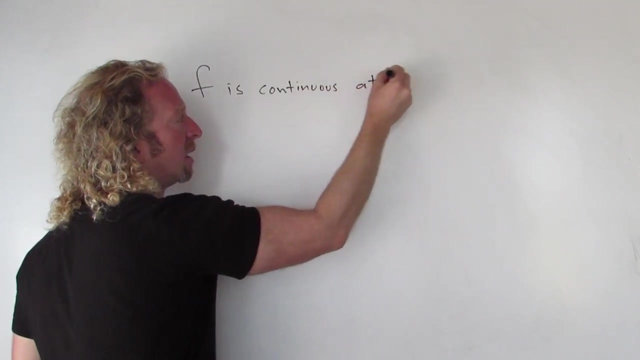 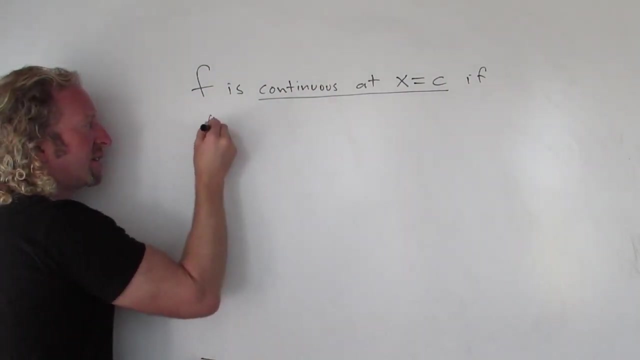 So let's do it. So we're going to say: a function is continuous, So f is continuous at x equals c, if the following three conditions hold: Okay. The first condition is that the function has to be defined there. Okay, So f of c is defined. 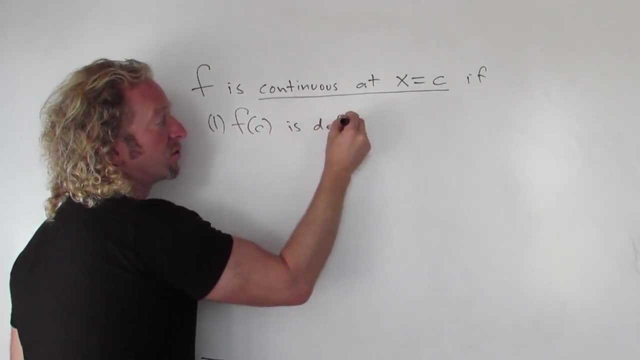 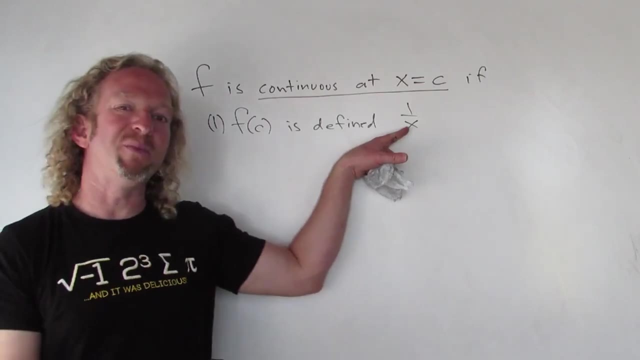 f of c is defined. So, for example, 1 over x would not be continuous at z. Okay, Because you could not plug in 0. So this function would be discontinuous at 0.. Right, Because 1 over 0 doesn't make sense. 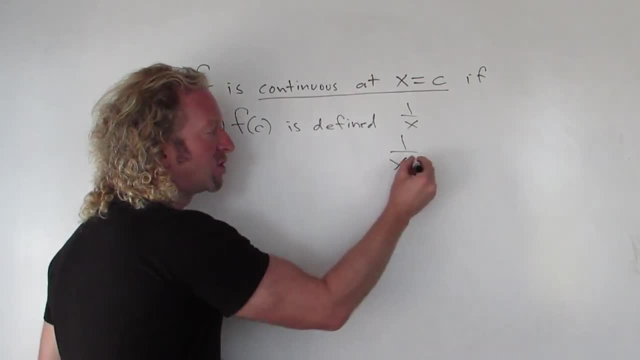 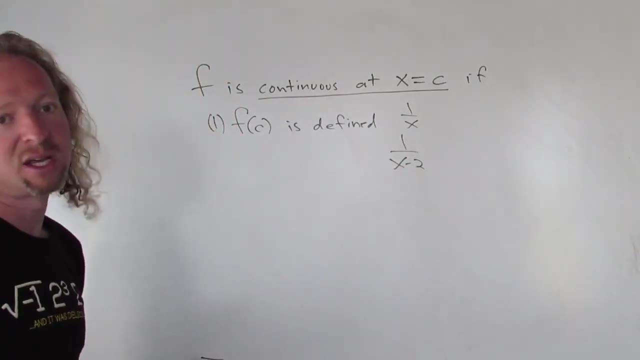 So this function is not continuous at 0.. Another example: 1 over x minus 2, this would not be continuous at 2.. Right, Because 2 minus 2 is 0. So you get division by 0. So that would not be continuous there. 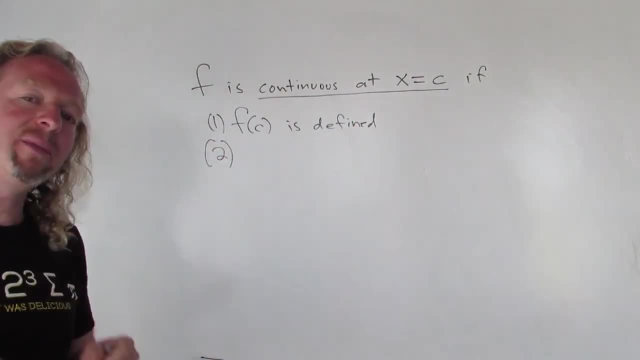 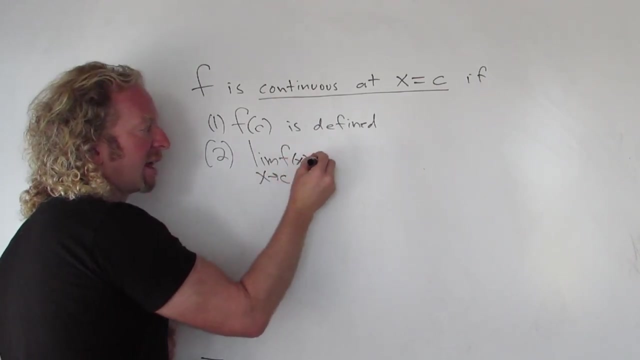 The second condition for continuity is that the limit has to exist at that number. Okay, So if the limit as x approaches c of f of x, that limit has to exist. Okay, The limit has to exist. What does that mean? That means it's equal to a real number. 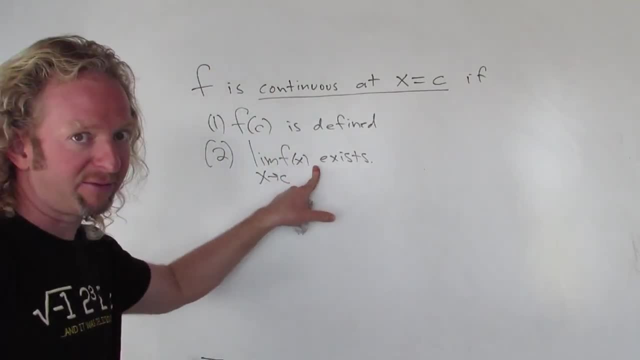 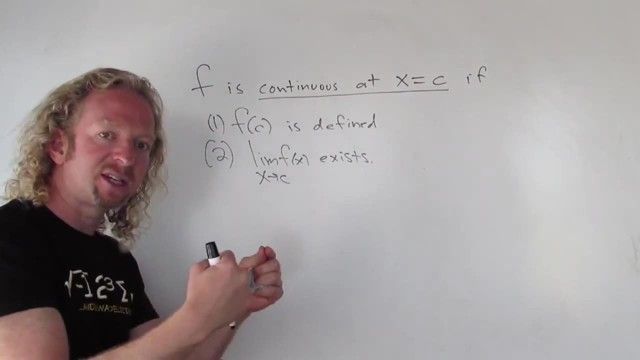 So it has to be equal to a real number. So it can't be infinity or negative infinity. And that means that both one-sided limits have to give you the same value. So, like from the left and the right, you have to get the same limit. 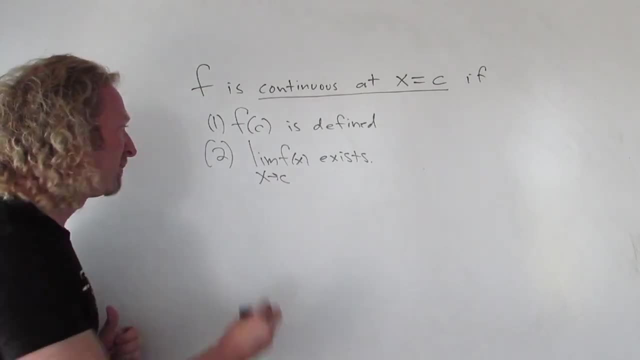 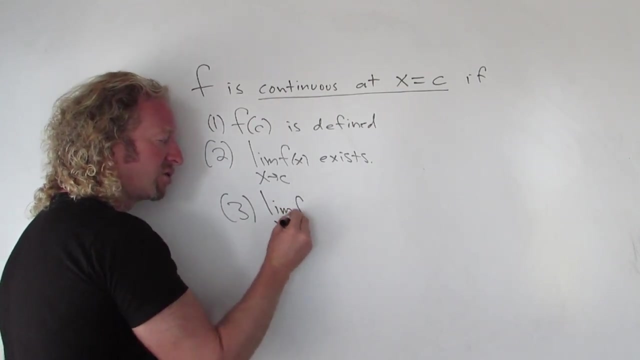 That's what this means, Right? This means the limit exists from both directions. And then three: not only does the limit exist, It has to be equal to the function value there. So when you take the limit of f of x, as x approaches c, it has to be equal to f of c. 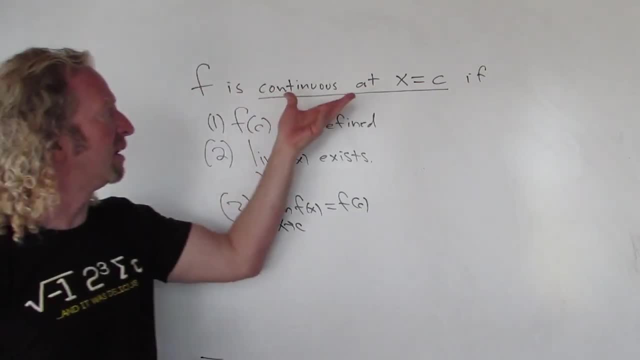 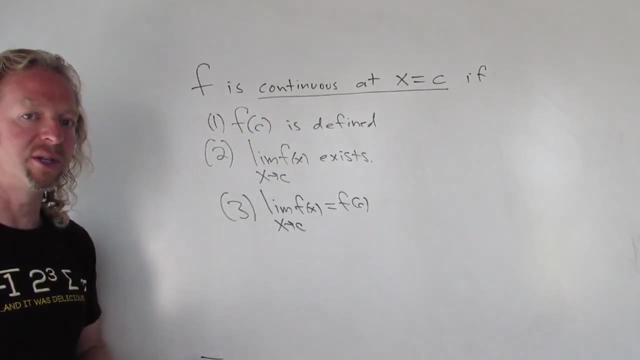 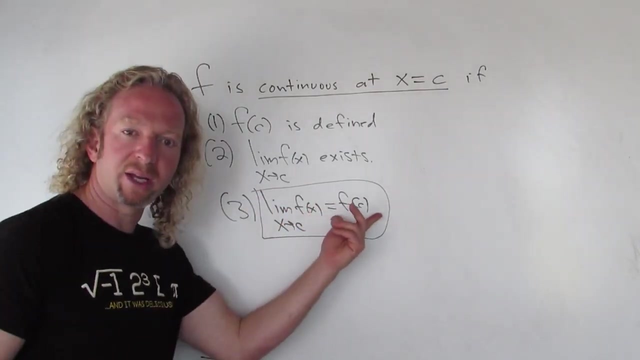 So these are the three conditions that make up the definition of continuity. So if a function satisfies these three things, then we say the function is continuous at x equals c. It turns out all you need is really this one. Check this out If someone writes this down, right? 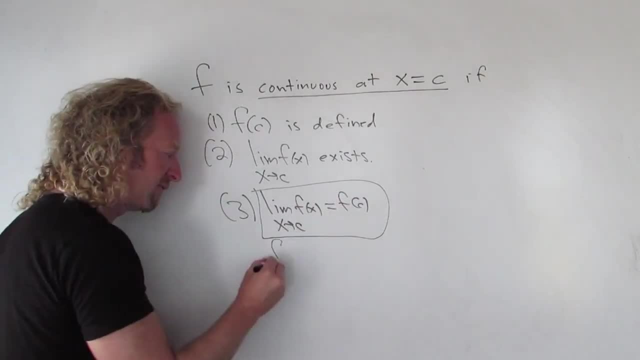 This limit. If someone writes down f of c, Like if you write down f of c, If you write down f of 2, well, it must be equal to something, right, Like you're implying: oh yeah, it's equal to 7, or it must be equal to something. 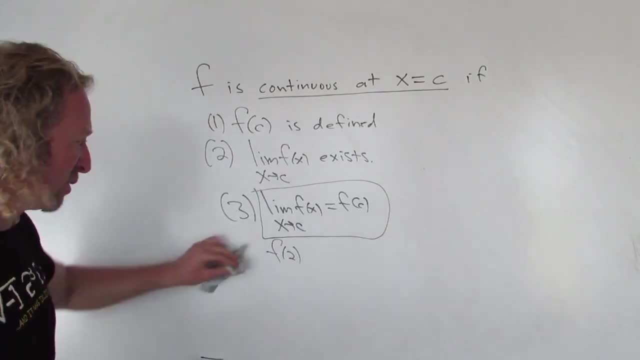 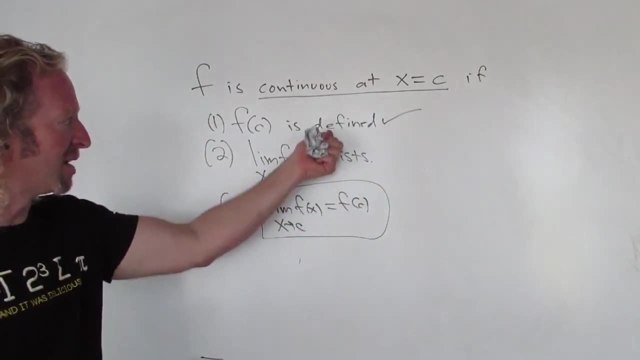 In other words it's a number, In other words it's defined. So if someone writes this down, they're already saying that f of c is defined. That takes care of the first condition. So this condition implies the first one. 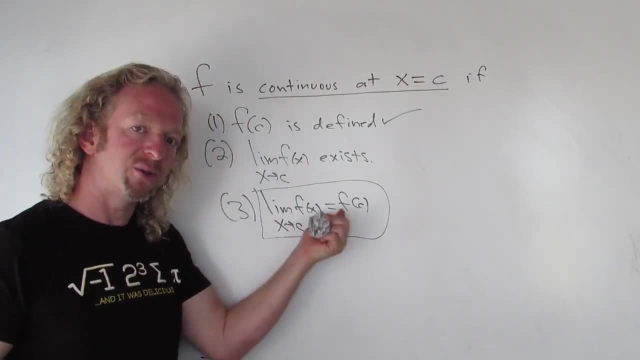 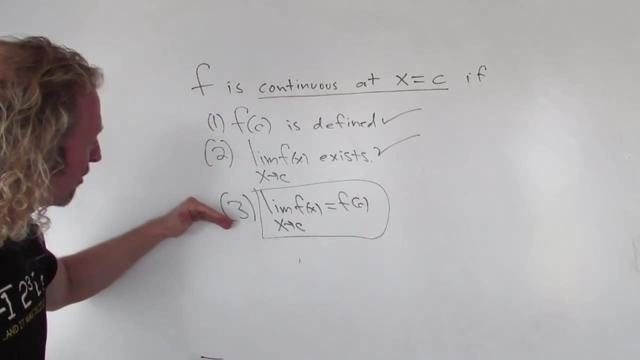 Oh, but look, The limit is equal to a number. The limit is equal to a number. That's precisely what it means for a limit to exist. That means the second condition is satisfied. Therefore the third condition in the definition of continuity. 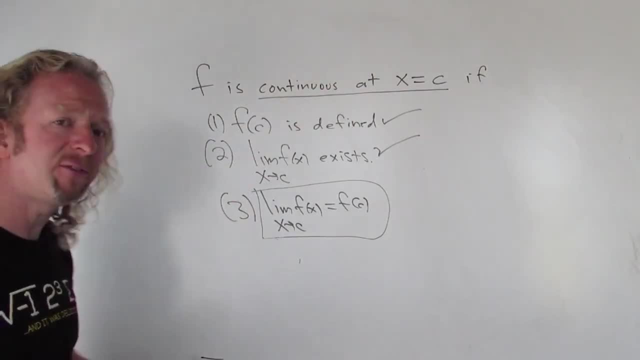 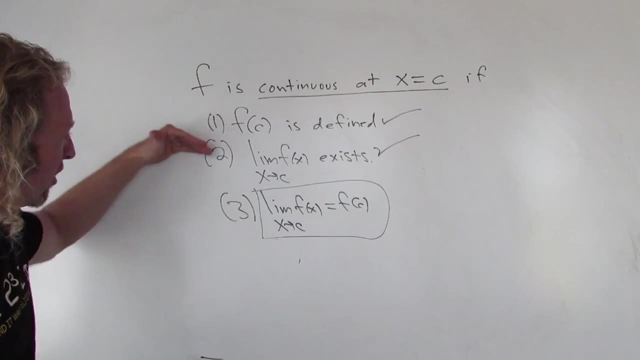 The third condition in the definition of continuity implies the first two. Typically, if you're reading like an advanced calculus book, this is the only definition they give you right. In a regular Calc 1 book you'll get all three. This allows you to break down the definition further by looking at some key examples. 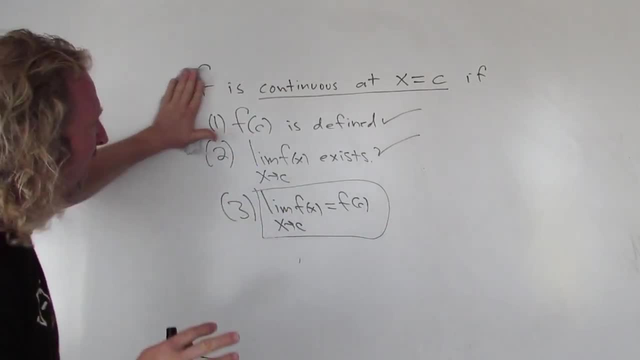 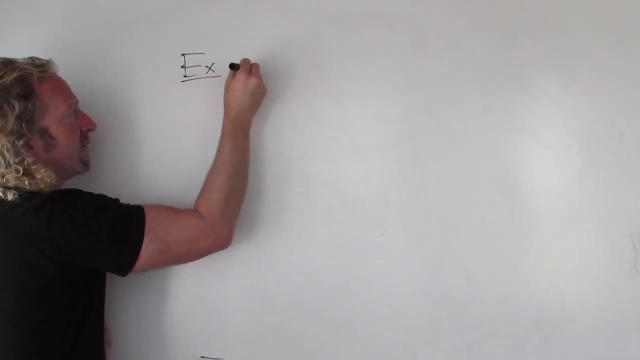 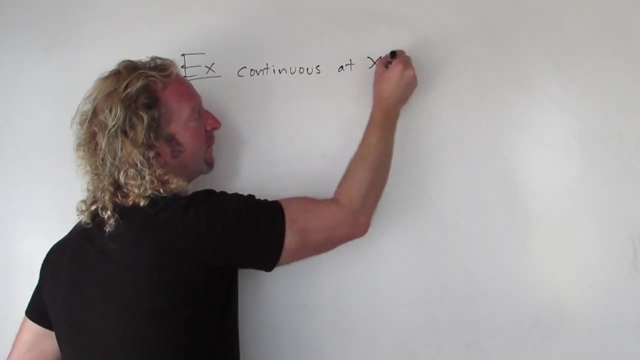 Let's do that. Let's look at some examples where we really overanalyze this definition. So the question will say: is the function continuous at f of c? Let's use a nice number. How about 2?? So continuous at x equals 2?. 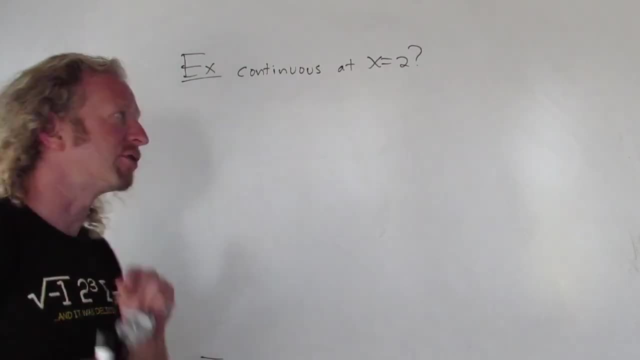 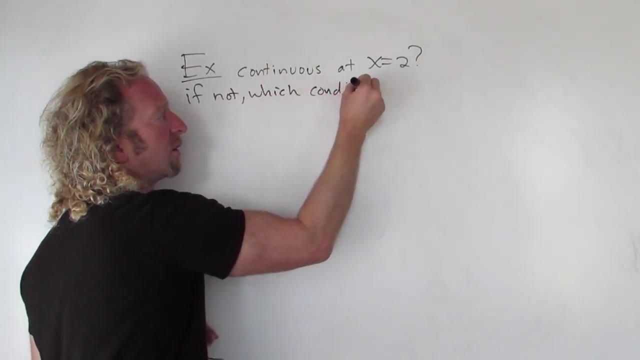 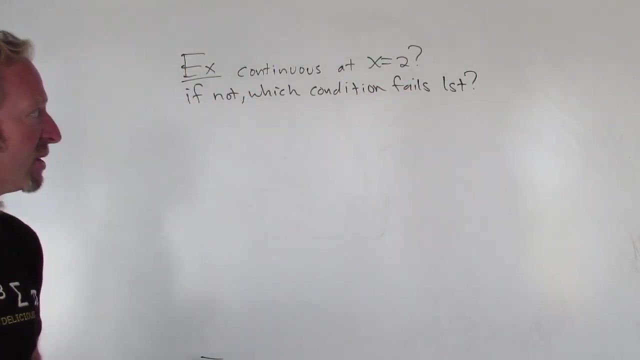 And if not, the question is: which condition fails first? So, if not, which condition fails first? So if it's not continuous, which condition will fail first? As a reminder, the conditions are here, I'll write them down. So the first condition: 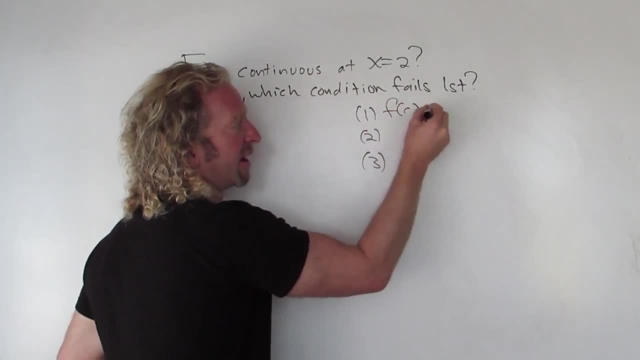 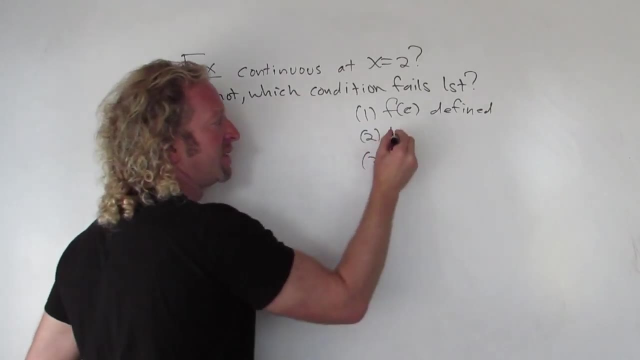 So the first condition was that the function has to be defined there. So f of c is defined. In this case our c will be 2.. 2, the limit has to exist right. So if you take the limit as x approaches c of f of x, it has to be equal to a number. 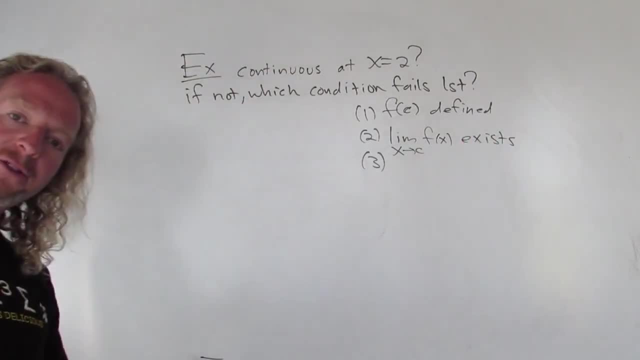 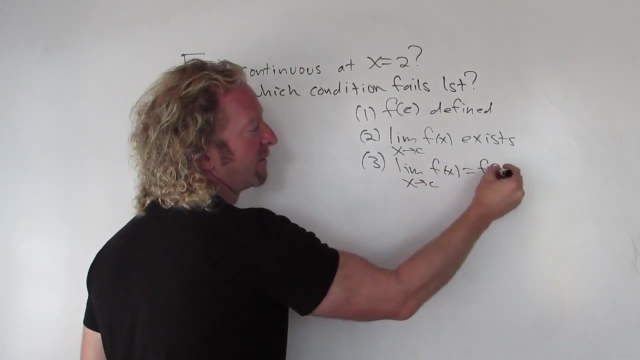 In other words, the limit has to exist. And the third condition was: not only does the limit have to exist, it's equal to your function value there. So it's equal to f of c. So that was the definition of continuity of a function. 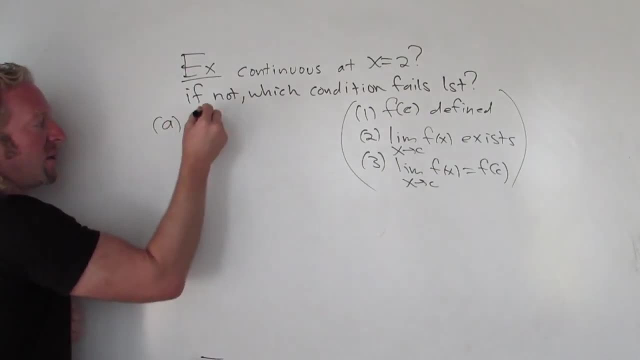 So that was the definition of continuity of a function. at x equals c. All right, So let's look at some examples. Let's say, we have here, Here's 2, 1, 2.. Simple example. Oh, a little hole there. 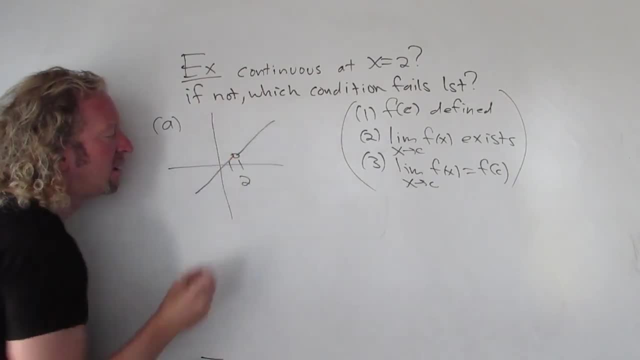 So obviously this violates our intuitive definition of continuity. right, There's a hole. We're not allowed to have holes or breaks. So the answer is no, It's not continuous. And which condition fails first? Well, there's a hole, right. 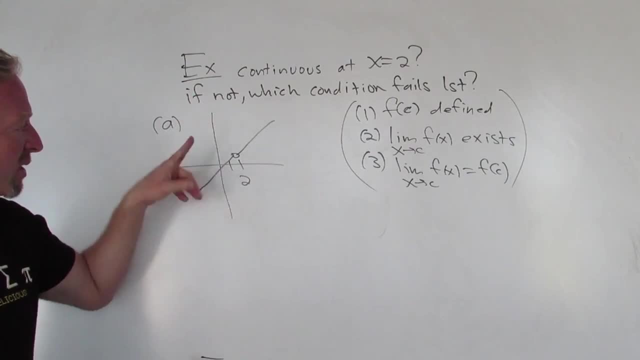 So it's not defined. So in this case it would be: condition 1 fails first. f of 2 is not defined in this case. So the answer is no, It's not continuous. And which condition fails first? Well, there's a hole, right. 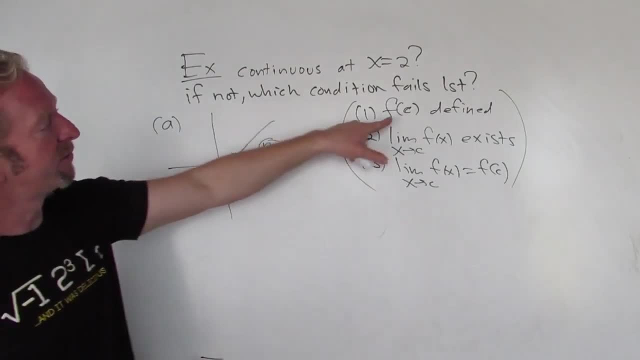 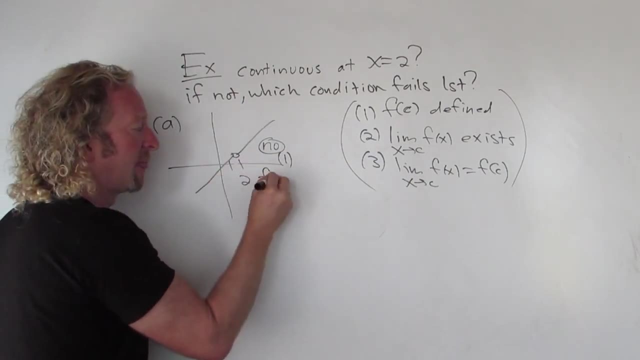 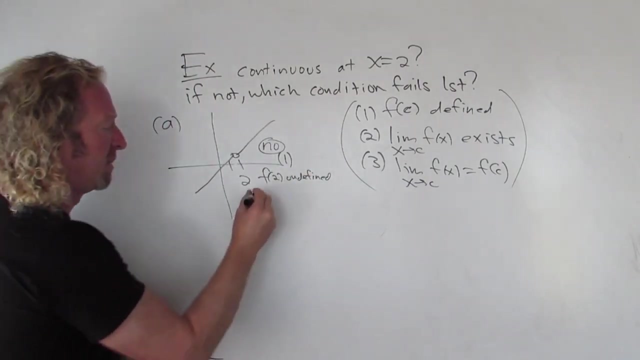 So it's not defined. So in this case it would be: condition 1 fails first. f of 2 is not defined in this case right. So f of 2 is undefined. Right, It's not defined, So condition 1 fails first. 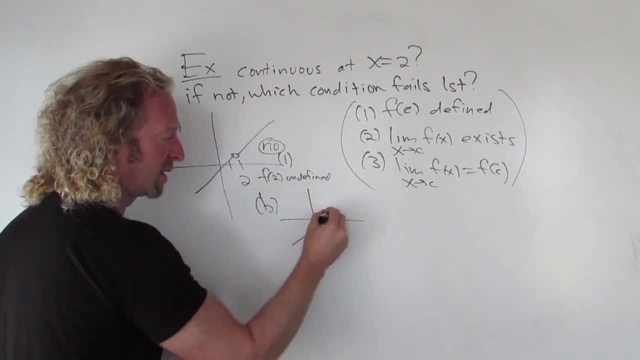 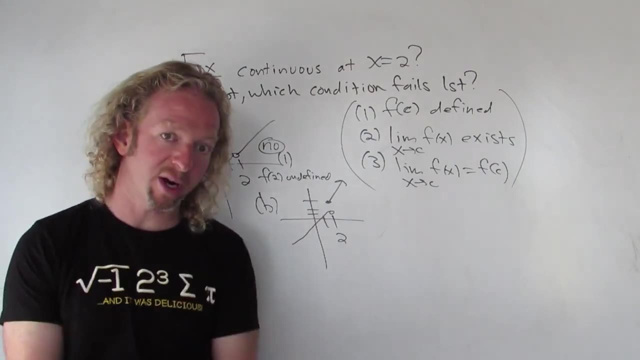 Condition 1 fails first B. So another example: Same thing: Here's 2.. The same picture with the hole, except this time let's fill in the hole up here. So in this case it's not continuous because there's a break right. 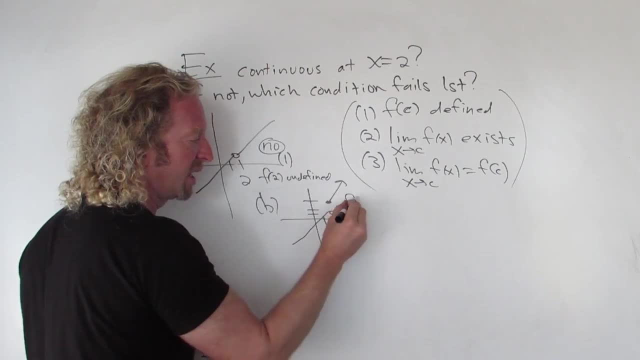 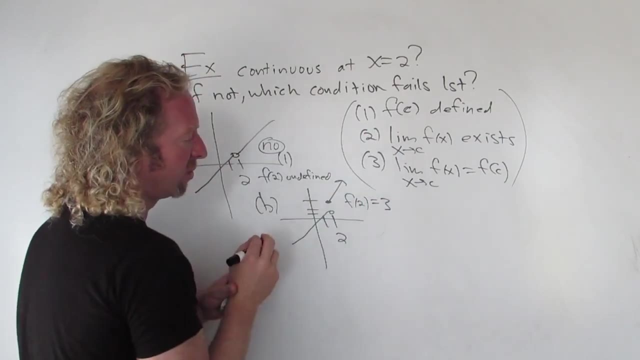 But But the first condition does work: f of 2 in this case. well, f of 2 is the y value when x is 2.. So f of 2 is equal to 3.. So the first condition holds. However, the limit does not exist, because if you take the limit from the left, you get 2.. 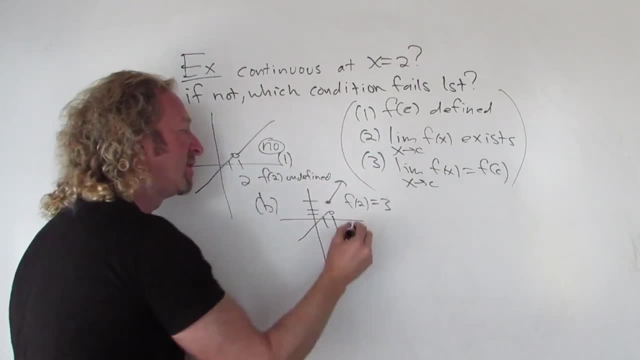 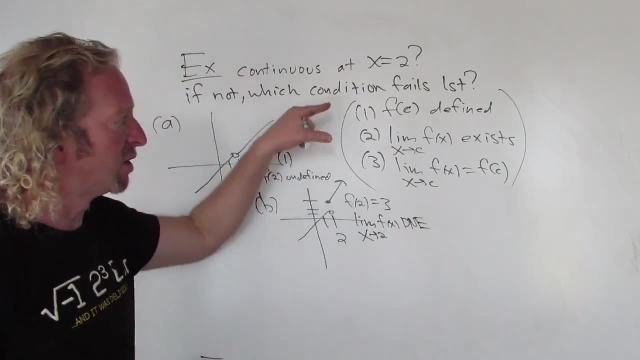 If you take the limit from the right, you get 3.. Therefore the regular limit does not exist. So the limit as x approaches 2 of f of x does not exist. This would mean that condition 2 fails first. So the answer here would be no and it would be condition 2, right, because the limit does not exist. 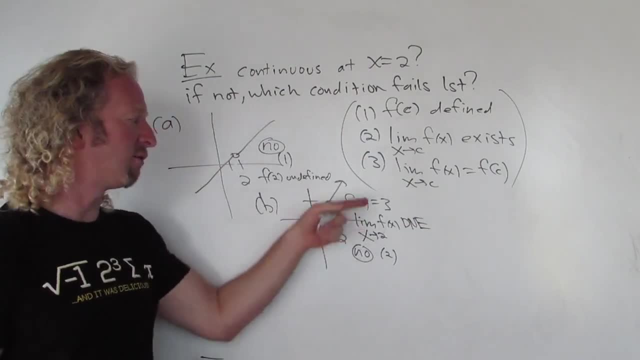 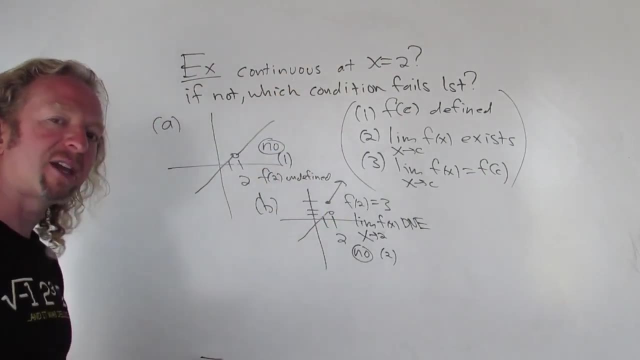 Again, the limit from the left is 2.. The limit from the right is 3.. Therefore the limit does not exist. So condition 2 fails. first, Kind of cool to see you know the different things, what different things can make a function not continuous. 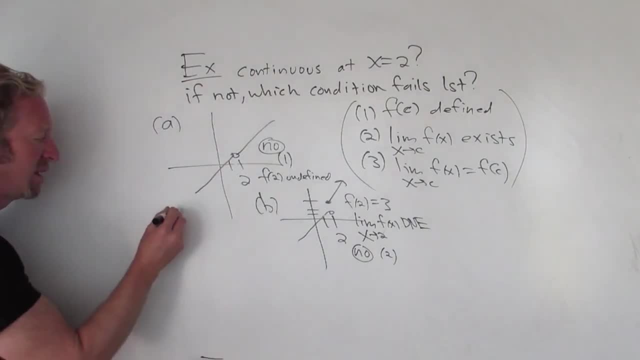 Let's do another one. So I'm going to erase. I think that'll squeeze it in here. C, Here we go. Oh, you can see all three on the board at the same time. So 1, 2.. So let's see here. 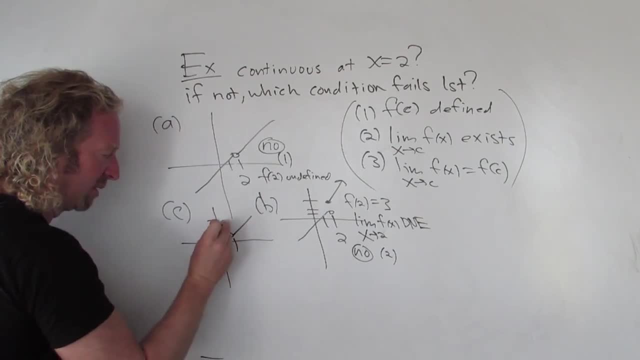 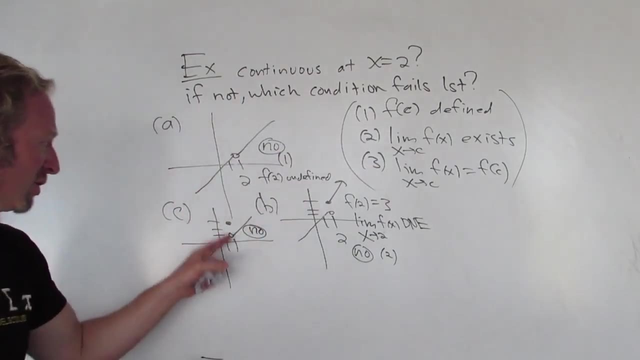 A little hole, All right, But then I'm going to fill in the hole up here, Okay, So in this case, the function is defined. Oh, it's not continuous. first of all, right, Obviously right, There's a hole. 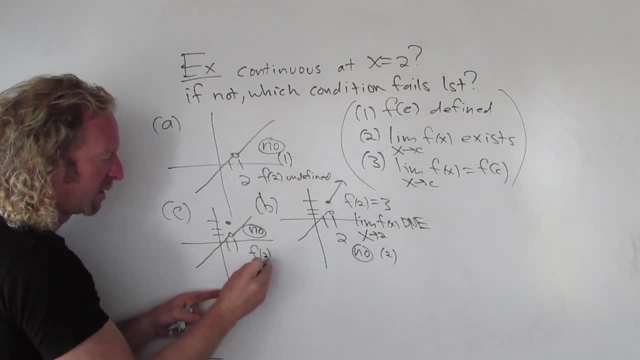 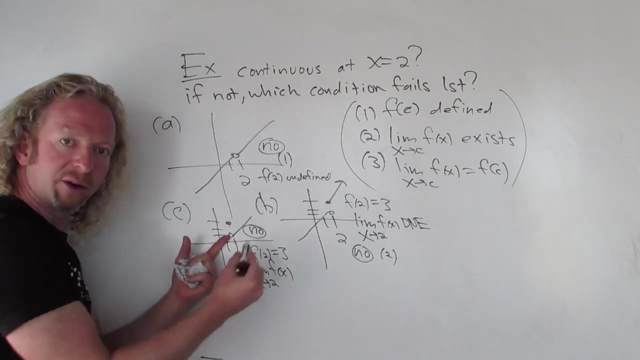 So the function is defined right because f of 2 is equal to 3, right. The y value, when x is 2, is equal to 3.. The limit actually exists right If you take the limit as x approaches 2 in this example. when you approach 2 from the left, you get 1.. 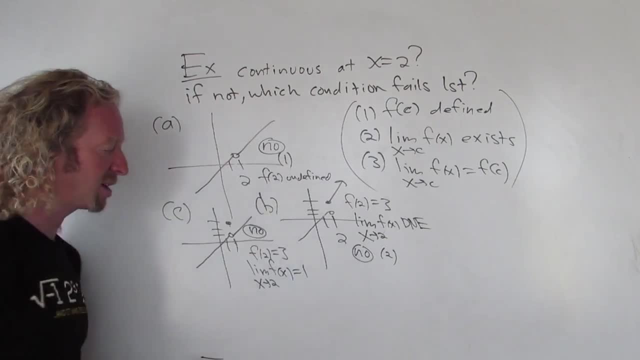 When you approach 2 from the right, you get 1.. Therefore, the limit is 1.. You get 1 from both directions. Therefore, the regular limit is also 1.. However, this is not true, right? The third condition fails, right. 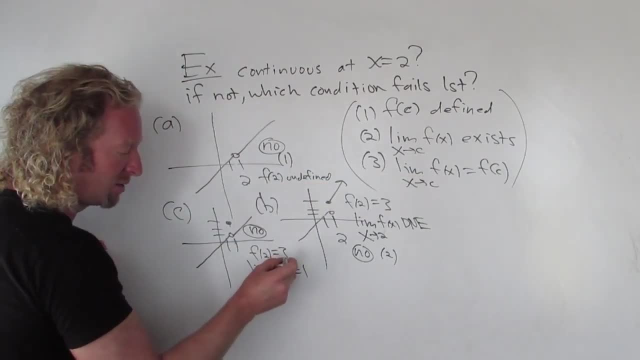 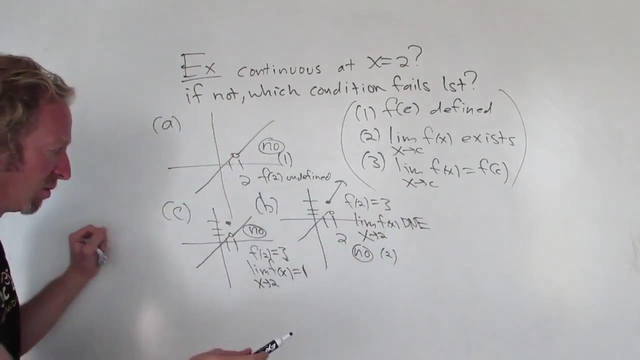 This limit needs to be equal to f of 2, right, That's what it means for a function to be continuous at 2.. But it's equal to 1.. So these numbers aren't the same. They have to be the same for the third condition to be true to be different. 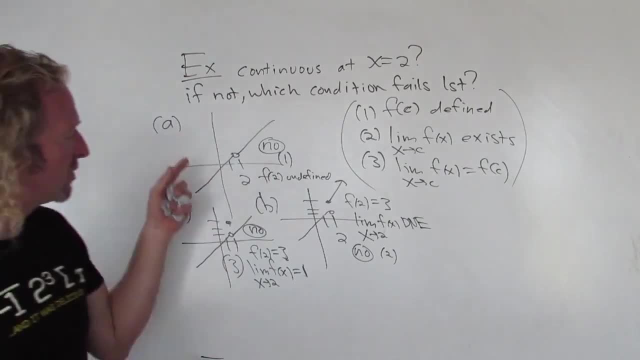 So in this case it's the third condition that fails. So now you see examples of how each condition can fail first in the definition of continuity. I think this is a really cool example. I saw it in a book a long time ago, a Concepts of Calculus book, not a regular calc book. 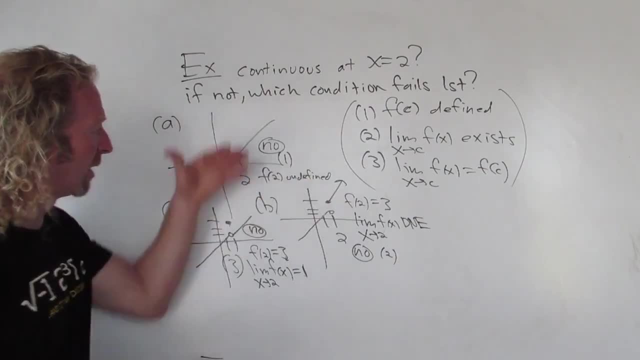 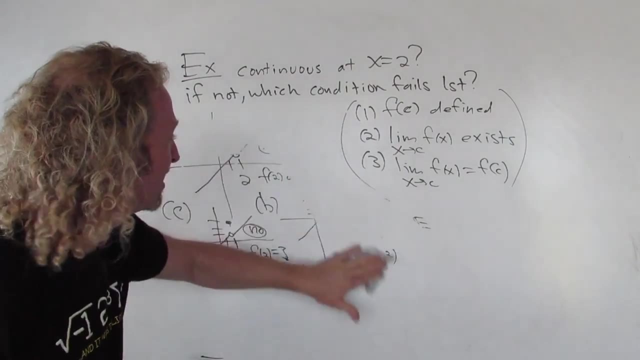 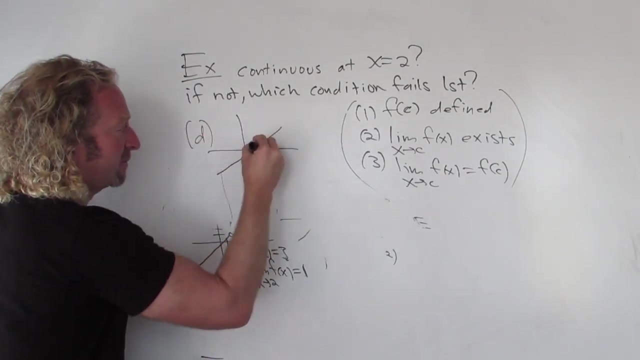 So kind of a cool example, because it shows you examples of how each condition can fail. first, Obviously, the last example is the easiest one, the most boring one maybe, So here's 2.. Then here's your line, So no problem there. 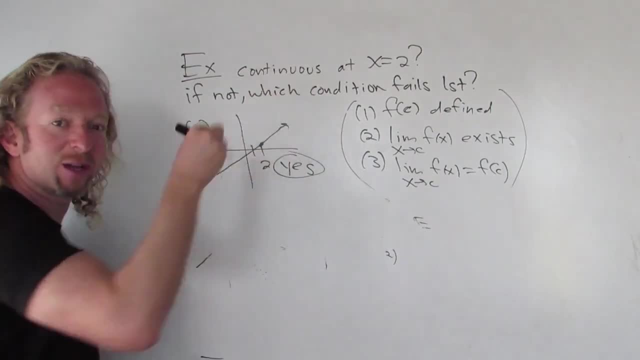 In this case, the answer is yes. right, The question was: does it continue? So we kept saying no. In this case it is continuous. So the main things you should get from this video are one: a function is continuous. 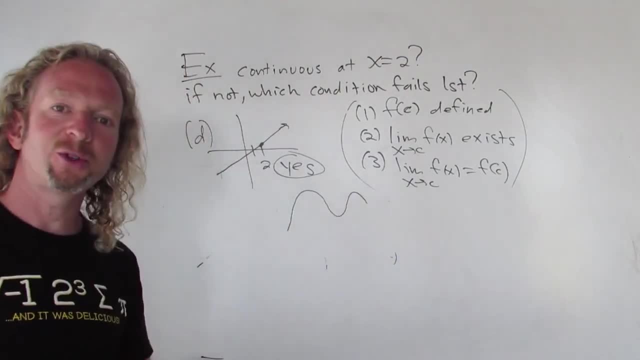 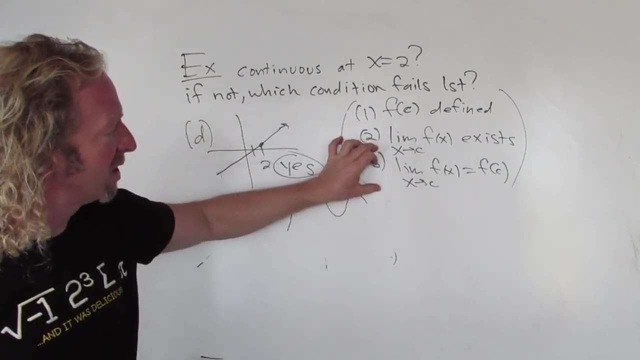 If you can draw it without picking up your pencil and there are no holes and breaks right. Continuous functions are really pretty, And this is the definition of continuity. And the third condition implies the first two, Kind of a subtle point worth keeping in mind. 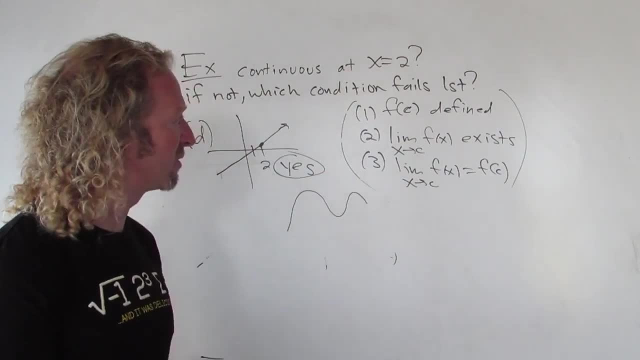 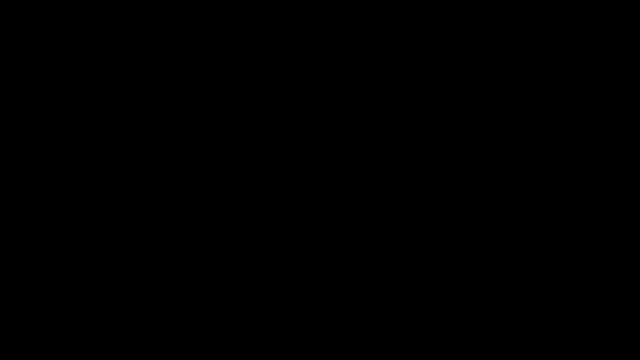 So I hope this video has helped you If you're taking a calculus class or just watching this for fun. thanks for visiting my channel. That's it, Hey, everyone. In this video we're going to talk about two different types of discontinuities. 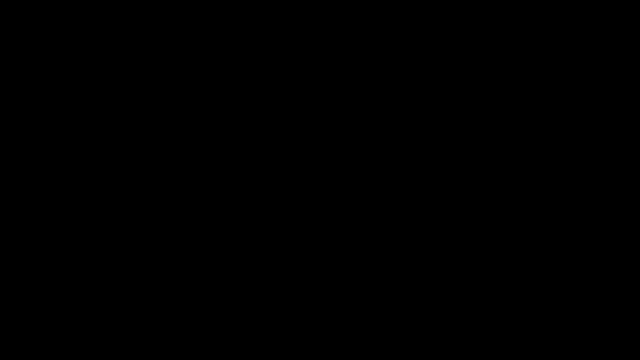 So a discontinuity is a number where a function is not continuous. So, for example, if you have 1 over X minus 2. So this function is not defined at 2.. So X equals 2, this would be a discontinuity. 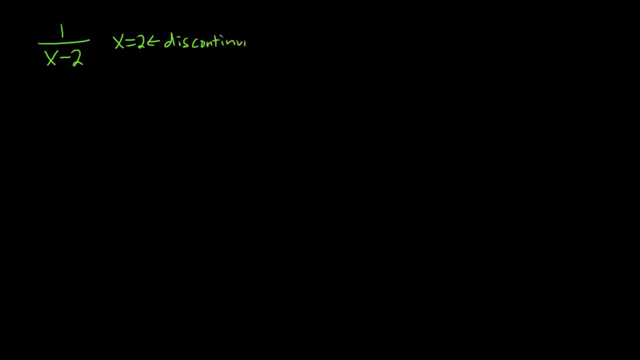 So discontinuity Okay. Because if you plug in 2 at 2, it's only a number Okay. So if you plug in 2 at 2, it's only a number Okay. So if you plug in 2 at 2, it's only a number. 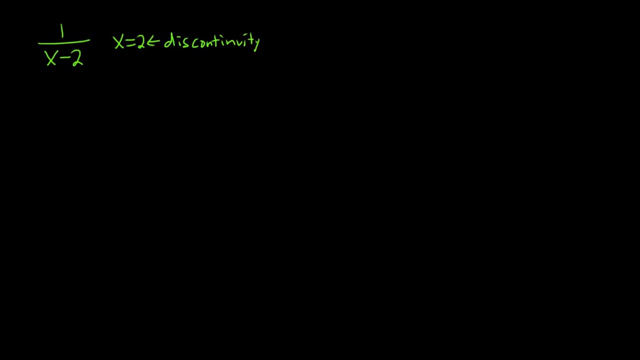 So discontinuity is not continuous. So discontinuity is not continuous. So in the bottom you get 1 over 0, so the function is not defined, so it's not continuous. Another example would be something like x plus 1 over x plus 1, x minus 3.. 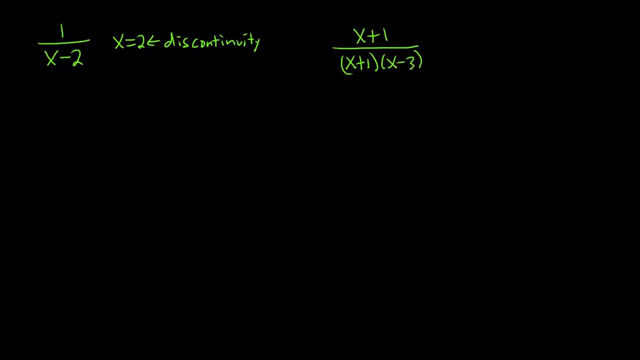 This function has two places where it's not continuous: right, It's not continuous at negative 1,. right because that makes the bottom 0, and also at 3, because that makes the bottom 0 as well. So both of these are discontinuities. so discontinuities. 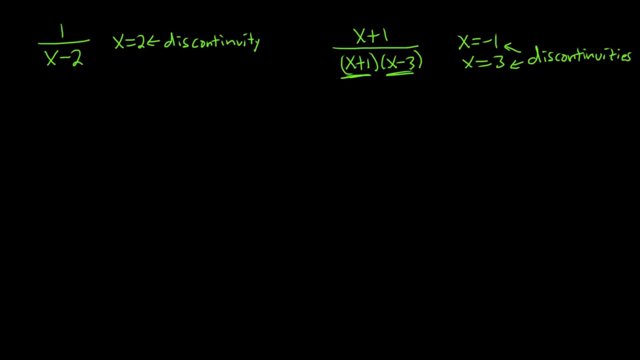 Okay, so in this video we want to talk about two special types of discontinuities. The first type is called a removable discontinuity, so removable. And the second type is called a non-removable discontinuity, so non-removable discontinuity. 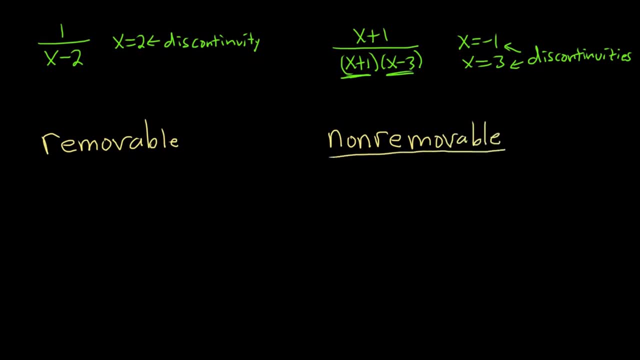 We want to differentiate between the two. So basically, intuitively, a removable discontinuity is a discontinuity that can be fixed. So you can take your function and you can make it continuous at that point by redefining it. So it's a discontinuity that can be fixed. 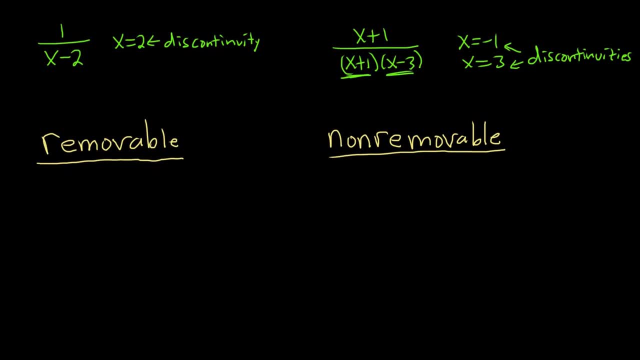 A non-removable discontinuity. well, it's a discontinuity that you can't remove. you can't fix it. So if it's removable, you can remove it and fix it. So an example: here is the example we already just saw. 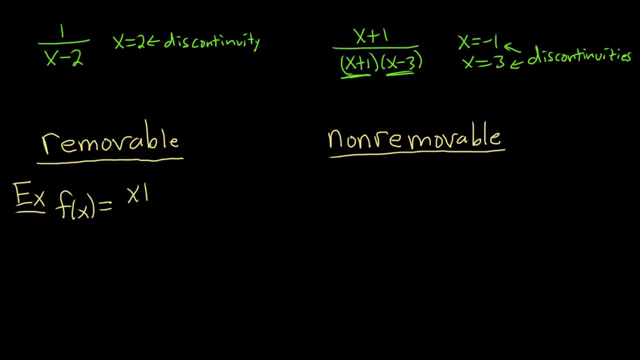 So f of x equals x plus 1.. Just so you understand the intuition: x plus 1, x minus 3.. So this function has two discontinuities. We talked about them, We know one of them is negative 1, because that makes the bottom 0.. 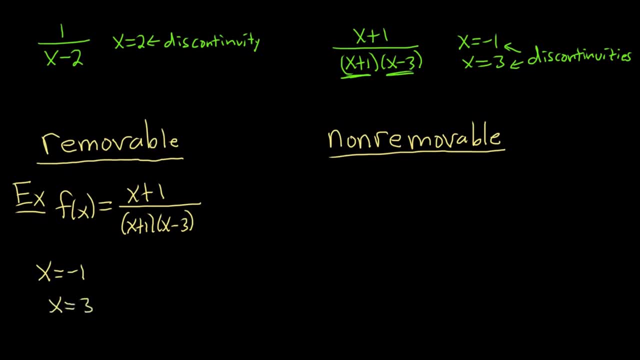 And the other one is 3.. That also makes the bottom 0.. Well, check this out, We can cancel this, And so when you cancel this, you're essentially removing the discontinuity. So boom. So now you get 1 over x minus 3.. 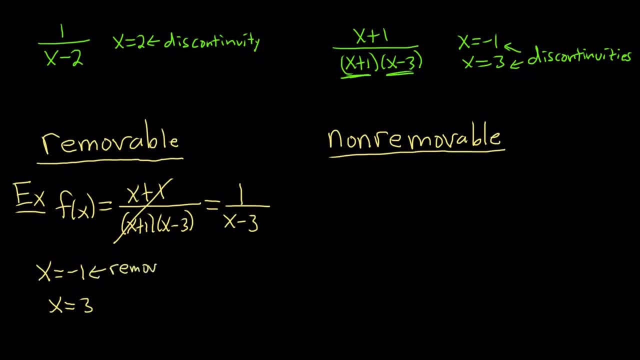 So this has been removed. So this is a removable discontinuity, And this one you can't get rid of it. There is no way. it's a non-removable discontinuity. So that's the intuition behind removable and non-removable discontinuities. 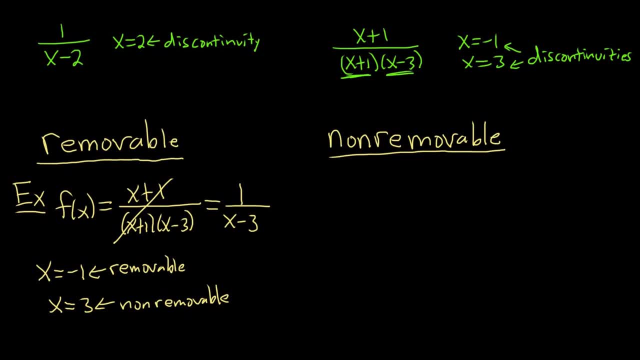 Removable discontinuities can be removed- by canceling in this case- And non-removable discontinuities cannot be removed. This still doesn't make any sense. It's not defined, So it's not continuous. So how do you find them when you're doing problems? 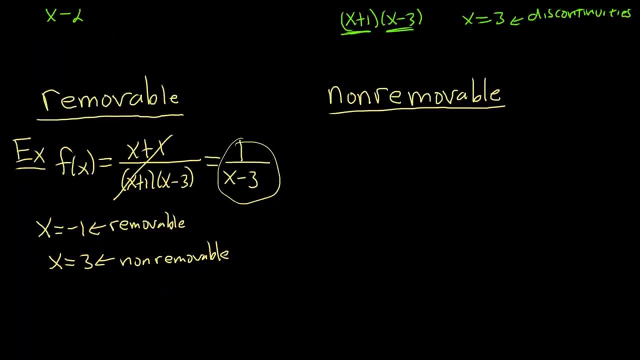 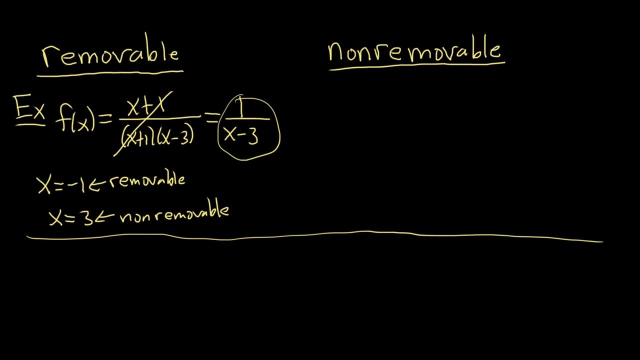 So first of all, let me give you a criteria which always works. So here is the invincible criteria. So let's say that x equals c, Say this is a discontinuity, Discontinuity, Okay. And then let's say that we take the limit as x approaches c of f, of x. 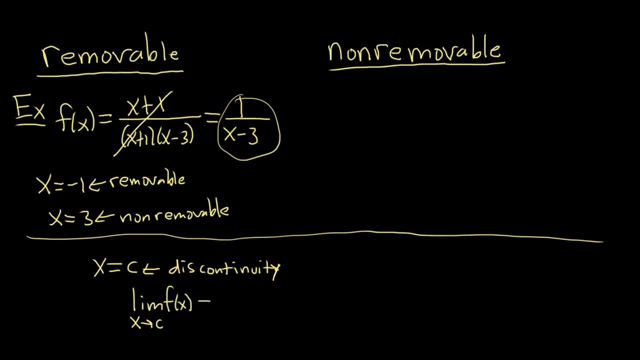 So if this limit exists and is equal to, let's say, l, So l is a real number. So if this exists, then x equals c is removable. Okay, So if this limit exists, so if you take the limit and you get a number, 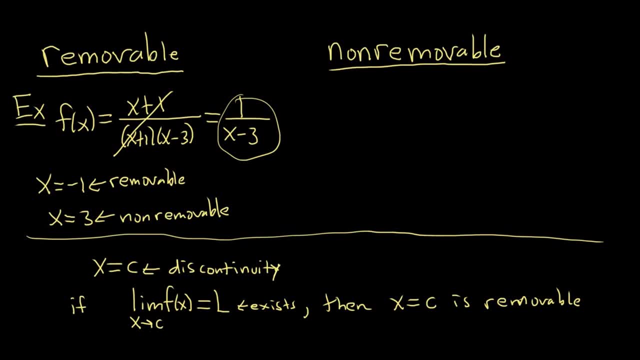 then you can remove the discontinuity, right. You can remove it In this case, here, in our fake example up here. let's think about that: If we take the limit as x approaches negative, 1 of x plus 1 over x plus 1, x minus 3.. 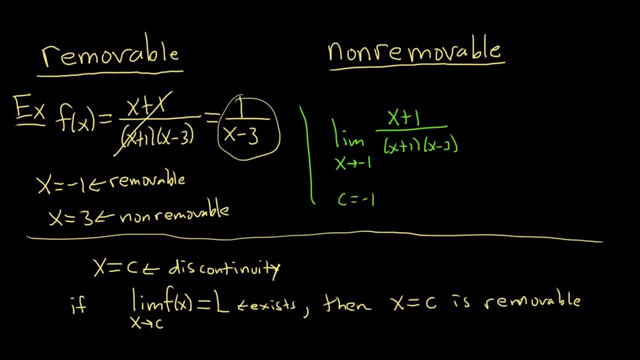 That's our f of x. Our c is negative, 1, right, And we're claiming that if the limit exists, then it's removable. Well, let's see. Well, what can you do? Oh well, you can cancel. 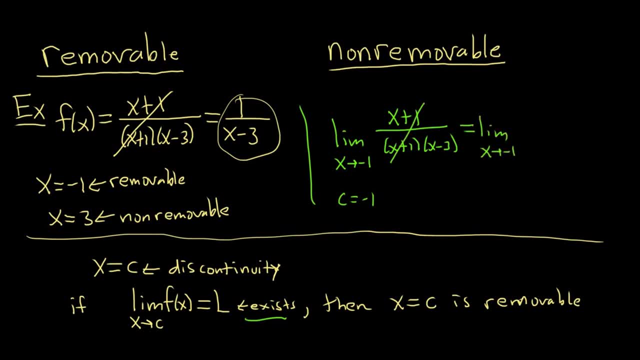 So we removed it right, using our powers, our superpowers of mathematics and calculus. And now you can evaluate this limit right. So you plug in negative 1.. You drop the limit sign, So you get negative 1 minus 3.. 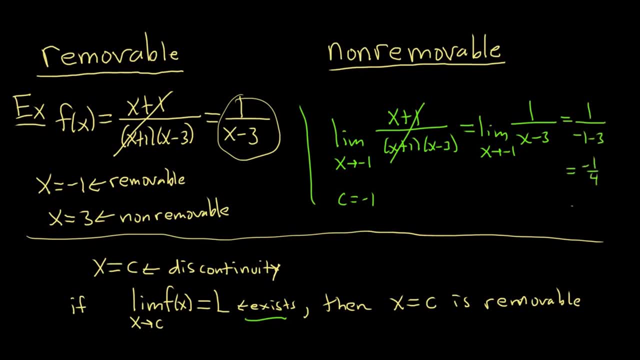 So you just get negative 1 over 4.. So the limit exists because it's equal to a number. Therefore it's removable, which we already knew via intuition, because we canceled it and we removed it. Hence it's a removable discontinuity. 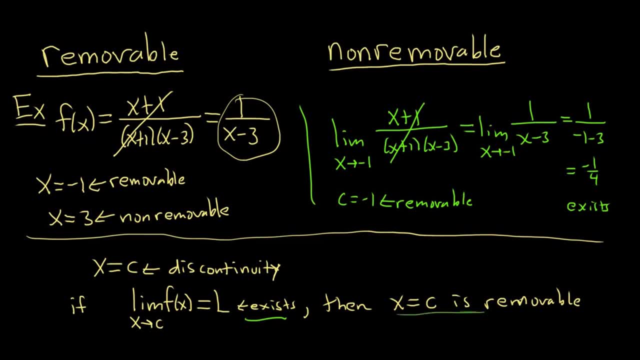 So this is a discontinuity. This is a nice criterion. It works both ways. If it's removable, the limit exists. Likewise, if the limit does not exist, it's not removable. So it does work both ways. However, in practice, you don't use it too often. 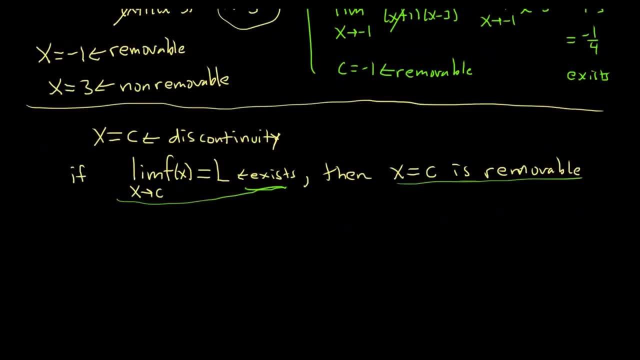 I mean, you do use it and it does work both ways. So let me write it down a little more formally. We're going to say that this limit exists if and only if. So if and only if, x equals c is removable. 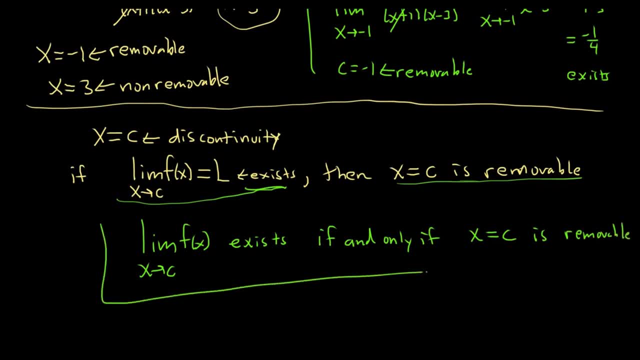 So this is something that we'll use for the harder problems involving removable and not removable discontinuities. So the limit will exist if, and only if, x equals c is removable. So what does that mean? That means if the limit exists, it's removable. 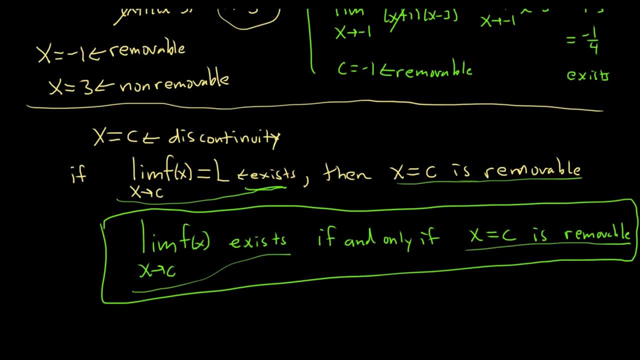 If it's removable, the limit exists. It also goes both ways and the other way. So if the limit does not exist, it's not removable. So not exist, not removable. I won't write that down, but really, really useful. 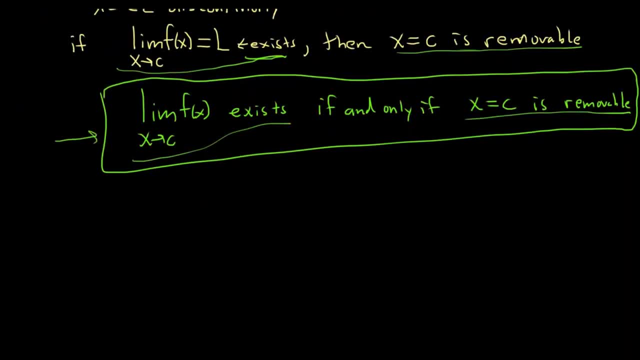 All right. So for all practical purposes again, we typically avoid this. So let me just give you two general rules that will help you do most of the problems. So typically we'll only use this when we have, like some piecewise function or some absolute value function in the harder problems. 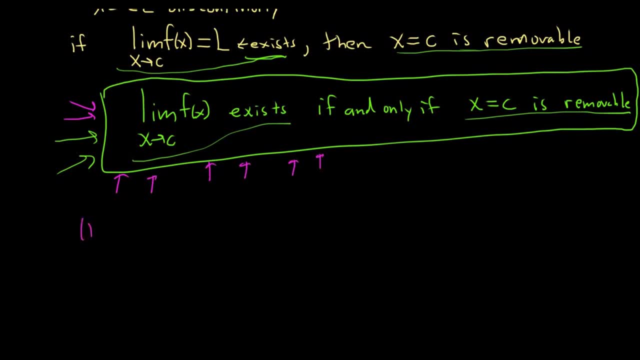 But most of the time we have these two rules. So the first rule is the following: In rational functions- which is the example we had above- polynomial over polynomial holes. so if you have a hole in the graph- and we'll talk about that in a minute- 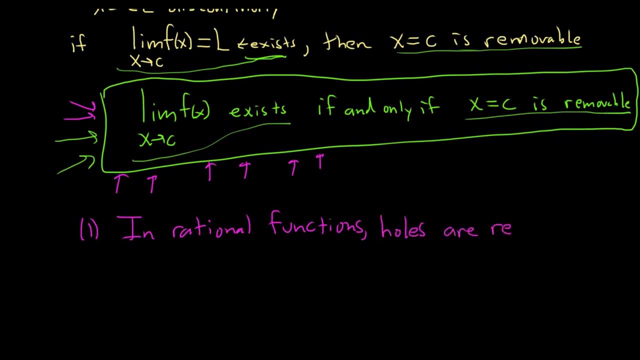 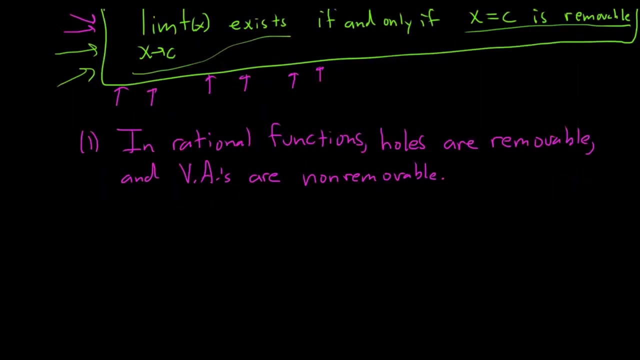 holes are removable- That's a lot of knowledge here- And VAs- vertical asymptotes- are non-removable. Okay, So in rational functions holes are removable and VAs are non-removable. So let's do a quick example here. 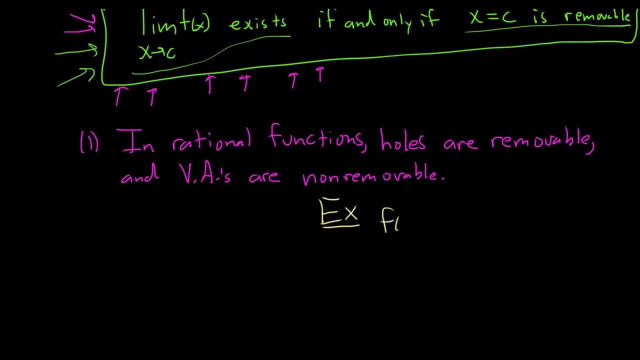 I'll make a new one up instead of using the one we just did. So if you have f of x equals x minus 3, x minus 3, x plus 7.. This is a rational function. It has two discontinuities. 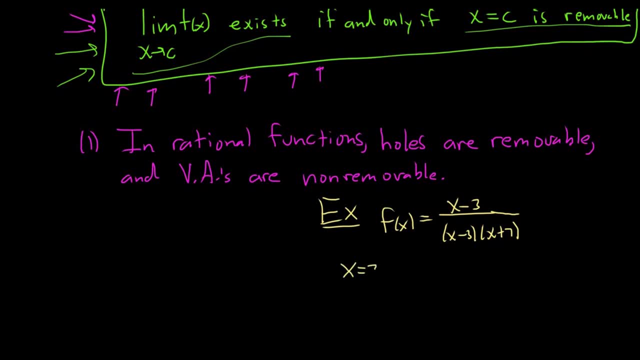 One of them is at 3, because if you plug 3 into the bottom, it's undefined. The other discontinuity is negative 7, because if you plug in negative 7 to the bottom, it's also undefined. So these are the discontinuities. 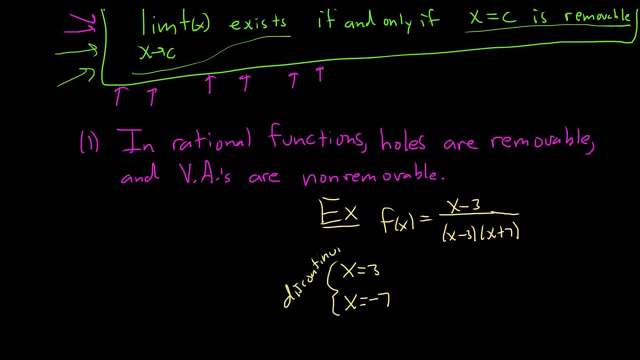 You just look to see what makes it undefined on the bottom to find the discontinuities, And then notice that you cancel this. So we've removed the discontinuity which you already knew, But this creates a hole. right, This creates a hole. 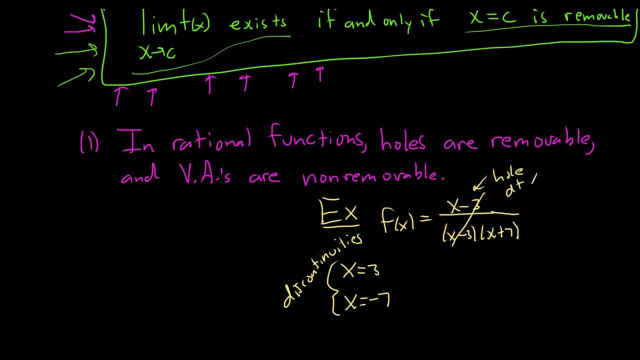 Whenever you have this cancellation, you have a hole at whatever makes this 0. So what makes x minus 3 0?? Well, 3.. So you have a hole there. So holes are always removable. So this is removable, Removable. 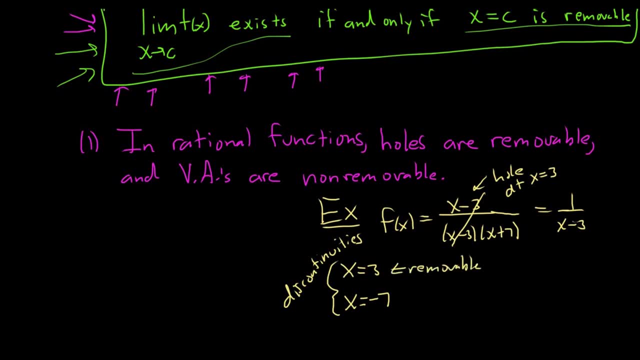 And here you have a vertical asymptote right. Oops, I messed up here. This is plus 7.. Whoops, Here you have a vertical asymptote right, And vertical asymptotes are always not removable, so not removable. So we kind of already knew this intuitively, because we talked about how the canceling is the removal process right. 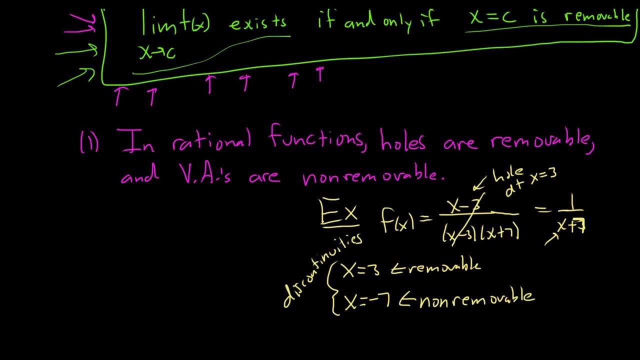 So even if you didn't know this, you kind of already knew it. It's just writing it down a different way. Two: in general, VAs are going to be non-removable. So VAs are non-removable in general. 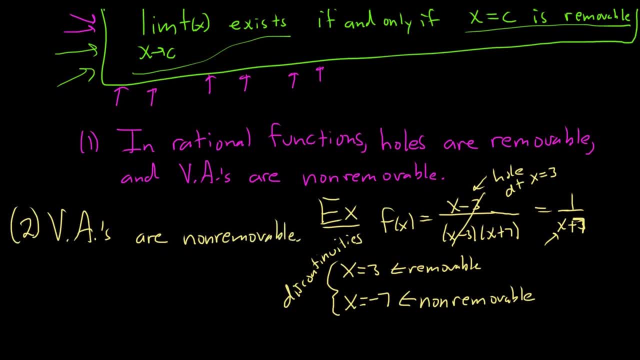 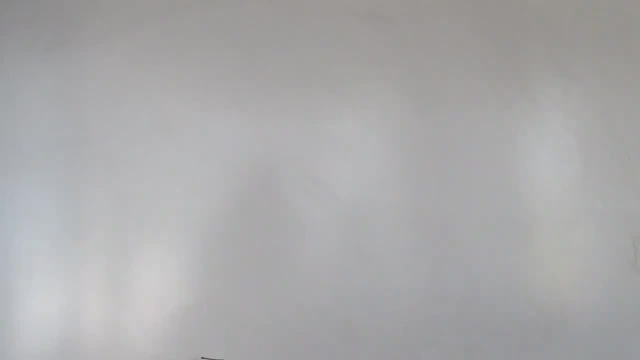 So this specifically also applies to, like trigonometric functions. If you have a trig function and you have a vertical asymptote, it's going to be non-removable. Hey everyone, In this video we're going to talk about what's called the intermediate value theorem from calculus. 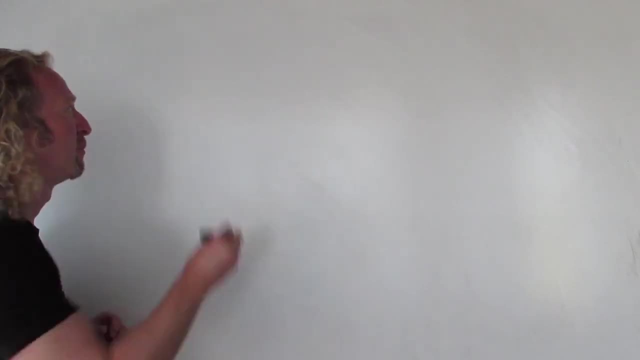 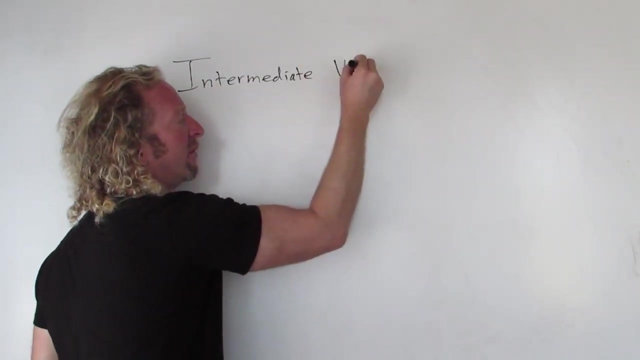 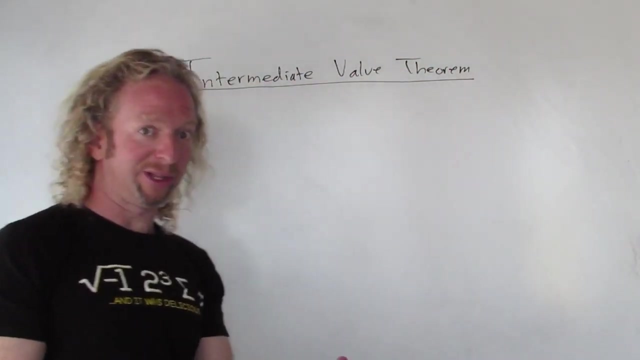 I'm going to go through the theorem and explain why it works and what it means and all that good stuff. So the intermediate value theorem is one of the big theorems in mathematics, especially in calculus. A theorem is something that's really, really important and has been proven. 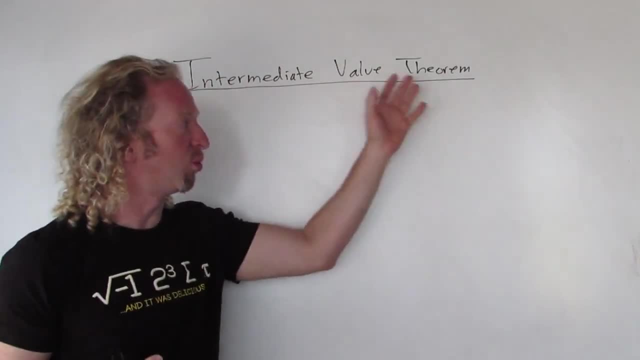 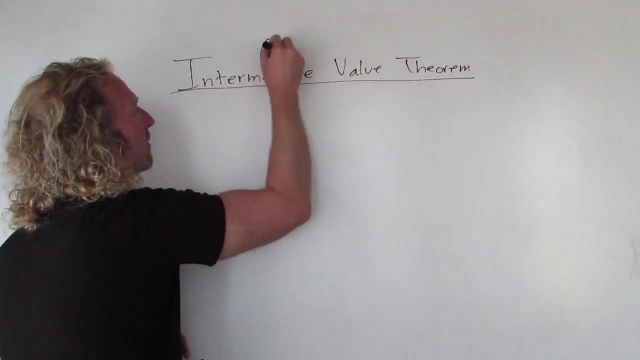 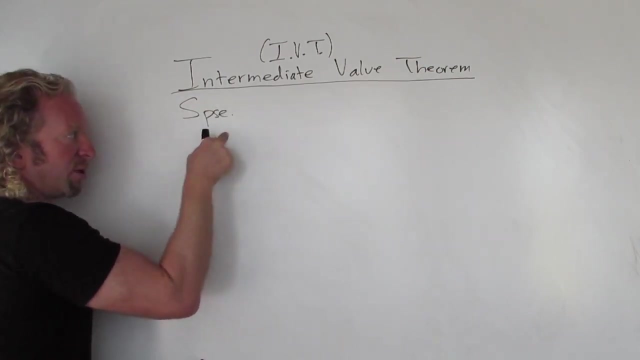 So the intermediate value theorem is one such theorem. It deserves the name theorem. We can abbreviate the intermediate value theorem by using three letters. We can just call it IVT. The intermediate value theorem says the following: It says: suppose I'll abbreviate, suppose just suppose. 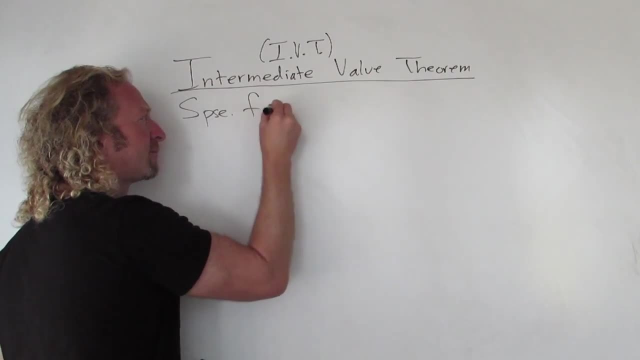 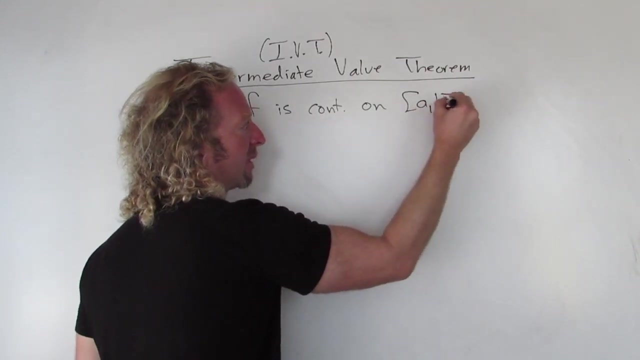 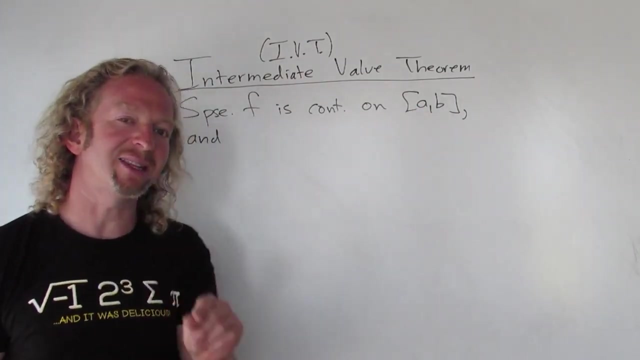 you have a continuous function on a closed interval, So F is continuous. I'll just put cont on the closed interval. A, comma, B And the values of the function at the endpoints are not the same, So F of A is not equal to F of B. 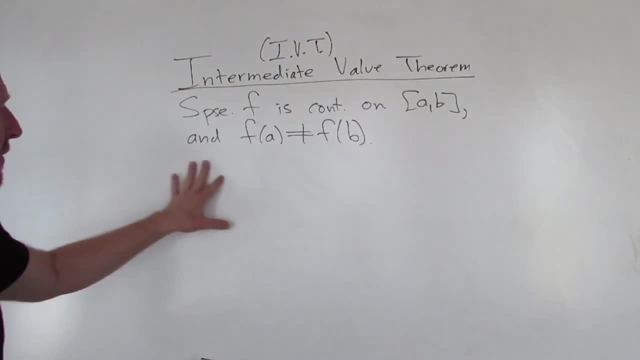 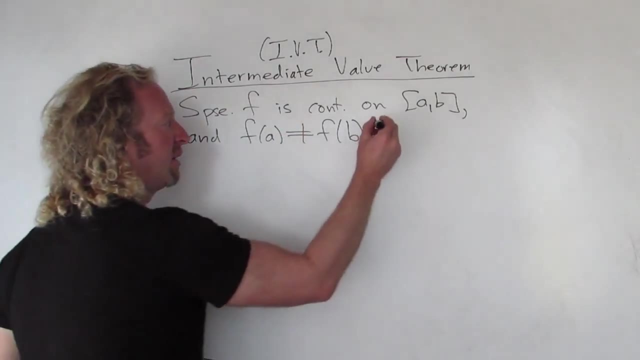 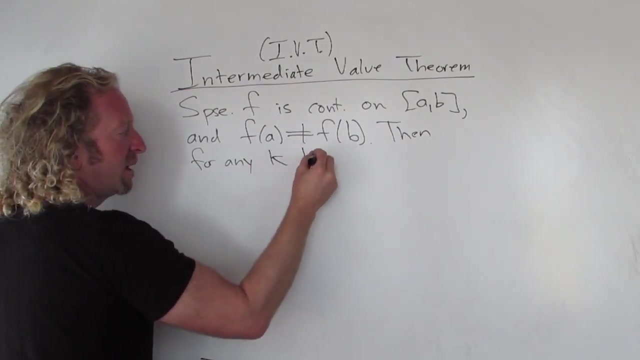 So those are the conditions. Those are the conditions for the intermediate value theorem. So if you have these two conditions, then for any number between these two, so then for any. I guess we can use K between F of A and F of B. 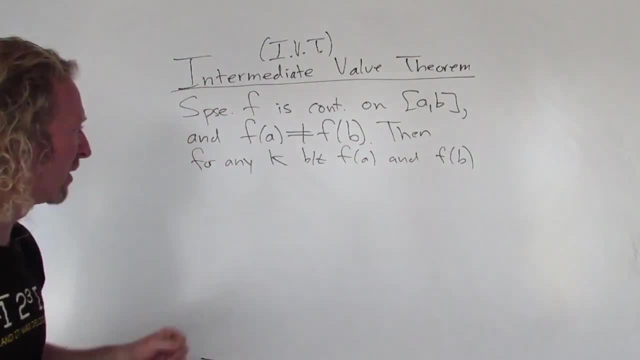 so we can assume F of A is less than F of B when we're talking about this. So for any K between these numbers it doesn't really matter. I guess This could be negative 4,. this could be negative 10.. 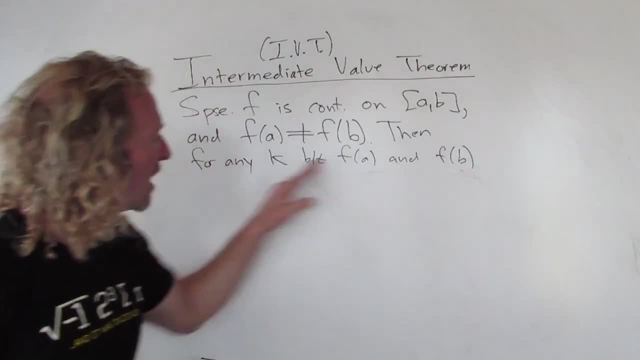 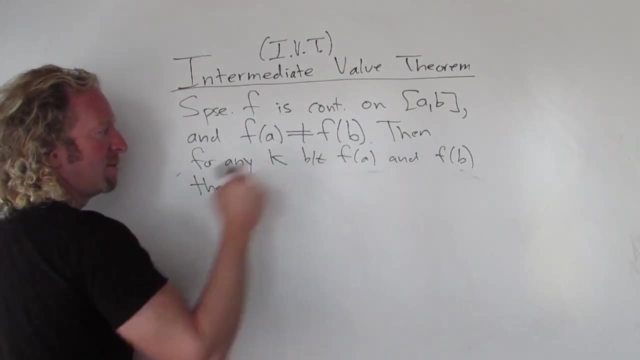 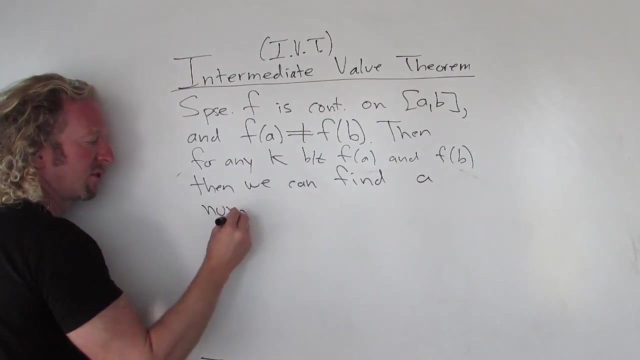 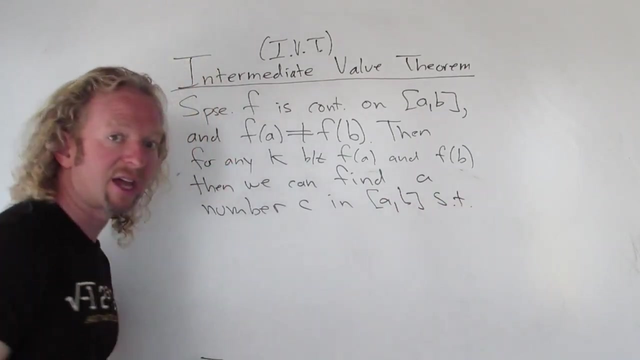 So any number between those two. So whenever you have a number between F of A and F of B, so for any K, then we can find. so, then for any K between these, then we can find A number C and A, B, such that ST means such that. 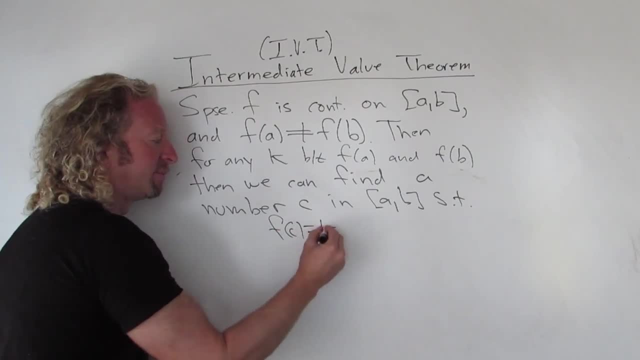 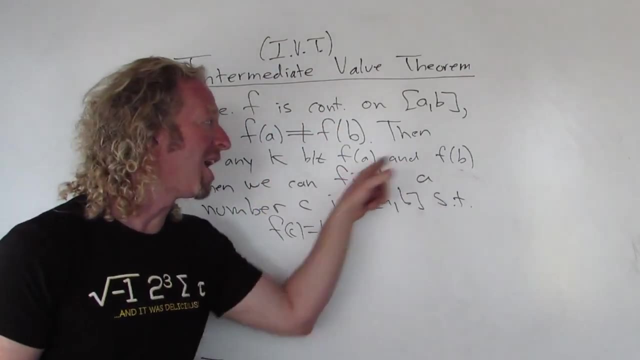 F takes C and sends it to A. So, given the continuous function on a closed interval where the values of the endpoints are not the same, if you take any Y value between these two right you can find the number C in the interval, such that F of C is equal to K. 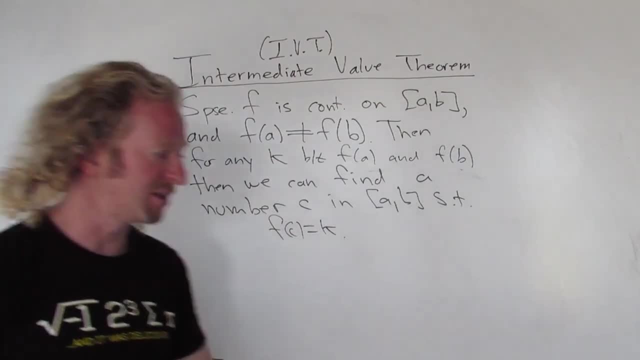 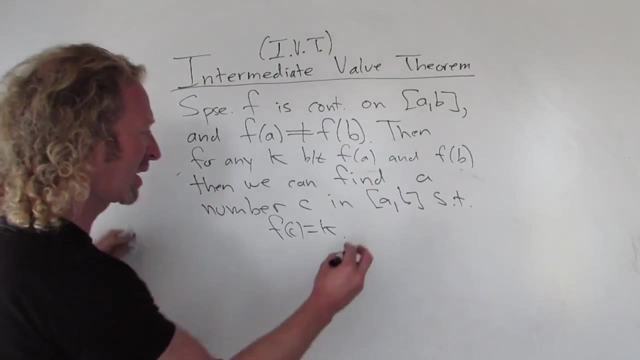 Let me show you what that means, like graphically. It's actually really, really simple. Just looking at a picture will make a lot more sense. So let me- I guess I can do it here. I'll do it here, then I'll do it again. 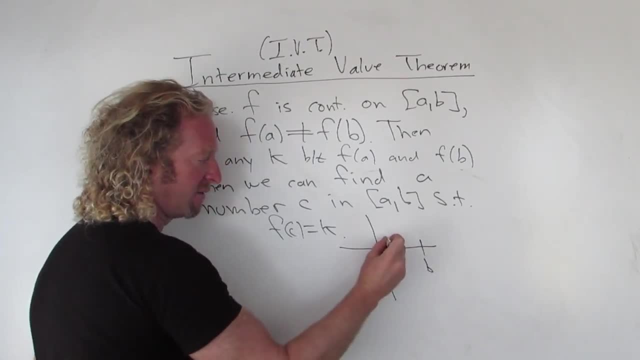 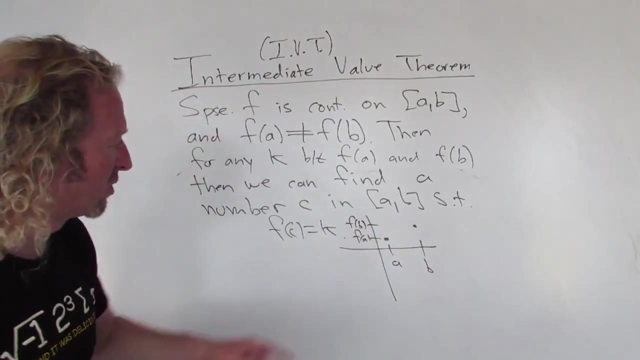 So let's say here's A and then here's B, And then let's say: this is F of A And this here would be F of B. Okay, F of B, Okay. so F of A is not equal to F of B in this picture. 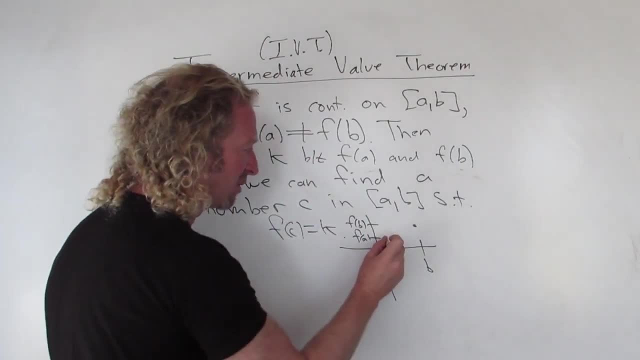 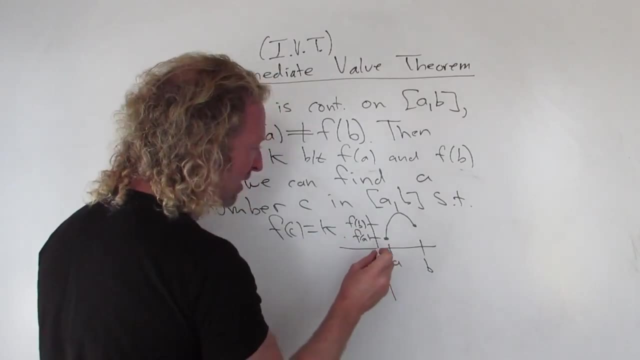 Now this function is continuous, so I have to connect the dots, so I'll just do this, Okay, And I can't have any holes or breaks because it's a continuous function. What this is saying is: given any number between F of A and F of B, 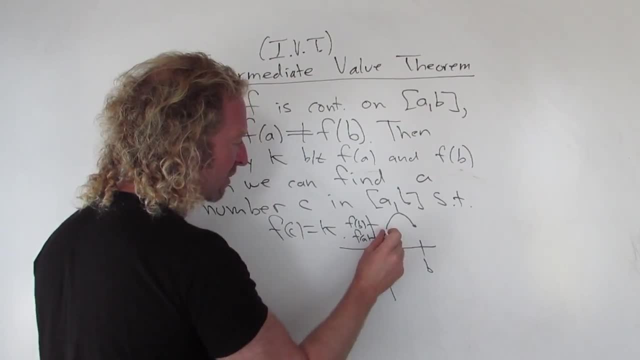 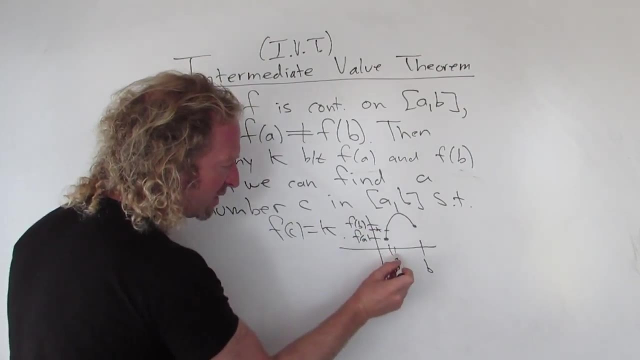 so, for example, say I pick this number here, Okay, that would be my K, That's a number between F of A and F of B, That there is a value of C, such that F of C is equal to K. Well, obviously right, you can just take that value there. 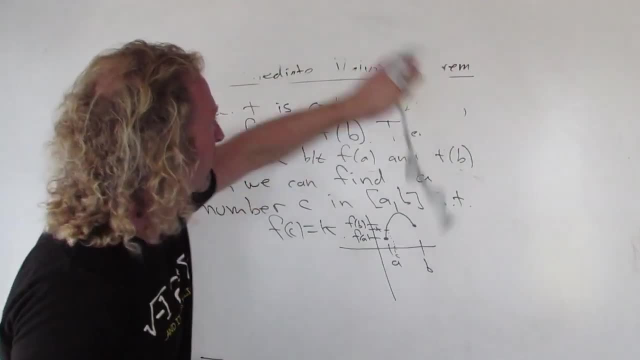 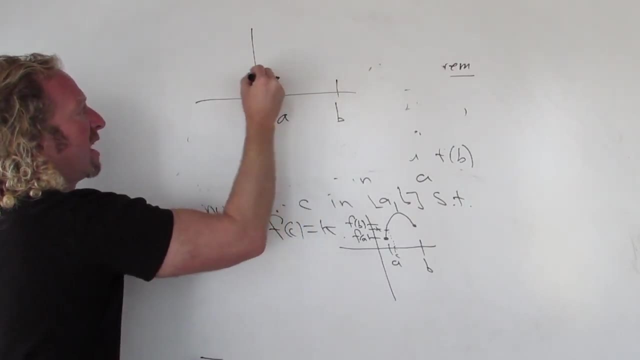 Let me do a bigger picture so you can see it a little bit better, so it makes a little more sense. So let's draw it again up here. So here's A, Here's B And let's say here's F of A. 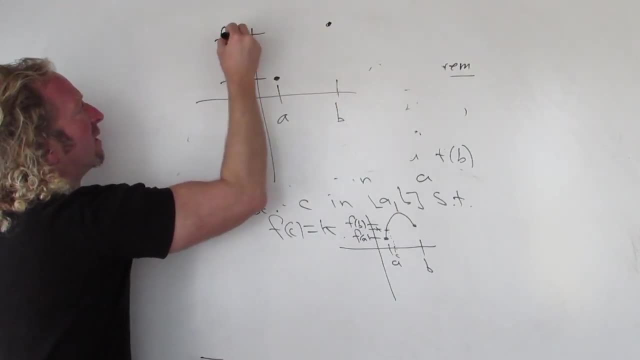 And then here's maybe way up here, it's F of B. So IBT says that for any number between F of A and F of B, so say the number here of K, you can find a value of C such that F of C is equal to K. 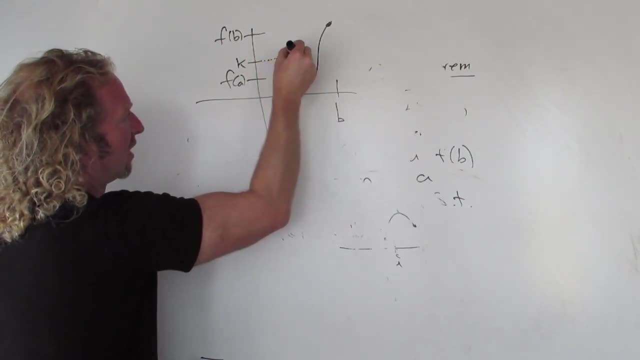 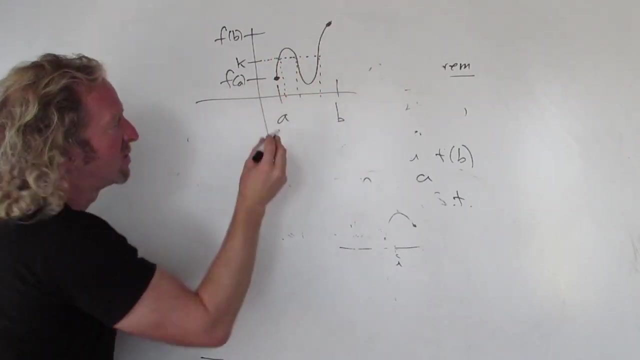 Well, in this case, here's K. So, K, K, K. So in this case, there's three values of C. right, There's three distinct values of C. I'll call them C1, C2, C3,. 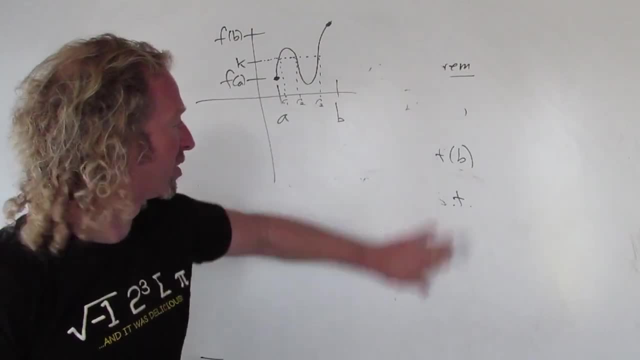 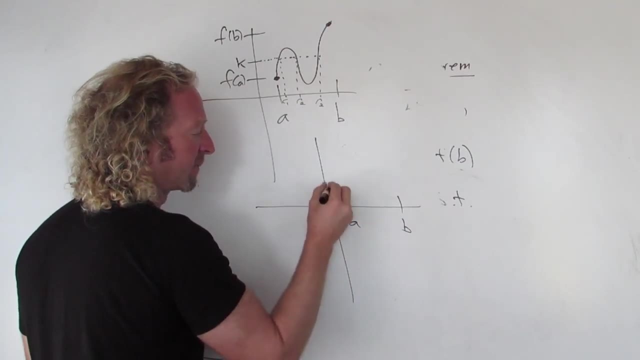 such that F of each of these values gives you K. Let's do another picture, just so you see it. So here's A, Here's B, Here's F. Let's see, Let's make this- that this is B. I guess I need a graph here. 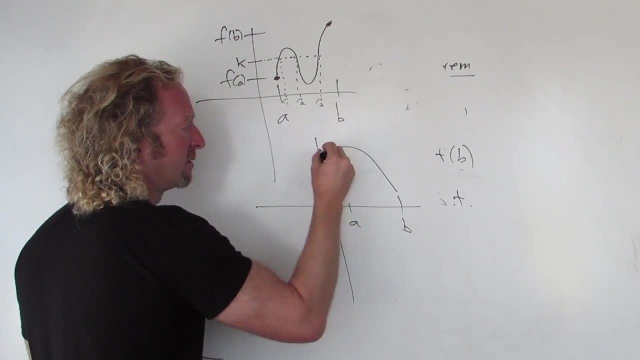 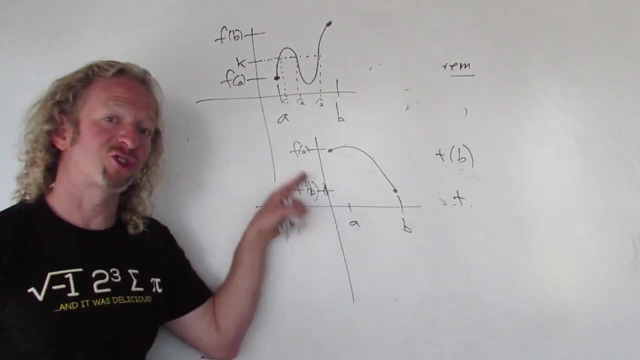 Let's do this. Let's make this F of A this time And let's make this F of B. So this time you see the case where F of B is smaller than F of A. right, Let's see if we can break the theorem. 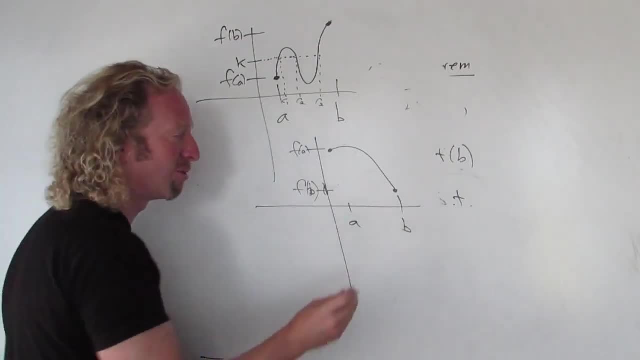 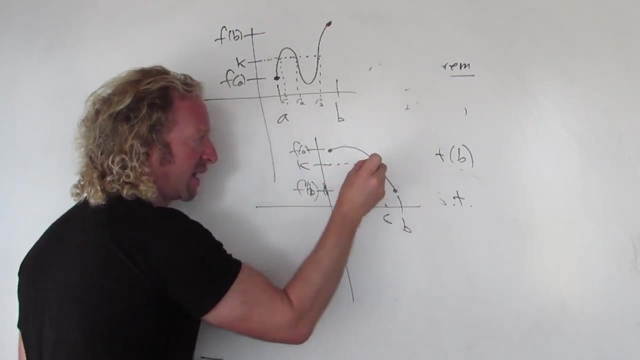 Well, we can't right, We can't break it because it's a theorem, right, It's true. So say, I pick a K here. Well, in this case, boom, there's our C. So F of C is equal to K. 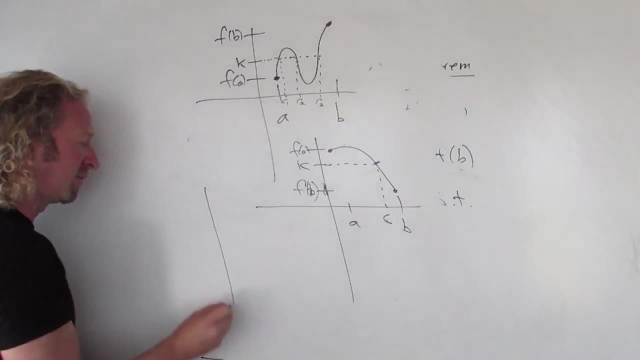 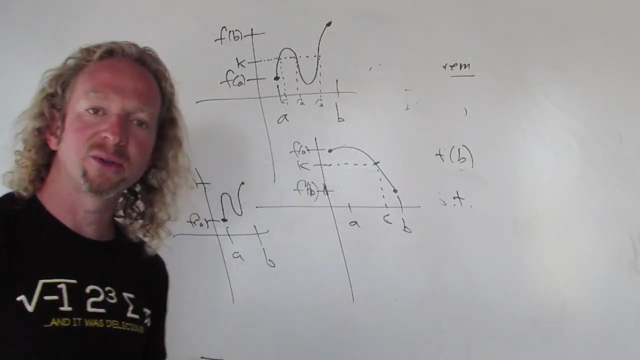 So it's called the intermediate value theorem. It's basically saying a function that's continuous on a closed interval takes on every intermediate value right between F of A and F of B. right It takes on all intermediate values between those numbers. 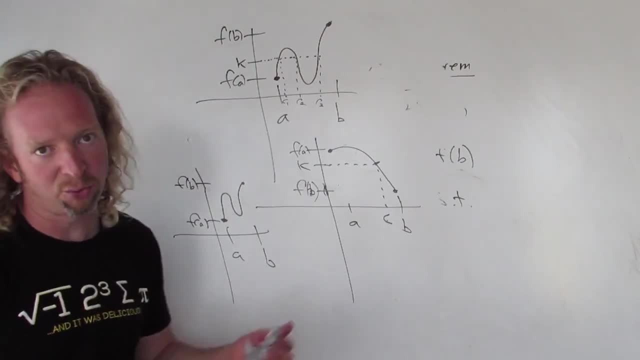 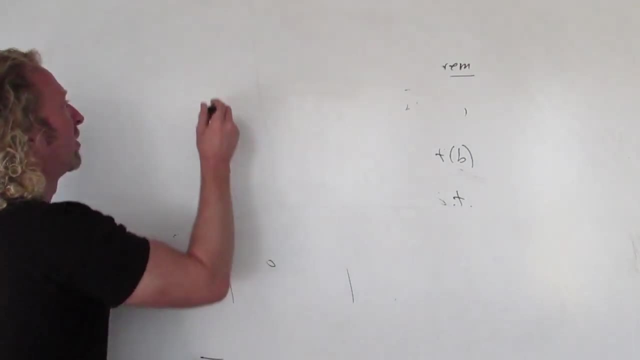 So the typical problem you would do in a math class with IBT is finding C. Let's do a simple example. I'll just make one up. So here we go. So let's say we have the function F of X equals X squared. 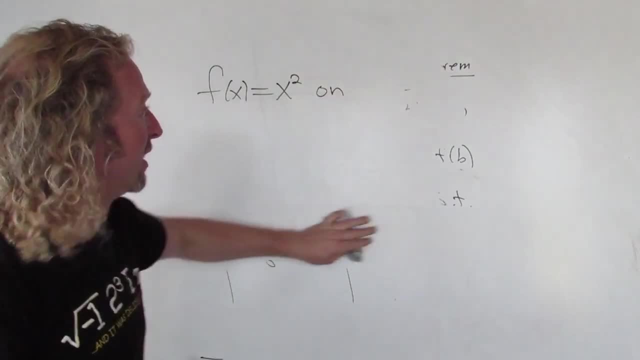 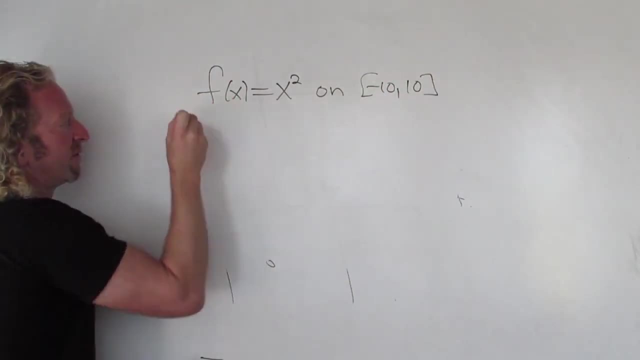 And we need an interval here. right, We need to give an interval. Let's do it on negative 10, 10.. It's continuous. And so find the value of C such that, well, given any value, any Y value. 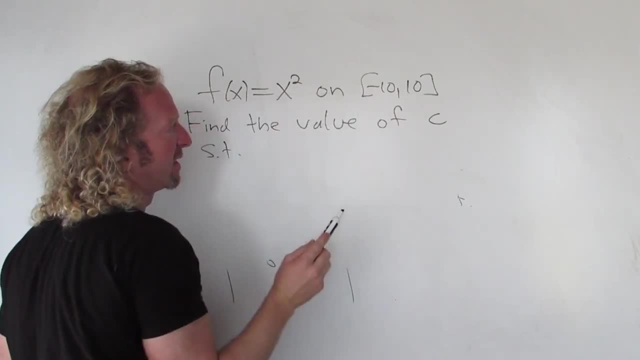 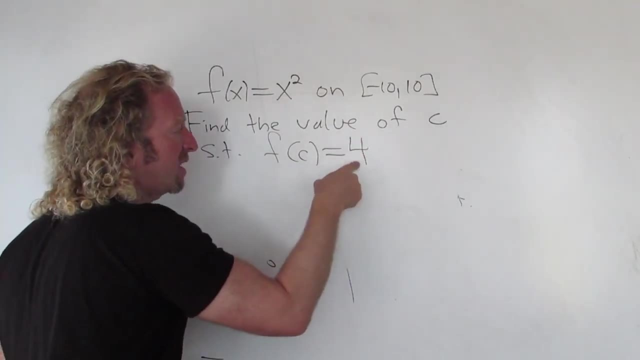 between F of negative 10 and F of 10,, we should be able to find C right, So such that F of C is equal to, let's say, 4.. That is the value between F of 10 and F of negative 10, right. 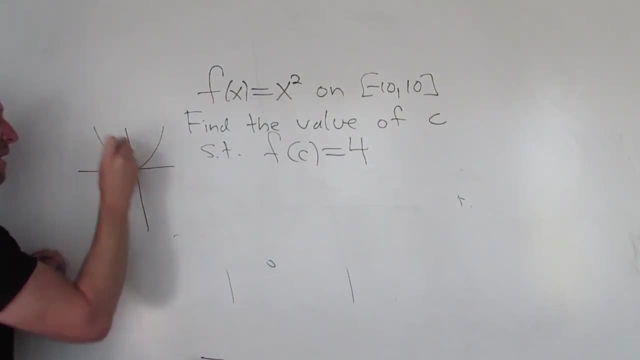 X squared is a parabola. It looks like this: If this is 10, then 10 squared is 100.. And this would be negative 10,. okay, So the value of 4, right, if you pick 4, 4 is not drawn to scale. 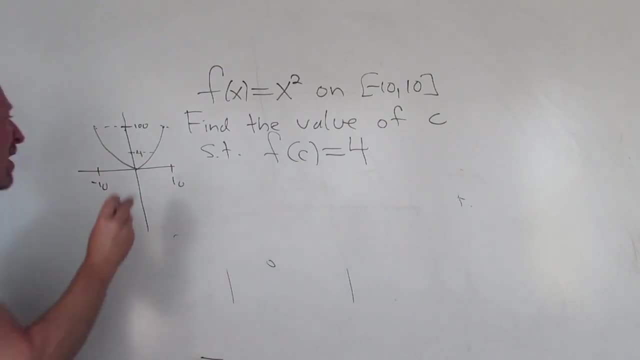 There's values of C, right? In fact, there's two values of C, such that F of those values is equal to 4, so C1 and C2.. Let's find those values. So how do you find these C values? 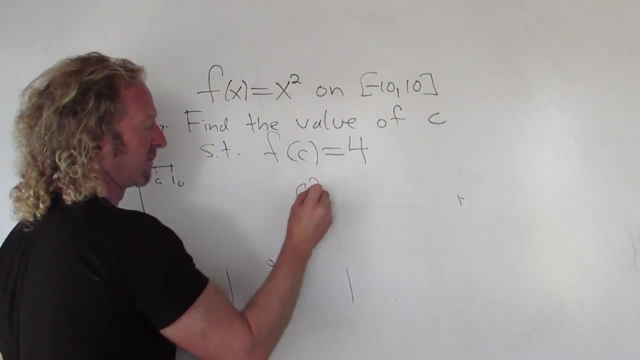 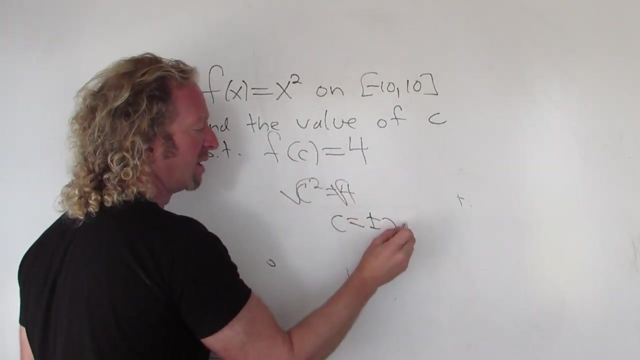 Well, all you have to do is plug in C for your X right, And then you just take the square root of both sides and you get C equals plus or minus 2. So these are the two values, such that F of those values gives you 4.. 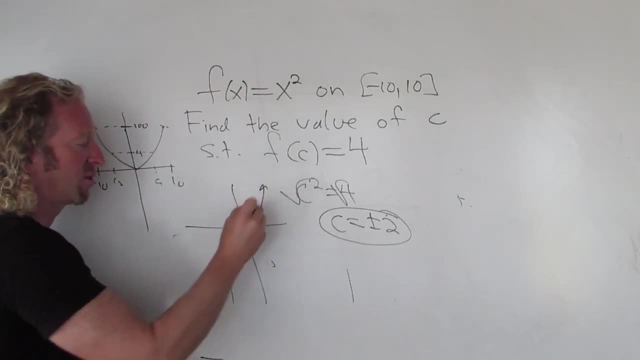 Let me do it again over here, so make sure you can see it. So here's X squared. Here's 10.. Here's negative 10.. That would mean that this is 100, okay, So we're cutting off the picture right there. 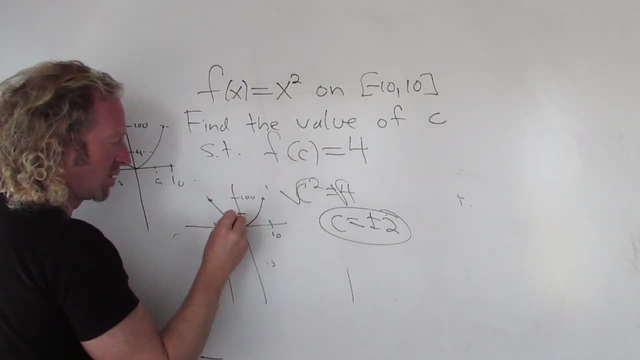 And the question is: given the number 4, again, this is not drawn to scale. what are the values of C that go to the number 4?? Well, there's two values, 2 and negative 2, right F of 2 is 4.. 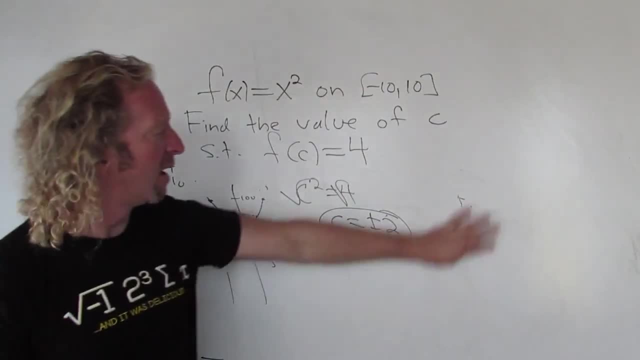 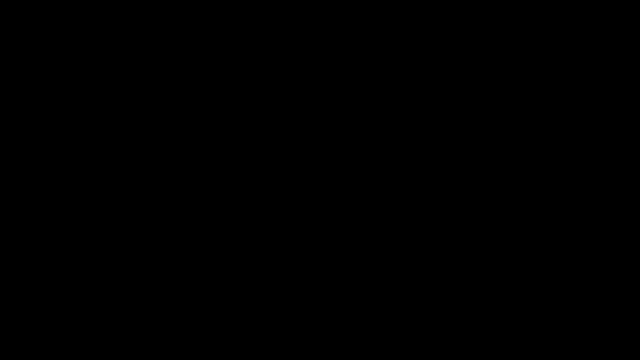 F of negative 2 is 4.. So that's the intermediate value theorem. I hope that made sense. Hi everyone. In this video we're going to discuss the notion of what's called infinite limits, So sometimes we'll write stuff like this: 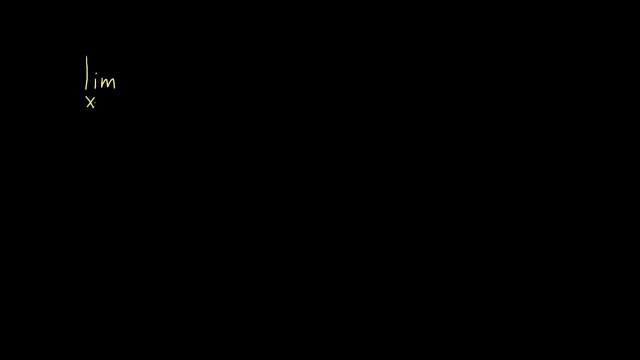 So limit X approaches C of F of X and we'll write the infinity symbol here. So in this case the limit does not exist. Recall that a limit will exist only if it's equal to a number. So what does this mean? 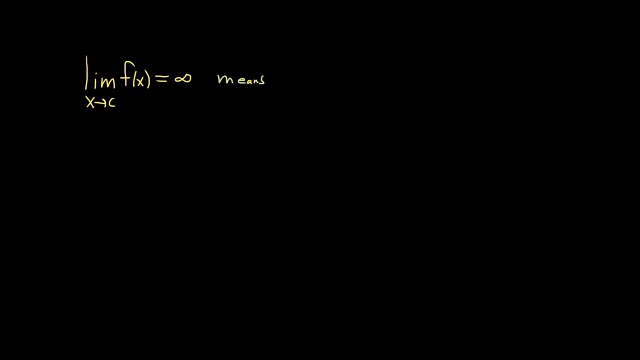 So this means that F of X. well, how would you read it? You would say: the limit of F of X as X approaches C is infinity. So as X approaches C, F of X approaches infinity. So that means that F of X grows without bound. 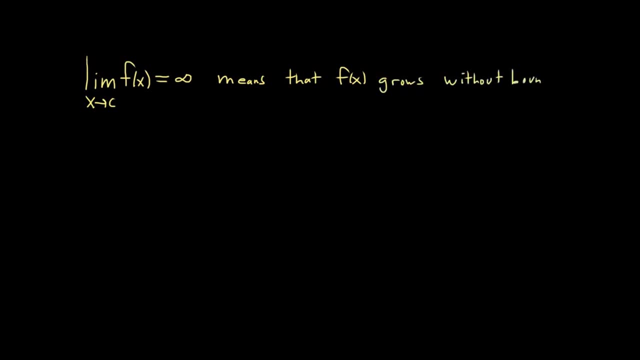 So, in other words, it gets really really big. So how big, Actually, as big as you want it to be. So F of X just goes up forever. It just gets really really big, So as X approaches C. So that's what that means. 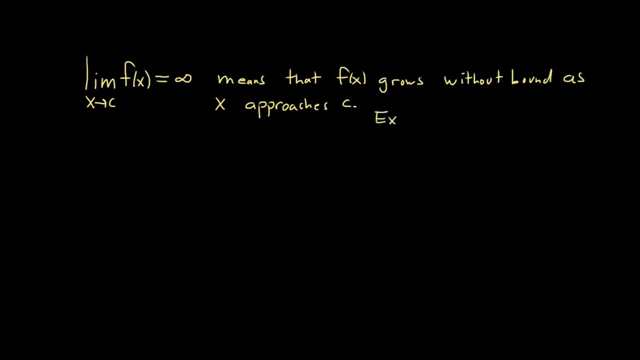 So here's a quick picture. So you see an example of this. Say, we have the y-axis and we have the x-axis, So this is X, this is Y, And so our graph here I'll draw it over here- Here is 1,, 2,, 3.. 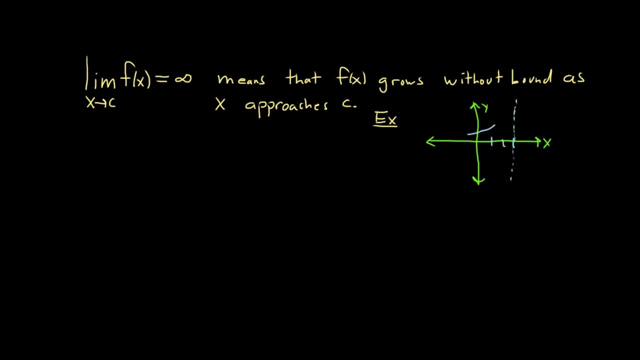 We have a vertical asymptote here And our function does this. It just goes up like this, And then it goes up like this, And this is the graph of F of X. So in this case, if we take the limit of F of X as X approaches 3,. 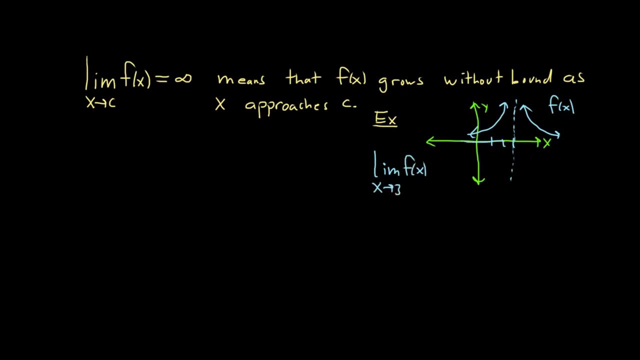 well, if you approach from the left, it goes up forever, so you get infinity. If you approach 3 from the right, you also get infinity. So from the left you get infinity, From the right you get infinity. So the answer is infinity. 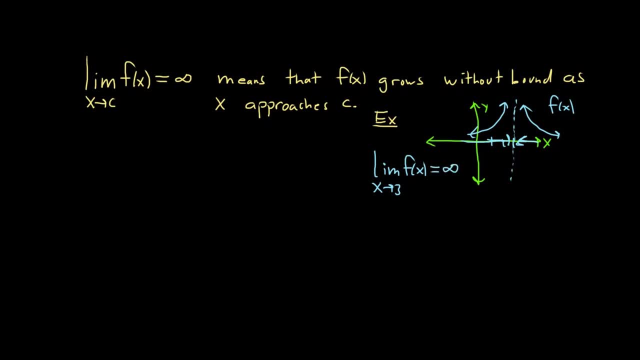 Now, it doesn't mean that the limit exists. The limit still does not exist, But this is a more descriptive answer. right, This is descriptive. It tells us what's happening to the function when X gets close to 3.. So it's better than just putting D and E. 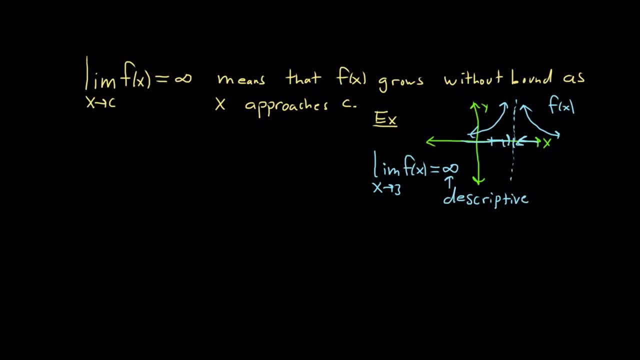 You can also clearly replace the 3 with one-sided limits and the results are the same. So in fact, you could write: X approaches 3 from the left is equal to infinity, And you can also write: limit: X approaches 3 from the right equals infinity. 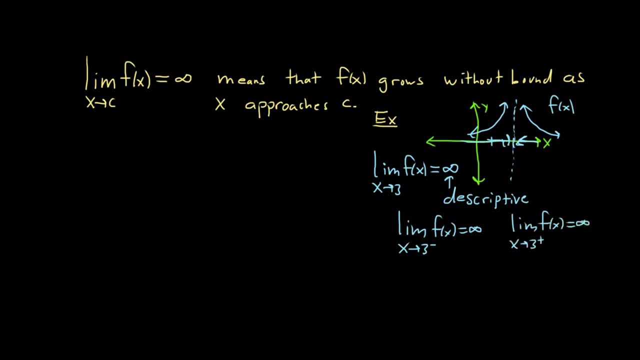 So both of these are acceptable as well. Likewise, we can do the same thing for negative infinity. If we write: limit X approaches C of F of X equals negative infinity. so this means this time it goes down forever. right, The graph will just go down forever. 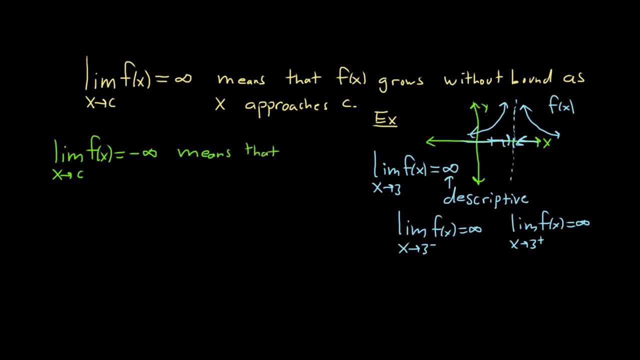 So this means that F of X decreases without bound. So decreases without bound as X approaches C. So as X approaches C, So it gets smaller forever. Let's look at a picture. Why not? Let's do it. It's kind of interesting. 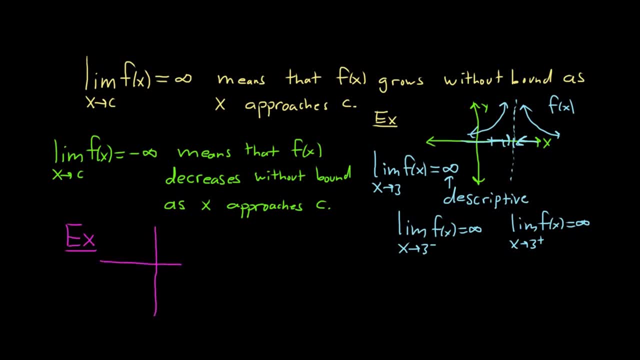 So here's an example. So here is the Y-axis, Here is the X-axis, And let's just take the example we had, but I'll move the asymptote to 2.. So here's our vertical asymptote. Let's make it go down this time, right. 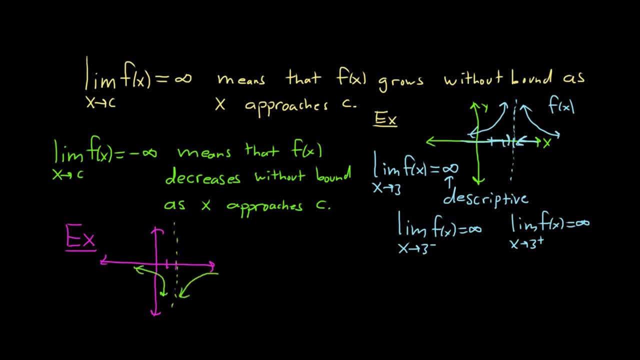 So now it goes down. So in this case, when we take the limit as X approaches 2 of F of X- let's say this is the graph of F of X- we get negative infinity right And from the left it's negative. 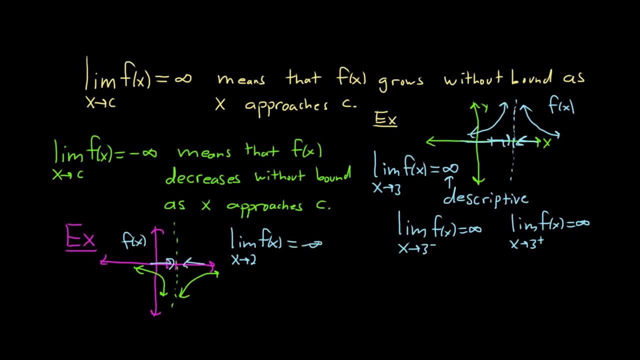 So from the left it's negative infinity, From the right it's negative infinity. Therefore, in general, it's negative infinity. So that's graphically what these limits mean. These are called infinite limits. Let's do a couple simple examples. 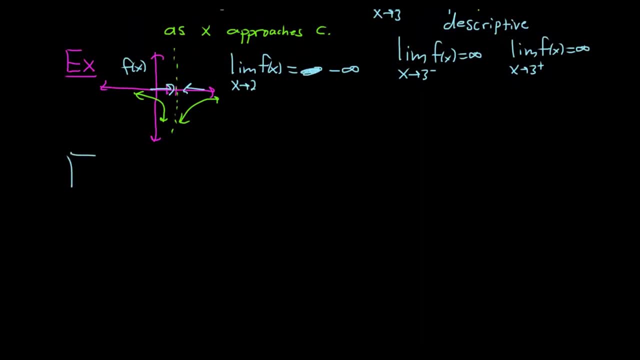 just maybe one or two, where we try to compute some of these without a graph, And this takes a little bit of practice. So in the examples that follow you'll have more examples of this. Let's approach 4 from the left of 1 over X minus 4.. 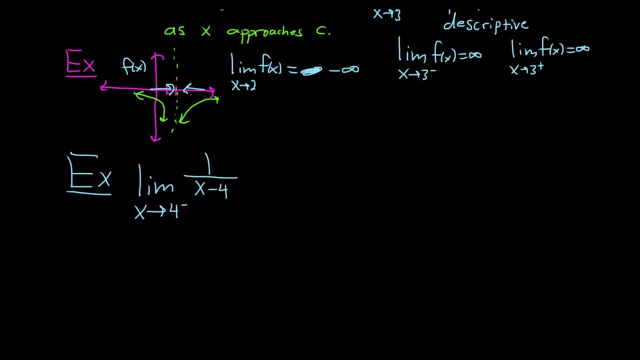 Let's think about this. So there's no real way to algebraically show the work here, So there's no real correct way of doing this other than using the definition, like with epsilon and n, which I didn't write, So it's a lot harder. 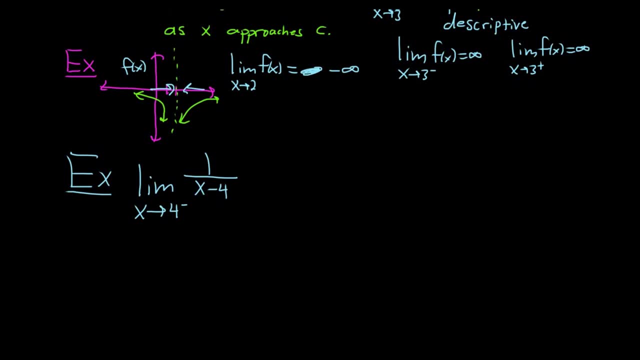 Typically you don't have to do that in a Calculus I course, Maybe Advanced Calculus, but not Calc I. So how do you do it? Well, you could draw a picture or you could use intuition. Let's do it using intuition. 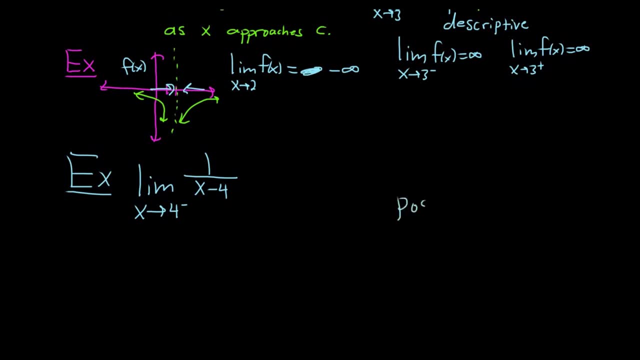 So up top we have a number which is 1.. So we have a positive number. What's happening on the bottom? Let me draw a little picture. So here's 4, and X is over here because it's approaching from the left. 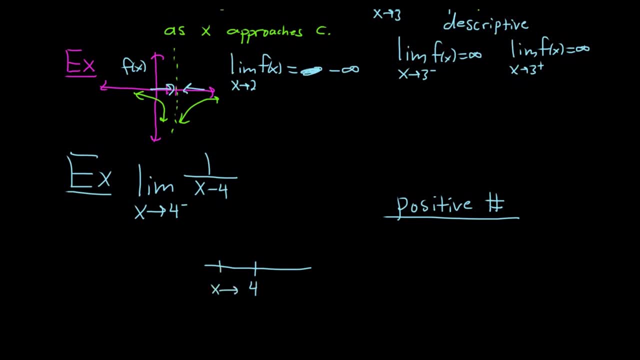 So it's getting really close to 4. from the left It's getting infinitely close to 4.. So pick a number less than 4 that's close to 4, like 3.99.. So if you do 1 over 3.99 minus 1,, 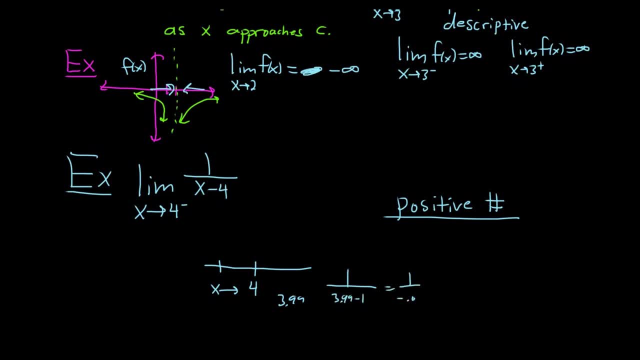 you get 1 over negative 0.01.. So as you get closer and closer to 4, you get a negative number here, and then this number here is really small. So you get something negative and you get something super small. 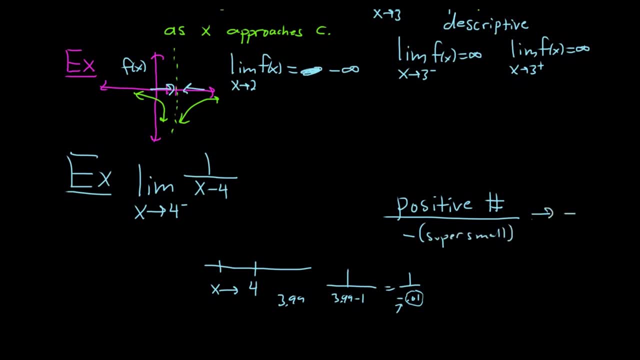 And I'm going to claim that this is going to approach negative infinity. So how do I do that? Well, if you have 1 over something small, that's big. Consider like 1 over 0.1.. 1 over 0.1 is 10.. 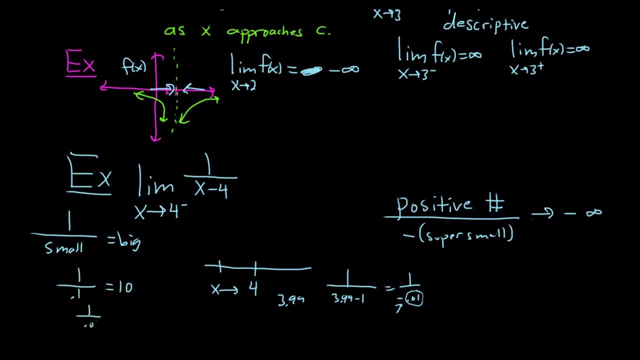 If you put it in your calculator you'll get 10.. 1 over 0.01 is 100.. 1 over 0.001 is 1,000.. So you see it gets out of hand really quick. So the smaller the bottom is, the bigger the fraction. 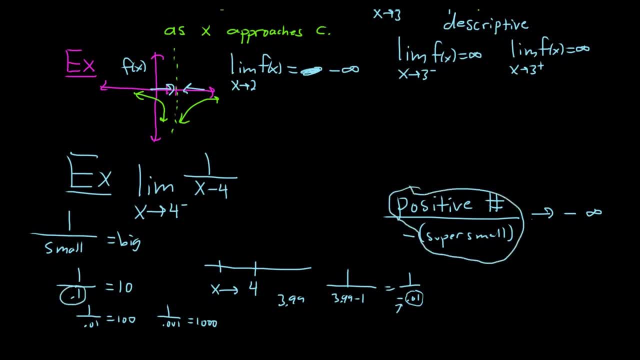 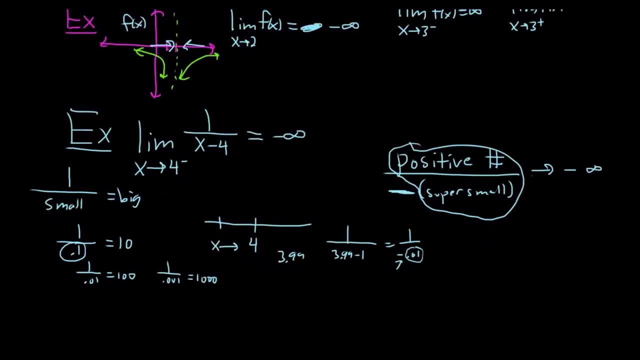 So this is super big Right, But then we have a negative here That's going to make it go to negative infinity. So the answer is negative infinity. Let's do one more. Let's do one more. This is a tough, tough concept for people to grasp. 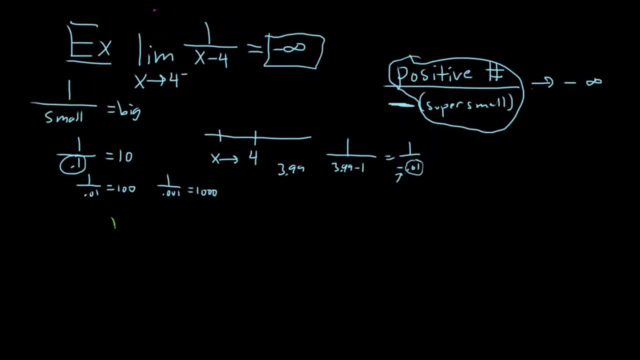 Sometimes people get it right away and then sometimes people don't. That's how it is in math, right? Some topics are easier than others for certain people. Let's approach 2 from the right and let's keep it simple again. 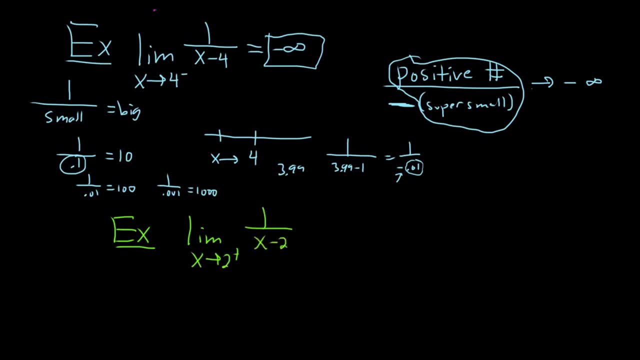 1 over x minus 2.. So again up top, we have a positive number- This is actually an easier example- And on the bottom we're approaching 2.. So here's a picture, Here's 2.. And we're approaching from the right. 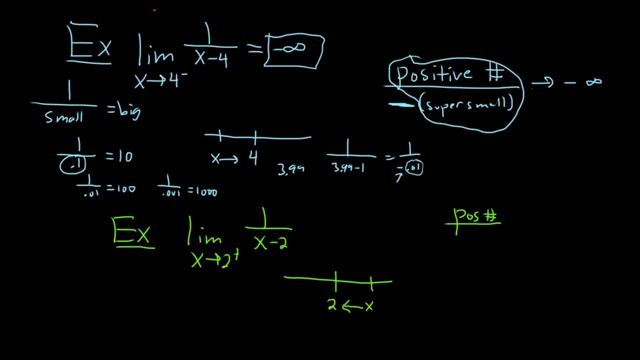 So here's x, and we're coming from this way. So think of a number bigger than 2, like 2.01.. That's really close to 2.. So 2.01 minus 2. It's a positive number over 0.01.. 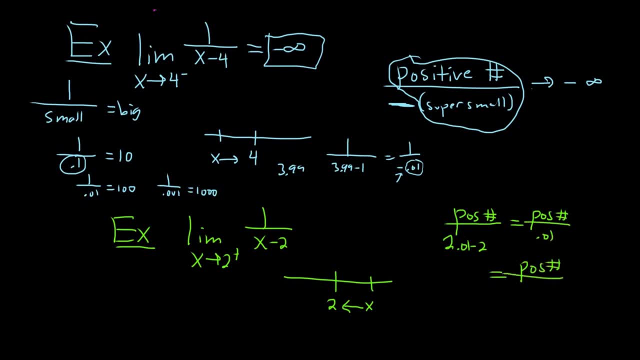 So that's a positive number over something small, super small. So that's big. So that should give us infinity. So you can just pick any number you like. I'm just pulling them out of thin air. That's what it seems like. 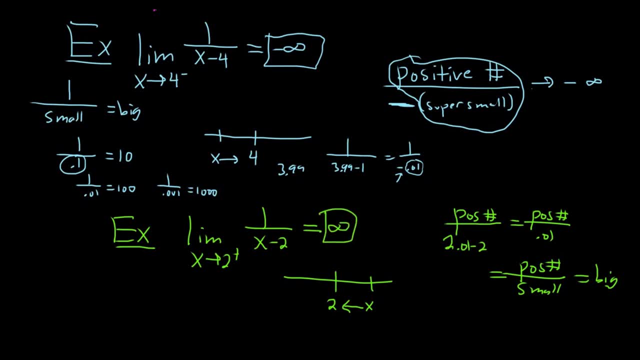 That's because I am. I'm picking numbers that are really close. You could have picked 2.0001 minus 2.. This is just a way to think about it. This is not really correct. The work here is not really correct. 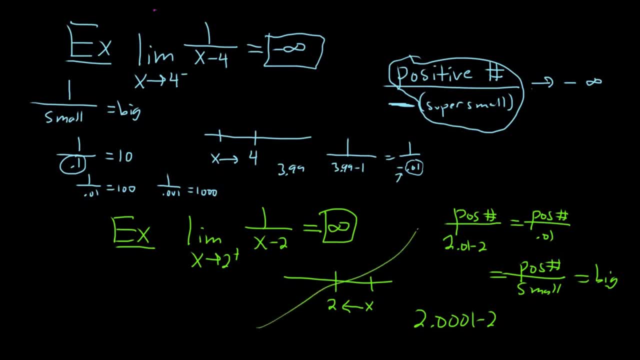 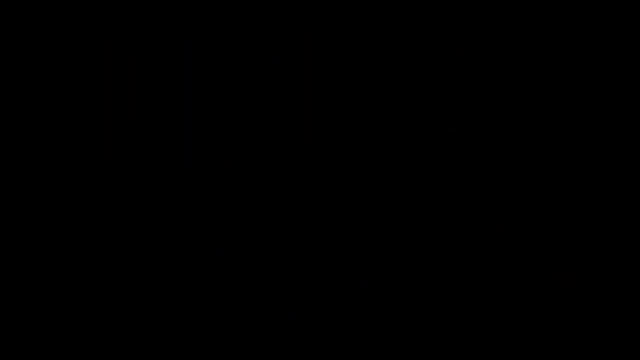 This is not correct mathematics. This is just us clarifying our thoughts Again. the only way to really show work here is to use like a proof. Hi everyone, In this video we're going to talk about vertical asymptotes. 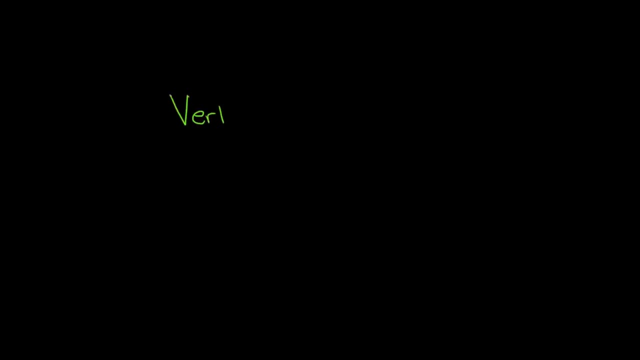 So vertical asymptotes. So a vertical asymptote is an invisible, infinite vertical dotted line that the function approaches. So, for example, say this is the y-axis and this is the x-axis, And then my line won't be invisible. 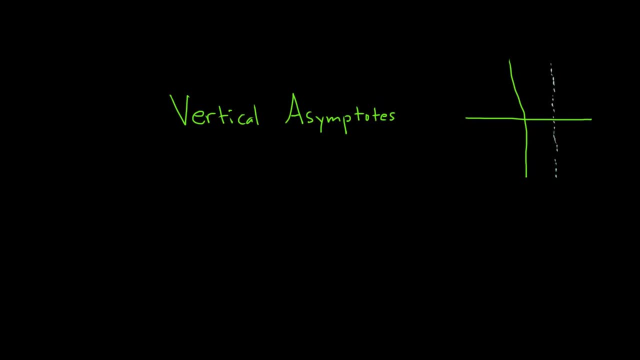 Because then you wouldn't be able to see it. So there is our vertical asymptote, And then maybe our function is here, So it approaches it like that. So the blue line is a vertical asymptote, or VA. So in calculus we define vertical asymptotes using limits. 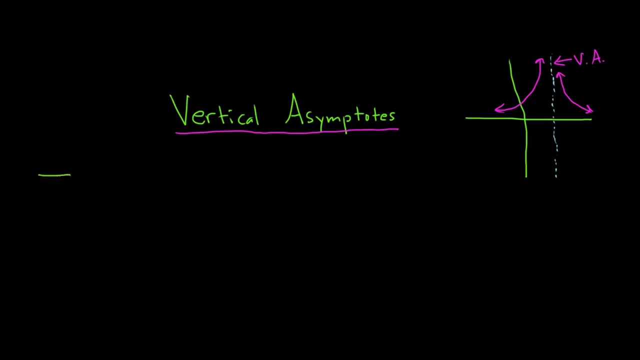 So here is the definition. So we say, if we take the limit as x approaches c of f of x and we get infinity or negative infinity- And by the way, here this can be a one-sided limit, So it can be one-sided. 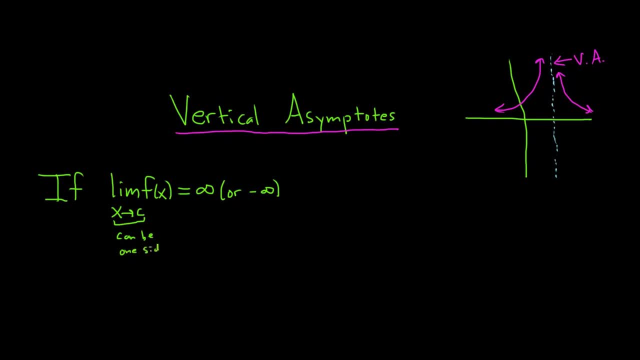 So maybe it just approaches from the left, And that's good enough, Or simply from the right. So if we take a limit from any direction, from the left or from the right, or just the regular limit, and we get infinity or negative infinity, 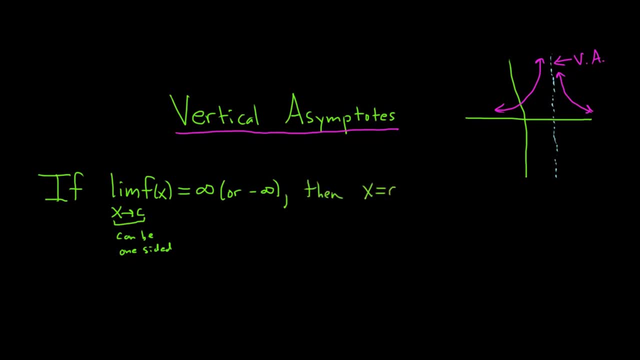 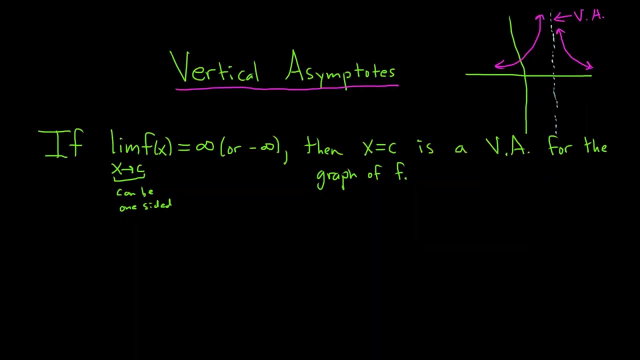 then x equals: c is a vertical asymptote, And I'm just going to say VA for the graph of f, So for the graph of f. So what a definition. The good news is, in practice we rarely use this definition. So let's just do a couple examples. 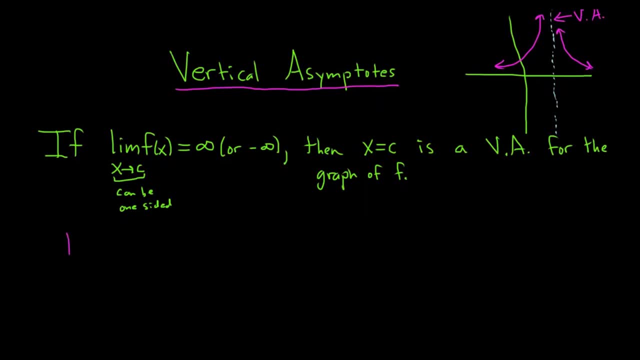 so you see how simple this actually is. So ex means example, And all of the questions will say the same thing. They'll all say: find the VAs, So find the vertical asymptotes. Okay, so A Let's do a really simple example. 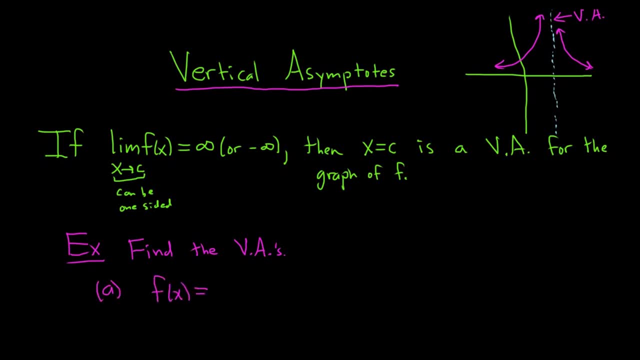 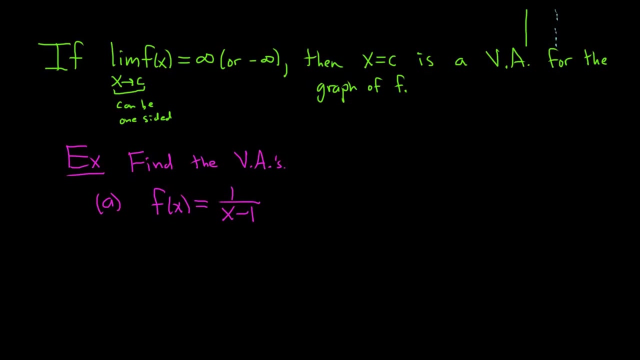 Let's do: f of x equals one over x minus one. So if you remember, from just regular math, I guess, algebra precalculus. whenever you have a rational function like this, when you're finding vertical asymptotes, what you do is you simplify first. 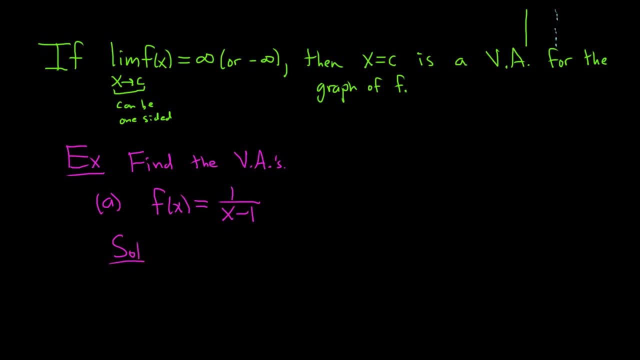 and then you set the bottom equal to zero. So all you do here is you simplify, You can't do anything, And then you set the bottom equal to zero, Then you solve for x, And so you get one, and that is the answer. 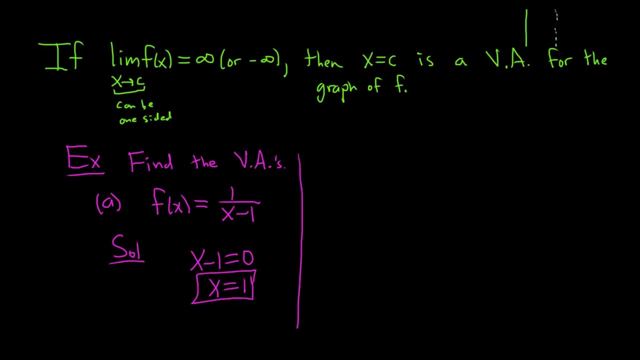 No calculus involved, okay, So let me write those steps down. So for rational functions, which is what we have right, Rational functions, That's a polynomial over a polynomial. Step one: simplify if possible. So simplify if possible. In this case it was not possible to simplify. 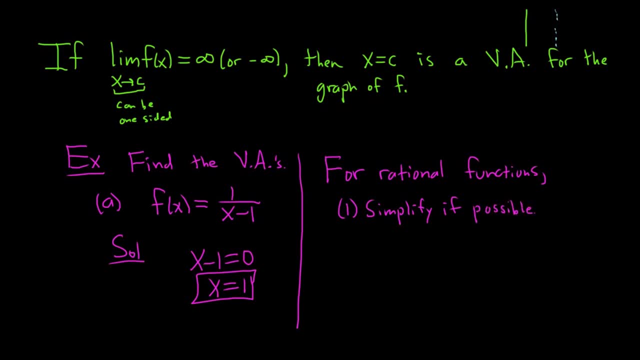 We were not able to Nothing canceled. If anything does cancel, it will give you a whole. So we'll talk about that in a minute when we do another example Two. set the bottom equal to zero. So I'll say set denom equal to zero. 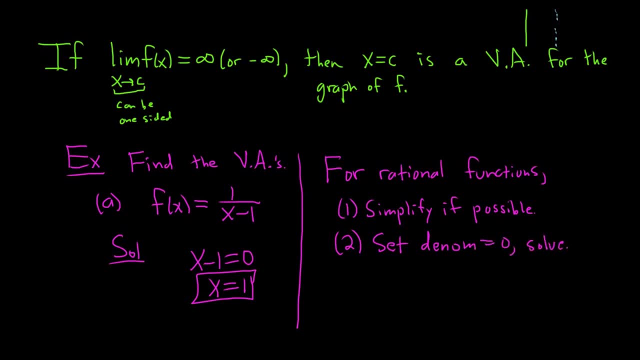 Solve Done right, No calculus involved. Now, what if you wanted to use calculus in this example? right, I mean, this is calculus, We're talking about calculus. So you would just take the limit as x approaches one. Now, if you take the limit as x approaches one, 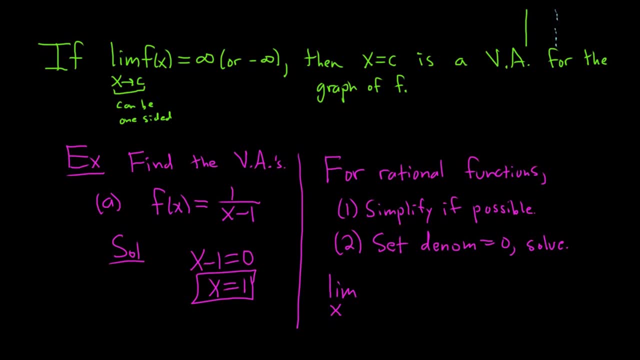 it's not going to exist, So you would have to use a one-sided limit. So let's like, approach one from the right just to show that it does have a vertical asymptote, right? So if you approach one from the right, 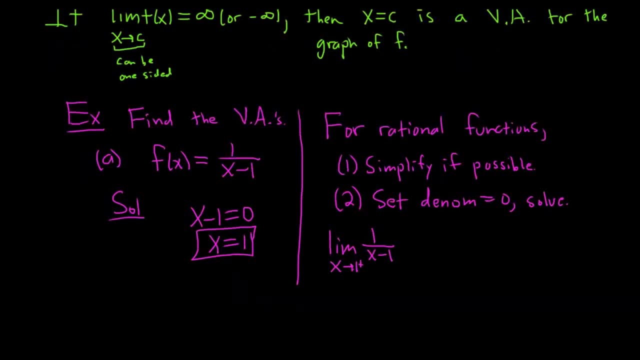 there's no real way to show the work here. So what you do is you think about what's going on. You have a positive number up top, so a positive number On the bottom, you're approaching one from the right, So here's one and here's x. 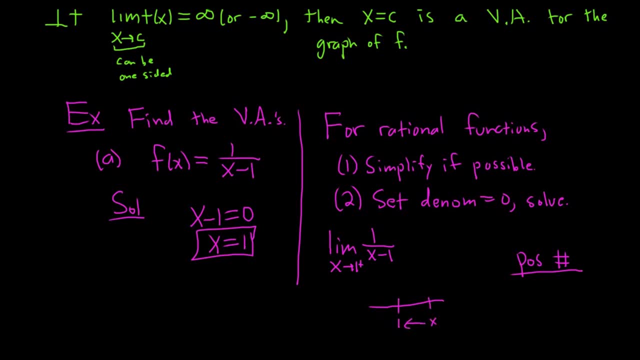 because you're approaching from the right. So it's this way. It's this way here. So think of a number that's slightly bigger than one, so like 1.01.. So you have like 1.01 minus 1, right. 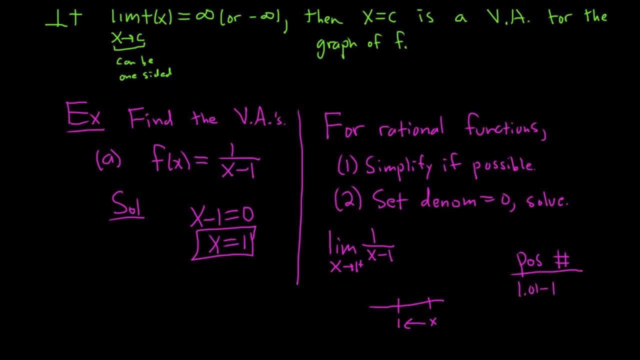 Because that's your x. Your x is 1.01.. Just plug in any number you like that's bigger than one and really close, So you get a positive number. POS number over 0.01.. So that's a positive number over something small. 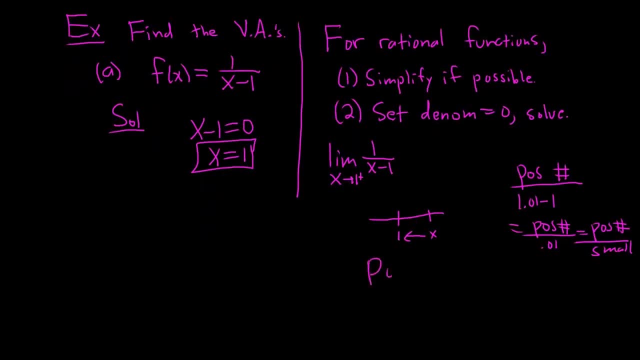 So if you have a positive number over something small, so you have a POS number over something small that's big. So this is infinity And therefore x equals 1 is a vertical asymptote. If you approach from the left you get negative infinity. 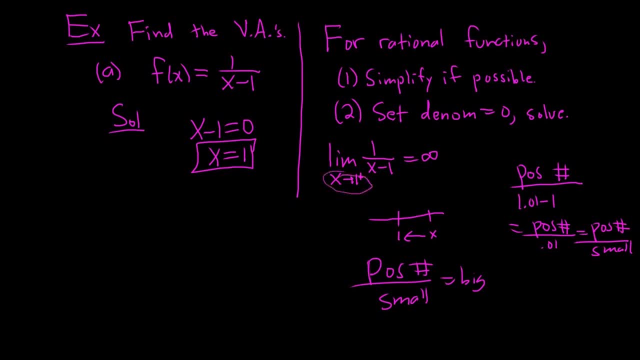 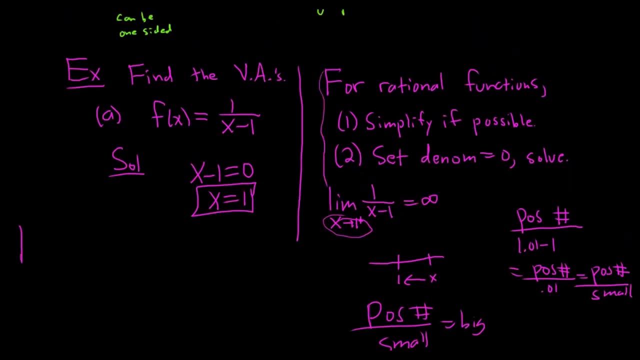 and the general limit will not exist. So I picked a one-sided limit just to make sure it would exist. But in general, you don't have to do any of this right. All you have to do is follow these steps. Let's do a better example. 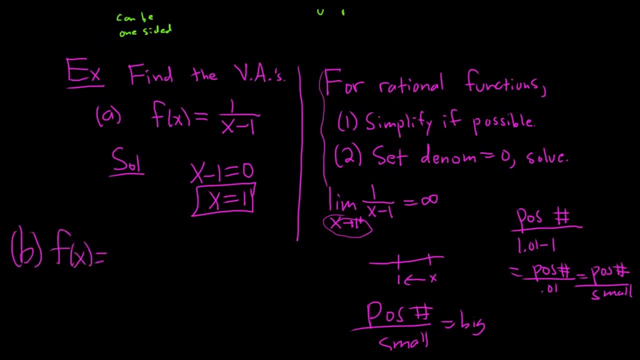 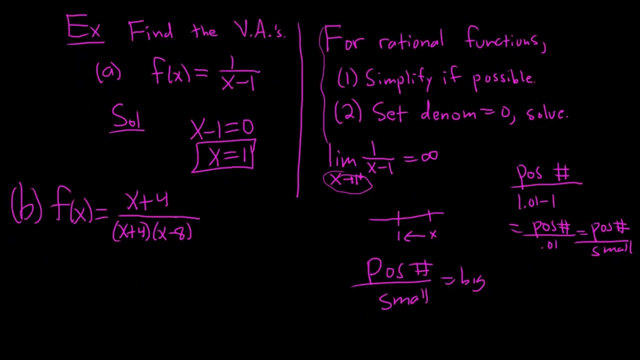 Here we go. B f of x equals. how about x plus 4? Over x plus 4.. Just being silly here- Sometimes it's good to be silly- x minus 8.. So in this case, here, the first step is to simplify first. 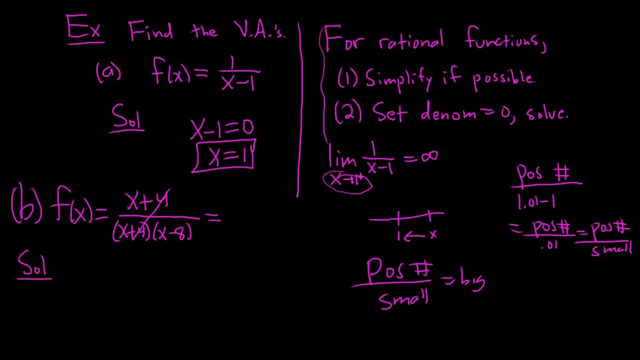 So this cancels. If you recall, that gives you a removable discontinuity. right, We just removed the discontinuity and that was at negative 4.. Whatever makes that 0 gives you a hole in the graph, if you remember from our discussion of removable discontinuity. 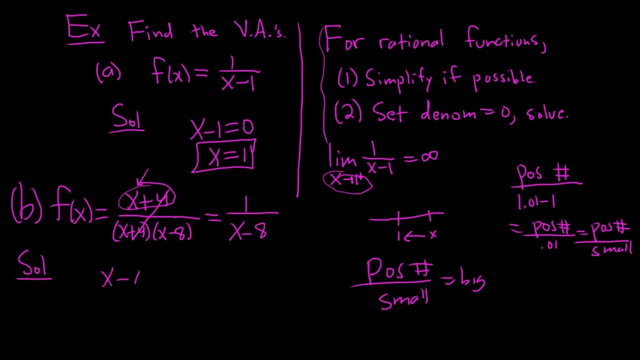 So we're left with this. Then you just set the bottom equal to 0. And so you get 8.. And so 8 is your vertical asymptote. So this is very similar to what we did earlier. If you've been watching these videos in order. 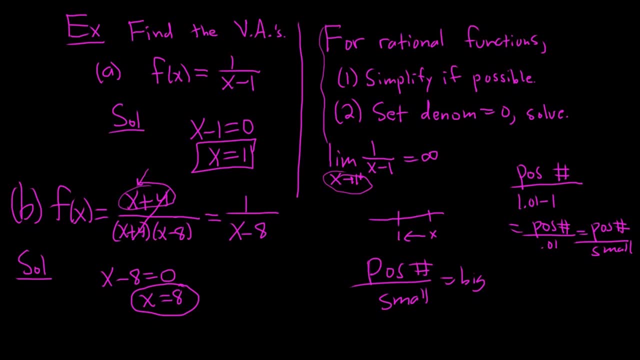 when we find removable and non-removable discontinuities, right Negative: 4 is a removable discontinuity and 8 is a non-removable discontinuity because it's a VA right. This is a vertical asymptote, Vertical asymptote. 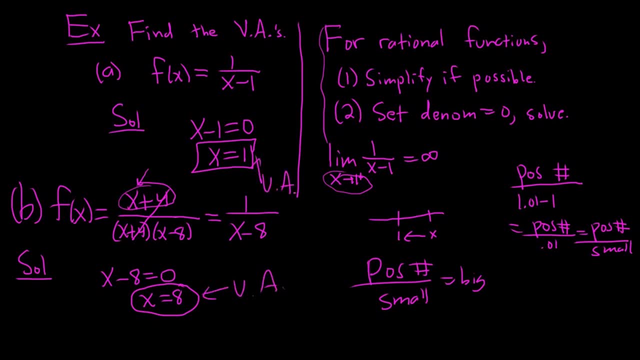 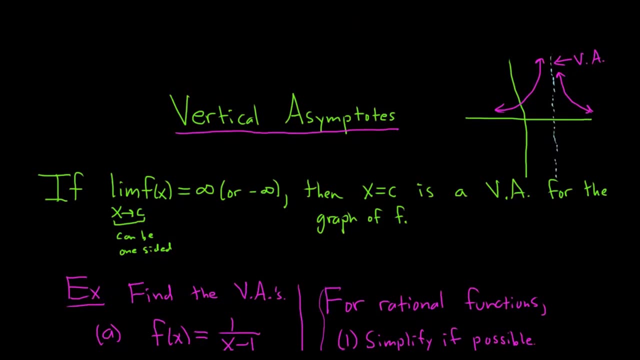 So, basically, we use our old school techniques to find vertical asymptotes, right, We don't really use the calculus, but this is calculus, We're studying calculus. so it's good to see the definition and it's good to see how it applies. 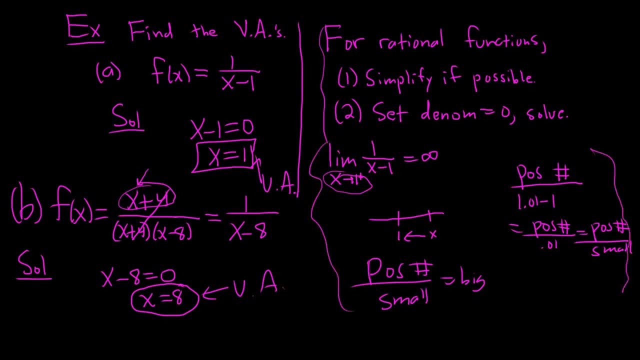 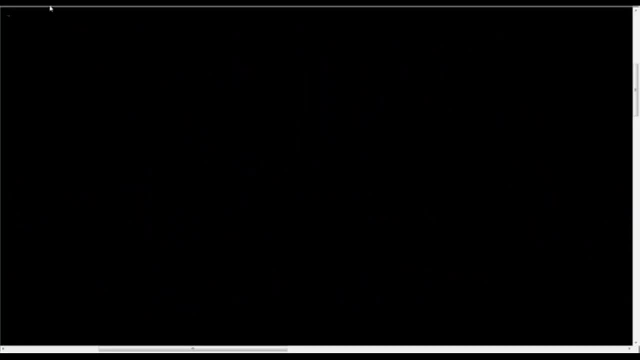 It's much more work to use calculus to find the vertical asymptote, So I hope this video has been helpful. This is just a quick video to talk about what a derivative is. So for notation, we're going to let y be equal to f. 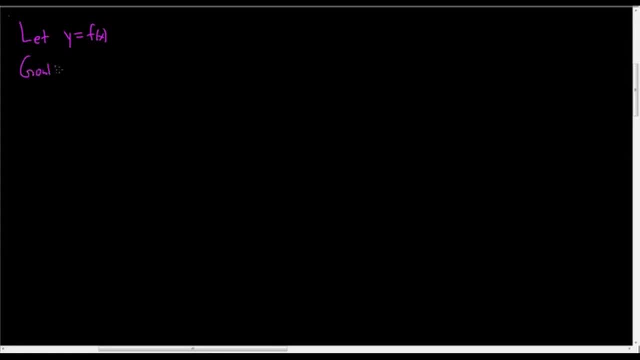 And the goal is to find the slope of this function at x. So find the slope of y at x. So we want to find the slope of y. You might say, well, that doesn't make any sense, It's just a function. 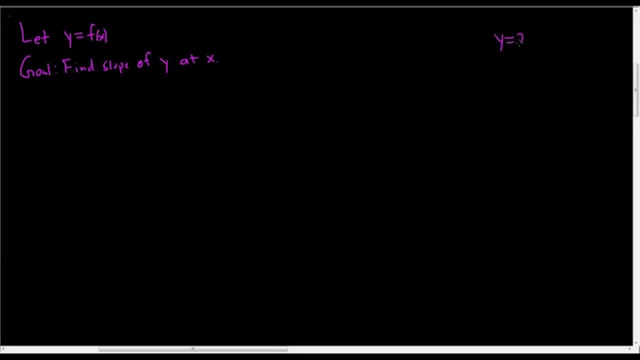 How can you find the slope of a function? Well, for straight lines it's easy. If you have y equals 2x plus 1, then that matches y equals mx plus b, And so we see the slope is m equals 2.. 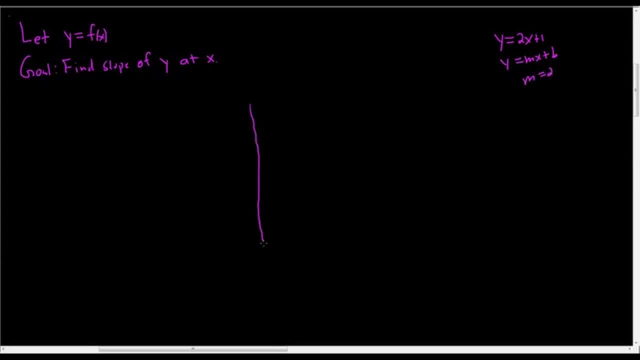 So in calculus, the notion of a derivative tries to extend the concept of slope to things other than straight lines. That's basically what it is. So let's go ahead and draw a picture of our function. Let's assume that it looks like this: 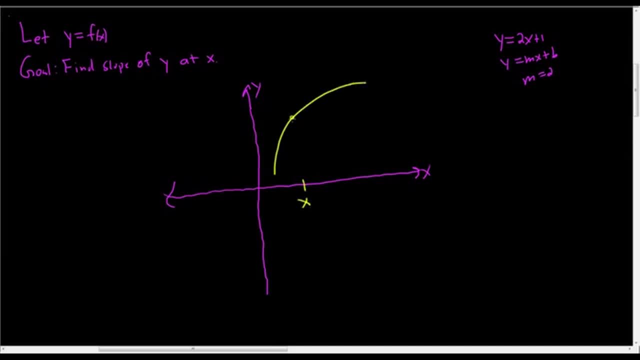 And maybe here's x. So we want to find the slope of this curve at this point, right here, at x. Now, if this is x, then the y value here is going to be f, And so the way we do this is we pick another point. 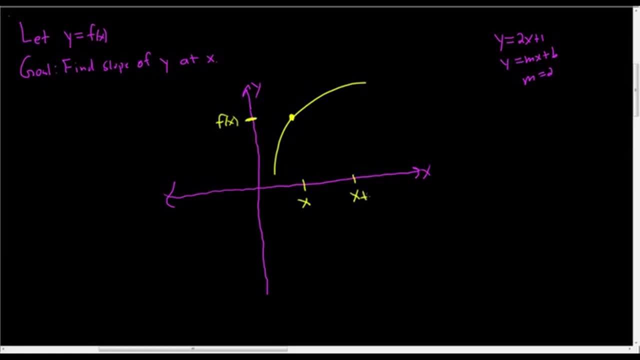 say over here and we call this point maybe x plus h, So that this distance here is simply h And the corresponding y coordinate is up here And let's see, if the x coordinate is x plus h, then the y coordinate is f. 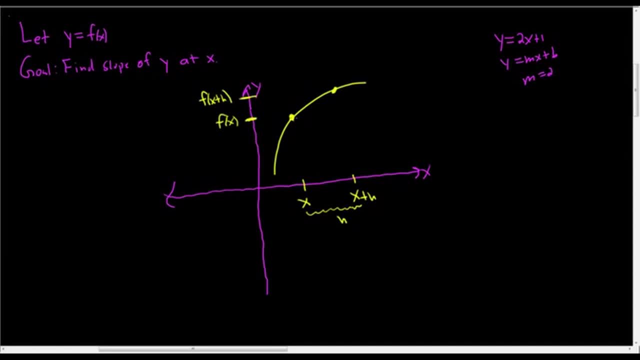 Then what we do is we draw a line that connects these two points. This line has a name. This line is called a secant line- Secant line. So what's a secant line? It's just the line connecting those two points. 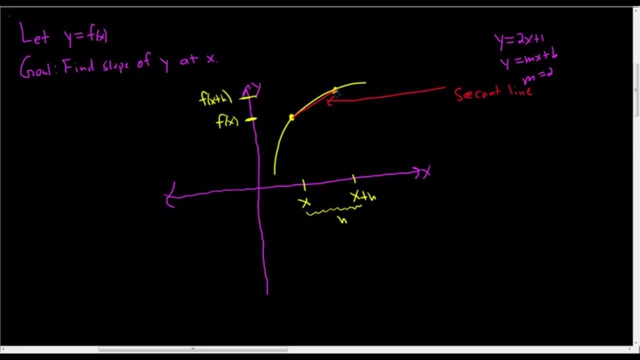 And what we'll do is we'll approximate, or rather find, the slope of the secant line. So slope is rise over run. So we have the run, The run is clearly h. We just have to figure out the rise. Well, we know that this distance here is f. 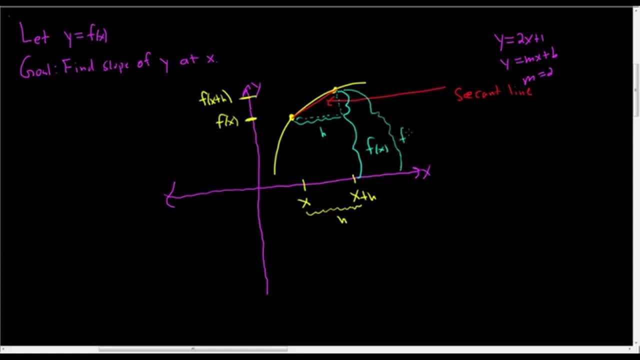 And we know that this bigger distance here is f. That means that this distance here is going to be the big distance minus the little distance, So it'll be f plus h minus f. So let's go ahead and write that down over here, so we know that the slope of the secant line 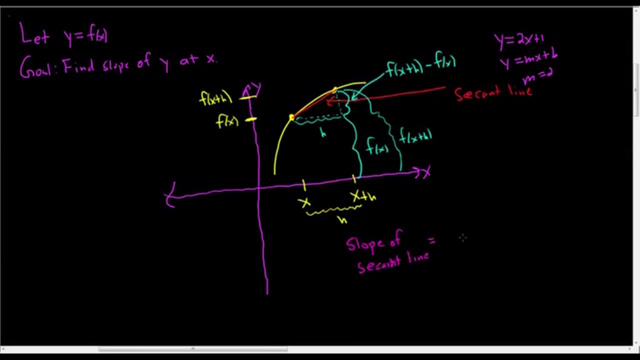 secant line can't spell it. it's rise over run, And so this guy here is the rise. So it's f plus h minus f, And the run in this case is simply h. All right now, here's where you have to use. 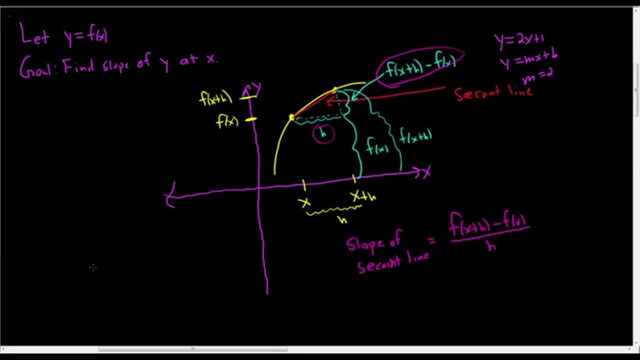 your imagination just a little bit. So what we're going to do is we're going to let h get closer and closer to 0. So as h gets really, really close to 0, so we write that with a little arrow. So as h approaches 0, what's happening? 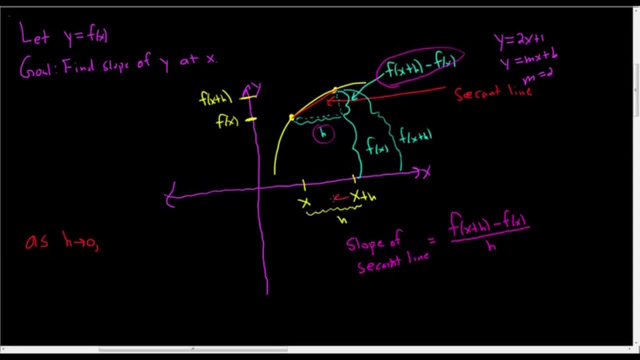 Well, as h approaches 0, x plus h is going this way. It's going to the left, And as it goes to the left, this point here is going to travel closer and closer to this point. So when that happens, let's see. 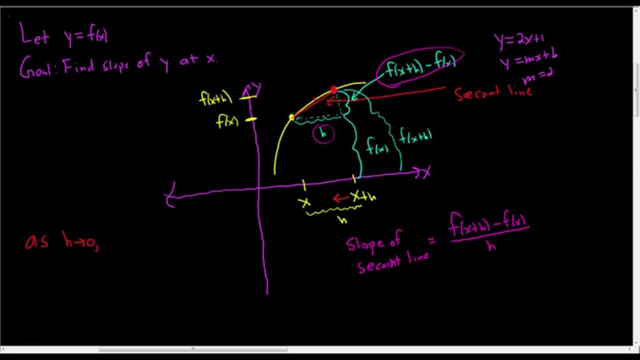 let's pick a stopping point. say here, When that happens, you're going to get another secant line, And when you're here, you're going to get another secant line. So eventually you're going to reach a line. 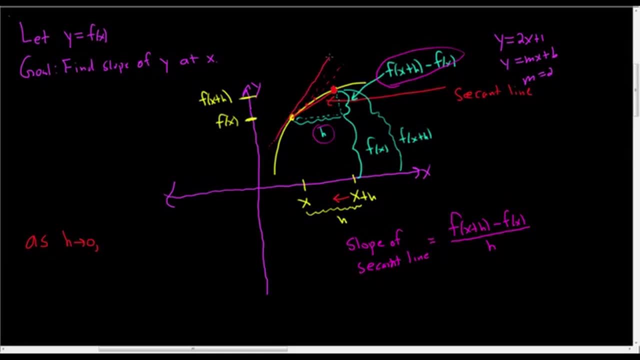 That just touches at x right. The secant lines will approach this other line here. This line here is called a tangent line, Tangent line. So as h approaches 0, the secant lines approach the tangent lines. Let me write that down. 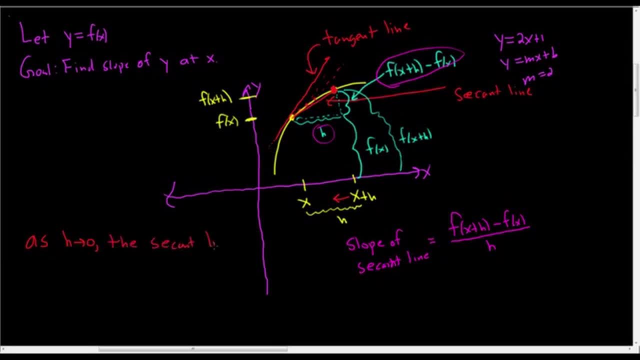 The secant lines approach another line called the tangent line, So approach The tangent line. So that means that the slopes of the secant lines approach the slope of the tangent lines. So the slopes of the secant lines approach the slope of the tangent line. 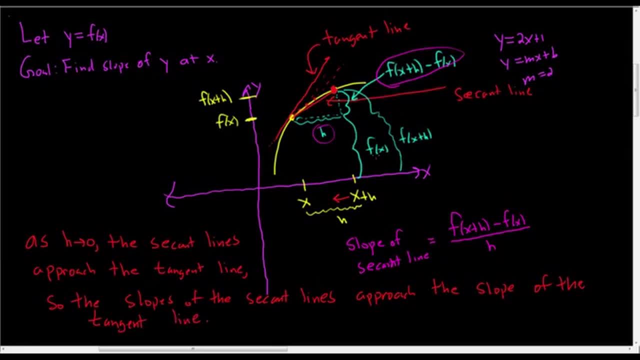 Let's go over that one more time. We're almost done. So we draw this picture, We pick two dots, We connect them, We call that a secant line. We find the slope of the secant line via the picture. This is the slope of the secant line. 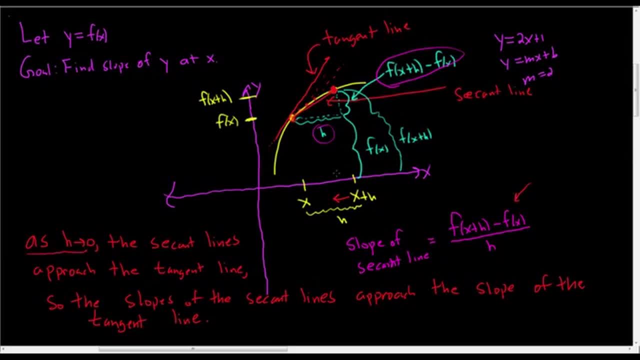 And then we say, as h gets really, really close to 0,, this point here travels to the left, This x coordinate here, this x value. So it's going this way. When that happens, this point is going to move down the graph. 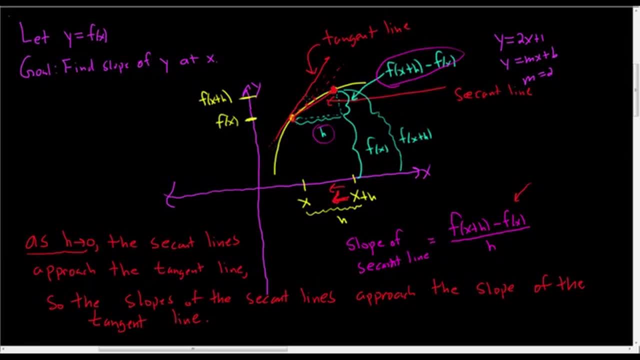 And you're going to get lots of secant lines. So all of these secant lines eventually will reach here or they'll get very close to it. So the secant lines approach this other line, which we call a tangent line. So, because the secant lines approach the tangent line, 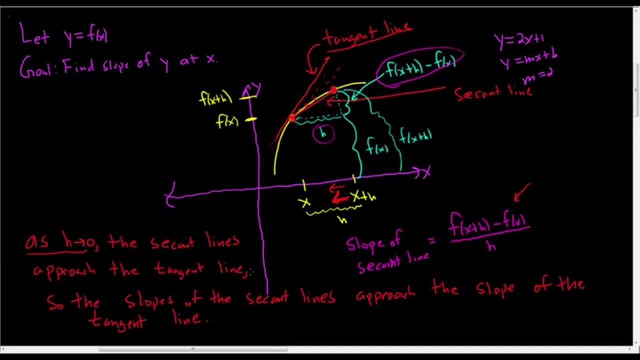 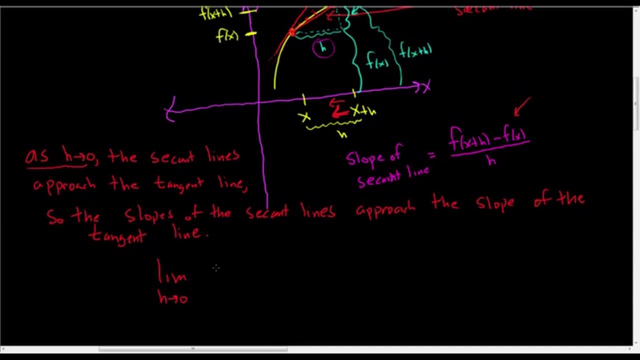 the slopes of the secant lines approach the slope of the tangent line. We can write that down using calculus. We can say the limit as h approaches 0 of the slope of the secant line. So that's this guy here. So if we take the limit of the slopes of the secant lines, 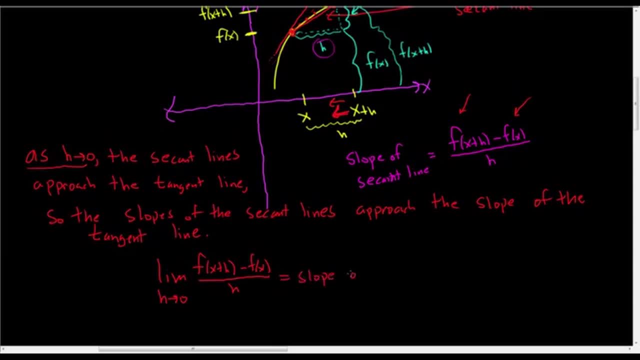 this is equal to the slope of the tangent line at x And we call this the derivative. When this limit exists, we say it's the derivative of f And we write: f prime of x equals this limit. So this is the derivative of x. 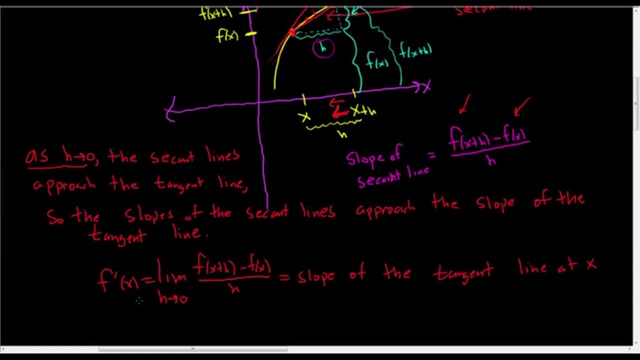 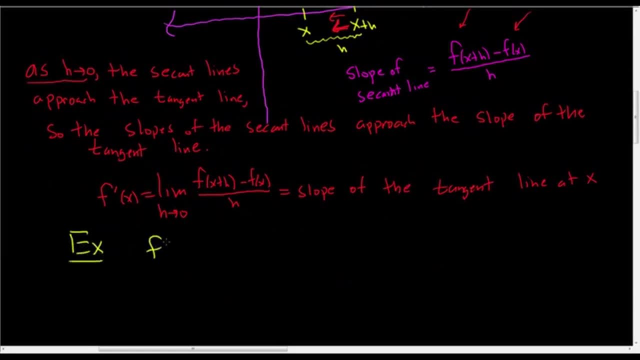 It is the slope of the tangent line to the graph of the function at x. Let's do a concrete example, really really quick, So simple, simple example, Easiest one. Let's look at: f of x equals x squared. So this is a parabola. 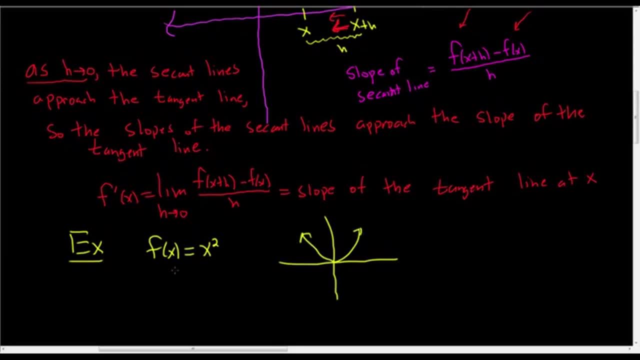 It looks like this: Boom, And let's find the derivative at x. So you probably already know how to find derivatives if you're watching this video. So you take the 2. You bring it down using the power rule formula And you subtract 1 from the 2.. 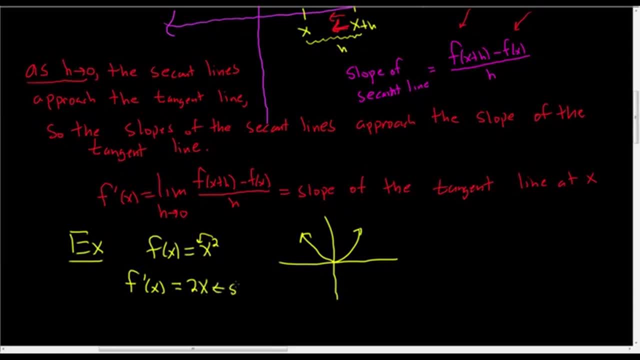 So you get x to the first power. so just x, So 2x. So this is the slope of f of x equals x squared at x. So to make it more concrete, let's look at f prime of 1.. Well, we plug it into our slope formula, right? 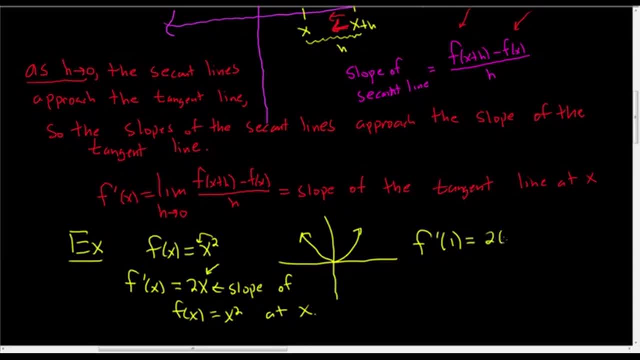 It's a slope formula, It's a slope function And you get 2 times 1, which is 2.. So we're saying that the slope of f of x, or more precisely, the slope of the tangent line to the graph of f, 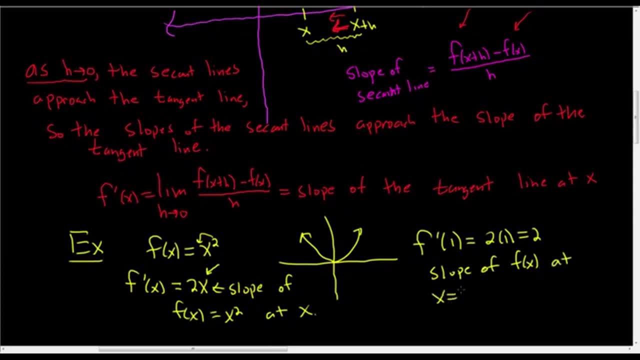 so the slope of f of x at x equals 1 is 2, right, Because this is the slope, So it's a slope function. So the tangent line may be: here's 1.. Maybe the tangent line looks something like that: 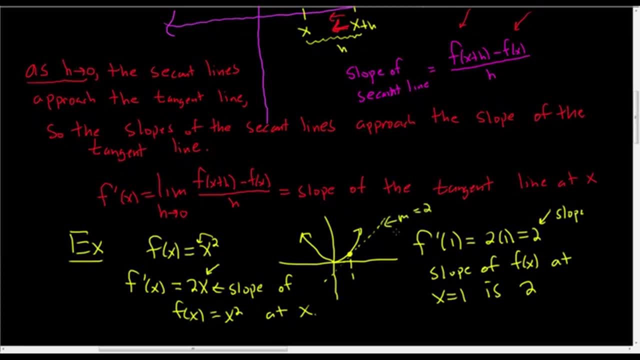 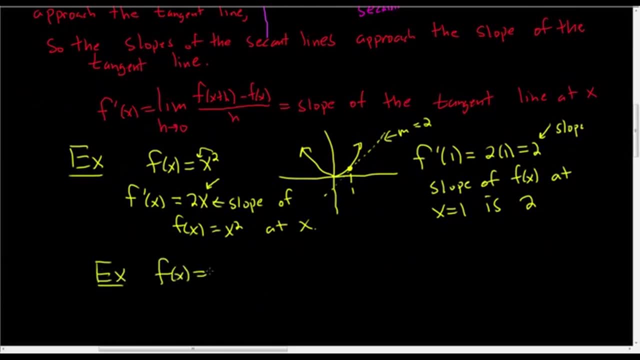 So 2 is the slope of this line. One more, really, really quick. Let's look at a simpler function: f of x equals 3x plus 7.. So we're taking the derivative using the derivative formulas. The derivative of 3x is simply 3,. 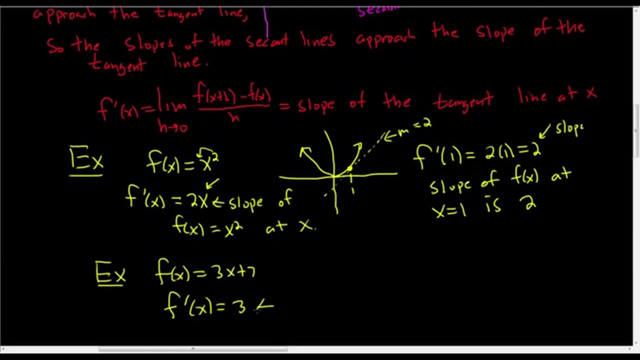 and the derivative of 7 is 0. So we get 3. And that makes sense. This is a straight line with slope equals 3. For every x right. So the slope of a straight line doesn't change, But for other functions the slope does change. 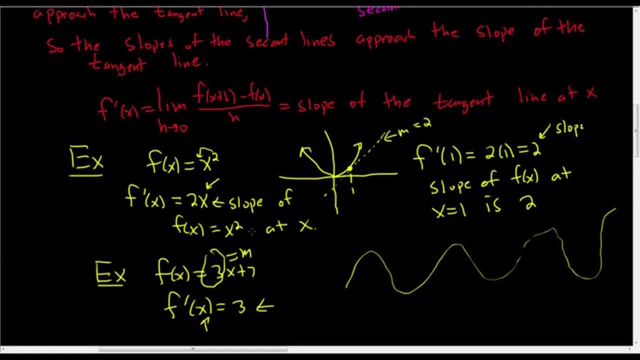 and it could change, and it certainly does. So that's why we use calculus, That's why we use derivatives to find the slopes of functions at various points. Hopefully that made some sense. I kind of just rushed this video and made it up on the spot. 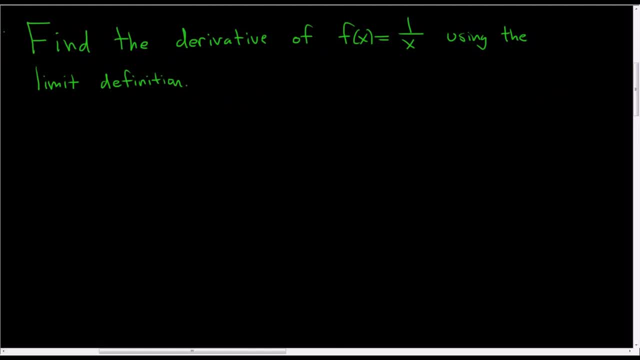 So that's it. We're being asked to find the derivative of 1 over x using the limit definition. Let's go ahead and do it. So the first step is to compute the difference quotient. So that's f of x plus h minus f of x, all divided by h. 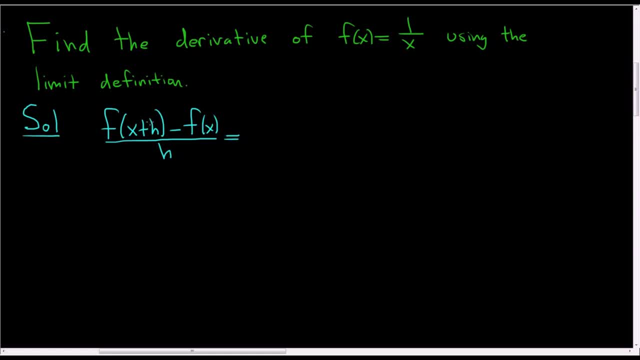 So this is equal to well, f of x plus h. you just replace x with x plus h. So this is 1 over x plus h, minus 1 over x, because that's f of x And all of this is being divided by x. 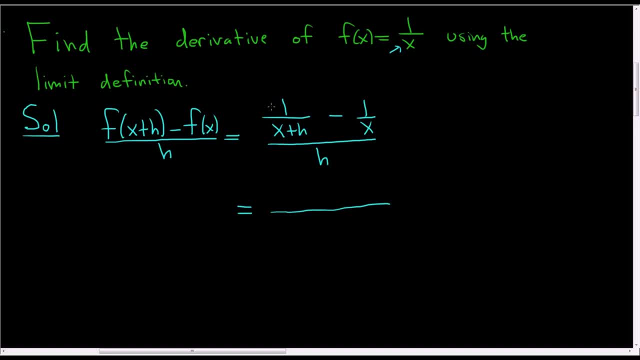 The next step is where it gets a little tricky. We actually have to perform the subtraction in the numerator, So the least common denominator is x x plus h. So I'm going to go ahead and write it down: x x plus h. 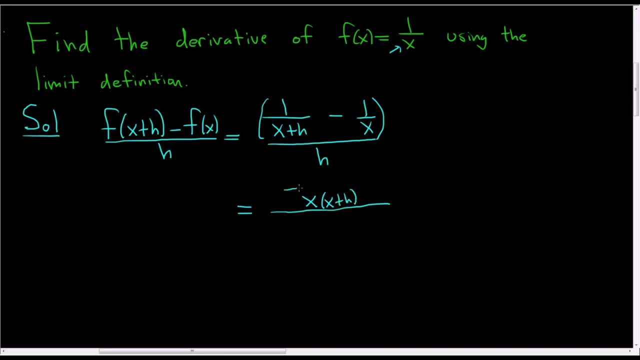 So we know that's going to be the denominator. Then, the way I do this, it's going to be 1 times whatever is missing here to get the LCD. So we're missing an x, so 1 times x Minus 1 times whatever is missing here to get the LCD. 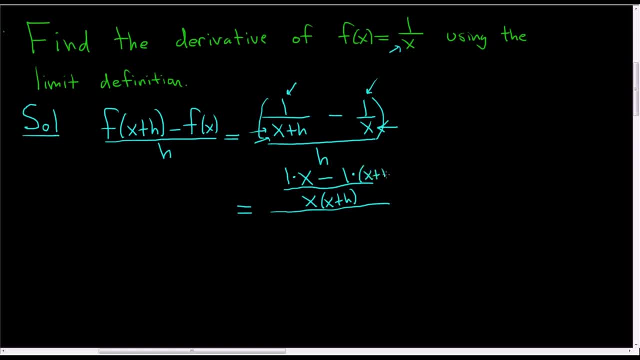 So we're missing an x plus h. So x plus h- And all of this is in parentheses. It's really important. It's all being divided by little h. Let's keep going. This will be x minus. distribute the negative 1,. 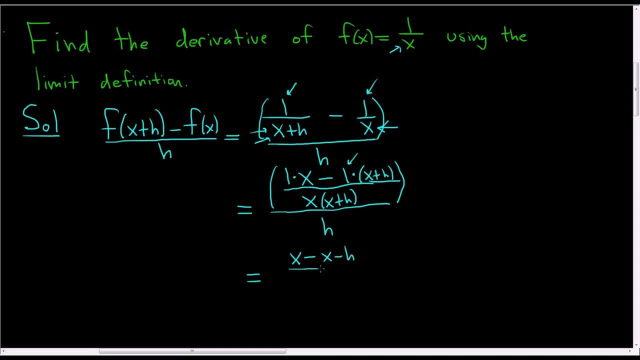 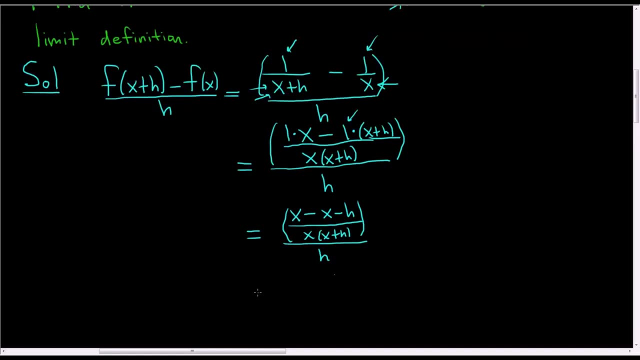 so minus x, minus h, all divided by x, x plus h, and this is in parentheses- and it's all being divided by h. Let's keep going. So this is equal to looks like the x. the x is cancel. yep. 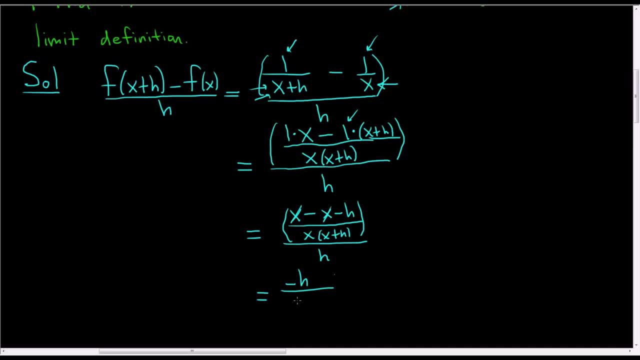 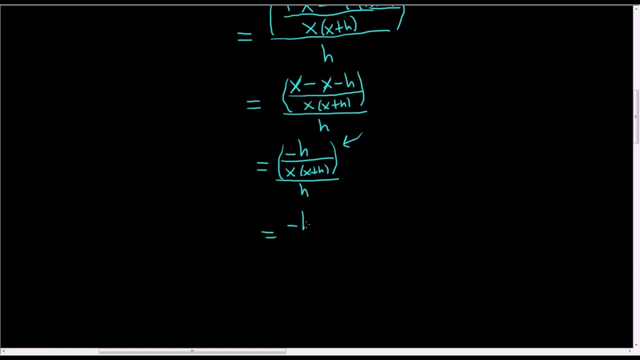 And so we have negative h over x x plus h, and all of this is being divided by little h, Almost there. So we have this, which is negative h times over x x plus h, and it's being divided by h. 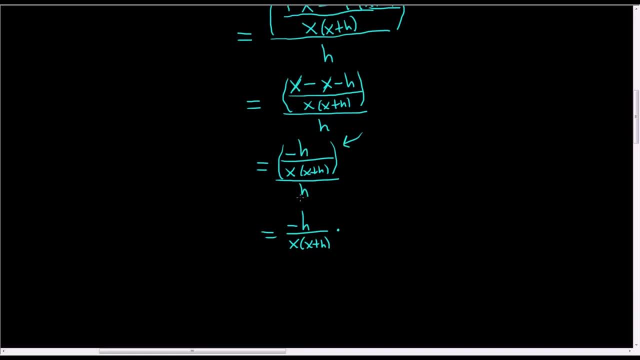 When you divide by h, you multiply by the reciprocal, So it's really h over 1.. So you multiply by 1 over h, The h's cancel and we're left with negative 1 over x, x plus h. So to finish, we'll take the limit. 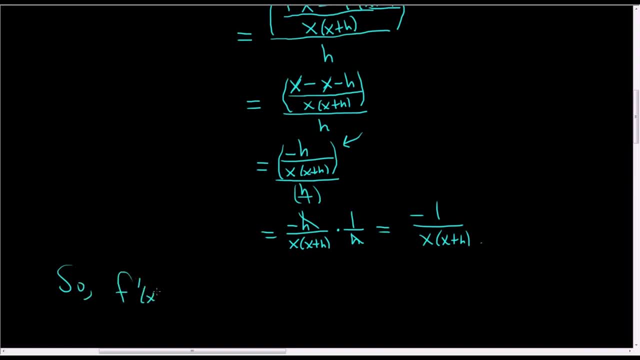 So the derivative of f with respect to x is the limit- as h approaches 0, of the difference quotient. That's what we computed. So f of x plus h minus f of x, all divided by h. But we simplified this. 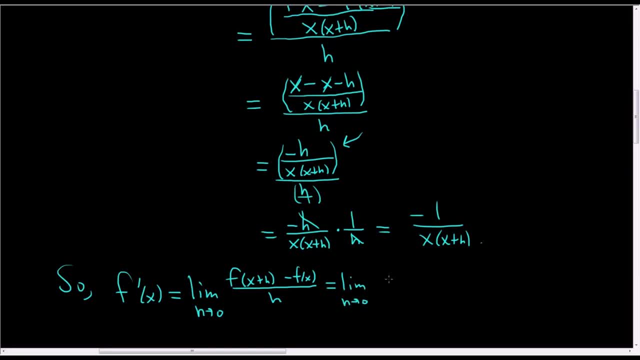 so this is the limit, as h approaches 0, of negative 1 over x, x plus h, And now we can go ahead and plug in 0. So we get negative 1 over x, x plus 0. And so we end up with negative 1 over x squared. 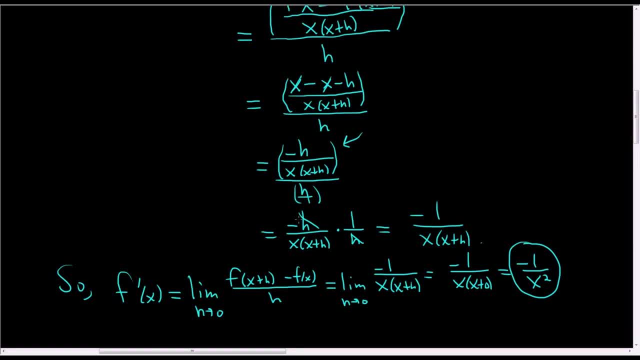 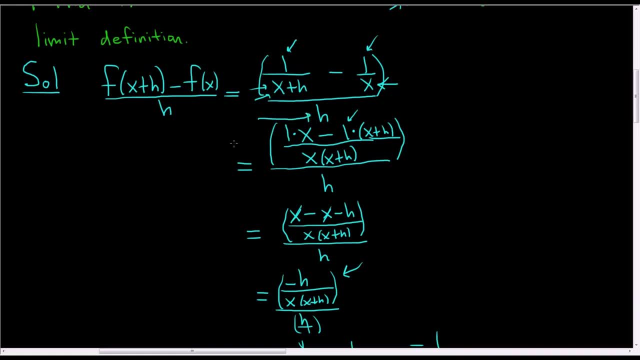 And that's the final answer. Now, the reason we couldn't take the limit at the beginning is because we had an h on the bottom, So we couldn't just plug in 0 for h, because that would be undefined. I hope this helps. 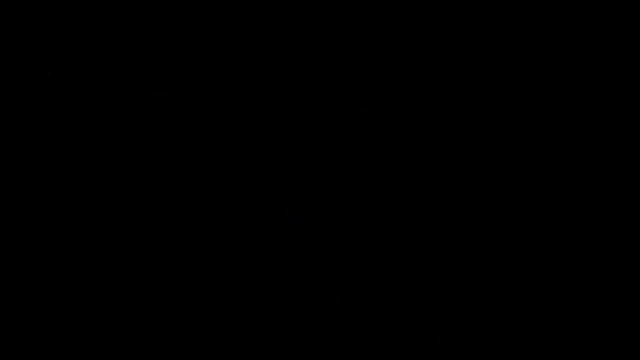 In this video we're going to discuss the basic differentiation rules. So first we'll start by letting y be equal to f of x, And so recall there's a couple different ways to denote the derivative of this function. So one way is y prime. 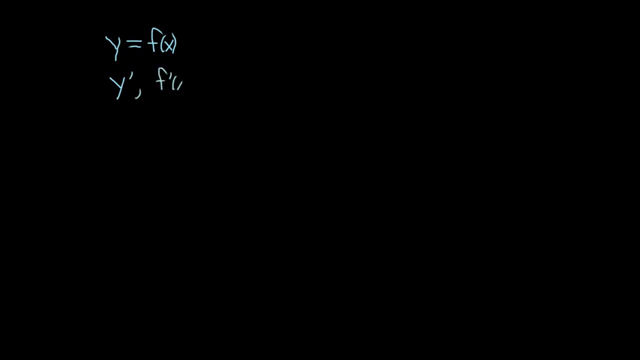 Another way is f prime of x. Another way is simply dy dx, And you could also even do df dx. So in the notation that follows we're going to use this notation here. So the first rule says: if we take the derivative with respect to x, 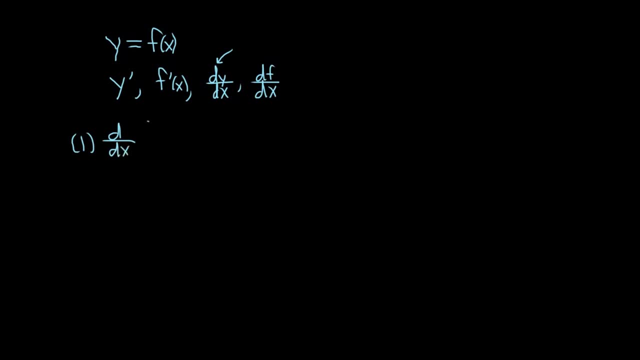 so ddx means: take the derivative with respect to x of a constant function. what do we get? Well, let's think about it. The derivative is the slope of the tangent line. So if you were to graph a constant function, say c: 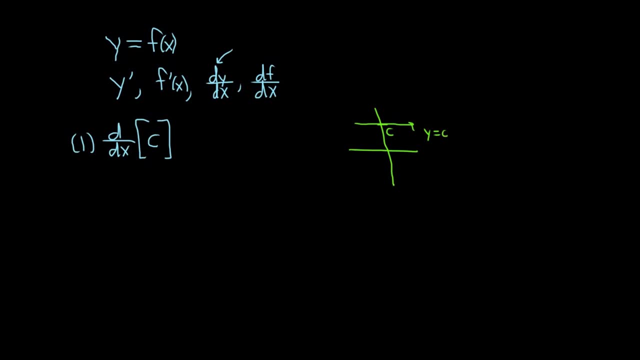 it's a horizontal line. So if you pick any point on this line and you draw a tangent line, you get the same line. So the derivative is the slope of this line. Well, horizontal lines have a slope of 0, therefore this derivative is 0.. 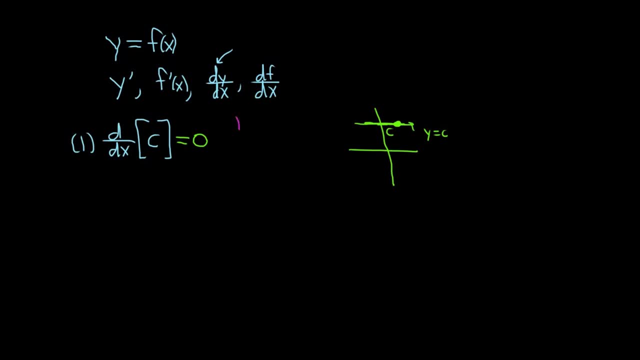 So the derivative of a constant is 0. It may sound silly, but let's do a simple example. Say we have f of x equals 2. And we're asked to find the derivative of this function. Well, all we do is we write f, prime of x. 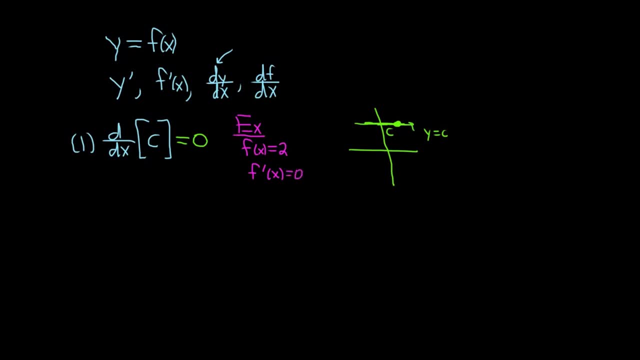 and the answer is 0. So the derivative of a number is always 0.. Super, super important rule. The second formula is extremely important. It's so important it's given a name. It's called the power rule. So power rule. 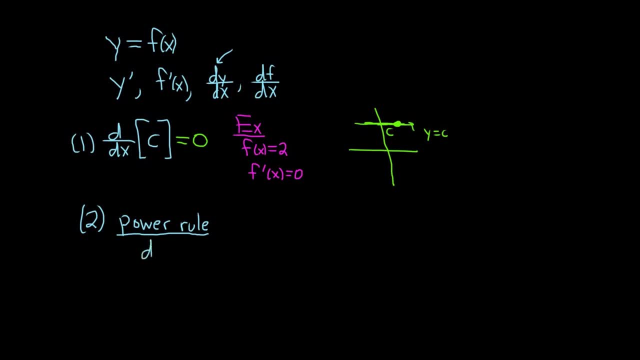 So the power rule says: if you take the derivative with respect to x, of x to a power, so x to the n, what you do is you just put the n in the front. So you put the n in the front and then you subtract 1 from the exponent. 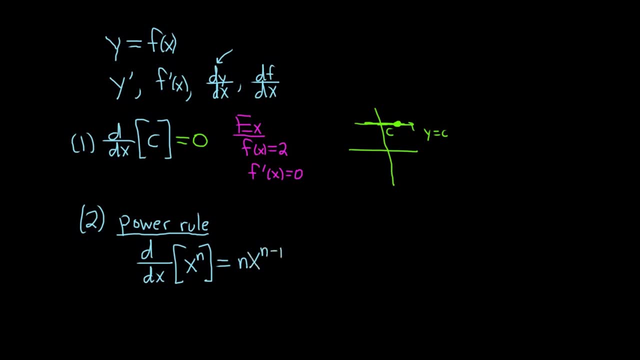 So you write n minus 1.. Okay, that's called the power rule. The power rule. Let's do a simple example. So say we have the derivative with respect to x of x cubed Of x cubed. This means: take the derivative with respect to x of x cubed. 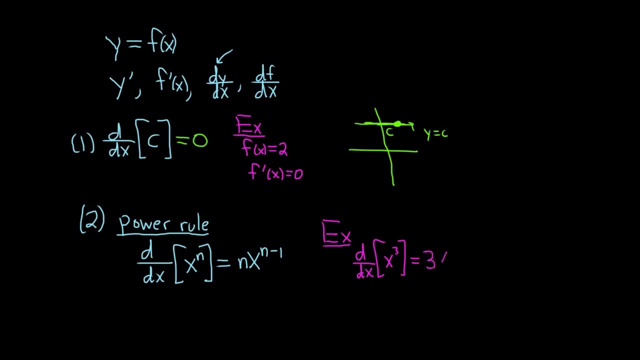 So you put the 3 in the front, so you get 3x. then you just subtract 1.. 3 minus 1 is 2.. Boom, there it is. We're doing calculus right. Let's do another one. 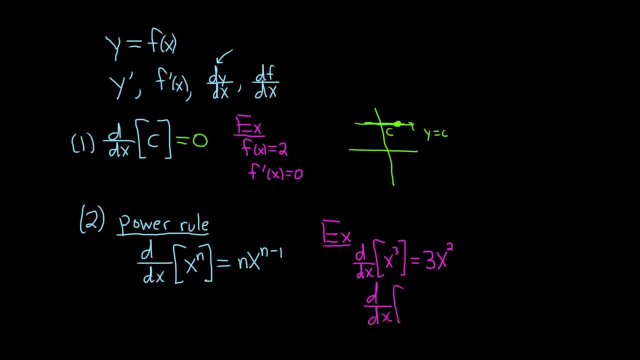 d, dx of x to the 4th. So you put the 4 in the front, you get an x. you subtract 1, so you get 3.. Boom, that's it. So that's the power rule. Put the number in the front. 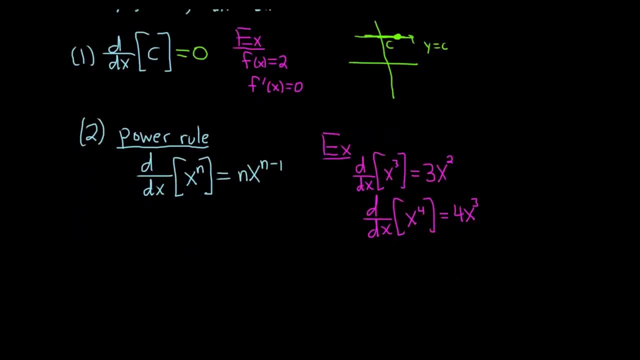 and subtract 1.. The next rule says if we have a constant times a function of x, the constant can hang out. So say we have ddx of c times some function of x that we'll assume is not constant, Or even if it's constant. 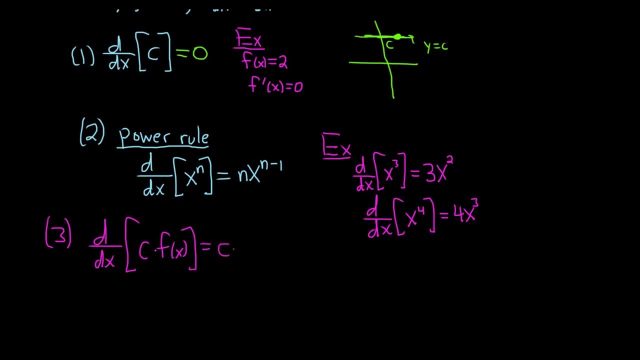 I think it'll still work. This is c times the derivative of f. Yeah, even if it's constant, it'll work, Because if f is constant, its derivative is 0, right, So everything makes sense. right, Because you get constant times constant. 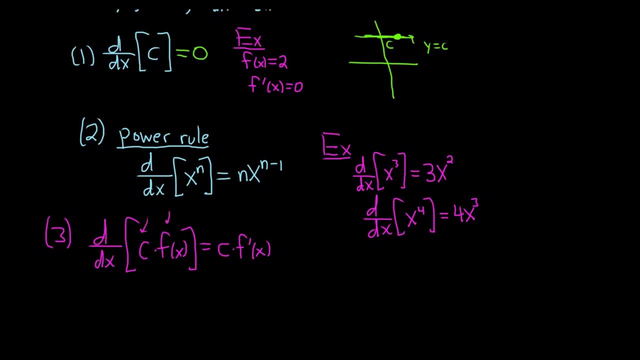 which is constant, so life is good. So very powerful formula. It basically says: constants hang out. So here's an example: Say we have f of x equals 4x to the 5th. Okay, so we take this derivative. 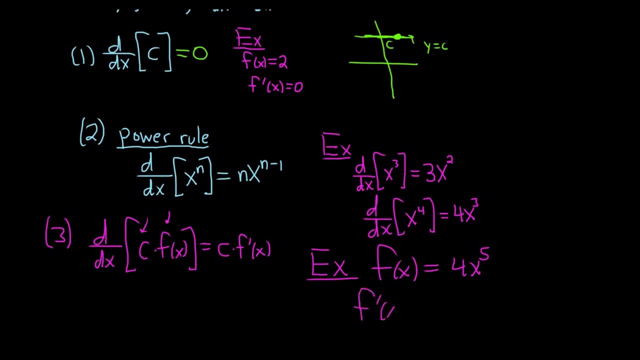 So f, prime of x. I'm using different notation just to show you that you could write the ddx or you could write f and then write f prime, Whatever works. So you put the 5 in the front, The 4 just hangs out. 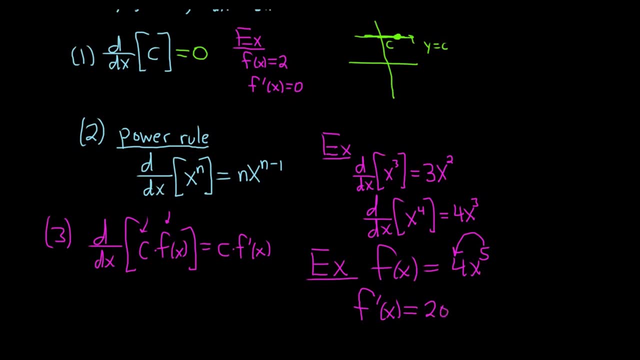 So you do 5 times 4,, so it's 20.. x and you subtract 1.. 5 minus 1 is 4.. So again, 5 times 4 is 20.. And you subtract 1, and you get 4.. 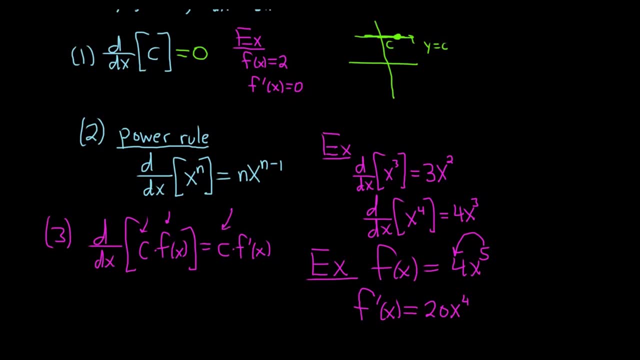 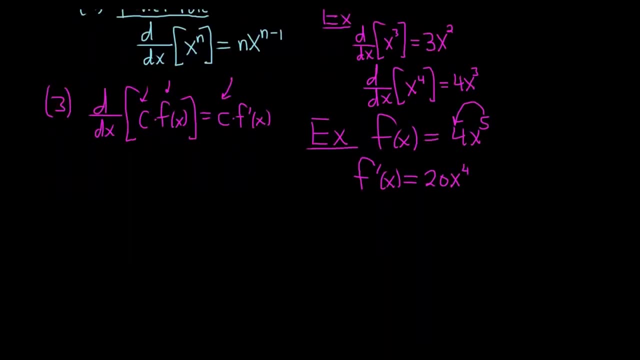 So we use this rule right. The 4 was the c, So it kind of just like stays back there and just kind of hangs out. All right, Then we have: let's look at the derivatives of some trig functions. Look at the derivatives of some trig functions. 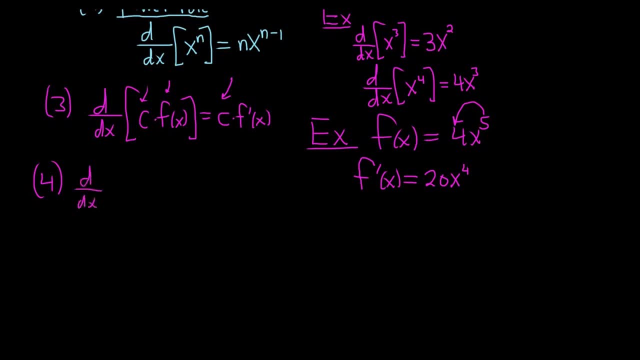 So we have the derivative of sine That's equal to cosine, Which is totally worth memorizing, right, Totally worth memorizing. The derivative with respect to x of cosine is equal to negative sine. Okay, A little bit harder to remember this one. 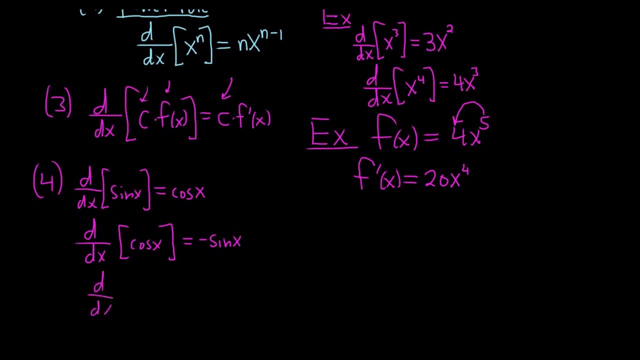 The derivative with respect to x of let's do tangent next, That's another common function. This one is secant squared. You might say, oh, I'm never going to memorize that, Don't worry, You will. You know. 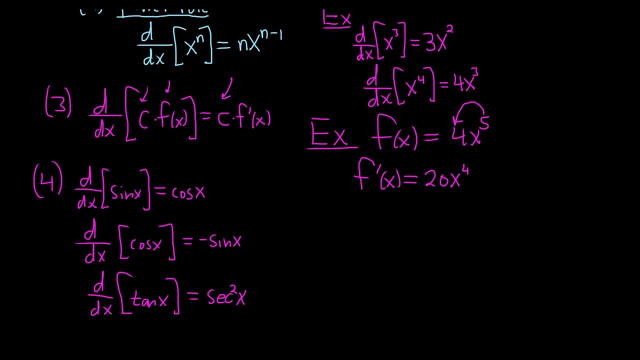 if other people can learn calculus, you can learn calculus. So the derivative of tangent is secant squared, Like you will know it after you do lots of problems. Then we have the harder ones. So the derivative with respect to x of secant. 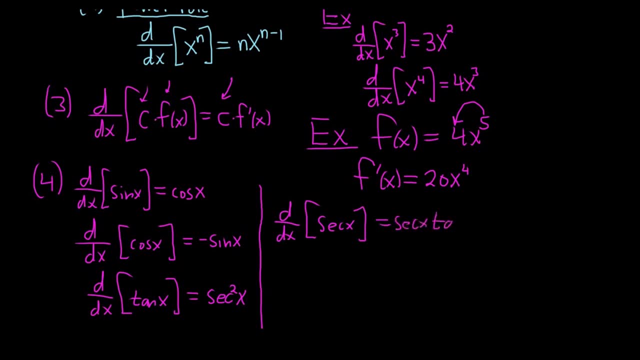 That one is secant tangent, Secant tangent, That one's not so bad. And the really uncommon ones are cotangent and cosecant. So the derivative of cotangent is negative cosecant squared x And the derivative of cosecant is negative cosecant cotangent. 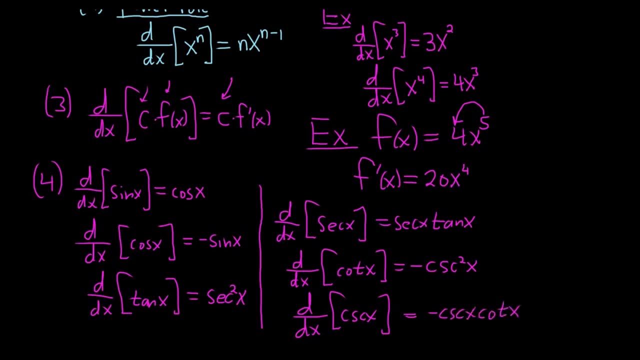 So there's a couple tricks. Let me pause here and let you catch up if you're writing this down. There's a couple tricks to memorize these. I don't use this trick, but here's one that someone told me once. If you take the derivative of anything, 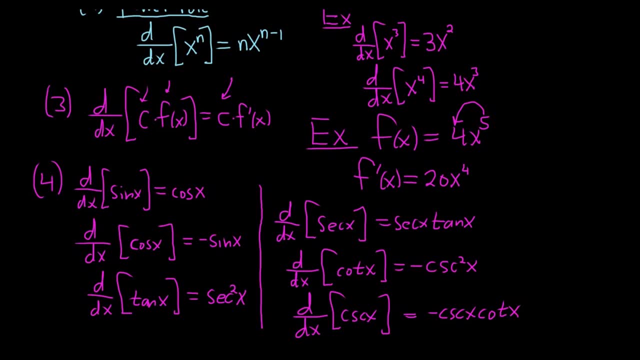 and it starts with a c, you're going to have a negative sign. Check it out. Look, Cosine has a c- Boom, There's a negative. Pretty cool Cotangent has a c Boom, There's a negative. 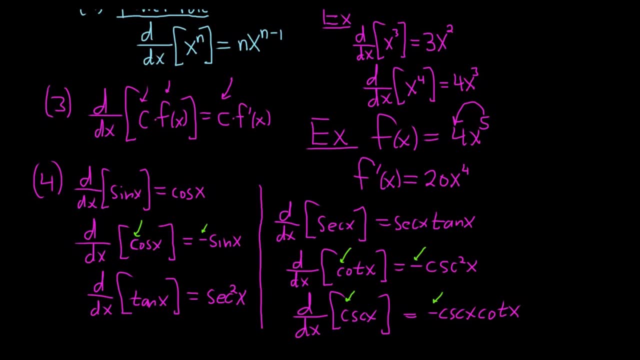 Cosecant has a c Boom, There's a negative. So that's kind of cool. How do I do it? I just memorize them. The derivative of sine is cosine. That one's easy. This is the annoying one. 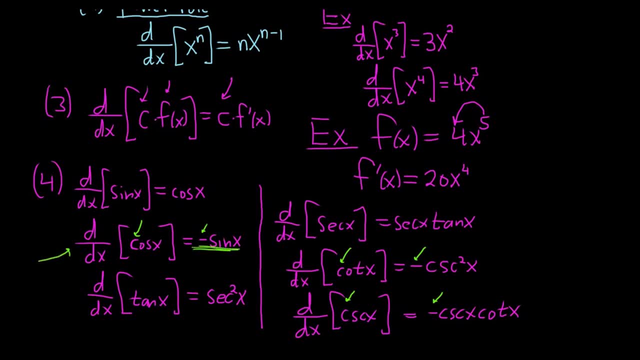 The derivative of cosine is negative sine. This is the one that causes constant mental anguish. The derivative of tangent is secant squared. Secant is secant squared- Pretty easy to memorize. The derivative of secant is secant tangent. And then these are weird. 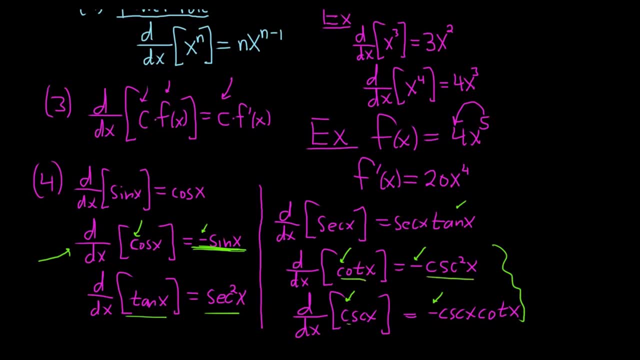 Derivative of cotangent is negative. cosecant- squared. Derivative of cosecant is negative. cosecant- cotangent. Notice that these cunt functions, secant and cosecant, appear in their own derivatives. Look See The derivative of secant. 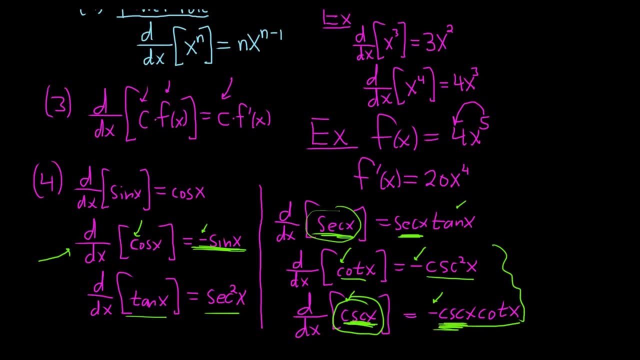 secant shows up. The derivative of cosecant. cosecant shows up. And when you take the derivative of, like cotangent and tangent, you get those cunt functions again Right. The derivative of tangent is secant squared. The derivative of cotangent is negative- cosecant squared. 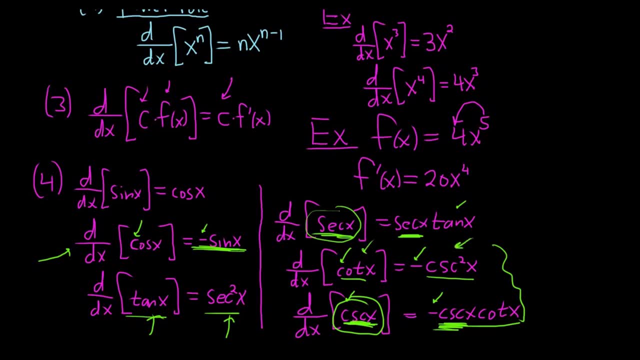 So there is some type of pattern that you can use. That's it for now. In the next video we'll look at some more important rules and we'll do examples using these trig functions. In this video, we're going to talk about a very 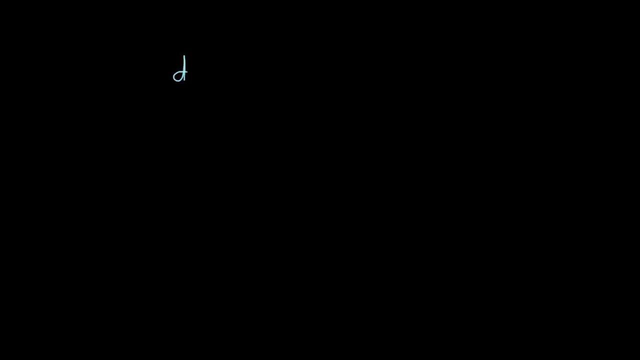 very simple differentiation formula. It says: if you take the derivative with respect to x of a sum or difference, so f of x plus or minus g of x, all you do is take the derivative of each piece. So you first take the derivative of f. 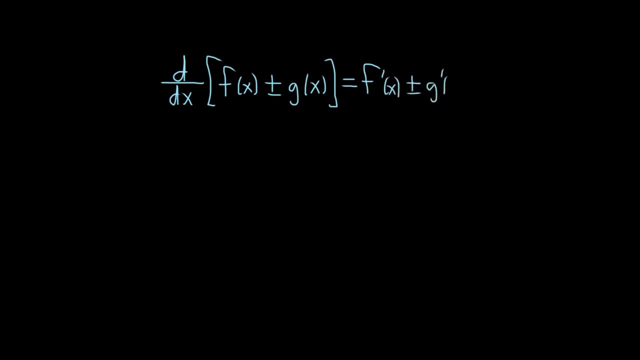 and plus or minus the derivative of g. So if you put this together with one of our other rules where constants hang out, you get the following: If you take the derivative with respect to x of, say, a constant alpha f of x, plus or minus beta g of x, 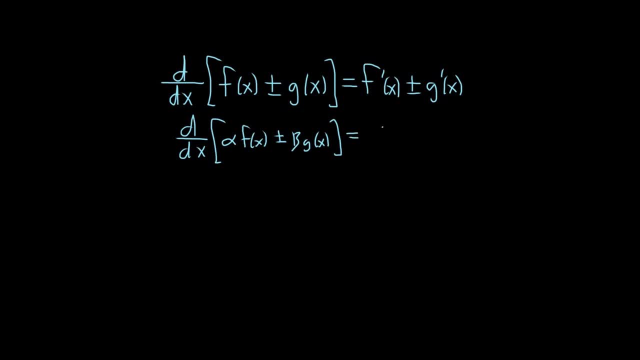 you can basically ignore the constants and just take the derivatives of the functions. So it's alpha f- prime of x, plus or minus beta g, prime of x. So let's go ahead and do some examples. So, by the way, this property that the derivative possesses, 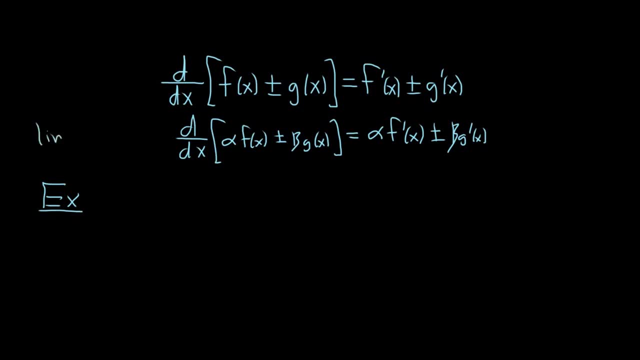 is called linearity. So linearity, We say that the derivative operator, we think ddx, we say ddx is an operator, Its operation is differentiation And we say it's a linear operator because it has this property. Okay, let's do some problems. 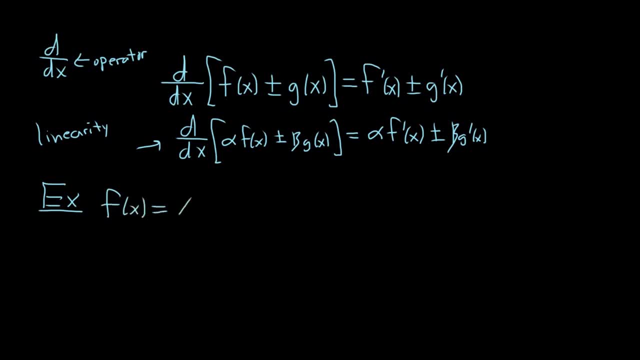 Let's find the derivative of x to the fourth plus x plus two. So, using the linearity property of the derivative, we can simply just take the derivative of each piece. So for the x to the fourth we can use the power rule. 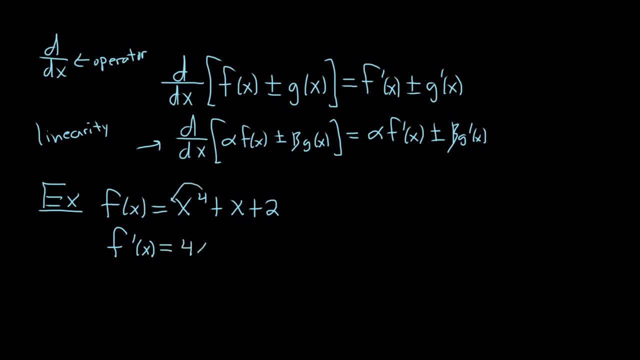 So we put the four in the front, So we get four x cubed, The derivative of x. Let's talk about that. Well, a couple ways to think about it. One: you can use the power rule. Think of it as x to the one. 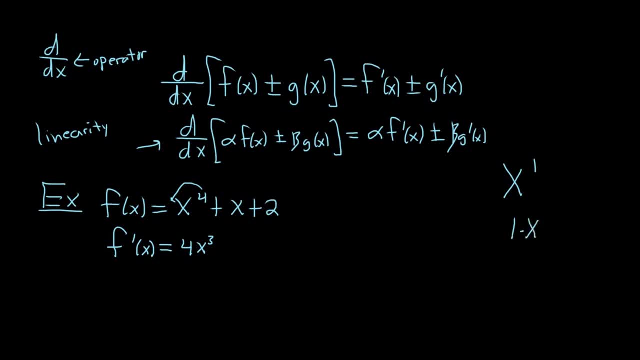 You put the one in the front, You subtract one. One minus one is zero, So you just get one times one, So you get one. Another way to think about it is to think about y equals x. If you think about y equals mx plus b. 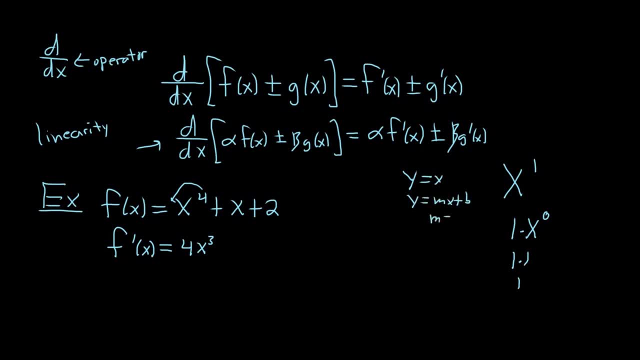 you see that using matching m is equal to one. So recall that the derivative of a function is the slope of a function. So the answer here is just one. I honestly just memorize it. The derivative of x is one. So if it was two x, it would just be two. 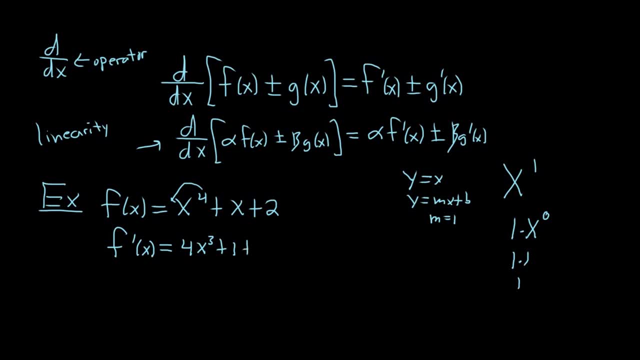 If it was three x, it would be three, And the derivative of two is zero because it's a constant. So the final answer here would be four x cubed plus one. Let's do another problem. How about? f of x equals three cosine x. 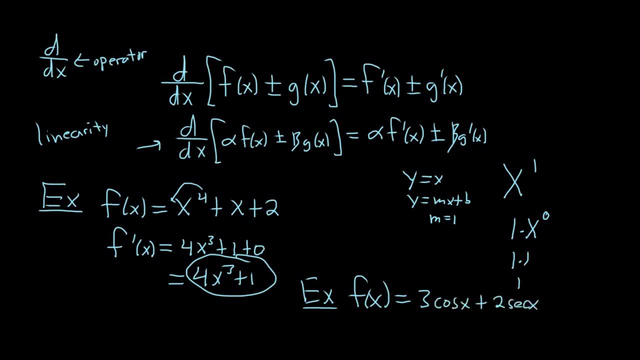 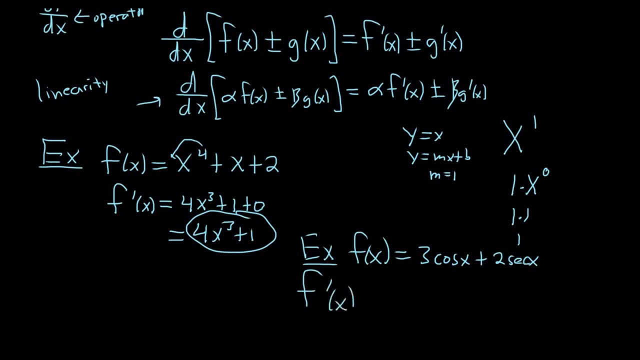 plus two secant x. So now all we do is just take the derivative of each, So f, prime of x. So the three is a constant. It hangs out. It's like the alpha in our formula. It just hangs out. So it's three. 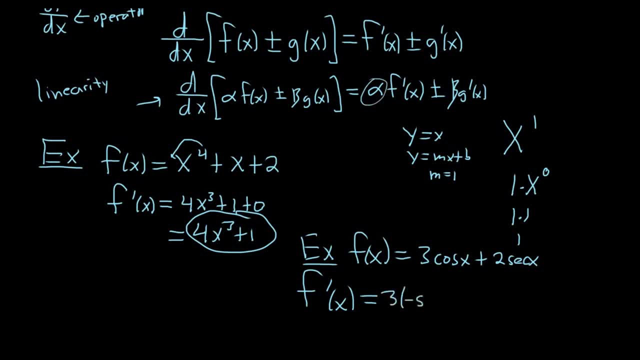 The derivative of cosine is negative, sine, And then plus two, And the derivative of secant is secant, tangent. So secant x, tangent x. Last thing we could do here is maybe put the negative in the front. So it's negative three sine x. 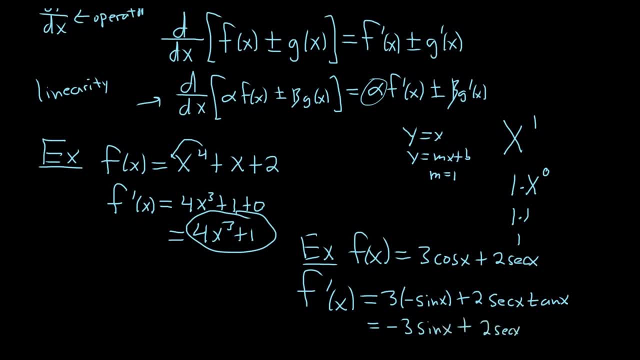 plus two secant x, tangent x, And that's it. So the moral of this video is, when you have more than one thing, you can just take the derivative of each thing, because the derivative has what's called the linearity property. It is a linear operator. 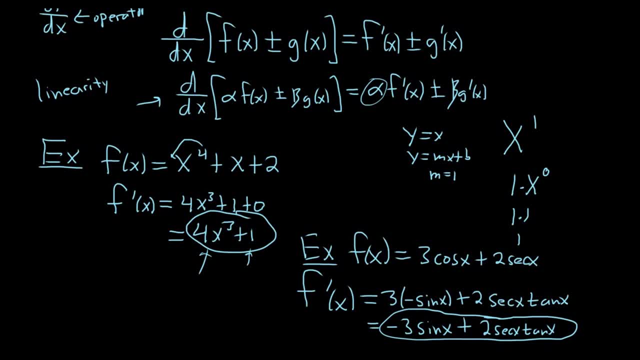 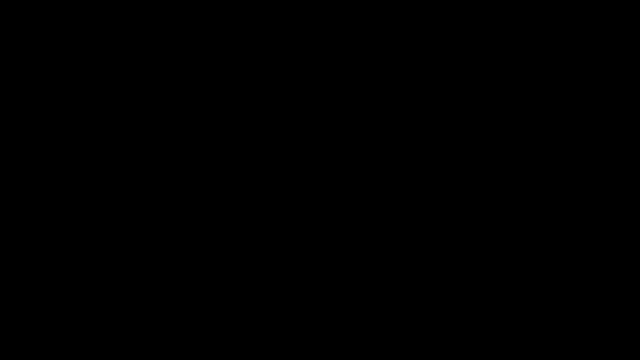 And so you are allowed to do that. I hope this video has been helpful. In this video, we're going to look at one of the most important rules in all of Calculus 1. It's called the product rule, So product rule. 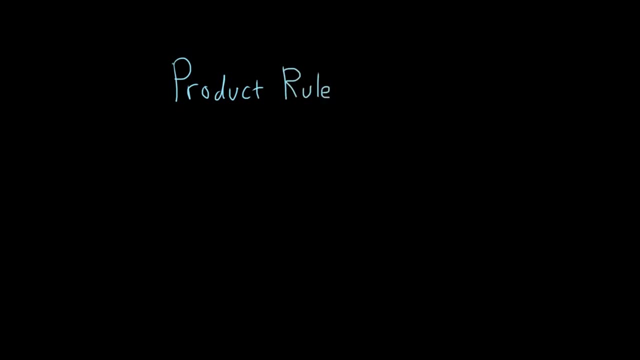 Product rule is extremely useful. It basically gives you a formula for the derivative of a product. So if we have ddx, the derivative with respect to x of a function, f of x times g of x, We get the product rule. 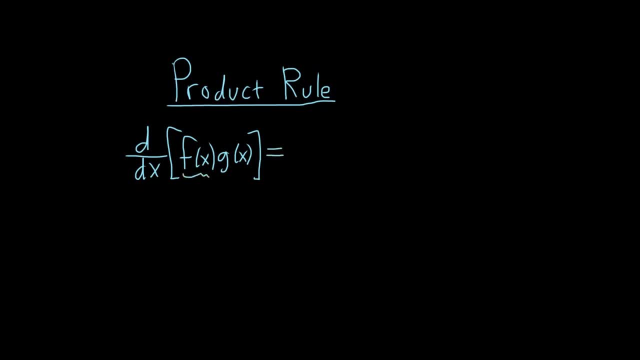 So the product rule. the best way to memorize it I have found is to think of this as the first piece and this as the second piece. The product rule says it's the derivative of the first times, the second plus the first. 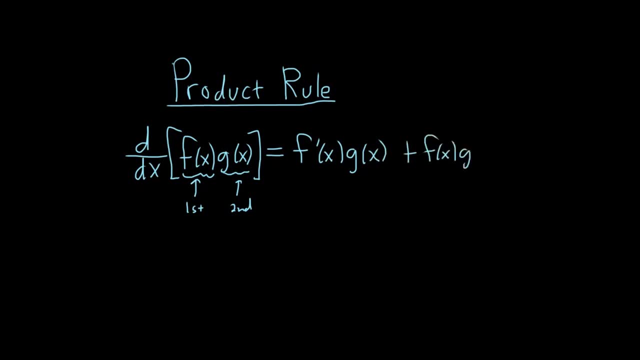 times the derivative of the second piece. So it's the derivative of the first times the second plus the first times the derivative of the second. Let's do a problem. So you see how it works. So I'll use a different letter besides f and g for my function. 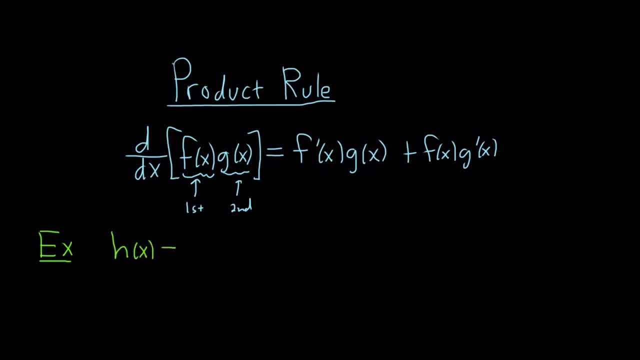 Let's say h of x is equal to how? about x to the fourth sine x? And we'll find the derivative of this function using the product rule. So you can think of this as your first function and this as your second function. 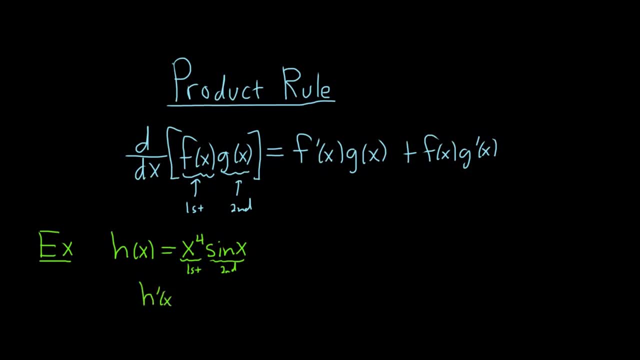 So h, prime of x. it's the derivative of the first, so 4x cubed times the second, so sine x, plus the first, so x to the fourth times the derivative of the second, So the derivative of the sine function. 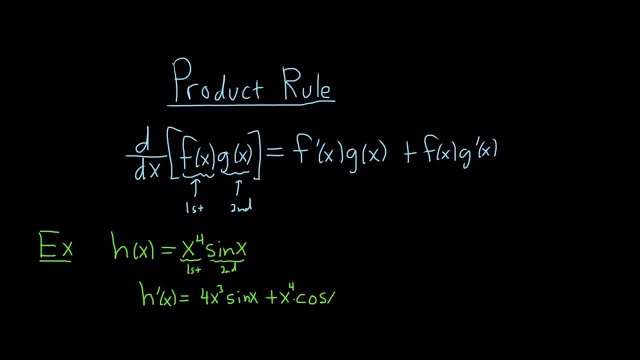 is the cosine function. And that's it. Let's double check our work. So it's the derivative of the first piece, so the derivative of x to the fourth. We use the power rule right. We put the 4 in the front. 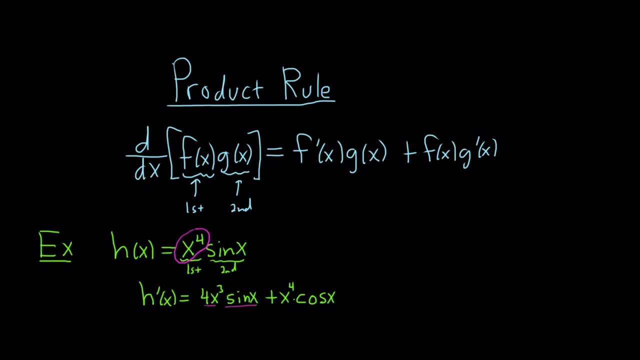 so we get 4x cubed times the second Plus the first times the derivative of the sine function. So that's just going to be cosine. So everything looks okay. Let's do one more. One more problem. How about this one? 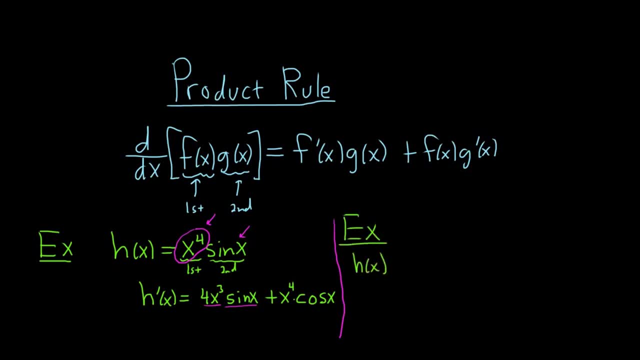 How about h of x equals? oh, I don't know. let's do x squared times tangent x. So again, this is the first and this is the second piece. So taking the derivative of h, so h prime of x. 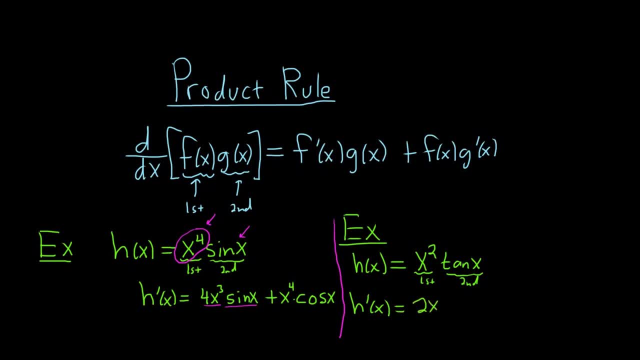 it's the derivative of the first, so 2x times the second, so tangent x plus the first, so x squared times the derivative of tangent which is secant, squared right. Remember the derivative of the tangent function. 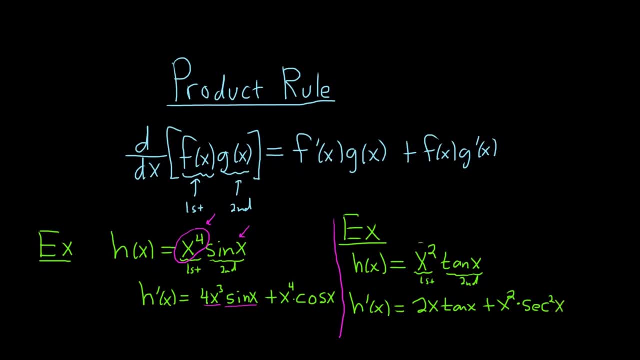 is secant squared. Let's check our work. So it's the derivative of the first, which is 2x times the second, which is tangent, plus the first, which is x squared times the derivative of the tangent function. 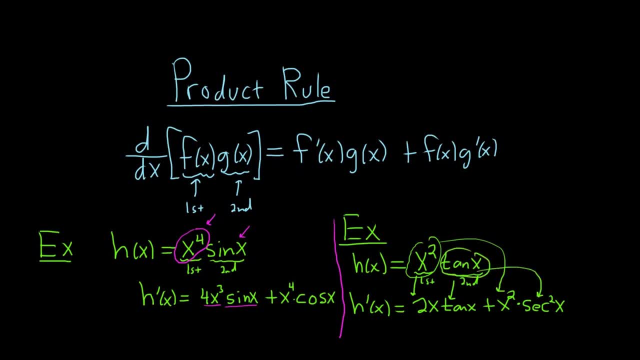 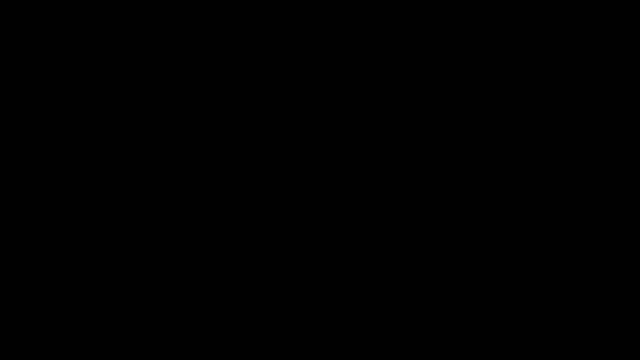 which is secant squared. And that's it. That's the product rule. I hope this video has been helpful. Hi everyone, In this video we're going to talk about the quotient rule. So quotient rule, So the quotient rule is a rule. 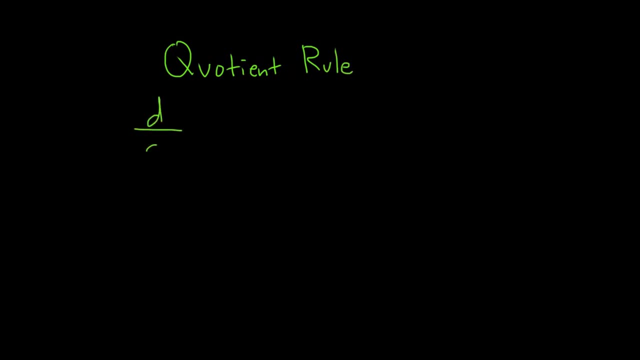 that tells you how to compute the derivative of a quotient or a fraction. So if you have the derivative of f of x over g of x, So here is how you do it. So I think of f as the top, or first, and g as the bottom. 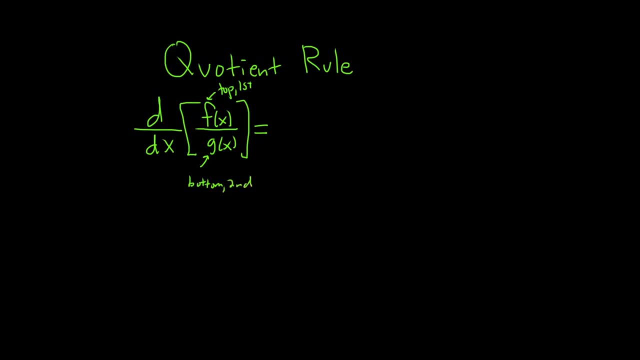 or the second. And so the quotient rule says you take the derivative of the first or the top times the second minus the first times the derivative of the second or the bottom piece all over the bottom one squared. So that is the quotient rule. 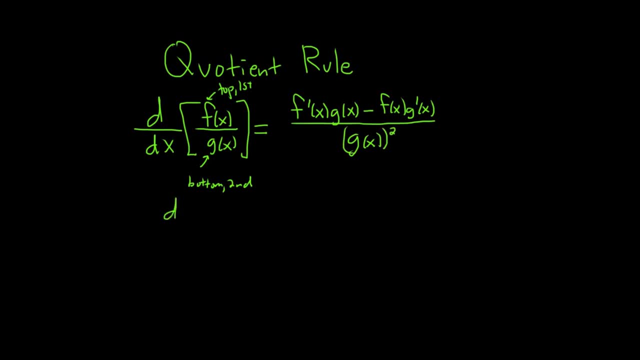 Let's briefly recall the product rule. So if you look at the product rule that tells you the derivative of f of x times g of x And look at this, Look how related this is If you think of this as the first. 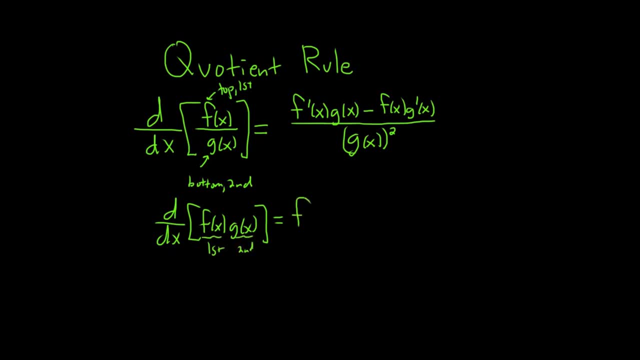 and this as the second. it's the derivative of the first times, the second plus the first times the derivative of the second. So you see, it's almost the same. The only difference is in the quotient rule. you have a minus and you're dividing by the g squared. 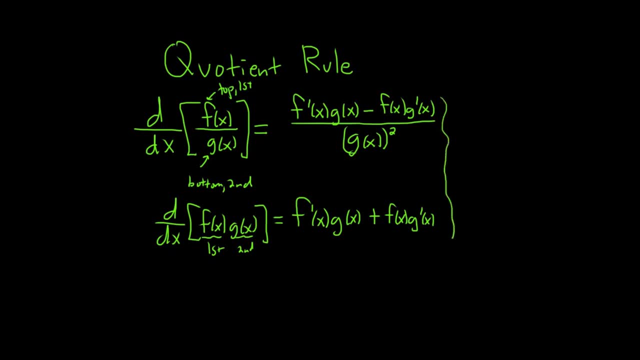 So that's the reason I do it this way. When I say that, I say that because if you look in most textbooks, they might do it a little bit differently, Like they might put the g prime here or something like that. It's the same thing. 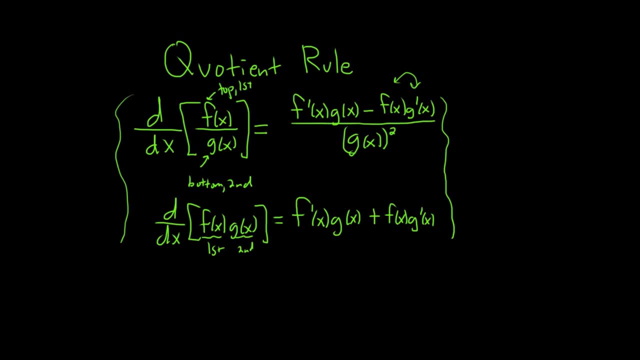 I like doing it this way because it matches right. It almost looks the same, so it's much easier to remember if you do it this way. Let's do an example of the quotient rule so you see how it works. It's actually not too bad. 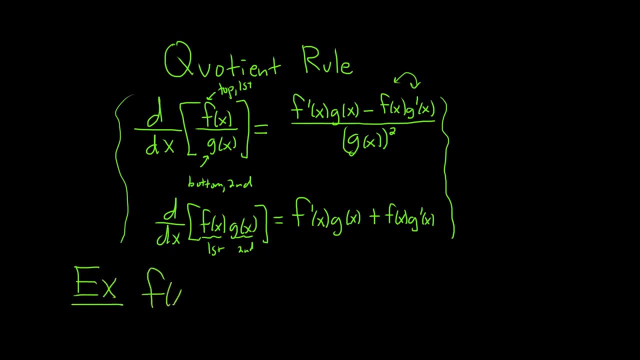 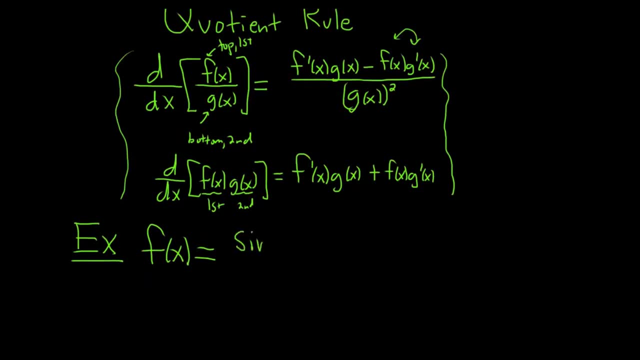 So say, we have f of x equal to- I don't know, let's keep it simple: sine x over x, And so we're going to use the quotient rule. So f prime of x. So let's see, So this is our top piece. 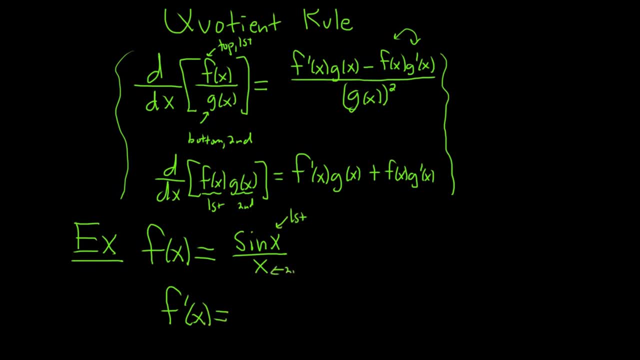 or our first piece and this is our bottom piece or our second piece. So it's going to be the derivative of the first or the top piece. So the derivative of sine is cosine times the bottom piece, so times x minus the top. 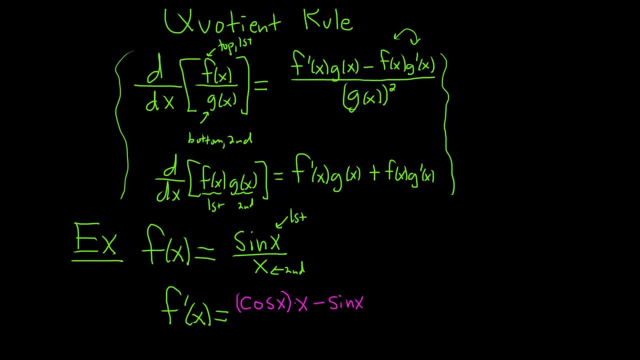 so sine x times the derivative of the bottom piece. Well, the derivative of the bottom piece is 1, all divided by the bottom piece squared. Let's go over that again. So it's the derivative of the top which is cosine. 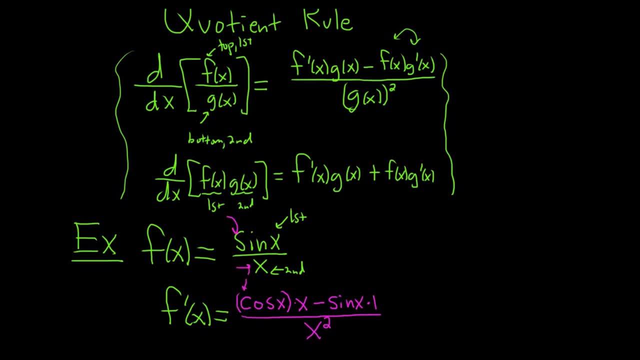 times the bottom, which is x, minus the top, which is sine, times the derivative of the bottom, which is 1,. all over the bottom, 1 squared. The last thing to do is maybe rewrite this, make it look a little bit better. 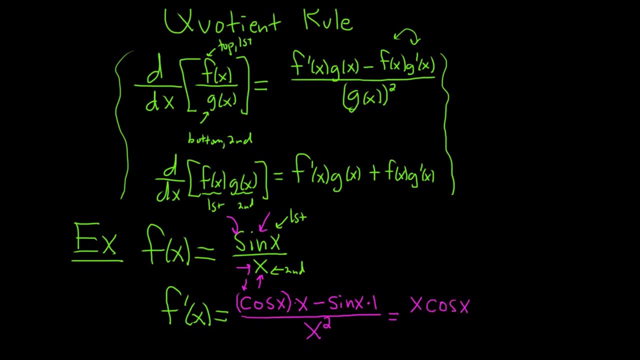 Typically you put the x in front of the cosine function so that there's no confusion between these x's here. Minus and sine x times 1 is simply sine x. That's all being divided by x squared, And that is the final answer. 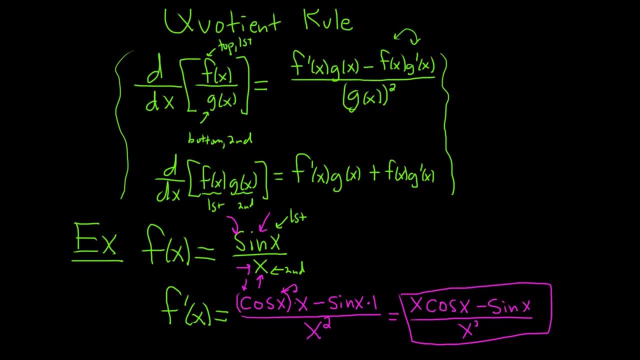 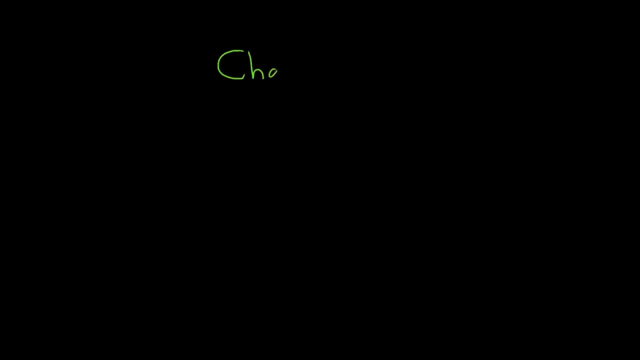 So that's it. I hope this video has been helpful. In this video we're going to talk about a very important rule in calculus. It's called the chain rule, So chain rule. The chain rule gives us a formula for the derivative of a composition of functions. 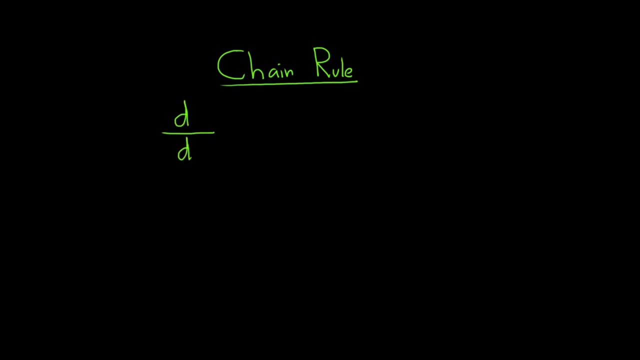 So it says: if you have d, dx the derivative with respect to x, of f, of g of x. So how do you use the chain rule and how do you memorize it? Well, you want to think of f as your outside function. 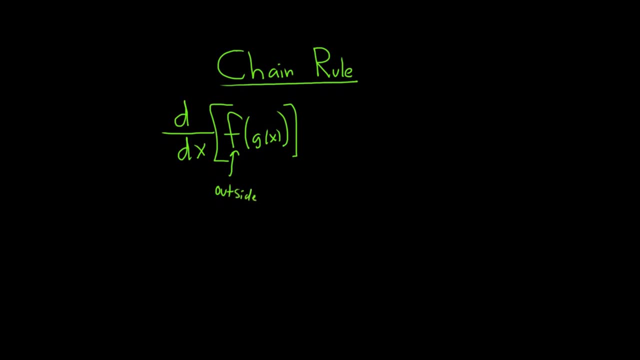 So outside, And then g is your inside function, So inside, And so the chain rule says that when you take this derivative, it's the derivative of the outside Evaluated at the inside, So you leave the inside untouched: It's the derivative of the outside. 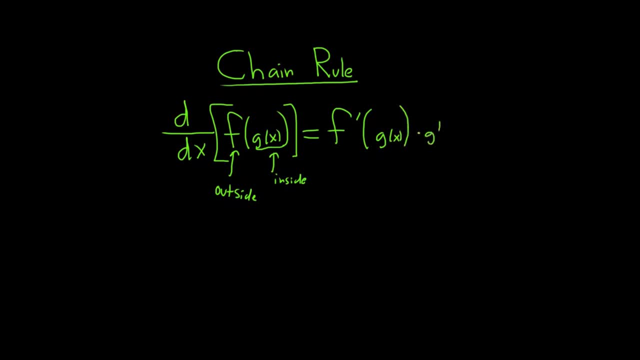 evaluated at the inside times, the derivative of the inside function. And that is the chain rule. So it's the derivative of the outside, evaluated at the inside times, the derivative of the inside. Let's do a couple examples of the chain rule. Say we have to take the derivative. 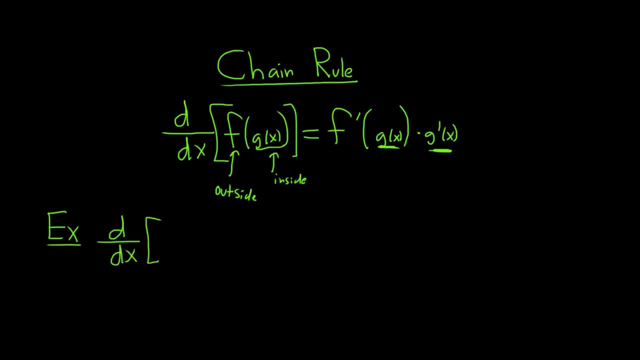 with respect to x. Let's do sine of, let's say, x cubed. Find the derivative of this with respect to x. So if it was just sine x, the answer would be cosine x, But here it's sine of x cubed. 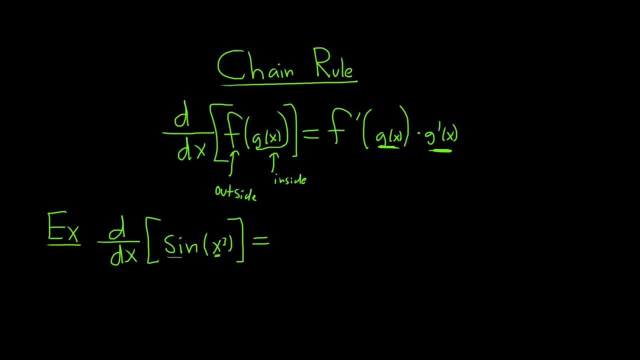 So the inside function is x cubed. Your outside function is sine x. So the derivative of sine is cosine. And then you evaluate it at the inside. You leave the inside untouched. So cosine of x cubed times the derivative of the inside 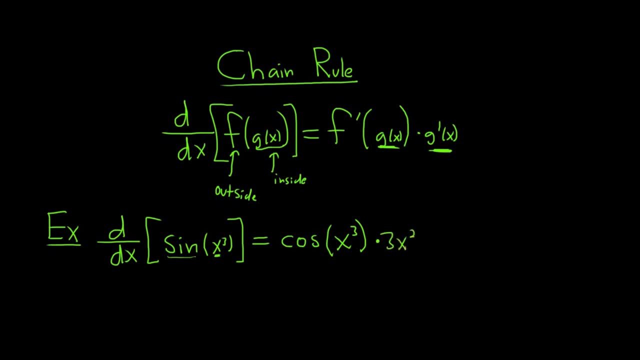 The derivative of x cubed is 3x squared. Again, it's the derivative of the outside, which is cosine evaluated at the inside times. the derivative of the inside. It's beautiful stuff. Last thing you could do is put the 3x squared in the front. 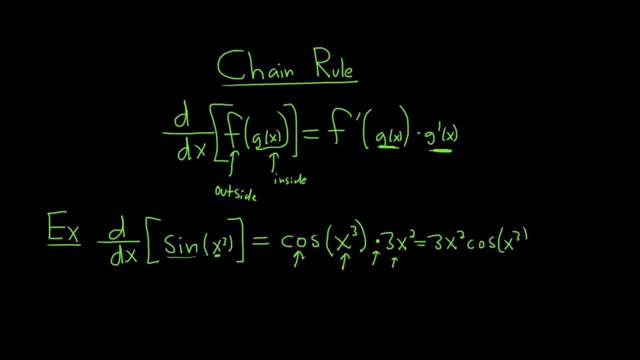 So it's 3x squared times the cosine of x cubed. Let's do another one, ddx of. and it's fun to practice these with trig functions. Let's try. oh, let's backtrack. Let's do that. Sine x. 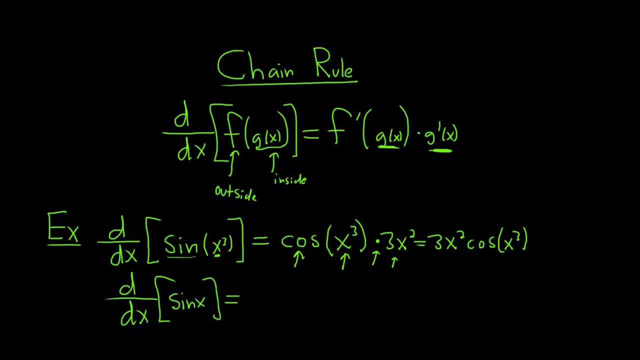 Well, we know the answer is cosine x. But let's be silly. Sometimes it's good to be silly. Let's take the derivative using the chain rule. So the inside function is x, So leave it untouched. So the derivative of the outside is cosine. 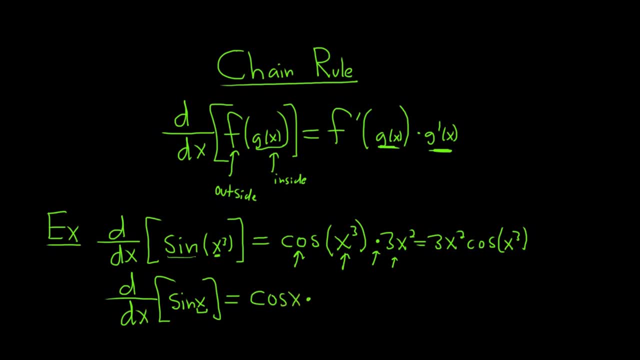 So the derivative of x, evaluated at the inside times, the derivative of the inside, Well, the derivative of x is 1.. Boom. So this is just cosine x. So it agrees with our formula. So life is good. Let's do another one. 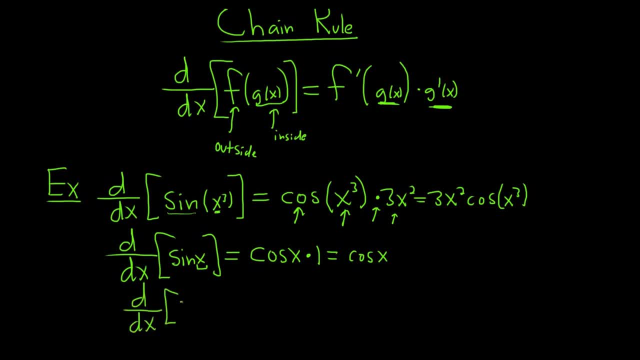 ddx, ddx. Let's make it uncomfortable. Secant of 2x, So the derivative of secant is secant tangent, So in this case it would be secant 2x. This is what makes it uncomfortable. 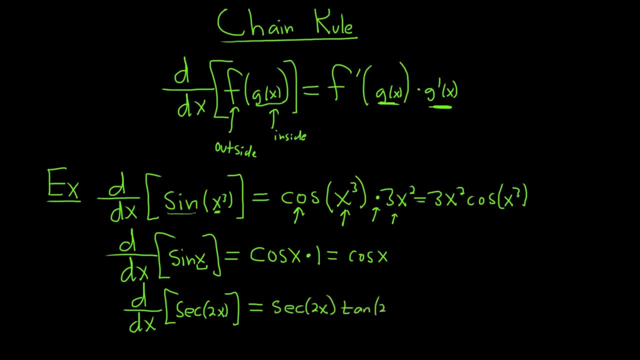 You have to write it twice. Tangent of 2x times the derivative of the inside. The inside function is 2x, So its derivative is 2.. So again, the derivative of secant is secant tangent, So here it's secant 2x. 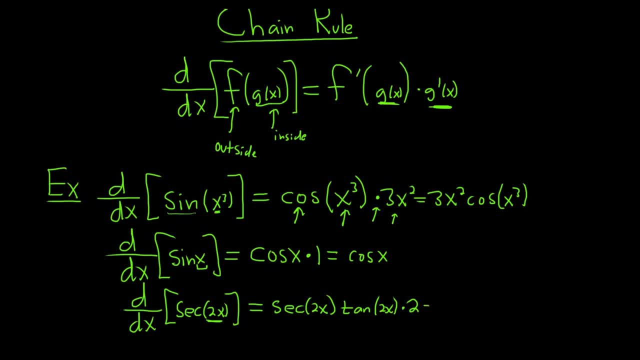 So it's secant 2x, tangent 2x times the derivative of the inside. So this is 2. Secant 2x- 2x, tangent 2x. Let's do another one. Why not ddx? 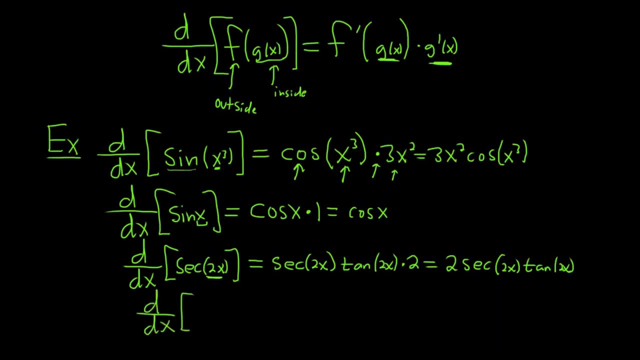 ddx of: Let's do something without a trig function. Here we go: x cubed plus 2 to the eighth Yuck. So our outside function is something to the eighth power. So this is the inside: x cubed plus 2.. 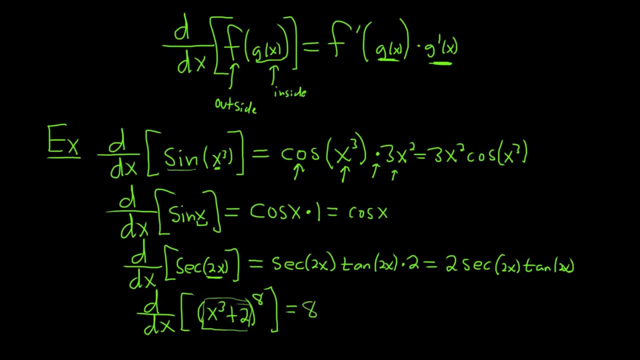 So we leave the inside untouched. We put the eight in the front. We have x cubed plus 2.. Subtract one So we get seven. That's the power rule, right Times the derivative of the inside, So 3x squared. 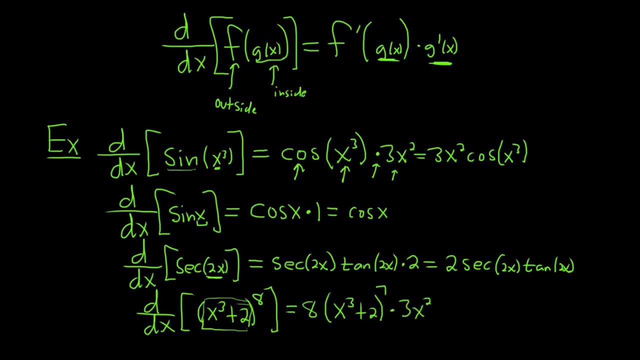 Again, we took the derivative of the outside, Brought the eight down, Subtracted one, Got seven, Left the inside untouched. Then times the derivative of the inside, 3x squared times eight, is 24x squared. Then we have x cubed plus 2.. 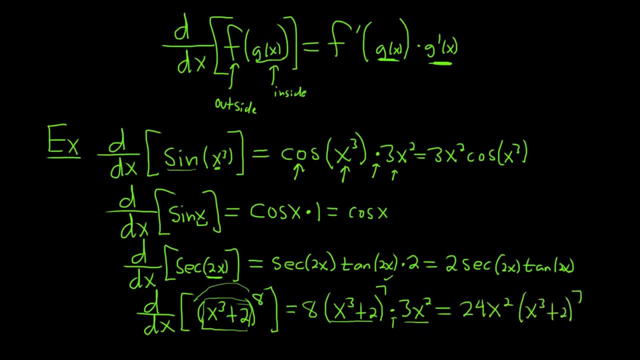 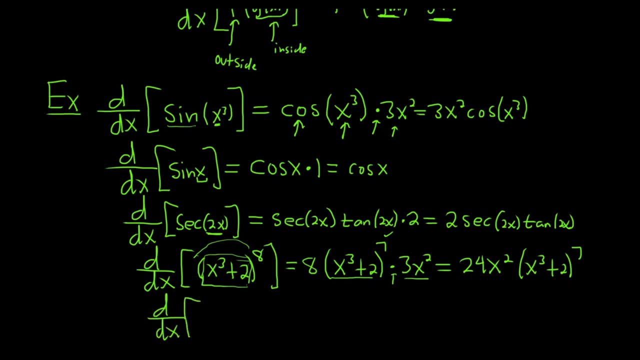 Subtract one Plus 2 to the seventh, Let's do another one. I love the chain rule, ddx, ddx. My favorite rule out of the product quotient and chain Chain is really the best one in my opinion. Oh, I don't know. 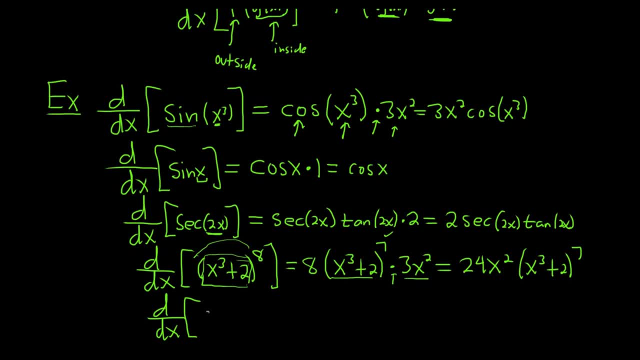 Oh, I know what we can do. I have a great idea. Let's do the sine. Let's have some fun. Let's do the sine of the tangent of x Game over. So let's mix it up. So the inside function is tangent of x. 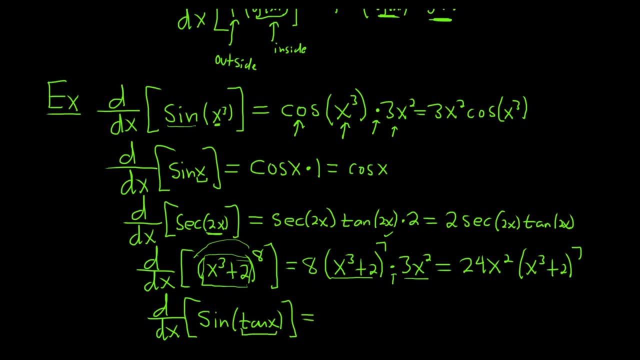 The outside function is sine of x. So we take the derivative of sine, which is cosine, We leave the inside untouched. So cosine of the tangent of x times the derivative of the inside. Well, the inside function is tangent, So its derivative is secant squared x. 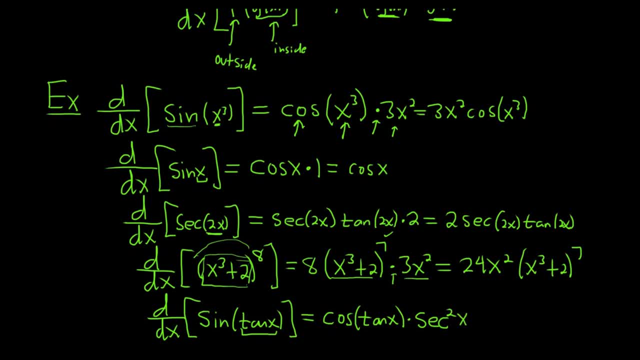 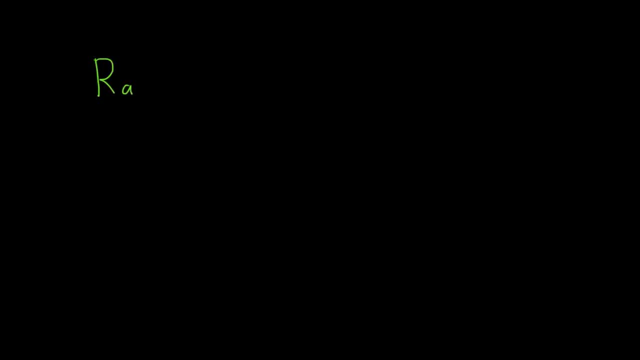 I think that's good. I hope this video has been helpful. That's it, Hi everyone. In this video we're going to talk about rates of change. So rates of change, And we're carefully going to go through a construction and do a simple example. 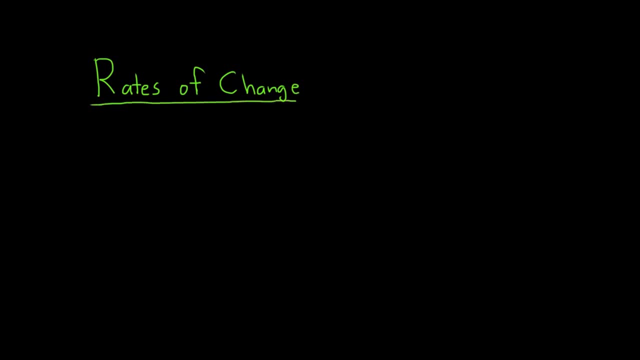 So rates of change. So we'll start with a function which we'll call f of x, So we're going to let y be equal to f of x And we're going to define something called the average rate of change. So the average rate of change. 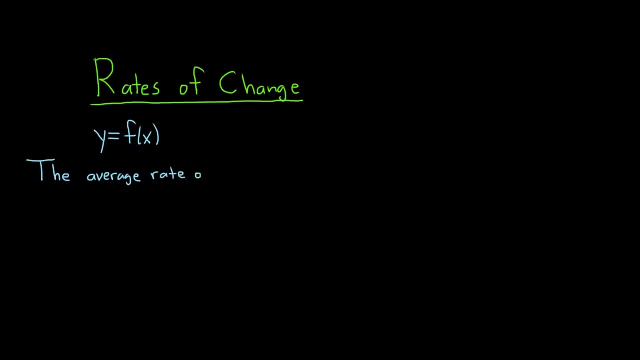 So average rate of change, So the average rate of change of a function. So our function here is f of x over an interval. So we're going to define it over. ab is well, it's the change in y over the change in x. 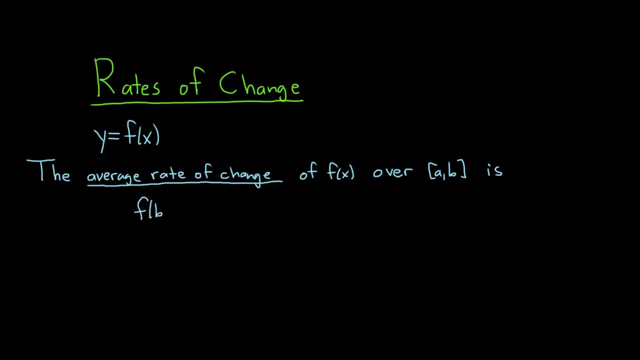 So it's f of b minus f of a. These are the y values. Remember, y is equal to f of x over. And then there's a really easy way to memorize the formula: You just use matching. There's a, b up there. 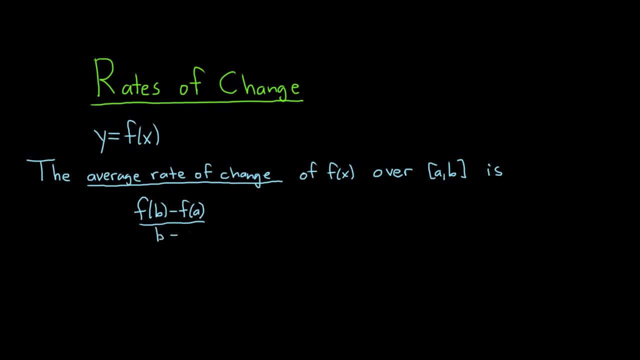 So you put a b down there And then minus, And there's an a up there. So you put an a on the bottom. So again, this is the change in y. Let me write down what I said in words: Change in y over the change in x. 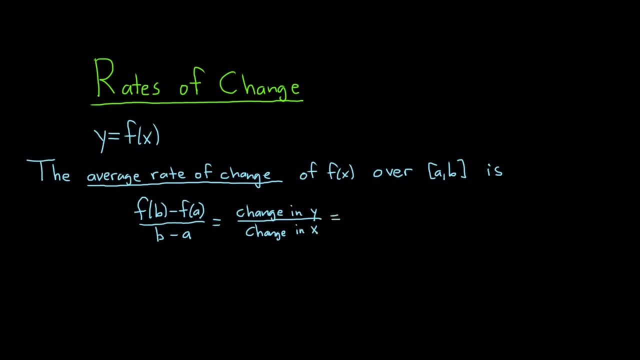 Okay, So you can think of the change in y as delta y, That's the Greek letter delta, And then over delta x, That's the change in x. It's a triangle, It's called delta. Let's change it up a little bit. 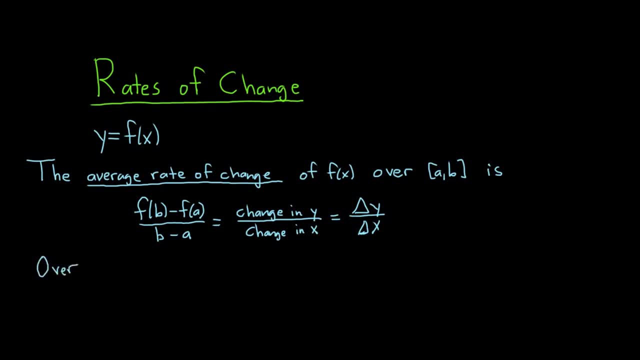 So over, say, we consider the interval x to x plus delta x, So x plus a little bit more Right. So some change. These are different numbers Then using the above formula we have. So this is kind of interesting. This is f worth seeing. 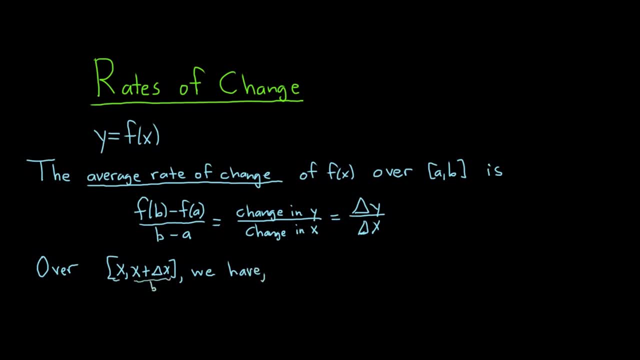 So instead of b. So this is our b, now Right, And this is our a, So it will be. Let me use a different color. This will be f of b, So it's x plus delta, x minus f of x over. 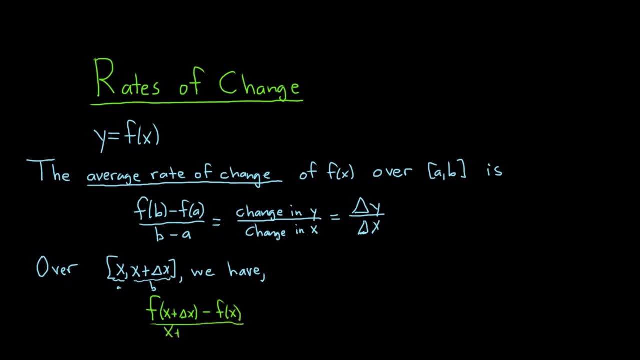 And on the bottom You just use matching, Right, So it's x plus delta x, And the magic happens- Minus x And the x's cancel, Right, So you just get f of x plus delta x, minus f of x. 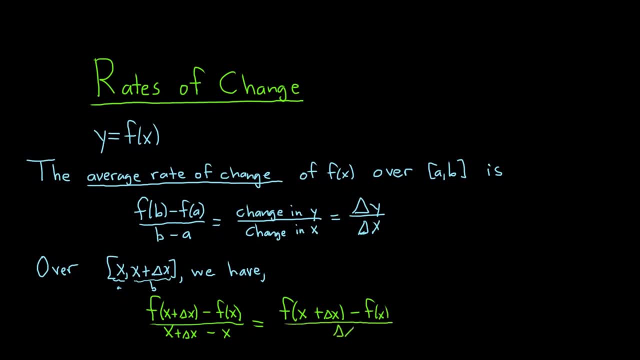 All divided by delta x Right. And again, you can think of this as the change in y Delta y over the change in x Delta x Right. Where, Just to be really pro and precise, Where delta y is the numerator. 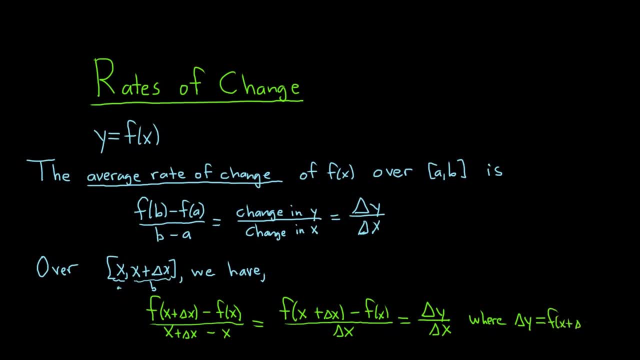 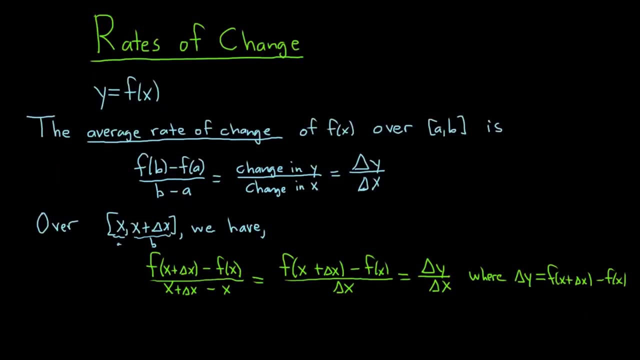 Right. So it's f of x plus delta, x minus f of x Right, Being really formal here And careful with our definitions. So what are we doing Is we're constructing something very important in calculus And we're about to do it. 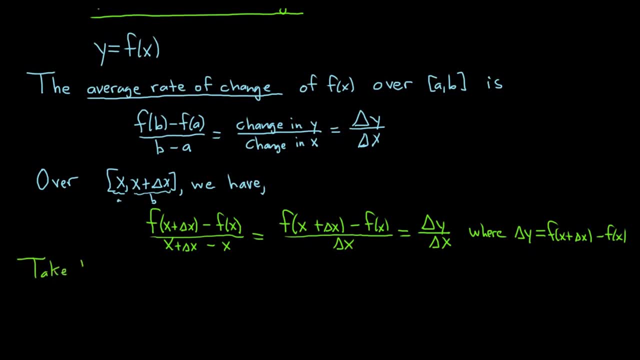 So we take the limit, So take the limit, Take the limit. And typically what we do in calculus: We construct something And we take the limit, And then we call it something else. We get. We get what's called the. 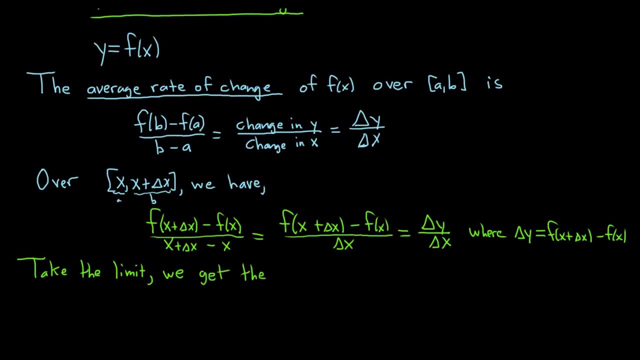 Here's a big word, Make sure I spell it right: The instantaneous rate of change. So instantaneous, Instantaneous Rate Of Change. We get the instantaneous Rate of change, The rate of change at a particular instant in time. 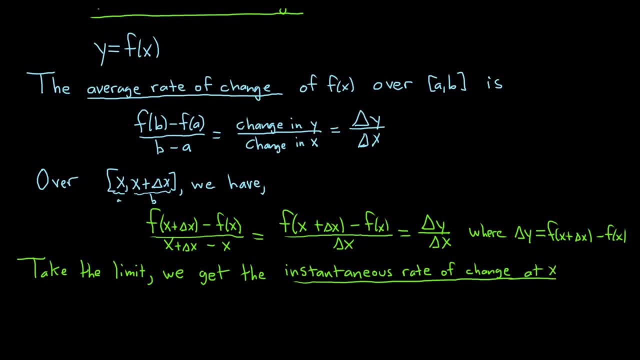 At x. And so when you take this limit, If you recall, This is the, This is the difference quotient, Right. So is this one Right? They're both difference quotients, They're both slopes of secant lines, Right. 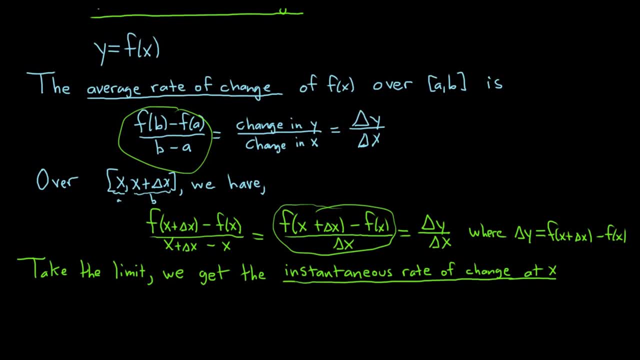 So when you take the limit of the slope of the secant line You get the derivative. So F at x Is also The instantaneous rate of change of the function. at x It's the limit of the average rate of change. 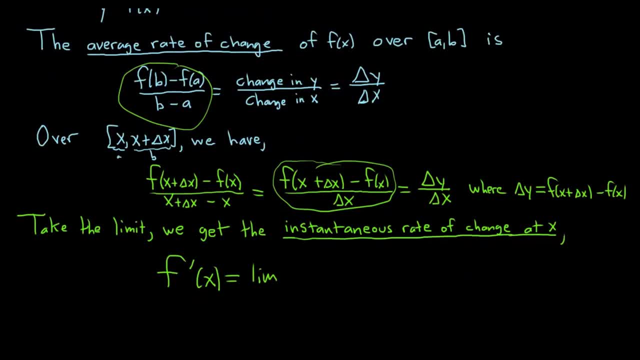 This is the limit, As Delta x Approaches zero Of f Of x plus delta x, Minus f of x. All over, All over delta x. Okay, And you can define it multiple ways. You can use h. 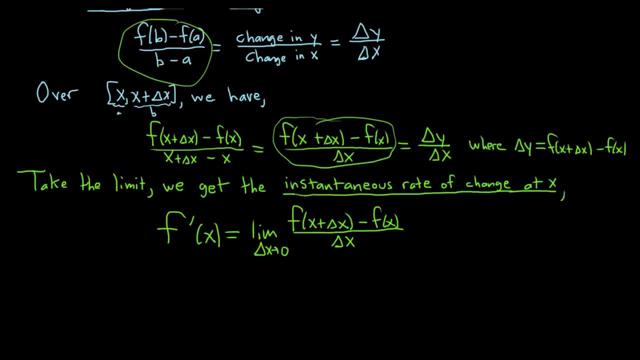 If you like, Or You can do it at c, Let's, Let's do it for this one up here. So Another way to do it Would Would be to say: Or at c, The other definition of the derivative. 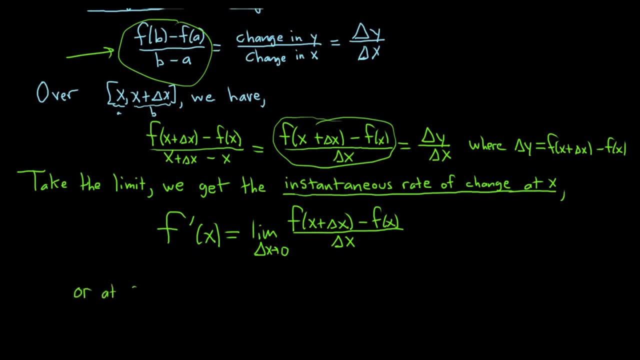 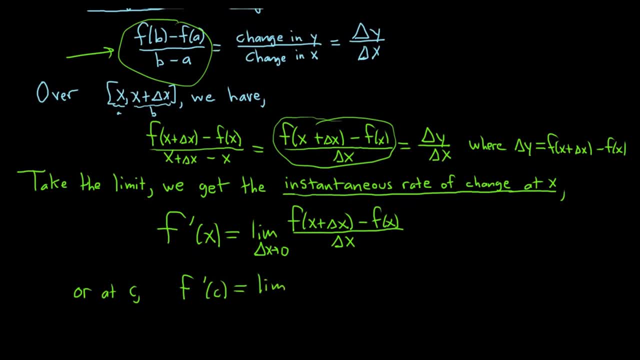 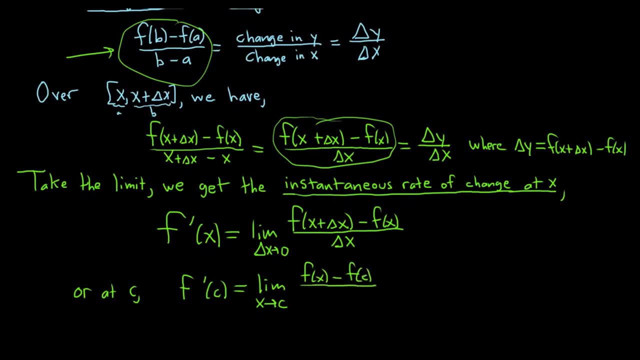 If you want to. If you want to, x approaches c Of f of x Minus f of c. It's not used often, But I wanted to write it for completeness, So you have As much knowledge as possible. Or 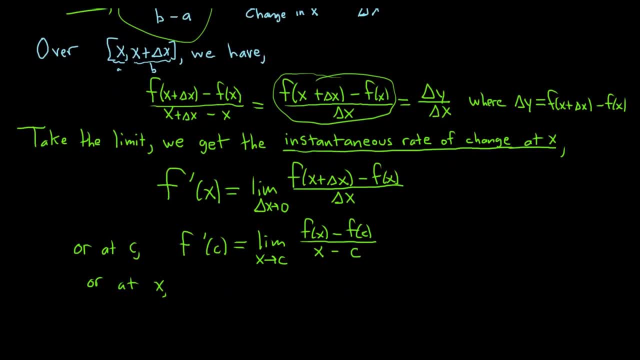 At x. Let's do it at x again. And let's do it a more nice way: F. prime of x. Instead of using delta x, You Can use h. So Instead of letting delta x go to zero, We let h go to zero. 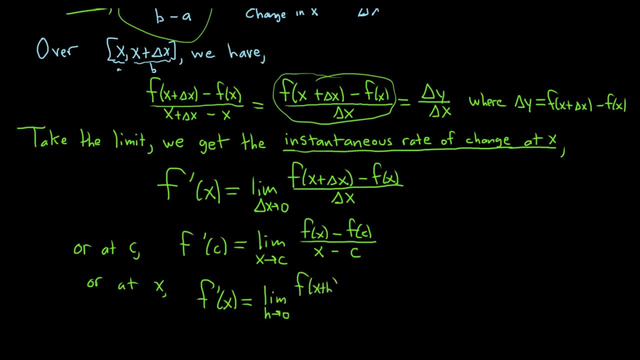 And so we write f of x, X plus H, minus F of X all over H. So that's the one I like, That's the one we typically use when we're finding the derivative, using the definition, et cetera. So just to give you the motivation here. 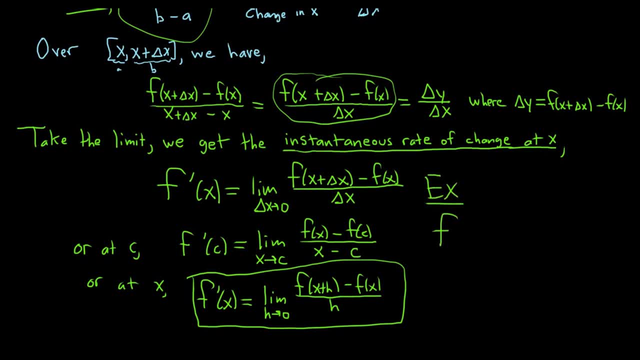 so what is a derivative? It's a rate of change, So like if you had F of T and this told you the temperature at time T. the derivative is how fast your temperature is changing with respect to time. So F, prime of T is the instantaneous, so instantaneous. 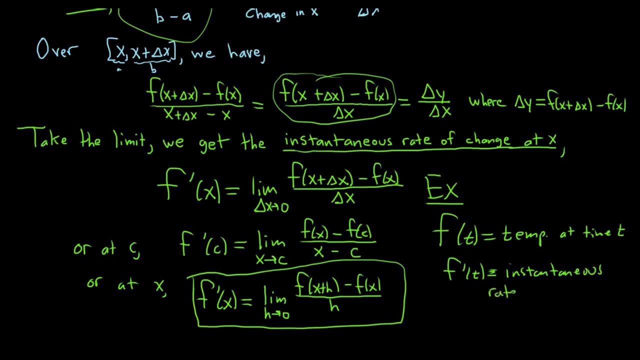 instantaneous rate of change. so rate of change at time T. So all theory, no examples. Maybe in the next video we'll do some examples of finding some average and instantaneous rate of change. I just wanted to construct it. So basically you take the slope of the secant line. 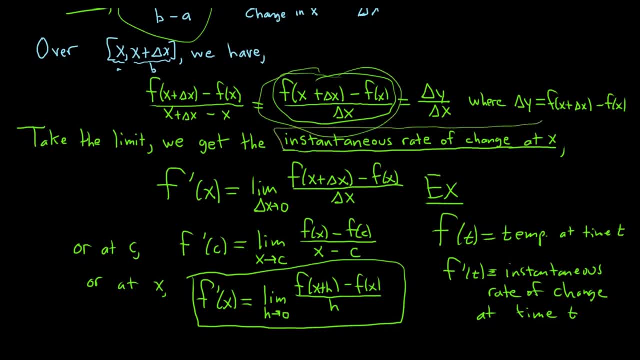 and you take the limit, and so all we're saying is that the derivative is now the instantaneous rate of change. And where does it come from? It's the limit of the average rate of change. That's it. In this video, we're given a function. 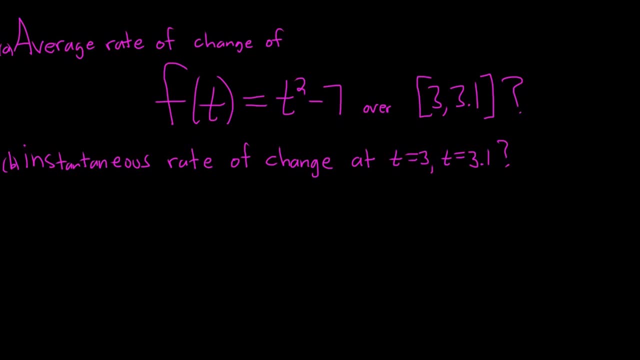 and we're being asked to find the average rate of change of the function over the interval 3 comma 3.1.. And we're being asked to find the instantaneous rate of change at the end points. so at T equals 3 and at T equals 3.1.. 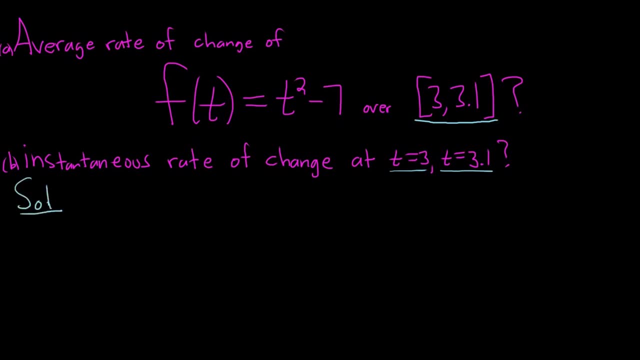 Let's go ahead and work this out. So solution. So part A: we have to use the formula for the average rate of change. Recall that the average rate of change of a function over the interval bracket A to B is given by the following formula: so it's F. 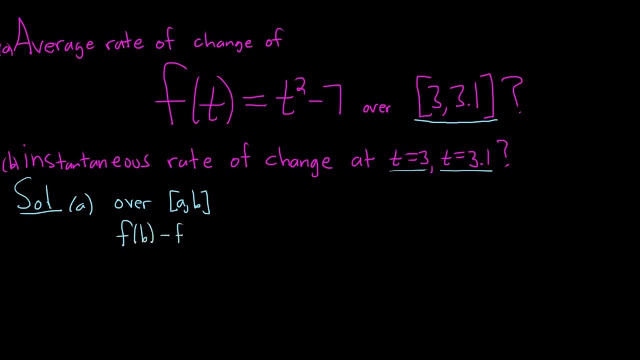 of B minus F, of A over B minus A. This is the formula for the average rate of change. So in this problem our A is 3 and our B is 3.1. So all we have to do is plug in those numbers. 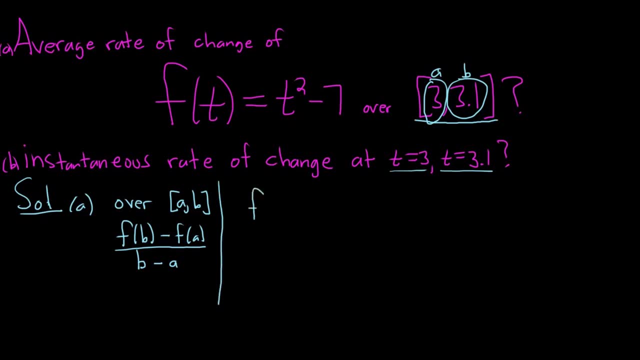 So we will have- I'll do it over here- of 3.1 minus f of 3, so that's b minus a f of b minus f of a over, and then you just match them. so 3.1 minus 3.. Just use matching. it's really easy to memorize the formula if 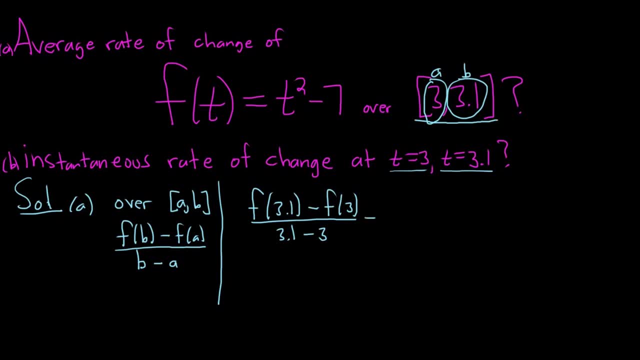 you just match the numbers, Okay. so f of 3.1 means you put a 3.1 where the t is right, So it'll be 3.1, parentheses squared, then minus 7, so that's f of 3.1 minus and then. 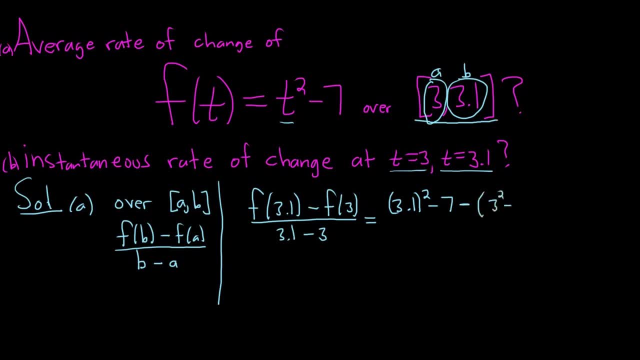 parentheses- 3 squared minus 7, right, So this is the first piece f of 3.1, and this is the second piece f of 3, over 3.1 minus 3,, which is just .1.. Okay, so this is equal. 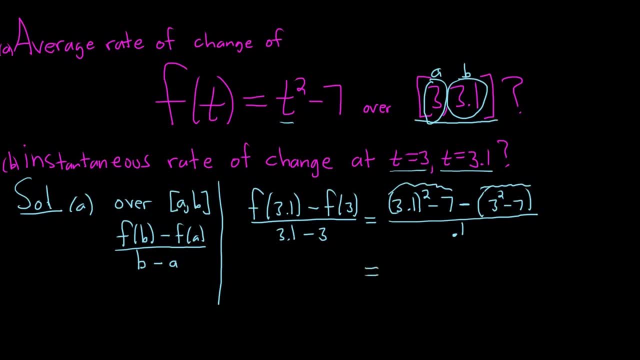 to. so I have a calculator here. let's see if it works. it does hurrah, So I'm going to plug it into my calculator. I haven't done this problem yet, So for the first expression here I got 2.61.. 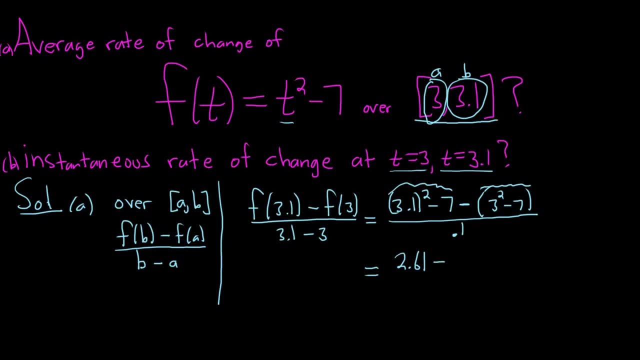 Minus, and this will be 9 minus 2, so 9 minus 7,. sorry, this is 9 minus 7,, so it's 2,, so 2 over .1.. So we end up with .61 over .1, and .61 divided by .1,, that's 6.1.. So we 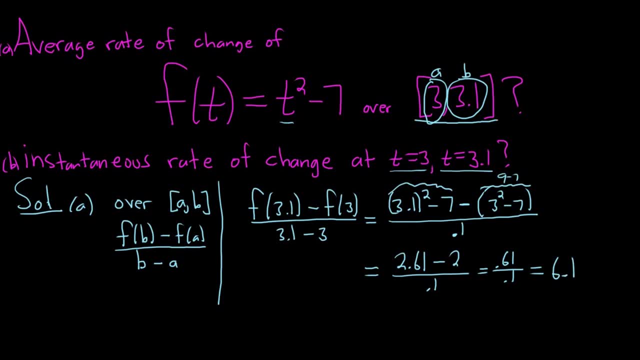 end up with 6.1 as our average rate of change. So that's part a. Part b wants the instantaneous rate of change at the m-points. So the instantaneous rate of change is just the derivative. it's the same thing. So f prime of t, super easy derivative right, Just use the power rule. 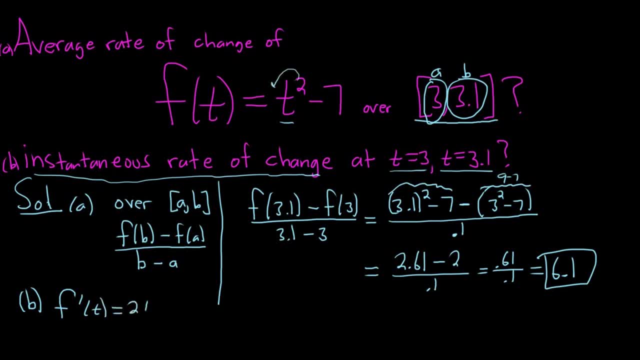 bring down the 2, so you just get 2t and the derivative of negative 7 is 0. So I won't bother to write it. So this is the instantaneous rate of change at t. We want it at 3 and at. 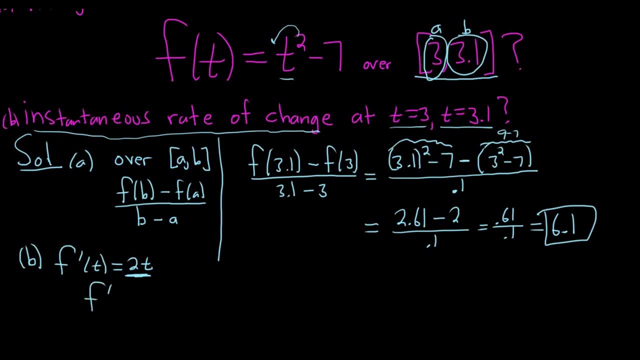 3.1.. So let's do it So. f prime of 3, this is the instantaneous rate of change at t. three is two times three, which is equal to six. that's the instantaneous rate of change at three. and then f prime of 3.1. it's two times 3.1, it's going to be 6.2. 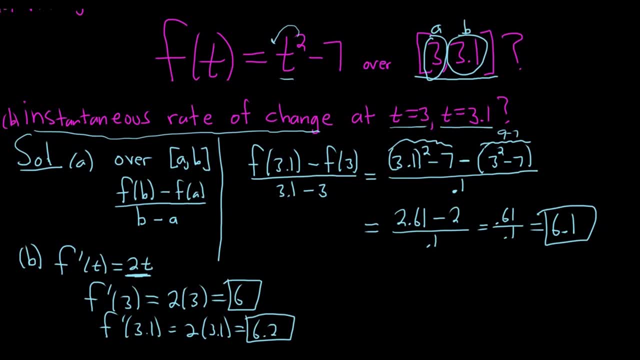 that's the instantaneous rate of change at 3.1. notice it's very close to the average rate of change. why? because this interval is so small, right, I mean, it's really really small. you're looking at a very, very tiny point. normally the average rate of change- well, normally it always is. it's the slope of this line. 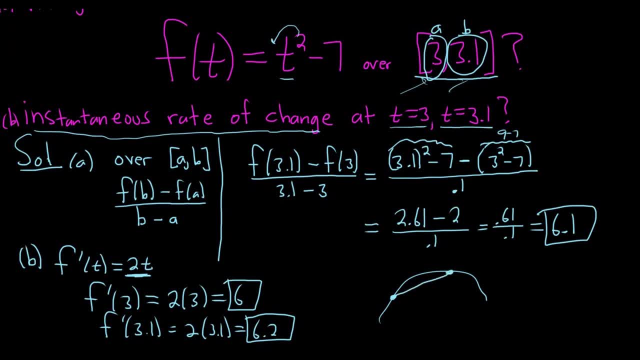 right, it's the slope of this line here. so if you, if you make the interval really small, what happens is it just? I can't even draw it. it's so small, it looks like that. so it's almost like the tangent line right, the slope of the. 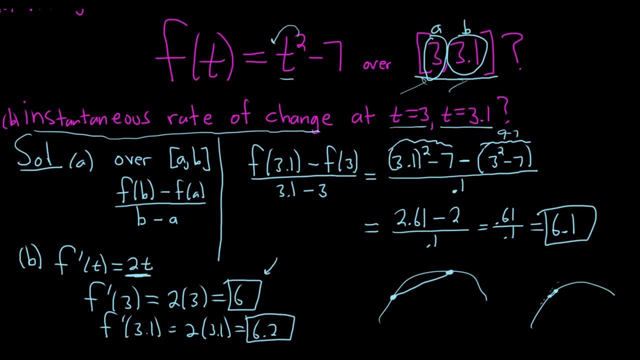 tangent line is the instantaneous rate of change. the slope of the secant line is the average rate of change. so if you make the interval small, your secant line is almost your tangent line. that's what's happened in this problem, right? that's why these numbers are so close to the 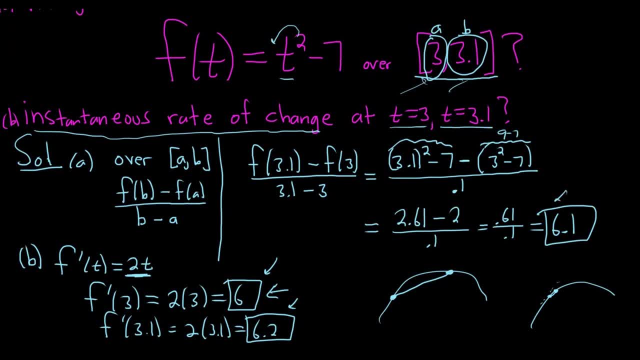 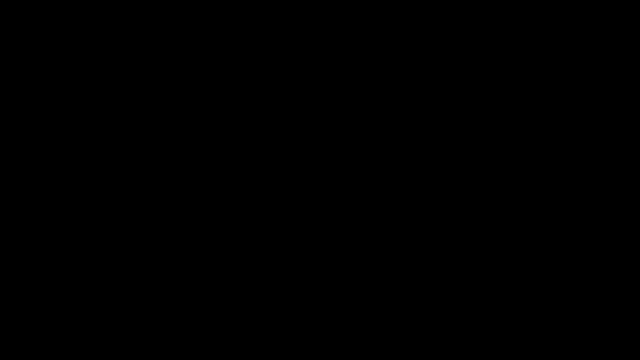 average rate of change. I hope this video has helped in some way. that's it, hi everyone. in this video we're going to introduce the notions of velocity and acceleration, so the setup is as follows: we will start by letting so let s of T, so s here is a function of time, and this will be the position. 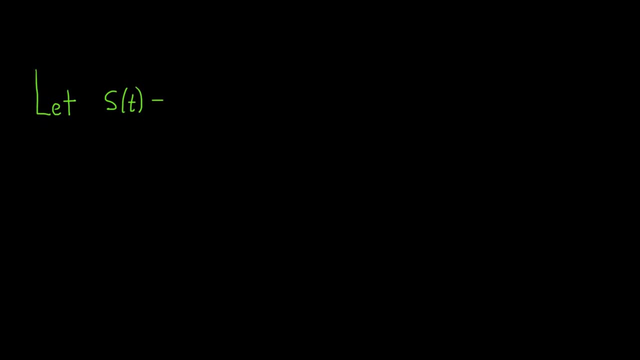 function of an object at time T, so this is the function, so position. put this in quotes: position: function of an object. so of an object at time t, so at time t. t can be in seconds or in minutes, depends on the question. 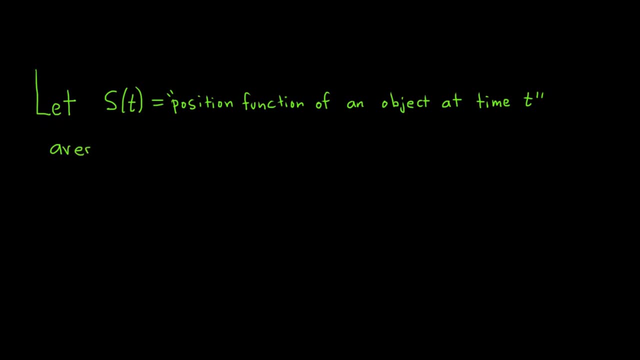 So the average velocity is going to be defined, just like the average rate of change, So the average velocity over a b, so over a b. well, if you recall, the average rate of change was f of b minus f of a, Over b minus a. 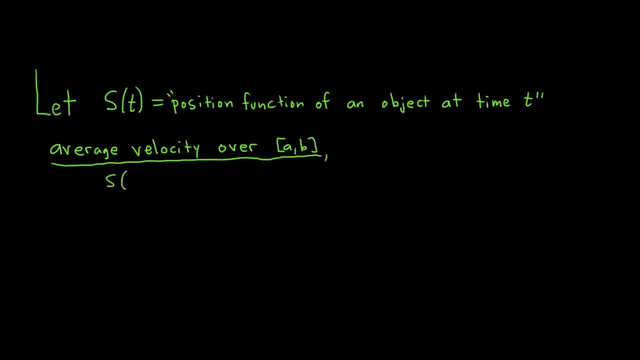 So here it's s, not f, so it's s of b minus s of a, over b minus a Or over a different interval, let's say over. say instead we take it over the interval t, t plus delta t, we would get s of t plus delta t minus s of t. 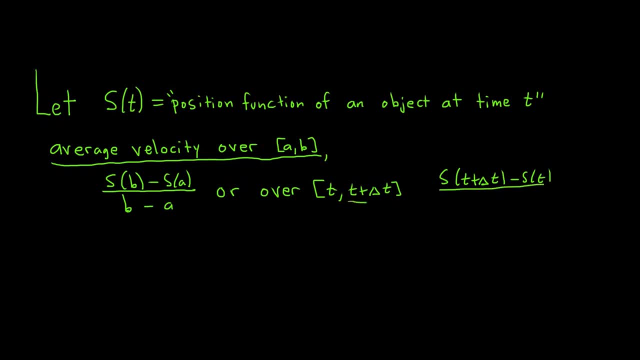 And then on the bottom, you subtract this minus this, so the t's cancel and you just get delta t. So remember, we did this before when we were constructing instantaneous rate of change. So what you do is you take the limit. so take the limit, take the limit. 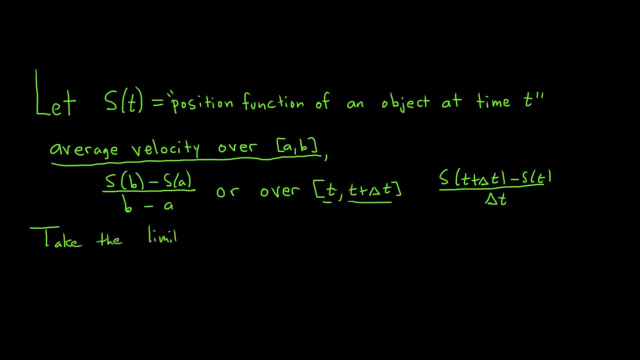 and you get the derivative right. So the limit is the derivative. So s prime of t is equal to the limit as delta t approaches 0 of s of t plus delta t. It's really scary. All the deltas make it look really frightening. 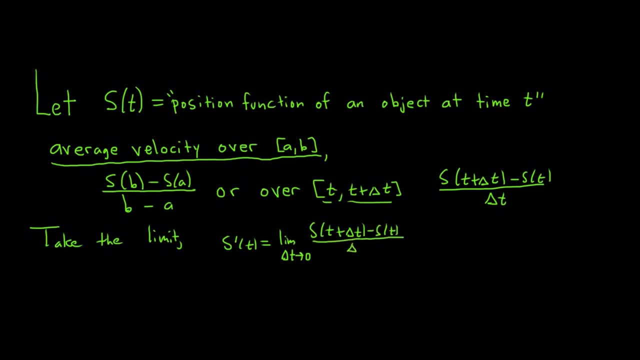 Over or beautiful right. So it's a matter of perspective. So the derivative of position is the limit of the average velocity, And so this is just called the velocity. So this is the instantaneous rate of change of the position at time t. 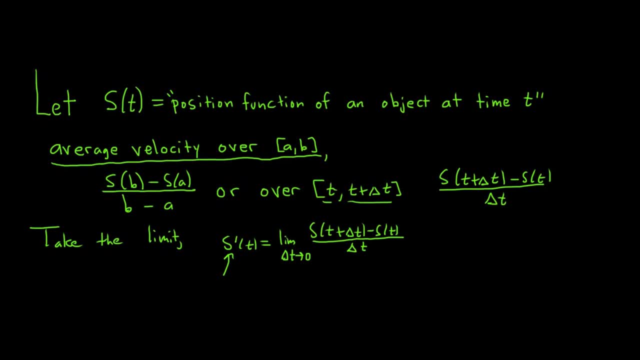 or the derivative of the position, or just, even better, the velocity. This is the velocity at time t. So when we say velocity, we mean instantaneous velocity. Unless we say average velocity, it's assumed to be velocity, So we can give it a new name. 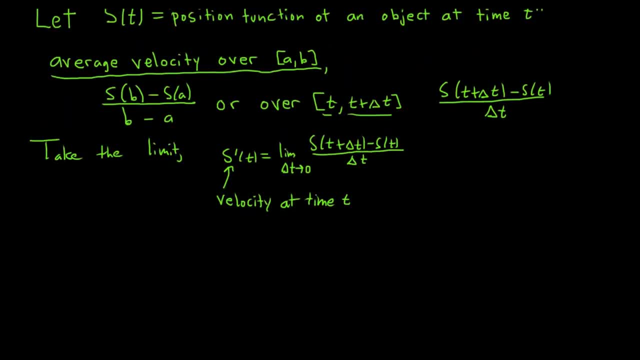 We can call it v, v for velocity, v for velocity. So we can say that s prime of t is equal to v And that will be our velocity at time t at time t. Likewise, the acceleration is defined as the rate of change of the velocity right. 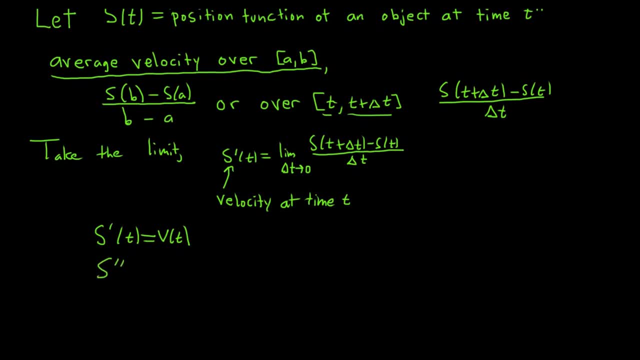 You're either speeding up or slowing down, So it's going to be the second derivative. So the second derivative of position will be the acceleration. so a of t. This is the derivative of velocity, right, The derivative of velocity. Let's recap everything so you have it all in one place. 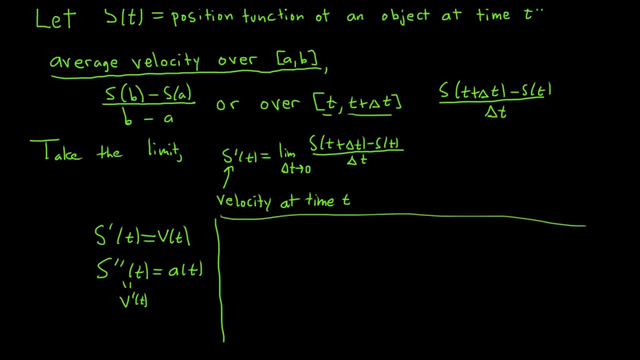 So a recap of everything we've just done quickly. So we have s of t. We know that this is the position function, So this is the position function And we know that v of t is the velocity function And that's equal to s prime of t. 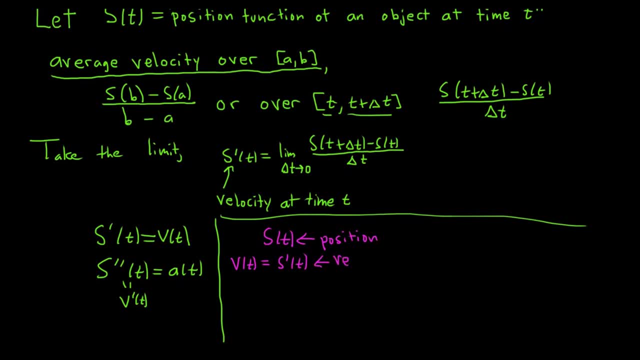 So this is the velocity at time: t. So this is the velocity velocity And we know that a of t is the acceleration. right, That's the acceleration. This is s double prime of t, So this is the acceleration: a, c, c acceleration. okay, 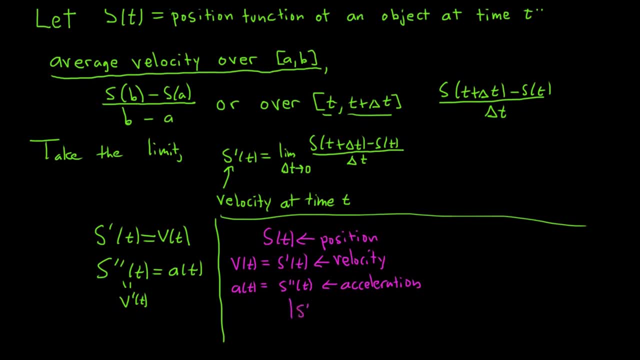 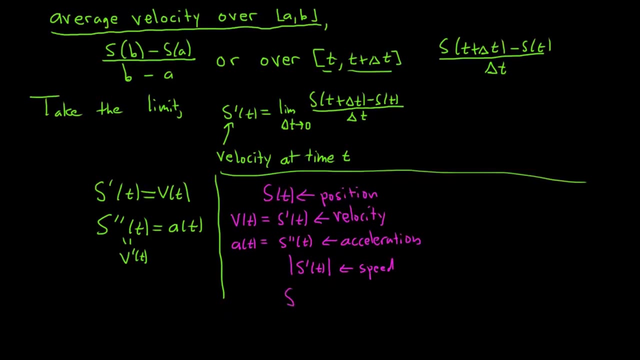 Extra life knowledge. If you take the absolute value of the velocity, that's called speed, okay, Because velocity has a direction. right, Speed is the magnitude or absolute value of that. Also, if you take the third derivative of position: right. 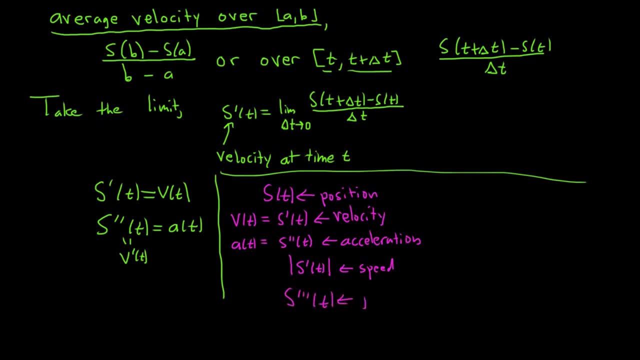 The third derivative of position, you get something kind of funny. It's called the jerk. So it's the rate of change of acceleration. So that's the important stuff, right. So you have a position function. How fast your position is changing with respect to time, that's your velocity. 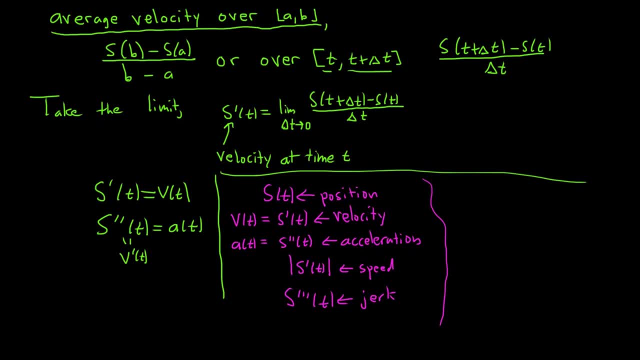 How fast your velocity is changing with respect to time. that's your acceleration. And then you have the magnitude or absolute value of velocity. that's speed. And the third derivative of position, or the derivative of acceleration. same thing is the jerk is the jerk. 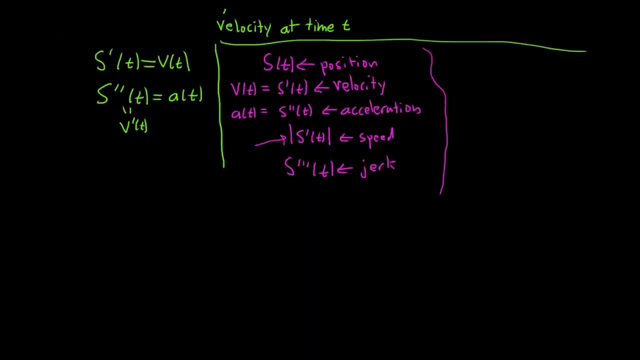 There's a formula that we'll use, that you'll see in some of the problems perhaps, And it's the formula for the position of a free-falling object neglecting air resistance. So the position of a free-falling object Free-falling object neglecting air resistance is: 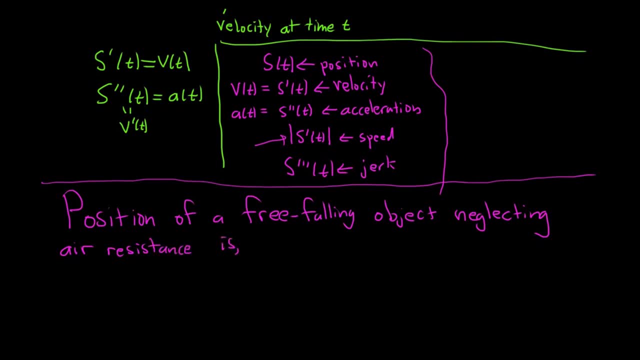 and it's typically given in the problems. You just have to know what everything means, So I'll write it down and then in the next video we'll do an example where we use it. It's 1 half g t squared plus v sub 0 times t plus s sub 0.. 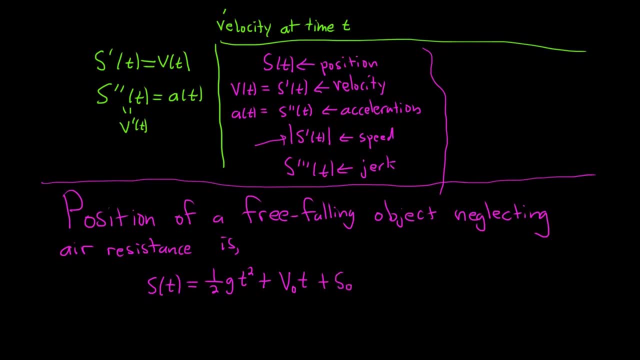 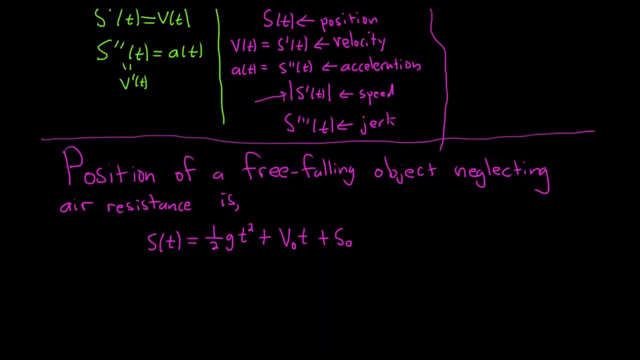 It's also read v naught or s naught. Nought is spelled n-a-u-g-h-t, So physicists often say s naught or s sub 0 works as well. And so what is everything here? Well, g is the acceleration due to gravity. 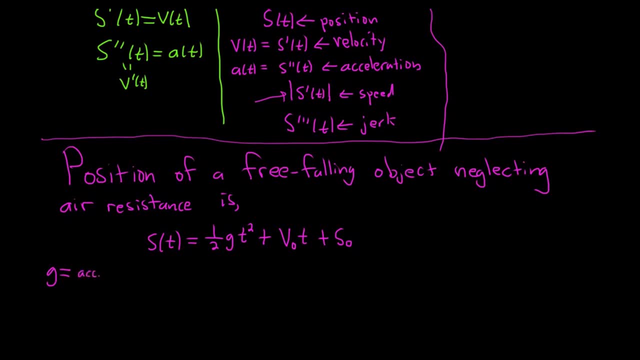 So this is the ACC. Okay, due to gravity, Usually it's going to be plugged in for us in the problems we do. So, like you won't actually see it, Okay, It'll be taken care of. If you know some physics, I'll just tell you anyways. 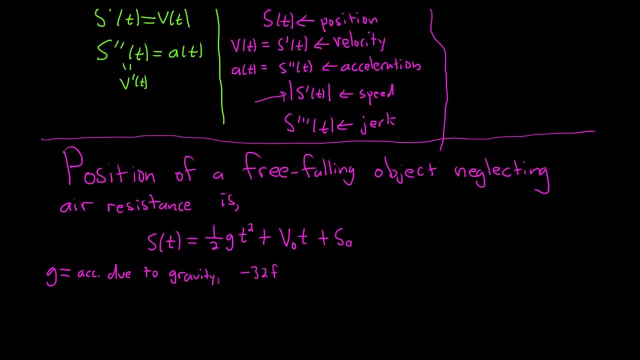 So this will be negative 32 feet per second squared, Or you can write it as negative 9.8 meters per second squared. That's another way to write it: S naught or s sub 0.. This is your initial position. 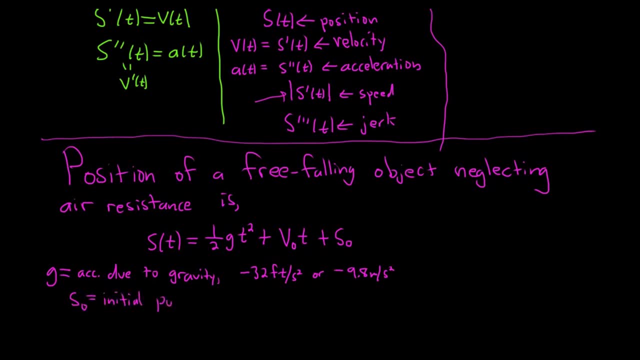 So this is your initial position. So if you're throwing something up from the ground, it's going to be 0.. If you're dropping something from a building, it will be the height of the building, And then v naught. this is your initial velocity. 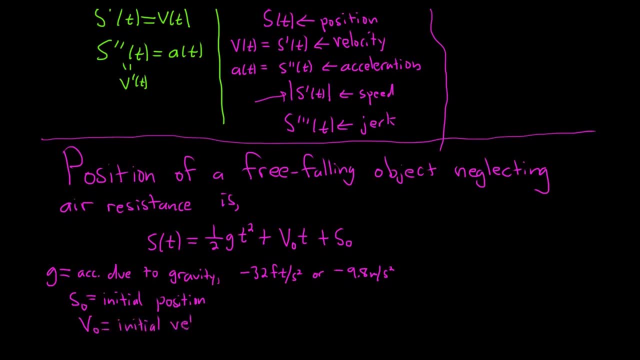 So initial velocity. So if you're dropping something, it's 0.. If you're throwing something, it's going to have a non-zero value. So that's it for now. In the videos that follow you'll see an example or two of how to use this formula and use all of this math. 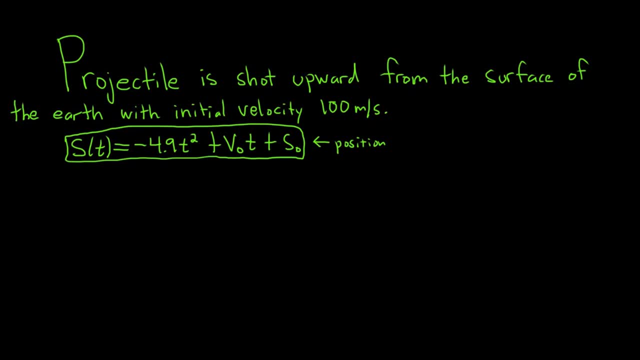 That's it, Hi everyone. In this problem we're going to do a problem involving velocity. So a projectile is shot upward from the surface of the Earth with initial velocity 100 meters per second And we're given the position at time t in meters. 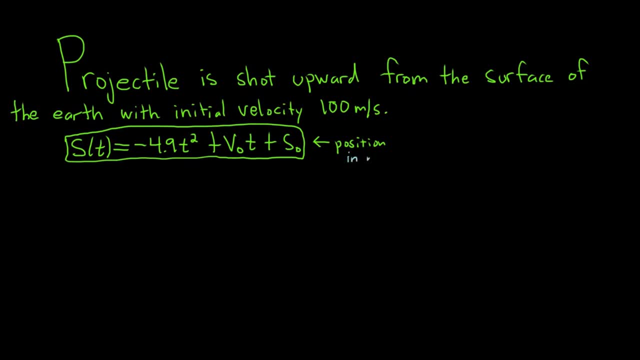 So this is the position- I should write that in meters- of this projectile And we're going to answer various questions. So part A: Let's find the velocity after 2 seconds. So velocity after 2 seconds. So we find the velocity after 2 seconds. 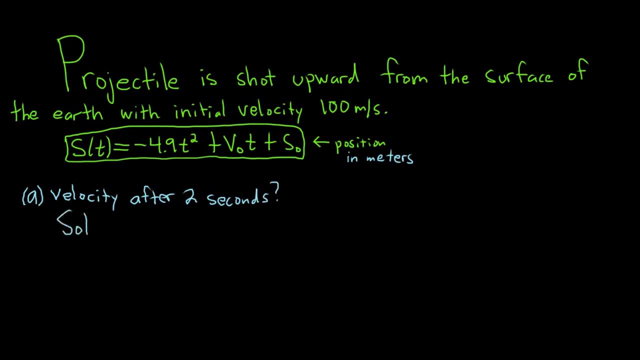 So to find the velocity after 2 seconds we have to work with the position function. Let's think about what's happening in the problem. So here's the Earth And there's a projectile, And it's going up from the surface of the Earth with initial velocity 100 meters per second. 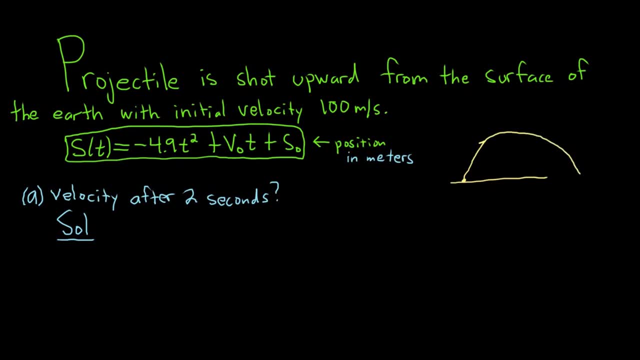 So it does something like this And it creates some parabolic shape And then it hits the ground. So the initial velocity is 100 meters per second. So we know that v sub 0 is the initial velocity, So v sub 0 is equal to 100. 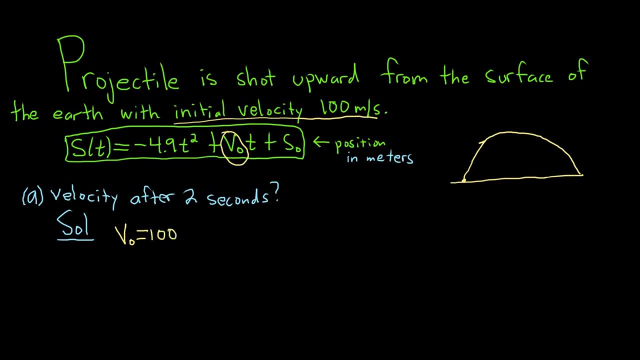 That's because it's going up. If it was going down, it would be negative 100.. s sub 0 is the initial position, So in this case, since it's being shot from the surface of the Earth, it should be 0.. 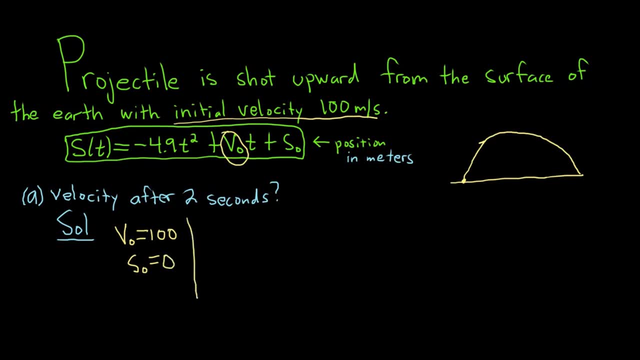 So now we can go ahead and rewrite our position function. So s of t is equal to negative 4.9.. t squared And we said v sub 0 was 100.. So plus 100t, And then s sub 0 is 0.. 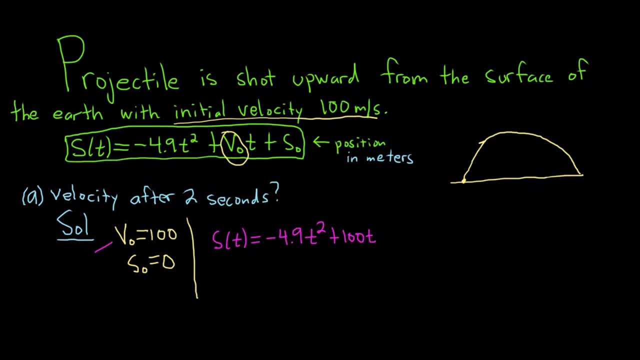 So everything looks okay. So again, v sub 0 is the initial velocity, s sub 0 is the initial position. Okay, so we want the velocity. Well, the velocity is the derivative of the position function. So all we do is take the derivative. 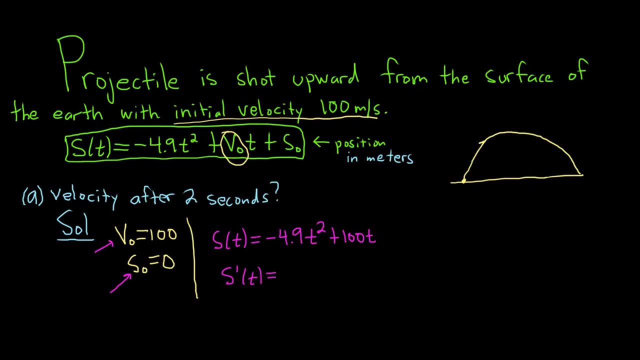 So s prime of t, And this is equal to, let's see, 2 times negative 4.9.. It's going to be negative 9.8t, And then the derivative of 100t is just 100.. So this is the derivative of position. 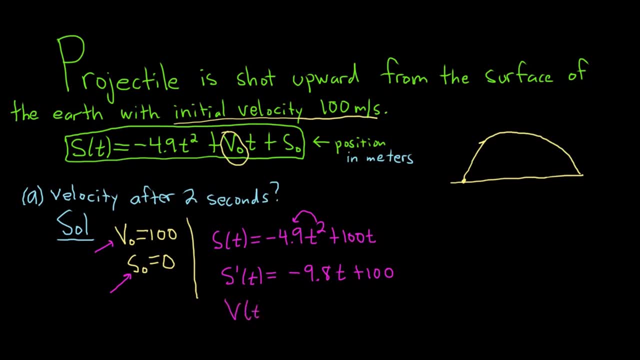 This is the velocity. So this is v of t. This is the velocity after t seconds or at t seconds. It's the instantaneous rate of change. right, Instantaneous rate of change. Okay, So it's the instantaneous velocity. You can think of it that way. 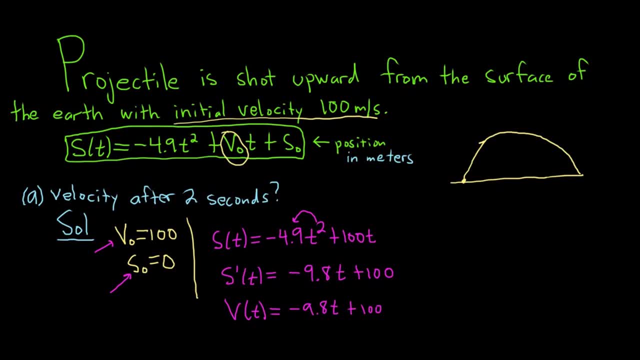 All right, So now we have to plug in 2. And that's it. That's it. It's that simple, I guess. So v of 2 is negative 9.8 times 2 plus 100.. And I suppose you could do this in your head. 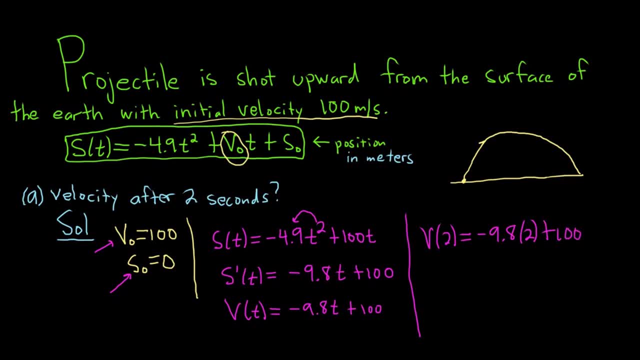 But I do have a calculator nearby. Let's see Negative 9.8 times 2 plus 100.. I got 80.4.. 80.4., 80.4.. And the units are meters per second for velocity right. 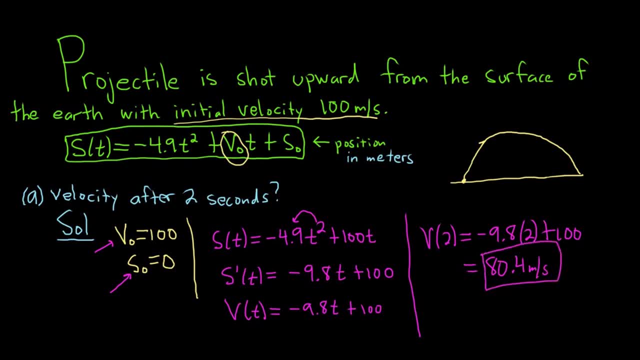 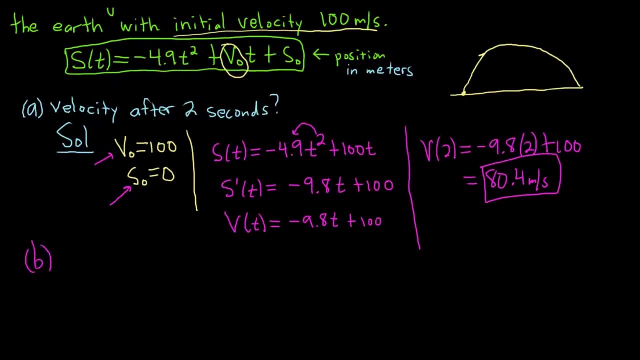 So, and that would be the velocity after 2 seconds. Let's do a harder problem now. Let's make it hard. Let's raise the bar B. Let us find the maximum height of the projectile. So max height of projectile, So the maximum height of the projectile. 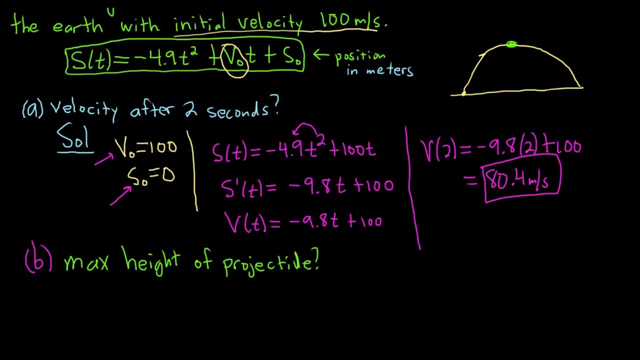 All right. So we have to find how high it goes, right. So there are 3 ways to do this I believe that I can think of off the top of my head. Method 1 is using intuition. That's really, really cool. 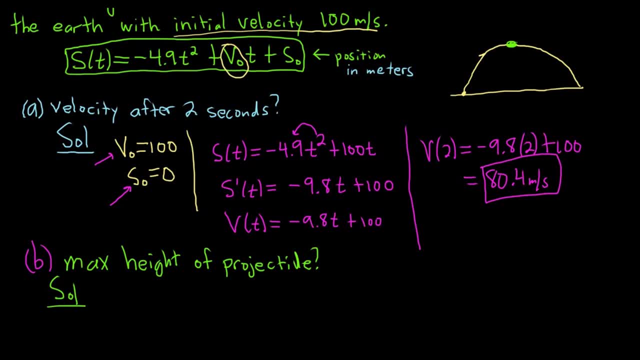 And I'm leaning towards taking that approach. It's really clever and beautiful. So method 1 is intuition. Method 2 is just using basic algebra. right, This is the vertex. Yeah, this is the position function. I made sure I circled the right thing. 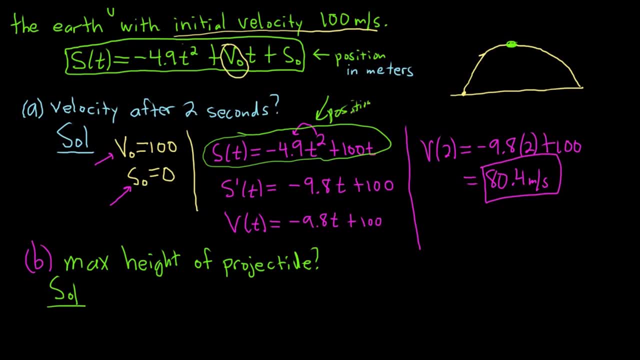 So this is the position, So, using basic algebra, So this is the vertex of a parabola, right, And so you could use the formula negative B over 2A, F of negative B over 2A, And you would use it on A, T squared plus B, T plus C. 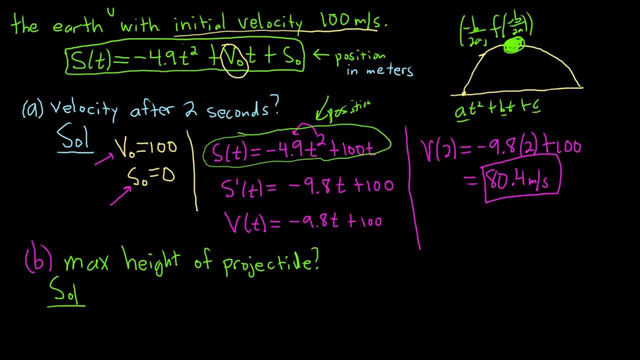 So you would find your A, B and C. I've never done it in this problem. So here A is negative 4.9.. And B is 100.. And that would be your X coordinate, And then you plug that into your Y coordinate. 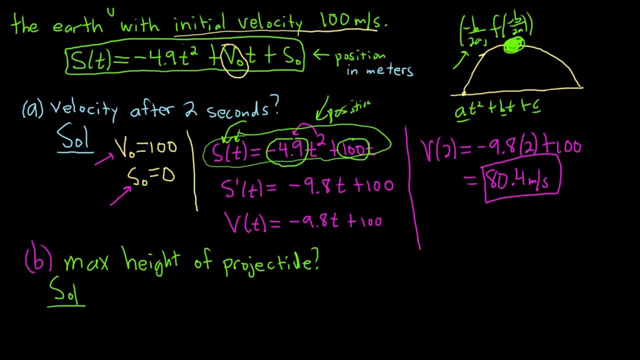 So into your function to get your Y coordinate. So you could do it with algebra Method 2, you could take the derivative and set it equal to 0. And find your critical number And you know, use the first derivative test. 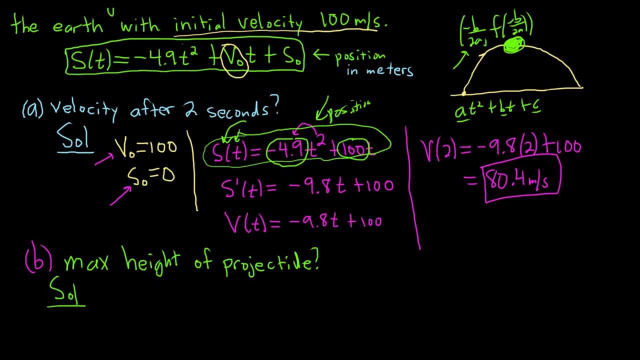 Actually, we haven't done that yet, So you can't do it that way. The only way so far that we've learned how to do this is using basic algebra, But once you know more calculus, you can use calculus to do it. 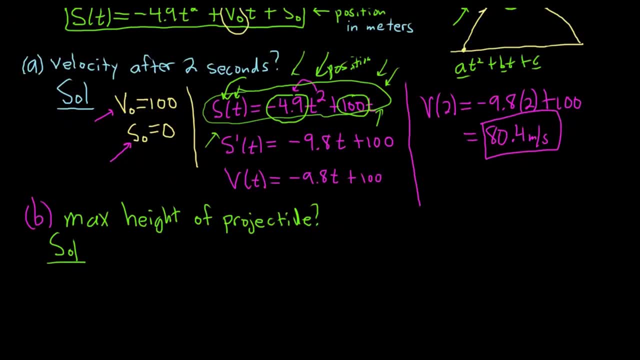 Anyways, let's do it the coolest way possible. in my opinion, Let's use intuition. So let me draw the picture again down here. This is really exciting. So we're looking for the maximum right. So let's think about this. 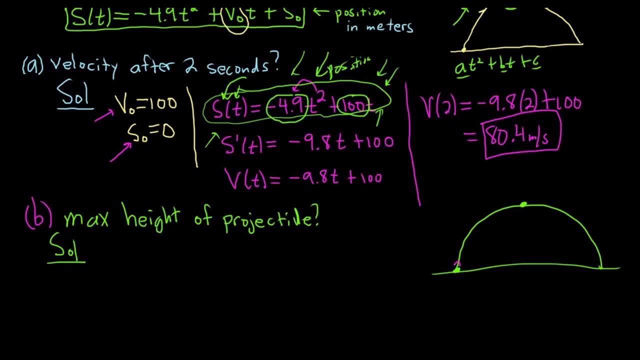 Let me use a different color. So the projectile is going up. There's a little projectile, It's moving along. Right now it has a positive velocity. Remember the velocity is the derivative of a position. So the velocity is the slope of the tangent line right. 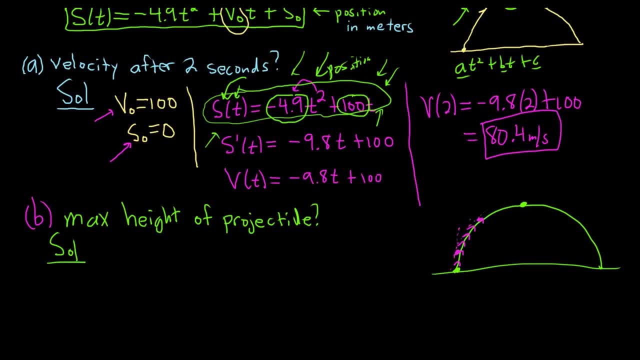 That's what's happening here, right? So it's positive, positive, positive And it gets to the top. There's the velocity And it's negative, So it's going to be at a maximum when the slope of the tangent line is 0.. 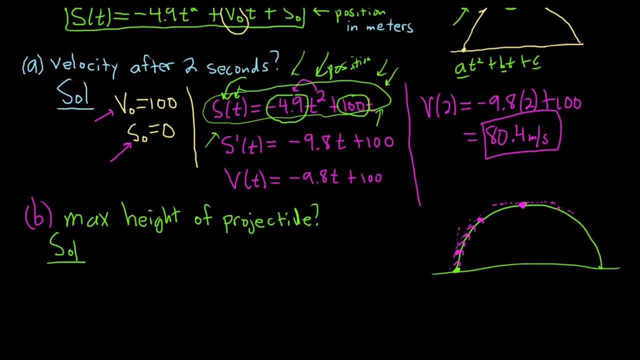 In other words, when it's stopped right, It's going up, up, up, up up, And then it stops at the very top And then it starts to fall. So that's going to happen when the velocity is 0.. 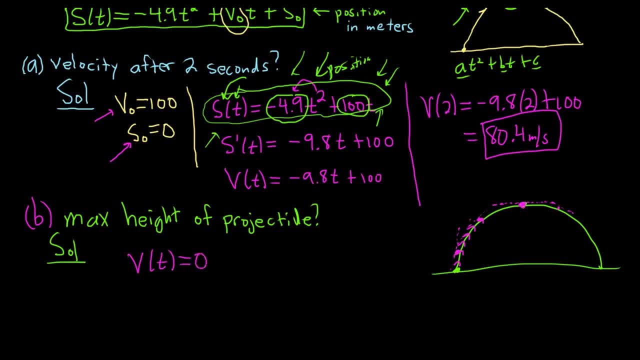 So it's at a maximum when the velocity is 0.. Remember, the velocity is the derivative of a position. The derivative is the slope of the tangent line. So you want the tangent line to be horizontal, because horizontal lines have a slope of 0.. 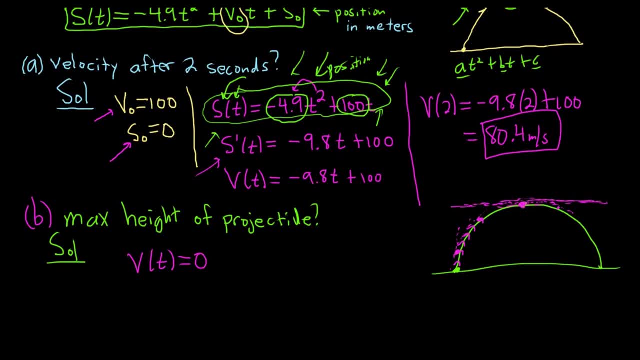 In other words, horizontal lines would give us a derivative equal to 0. So velocity equal to 0. So it goes up, up, up, up, up, up up. It stops, That's when the velocity is equal to 0.. 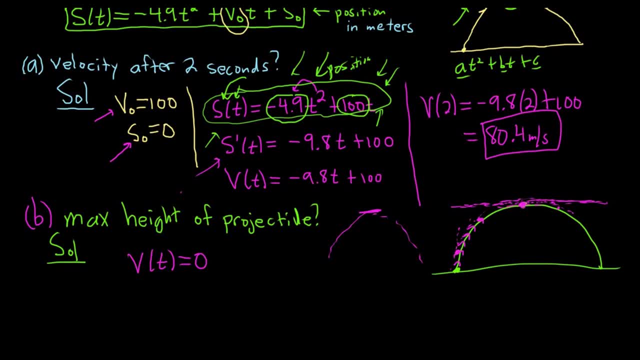 Then it comes down. So this is when it's going to be at a max. So it's at a max when this is true. So what is v of t? Well, you just replace it with negative 9.8t plus 100.. 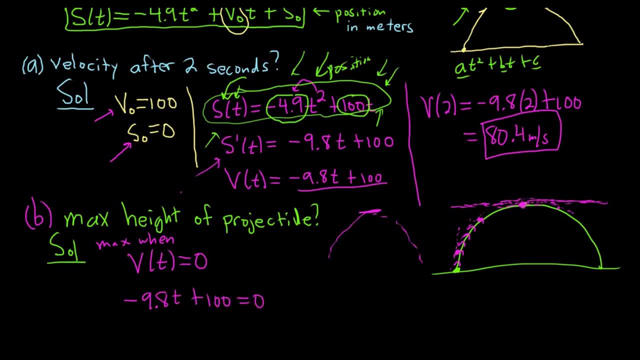 Set that equal to 0. And then subtract 100. So you get negative 9.8t equals negative 100. So t equals 100 over 9.8.. I'm going to put this in my calculator. So 100 over 9.8 is about 10.2 seconds roughly. 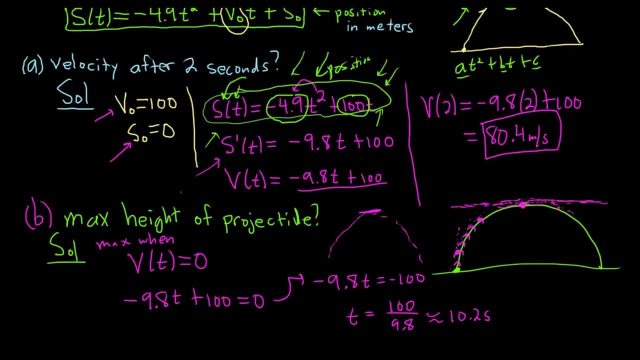 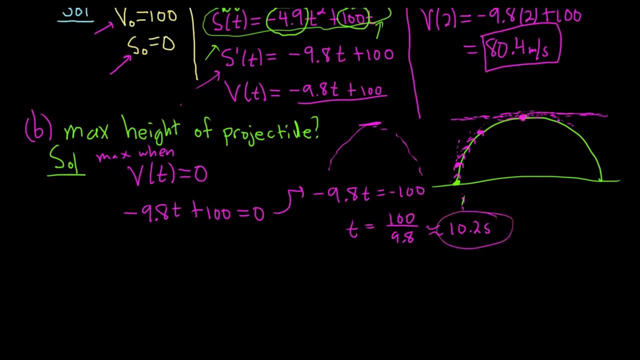 So that's when it takes 10.2 seconds to reach a max. Wow, So it went pretty high up. So how high did it go? Well, all we do now is we plug this into our position function. Recall: the position function was: s of t equals negative 4.9t squared plus 100t. 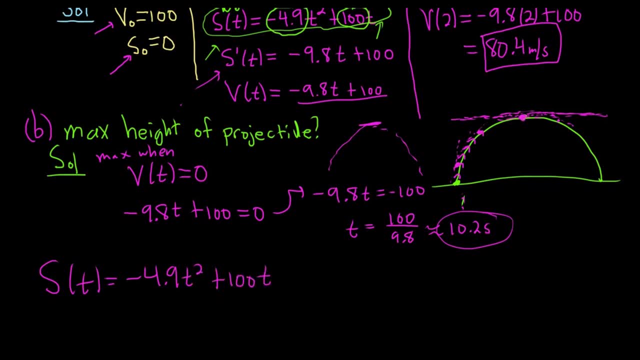 So now we just take this and plug it in, So that will be: s of 10.2 equals negative 4.9t squared, And then 10.2 squared plus 100t, which is 10.2.. And let me put this in my calculator: 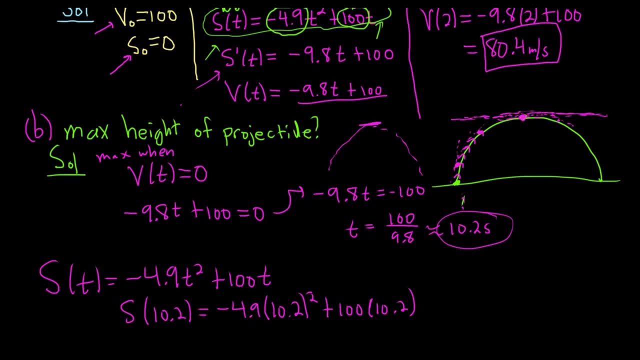 Let's see It's going to be negative. 4.9 times 10.2 squared plus 100 times 10.2.. Okay, I got 510.2, roughly, So approximately equal to 510.2.. And the units were meters. 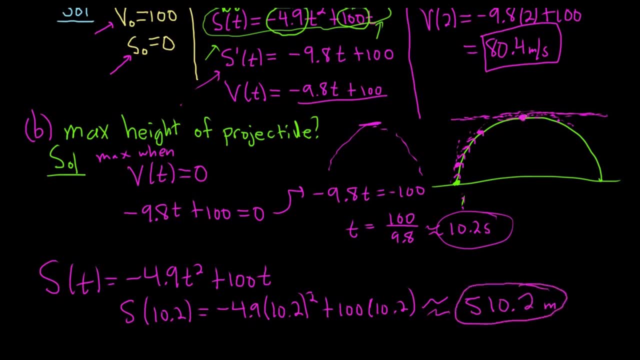 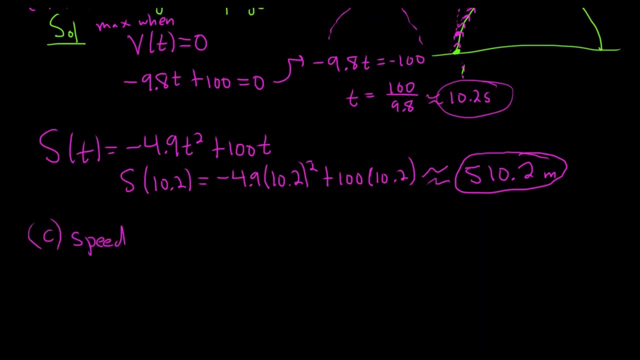 That's pretty high up there, So that's going to be the maximum height of the projectile. So kind of interesting. Part C, Part C, let's find. Let's do one more: Find the speed after 13 seconds, Why not? 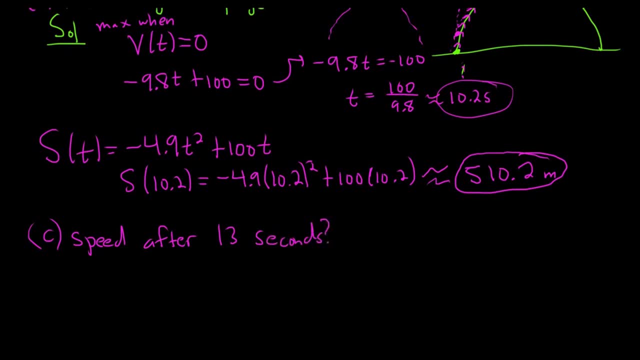 It's a long video, but if you're still with me, that's awesome. We're going to do one more interesting problem. So to find the speed, we have to take the absolute value of velocity. So we know that our velocity function is negative: 9.8t plus 100.. 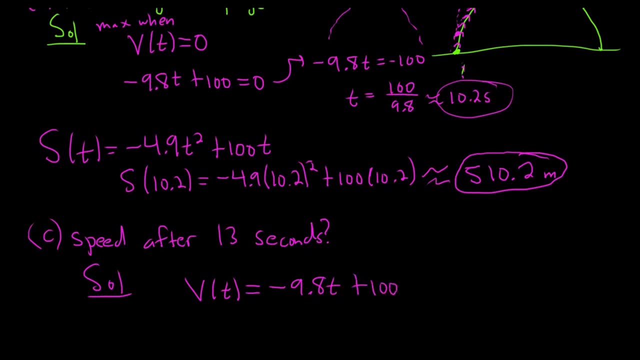 Okay, So all we have to do now is plug in 13 and take the absolute value, because speed is the absolute value of velocity. So v of 13 is negative 9.8 times 13.. Times 13 plus 100.. So this is going to be negative 9.8 times 13 plus 100. 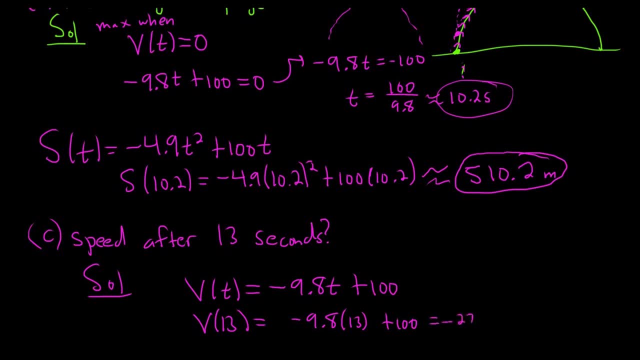 Negative: 27.4.. That makes sense, right, Because if you think about what's happening, it reaches a max at 10.2 seconds. So this is 10.2.. And so now your 13 seconds is over here. 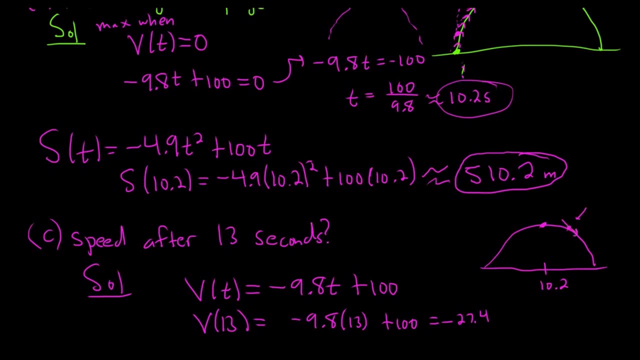 So the velocity is negative because it's going down right. So we want the speed. So the speed is the absolute value of this. So you just take the absolute value of that and just make it positive. So it's going to be 27.4 meters per second right. 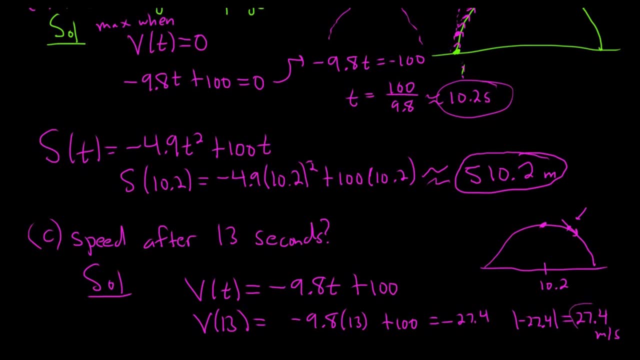 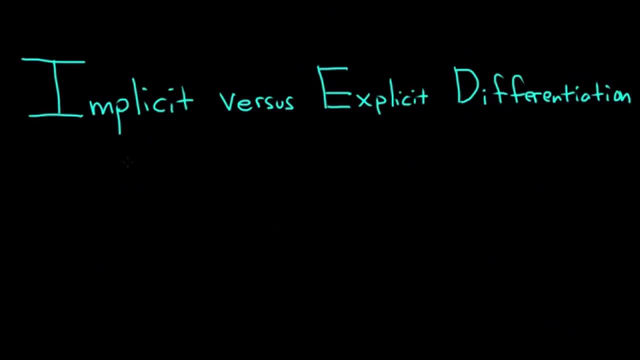 Meters per second. So that would be the speed. So I hope this video has been helpful. That's it, Hey everyone. In this video we're going to talk about the differences between implicit and explicit differentiation. So first let's talk about explicit. 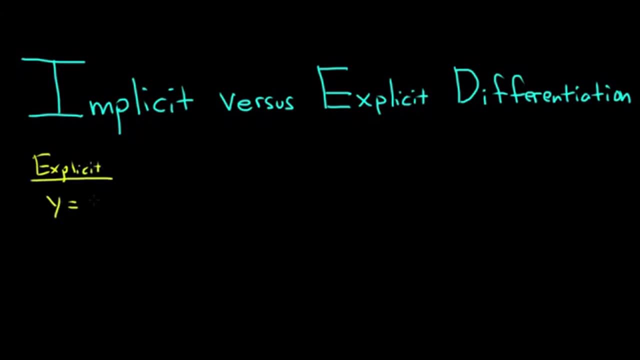 So if you have something like y equals, let's say, x squared plus sine x, Here y is being explicitly defined in terms of x. So over here you only have x's, So only x's. You don't have any y's here. 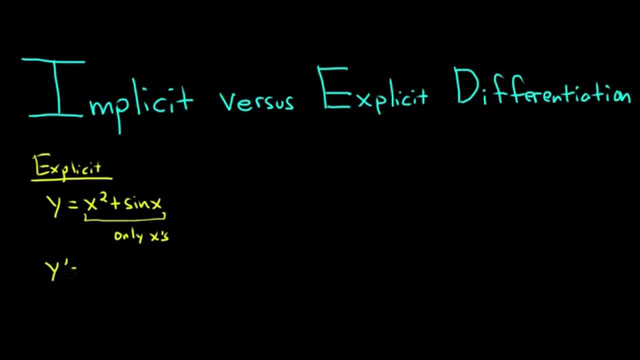 You could easily take the derivative here. So y prime would be 2x using the power rule, and the derivative of sine is cosine Piece of cake. So here y is explicitly defined in terms of x. We only have x's. 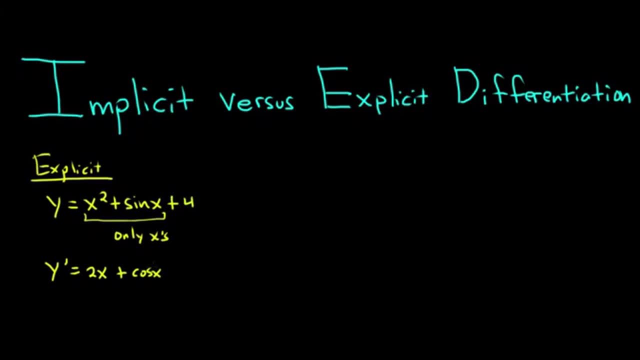 We could have a number here. Let's do it 4.. The answer still remains the same. So there's no other y's here. right, There's no y's here. So that's what we mean by explicit differentiation: Y is explicitly given and we can find the derivative. 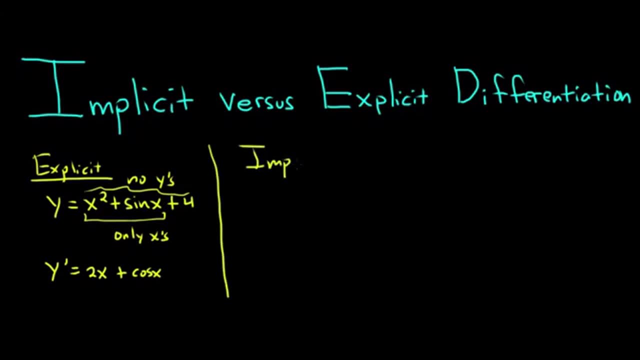 Implicit is a bit different. So in implicit differentiation y is implicitly defined by an equation. So for example, you could have x squared, Y to the fourth equals 7.. So in this case we don't have y, We just have an equation and y is in that equation. 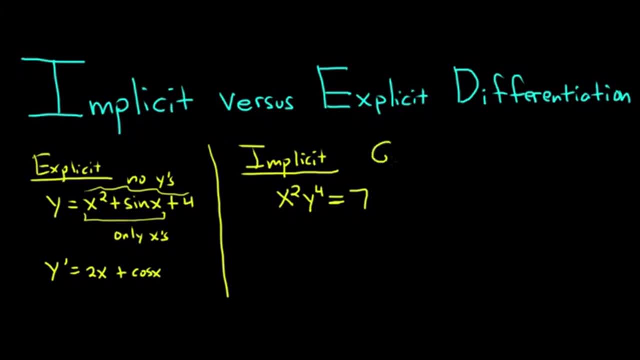 So it's mixed in with the x's and y's. So the goal is to find y prime, Except we tend to call it dy, dx when we do implicit differentiation. So the goal is to find the derivative without actually finding y. Let's go ahead and do an example and I'll show you how to do it. 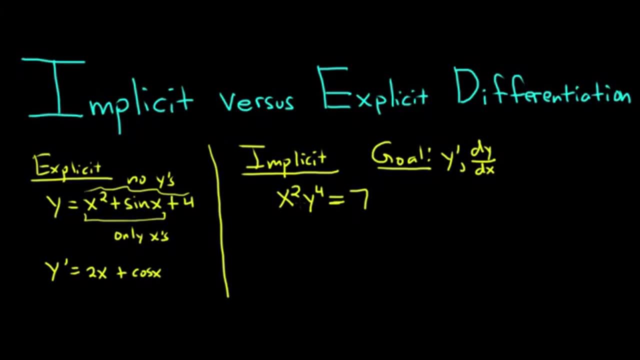 So to find the derivative of y without finding y, we have to take the derivative of both sides of this equation. Now, on the left-hand side, we have x squared times y to the fourth. That's going to require the product rule. 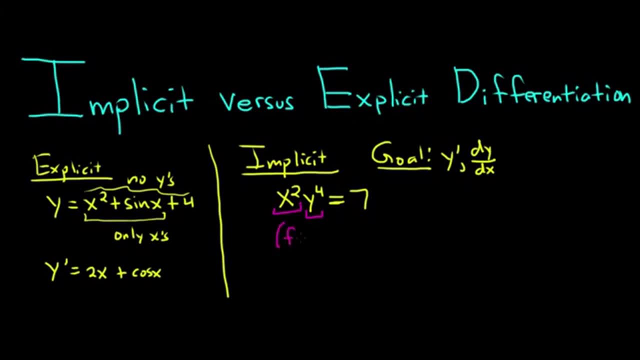 Recall. the product rule says: if you have f times g and you take the derivative, Think of f as the first piece and g as the second piece. So it's the derivative of the first times, the second plus the first times, the derivative of the second. 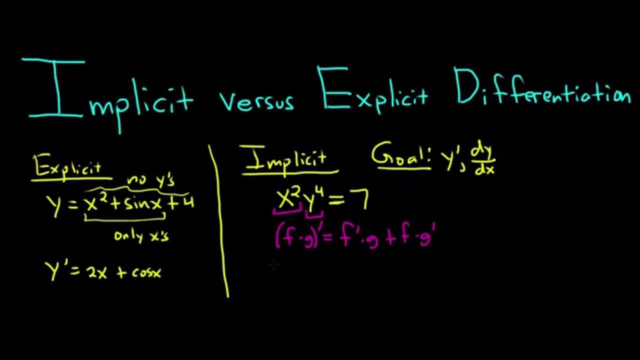 All right, so let's go ahead and do it. So in this case it's the derivative of x squared, So it's 2x times the second plus the first, So just x squared. And here's the tricky part. Now we're going to multiply by the derivative of y to the fourth. 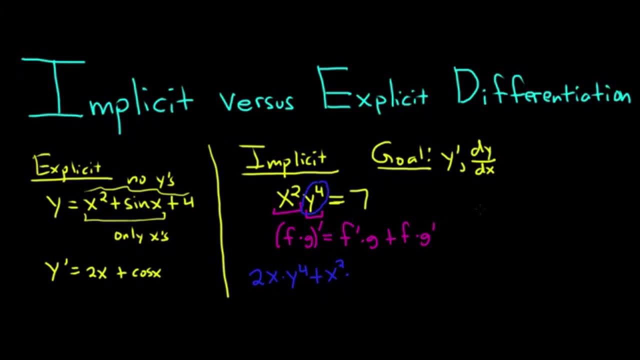 Now we're taking the derivative with respect to x, So we have y to a power. So when we take that derivative, we put the 4 in the front, So we get 4.. And then we get 4y. We subtract the 1, so we get 4y cubed. 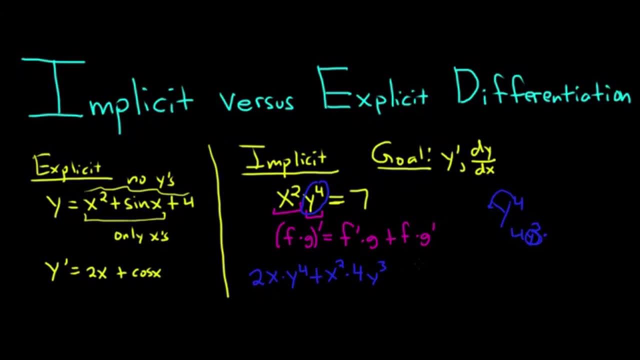 But then we have to multiply by the derivative of the inside piece. So the inside piece here is just y. So what's the derivative of y? Well, that's just y prime or dy dx. So we just write dy dx. Okay, so whenever you're using implicit and you take a derivative, 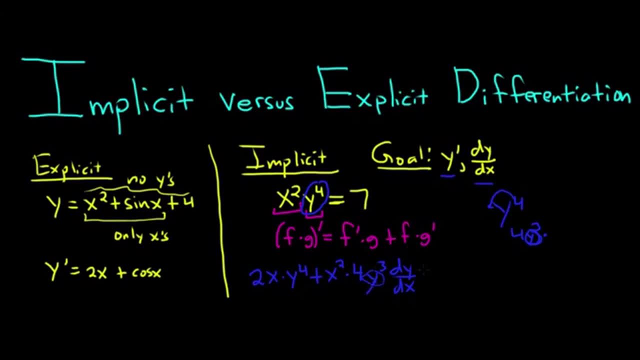 and there's a y, you always have to put a dy dx And this is equal to. and then here the derivative of 7 is 0.. So it comes from the chain rule. right, This is from the chain rule. And then, to finish, you would just solve this for dy dx. 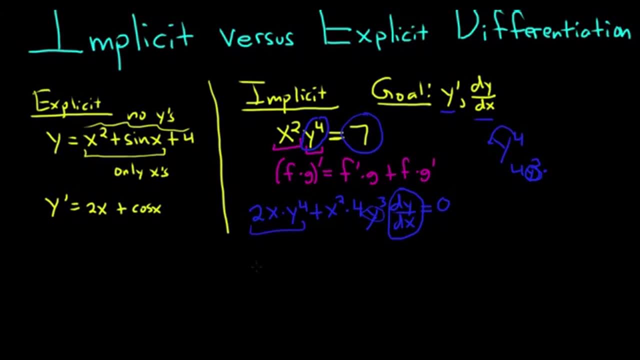 Let's go ahead and do it. We would subtract this piece So we would get 4x squared y cubed. dy dx equals negative 2xy to the fourth, And then, to finish, we would divide by 4x squared y cubed. 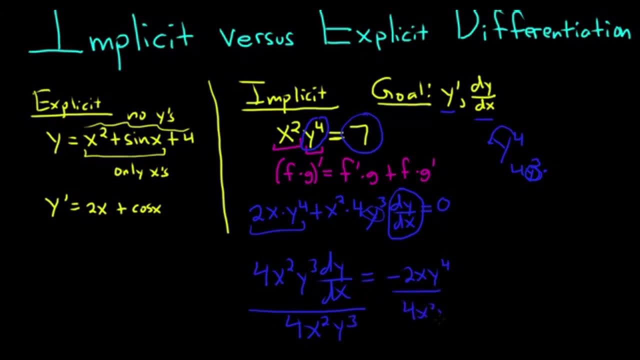 4x squared, y cubed, These cancel, And so this is equal to dy. dx equals. let's be really careful here. So the 2 and the 4, that's going to give us a negative 1, half The x and the x squared is going to leave us with an x on the bottom. 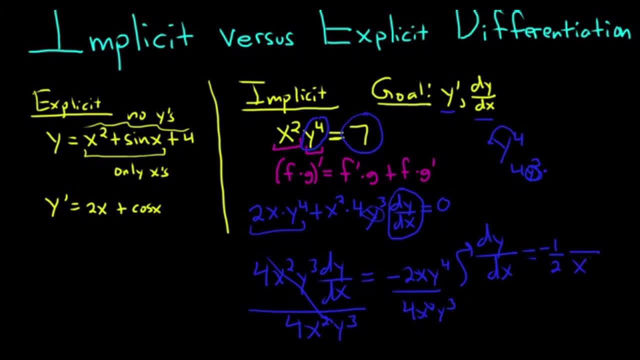 And the y to the fourth and the y cubed leaves us with a y up top. So we found the derivative of y without finding y. And again, the tricky part is this part here. This is the part that people have a really hard time with. 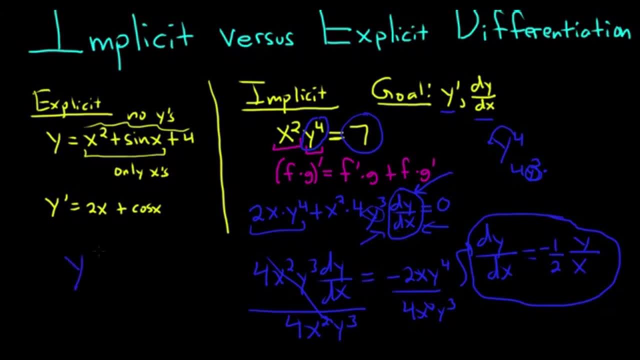 It's just the chain rule. So if you had like y to the fifth and you were taking the derivative with respect to x- That's what this means- d, dx, You would just get. you bring down the 5, so you get 5y to the fourth times the derivative of your inside function. 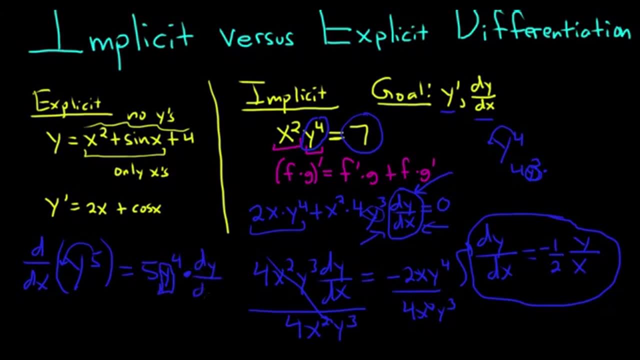 Your inside function is y, so you would just get dy, dx. So in explicit you have a formula for y and you can just take the derivative like you normally do. In implicit you don't have a formula for y, so you just take the derivative of both sides and go with it, right? 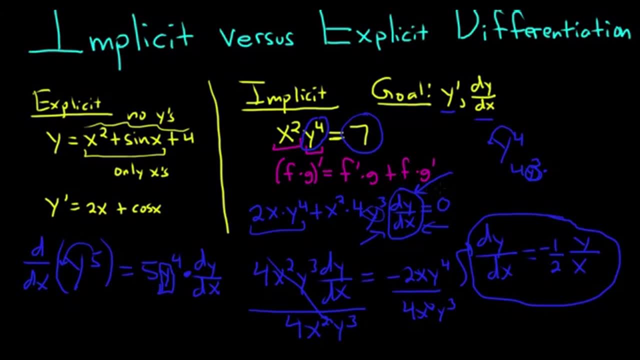 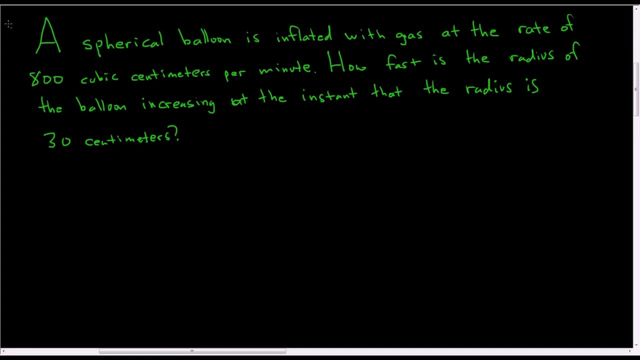 And then, whenever you have a y, you have to remember to use the chain rule. That's it. A spherical balloon is inflated with gas at the rate of 800 cubic centimeters per minute. How fast is the radius of the balloon increasing? at the instant that the radius is 30 centimeters, 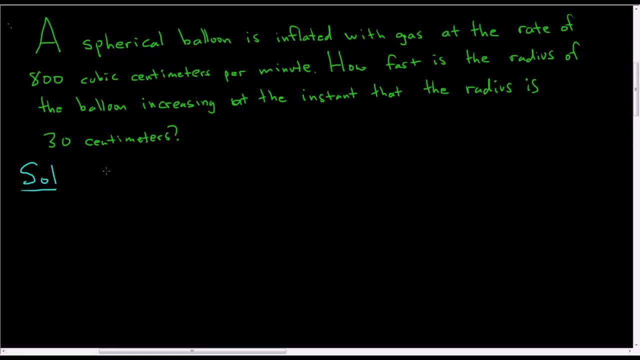 So let's work it out. Solution First: the formula for the volume of a sphere is 4 thirds pi r cubed. So we have that And let's read the question again and figure out what we're given And then figure out what we need. 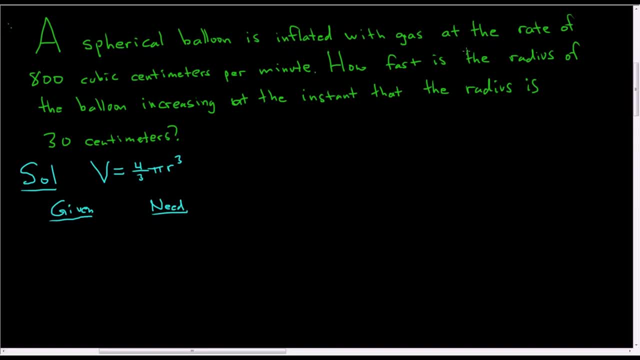 So we're told that the balloon is inflated with gas at the rate of 800 cubic centimeters per minute. So the key word there is cubic. It's telling us something about the rate of change of the volume. So we're given that dv dt is equal to 800. 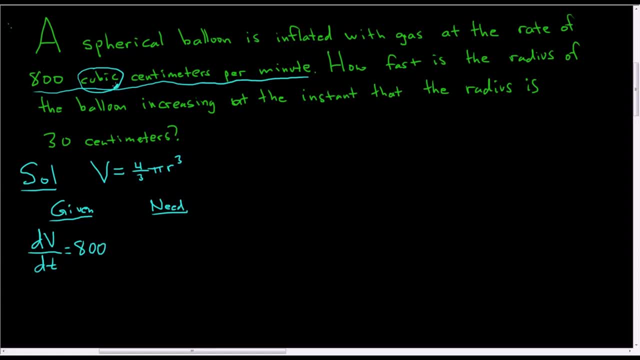 We know it's volume because it says cubic, And we know it's a rate of change because it says rate. What do we need? The question says how fast is the radius of the balloon increasing? So we need dr dt At the instant that the radius is 30 centimeters. 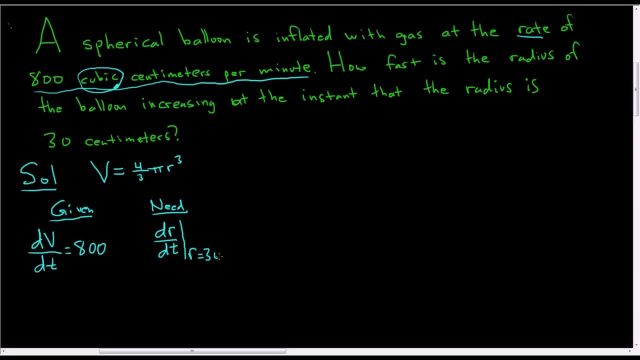 So when r is equal to 30. So whenever you're doing a related rates problem, if you write down what you're given and what you need, usually you can figure it out Alright. so now we will create a relationship between dv dt and dr dt. 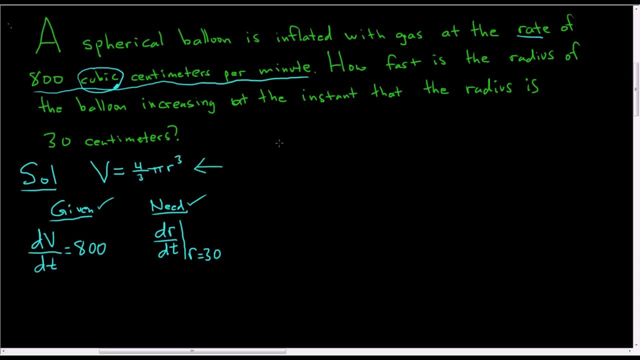 by differentiating both sides of this equation. So dv dt is equal to. Well, this is a constant 4 thirds pi, So it just hangs out. You bring the 3 down, So you get 3 times 4 thirds pi. r squared times the derivative of the inside, which is r. 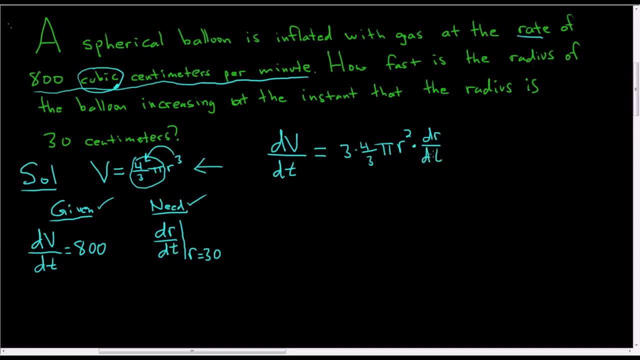 So dr dt, That's the chain rule. Alright, that's just the chain rule. So these cancel. So we get dv dt equals 4 pi r squared. And we know, Well, we don't know- We still have dr dt. 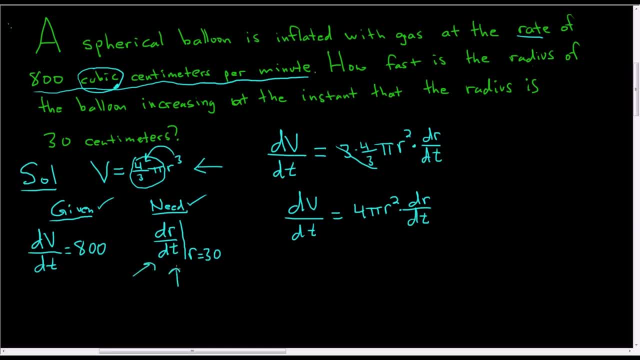 Alright, so we don't know dr dt, We're looking for dr dt, We know dv dt And so we just plug in 800 for dv dt. See in different variations of this problem. you know they'll give you dr dt and they'll have you find dv dt. 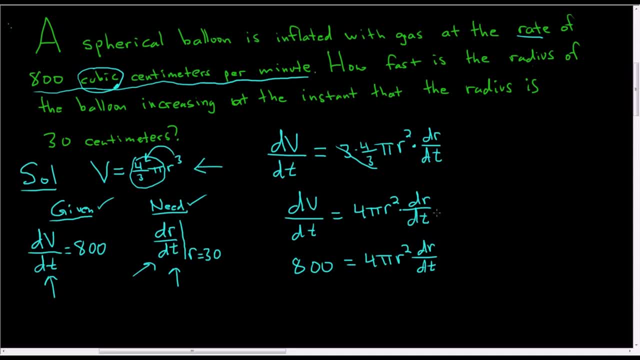 In this case they gave us dv dt and they're asking for dr dt. So When you work these out, just carefully write down what you need, Take the derivative and then plug in what you're given. In this case, we were given the 800. 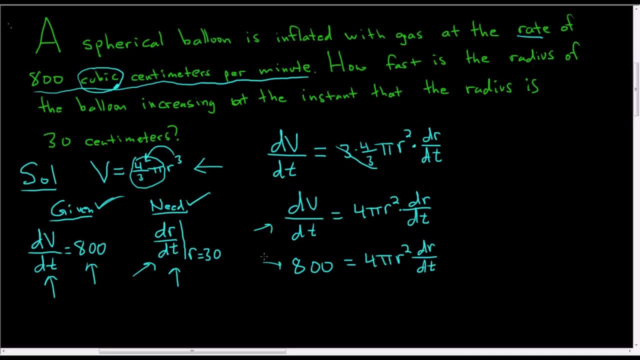 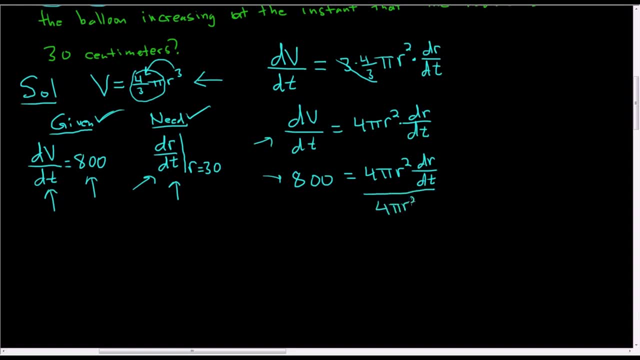 So it worked out nicely. Now we'll solve for dr dt. So let's go ahead and do that. So we'll divide both sides by 4 pi r squared, So these cancel. So we're left with dr dt equals. Well, 4 goes into 800 200 times. 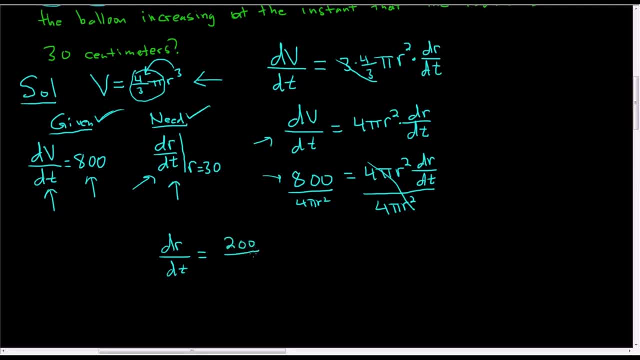 So we have 200 over pi r squared right, Because 800 over 4 is equal to 200.. Alright, now we need to just plug in 30, it seems So when r is 30.. Let me write it again. 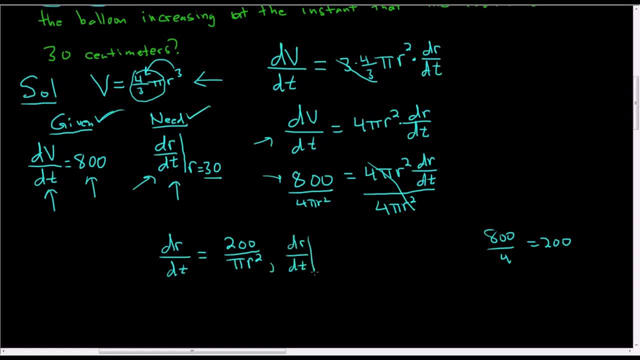 So dr dt, When r is equal to 30. That's going to be 200 over pi times 30 squared. So that'll be 200 over 30 squared is 900. So you get 200 over 900 pi. 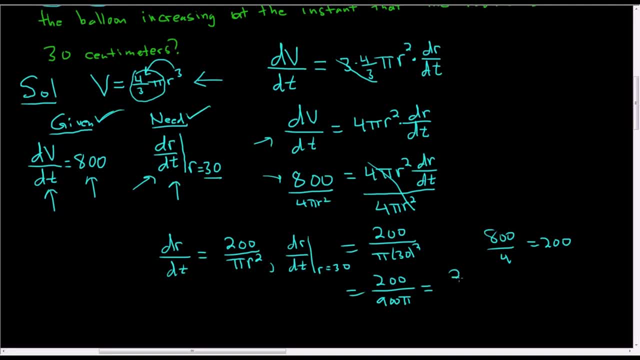 So you end up getting- Let's see, divide by 100.. So you get 2 over 9 pi And this is the rate of change of the radius. The units in this problem were centimeters, So it's centimeters per. 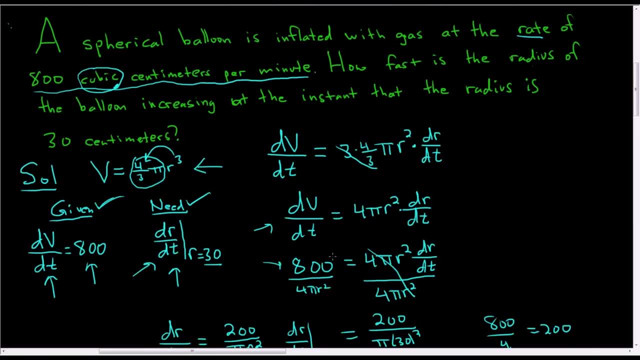 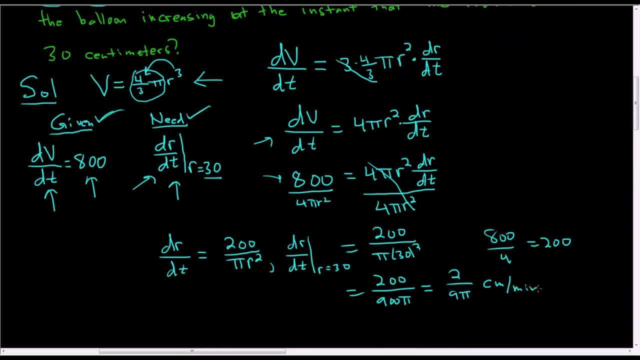 And I believe the time was minutes. Yep, it sure was. It's minutes. So per minute, So per minute, And that's the answer, Not a super tough problem. Just write down what you're given, Write down what you need. 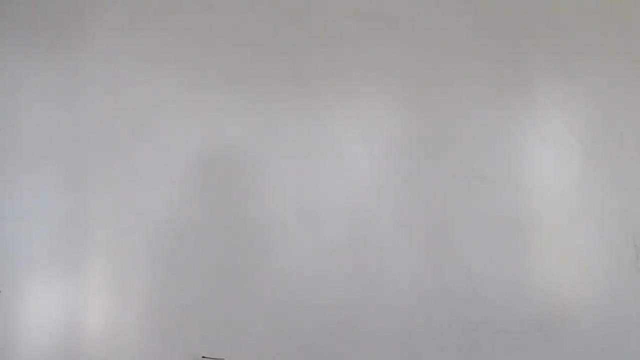 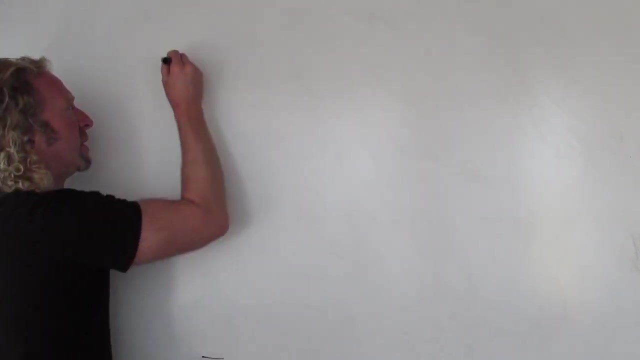 And you got this. That's it, Hey, YouTube. In this video we're going to talk about critical numbers. I'm going to write down the definition of a critical number And we'll look at some examples. So we say: x equals c is a critical number. 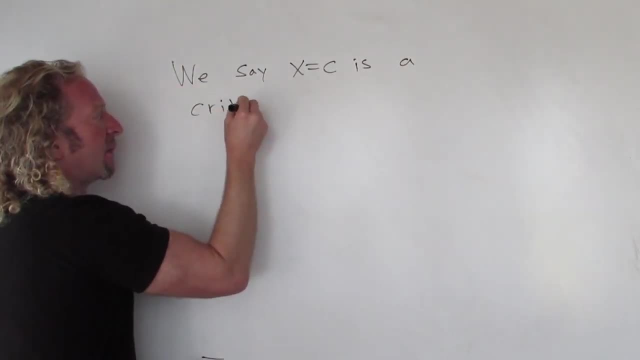 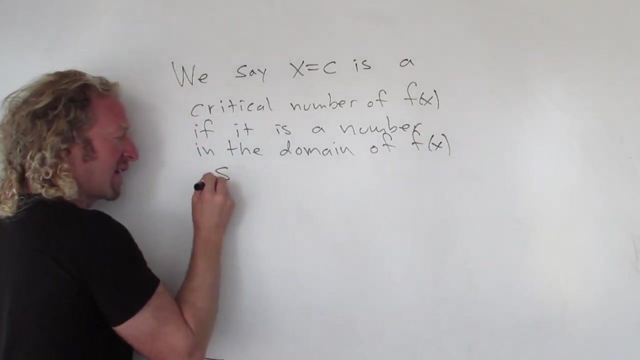 So it is a critical number of f of x. if it is a number in the domain of f of x, So it has to be a number in the domain of f of x, Such that, So a critical number has to be a number in the domain of the function. 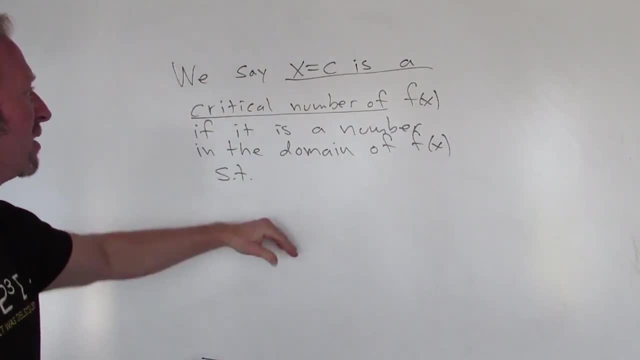 That's super key. So even before we define the conditions, that's kind of like a prereq. So a critical number has to be in the domain, So it's a number in the domain of the function, Such that one of two things happens. 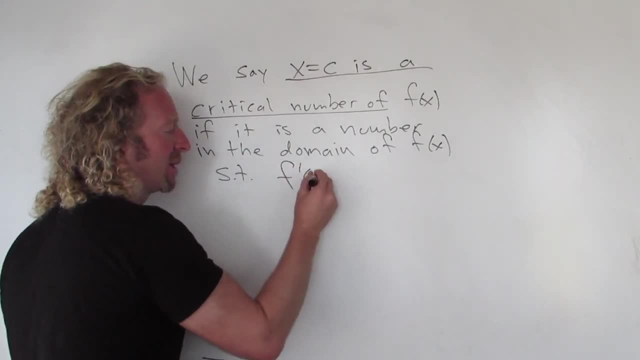 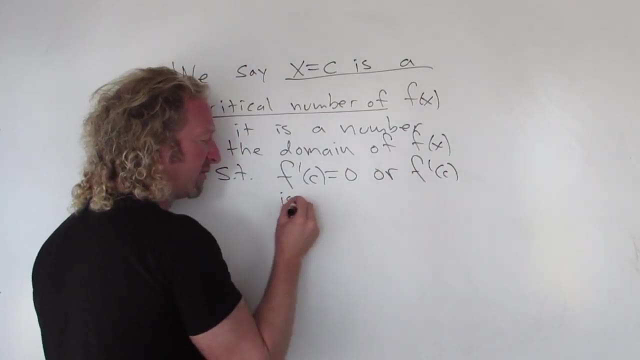 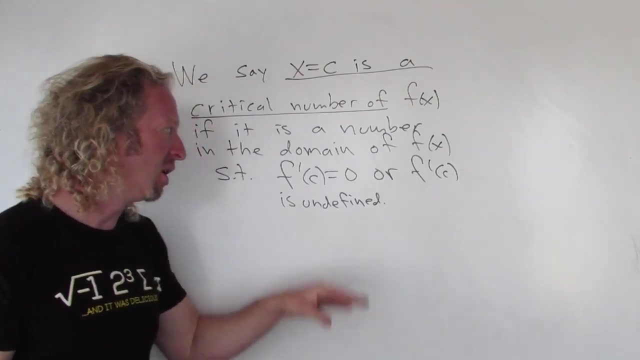 Either the derivative is equal to 0 at that number Or the derivative is undefined. there f prime of c is undefined. So a critical number is a number in the domain of the function where the derivative is 0 or the derivative is undefined. 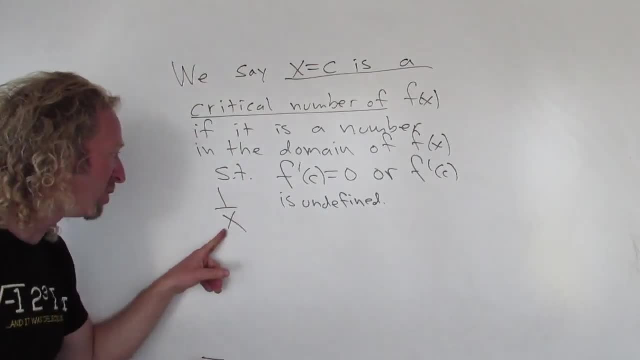 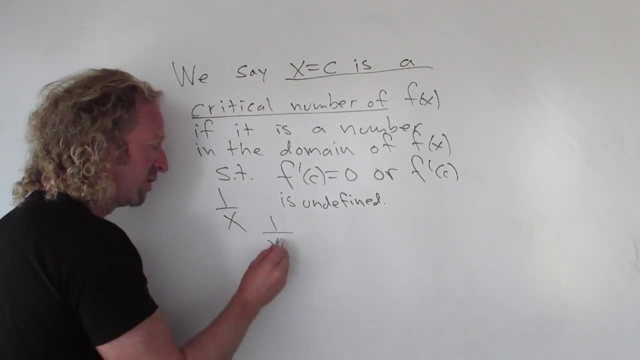 Just for example, say you have 1 over x, Right away you know that 0 could never be a critical number Because 0 is not the domain of the function. Or if you had 1 over x plus 2,, right away you would know negative 2 could never be a critical number. 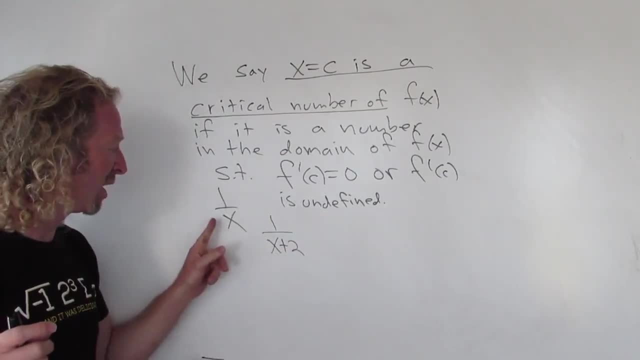 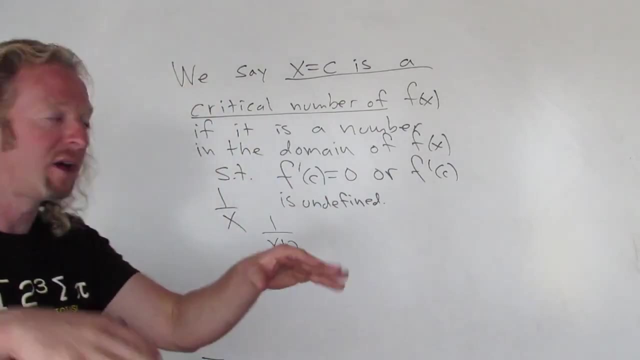 Because it's never in the domain of the function. By the way, x equals 0 and x equals negative 2 are both vertical asymptotes. Therefore, an easy way to think about it: vertical asymptotes can never be critical numbers for functions. 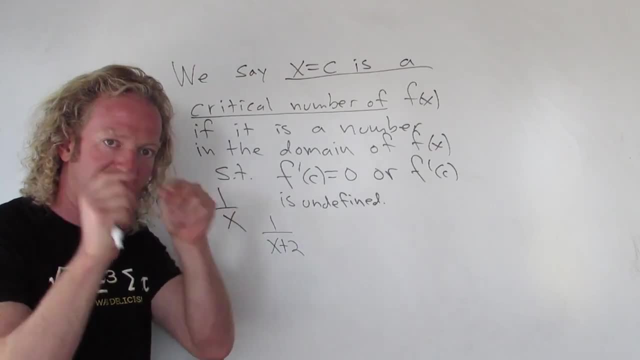 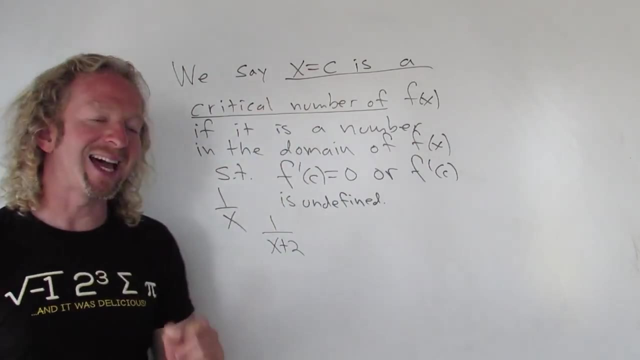 Because at those numbers the function is undefined. So a critical number is a number where the derivative is 0 or undefined, And a prerequisite to the definition is that it's in the domain of the function. Let's do some simple examples of finding critical numbers. 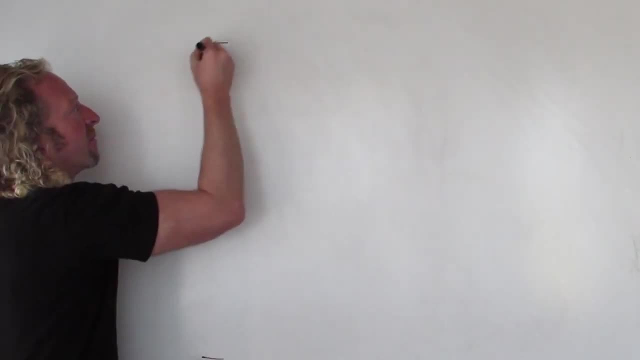 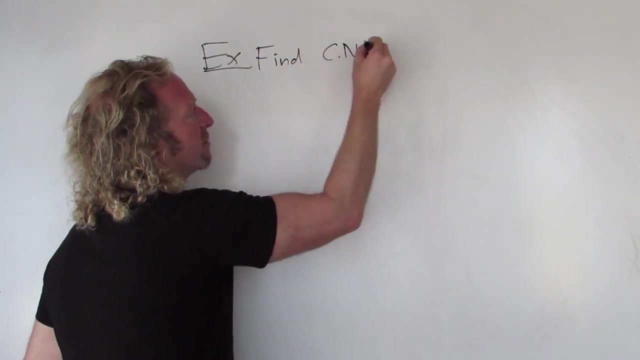 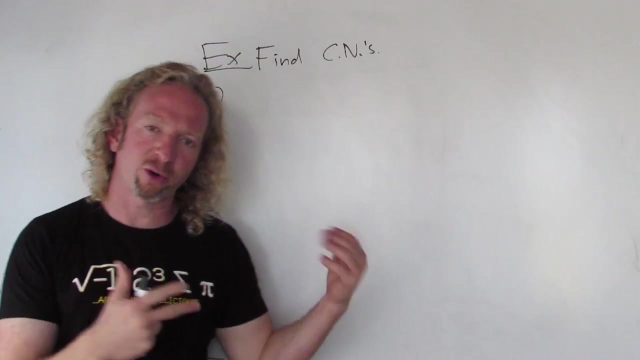 Just tricky, simple examples. So find, let's call them cn's just to abbreviate things. Find cn's, find critical numbers, if any, if possible. There might be none in these examples. So a By the way, what are critical numbers for? 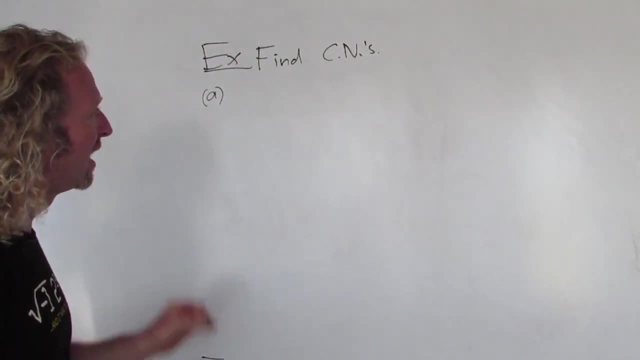 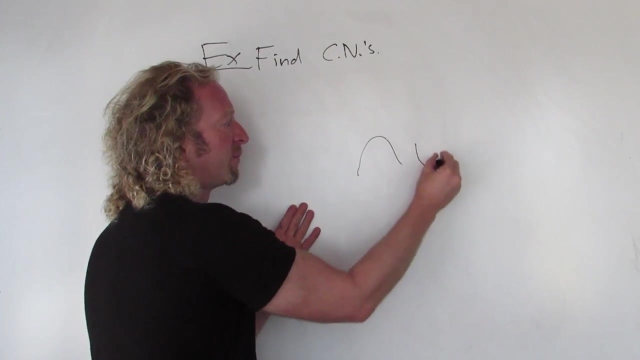 There's a big result in mathematics. It says if you have a relative maximum or a minimum, you have a critical number. So relative maximums and minimums are y values that are bigger than the points around them or smaller than the points around them. 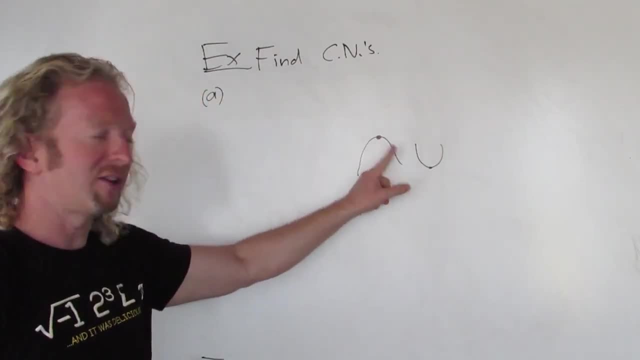 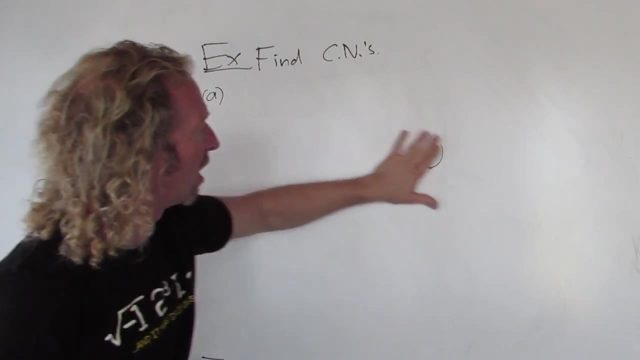 So, relative to the points around them, that's the biggest y value. Relative to the points around it, that's the smallest y value. So if you have one of these, you have a critical number. So as we go through these examples, we'll investigate the graphs. 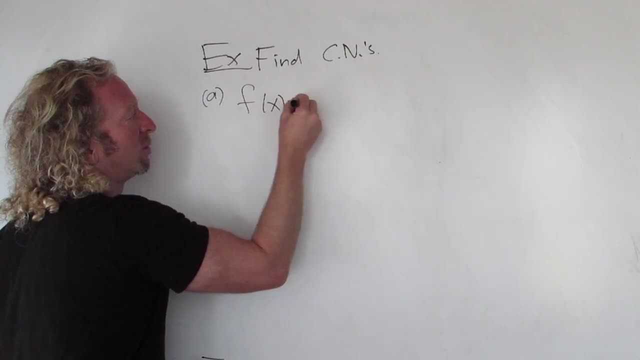 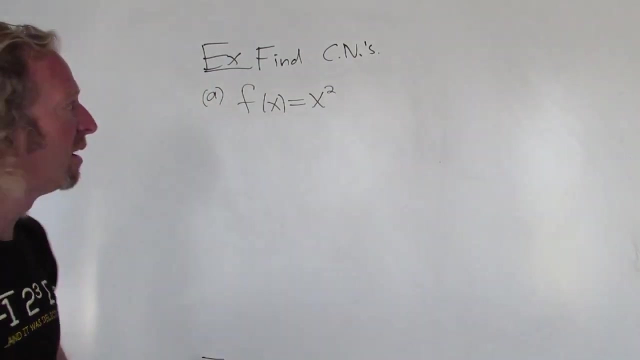 So let's look at: f of x equals x squared. Okay, so this is a quadratic function. right, x squared's a parabola. The domain is all real numbers. So, solution: let's find the critical numbers. So to find the critical numbers, you take the derivative. 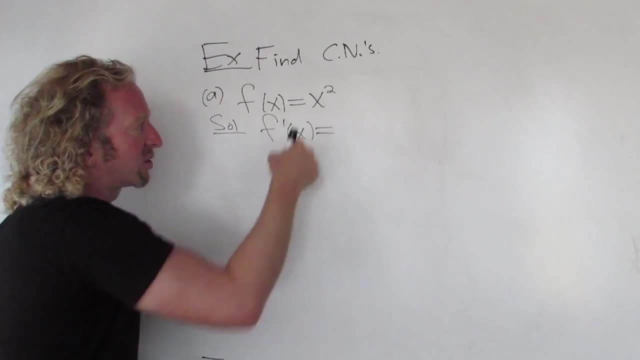 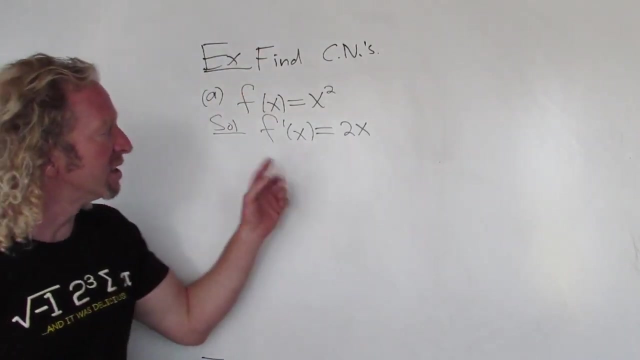 And you study it. So the derivative of x squared is 2x, right? You just use the power rule, All right. so a critical number is a number in the domain where the function is undefined, where the derivative is undefined or equal to 0.. 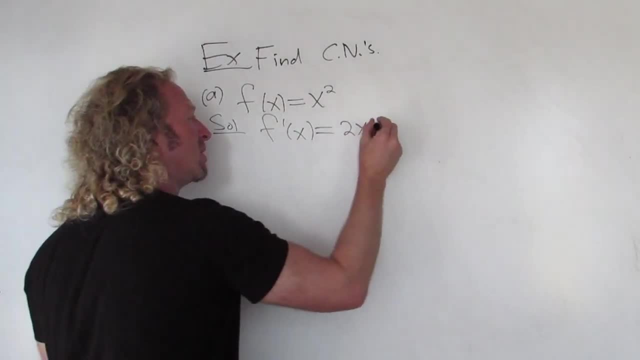 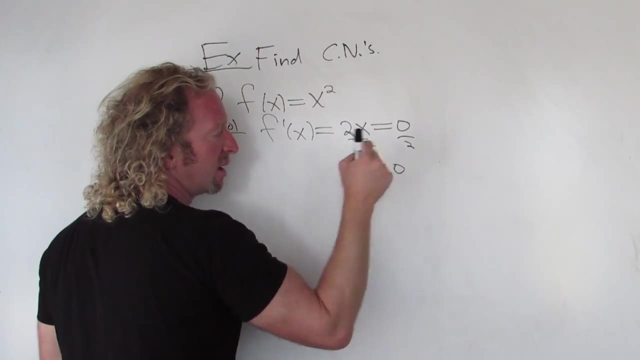 In this case, the derivative is never undefined, okay, So we set it equal to 0.. We can solve this by dividing by 2.. So we get x equals 0.. So 0 is a number in the domain of the function where the derivative is 0. 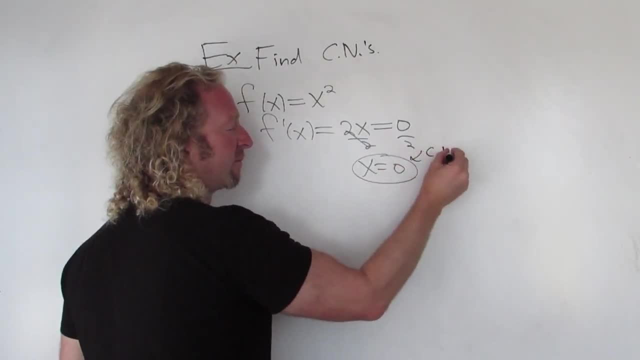 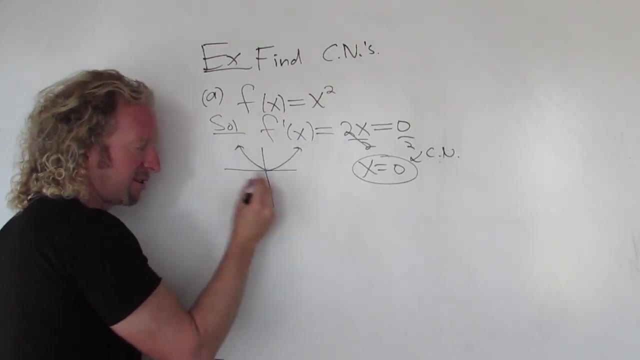 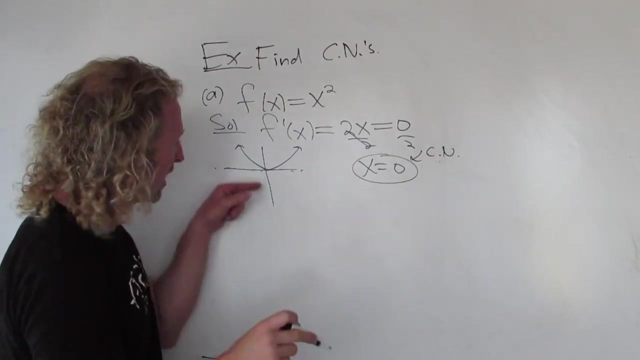 So this is a critical number. If you look at the graph of x squared- it's a parabola- It would make sense that the derivative there is 0 because you have a horizontal tangent line. Remember, the derivative is the slope of the tangent line. 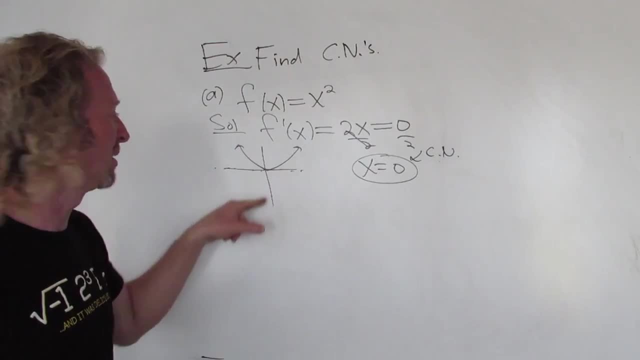 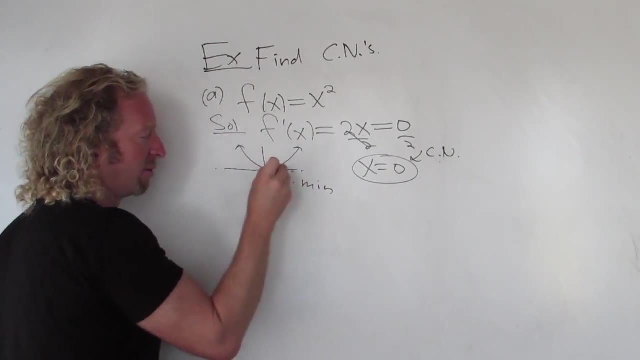 So you have a horizontal tangent line at 0. Therefore, the derivative should be 0 when x is equal to 0. In this case, you have a relative minimum. here. You have a relative minimum because this y value is smaller than the points around it. 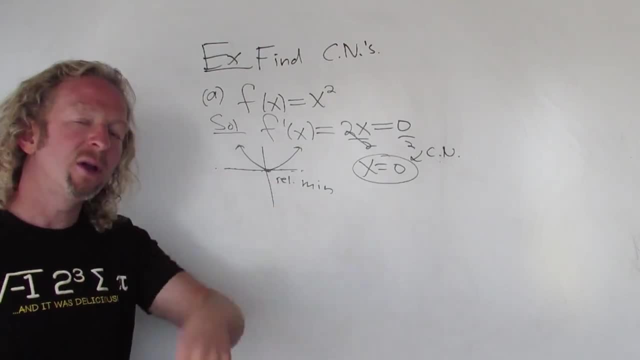 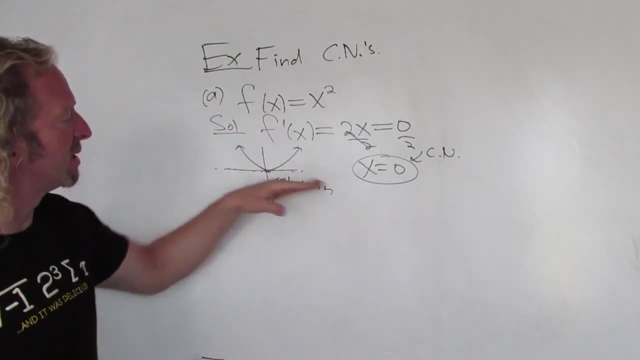 Remember that thing I mentioned earlier: If you have a relative minimum or a maximum, you always have a critical number. It doesn't go the other way, as we'll shortly see. So this is an example of a function that has a critical number at 0 and does have a relative minimum. 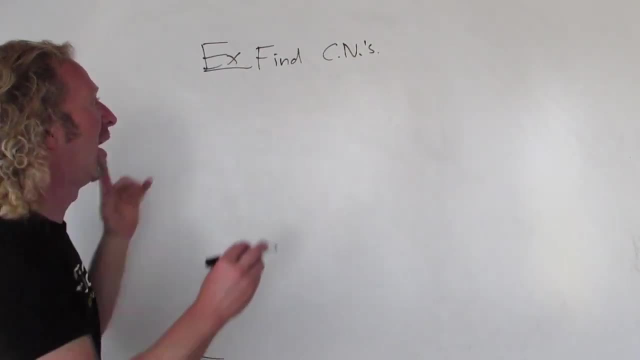 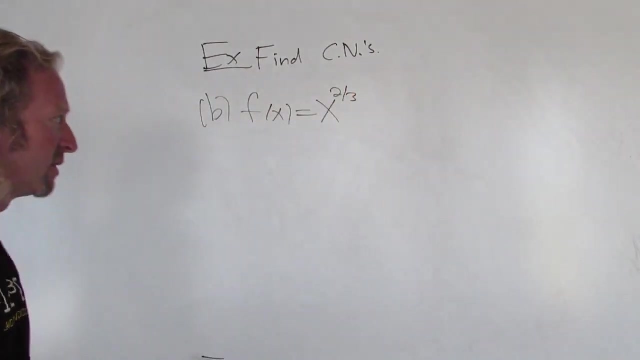 Let's do another example. How about this one? b f of x equals x to the 2 3rds. Okay, x to the 2 3rds. So the domain of this function is all real numbers, no problems. 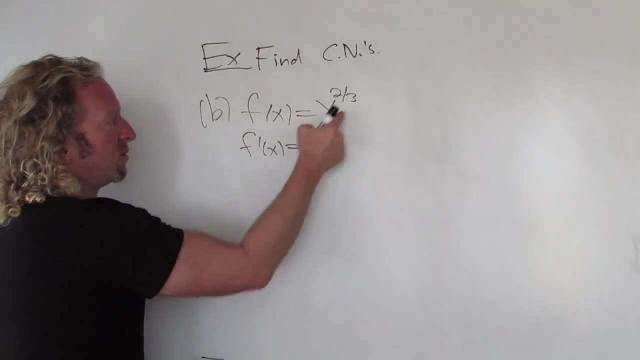 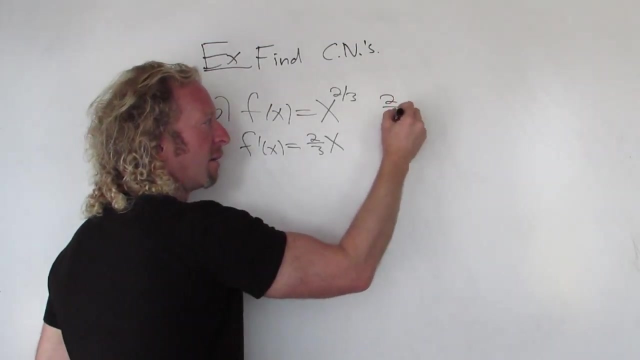 Let's take the derivative. So here we bring down the 2 3rds and we subtract 1.. So 2 3rds minus 1 is really 2 3rds minus 1. So it's 2 3rds minus 3 3rds. 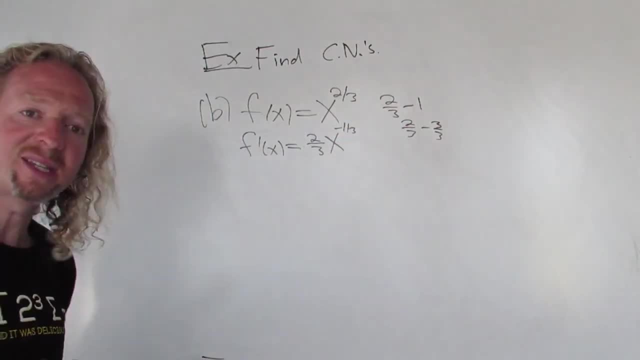 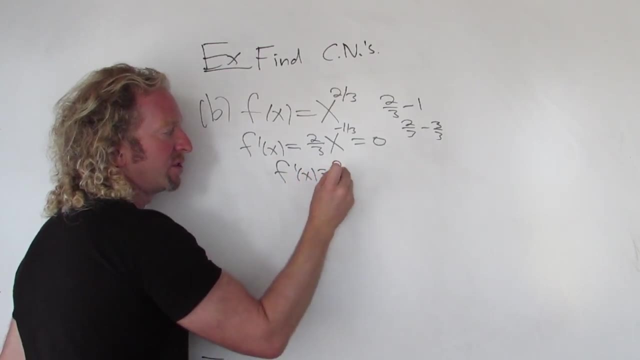 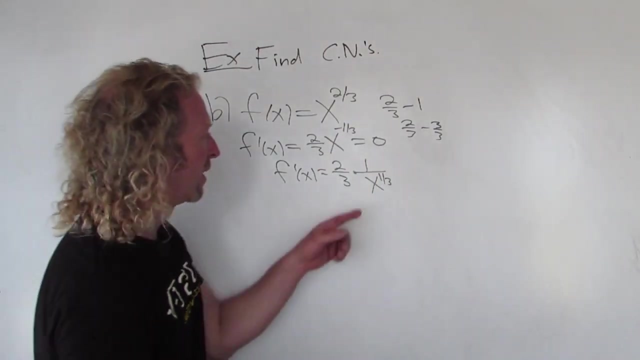 So it's negative 1- 3rd And we set that equal to 0.. You'll notice that you can rewrite this derivative as 2 3rds times 1 over x to the 1- 3rd. You can bring this down and the exponent becomes positive. 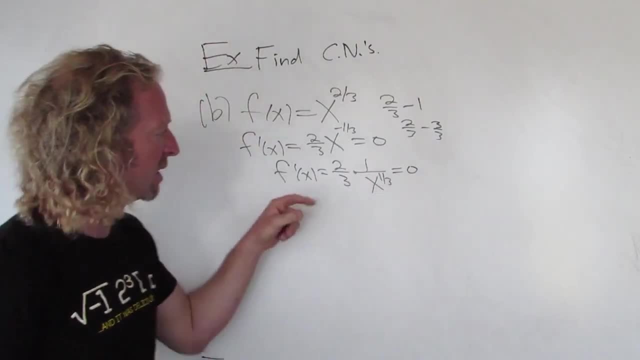 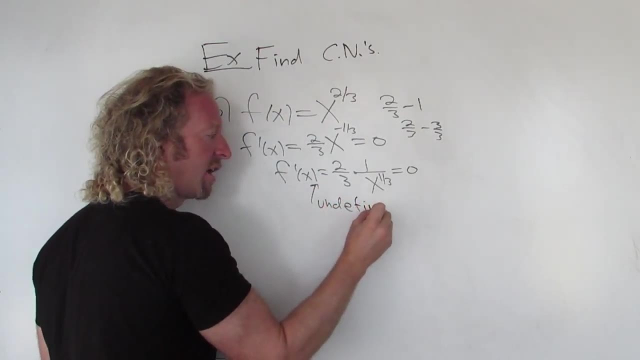 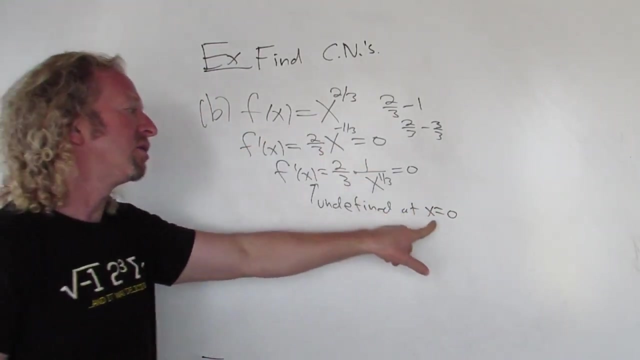 And we set it equal to 0. This has no solution. There's no way you can get 0 from this, But this derivative is undefined. This is undefined at x equals 0.. It's undefined at 0.. And 0 is in the domain of the original function. 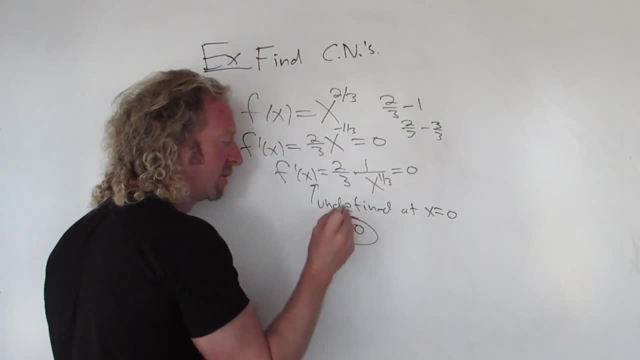 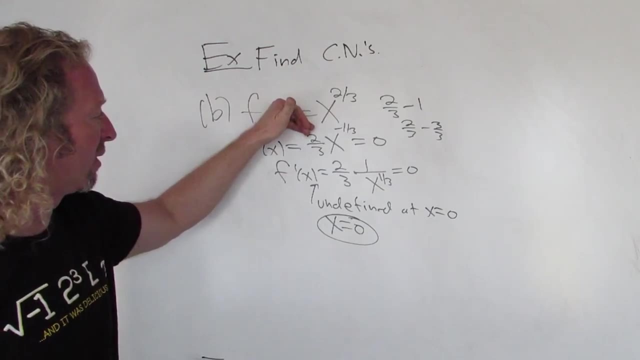 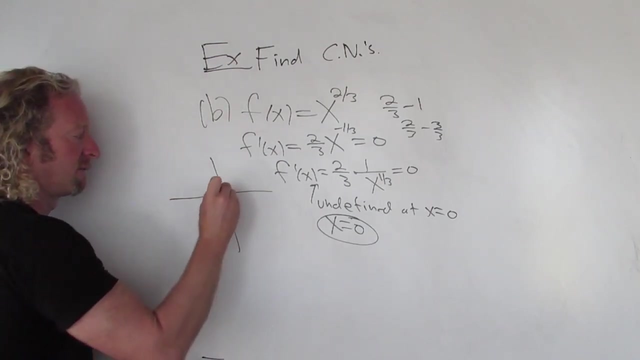 So this is actually a critical number. So x equals 0 is a critical number. Sneaky right, Sneaky stuff. So this is an example of a function that has a critical number that arises from the derivative being undefined. If you look at the graph of this function, it looks like this: 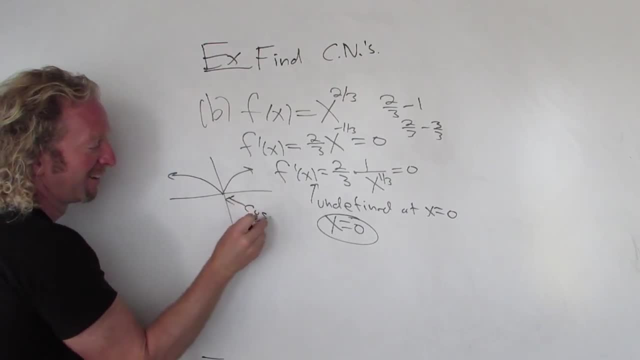 What is that? It's called the cusp. What's a cusp That It's called the cusp, Cusp. So you see, in this case you do have a relative minimum. So you have a relative minimum. 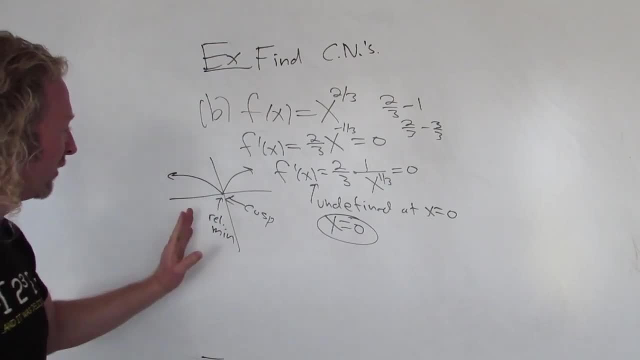 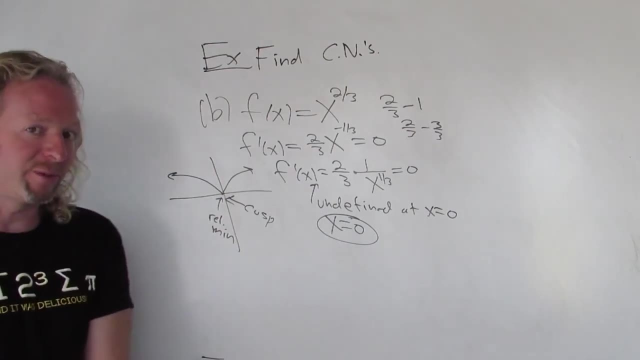 This is a good example. You have a function that has a relative minimum And the critical number arises because the derivative is undefined. It's a little bit different than the previous example. Let's do another example, Another one, C. Let's look at this one. 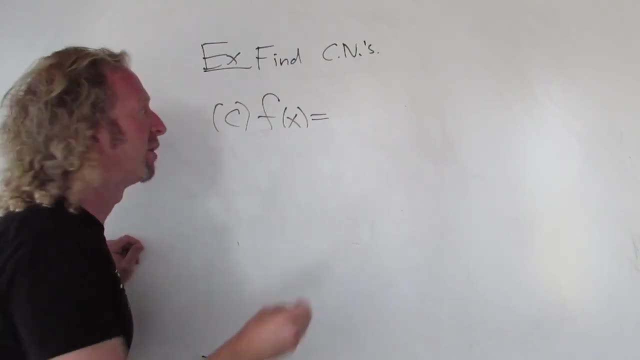 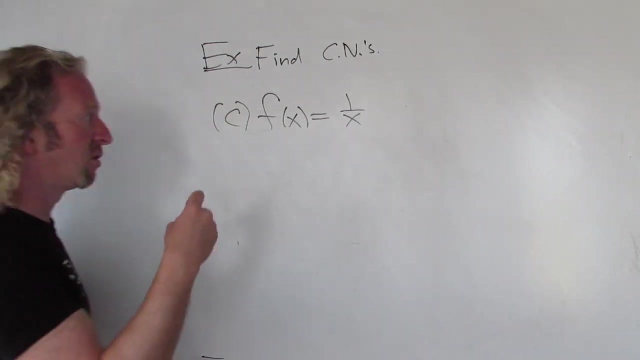 f of x equals 1 over x. So the domain here is all numbers except 0. So 0 could never be a critical number. So how do we do this? We start by taking the derivative. So to take the derivative of this, you first write it like this: 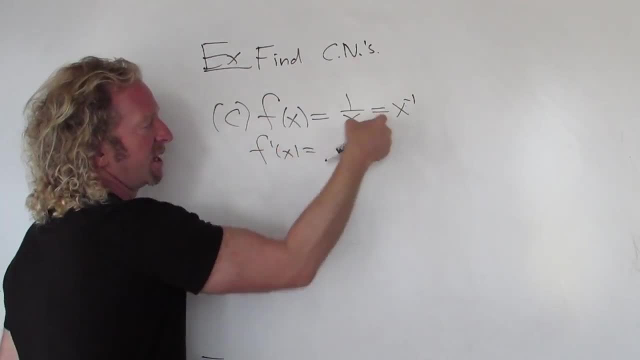 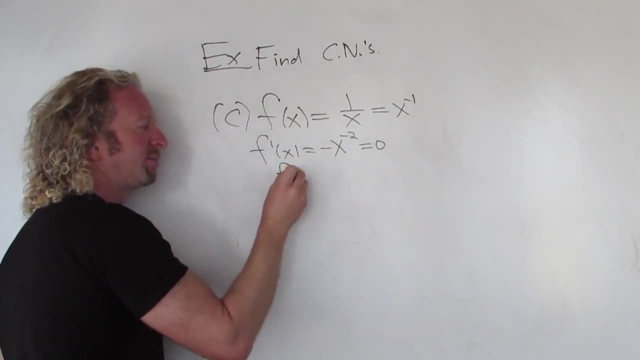 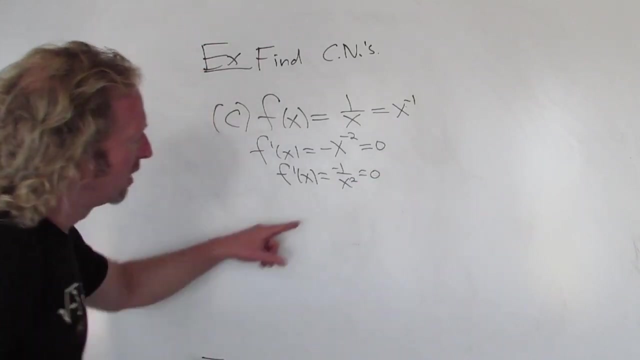 Then you go ahead and differentiate, So you bring the negative down, So you get negative x to the negative 2. And we set this equal to 0. So, rewriting this derivative, We just subtract 1. Write negative 1 minus 1 is negative 2.. 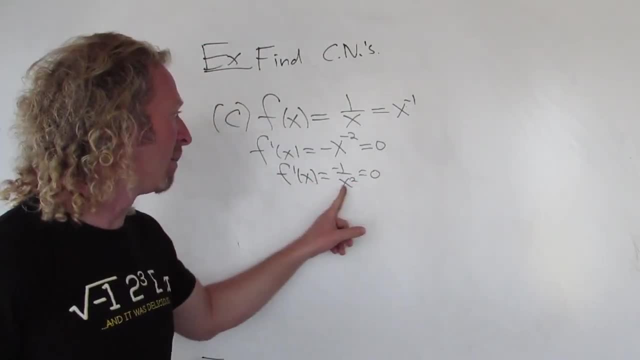 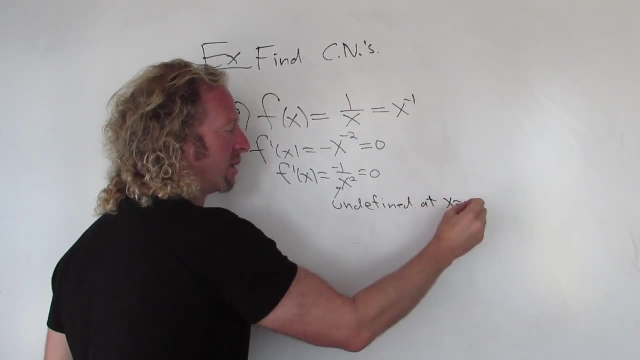 So this is never equal to 0.. That will never be 0. But this is undefined at 0.. So this is undefined at x equals 0.. This is undefined at x equals 0.. However, 0 is not a critical number of this function. 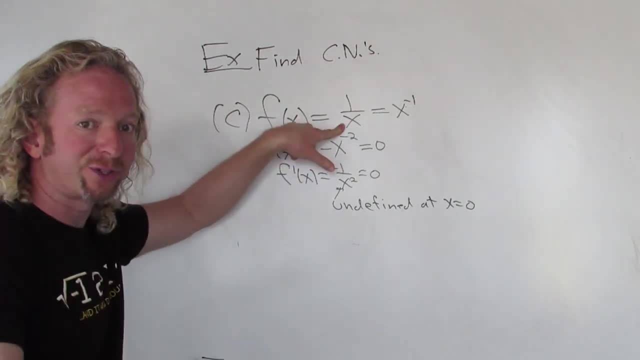 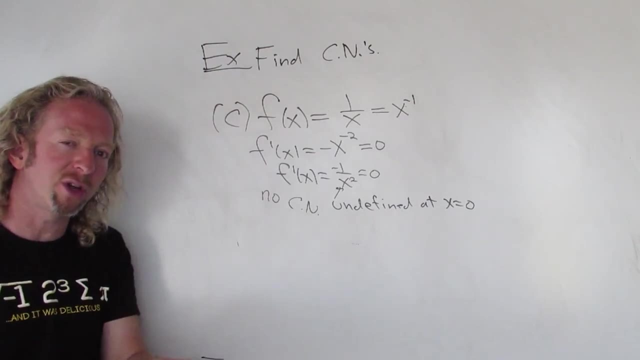 And the reason is: 0 is not in the domain, It's in the domain of the original function. So in this case there are no critical numbers. So you have to be really, really careful. So when you're looking for critical numbers, you take the derivative. 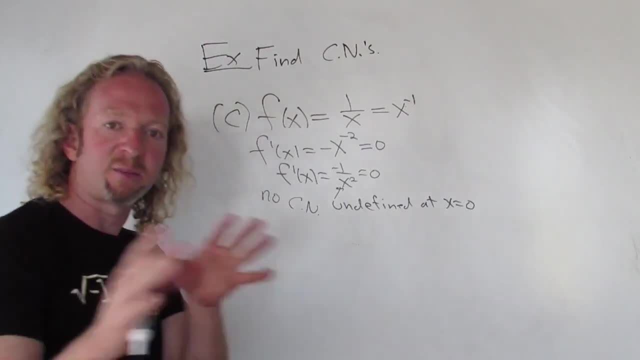 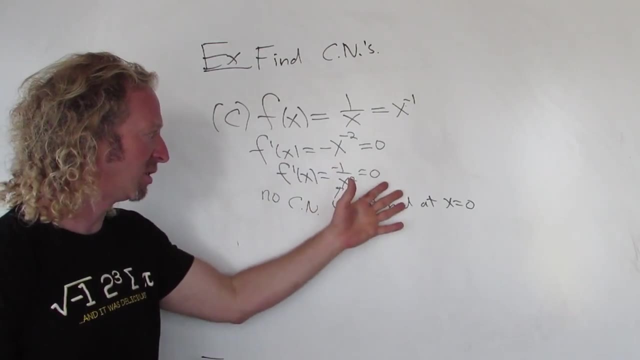 You look at it, You ask yourself: OK, is it undefined? If it is, it's a possible critical number. You set it equal to 0.. Look for those answers. You take all of those numbers, the ones where it's undefined and where it's equal to 0.. 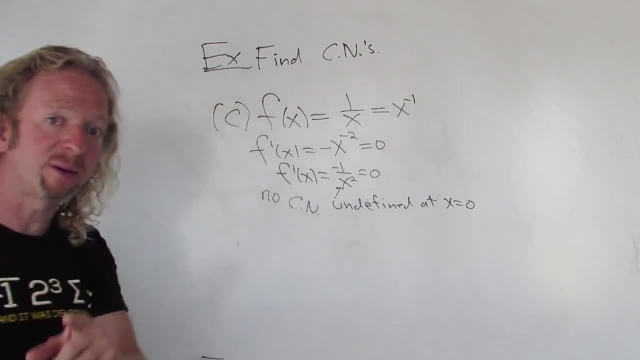 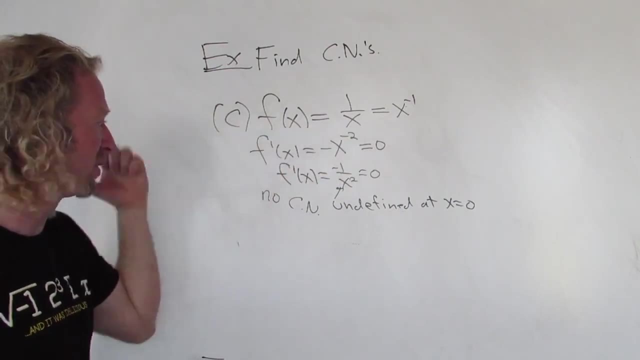 And you ask yourself: are they in the domain of the function? If they are, they're critical numbers. If they're not, then no good. So in this case, it's never 0. It's undefined at 0. However, 0 is not in the domain of the function. 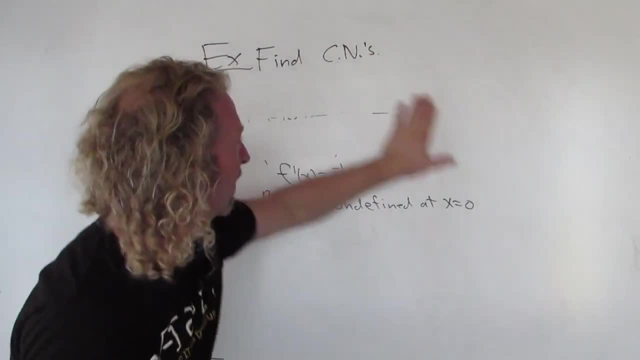 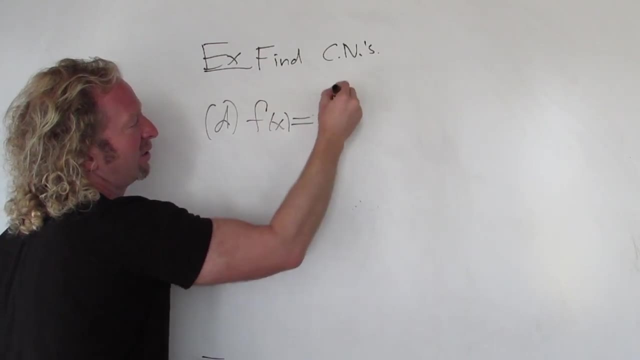 Fail No critical numbers, Let's do another one. D: How about this one? f of x equals x cubed, x cubed, x cubed. By the way, that had a vertical asymptote at 0, right. 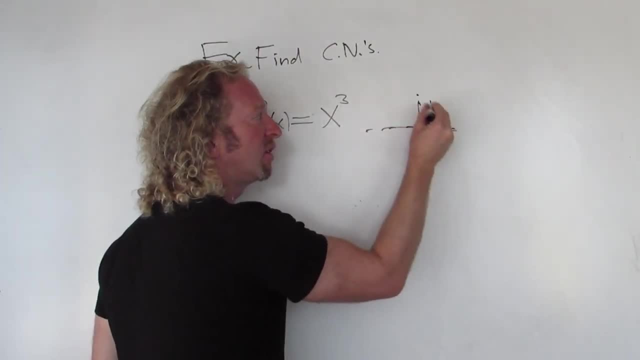 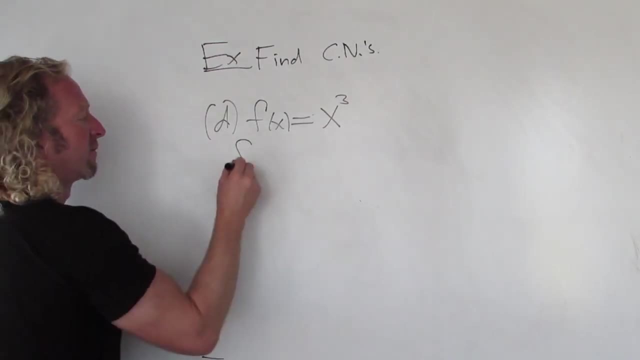 1 over x. I forgot to mention it Looks like that right. So not even defined there. right Doesn't make any sense. x cubed, So let's take the derivative. Oh, this is defined everywhere, right. 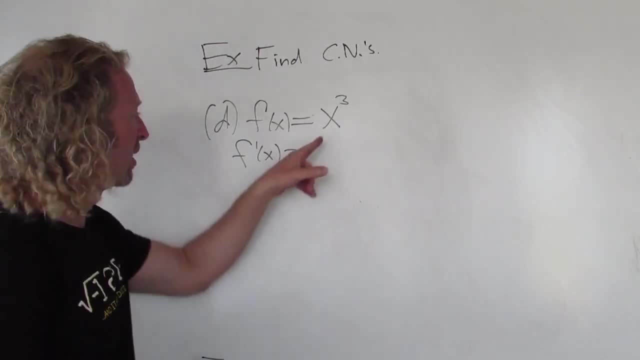 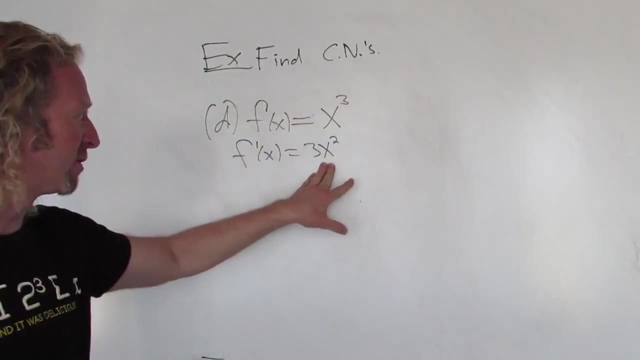 x. cubed is a nice, pretty graph. It's a polynomial, so the domain is all real numbers. When you take this derivative you put the 3 in the front, so you get 3x squared. This is never undefined, so we're not going to get any critical numbers by looking to. 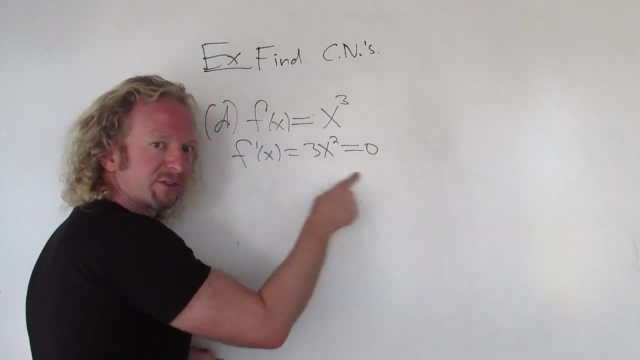 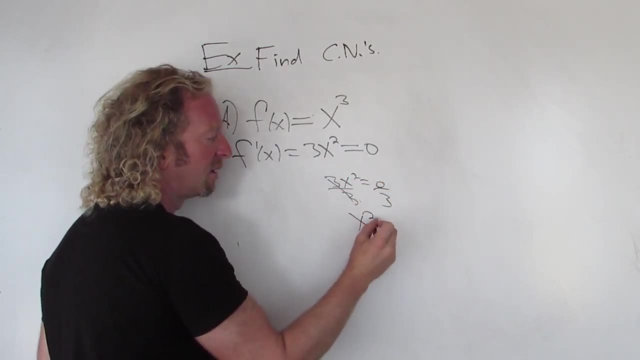 see where that's undefined: 7 equal to 0. We can solve this for x by dividing by 3.. So you end up with this. Then you divide by 3.. Take the square root, so you get 0.. So 0 is a number where the first derivative is 0.. 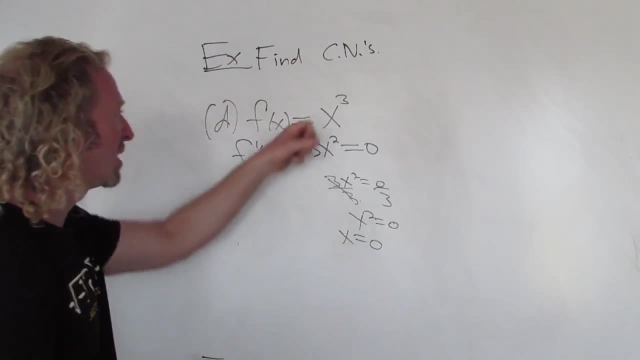 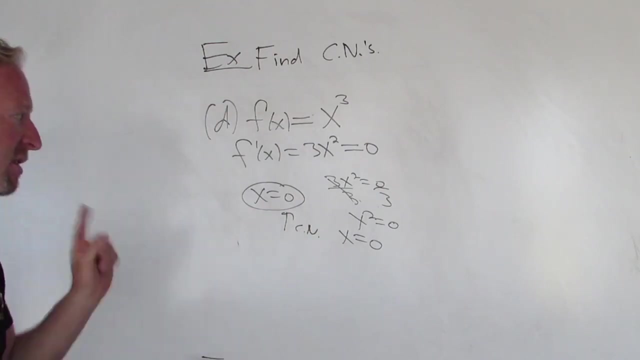 Then you ask yourself: OK, Is 0 in the domain of the function? Well, yes, it is right. So in this case, this is a critical number. So this is a critical number. This is an interesting example, because in this case you have a critical number. 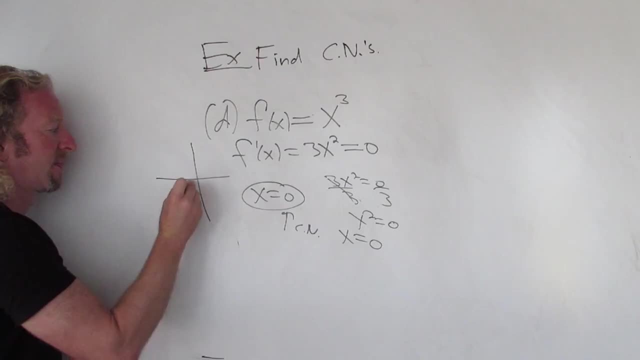 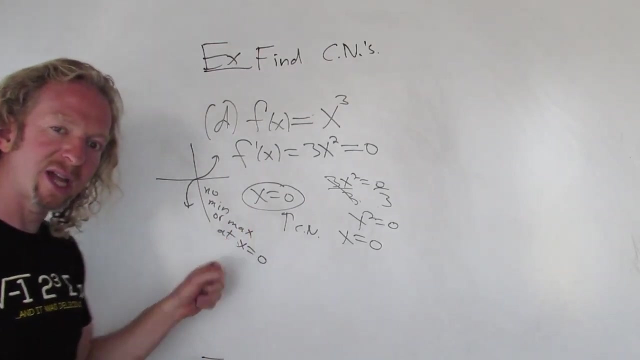 But if you look at the graph of x cubed it looks like that right. So there's no max or min. So there's no min or max at x equals 0.. So this is an example of a function that has a critical number but does not have a relative max. 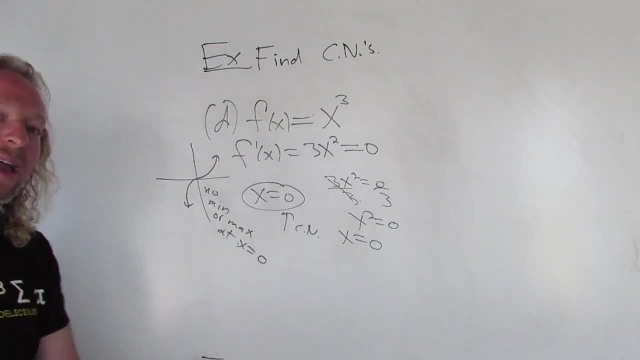 You might say what You said it did No. no. If you have a relative max or a min, then you have a critical number. If you have a critical number, that doesn't mean you have a max or a min. 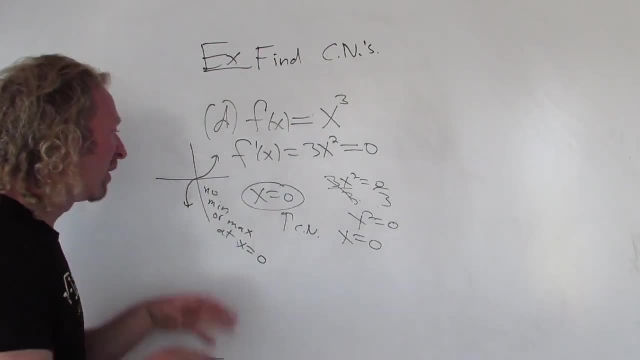 So again, if you know you have a max or a min, then you know you have a critical number. But if you have a critical number, that doesn't mean you have a max or a min. So it only goes one way. So I hope this video helped your understanding of critical numbers. 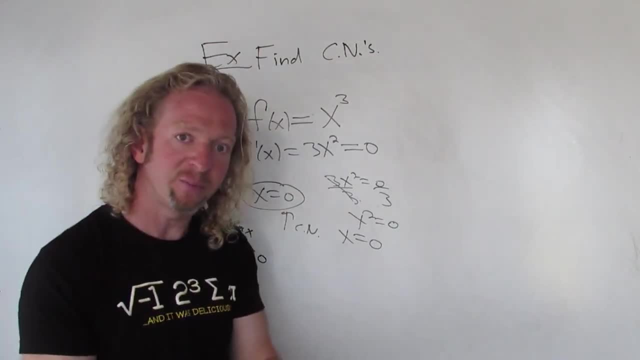 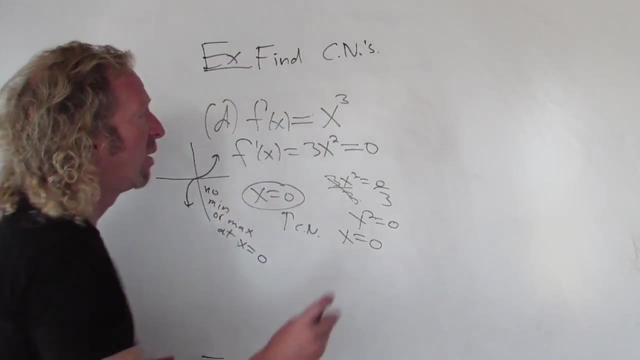 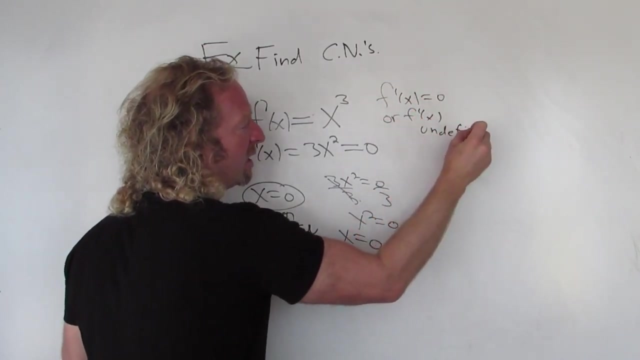 So recap, Critical numbers are numbers in the domain of the function Where the function's derivative is 0 or undefined. So again, critical number is a number of the domain where either the derivative is 0 or the derivative is undefined. So they're numbers in the domain of the function where the derivative is undefined or at 0.. 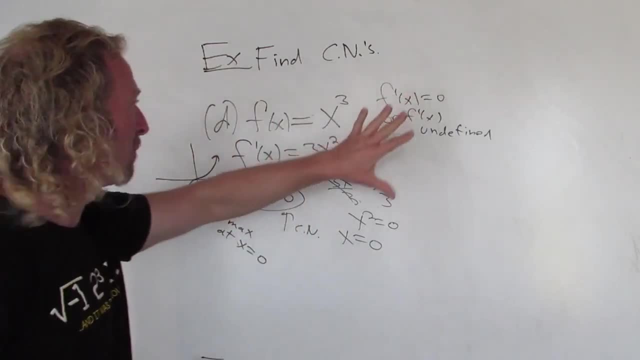 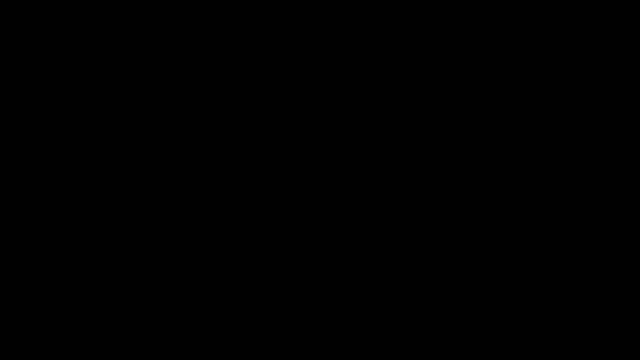 Derivative is undefined or at 0. And they have to be in the domain of the original function. Super, super key. In this video we're going to discuss one of the most important theorems in calculus. It's called the extreme derivative. 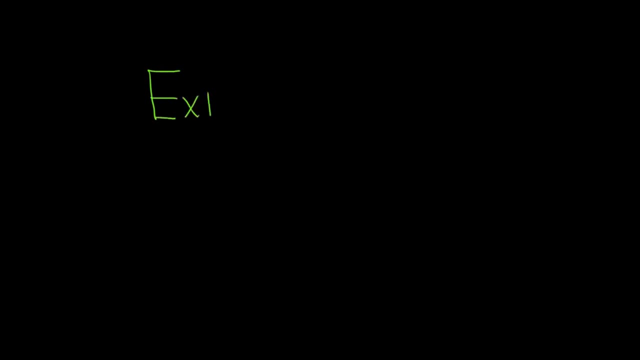 Extreme value theorem. So extreme value theorem. The extreme value theorem basically says that every continuous function on the interval a, b has an absolute maximum and minimum And the interval has to be closed, So we have to include the endpoints. So it says that every 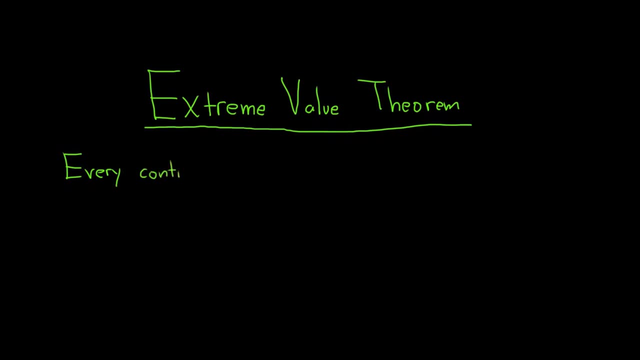 Continuous function. So continuous function On the interval a- b Has an absolute maximum and an absolute minimum. Has an absolute maximum And an absolute minimum. So I'll just say: and minimum. Well, I'll say it again, And an absolute. 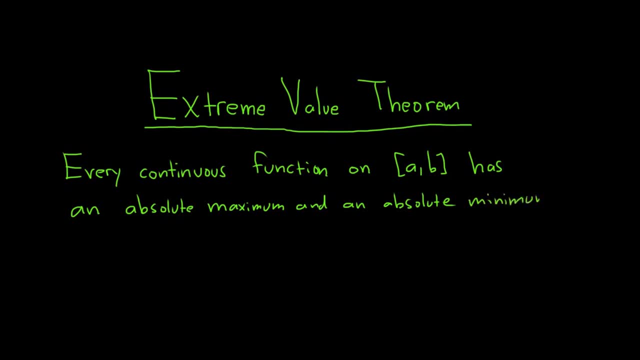 Minimum, Both. So let's go ahead and do an example of applying the extreme value theorem To find the absolute maximum and minimum of a function on a closed interval. So I have one here. I haven't done it, But it looks like a decent first instructive example. 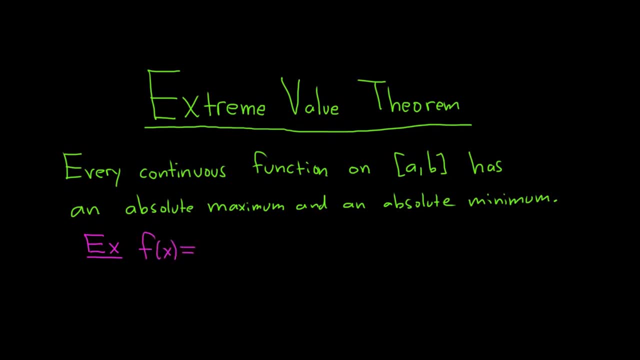 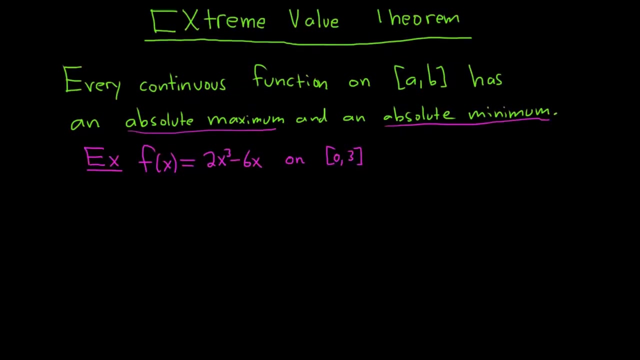 So f of x is going to be equal to 2x cubed minus 6x, And we're going to find the absolute maximum and absolute minimum of this function on the interval. So the way to do this is think about it as follows. 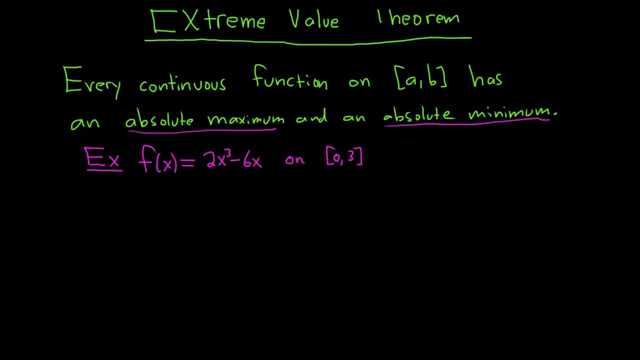 Recall if a function has a critical number. Or rather, if a function has a maximum or a minimum, Then it has a critical number. So critical numbers could be maxes and mins. The other place where you could have a max or a min is at the end points. 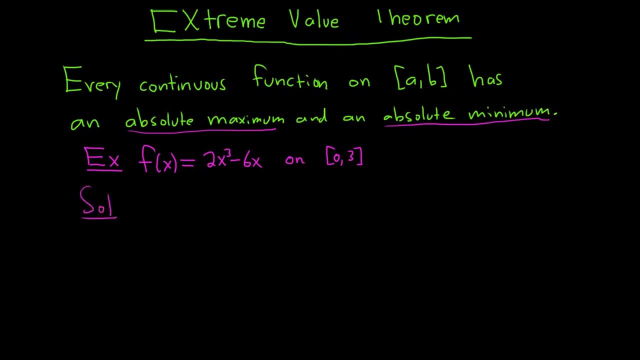 So in these problems all you do is you first find the critical numbers That are between 0 and 3. So step 1.. You find the critical numbers, So find cn's In 0, 3. Because critical numbers could lead to maxes and mins. 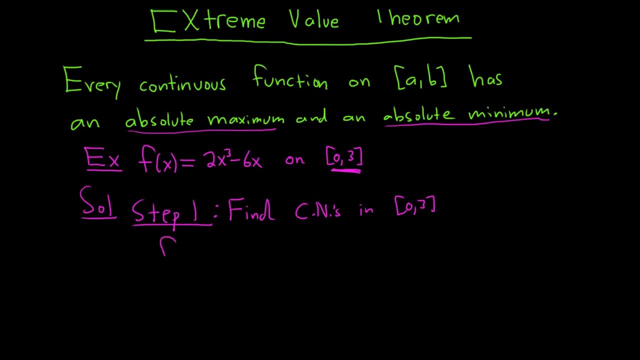 Not always, but they could. So to find the critical numbers, you take the derivative of the function And you look to see where it's undefined or where it's 0. So taking the derivative here, we will get 6x squared minus 6.. 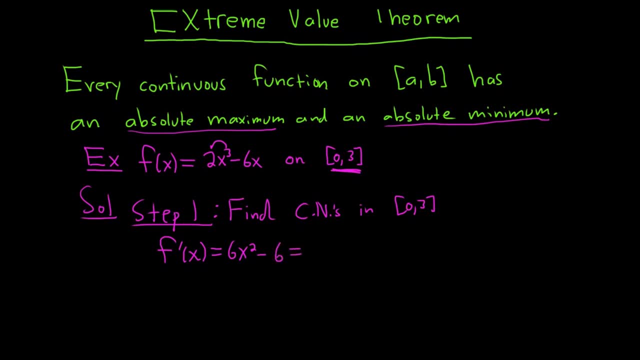 So this is never undefined, And so now we set it equal to 0.. Alright, So let's see, I guess we can add 6.. So we get 6x squared equals 6.. Divide by 6.. Divide by 6.. 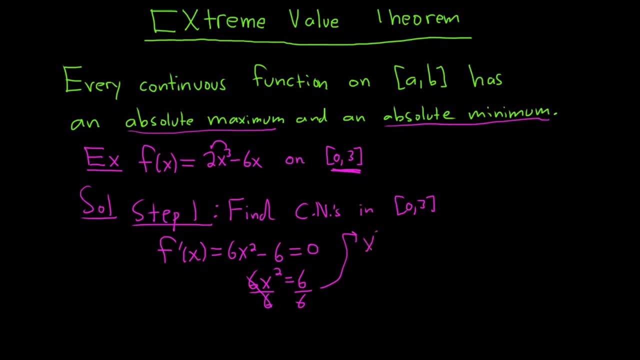 So we end up with x squared equals 1.. And when we take the square root, we do get x equals plus or minus 1.. However, we only care about critical numbers that are in our intervals. So negative 1 is not between 0 and 3.. 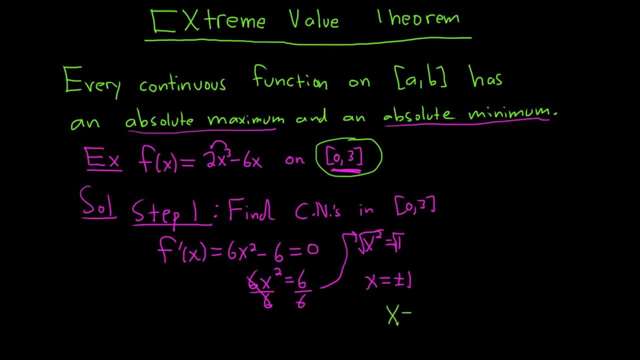 Right, So we only include 1.. So 1 is our critical number. This is our cn critical number. Alright, Now we just have to figure out if it's actually a maximum or a minimum Or nothing at all. So what we do is we just take it and we plug it into the function. 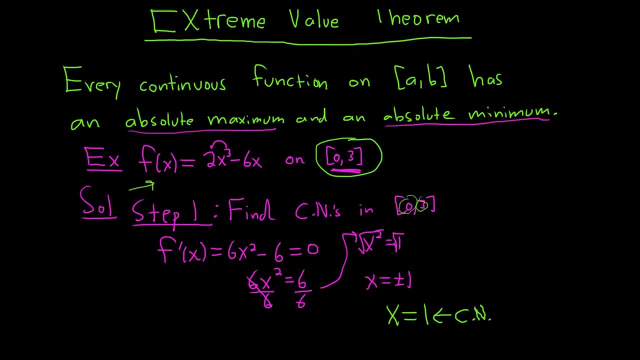 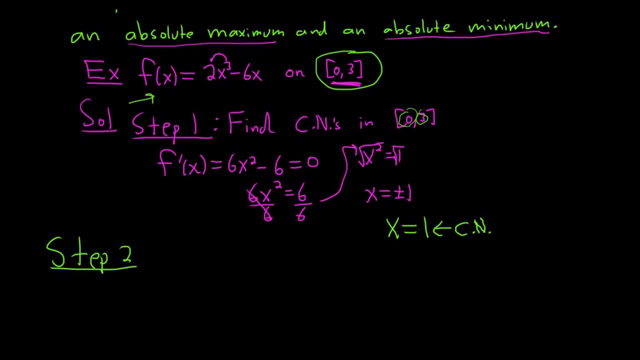 Along with the endpoints. The biggest number we get is the max and the smallest is the min. So step 2. Is plug cn, Cn's, So critical numbers If there's more than 1.. And endpoints. So the endpoints are the a and the b. 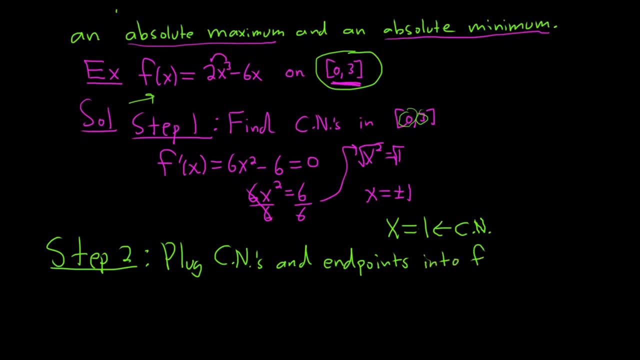 So the 0 and the 3. Into f of x, And the biggest number is the max, The smallest is the min. So let's go ahead and do it. Let's do f of 0. So plugging in 0 into our function here. 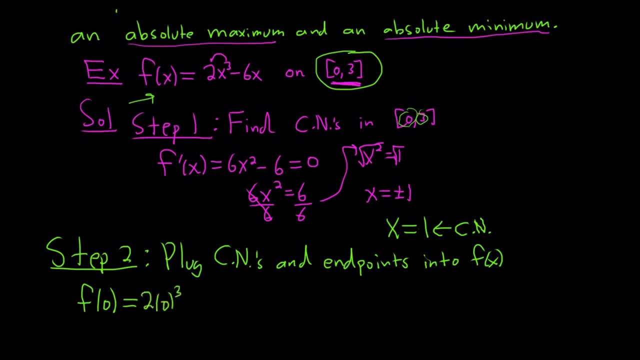 We get 2 times 0 cubed Minus 6 times 0. So we just get 0.. So f of 0 is equal to 0.. Let's do 3 now f of 3. So we get 2 times 3 cubed. 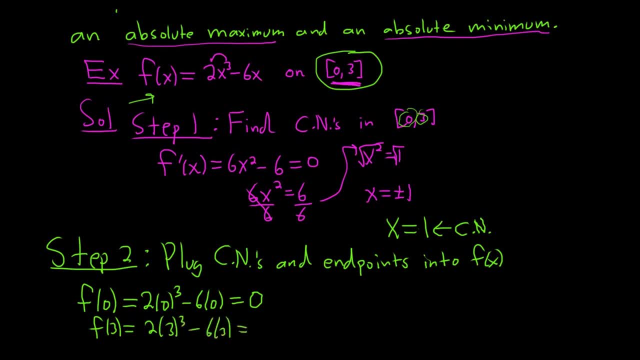 Minus 6 times 3.. Okay, So 3 cubed is 9 times 3.. Right, 3 times 3 times 3.. So 2 times 3 cubed is going to be 54.. So this is 54.. 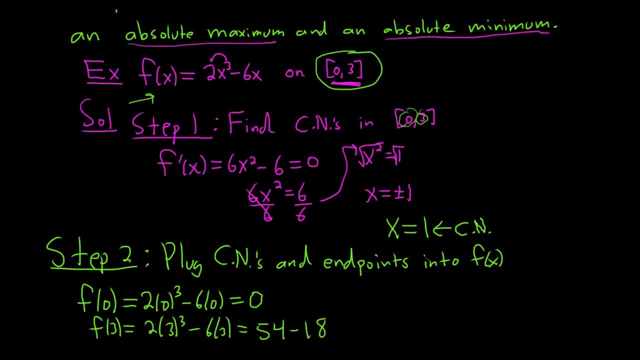 Minus, And then 6 times 3 is 18.. And 54 minus 18 is 30. 36.. So 36.. So we've checked our endpoints And now we just have to check our critical number. So f of 1.. 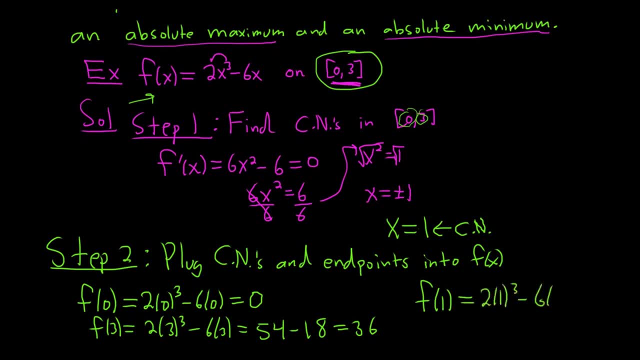 This is 2 times 1, cubed Minus 6 times 1.. This is 2 minus 6.. So it's negative 4.. So that's negative 4.. Okay, So all we do now is write the answers down. 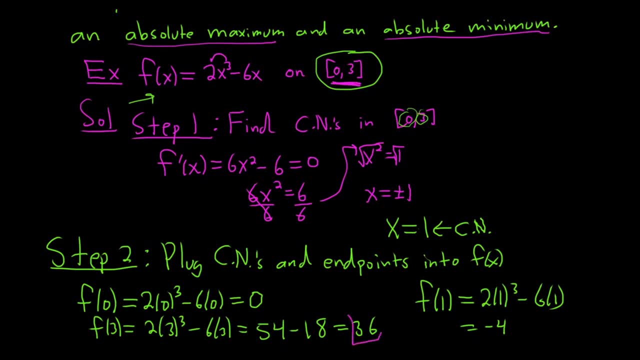 So the biggest number is going to be our maximum, So it looks like 36 is our maximum- So we did have the max at an endpoint in this case- And our minimum, Our minimum, is negative 4.. That's the smallest one. 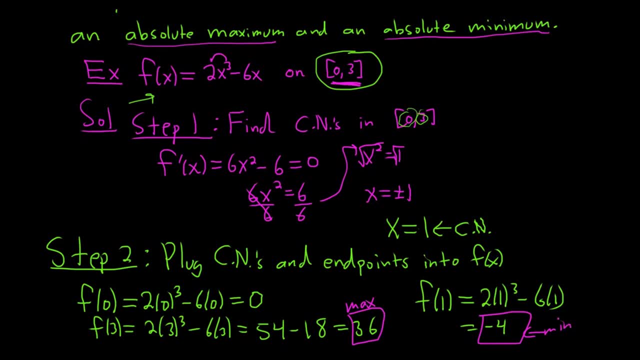 So that's our minimum, And that's it. That's the extreme value theorem and how you use it. So the extreme value theorem says that whenever you have a continuous function on a closed interval, you're always going to have an absolute max or an absolute min. 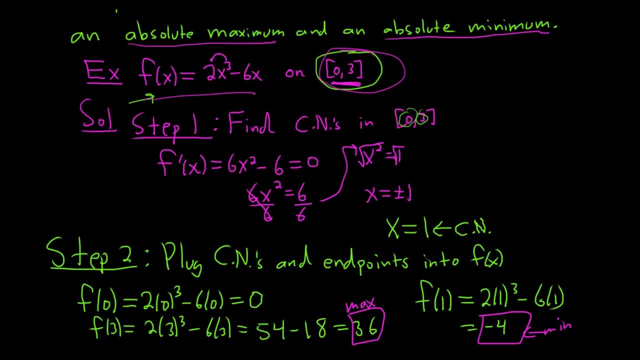 And the way to find it is: you take the critical numbers, Find those, Find the ones that are in your interval. Then plug in the critical numbers, along with the endpoints, into your original function. The biggest answer you get is the max, The smallest is the minimum. 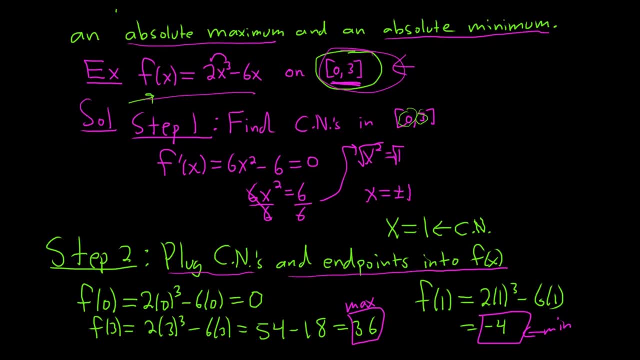 The smallest is the min. Sometimes you can have the max appear twice. You could have a function that does this. You could have the max appear three times. You have 1,, 2, 3 maxes, 1, 2,, 3, 4 mins. 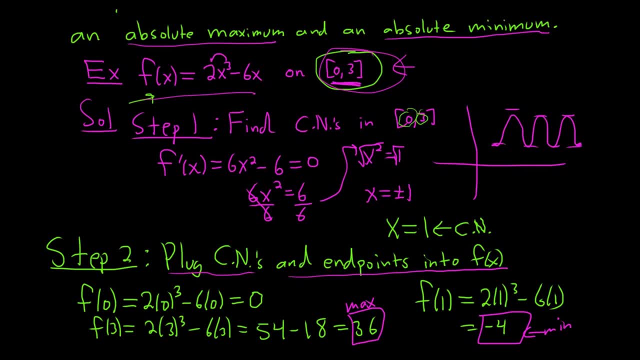 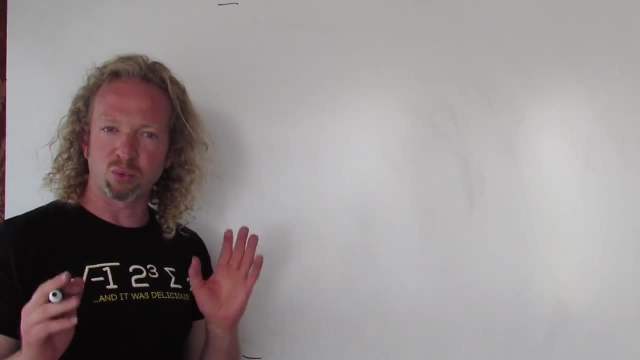 That could happen. It could happen multiple times. I hope this video has been helpful. Hey everyone, In this video we're going to talk about a very important theorem in calculus called Rawls theorem. So let's go through it carefully and then we'll do an example. 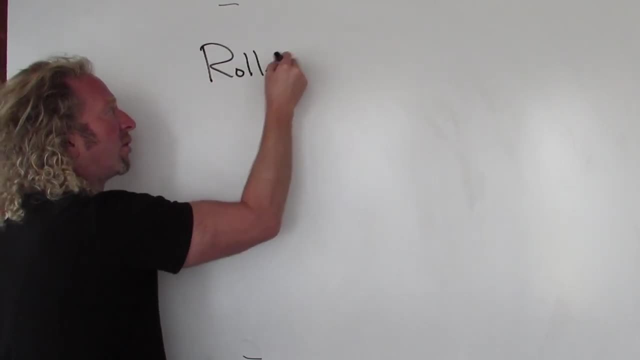 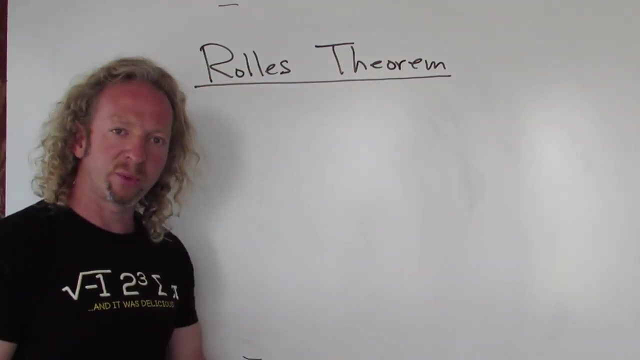 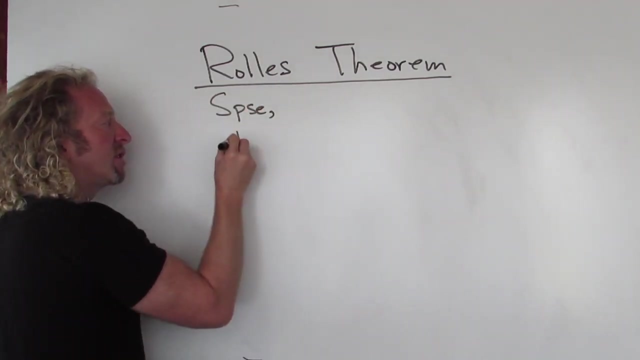 So Rawls theorem, Rawls theorem. So the conditions for Rawls theorem are really, really important. So let's state them carefully. So suppose there are three conditions. So the first condition is that your function is continuous on a closed interval. 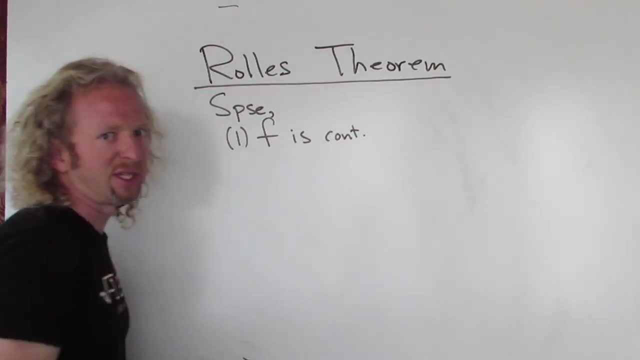 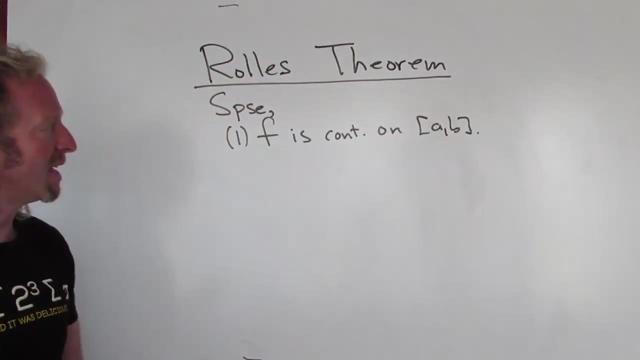 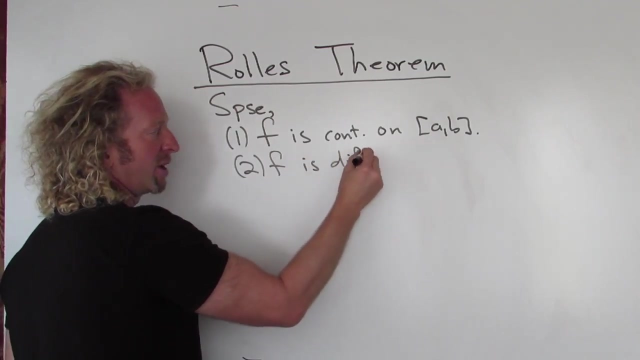 So f is continuous. I'll just put c, o and t on, say, the closed interval a- b. Second condition is that it's differentiable on the open interval, So 2. f is- I'll just put diff- differentiable on the open interval a b. 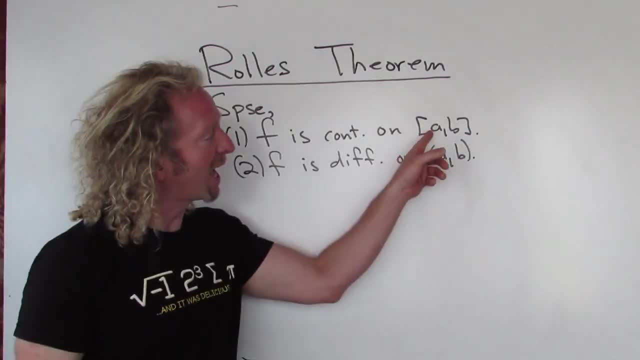 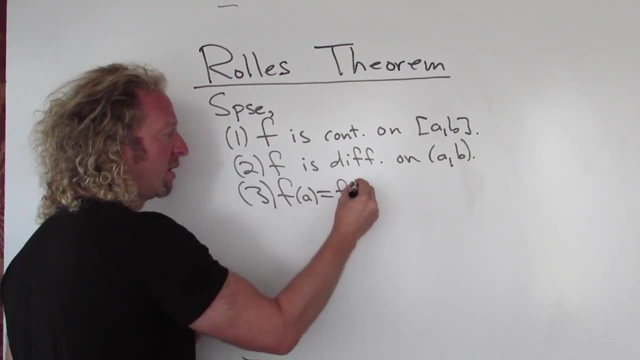 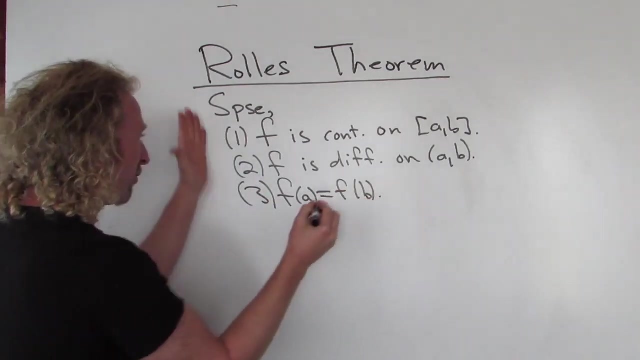 Third condition is that the function values at the endpoints are the same, So 3.. f of a is equal to f of b. So if these three conditions are satisfied, then you can invoke Rawls theorem. So if all three conditions hold, then there is a number. 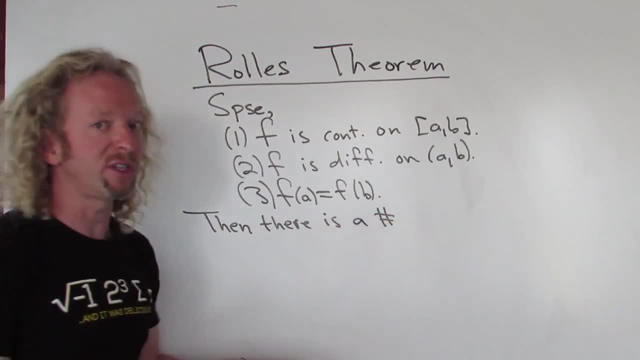 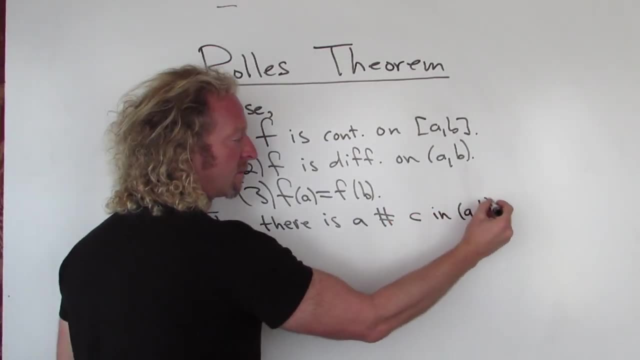 I'll use the pound sign for number. Now there could be more than one, as you'll see in a minute when we look at the pictures. So then there is a number c in the open interval, such that as t means such that, 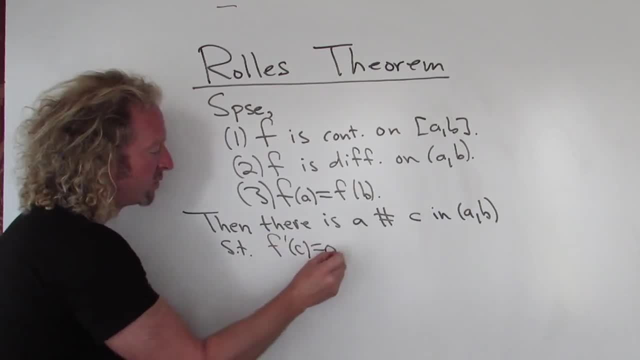 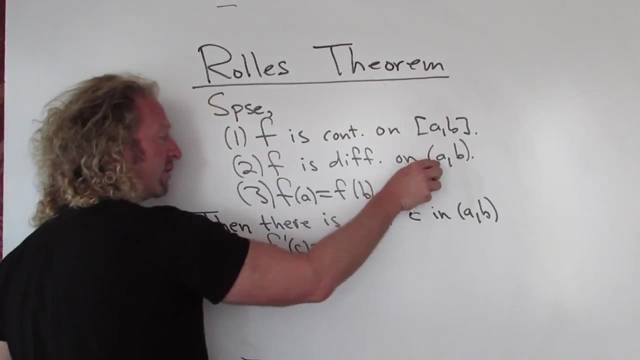 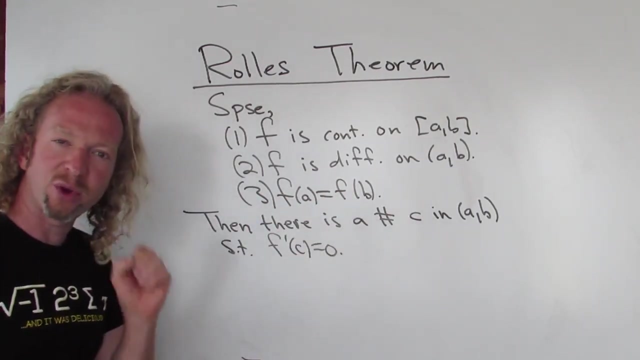 the derivative at c is equal to 0.. Rawls theorem says: if you have a continuous function, if the function is continuous on the closed interval, differentiable on the open interval and the y values are the same at the endpoints, then you can find the number in the interval where the derivative is 0.. 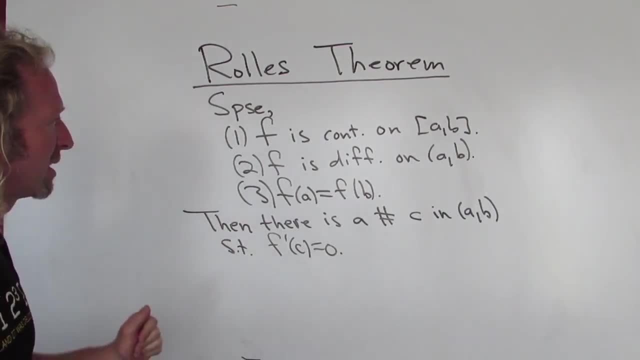 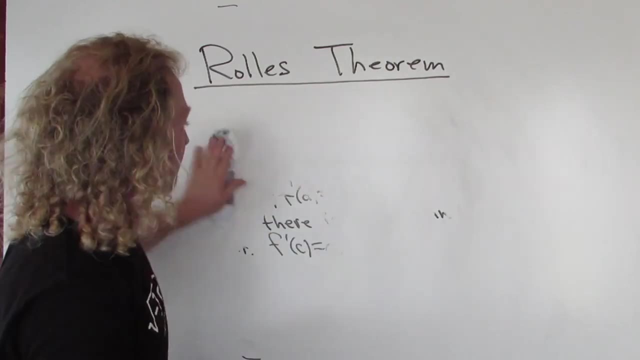 So let's look at a picture so that it makes sense. I'm going to go ahead and erase the conditions and we'll go through them again in a minute. So I'm going to erase this. I'll leave the title of the theorem up. 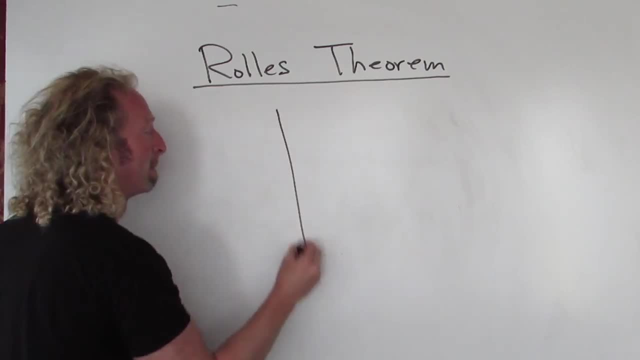 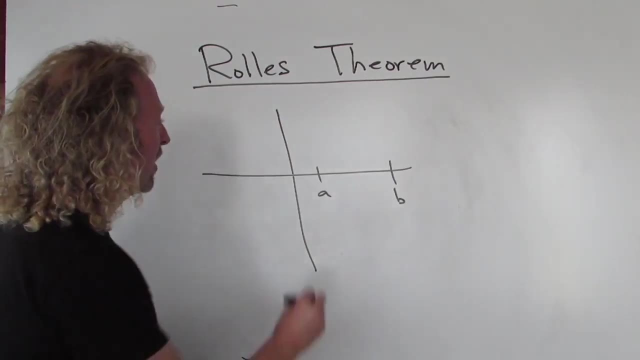 It looks good, All right. So here's some pictures. Check this out. So here's a and here's b. Let's try to violate Rawls theorem, see if we can do it. So maybe this is f of a, Oh, but the y values have to be the same. 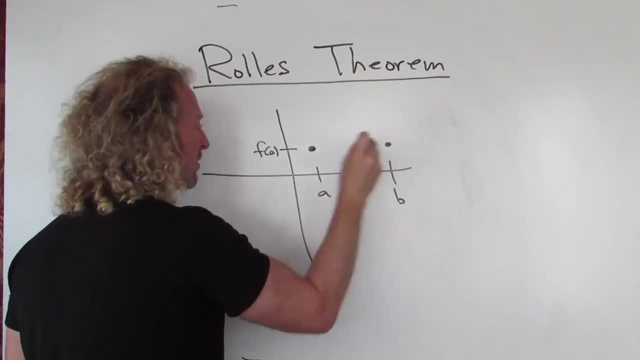 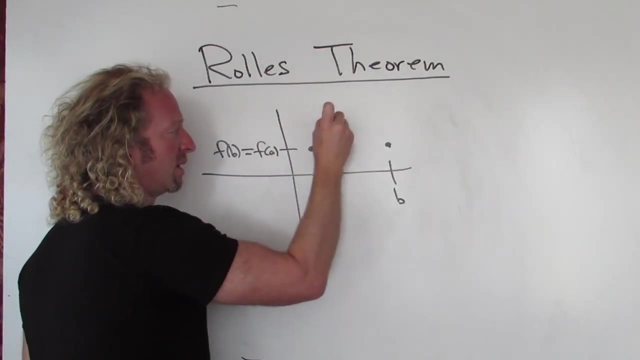 So wherever we start, we have to finish. So this is also f of b. It's one of the conditions in Rawls, And so we have to get from here to here. So one way to do it is like this. Well, if we do that, sure enough, there is a number c. 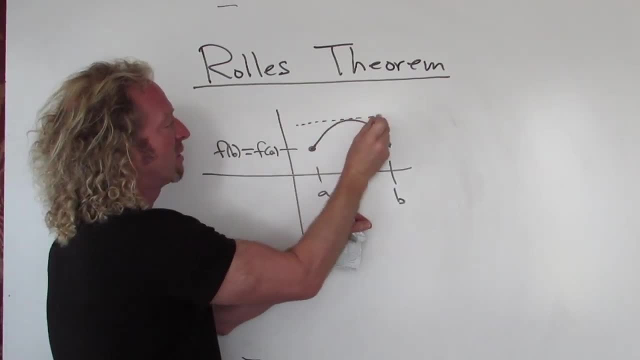 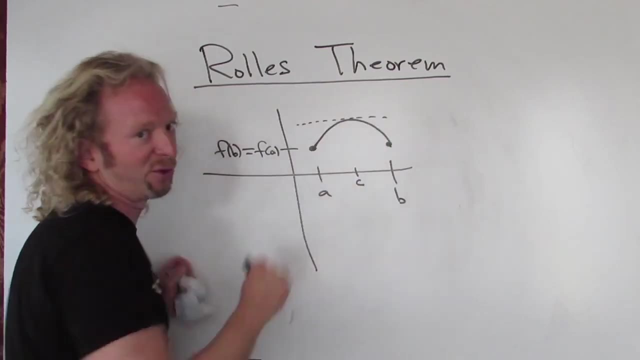 in the open interval where the derivative is 0.. Remember, the derivative is the slope of the tangent line. So in this case you would have a horizontal tangent line here, so the derivative would be 0.. So there would be our number c, where the derivative of the function is equal to 0.. 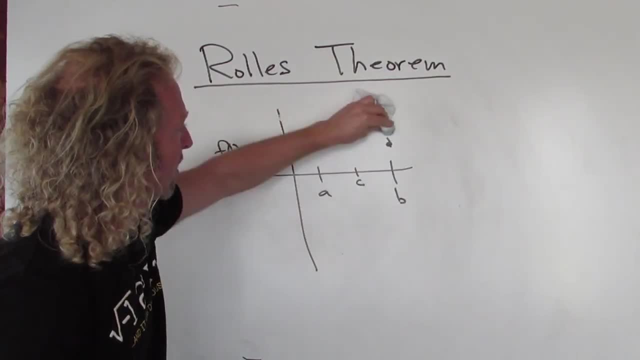 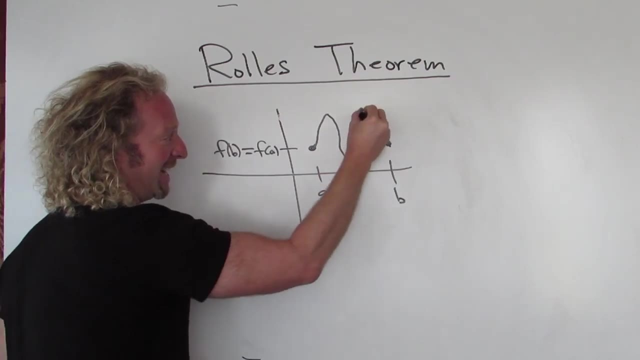 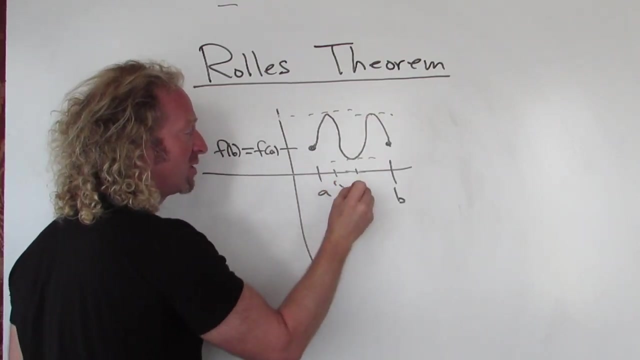 Let's try to break it. What if we do something like this? Let's see What if we do. I got to get to b, All right, Okay, So now there are three numbers. right, There's three numbers. Call it c1, c2, c3.. 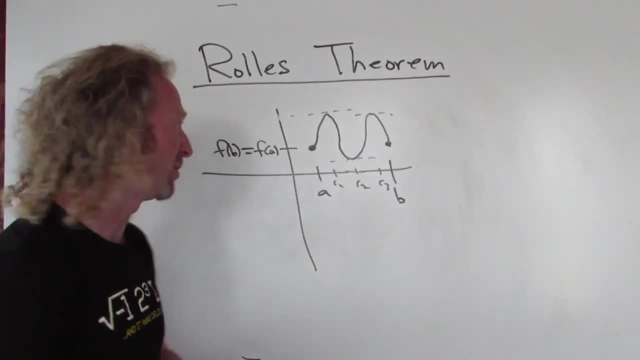 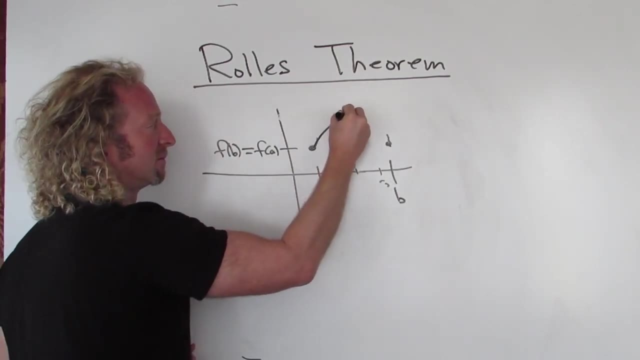 There are three numbers where the derivative is 0. So we weren't able to break Rawls' theorem. What if we try to cheat? Well, we could do something like this, But then that would mean the function is not continuous. So Rawls' theorem requires the function to be continuous. 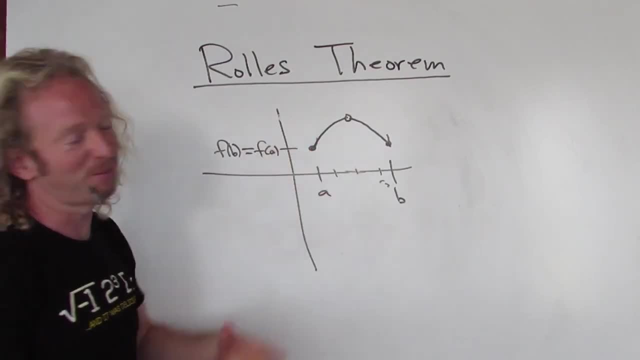 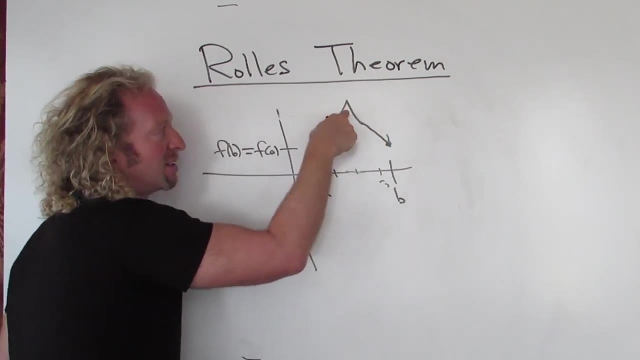 If it didn't. we can break the theorem by doing something like this? right, But we can't because it's continuous. So another way to try to break the theorem is to do something like this: have a sharp edge. In this case, the derivative would be undefined. 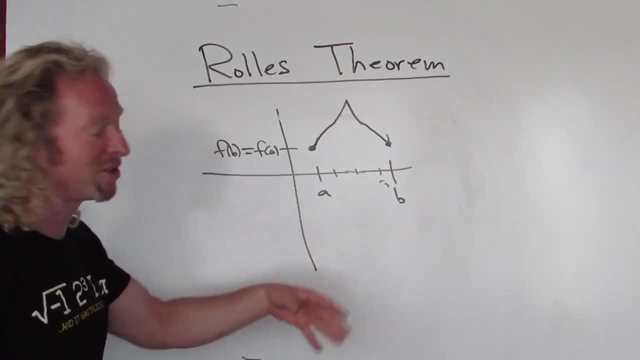 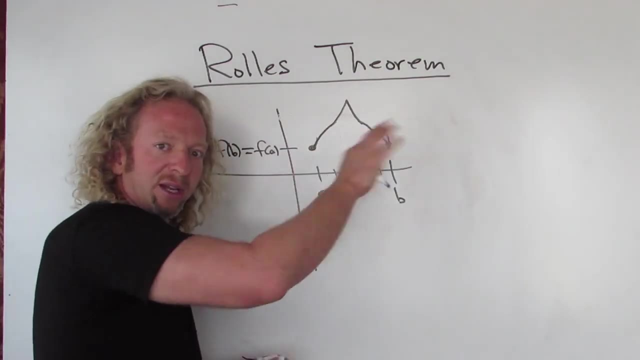 However, we can't do that either, because Rawls' theorem requires differentiability. So now you see why the theorem has those conditions right. It requires continuity because otherwise you could put a little hole there and like the theorem wouldn't work. 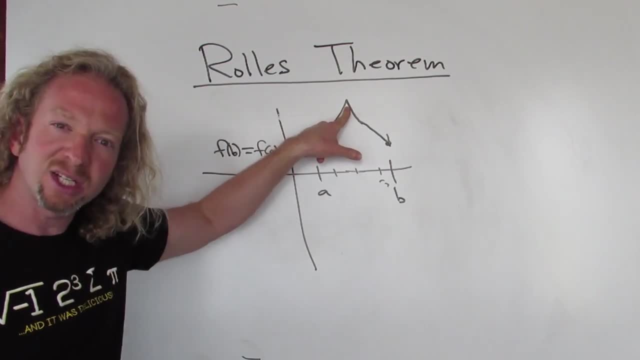 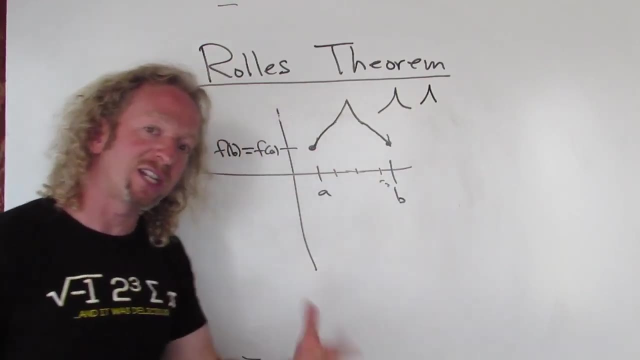 And it requires differentiability, because otherwise you can make little sharp edges like this or cusps- Remember this is called a cusp, That's just a sharp edge, And in both of these cases the function is not differentiable. But we can't do that because Rawls' theorem requires it. 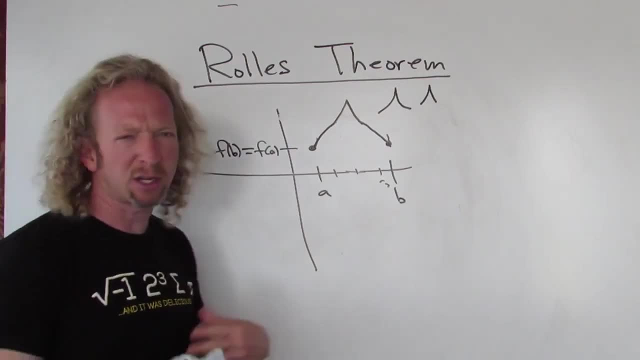 It requires differentiability, So most of the time when you're studying Rawls' theorem, you're in a classroom setting, or maybe you're just, you know, learning about this on your own for fun. Most of the time, though, you have to find c. 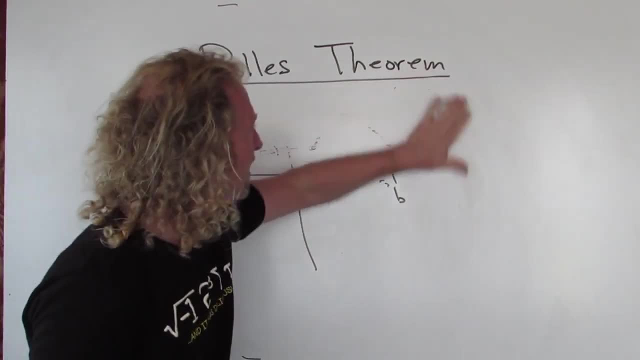 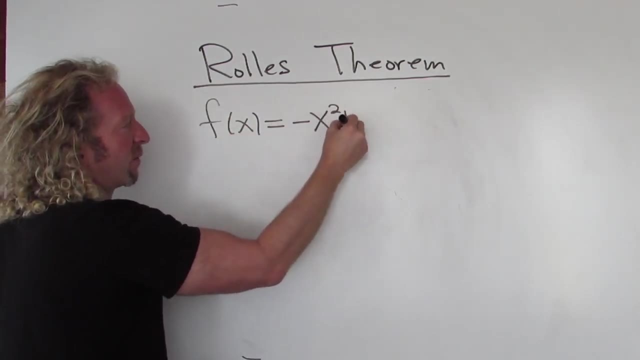 So let's go ahead and do a really simple example of just finding c. So here's a simple example. The function f of x equals: how about this one negative x squared plus 4x? Hmm, I think that'll work. 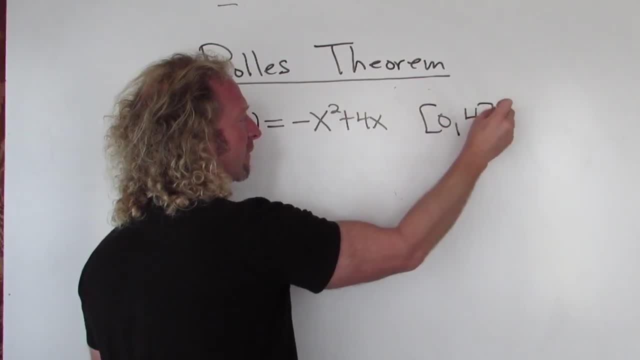 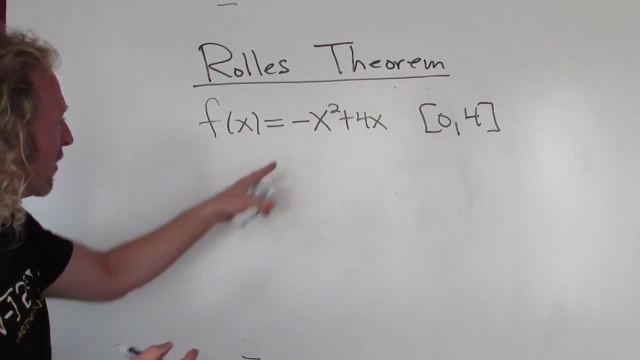 And let's look at the interval 0, 4.. Okay, Yeah, it should work. So let's find the value of c, under which Rawls' theorem holds. By the way, this function is continuous right, because it's a polynomial. 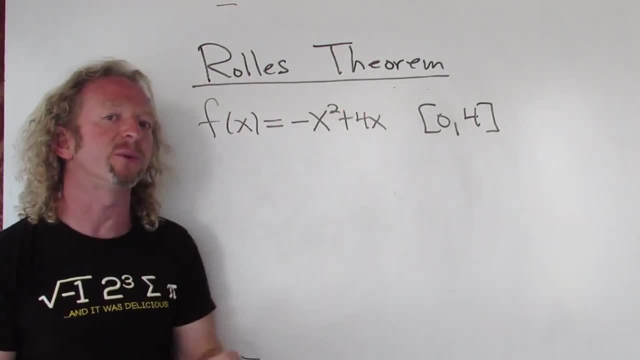 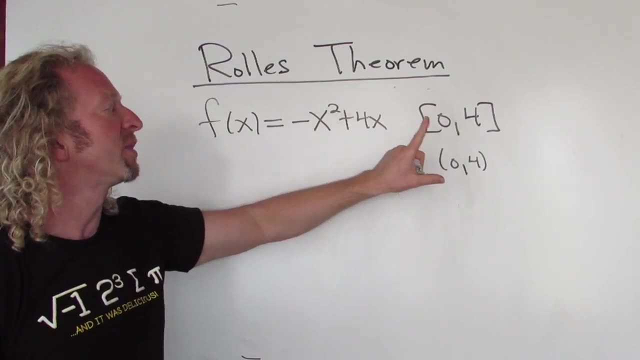 So it's continuous everywhere. In particular, it's continuous on this closed interval. It's differentiable everywhere. In particular, it's differentiable on the open interval. So it's continuous on the closed interval, It's differentiable on the open interval. 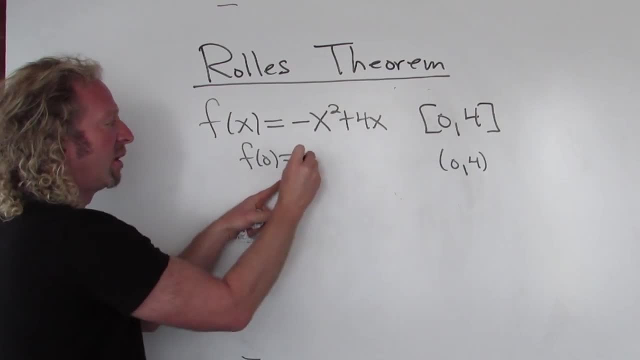 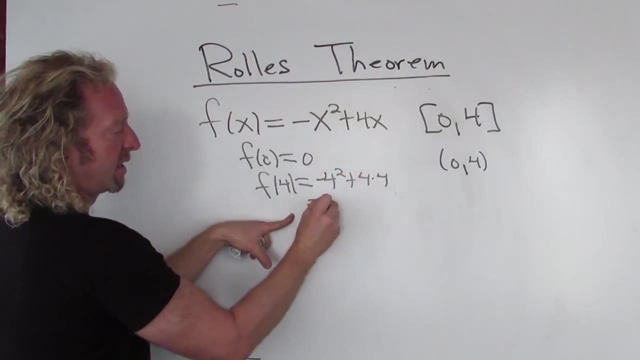 And you can check. You can plug in 0 and get 0.. You can plug in 4. if I did it right, It would be negative 4 squared plus 4 times 4.. This is negative 16 plus 16, so it's equal to 0.. 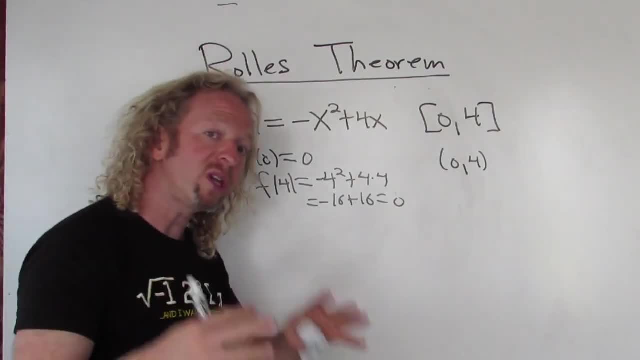 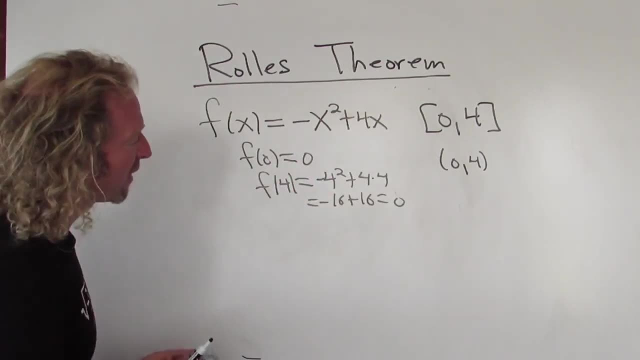 So f of 4 is equal to f of 0.. So all three conditions in Rawls' theorem are satisfied. So there is a number in this open interval where the derivative is 0. Let's find that number. Let's see if we can find it. 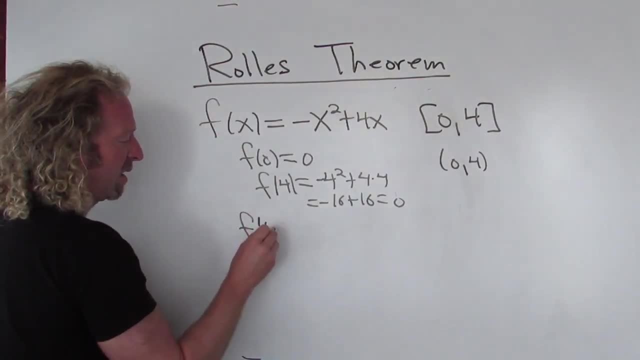 So to find that number, you would take the derivative and you would set it equal to 0.. This is a pretty easy derivative. You just use the power rule, So negative 2x plus 4, and you set it equal to 0. 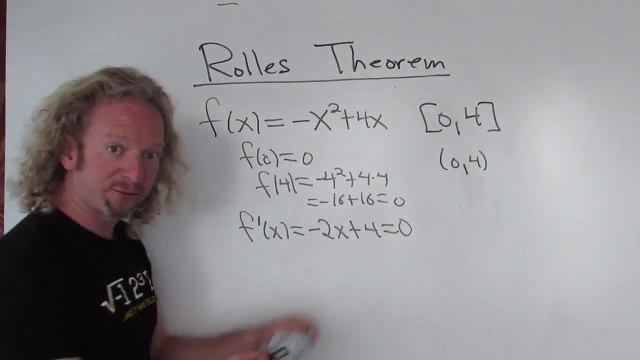 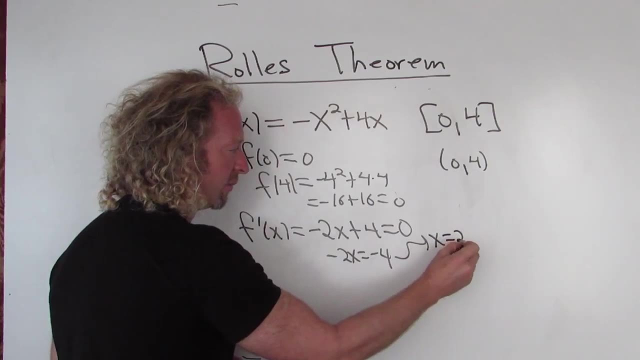 Then just subtract the 4. So you get negative 2x equals negative 4. And then divide by negative 2, so you get x equals 2.. So that would be the value of c. This would be the value of c. 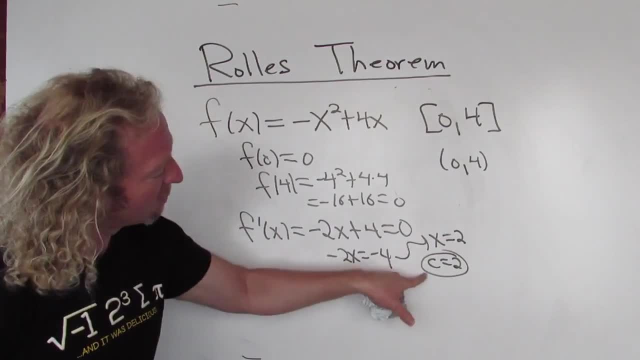 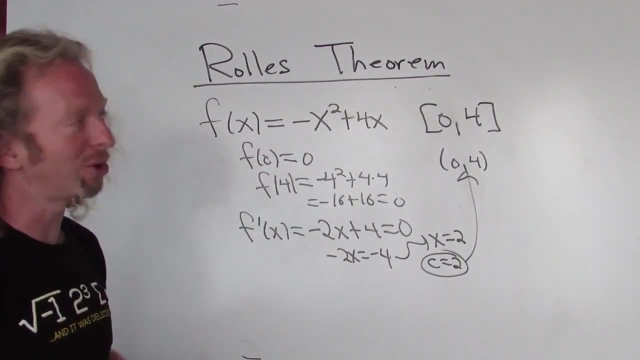 Dividing by the negative gives you a positive. That would be the value of c that lies in this interval. so things are good where the derivative is 0. So Rawls' theorem does work for this, and that's how you find c. 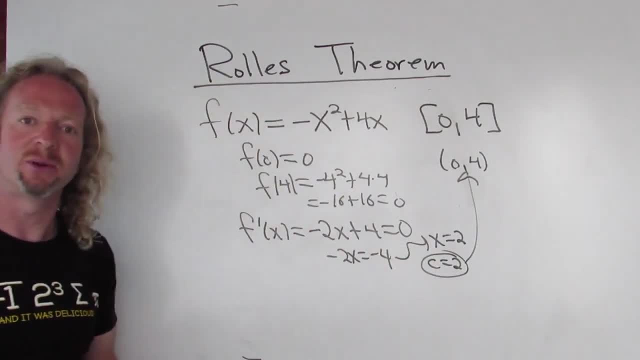 So to find c in Rawls you just take the derivative and set it equal to 0. It's usually pretty straightforward. I hope this video has helped Remember the conditions for Rawls. are it has to be continuous on the closed interval? 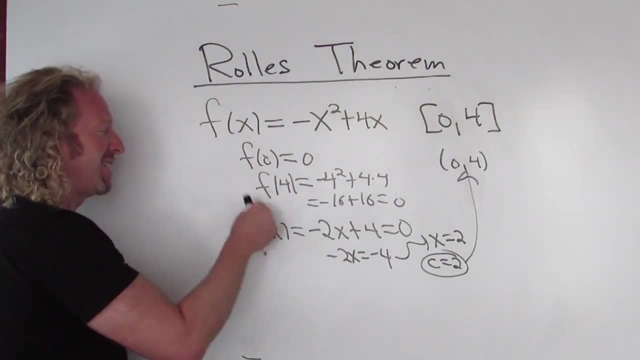 differentiable on the open interval and the endpoints have to have the same function values. And whenever that happens, all it's telling us is there's going to be at least one place where the derivative is 0. In other words, there's at least one place where we have a horizontal tangent line. 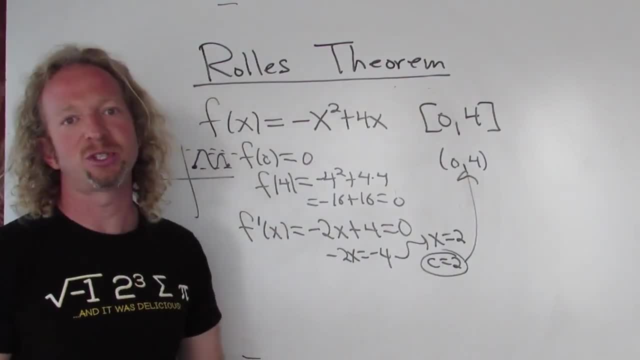 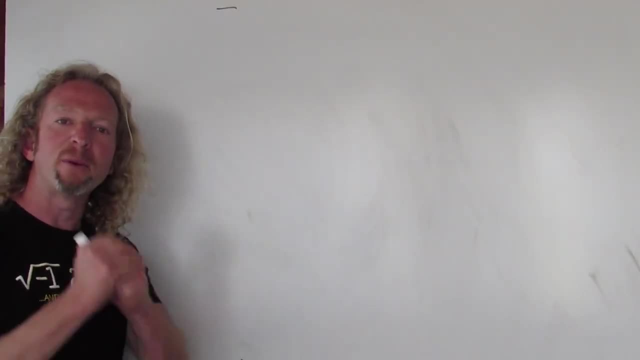 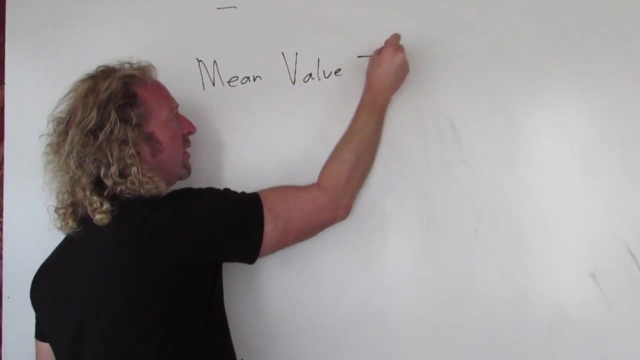 That's it. Thanks for visiting my channel. I hope this video has helped you in some way. Bye, In this problem we're going to talk about one of the important theorems in calculus, called the mean value theorem. So the mean value theorem. 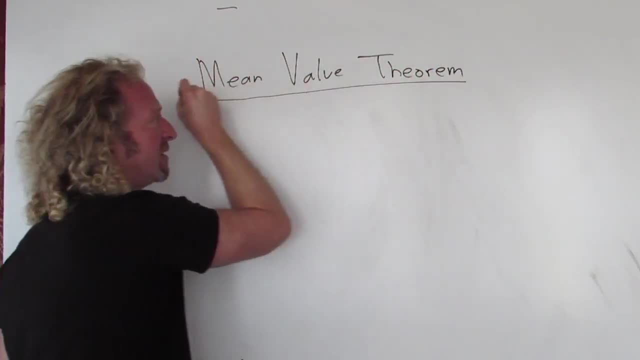 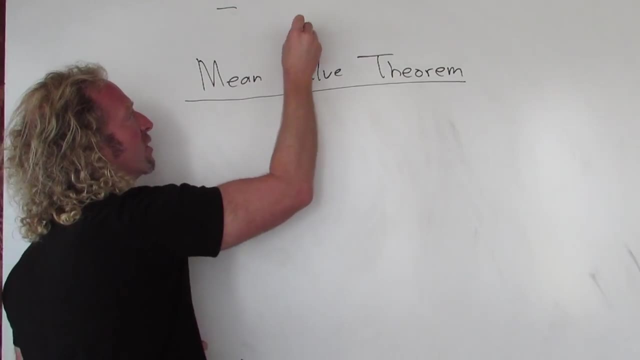 There's a couple mean value theorems in calculus. This is the mean value theorem. This is the first one, the most important one, maybe It's the first one you learn. We can abbreviate it with three letters: m, b, t. 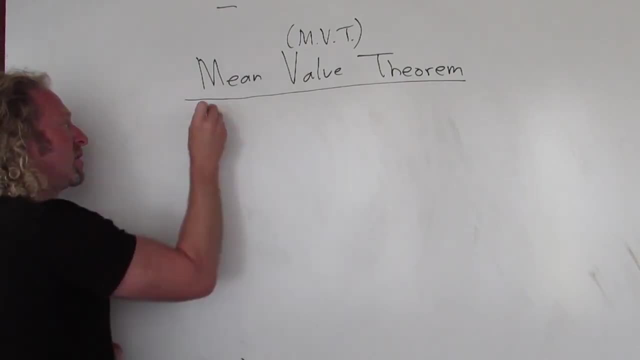 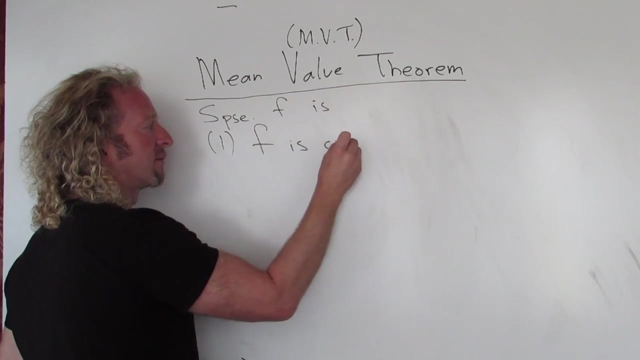 All right. so what does the mean value theorem say? Here are the conditions. So suppose you have a function, f and there's two conditions. So the first condition is that the function is continuous on the closed interval. So f is continuous on the closed interval a, b. 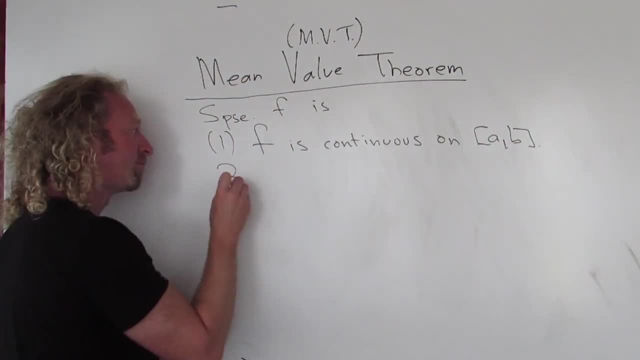 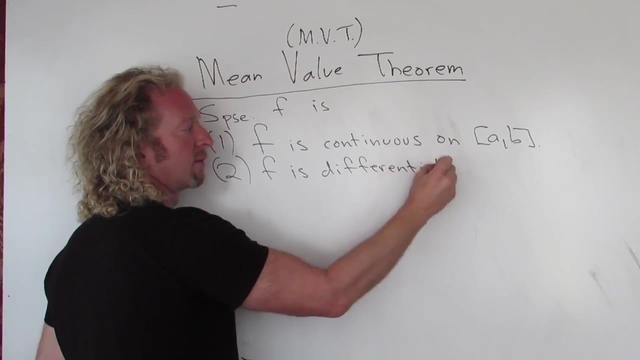 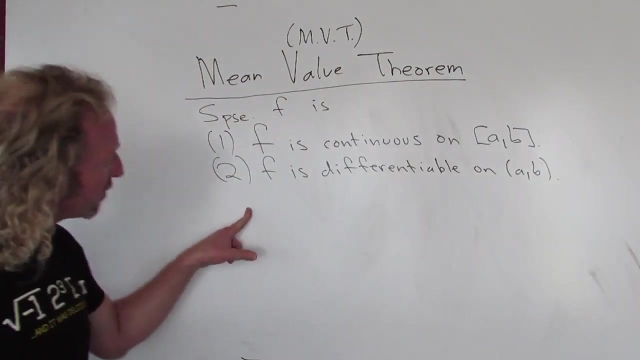 So so far it looks just like Rawls'. theorem Two: f is differentiable. The second condition is that the function is continuous on the open interval. a, b, So far identical to Rawls'. The third condition, well, that's it. 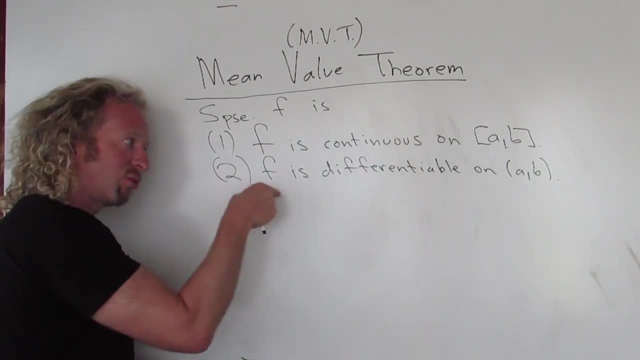 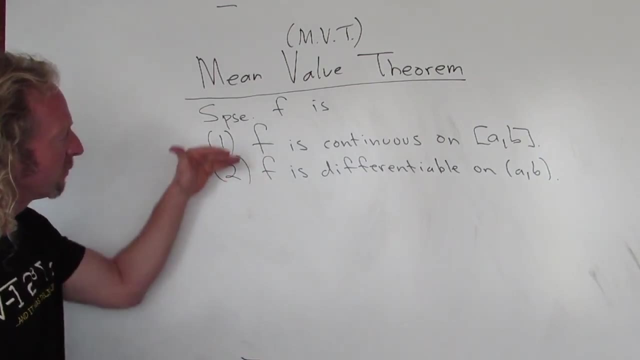 There is no more. If it was Rawls', you would have that third condition where the endpoints are the same right. The y values at the endpoints are equal. But it's not. It's the mean value theorem. So the first two conditions are very similar. 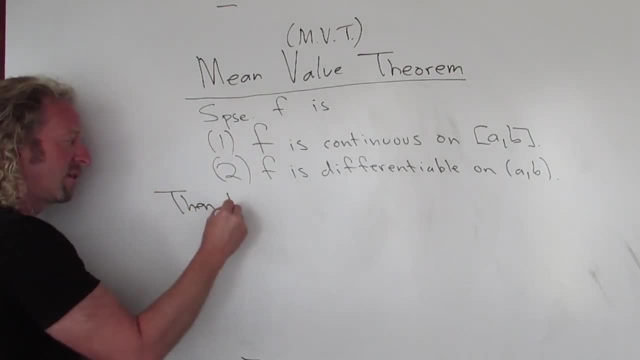 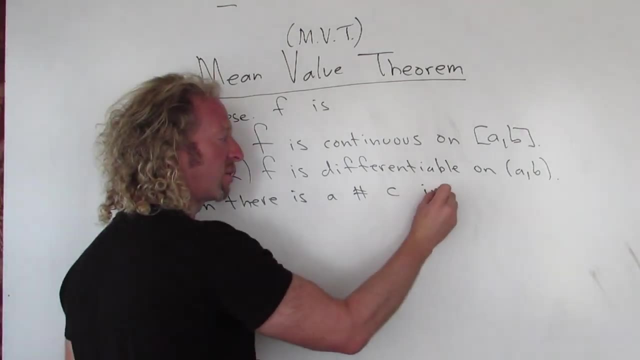 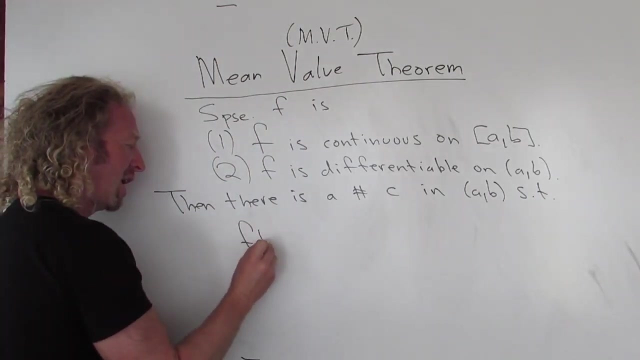 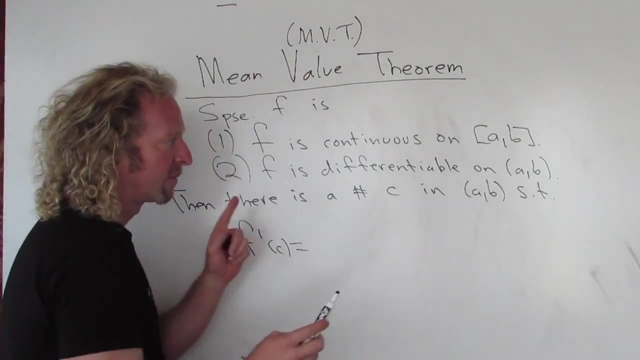 So if these two conditions hold, then there is a number, There is a number, c in the open interval. so just like Rawls', such that the value of the derivative at c is equal to the slope of the secant line connecting two points. 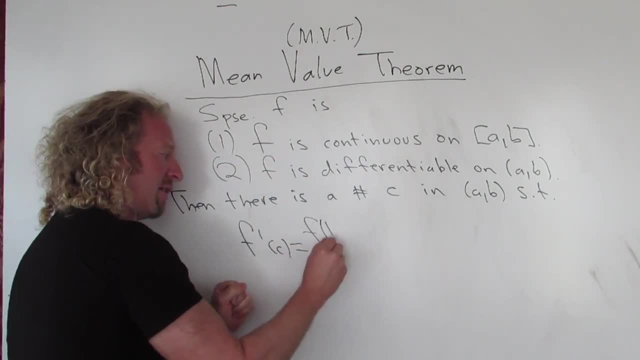 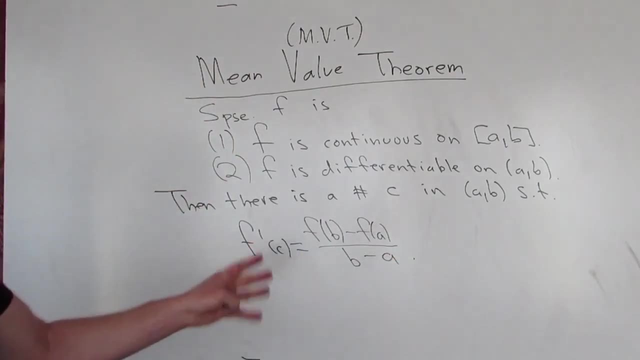 which I'll show you what they are in a minute. So it's f of b minus f of a over b minus a. So we get this. So we get this perhaps peculiar-looking equations, which I'll explain in a minute graphically. 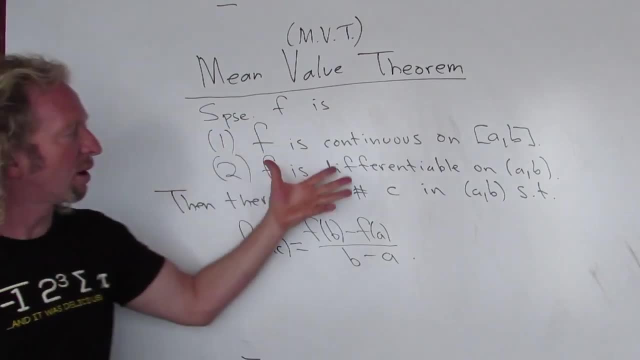 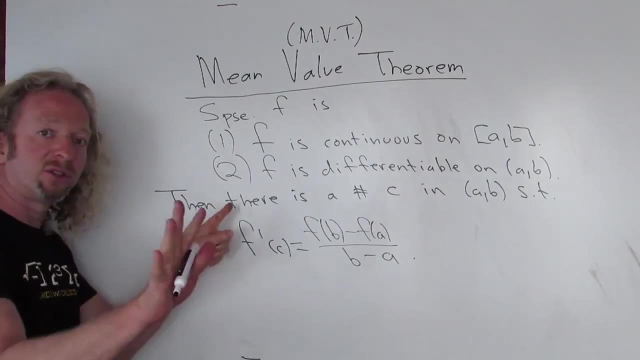 So the mean value theorem, the first two conditions are pretty much identical to Rawls' theorem, But the conclusion is different. right, We're missing the third theorem from Rawls' You'll notice. you'll notice if we had that third condition from Rawls' remember Rawls'. 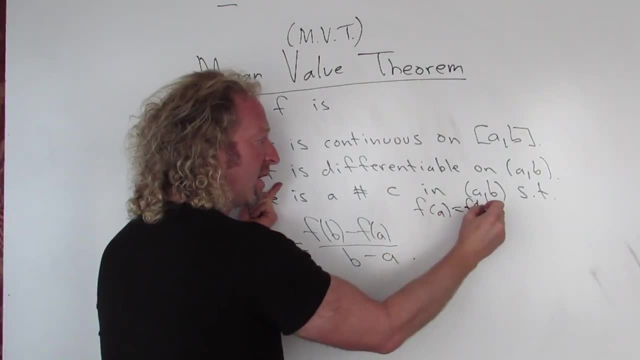 says that f of a is equal to f of b. If that was the case, then you would get: these are the same, so you'd just get zero. So you would end up getting zero here, which is exactly the statement of Rawls' theorem. 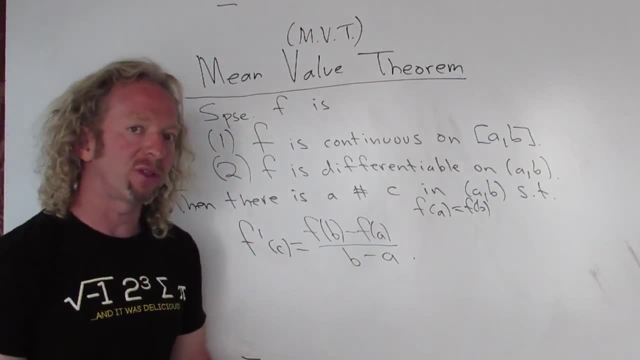 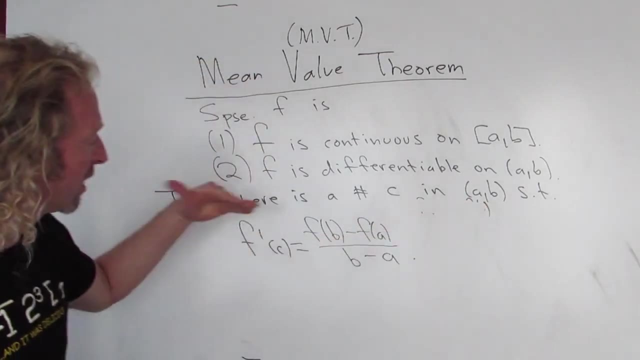 So Rawls' theorem is a special case of the mean value theorem. However, in order to prove the mean value theorem, you have to use Rawls' kind of a random fact over here. Okay, so let's look at a picture so we can explain what's going on here with the mean 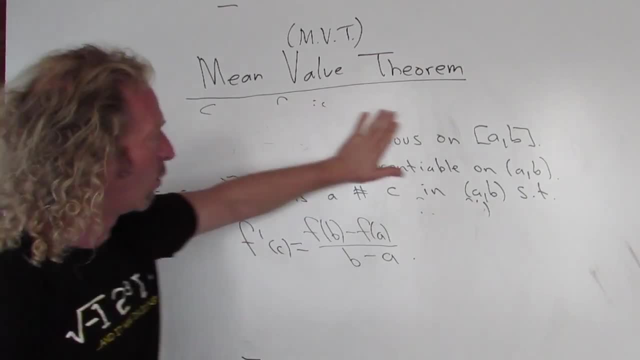 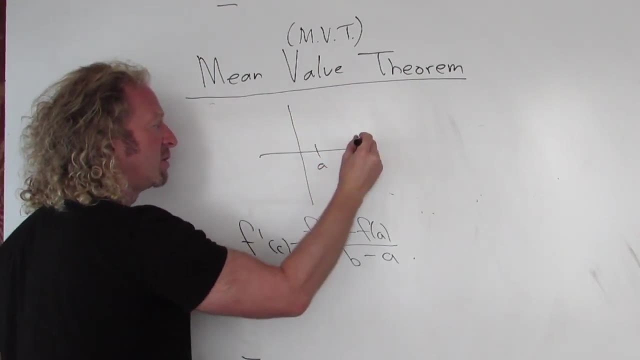 value theorem. I'm going to leave this up so we can see what exactly it means. So here's a picture, So here's a and here's b, okay, And then maybe here's f of a And then f of b. 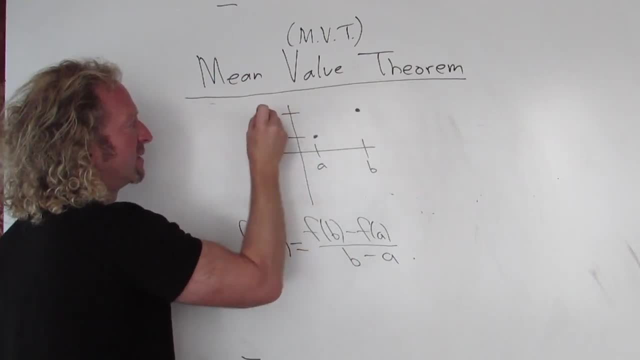 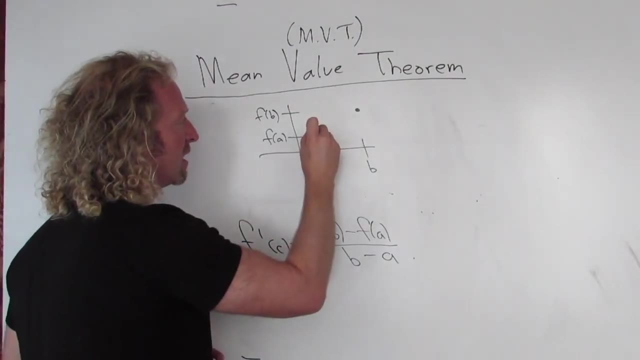 Let's just put it here. Let's put f of b here. This is f of b, All right, so what does the mean value theorem say? Well, the function has to be continuous and differentiable. So to keep it simple, I'll just do this, okay. 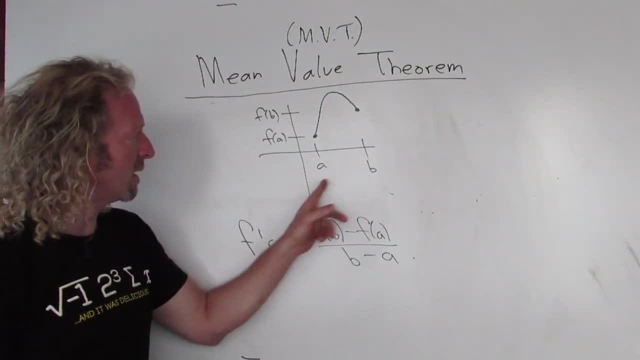 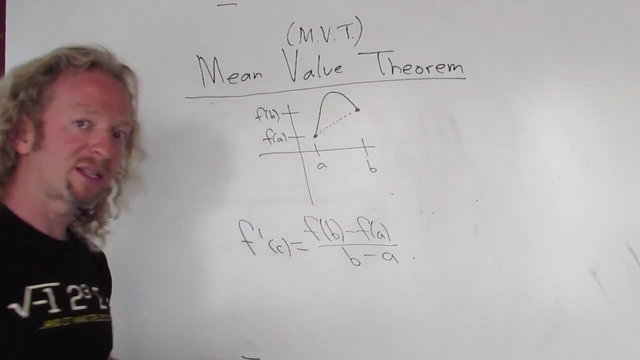 So it's saying: there is a number somewhere between a and b, such that the derivative is equal to this. Well, what is this? Well, if you draw a line here, you get the secant line. Remember, it's called the secant line. 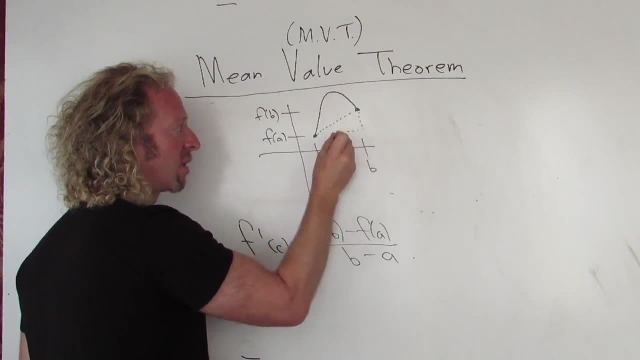 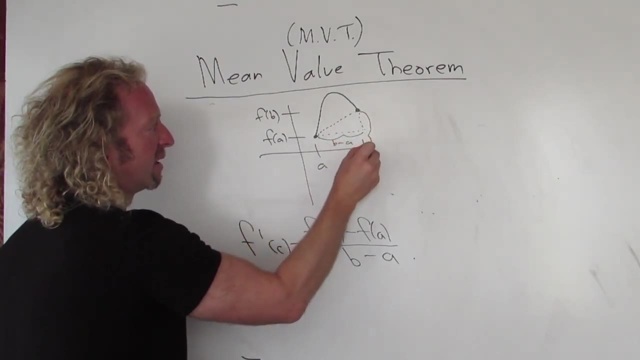 And you can find the slope of this line by drawing a triangle right. This distance here is b minus a. okay, This big distance here is f of b. This little distance here is f of a. So this little distance here is f of a. 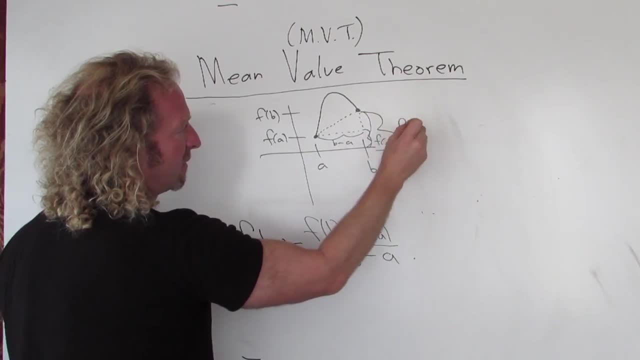 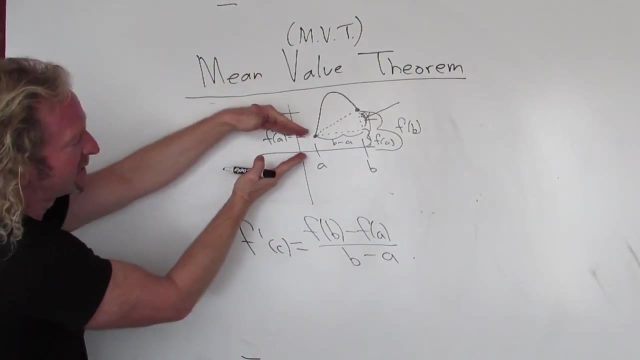 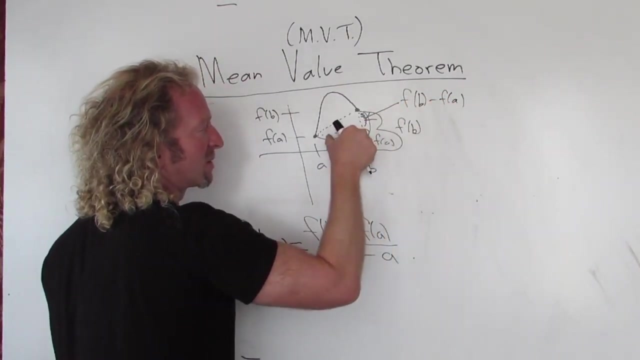 This big distance here is f of b. So this distance here, that's big minus little, f of b minus f of a, f of b minus f of a, So that's f of b minus f of a. So that's the rise and that's the run. 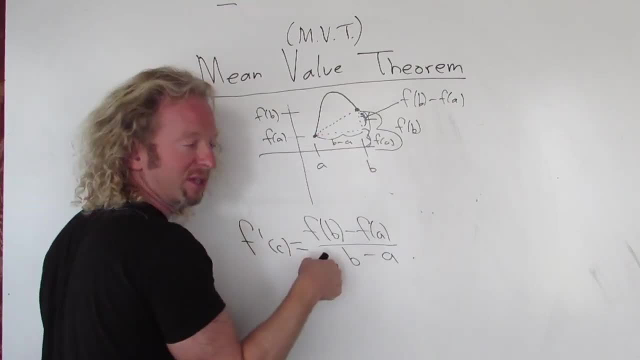 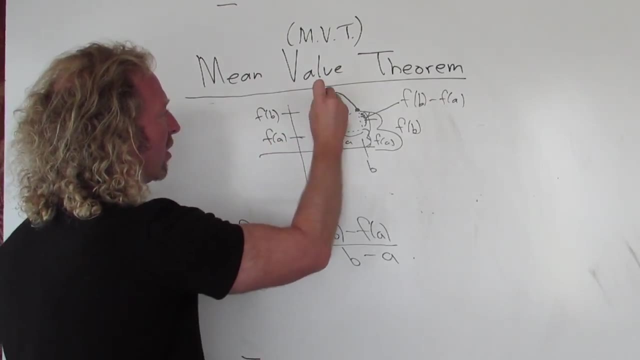 So the slope of this line, the slope of this line, is equal to this. So what it's saying is that there is a number c in the open interval where the slope of the secant line is equal to the slope of the tangent line or the slope of the tangent. 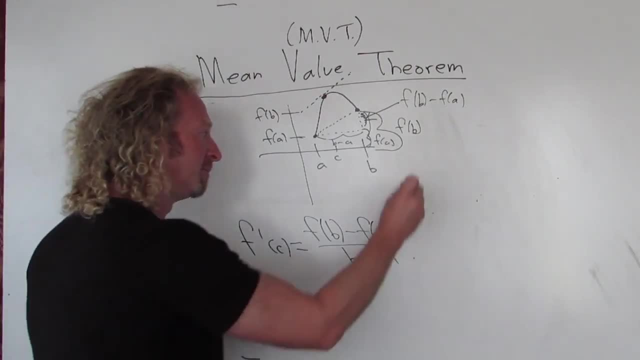 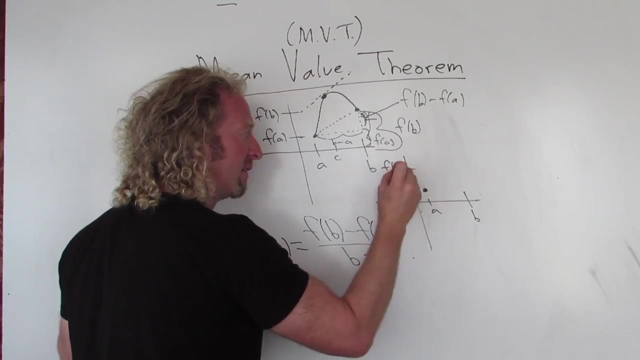 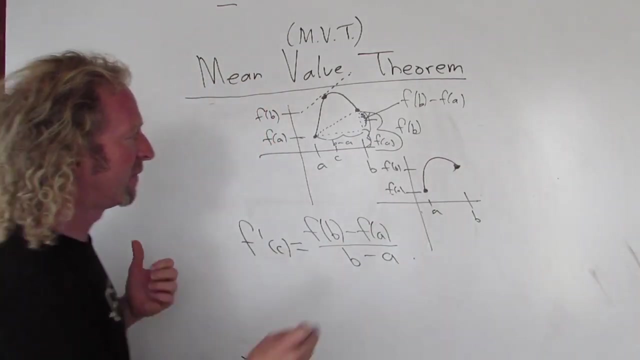 line is equal to the slope of the secant line. So again, given a and given b, and then say this is f of b and this is f of a. I'm going to draw it one more time. Given any two points like this, if you connect the secant line, what this says is that there 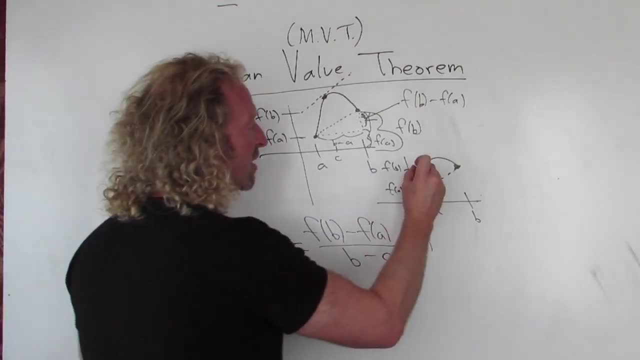 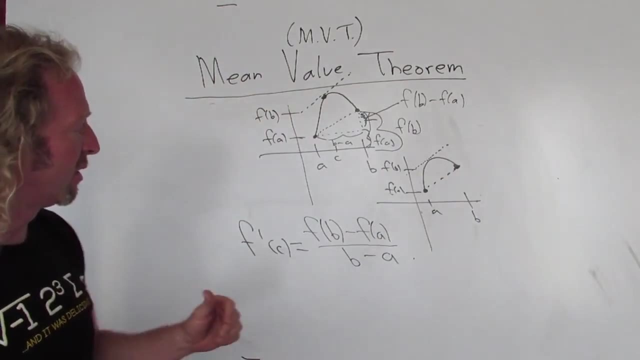 is a point c, a number c, between a and b, such that the tangent line at that number is parallel to the secant line right. In other words, the slope of the tangent line is equal to the slope of the secant line. 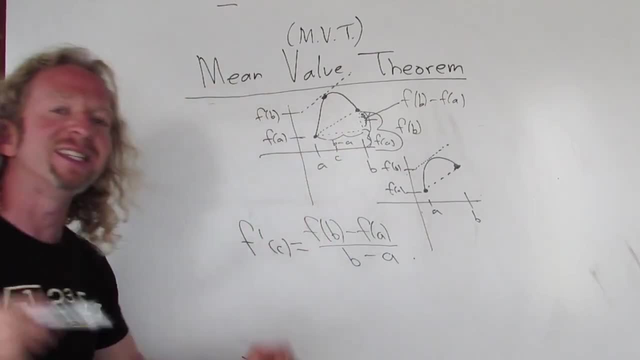 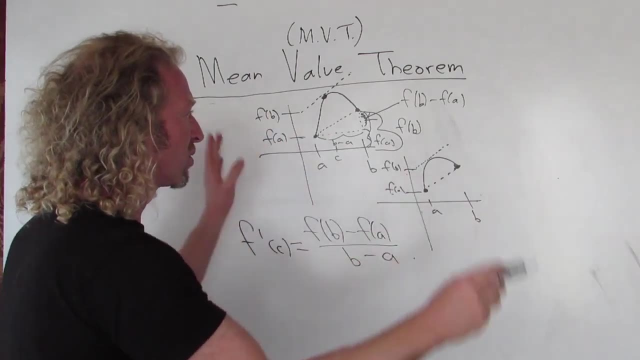 Another way to think about it. The slope of the secant line is the average rate of change. The derivative is the instantaneous rate of change. So somewhere in the open interval the average rate of change is equal to the instantaneous rate of change. 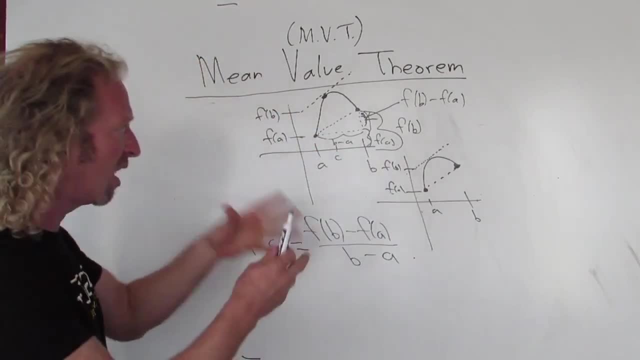 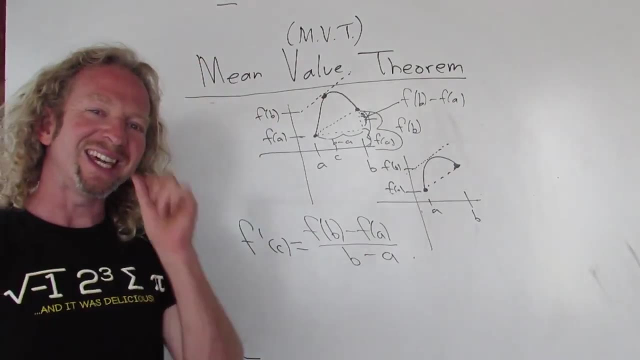 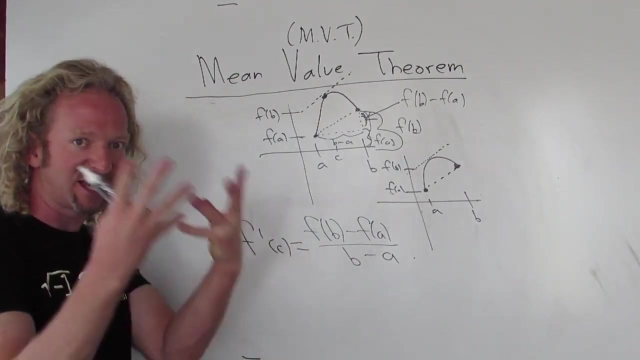 So, given a continuous function that's differentiable on an interval, a, b, continuous in the closed differentiable on the open interval, there is a number somewhere in the interval where the instantaneous rate of change is equal to the average rate of change. If you're thinking of velocity, the average velocity is equal to the instantaneous velocity. 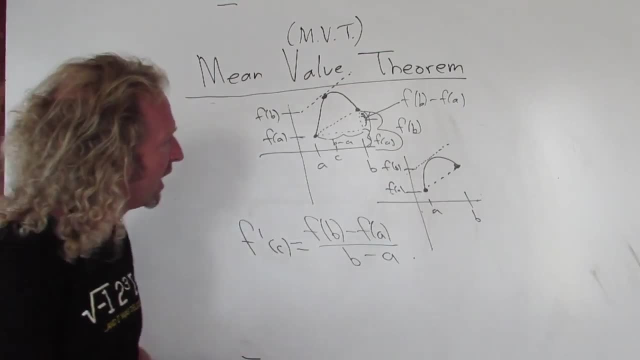 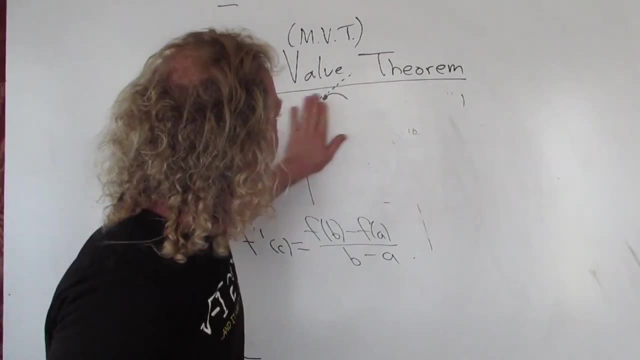 at some point in that interval. Okay, let's go ahead and do an actual problem where we find c. I'll just make one up and we'll do it. Let's do it. So just making it up, let's be bold. 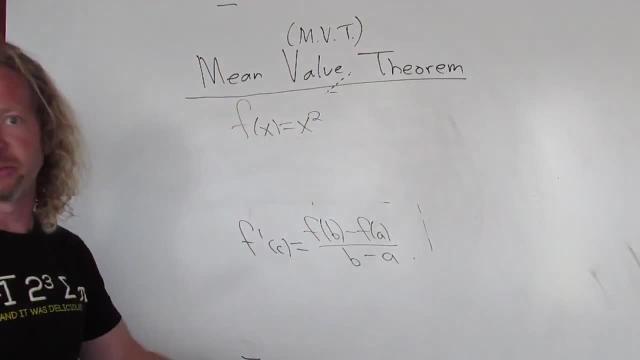 f of x, is x squared. Let's make up a nice interval. How about 0, 1?? And let's find c. We should be able to find c right. This is a polynomial, so it's continuous and differentiable everywhere. 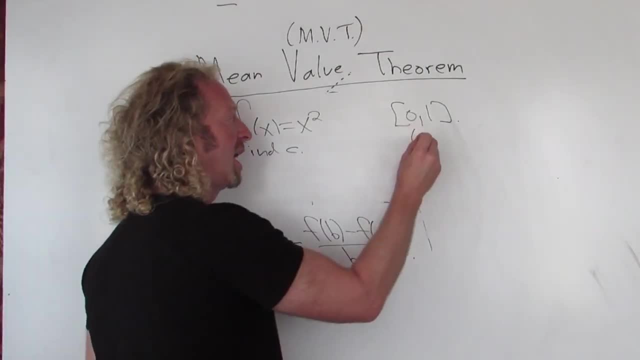 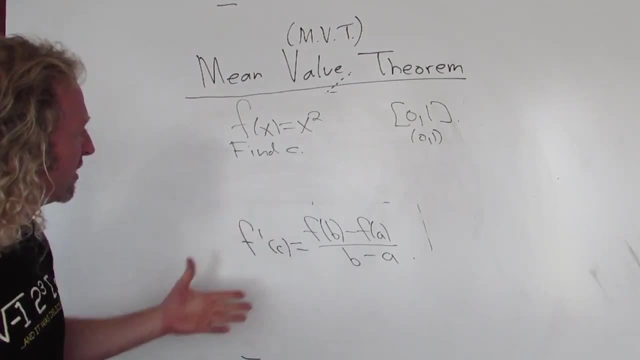 In particular, it's continuous on this closed interval and it's differentiable on this open interval. Therefore it satisfies all the criteria of the mean value theorem. So to find c, all we have to do is use this equation, right? So we take the derivative. 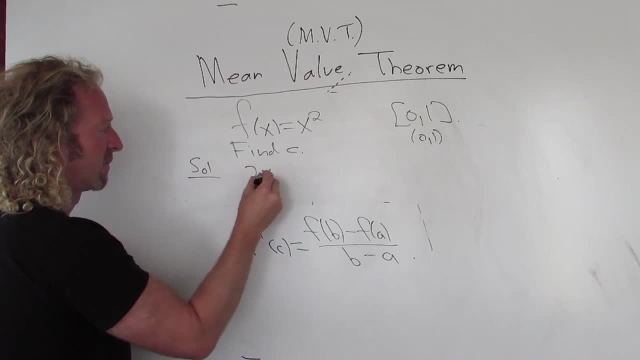 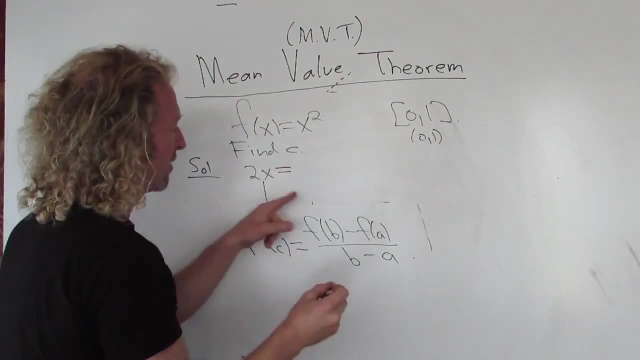 The derivative is 2x, So 2x, that's what's going to go here. Here there's a c. I'm using an x instead. right? The derivative of x squared is 2x, And we set it equal to f of b minus f of a. 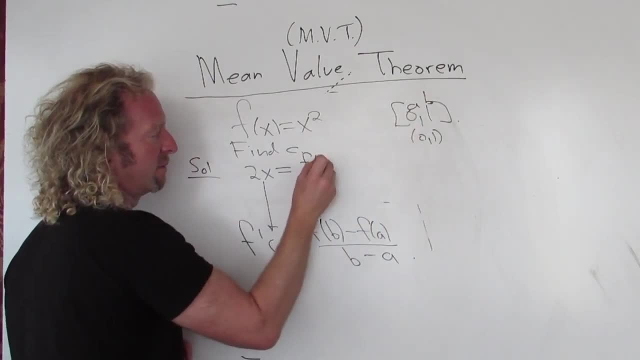 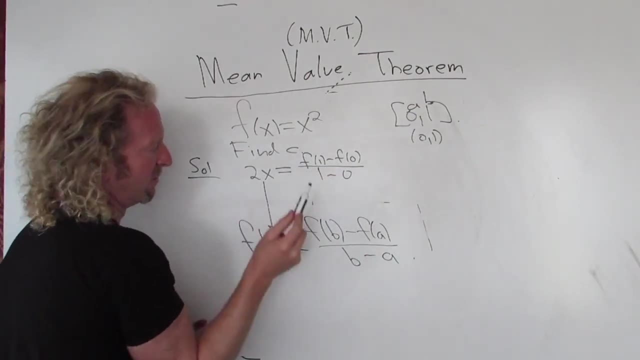 So this is your a, This is your b, So it'll be f of 1 minus f of 0 over b minus a, So 1 minus 0.. You can think of this as 2c- Same thing. You can just call it x. 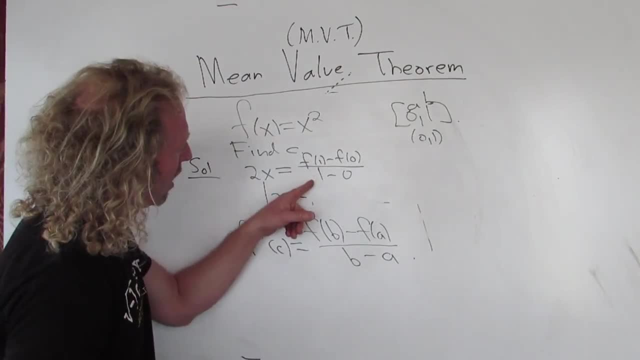 It doesn't really matter. So 2x equals. let's see: f of 1 is 1, right 1 squared is 1.. f of 0 is 0. You get 1 minus 0. So 1 over 1 is 1.. 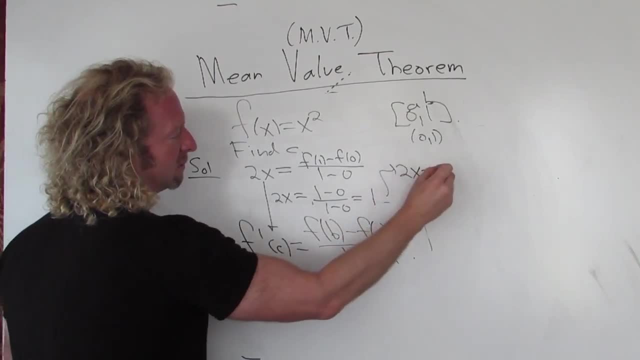 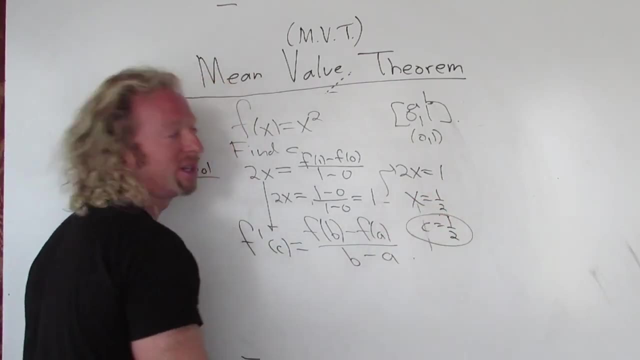 So we get 2x equals 1. It's really easy. This is divided by 2. And so you get x equals 1 half. So that's your c. That was a pretty easy example. It was a good example because it was easy. 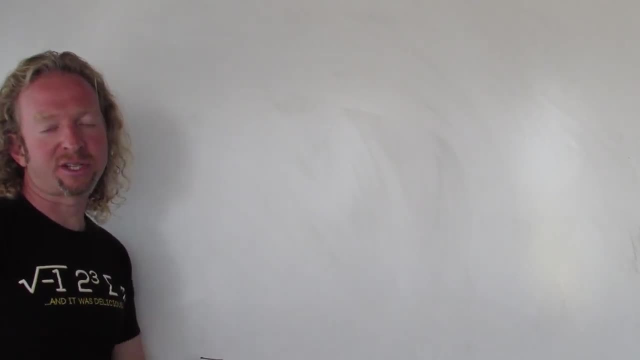 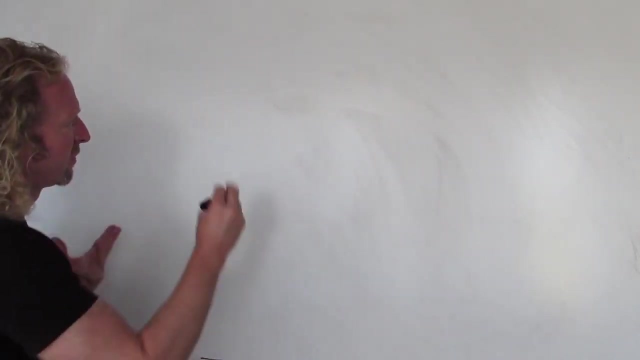 Hey YouTube. In this video we're going to talk about increasing and decreasing functions and how we can use calculus to identify where a function is increasing and where a function is decreasing. Let's just do it from an intuitive approach. So here's a function. 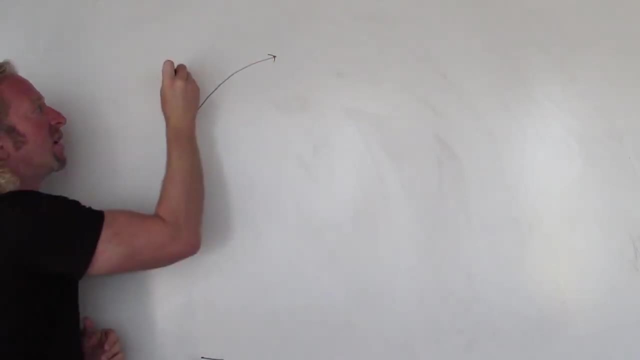 And it's increasing, obviously right. So this is an example of a function that is increasing, OK, So, if you look at the derivative of this function, so what is the derivative? Well, the derivative is the slope of the tangent line. 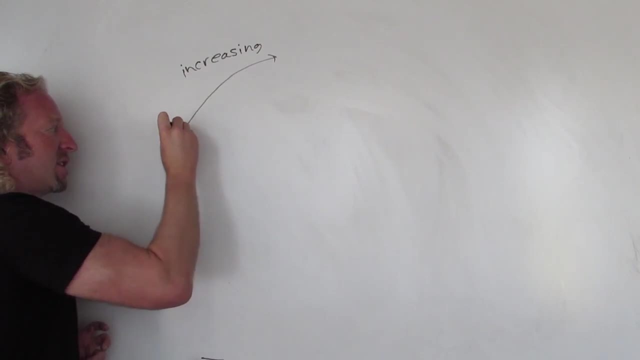 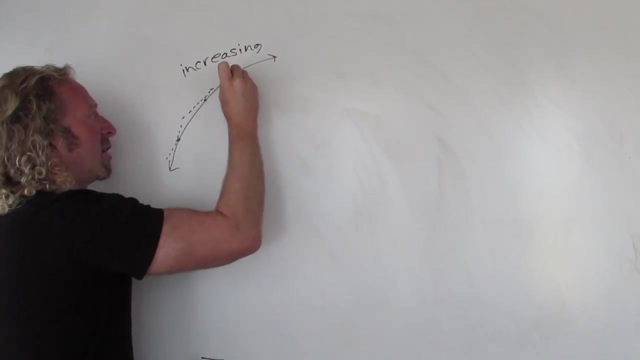 So you pick any point on this graph and look at the slope of the tangent line. That's what the tangent line looks like. That tangent line has a positive slope. Pick another point: You have a positive slope. Pick another point: You have a positive slope. 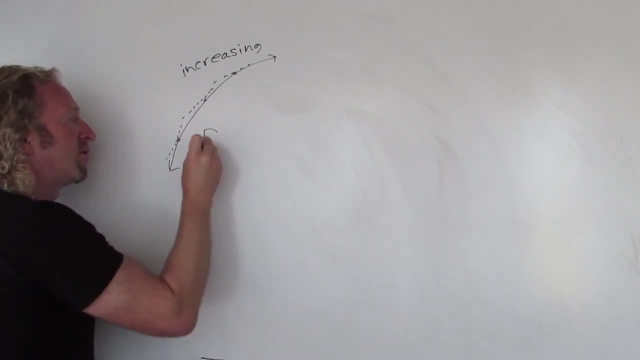 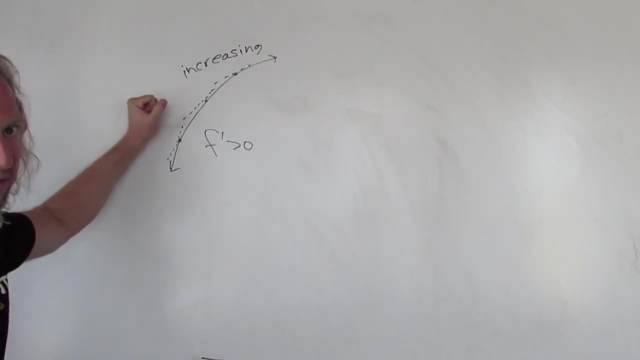 So it looks like that whenever a function is increasing, the first derivative is positive, because the first derivative is the slope of the tangent line. So positive first derivative increasing function. Positive first derivative increasing function. This has to be true on an interval. 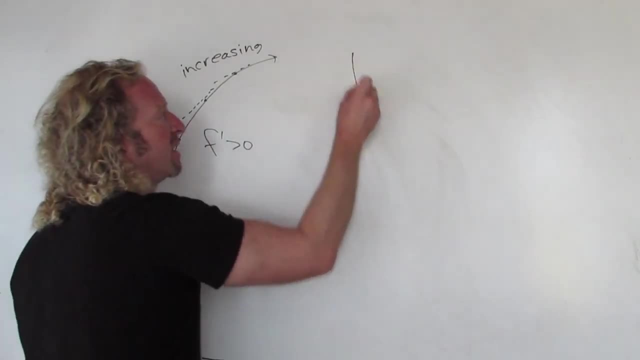 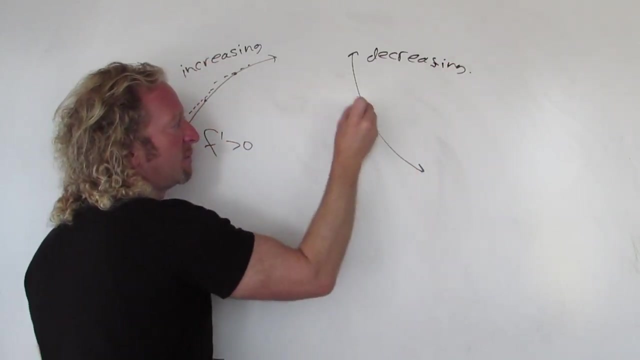 This has to be true on an interval, by the way. OK, If you have a decreasing function, it looks like this: Decreasing. In this case, if you pick a tangent line at any point on this graph, you'll see the tangent. 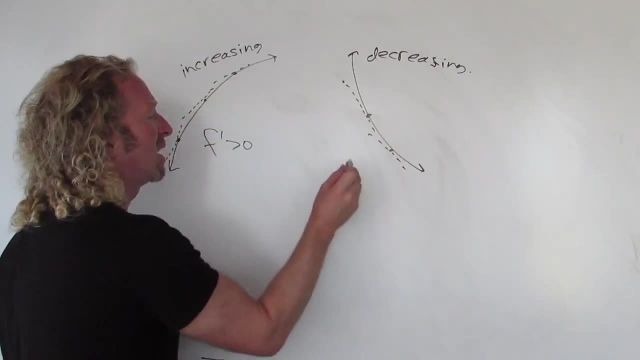 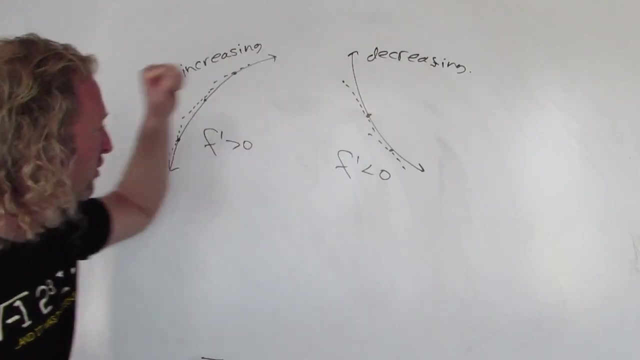 line has a negative slope, Well the derivative is the slope of the tangent line. So in this case the first derivative is negative. So if you have a negative first derivative on an interval, their function is decreasing. So positive, increasing, negative, decreasing. 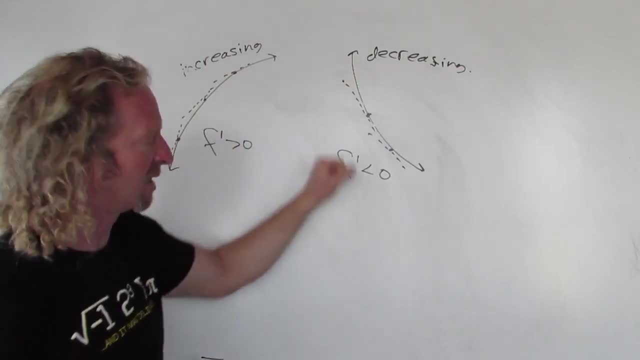 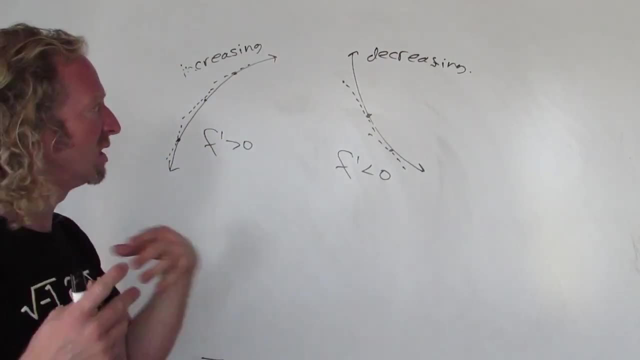 Positive: increasing, negative decreasing. Positive: increasing, negative decreasing- Really easy to memorize. Let's do a really simple example of finding intervals where a function is increasing and or decreasing. So let's do a simple problem. Let's try this one. 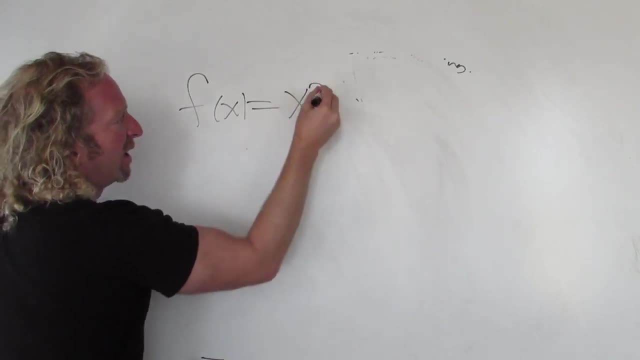 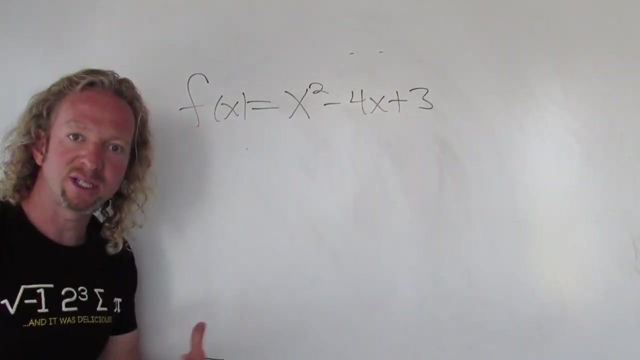 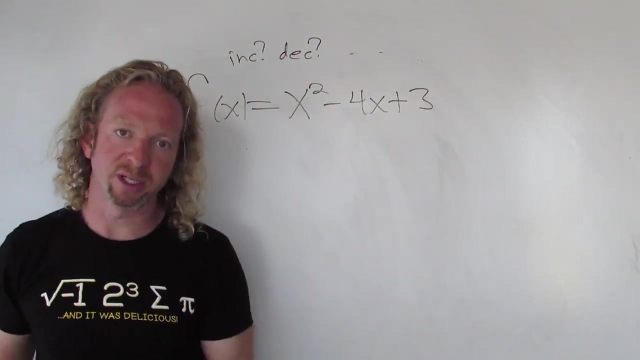 f of x. Let's make one up: x squared minus 4x plus 3.. So we're looking for where the function is increasing and decreasing. So what intervals can we find where this function is increasing and decreasing? So to find out where a function is increasing or decreasing, the first thing you do the 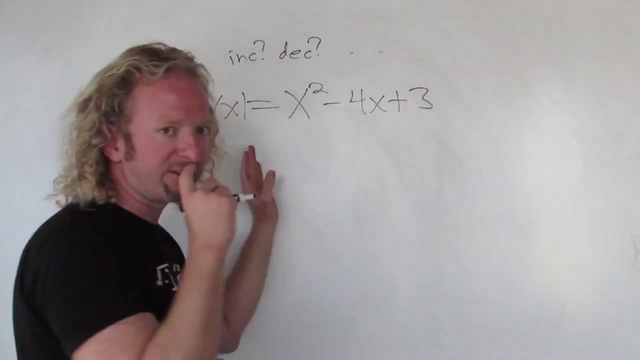 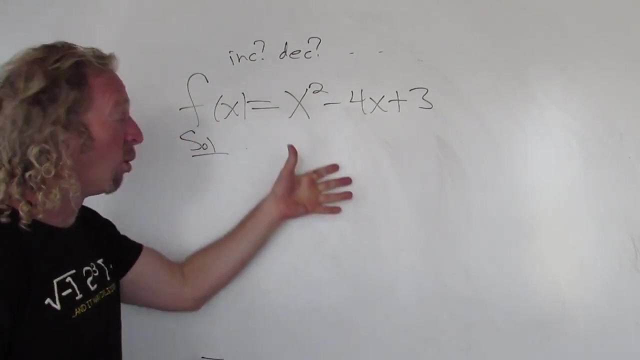 very first step is you take the derivative and you set it equal to 0. And you're basically looking for critical numbers or places where the derivative is undefined that aren't critical numbers. So, even like vertical asymptotes, You'll want to care about those as well. 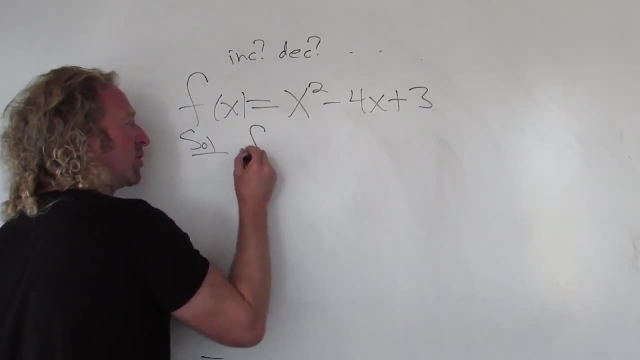 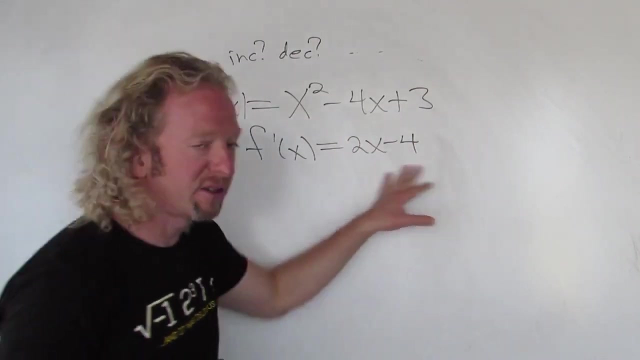 So critical numbers and any vertical asymptotes. So you take the derivative: In this case it's 2x minus 4.. So this is not undefined. There's no vertical asymptotes And you're not going to get any critical numbers from the derivative being undefined. 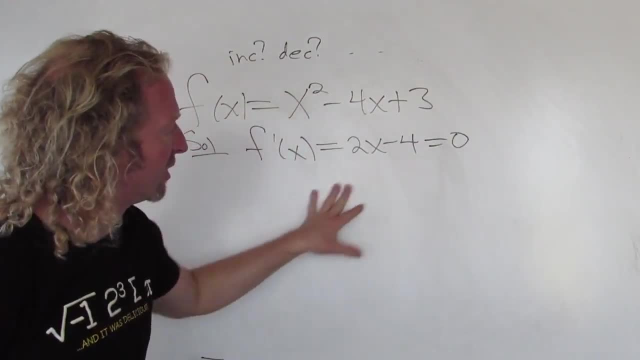 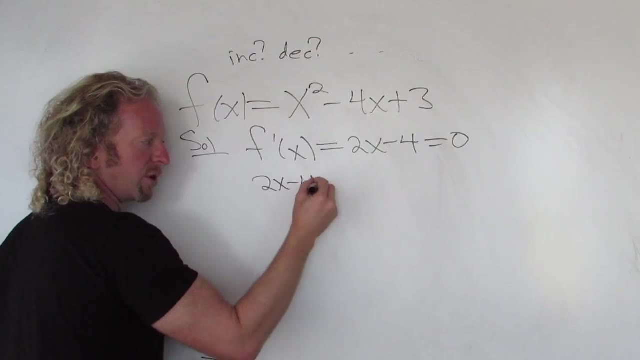 But you can set it equal to 0 to find critical numbers. So you get here. Now you can solve this for x, So I'm going to do it again over here. So 2x minus 4 equals 0. You can add 4.. 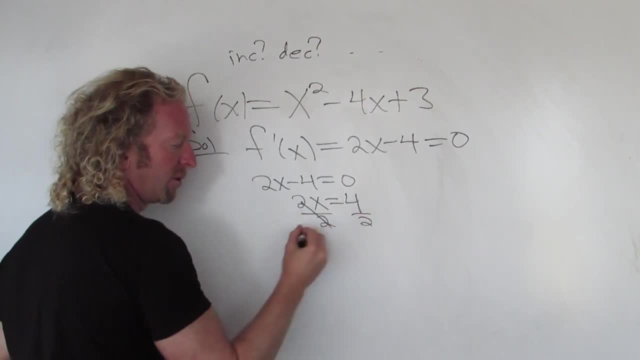 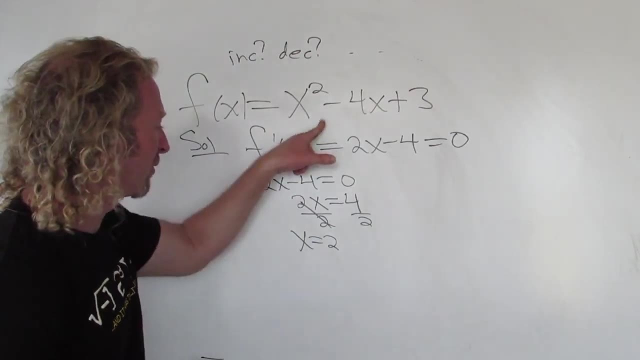 Then you would divide by x, Then you would divide by 2.. So x equals 2.. So this is actually a critical number. in this case, This is actually a critical number because it's in the domain of the original function, So we care about this. 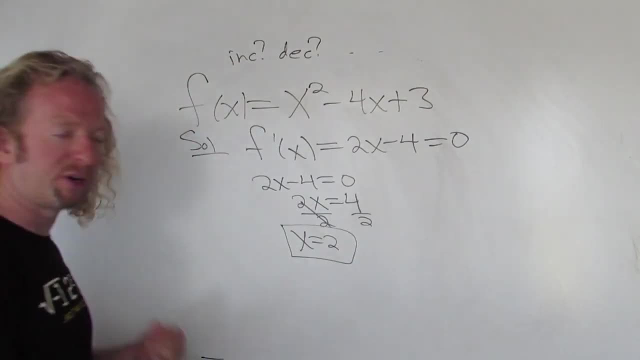 I'm going to put it in the box. So you take this number And now what you do is you put it on a graph. So again, step one: take the derivative. You look to see if it's undefined anywhere, even if it's a vertical asymptote. 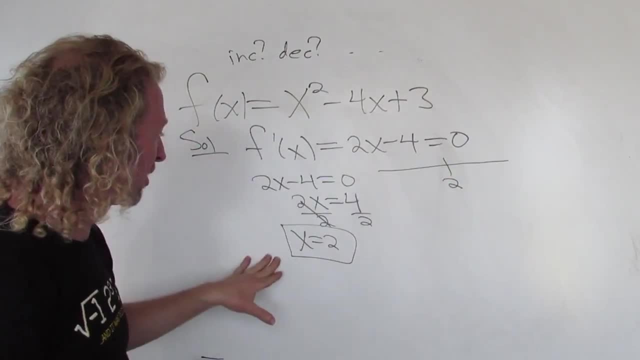 You care about that, You make note of it, Then you set it equal to 0. And then you solve. So that's what we have. So this is a point of interest, right? This is a point we care about. Plot it on a number line. 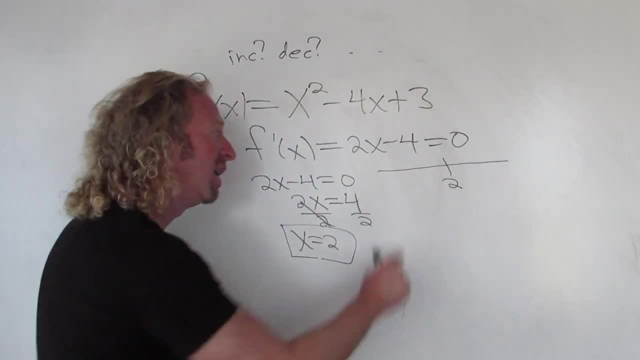 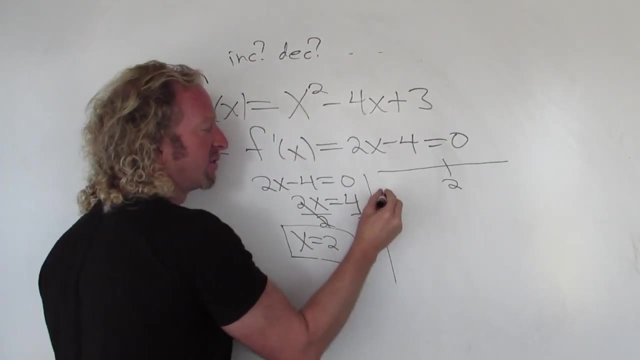 Now what you do is you pick test points. You can pick any number you want, that's less than 2.. The easiest number in the world is 0. So let's use 0.. And you plug it into the first derivative. So f prime of 0. 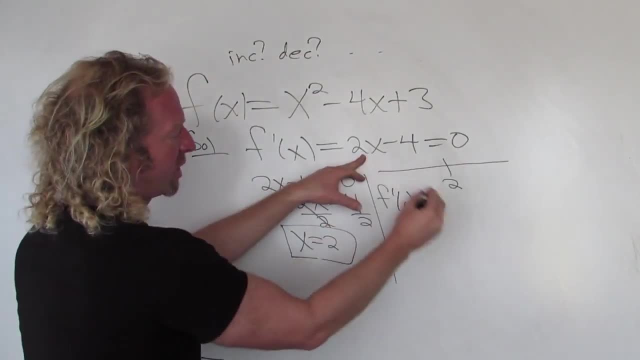 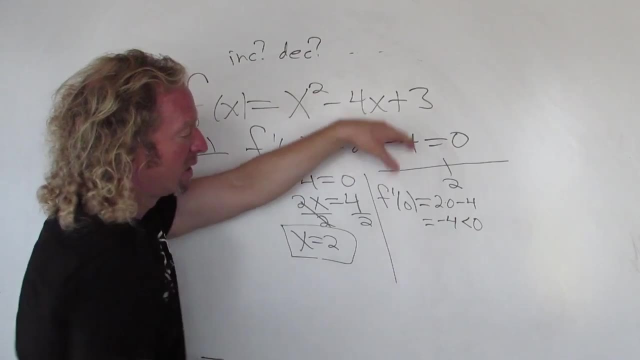 So plugging it into the first derivative, you would get 2 times 0 minus 4.. So you get minus 4.. So that's less than 0. So we have a negative first derivative. So in this case the function is going to be decreasing here. 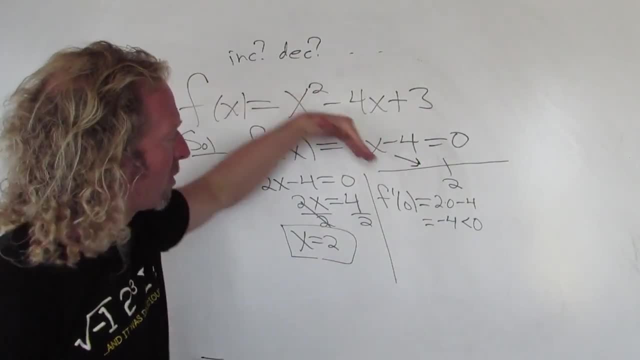 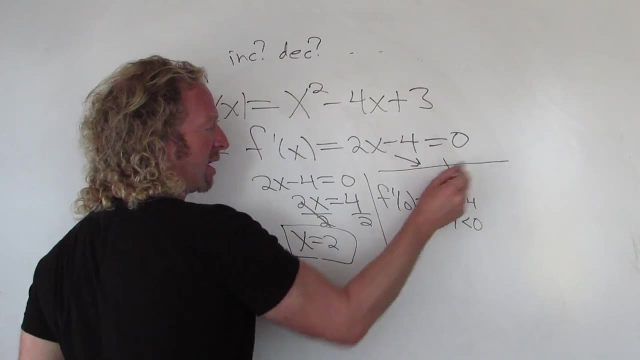 I like to draw a little arrow: right, It's going down. I always draw arrows going that way, right. So down, up, down, up, right, Down, up, down, going that way. Now we pick another number over here. 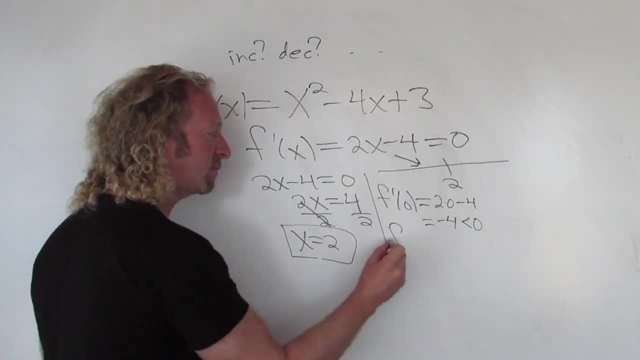 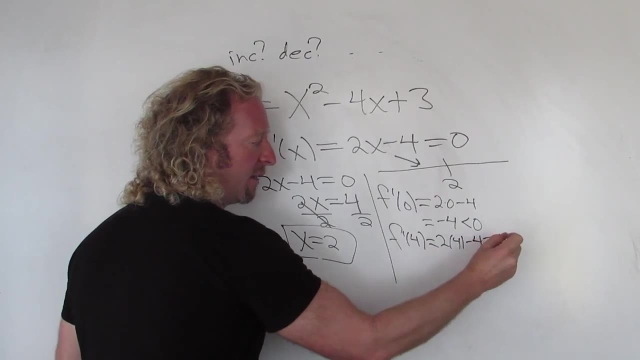 Anything bigger than 2.. How about 4?? So plugging in 4, we get 2 times 4 minus 4.. So 8 minus 4, that's equal to 4.. That's positive. When you have a positive first derivative, it means the function is increasing. 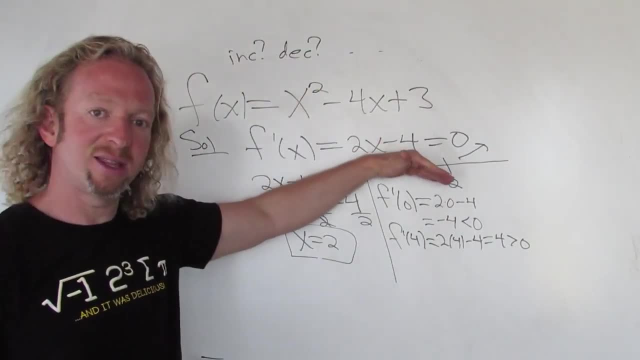 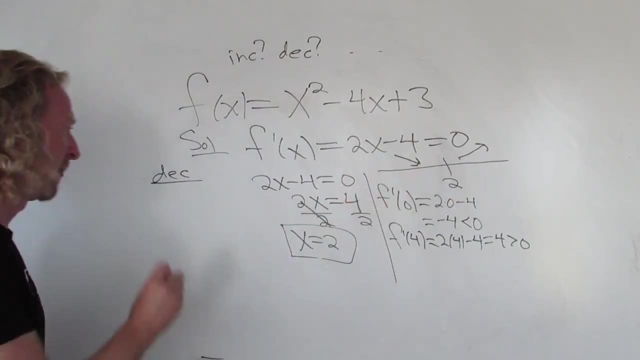 So it's decreasing all the way until it gets to 2. And then it starts increasing. So it looks like it's going to be decreasing And you can get the answer from the picture. Negative infinity to 2 is always a parentheses. 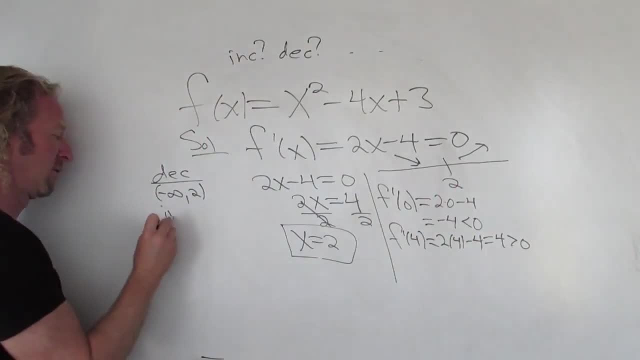 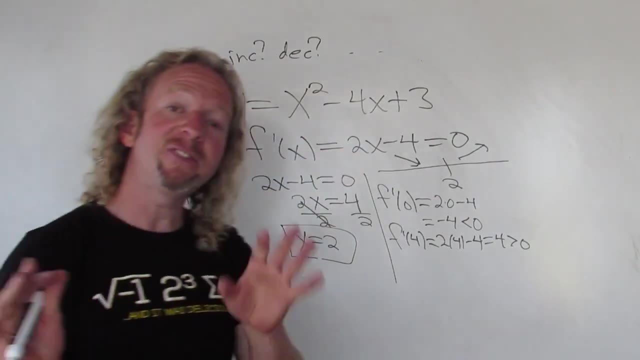 And then increasing would be 2 to infinity. So increasing would be 2 to infinity. So step 1, when you're finding increasing and decreasing is, take the derivative. Look to see if it's undefined, right Anywhere. If it's undefined, make a note of it. 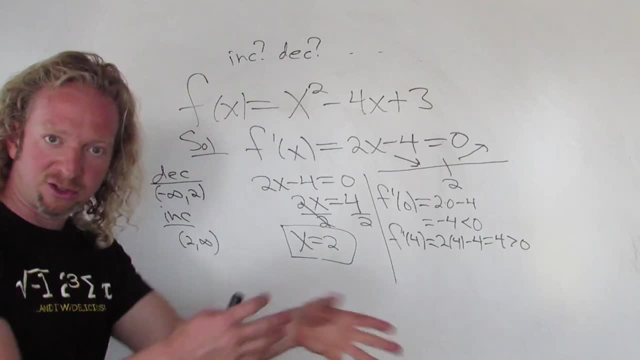 Then you set it equal to 0 and you solve. Then you take all of the answers that you just got from that process and you put them on a number line. Then you pick test points. You can use any number you want over here, any number you want over here. 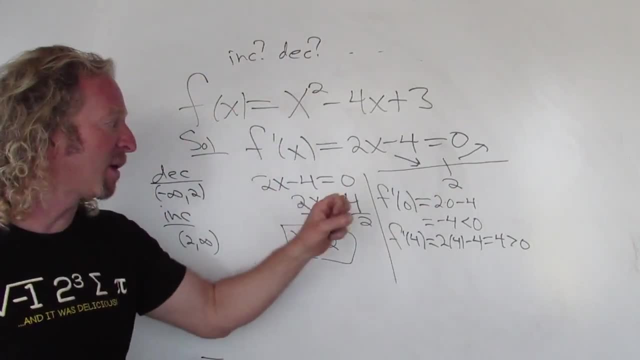 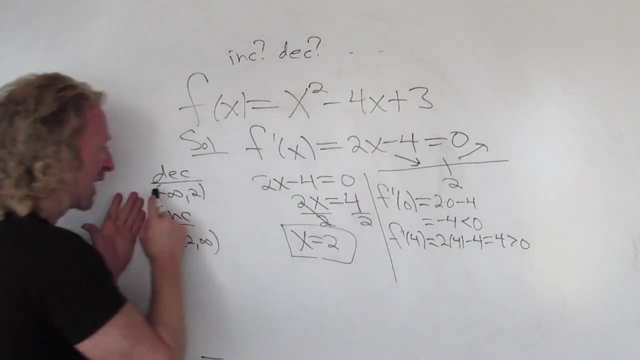 Plug them into the first derivative. Super important, right? If it's positive, the function is increasing there. If it's negative, the function is decreasing there. Then you can get your answer from the picture, right? So decreasing from negative infinity to 2, increasing from 2 to infinity. 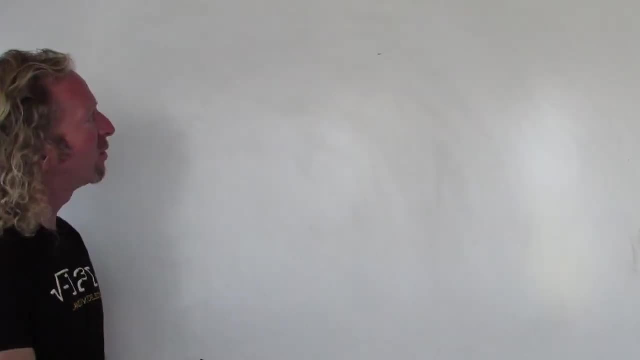 So I hope that made sense. That's it. In this video we're going to look at something called the first derivative test. Let's just do an example and I'll explain it through a very, very simple example. So a really easy problem. just to explain the concept. 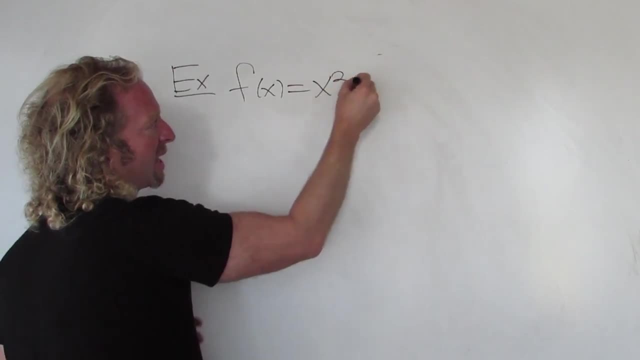 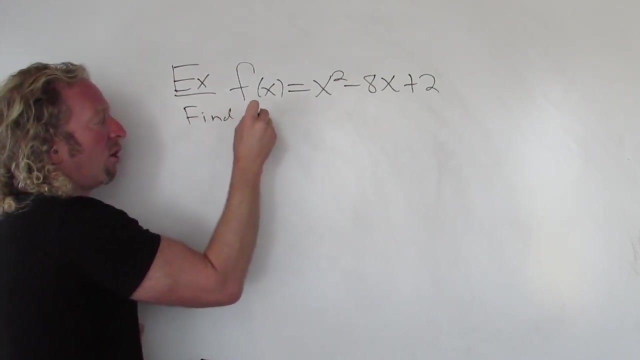 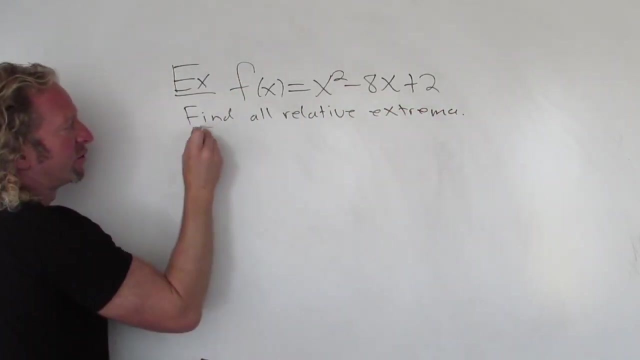 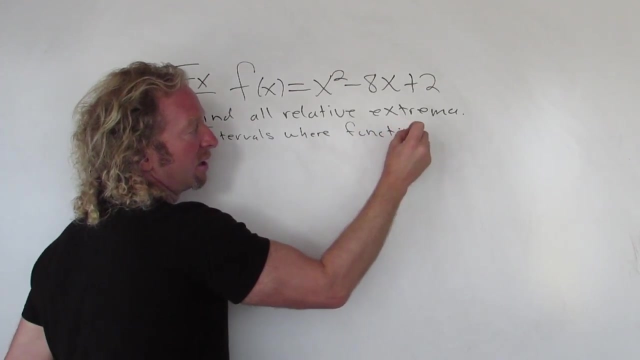 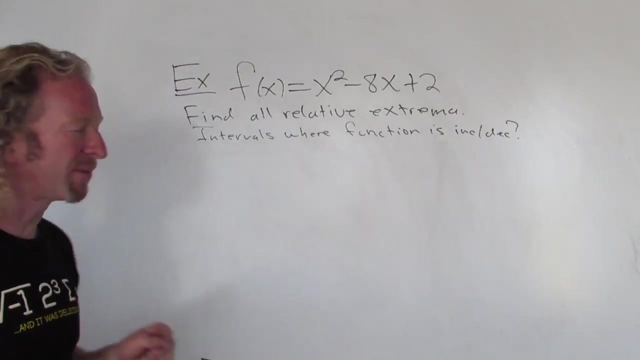 So we have a function f of x equals x squared minus 8x plus 2.. And the question is to find all relative extrema and also find the intervals Where the function is increasing, slash, decreasing, Increasing or decreasing or both. So to find each extrema we're going to use something called the first derivative test. 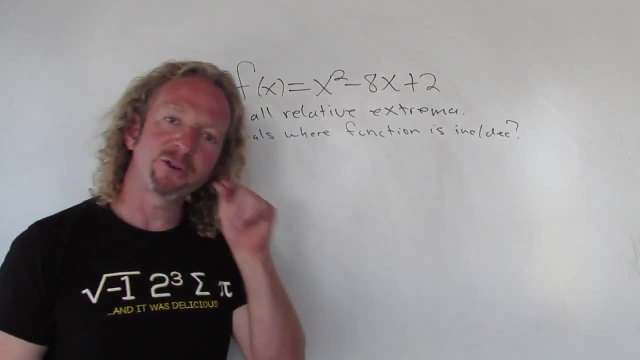 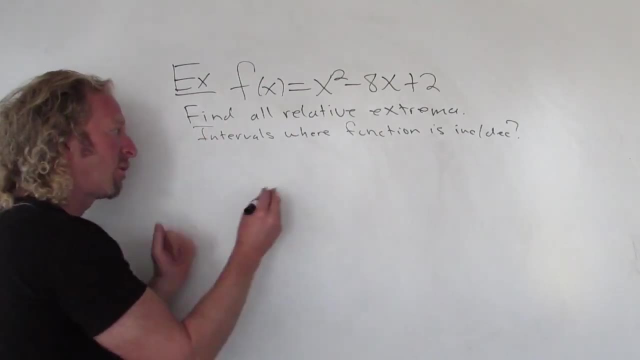 So the first derivative test basically says the following: If your first derivative changes sign at a critical number, you're going to have a relative maximum or a relative minimum. So for example, even before we do the problem, say we have critical numbers of 2 and 4 and 6.. 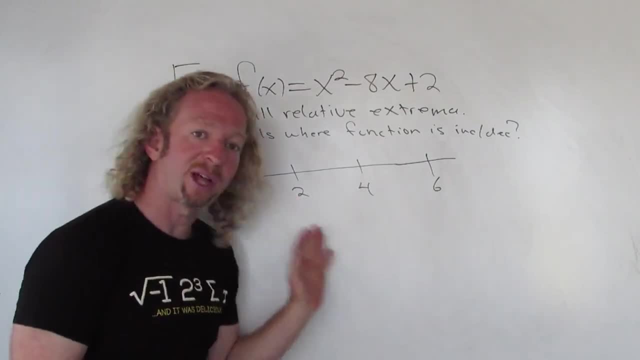 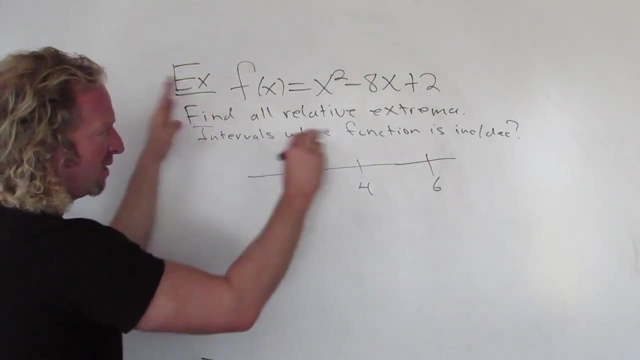 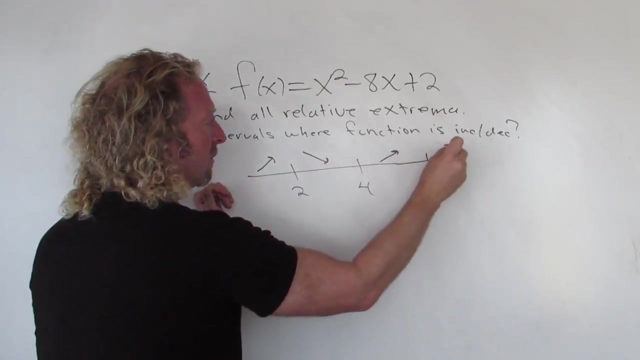 These are all critical numbers, So they're not vertical asymptotes or anything. They're critical numbers. So these are numbers in the domain of the function where the derivative is 0 or undefined. And say, you draw your little sign diagram for your increasing decreasing and it looks like this: 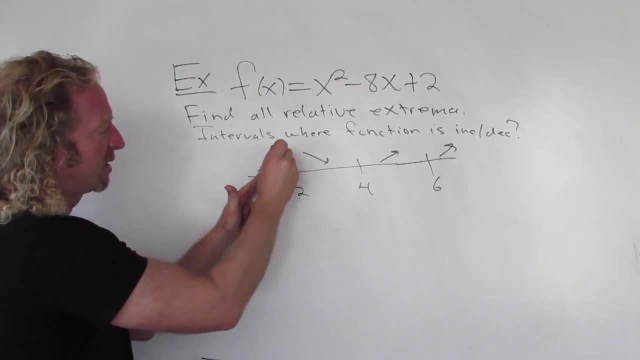 So that means the function here would be increasing, increasing, increasing, increasing, increasing, and then all of a sudden starts decreasing, Decreasing, decreasing, increasing, increasing, and it increases forever. So here you have a little hump. 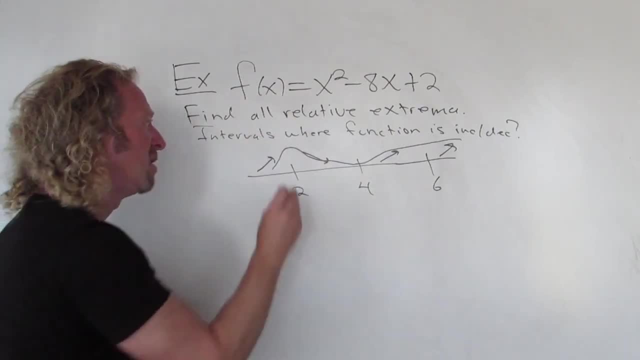 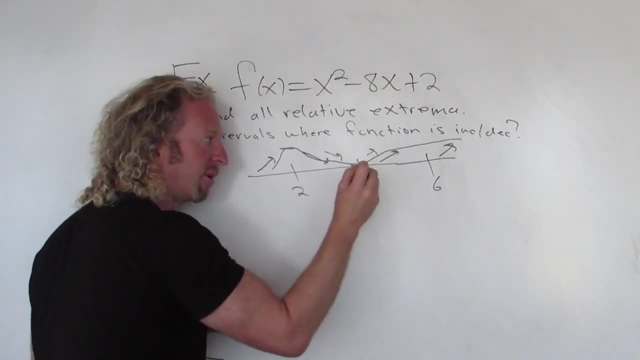 It goes from increasing to decreasing, Increasing to decreasing, Increasing to decreasing. You have a relative maximum at 2.. Here it goes from decreasing to increasing, So you have a relative minimum at 4.. And then here it keeps going, so you have nothing interesting going on at 6.. 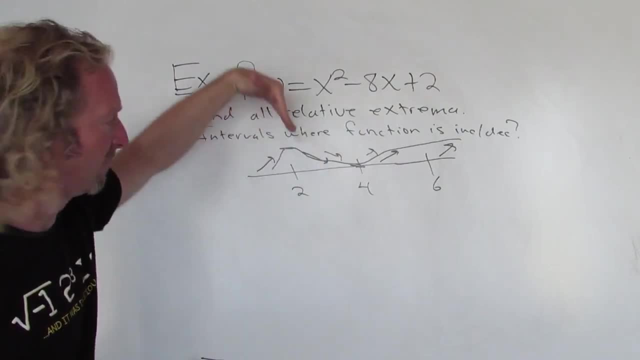 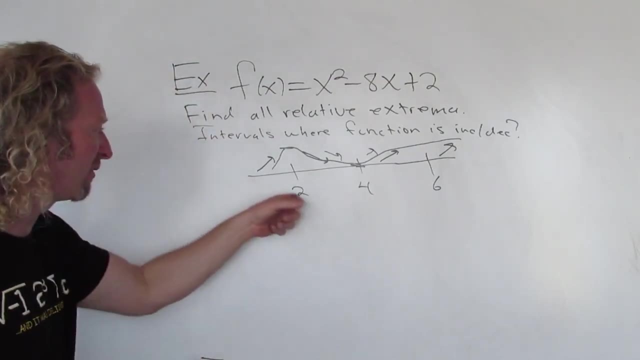 So if you have a hump like that, that means you have a max. If you have a dip like that, that means you have a min. That's called the first derivative test. But that has to happen at a critical number. So if this happens at a vertical asymptote, game over. 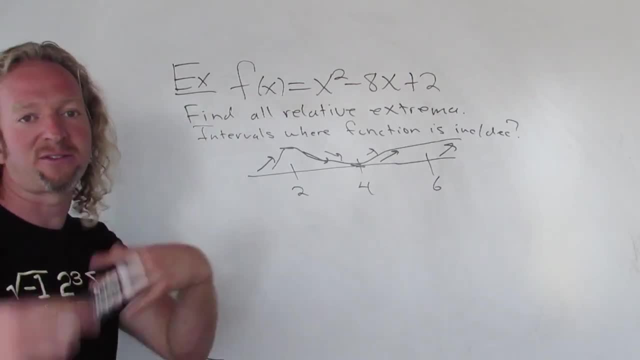 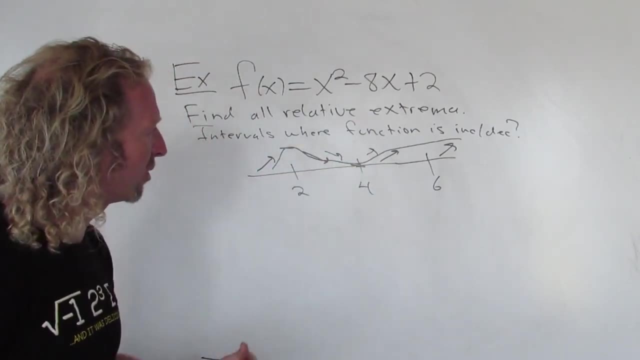 It's not a max or a min, And if you think it is and you actually try to find it, it won't work Because your function will be undefined there, So it takes care of itself. So if the derivative changes sign at a critical number, you'll have a relative max or a min. 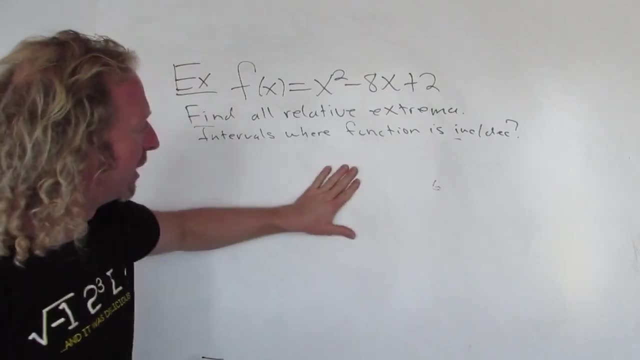 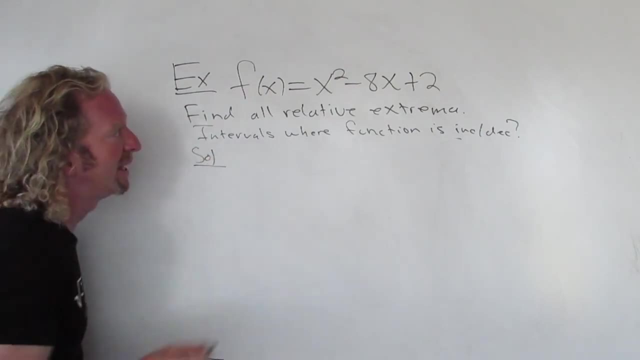 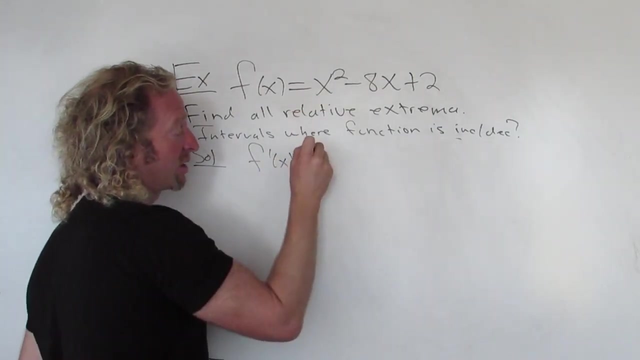 So let's go ahead and do some problems. So let's do this one. We'll start by taking the derivative. So the derivative here of x squared is 2x, The derivative here is minus 8.. So whenever you're doing these problems, the first step is to take the derivative and you ask yourself: 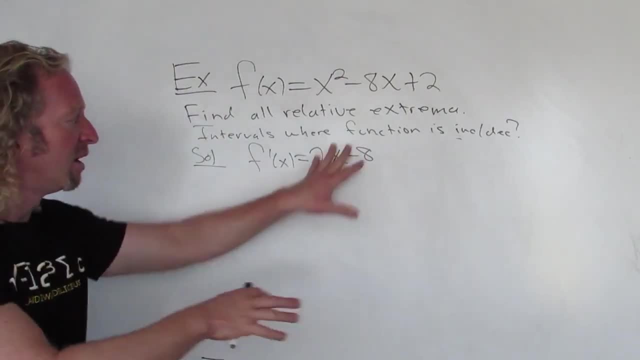 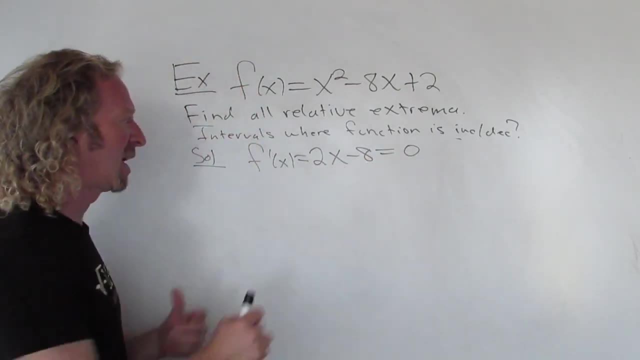 is it undefined anywhere? Are there any vertical asymptotes? Well, this is not undefined anywhere. so life is good, So we're good. Then you set it equal to 0.. I'm going to write it again. I don't like messing with my derivative. 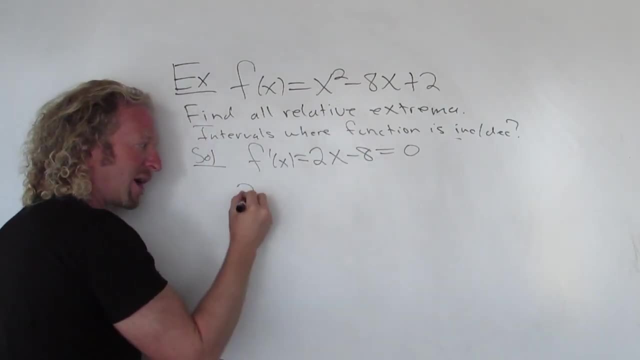 We're going to use this for test points later, So I always rewrite it again down here when I'm solving for x. I don't want to do like plus 8, plus 8.. I don't want to like taint it. 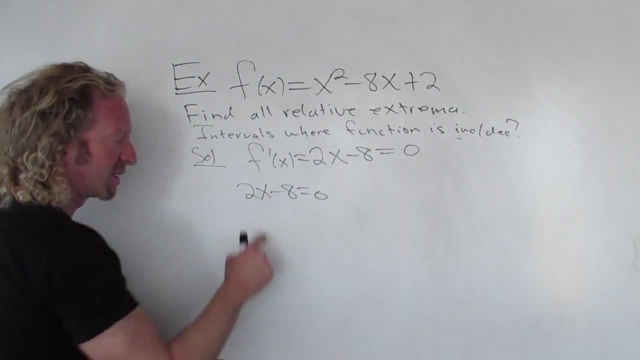 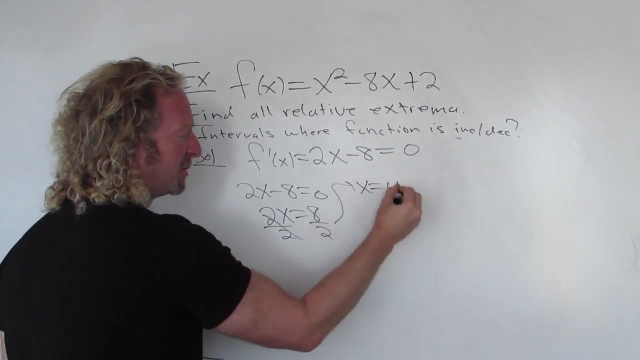 Because we're going to use it later to plug in test points. So you solve this for x, So you add 8. Divide by 2. So you end up with x equals 4.. This is a point of interest. It also happens to be a critical number, right. 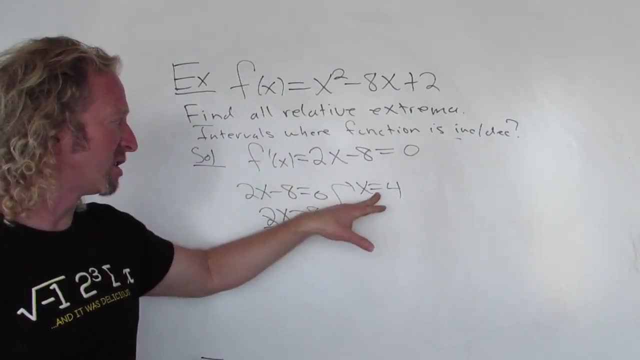 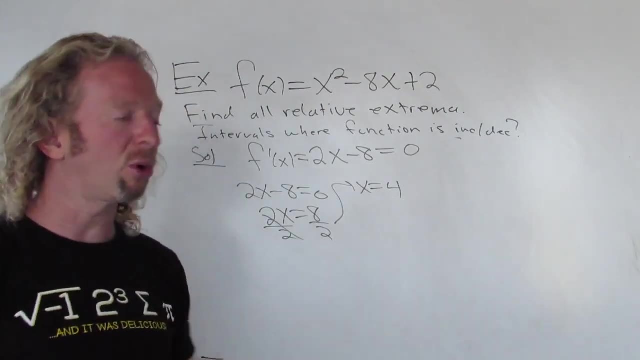 This number is in the domain of the original function and it is a number where the first derivative is 0. Therefore, it is a critical number. Remember, critical numbers are numbers in the domain of the function, where the derivative is 0 or where it's undefined. 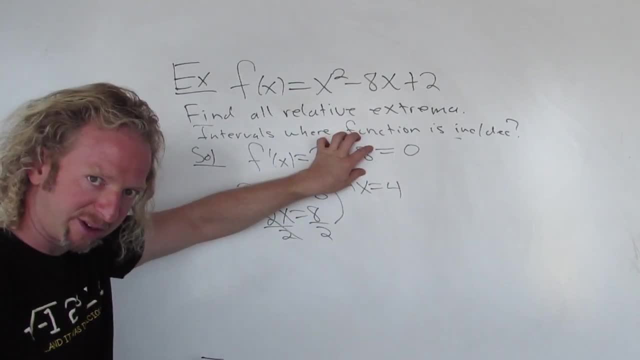 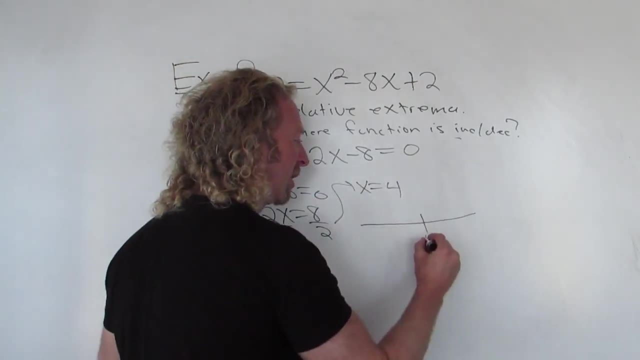 Anyways, in this problem, you take the derivative. look for any places where it's undefined, even vertical asymptotes, No issues. Set it equal to 0. Then you solve, Then you take this number and you put it on a number line. 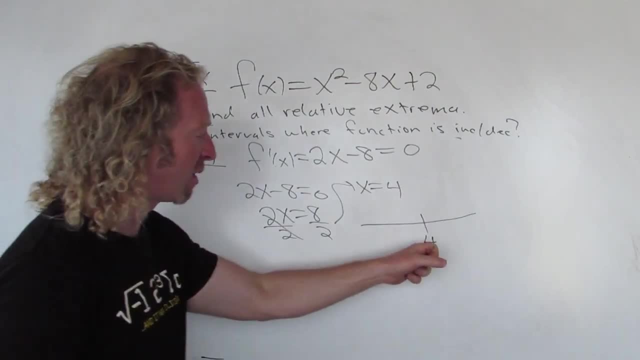 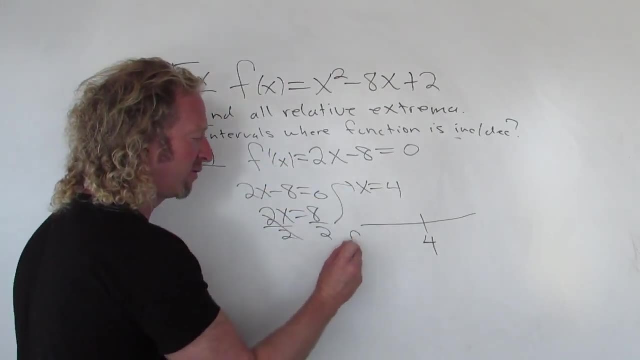 Then you pick test points. You can pick any number in the world smaller than 4 or any number in the world bigger than 4.. Let's pick 0, because 0 is less than 4.. And you plug the test points into your first derivative. 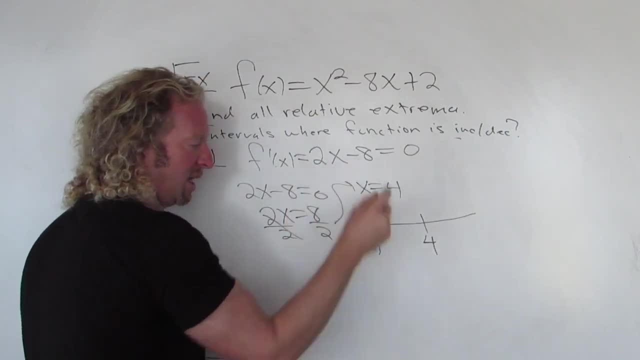 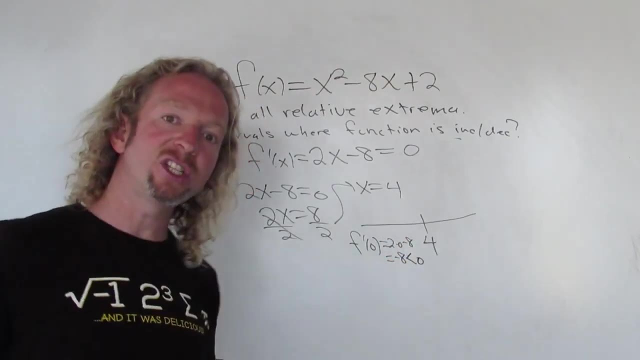 So f prime of 0. So 2 times 0 minus 8. So 2 times 0 minus 8. So that's going to be minus 8. That's less than 0. That means our function is decreasing. 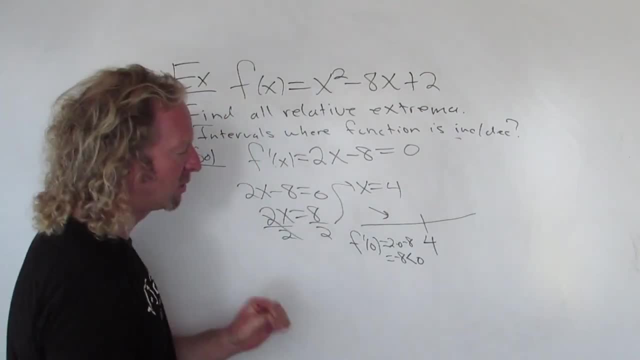 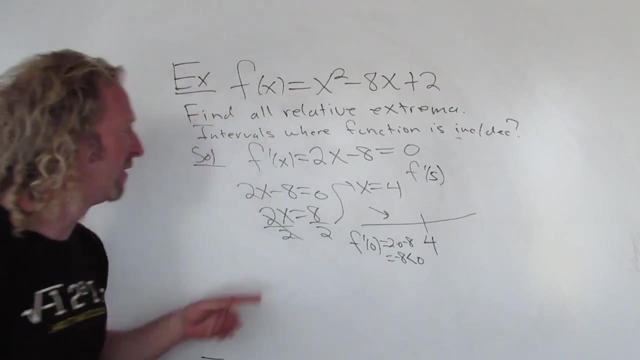 Remember negative derivative decreasing, Positive derivative increasing. Now we have to pick a number bigger than 4.. Let's do like I don't know 5.. f prime of 5. That would be 2 times 5.. So 2 times 5 minus 8.. 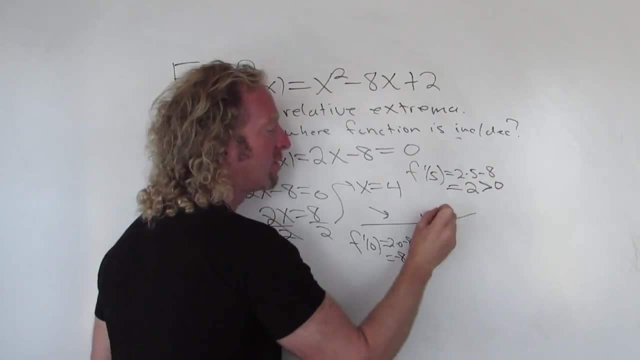 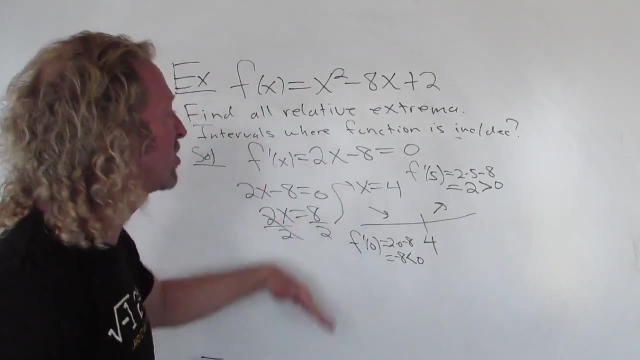 So 10 minus 8 is 2.. So it's positive. So here the function is increasing. So remember negative first derivative decreasing, Positive first derivative increasing. So the function goes from decreasing to increasing. 4 is a critical number. 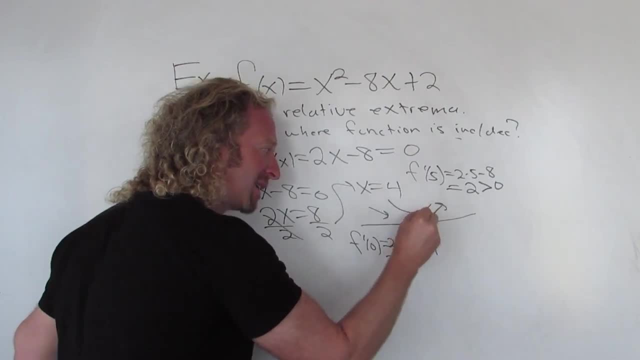 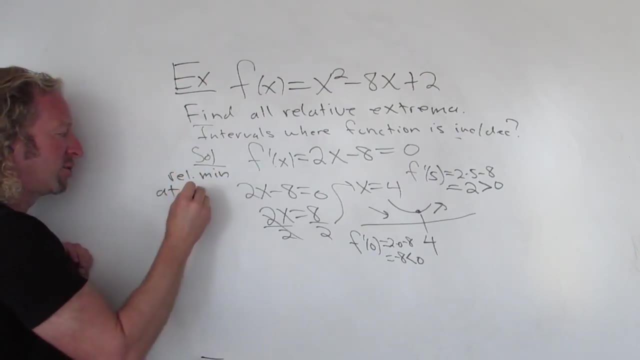 So we have a relative minimum. We have a relative minimum at x equals 4.. So that's the first derivative test, right? So we have a rel min at x equals 4.. Do you actually find the value of the relative minimum? 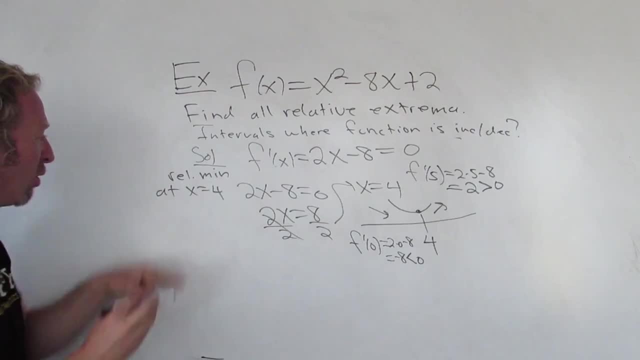 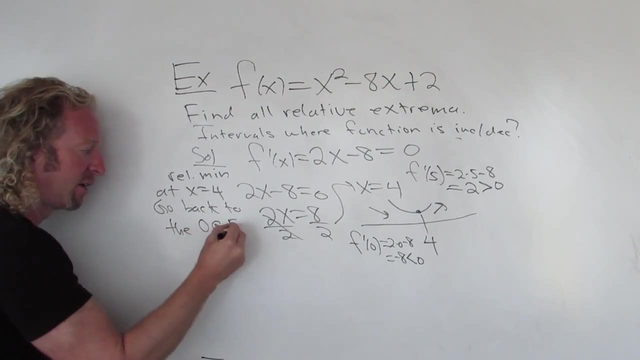 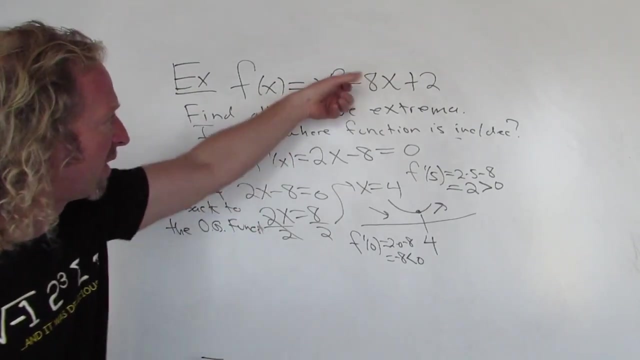 You have to go back to the original function, right? So you go back to the OG function. So go back to the OG func. Go back to the OG func. Func means function, So go back to the OG func. right, So go back to the OG function. 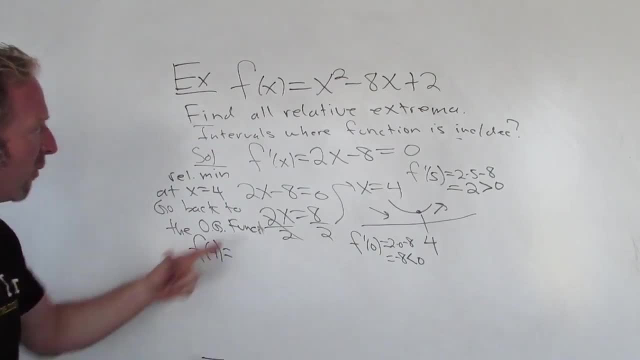 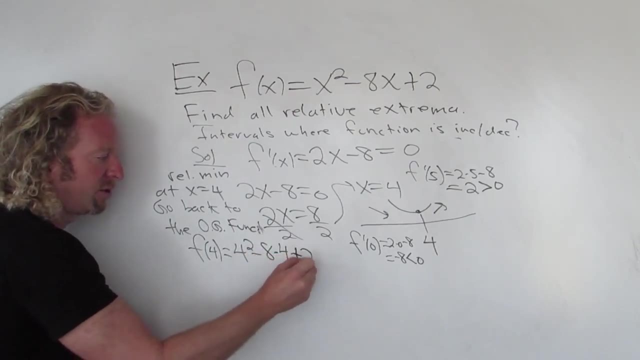 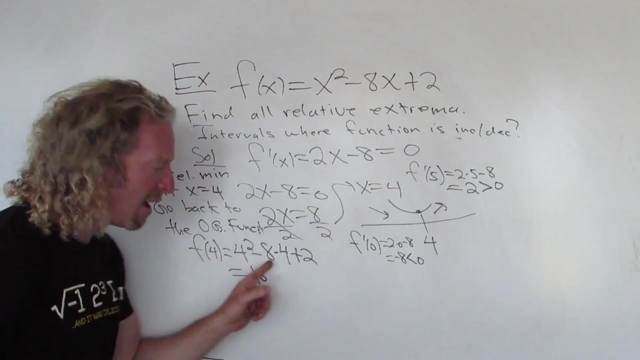 So f of 4 is going to be 4 squared minus 8 times 4 plus 2.. I don't want to mess up. So 4 squared minus 8 times 4 plus 2.. Yes, that is correct 16.. 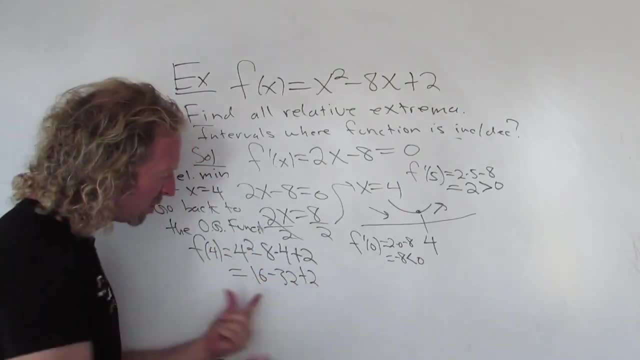 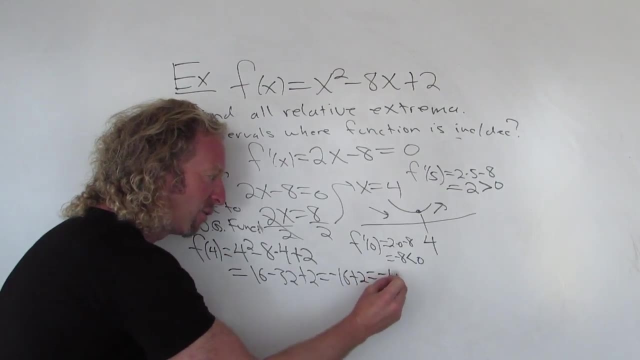 4 times 8 is 32.. So 32 plus 2.. So we get negative 16 plus 2.. Negative 16. I'm going to write it. I'm going to write it: Negative 16 plus 2 is negative 14.. 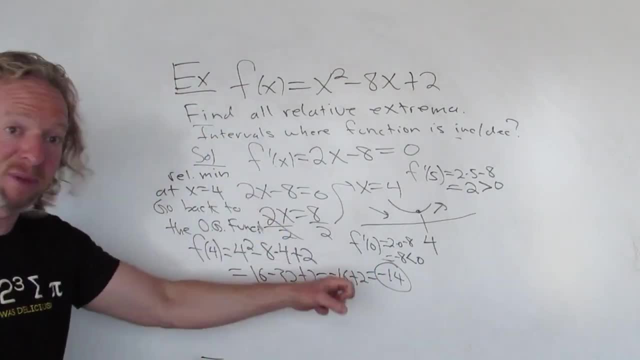 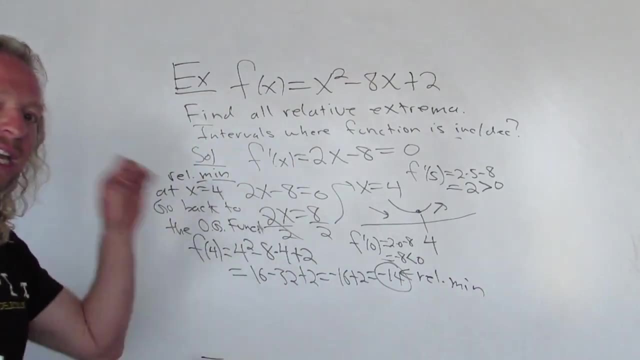 That, my friends, is the relative min. I had to look Relative min. Relative min, That's the relative min. So negative 14 is the relative min. It's the smallest y value relative to the points around it. Now, if you're taking a math class or something or you're looking at a math book, 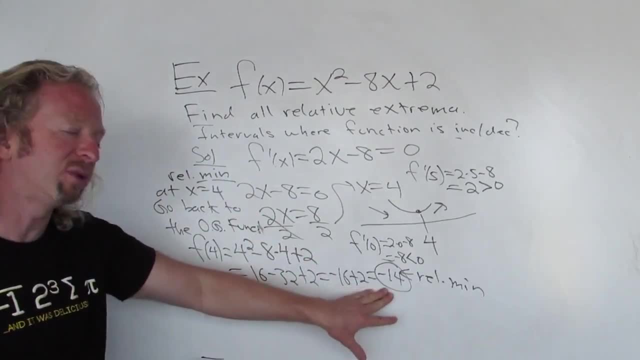 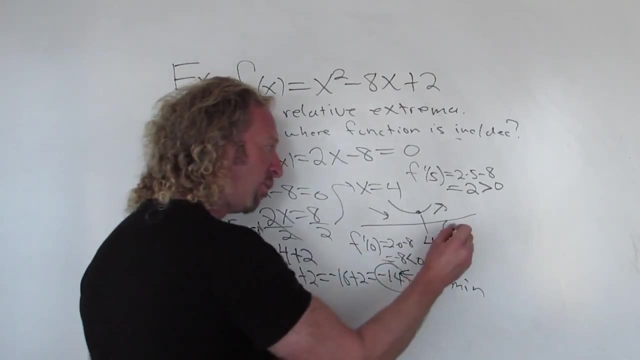 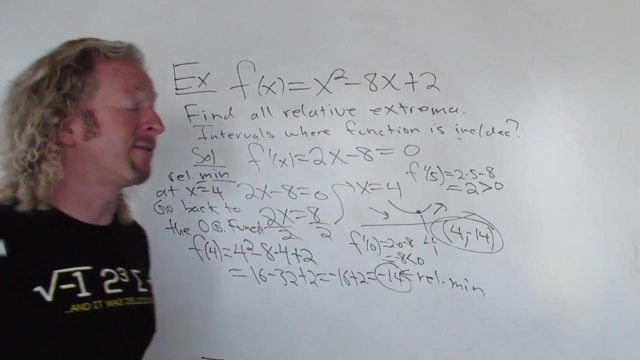 or you're doing a problem or something. usually people don't just put negative 14.. A lot of people put the ordered pair. So the ordered pair here would be 4 comma negative 14.. That's where the relative min occurs. Keep in mind: the actual relative minimum is negative 14.. 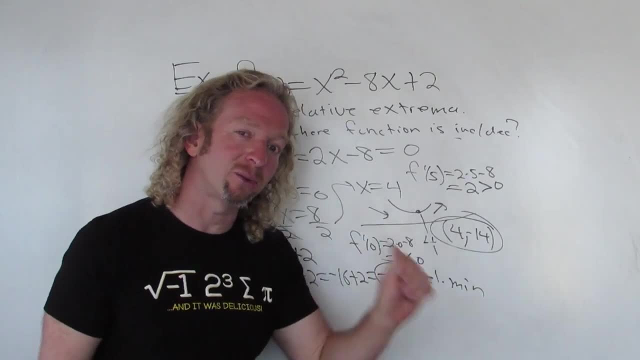 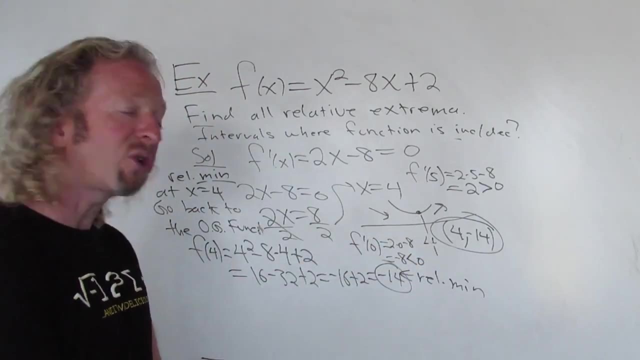 So for us to say that's the relative minimum is technically incorrect, right? Relative minimums aren't ordered pairs, No, no, no, They're y values that are smaller relative to the points around them. They're also called local minimums, by the way. 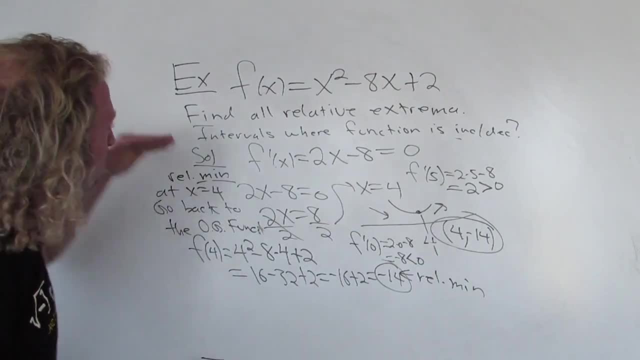 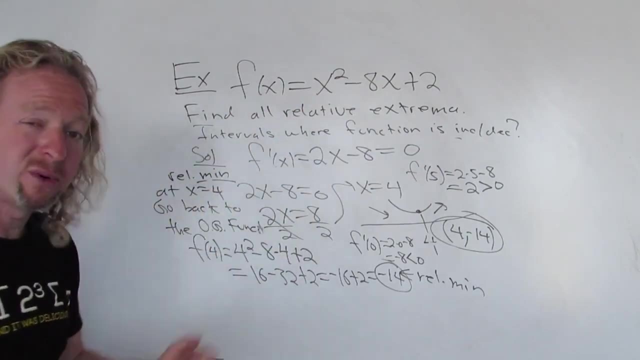 So local minimum, relative minimum, they're all the same. So a recap: We have this problem. We have to find all relative extreme out. We have to find where the function is increasing and decreasing. We're using something called the first derivative test. 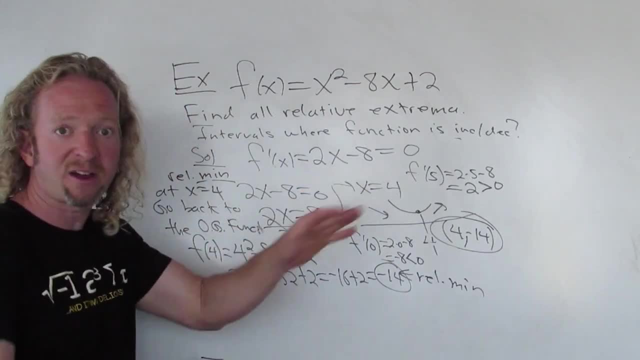 First thing you do is you take the derivative and look to see if it's undefined. Is it undefined? No, no, it's not. Things are good. Then you set it equal to 0.. You solve, You get 4.. 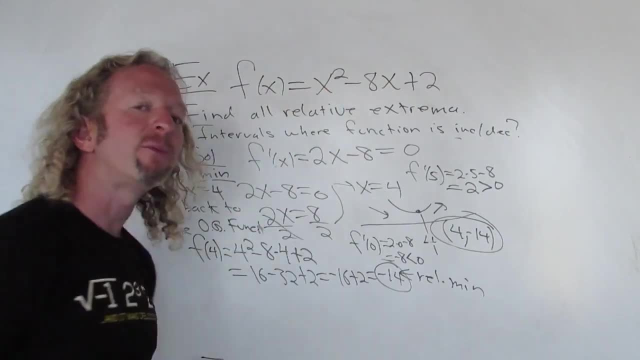 4 happens to be a critical number because it's in the domain of the original function. Remember, critical numbers are numbers in the domain of the function, where the derivative is 0 or where the derivative is undefined. right, So we take 4.. 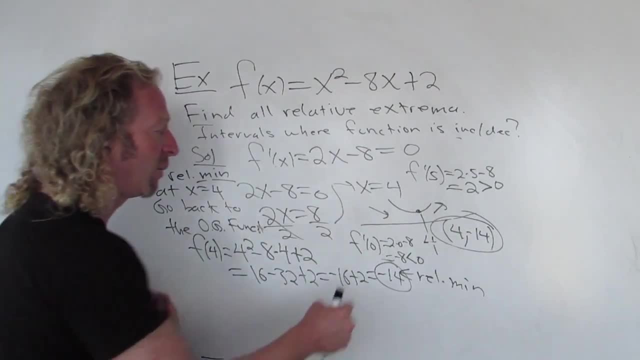 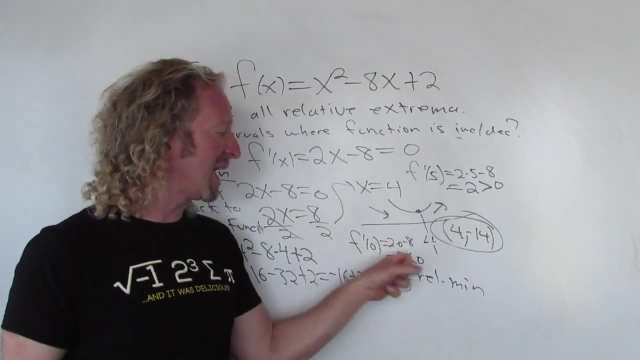 We put it on a number line. Pick test points. Pick any points you want, right? We pick 0 and 5.. Plug in 0 to the first derivative, Super key. Plug it into the first derivative. We got a negative number. 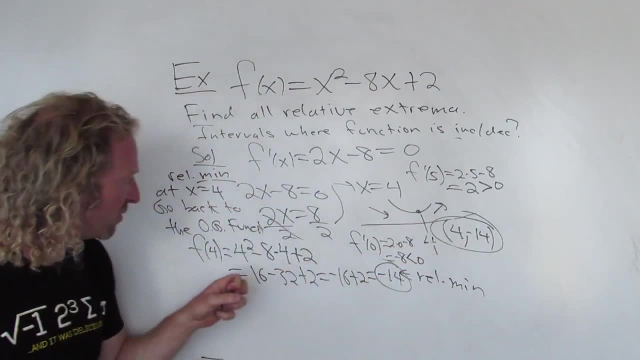 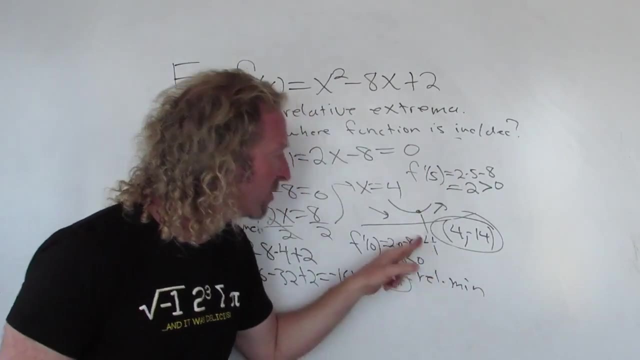 That means it's decreasing. Plug 5 into the where we do that over here, into the first derivative. We got a positive number. so it's increasing, So decreasing to increasing and it's a critical number. So we have a relative minimum at x equals 4.. 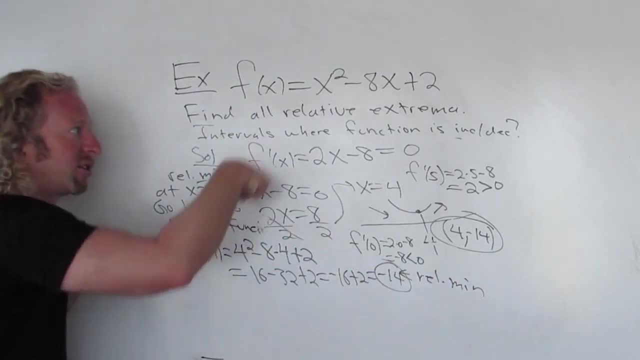 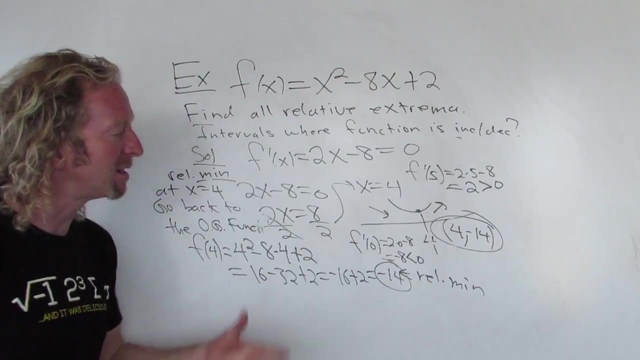 Then we took x equals 4.. We went back to the OG func- func means function- went back to the original function, plugged it in and we got negative 14.. Negative 14 is the relative minimum And keep in mind some people like to write the order pair. 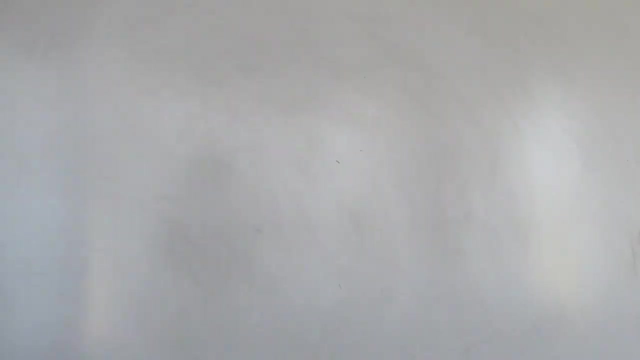 That would be 4 comma, negative 14.. Hey, what's up YouTube? In this video we're going to talk about how to use the second derivative in calculus to describe whether a function is concave up or concave down. We're going to take a very intuitive approach and do a very simple example. 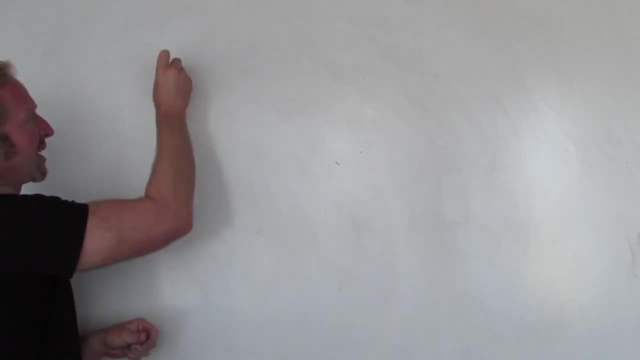 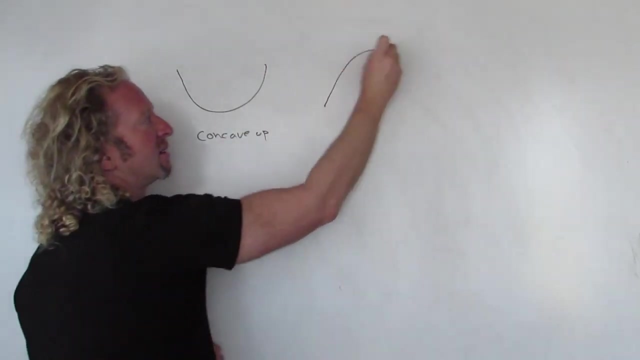 So what does it mean for a function to be concave up? So if it looks like this, we say it's concave up, Concave up. And if it looks like this, we say it's concave down, Concave down. 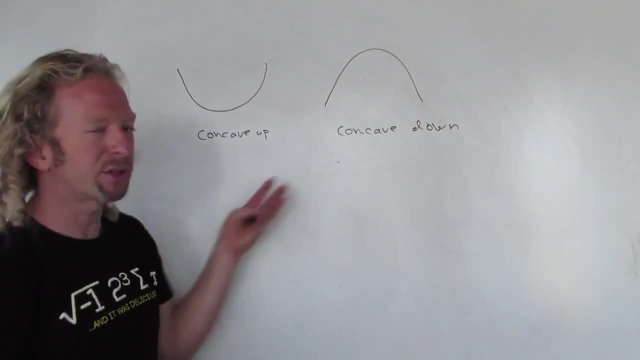 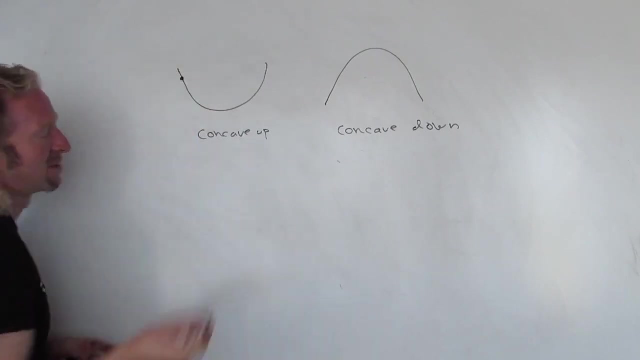 So let's investigate how we can use calculus to describe concave up and concave down. So let's see, Let's look at the slopes of the tangent lines. That's what we do in calculus: We take derivatives, So we have a function. 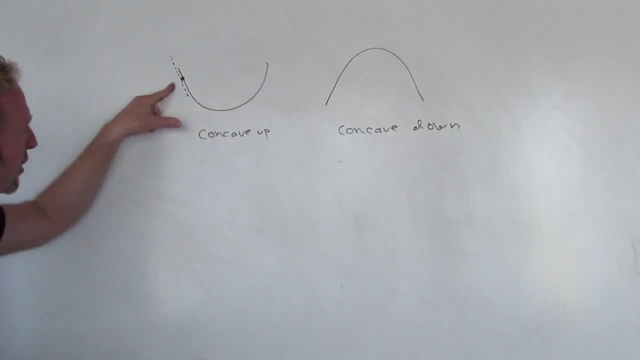 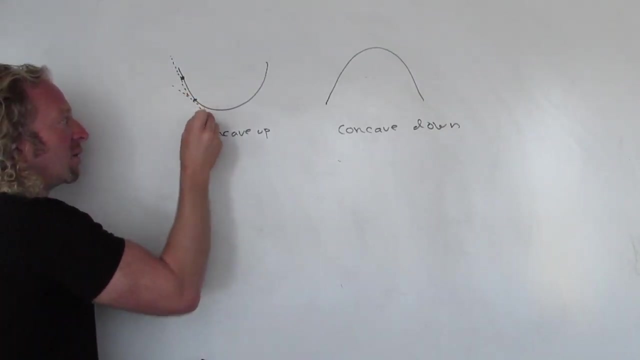 So here's the slope of the tangent line. So at this particular point the slope is negative. What about here? Well, it looks like the slope is still negative. Then here it's not as steep, though. right, It's negative, but not as steep. 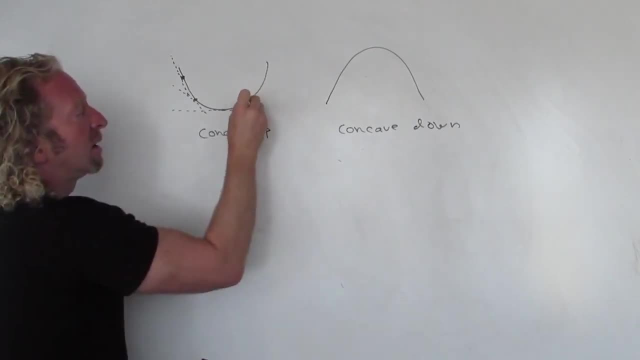 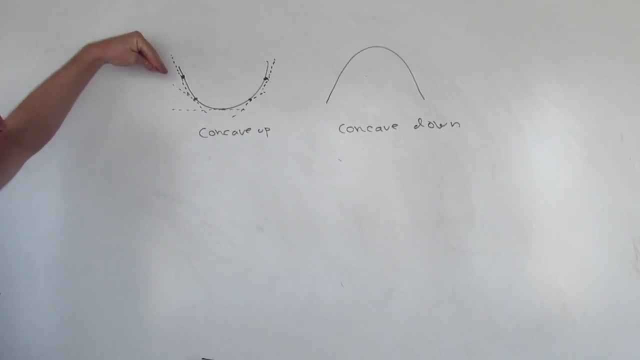 Here it's 0.. Here it's positive, And here it's even bigger because it's steeper right. So it looks like the slopes go from negative to 0 to positive, From negative to 0 to positive. 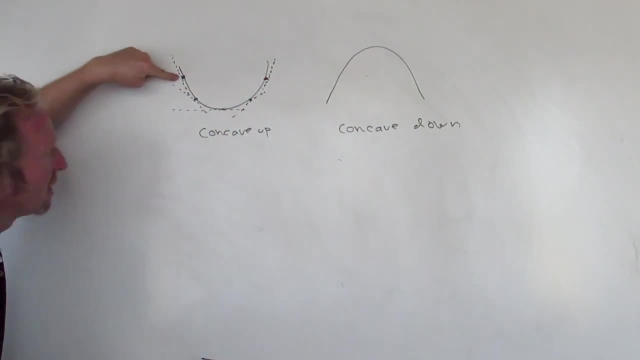 And if you look at it very carefully, this is like maybe this is negative 10.. I'm just making it up. Then this is not as steep. That might be negative 4.. This would be 0. Maybe this is 2.. 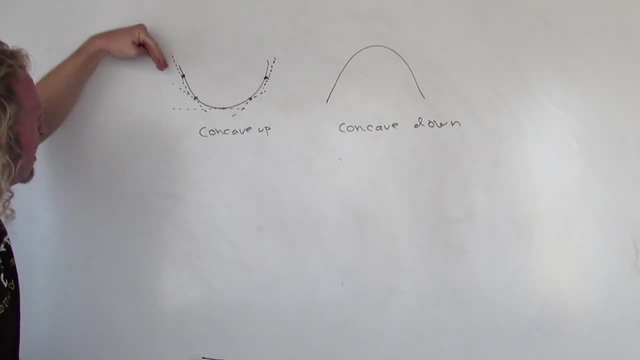 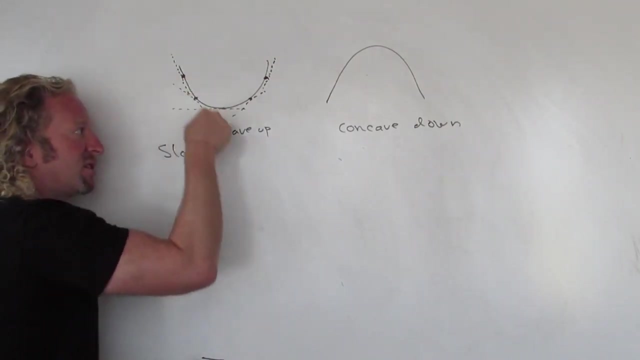 This is more steep, It's a bigger number, so like 5.. So it looks like the slopes are increasing. So the slopes are increasing. So the slopes they're going from negative to 0 to positive, So the slopes are increasing. 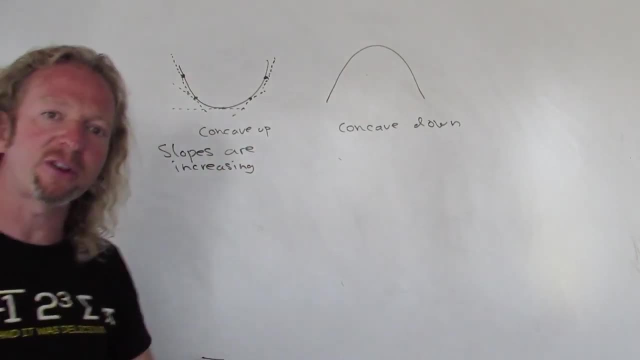 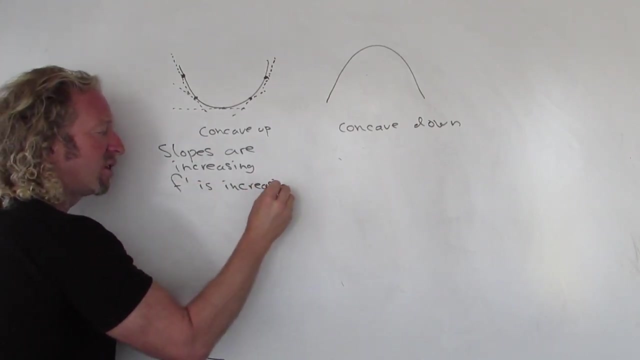 The slopes are increasing. But what are the slopes? The slopes are the values of the first derivative. So the first derivative is negative. The second derivative is increasing. So if the first derivative is increasing, that means its derivative is positive. Remember, if a function is increasing, it has a positive derivative. 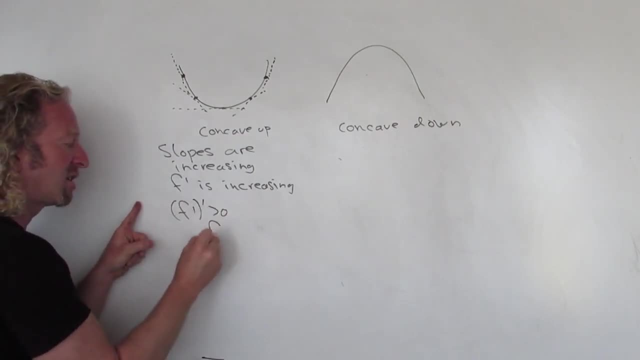 So the derivative of the derivative is positive. So the second derivative is positive. Boom. So if it's concave up on an interval, the second derivative is positive. So if you have a function that's concave up on an interval, the second derivative is positive. 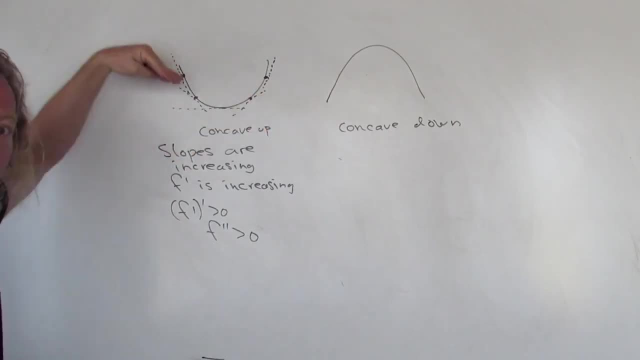 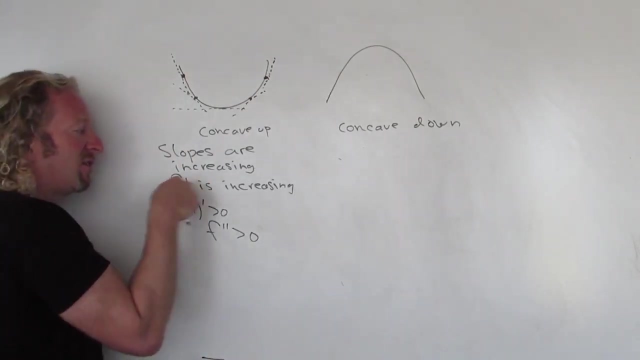 We do that again. Slope is negative, 0, positive, So the slopes are increasing. Slopes are increasing. The values of the slopes are the values of the first derivative. That means the first derivative is increasing, So its derivative is positive. 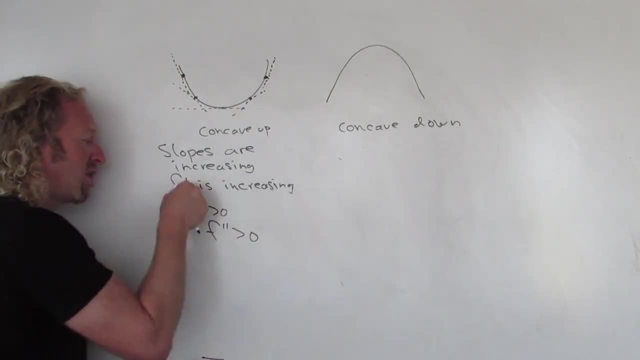 Remember: if a function is increasing, its derivative is positive. Therefore, the derivative of the derivative is positive. So concave up positive, Really easy to memorize it right. Concave up positive First derivative—positive, second derivative. 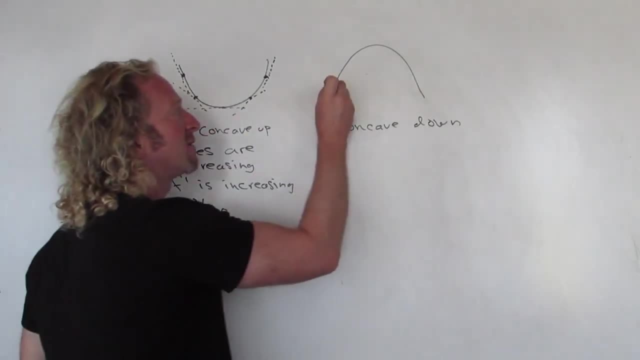 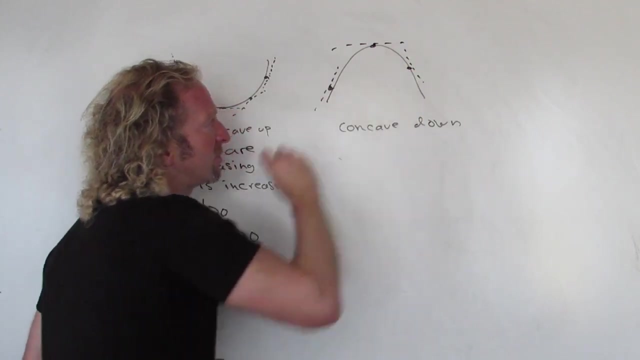 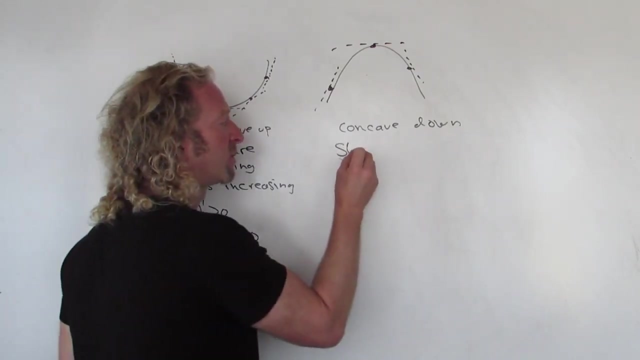 Concave up. positive second derivative: What about here? Here we have a positive slope, Here we have a slope of 0. Here we have a negative slope. So it looks like the slopes are going from. the slopes are going from positive to zero to negative. So the slopes are decreasing. So slopes 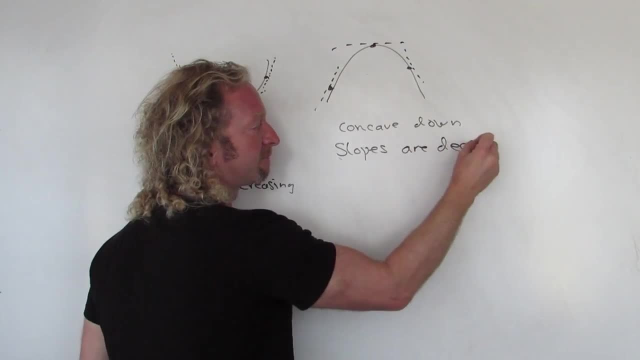 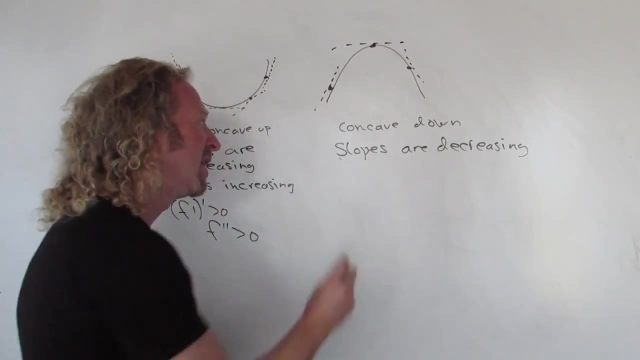 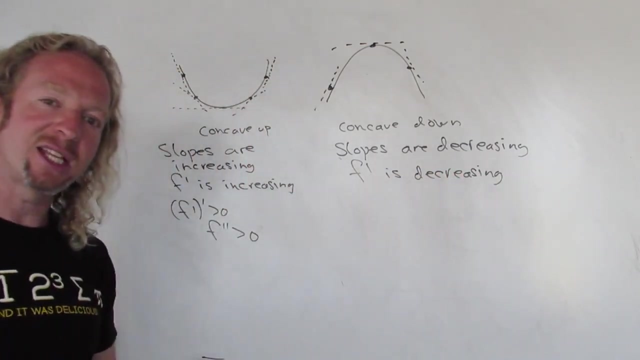 are decreasing. Okay, the slopes are decreasing. The values of the slopes are the values of the first derivative. That means that the first derivative is decreasing. First derivative is decreasing. If you have a function that's decreasing on an interval, that means its 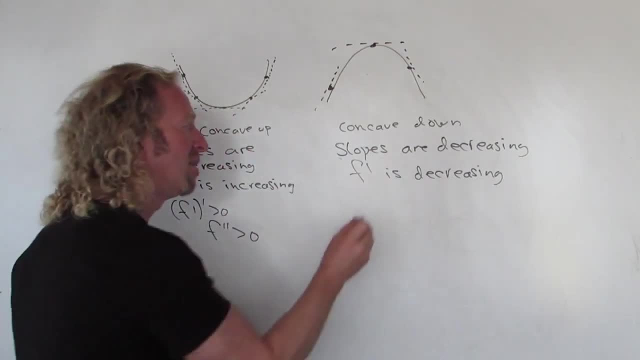 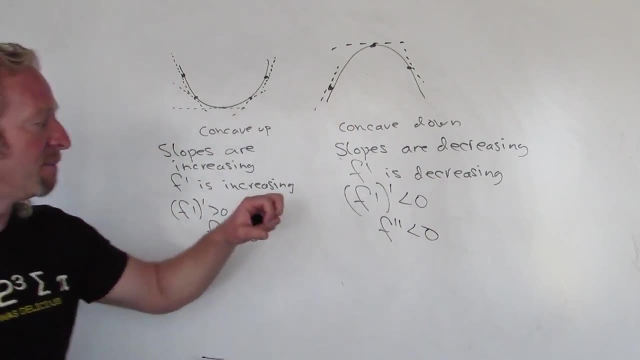 derivative is negative, So this function is decreasing, So its derivative is negative, So the derivative of the derivative is negative. So concave down means you have a negative second derivative. Concave down means you have a negative second derivative on an interval. 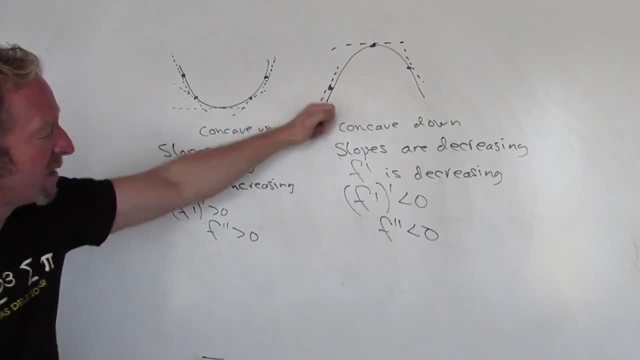 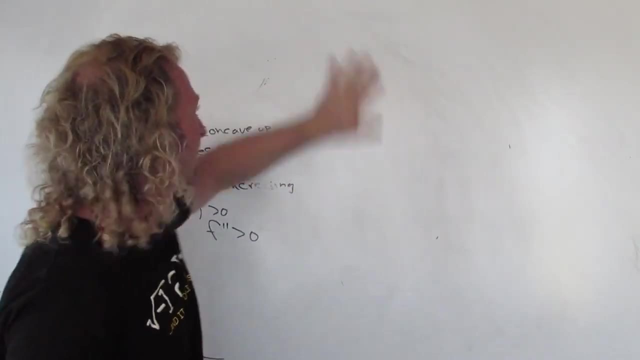 on an interval. Okay, so concave up- second derivative is positive, Concave down- second derivative is negative. Let's go ahead and do a really, really, really simple example. I'm just going to make one up and we'll do it I'm trying to think of like the easiest possible. 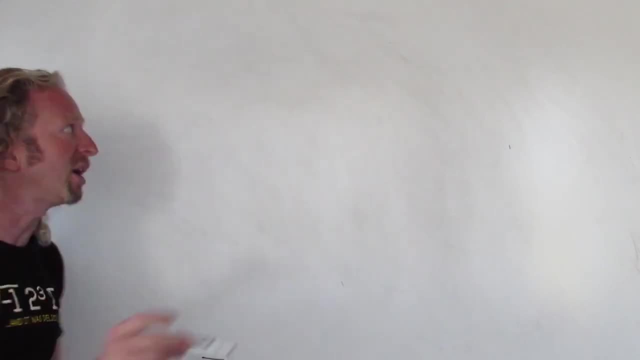 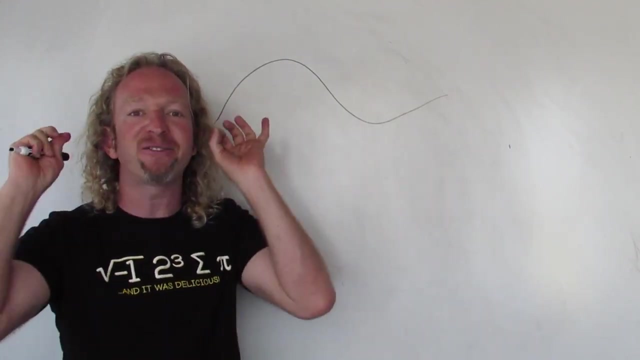 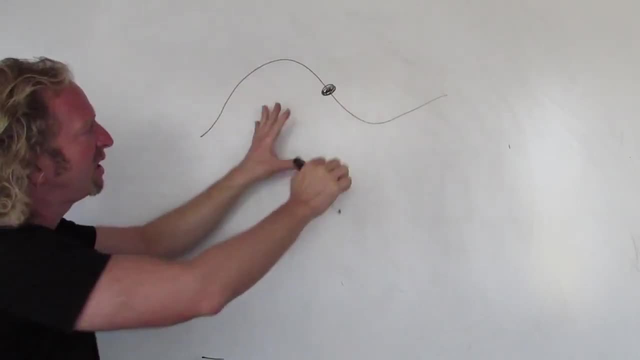 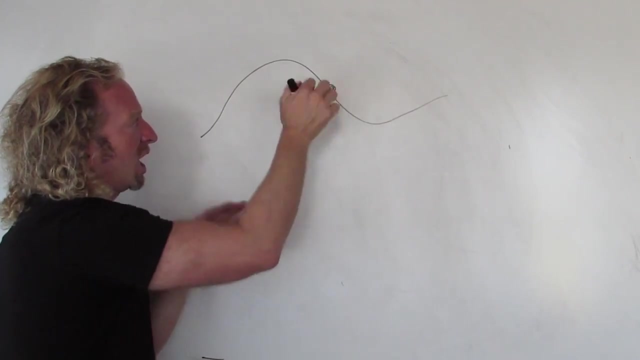 con down. At some point here, at some point here, it will change to concave up. Where's that point? I have no idea, but it's somewhere there, right? So concave down, concave up, So it will change. 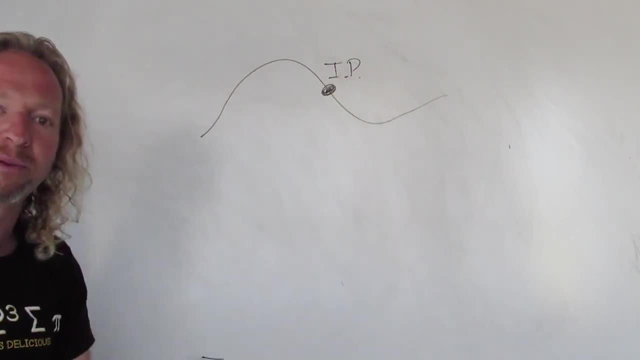 That's called an IP, inflection point, inflection point. Let me write that down. It's called an inflection, So you know how to say it. It's called an inflection point, So you know how to say it. 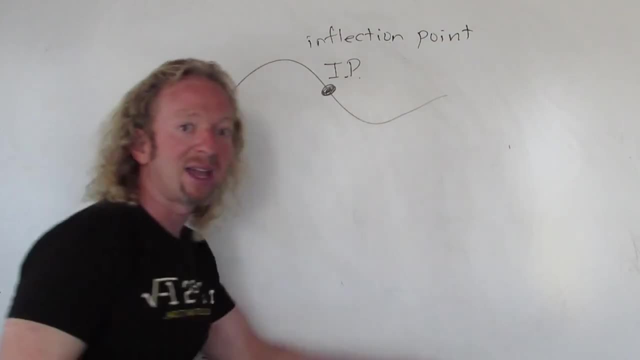 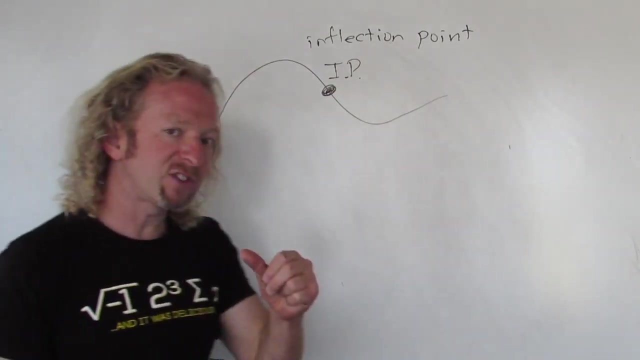 So it's an ordered pair. It's an X comma Y, hence the word point. So whenever you're doing homework or just doing this for fun, it's always an ordered pair. for inflection point: All right. so positive second derivative concave up. Negative second derivative concave down. If a point on the graph 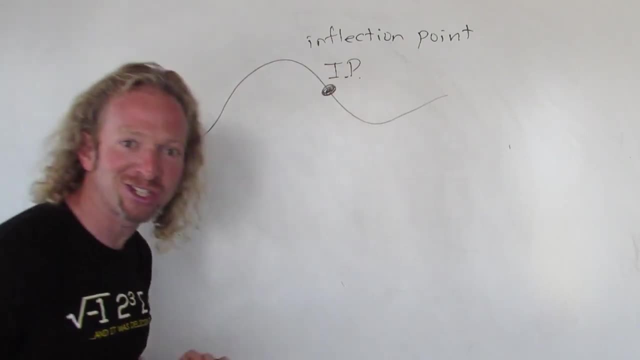 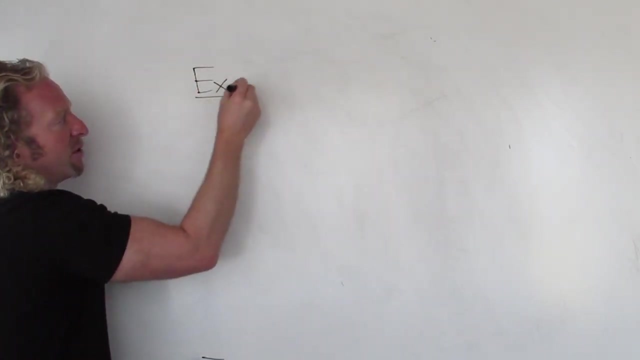 with a concavity. there's a fun word: where the concavity changes, it's called an inflection point. Let's do a simple, simple, simple example. EX means example. Let's do F of X. This one should be pretty easy. 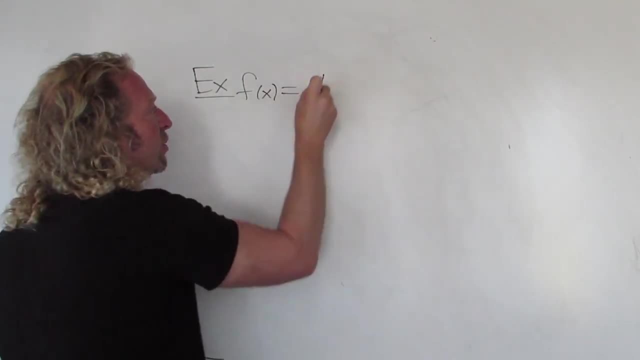 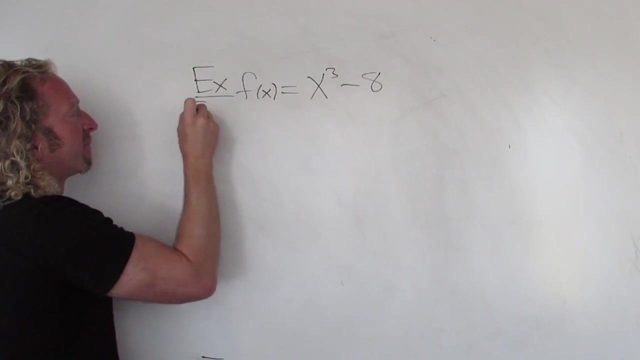 I think F of X equals X cubed. Yeah, X cubed. Oh minus 8.. Why not, Let's make it a little bit harder- It's not going to affect anything, And we're going to find the intervals where it's. 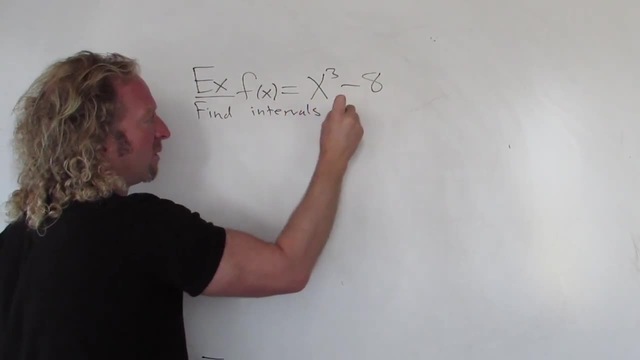 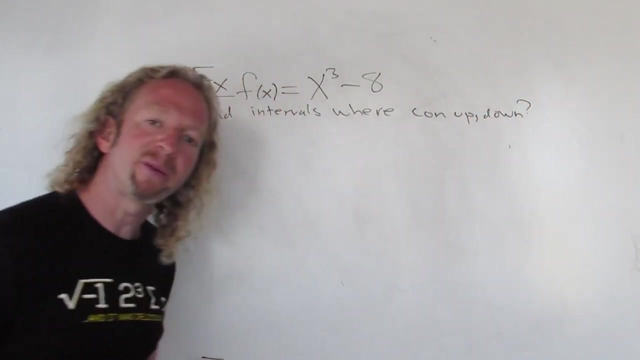 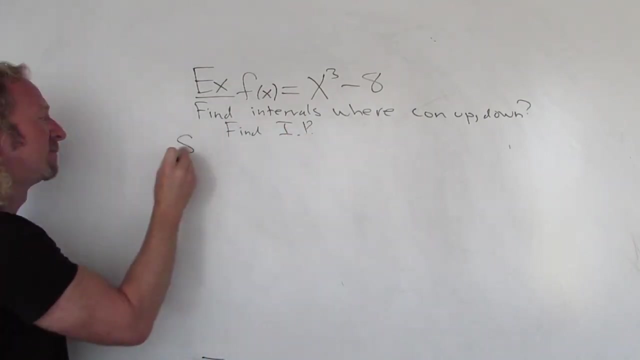 intervals where- let's use bad English- intervals where con up down, intervals where the function is concave up and concave down, And let's find any inflection points. So find inflection points, if any. Okay solution. So whenever you're looking to see where a function is concave up or concave, 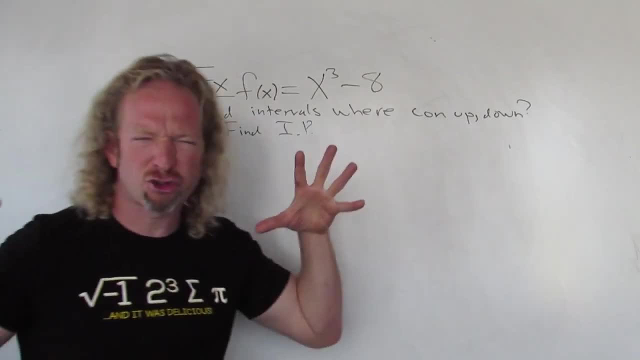 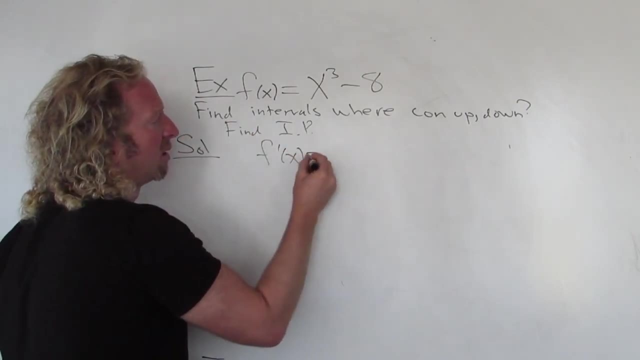 down and you're looking for inflection points, you have to go straight to the second derivative, okay, So you take the derivative twice. So you take the derivative once. The derivative here use the power rule, right, So it'd be 3X squared. The derivative of negative 8 is: 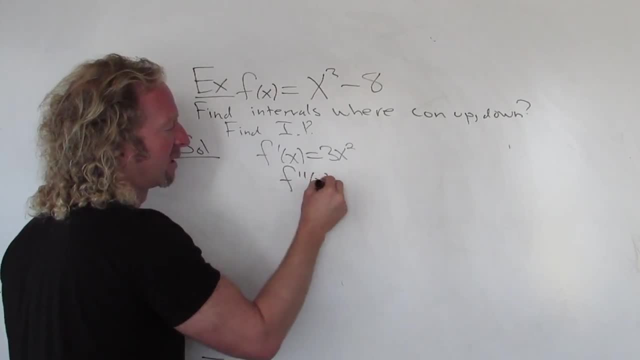 0,. so piece of cake. Take the derivative again, You get 6A. So you go straight to the second derivative. Don't do this. You don't need to do this. You don't need to do this, You don't. 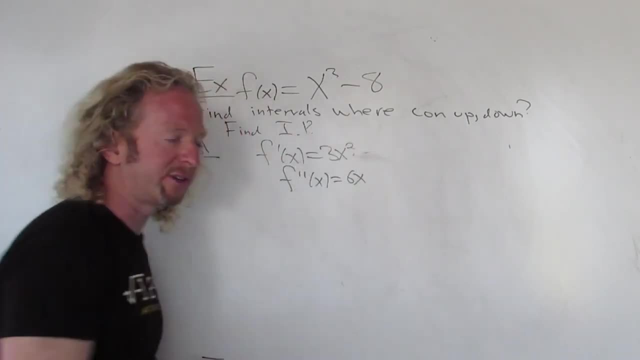 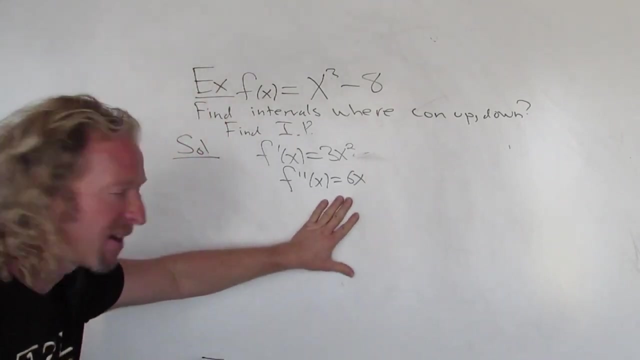 need to do that, right? No, no, All we care about is the second derivative. okay, And what you do now is you look to see if it's undefined. okay, So, is it undefined anywhere? right? Are there any places where it's undefined? No, Then you set it equal to 0, and then you 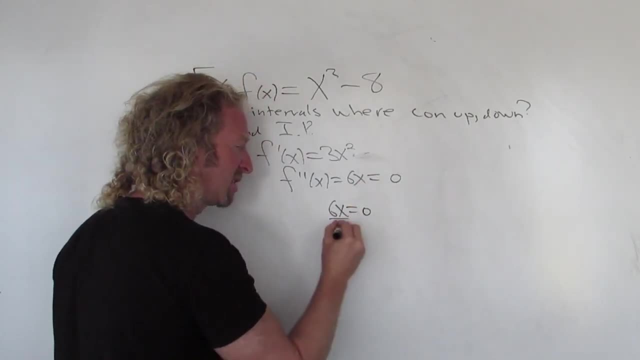 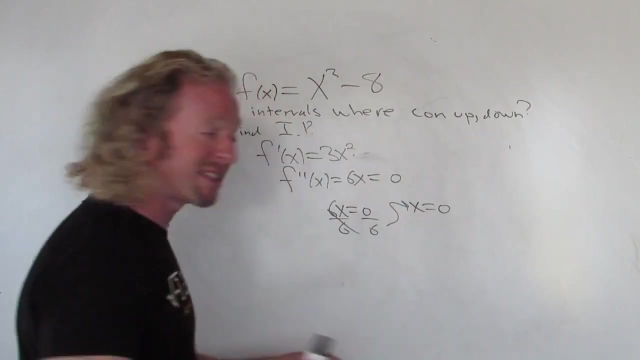 solve for X, So divide it by 6,, so we get 0.. So what is this? Is this a critical point? No, no. Is it a critical number? No, no, It's not a that. It doesn't have a name, right. 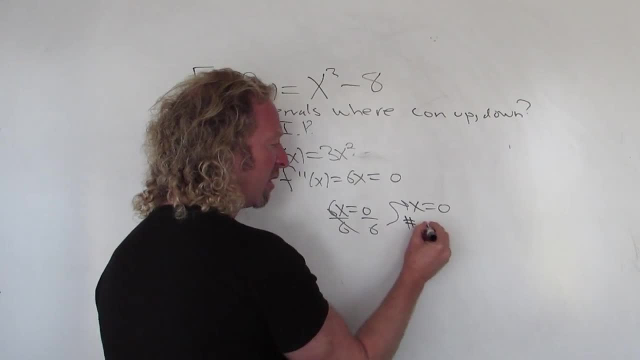 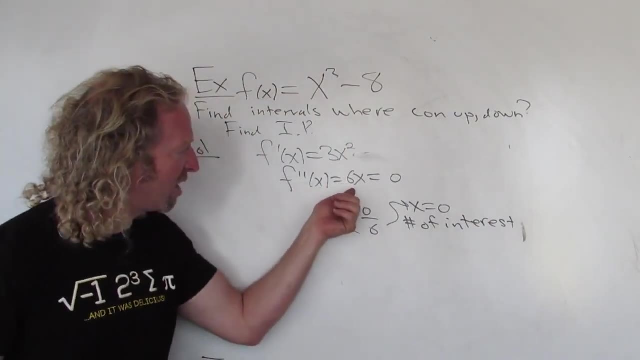 It doesn't have a name. This is a point of interest. It's a number of interest. It's a number of interest. It's a number of interest. So we're looking for the numbers of interest. Numbers of interest, just making that up- are numbers where the second derivative does not make any sense. 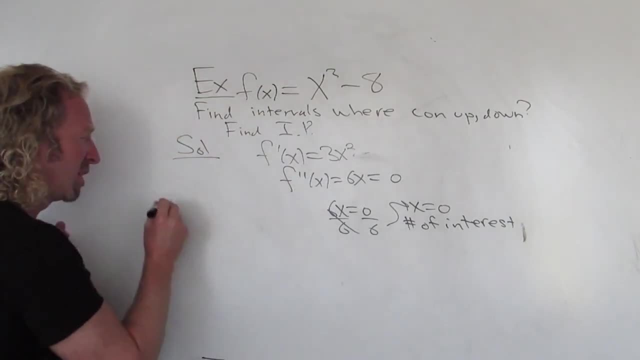 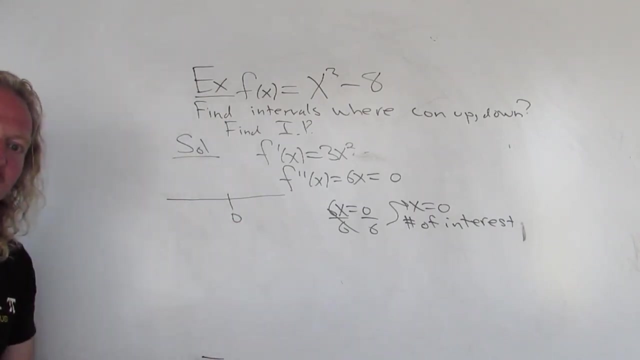 or where it's equal to 0,. okay, That what you do is you take those numbers of interest and you put them on a little graph- This is called a sine diagram- okay, And you pick test points and we're checking for concavity, So we care about the sine of the second derivative. 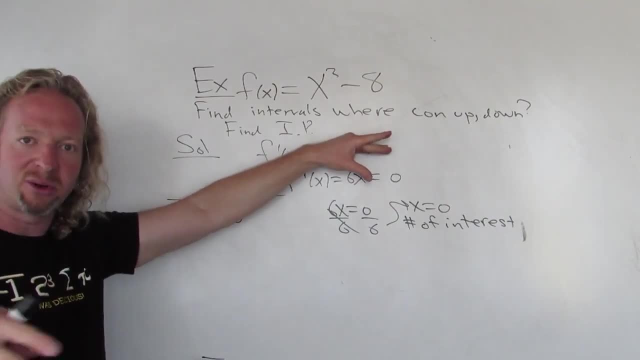 We were doing increasing, decreasing. It's different. That's, when you set the first derivative equal to 0 and all that stuff Con up, con down, you use the second derivative, okay. So let's take a nice number, less than. 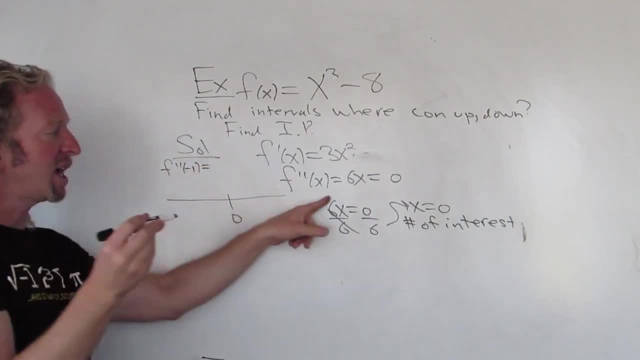 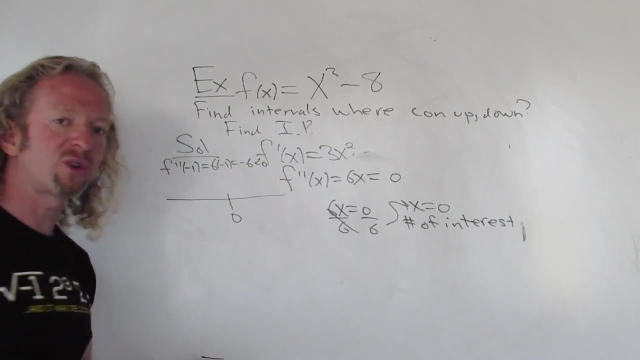 0. How about negative 1?? If you plug in negative 1 into the second derivative, you get 6 times negative 1, so you get negative 6. That's less than 0. And remember, when the second derivative is less than 0, it's concave down right. So this is con down. Let's not do that. 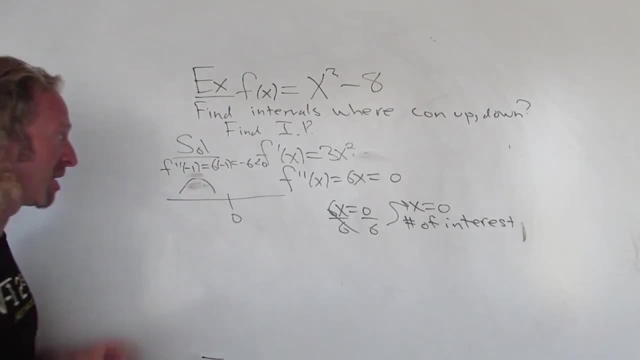 So put little faces there and stuff, but no, So it's con down, So con down. Then I think a number over here: How about 1?? That would be 6 times 1.. That would be 6.. It's positive, so it's con up. So second derivative: negative con down. 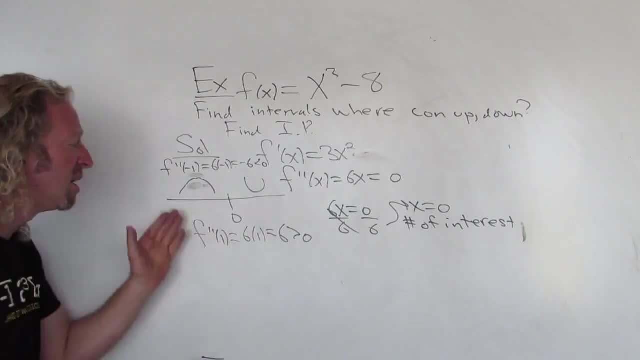 Second derivative positive con up. You can pick any number you want. You can pick negative a million. So now we know the answers to con up and con down. So con up would be from 0 to infinity. Always use parentheses. That's the interval where it's concave up, Con down. 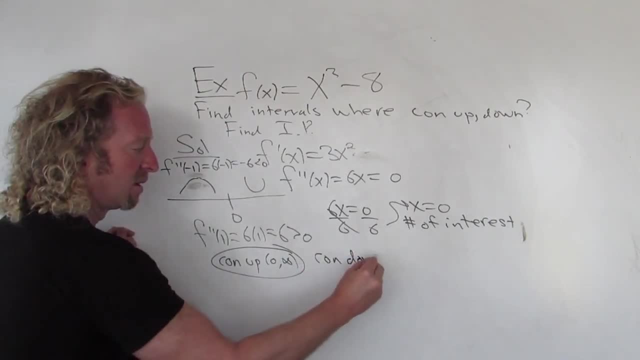 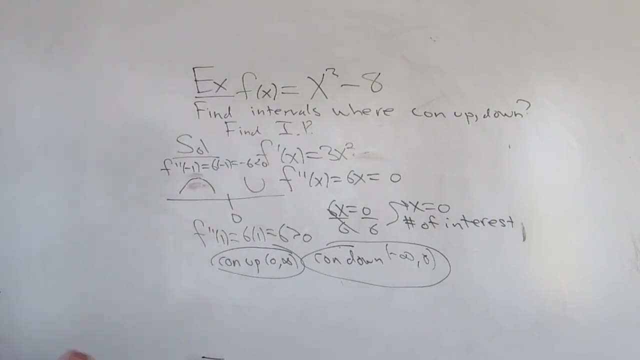 would be negative infinity to 0. So con down would be negative infinity to 0.. Negative infinity to 0. That would be con down. So con down would be negative infinity to 0.. Recap just from the beginning. We're looking for the intervals where the function is concave. 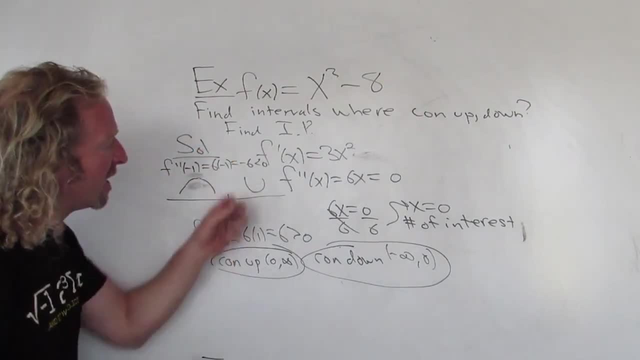 up or concave down, And we're looking for the inflection point, which we haven't yet to do. Go straight to the second derivative. Take the second derivative, look at it. Is it undefined anywhere? Is there anywhere where it doesn't make sense? No, Everything's. 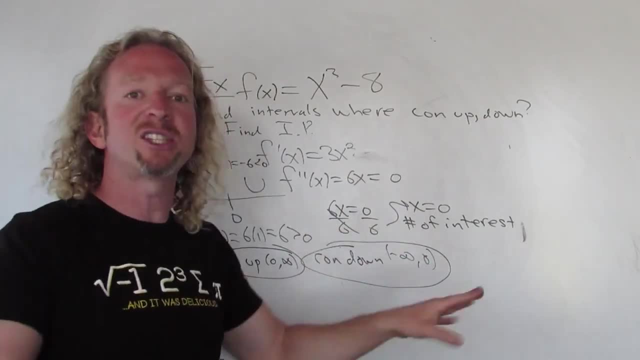 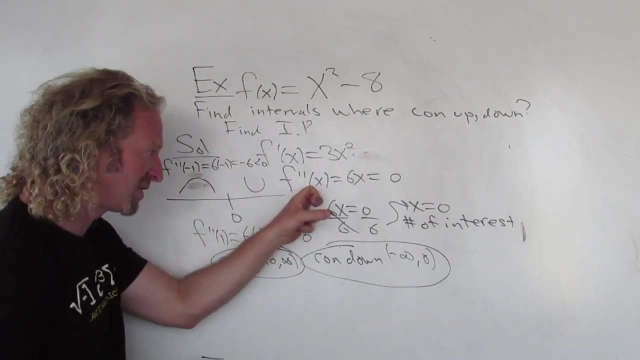 okay, right, Set it equal to 0, solve: You get x equals 0.. What is that called? that has no name. We called it a number of interest. Take your numbers of interest. What are those? Those are numbers where the second derivative is 0 or where the second derivative is undefined. 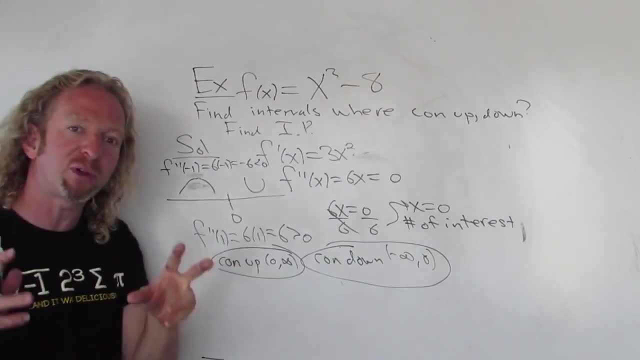 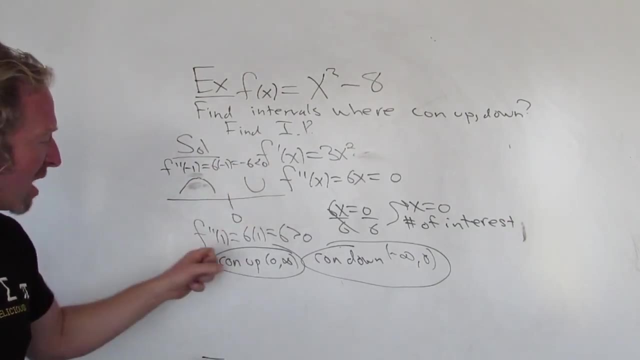 These are numbers of interest. You plot them on a number line, You pick test points, You plug them into the second derivative. We use negative 1.. We've got a negative number, so it's con down. We use 1.. We've got a positive number, so it's con up. So it's going to be. 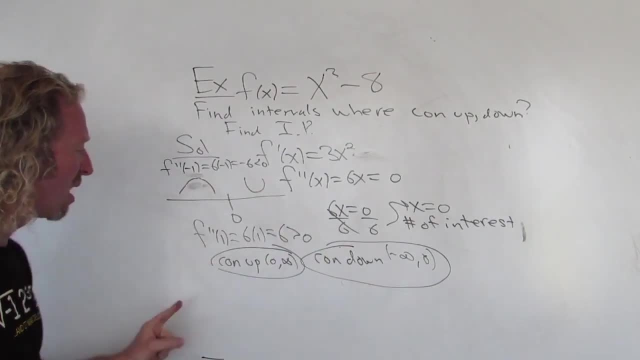 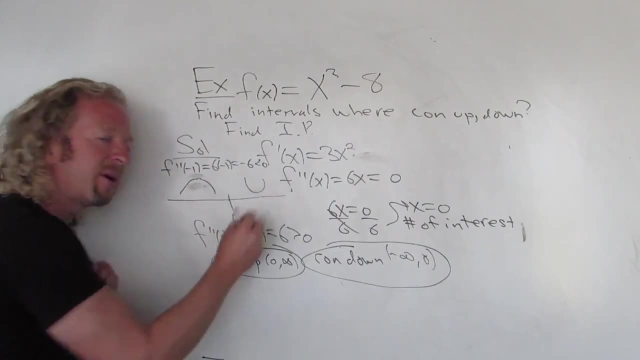 concave down from negative infinity to 0.. Boom, there it is. Concave up from 0 to infinity. Boom, there it is. Look, the concavity- there's that word again. The concavity changes from down to up. at x equals 0. That means that at x equals 0, we have an inflection point. 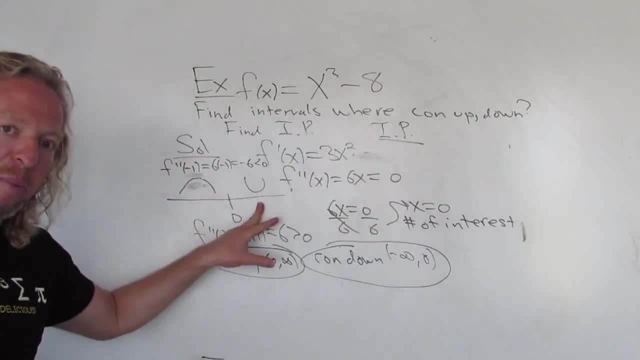 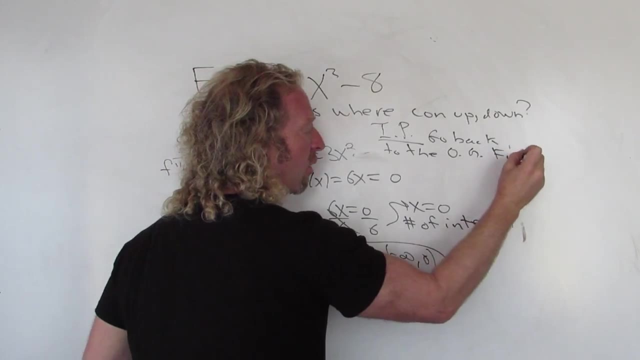 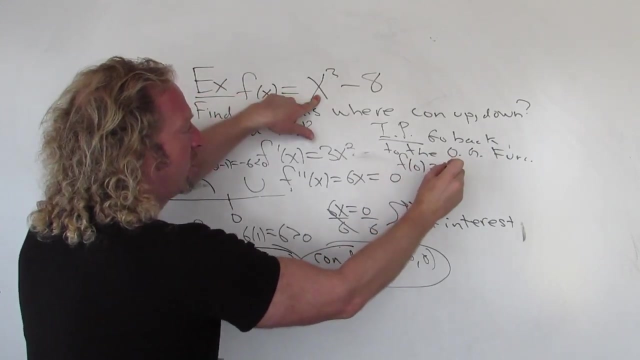 To find the actual point. you go 0 and you go back to the OG func, Go back to the OG func, Go back to the OG func. OG means original function, Original function. So you take your 0 and you plug it back in here. So f of 0, that's 0 cubed minus 8. So that's negative 8.. Is that the? 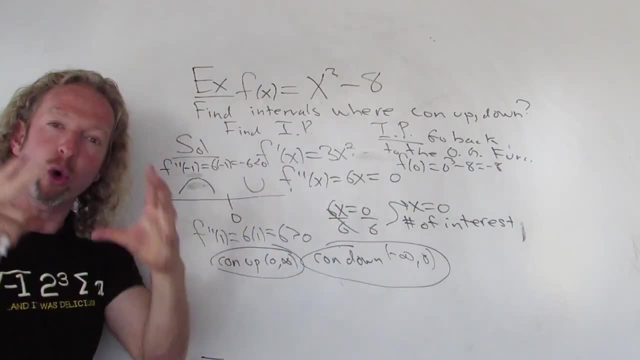 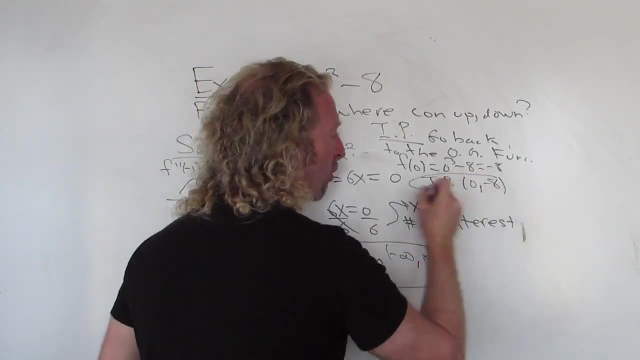 inflection point. No, it's not. The inflection point is an ordered pair, It's a point, Hence the word point. So the IP would be 0, negative 8. That would be the point on the graph of this. 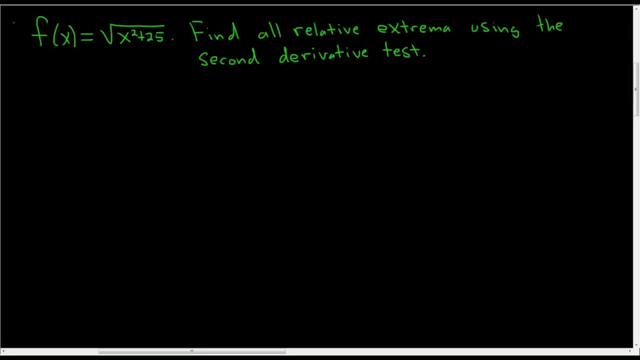 function where the concavity changes Find all relative extrema using the second derivative test. So solution: So to use the second derivative test. you start by finding the critical numbers, Then you take the critical numbers and you plug them into the second derivative. If it's positive, you have a min. 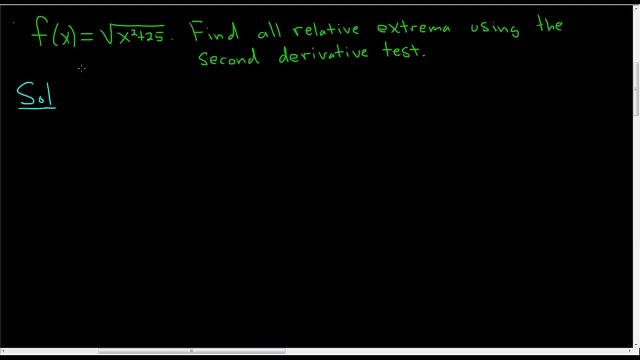 If it's negative, you have a max And you're pretty much done. So let's start by taking the derivative and finding the critical numbers. So let's rewrite this first. This can be written as x squared plus 25 to the 1 half. It makes it much easier to take the first. 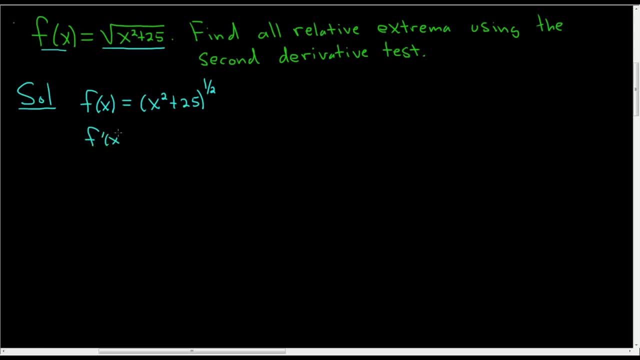 derivative. So f prime of x is equal to. you take the 1 half and you bring it down, So we get 1 half x squared plus looks like 25.. And then 1 half minus 1 is negative, 1 half times the derivative. 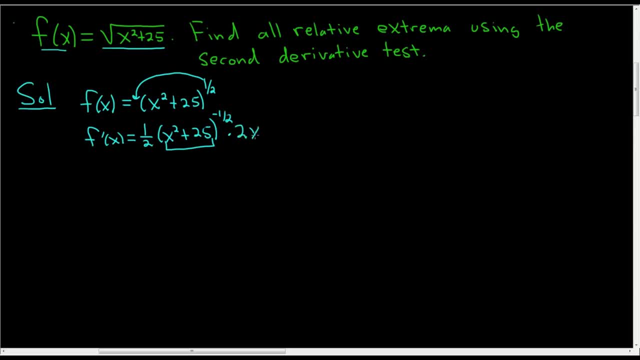 of the inside. So we have to use the chain rule. So that's 2x And we set this equal to 0. This can be rewritten as follows: So f prime of x is equal. to see the 2s cancel, The x will stay upstairs And we can bring. 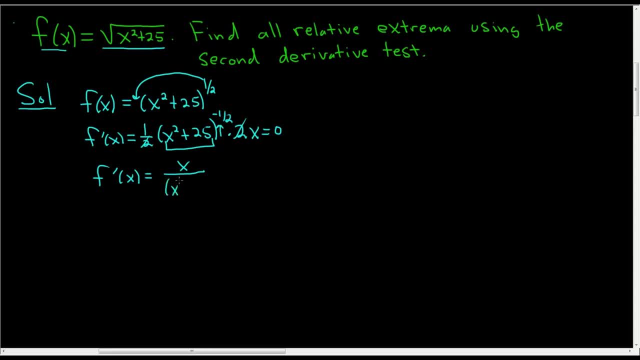 this guy downstairs and it becomes positive. So x squared plus 25 to the 1 half, And we set this equal to 0.. Okay, This is a fraction. There's no common factors, So we can automatically set the numerator equal to 0.. And that's going to. 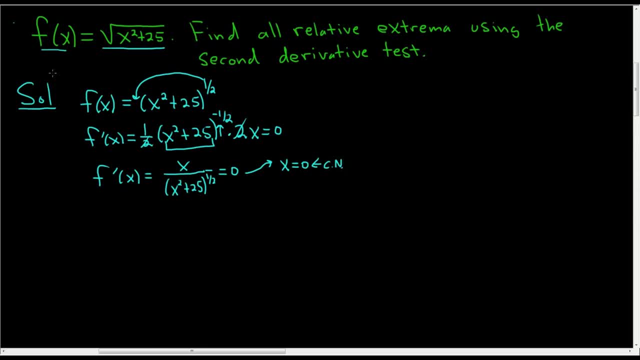 be our critical number. Now we have to take the second derivative. So step 1 of the second derivative test was finding the critical numbers. We did that And now we'll take the second derivative. So f, double prime of x, We'll use the quotient rule, So it's the derivative of the first. 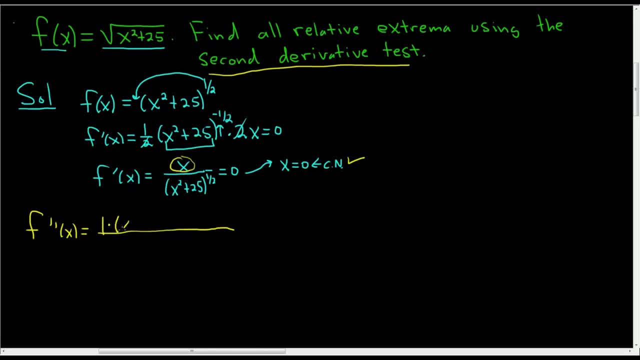 or the top piece. So 1 times the second piece. Okay, So x squared plus 25 to the 1 half, minus the first piece or the top piece times the derivative of the second piece or bottom piece. So here we have to use the chain rule. So we'll bring. 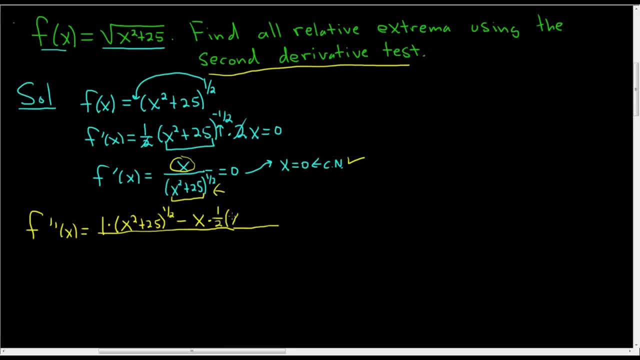 the 1 half down And we'll leave the inside untouched. So x squared plus 25.. Subtract 1. We get negative 1 half And then chain rule. Chain rule says we multiply by the derivative Of x squared plus 25.. So 2x. And all of this is being divided by this thing here with all. 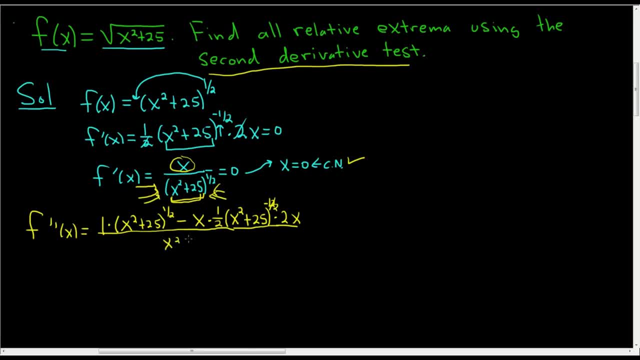 the arrows squared, So that would just be x squared plus 25.. And do we set this equal to 0? No, No way. We find the second derivative And we plug in the critical number. That's it. So f double prime of 0. So this is 0 plus 25.. So it's 25.. 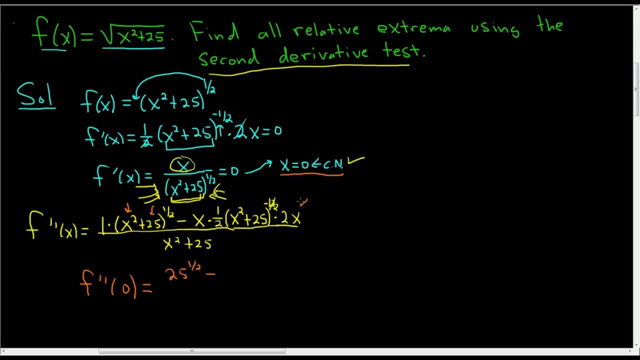 So we can actually get a derivative of 25 to the 1. half minus x is 0. Right, So there's 0's here And 0 times the number is 0. So all of this is just 0. So you get 0. And in: 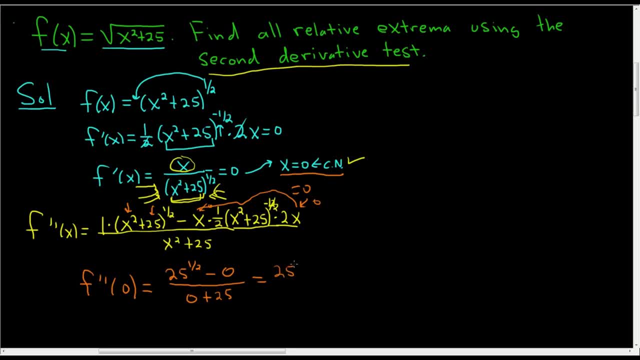 the bottom you get looks like 0 plus 25.. So we end up with 25 to the 1 half over 25, which is positive. So we have: Okay, a min at x equals zero, right? That's the second derivative test. You find the critical numbers. 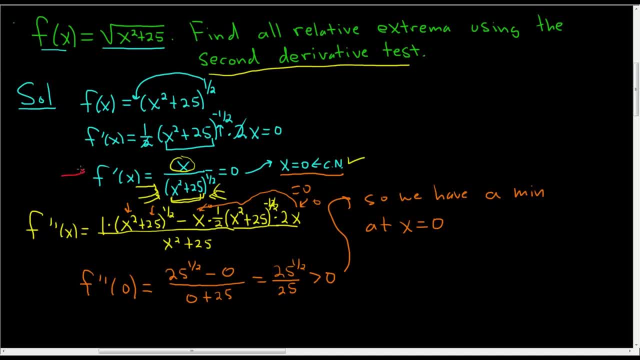 which we did. So to find the critical numbers, you take the first derivative, set it equal to zero. There it is Boom. Take the second derivative, plug in your critical number. If it's positive, you have a min, If it's negative, you have a max. So we have a min at x. 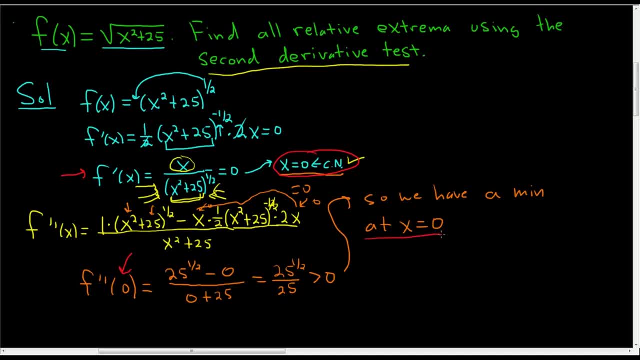 equals zero. To actually find the minimum, we take the zero and plug it back into the original function. So f of zero is the square root of zero squared plus 25.. That's the square root of 25, which is equal to five. So five, that's the minimum Minimum right, And that's it. That's. 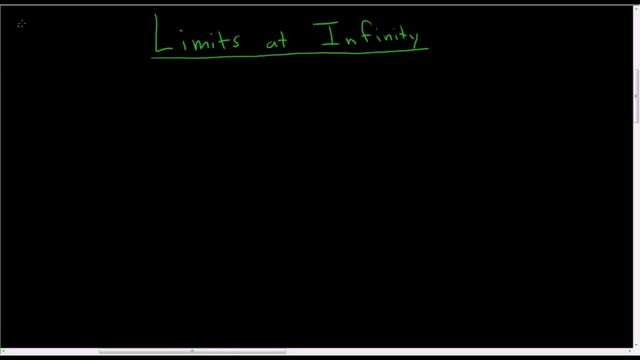 how you use the second derivative test. This will be a really quick video on limits at infinity. We're just going to look at the easy examples in this video, So let's start by looking at the limit as x approaches infinity. Let's say 3x squared plus 2x plus 10 over 5x squared. 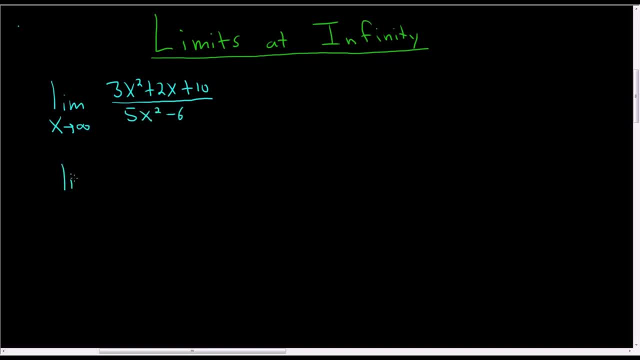 minus 6.. Then we're going to look at the limit as x approaches negative infinity. let's say, And we'll look at 4x to the seventh minus 2x over x to the tenth plus 5.. Then we'll be looking at the limit as x approaches negative infinity. 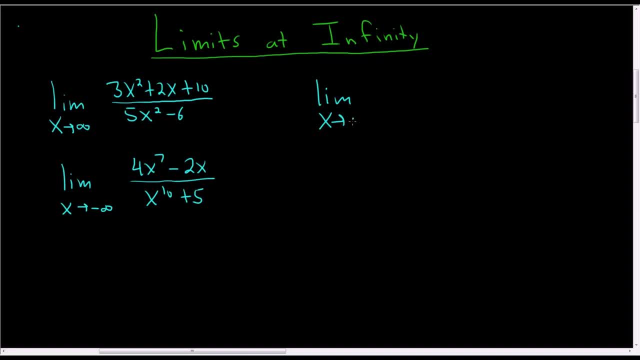 Over here we'll look at the limit as x approaches infinity. Just making them up, We can do this: 3x plus 2x to the fourth plus 5.. And then one more. Let's look at the limit, as x approaches infinity, of about x to the tenth plus 5 over x to the ninth minus 1.. So in this, 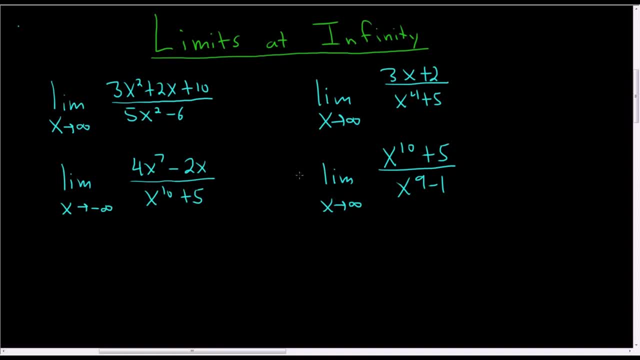 video. I'm not going to show any work, I'm just going to show you some tricks to get the answers. So in this first limit we're going to look at the limit as x approaches infinity. So in this first limit we have a polynomial over a polynomial. In fact, in all of the limits we have a polynomial over a polynomial. 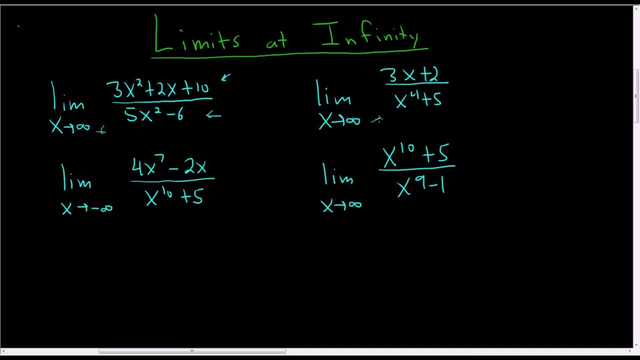 And x is approaching infinity in this case. infinity in this case, and infinity in this case. In this case, negative infinity, no big deal. The degree here- let me use a different color- the degree here in the denominator is 2.. 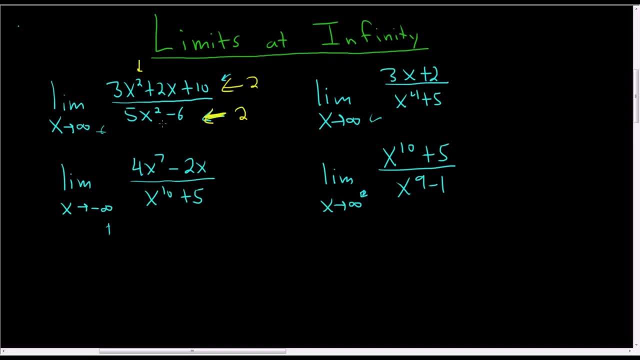 The degree in the numerator is 2, right, It's the biggest exponent. When that happens, when they're the same number, the answer is the ratio of the leading coefficient. So this is equal to. I'm going to squeeze in the equal sign: 3 over 5, equal to 3 over 5.. 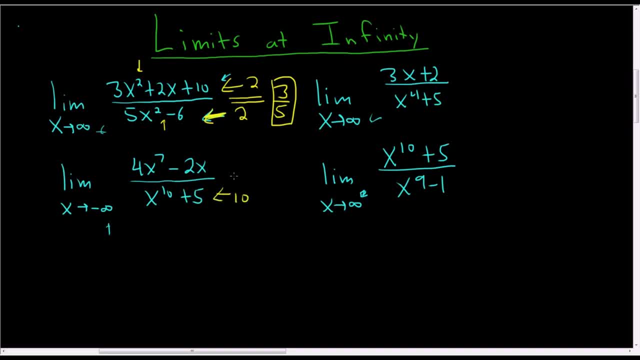 Over here, the degree in the denominator is 10.. The degree in the numerator is 7.. When that happens, the answer is 0.. Over here again, bigger on the bottom, it's 4.. Here it's 1, so the answer is 0.. 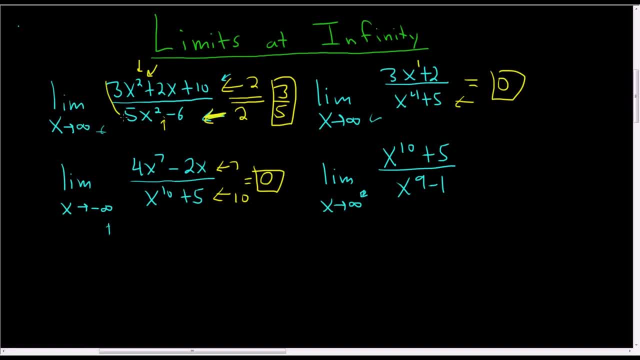 So if the degrees are the same, it's just this fraction 3 over 5.. If it's bigger on the bottom, it's 0.. Bigger on the bottom, it's 0.. If it's bigger on the top, you have to think a little bit. 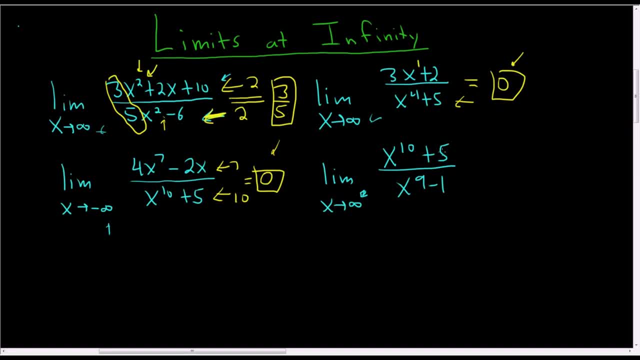 Well, first of all, x is approaching infinity, so who cares about the 5 and the negative 1?? So this is really. this is really bad. here We're waving hands. This is not showing any work. It's really this which is really x. 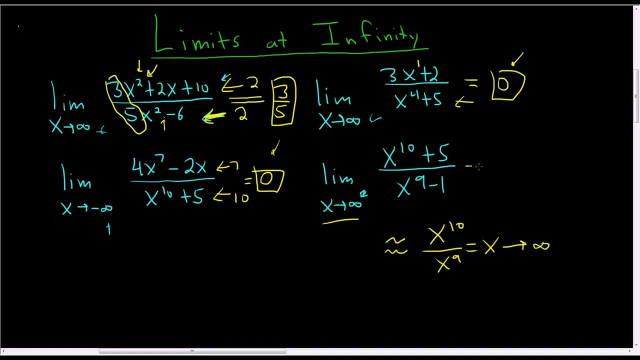 And as x approaches infinity, this approaches infinity as well, So this is equal to infinity. So just a really, really quick video to show you how to compute some limits at infinity without showing any work. So again, if the degrees are the same, so 2,, 2,. 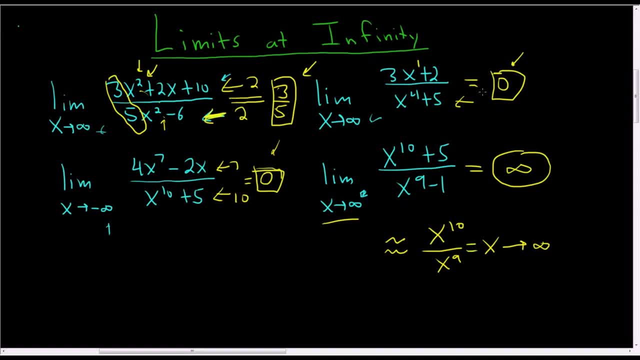 you get 3 over 5.. If it's bigger on the bottom, you get 0.. And if it's bigger up top, just do something like this: Ignore the numbers and just look at these guys here, Divide them, you get x. As x approaches infinity, you get infinity. 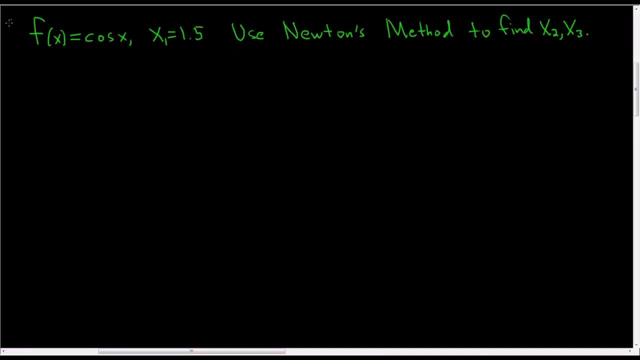 I hope this helps. So we have f of x equal to cosine x x 1 is equal to 1.5. And we want to use Newton's method to find x sub 2 and x sub 3.. So solution: The first thing we should do is write down the formula for Newton's method. 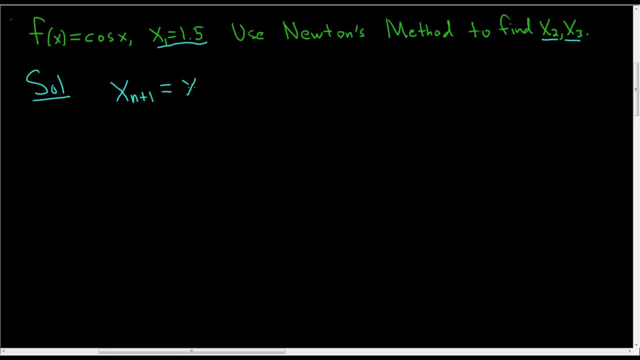 So x sub n plus 1 is equal to x sub n minus f of x sub n divided by the derivative of f evaluated at x sub n. Now the way I remember the formula is, the derivative just always goes in the bottom. It's pretty easy not to forget the minus and this is pretty easy to memorize. 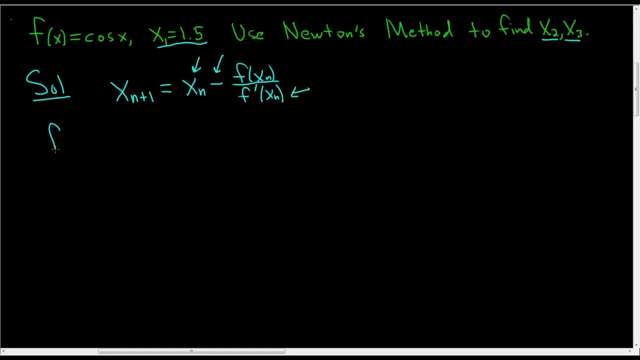 But just remember, the derivative goes on the bottom, All right. So in this problem f of x sub n is just the cosine of x sub n. Just replace x with x sub n And the derivative of cosine is negative sine x. So here it's: f prime of x sub n is negative sine of x sub n. 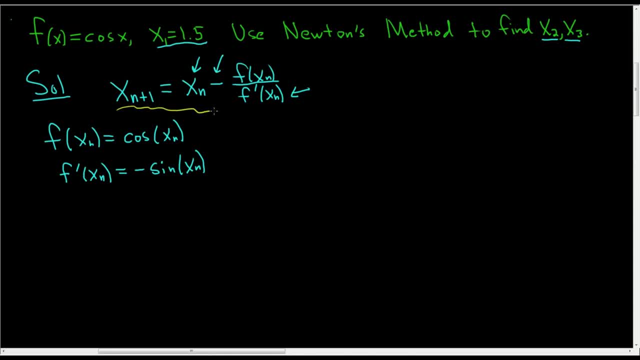 And that's it. Now we're just going to plug everything back into our formula here. So x sub n plus 1. This is equal to x sub n minus f of x sub n. That's a lot to say. That's just the cosine function. 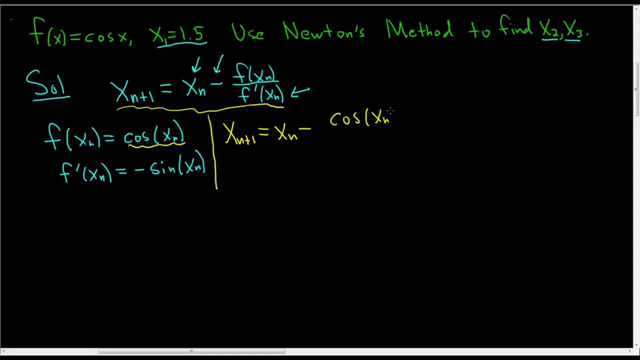 So cosine x sub n divided by the derivative. So this: So negative sine of x sub n. We have two negatives, so we're going to get a positive. So x sub n plus 1 is equal to x sub n plus cosine x sub n over sine x sub n. 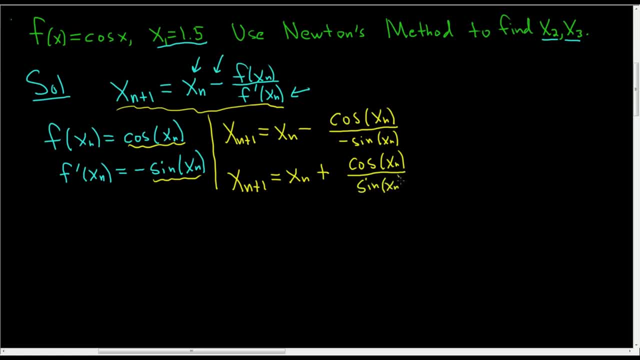 Sine of x, sub n. All right, We're ready to go. We have the formula. All we have to do now is find x2 and x3.. So x2 is equal to Well. here, n is equal to 1.. 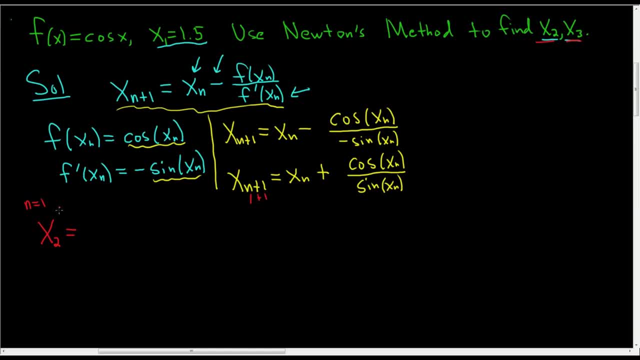 Right, And then 1 plus 1 is 2.. That's how we get x2.. So here n is 1.. So we get x1 plus cosine Of x1 over sine of x1.. And x1 was 1.5.. 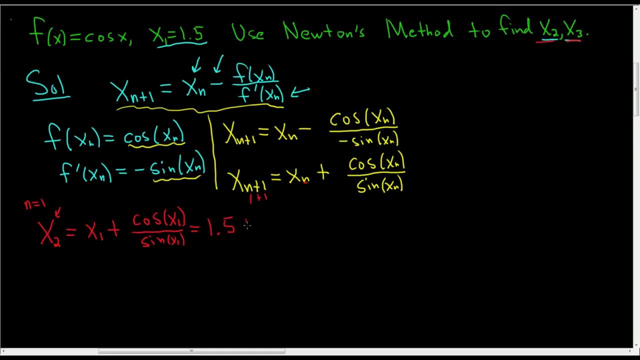 So this is 1.5 plus cosine, 1.5 over sine of 1.5.. Right, Just replacing all the x1s with 1.5.. If you put this in your calculator, make sure it's in radians. 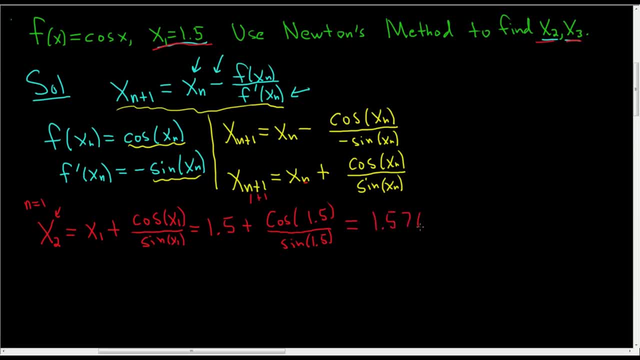 You end up with 1.5.. You end up with 1.5709.. I'm using four decimal places throughout this video. Now we have x2.. So that's x2.. So now we can find x3.. So x3 is 1.5709. 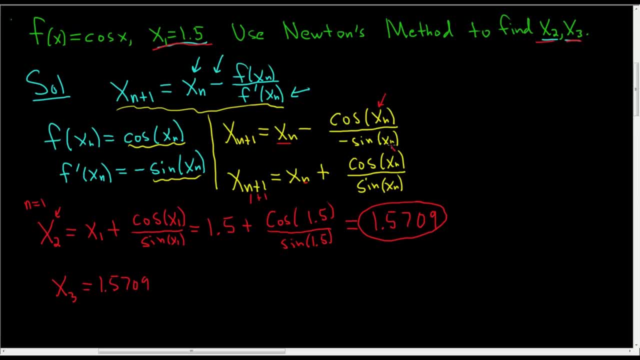 Right, Just plug it back in here. Right, You plug this. This is x2.. You plug it back into the formula Plus cosine 1.5.. 709 over sine of 1.5709.. And if you put this in your calculator, make sure it's in radians. 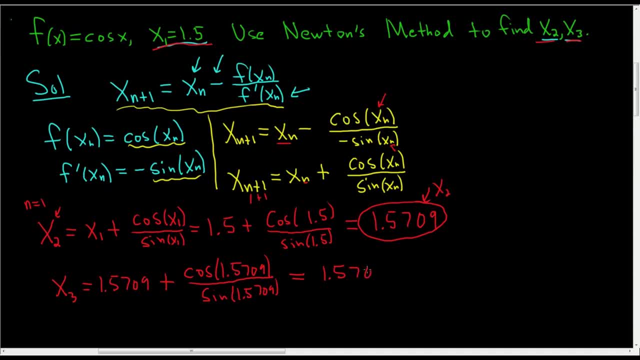 You get 1.5708.. And that's it. That's x sub 3.. So, to recap, whenever you're using Newton's method, just write this down Right, Take your derivative- We did that here- And clean it up. 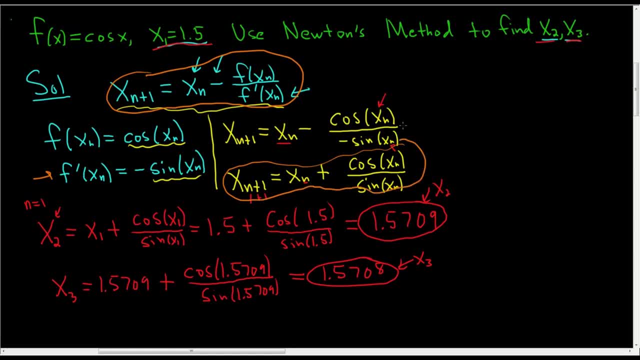 And so here's our formula: We have x1. So you just replace x sub n with x1. And work it out. We did that here. There's x sub 2. We replaced all the x1s with 1.5s. 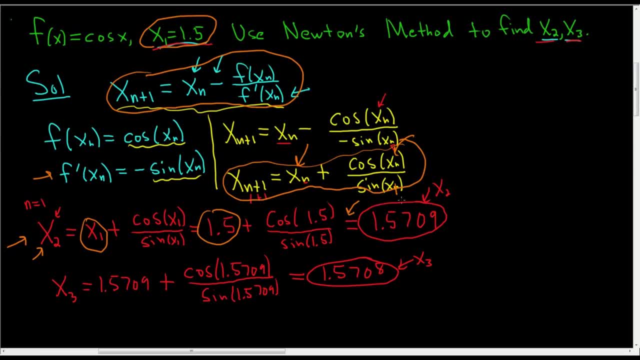 Put it in your calculator. Make sure you're in radians, Otherwise you'll get a different answer. And here's x sub 2.. Once you have x sub 2, you plug it back into the formula. So here's x sub 2.. 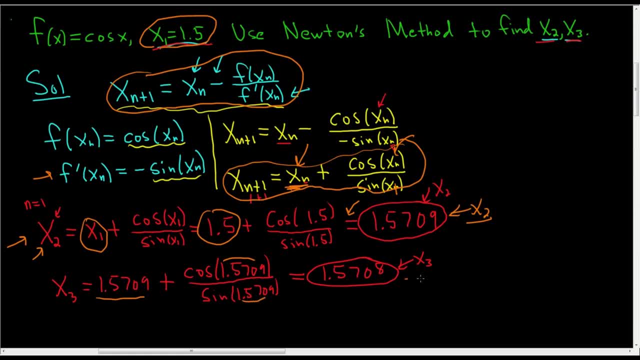 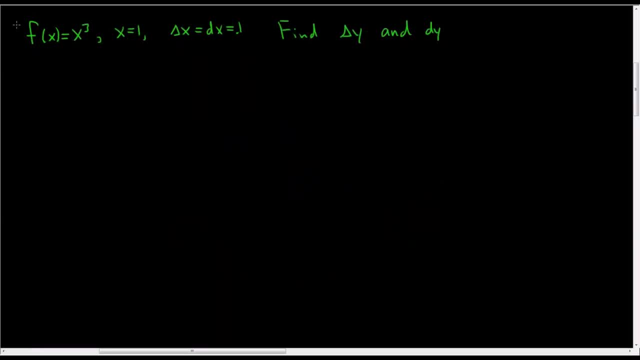 x sub 2.. x sub 2.. And that will give you x sub 3.. Really, really easy. It's just about knowing the formula and being careful. I hope this helps. We have f of x equals x cubed. 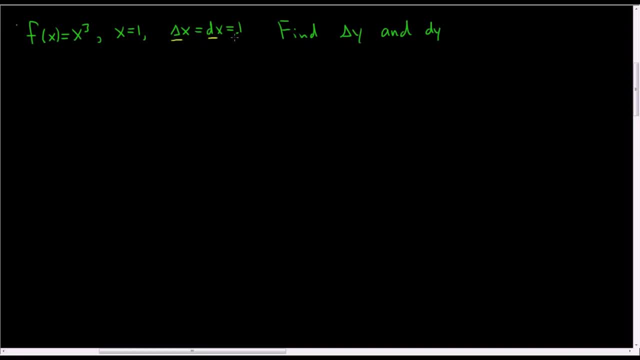 x equals 1.. And delta x and dx are both equal to 0.1.. And we're being asked to find delta y and dy as well. So solution: This is a really easy problem. All we have to do is use two formulas. 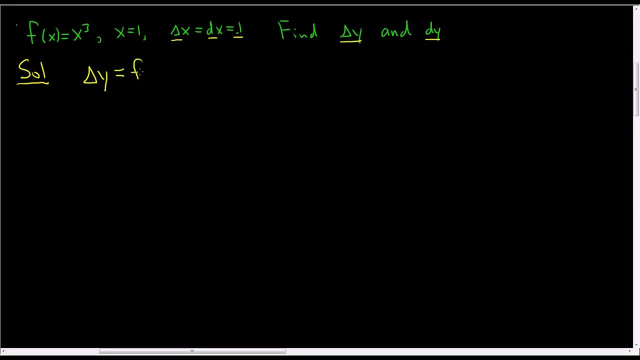 So delta y is equal to f of x Plus delta x Minus f of x. So that's the formula we'll use to find delta y, And then dy is equal to f prime of x- dx. Okay, let's do it. 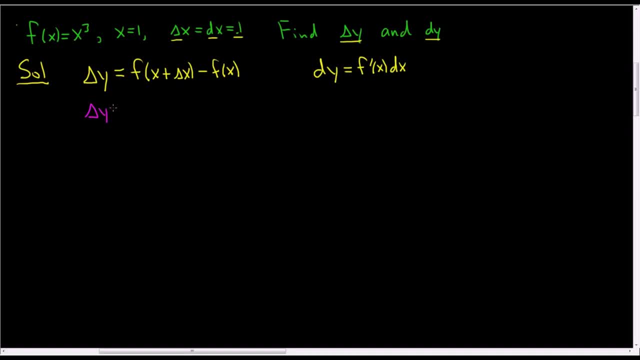 Let's do this problem. So delta y is equal to f of well x, x is equal to 1.. So it's 1. Plus delta x, But that's 0.1.. So 1 plus 0.1.. 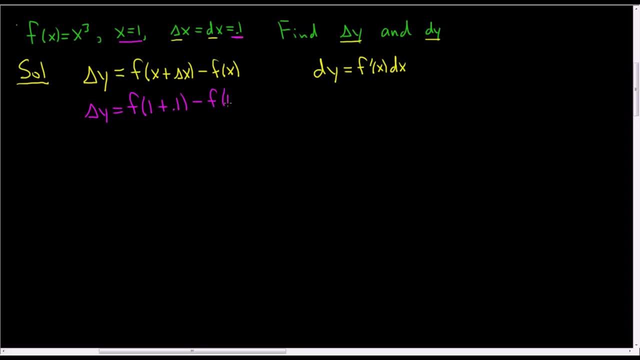 Minus f of x. But again, x is 1.. So this is equal to f of. well, 1 plus 0.1 is just 1.1. Minus f of 1.. To figure out what f of 1.1 is, just evaluate f at 1.1.. 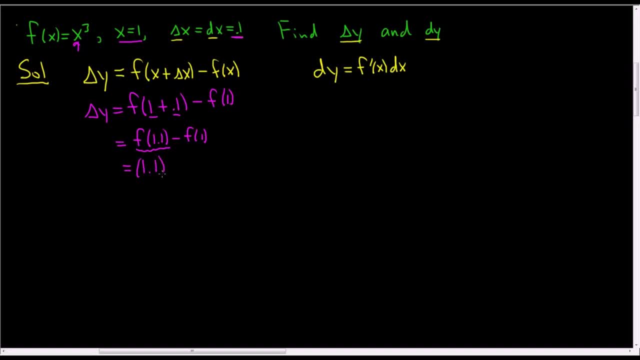 So you get 1.1.. So this is equal to 0.331, if you just plug it into your calculator. So super, super easy problem. It's all about knowing the formula. Okay, Let's do the other one. 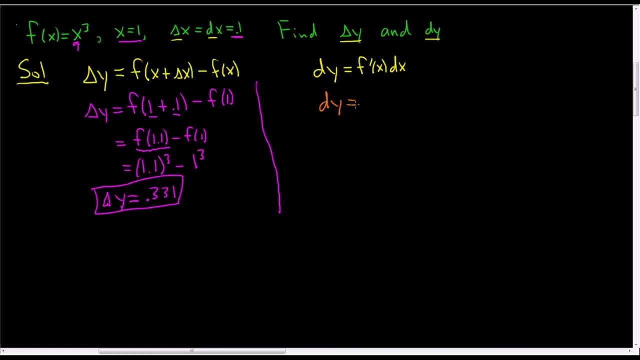 So dy is equal to f. prime of x. Well, the derivative of x cubed is 3x squared, And then we have the dx: Okay, So this is 3x squared. So this is 3x squared, And then we have the dx. 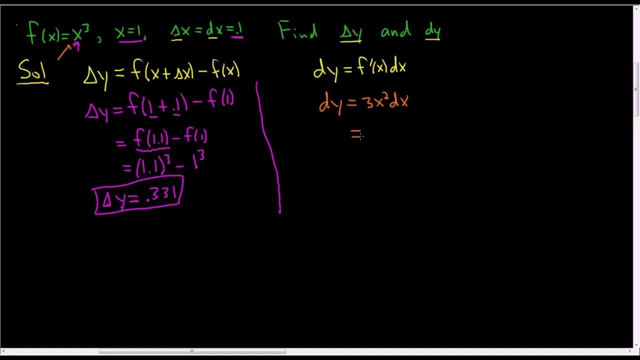 So dy is equal to f, prime of x. So this is 3x, And then we have the dx, So this is 3x squared. This is equal to well, x is equal to 1, so this is 3 times 1 squared and dx is 0.1,. 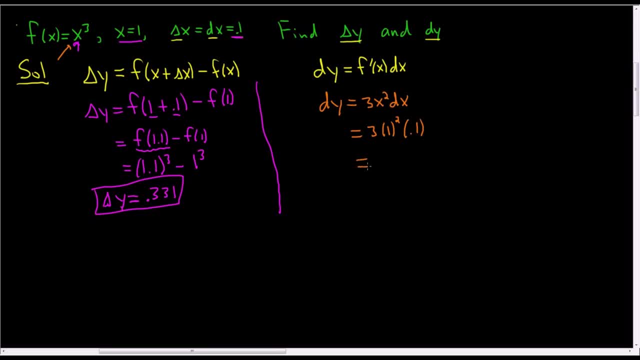 so times 0.1. This is equal to 0.300, so there is dy. Why am I using three decimals? The original problem: I didn't write it down, but it wanted us to use three decimals. So again, it's all about knowing these two formulas. 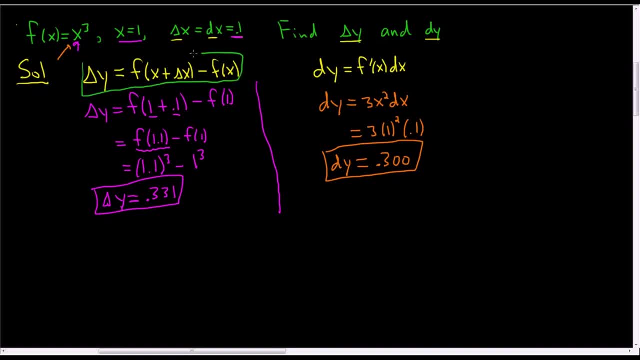 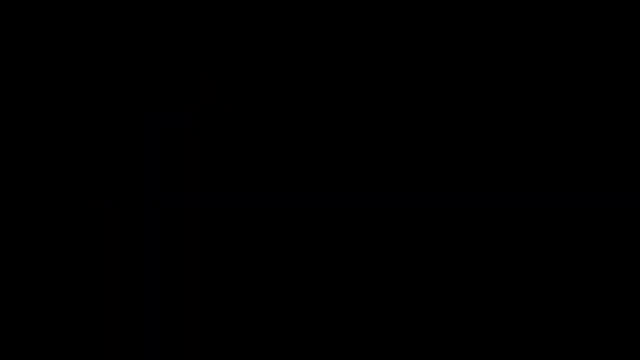 All right. so this formula here gives you delta y and this formula here gives you dy. Very, very easy stuff. Hi everyone, In this video we're going to introduce the notion of integration. So here is the idea. So we can start with a question. 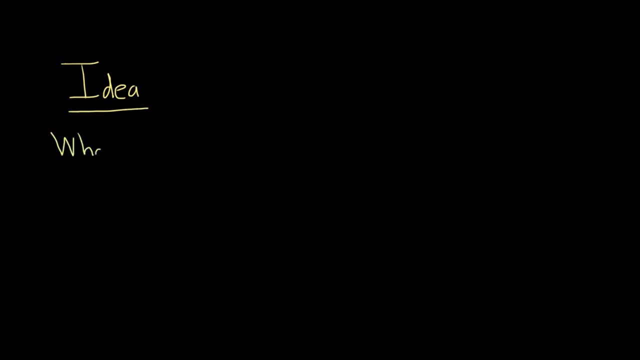 The question is: what is a function Whose derivative is 2x? So what is a function whose derivative is 2x? So one possible example would be f of x, and I'll use a capital letter, for f equals x squared, because if you take the derivative, 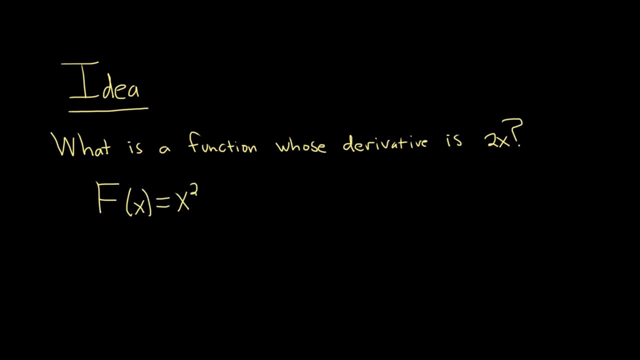 of x squared, you get 2x via the power rule. You might say: well, what about big F of x equals x squared plus 1? That is also a function whose derivative is 2x. Likewise, we can look at: big F of x equals x squared plus 3.. 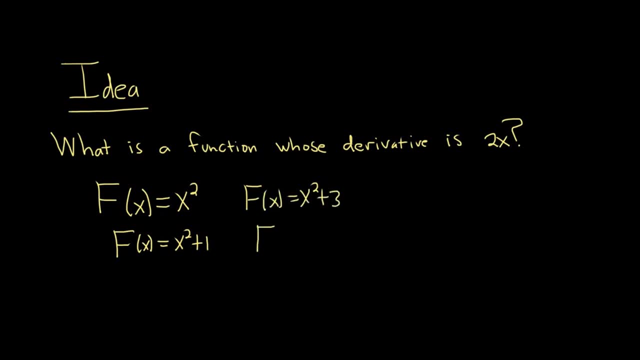 In fact, we can take any number right. We can look at big F of x. We can look at big F of x: equals x squared plus c, where c here is a constant. So there are infinitely many functions, right? There are infinitely many such functions whose derivative is 2x. 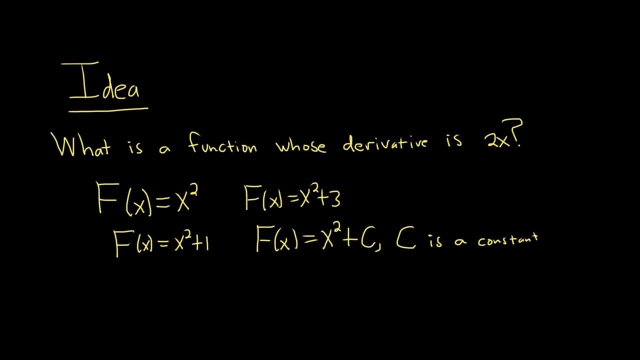 So there's infinitely many functions where you can take the derivative and you get 2x. So each of these functions, so each big F of x, each one of these is called, it has a name, it has a special name. 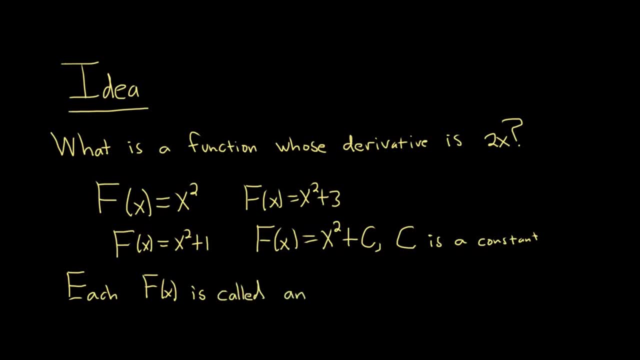 It's called an antiderivative of big F. So it's called an antiderivative. It's a very delicate thing, mathematics of big F. So 2x has infinitely many antiderivatives. Let us formally define it. 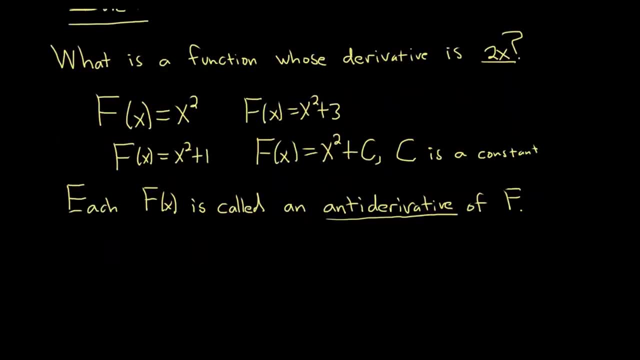 Let us formally define it. Let us formally define it, Let us formally define this idea of antiderivative in a formal, precise and rigorous way. So definition, And, by the way, this is the beginning of what people usually call integral calculus. 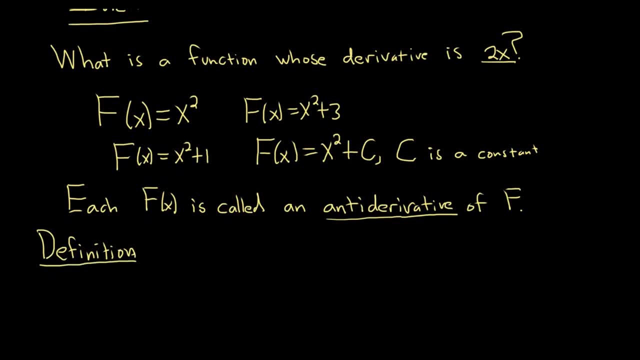 Back in the day people would go to school. they would take two courses. They would take differential calculus that was like calculus 1, and they would take integral calculus that was like calculus 2.. So we say We say big F. We say big F is an antiderivative. 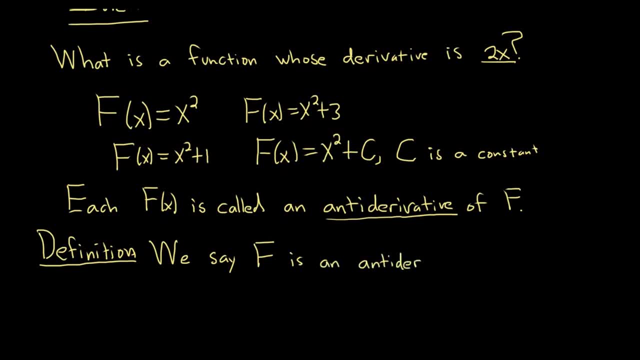 So antiderivative. So big F is an antiderivative of little f? If well, let's just think about it. What does it mean? Well, if you take the derivative of big F, you should get little f, right? 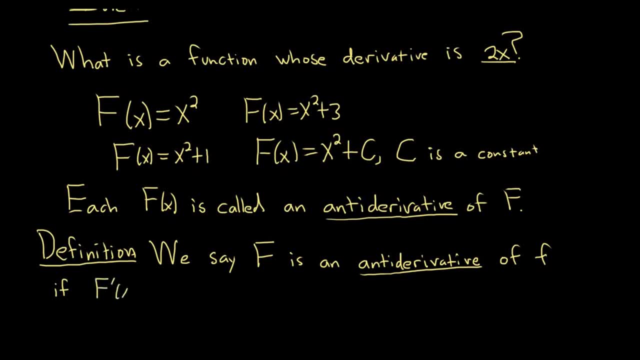 And that's precisely what we have in our example above right. The derivative of all of these big F's is equal to little f. This could be our little f here. right, Little f could be our 2x. So the derivative of big F in any case is equal to little f. 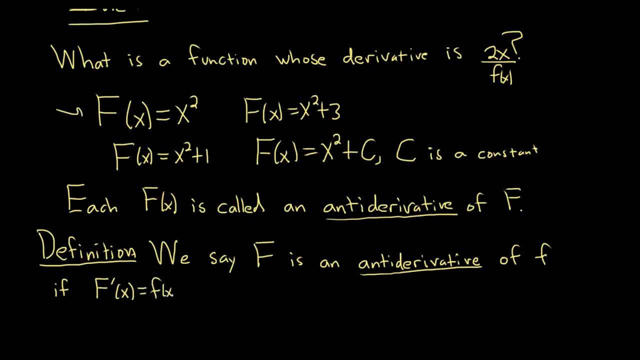 So this should be equal to little f, And this must be true for all x in some interval. i So for all x. So this must be true for all x in some interval, i So in some interval i. So we're going backwards. 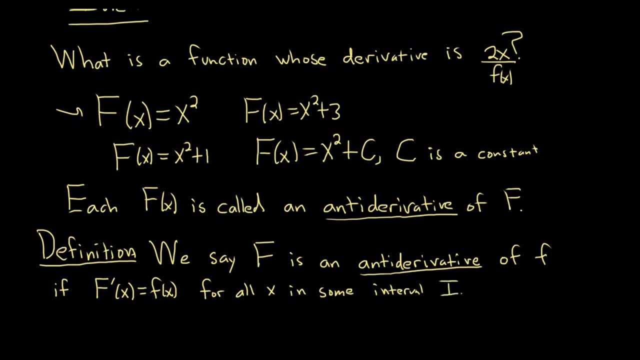 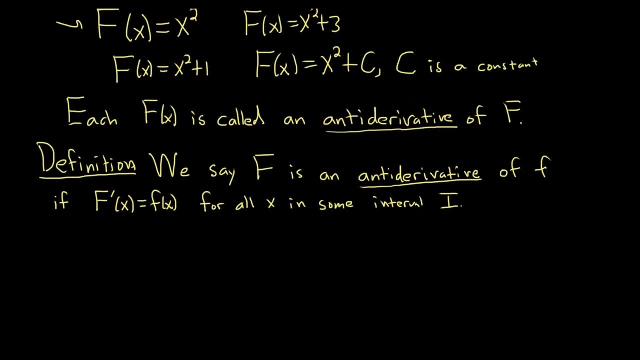 Instead of computing derivatives, we're computing antiderivatives. So instead of differentiating, we are anti-differentiating. This particular case up here, let me circle it in green, so you see it, This one is special, This one has a name. 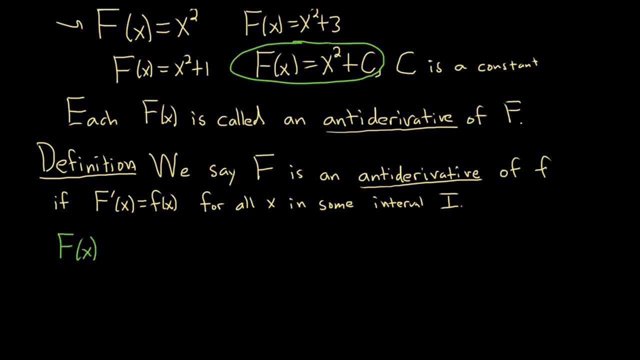 So in the case where we have big F, big F of x equal to x squared plus c in our example above, this one was special. This one is called the general, the general antiderivative of little f of x equals 2x. 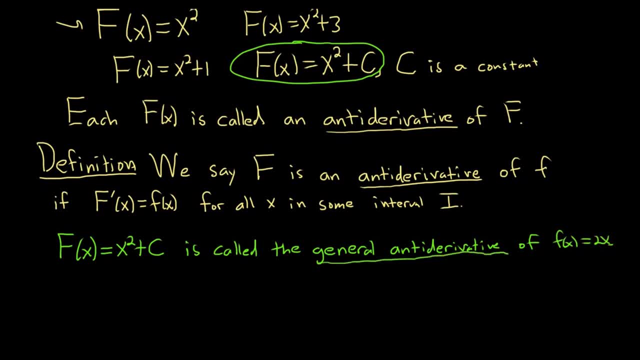 So basically, it's going to be the general antiderivative whenever you add the plus c. okay, So when you add the plus c, it's called the general antiderivative because it encompasses all of the antiderivatives, right? 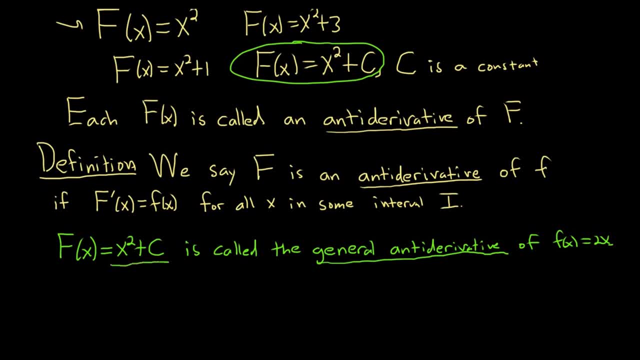 There's infinitely many functions here. right, It's an infinite family of functions. The process of finding an antiderivative is called anti-differentiation or indefinite integration, So let me go ahead and write this down. Okay, I'm going to write that down. 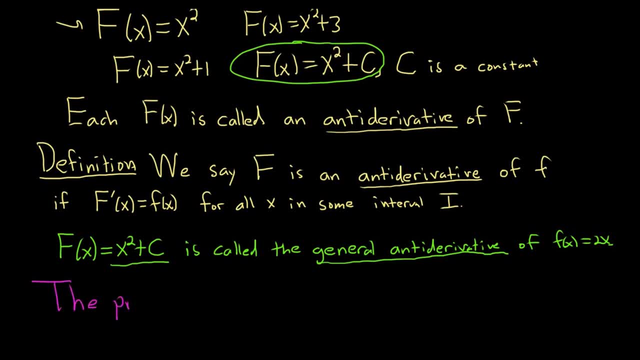 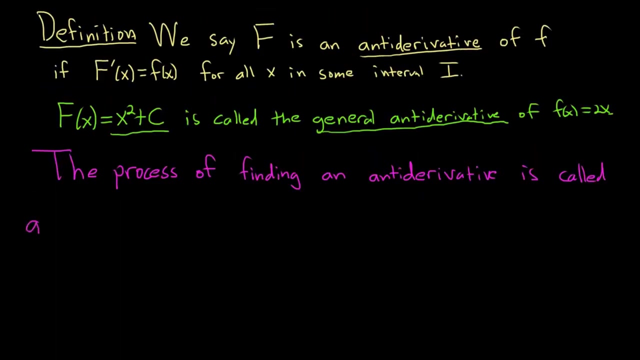 We have time. So the process, the process of finding an antiderivative, so the process of finding an antiderivative, anti-derivative is called, it's called anti-differentiation or indefinite integration, So it's called anti-differentiation. 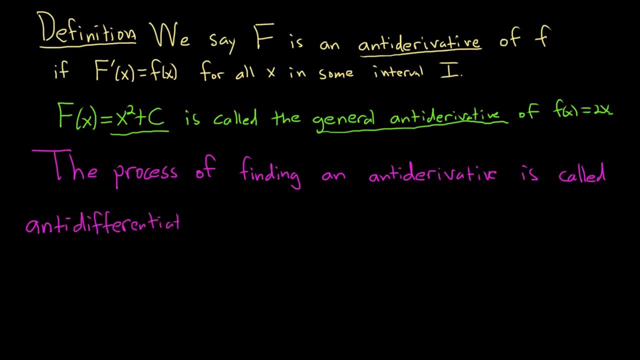 differentiation- let me underline this- anti-differentiation, or indefinite integration. You might be wondering: why is it indefinite? Well, definite is actually something else: Definite integration. we'll talk about that later. Definite integration is a little bit different, so. 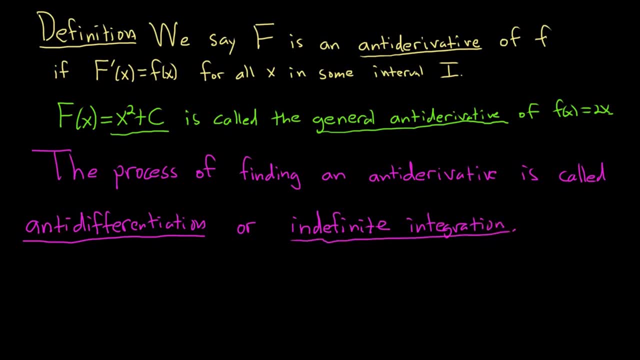 Basically definite integration is going to be used in some cases to find the area under curves. C has a name as well. So our big C in all of this, so big C, this is called the constant of integration. so constant, constant of integration. 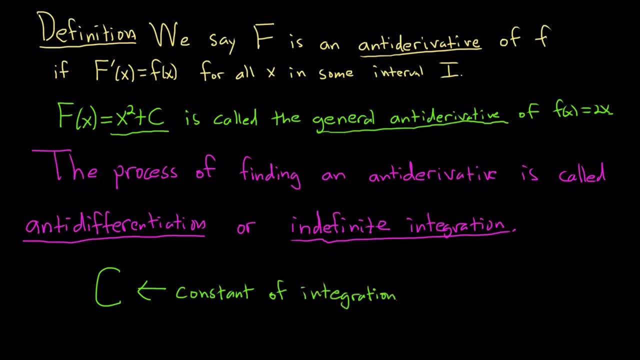 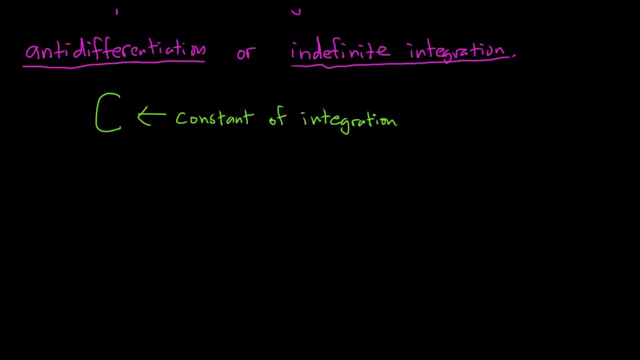 It's called the constant of integration. Let's talk about the notation. So what is the notation that we use when we study anti-differentiation? So notation, notation. So the notation is key, the notation is key. So we write a symbol that looks like this: 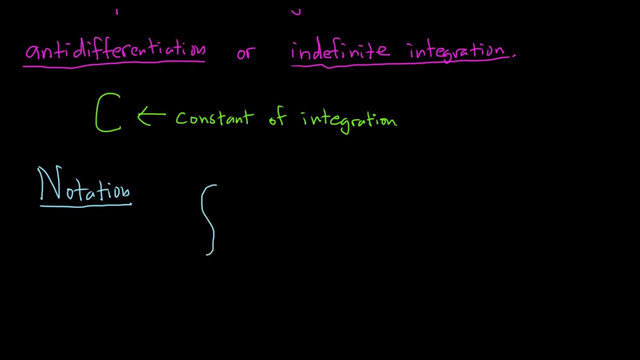 So this is a really interesting symbol. It's called the integration symbol. It kind of looks like someone took the letter S and then they stretched it right And the thing is the word sum starts with the letter S. so It turns out definite integrals can be written as limits of sums. 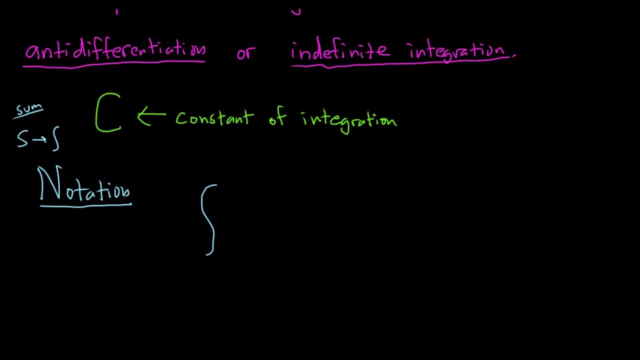 So, in other words, a definite integral can be written as an infinite sum, right? So it's like they took the letter S and they made it longer, Maybe because of the word sum. I'm not positive, but I heard that once, so it might be true. 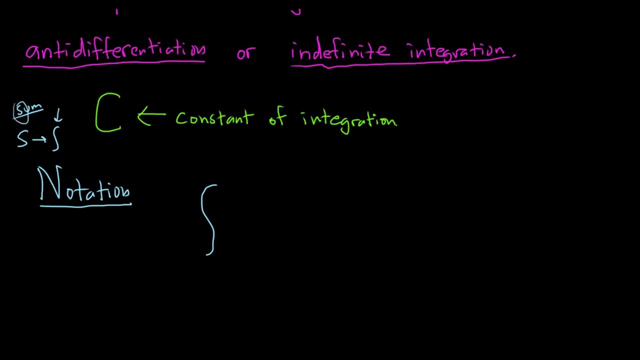 So it's like an elongated S, because definite integrals can be written as infinite sums. Okay, So this is the integral symbol. We have a function here, f of x, and we have this symbol here- dx, and I'll explain what this means in a minute. 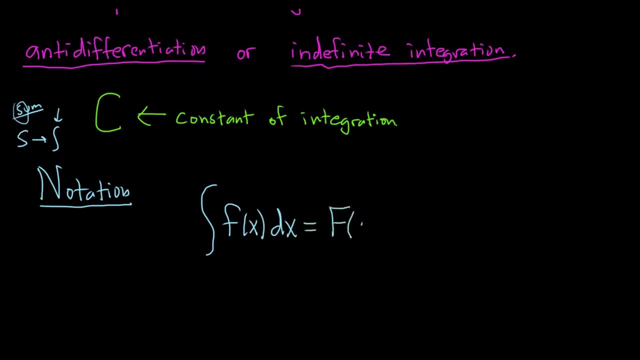 And we'll say: this is equal to big F of x, big F of x plus capital C. Okay, So what does everything mean and what is going on? So this piece here, this is called the integrand, So integrand. 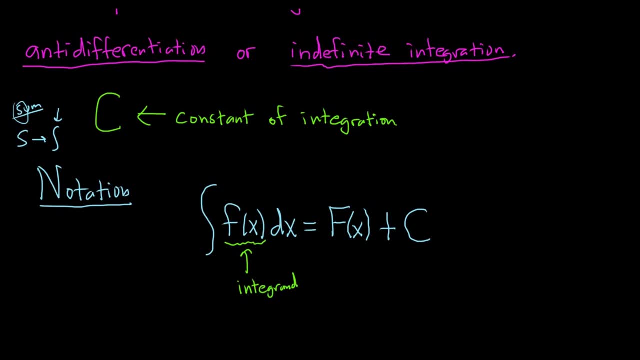 So when someone says: oh yeah, my integrand is, you know, really scary, they're talking about what you actually have to integrate. This dx here it tells us what the variable that we are integrating with respect to So this means- in this case it means x- is the variable. 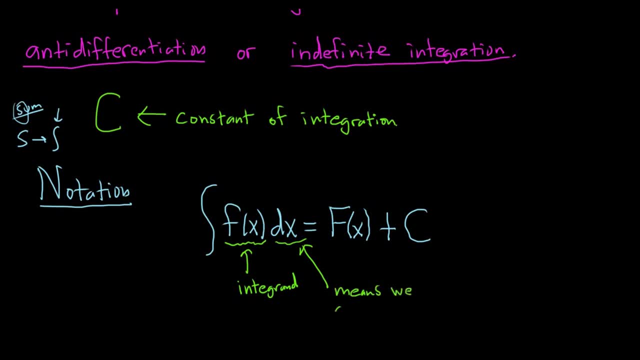 So it means we are integrating right because there could be more than one variable. We are integrating with w means, with r means respect to, With respect to Wrt, with respect to x In calculus three or the study of the calculus of multivariable functions. 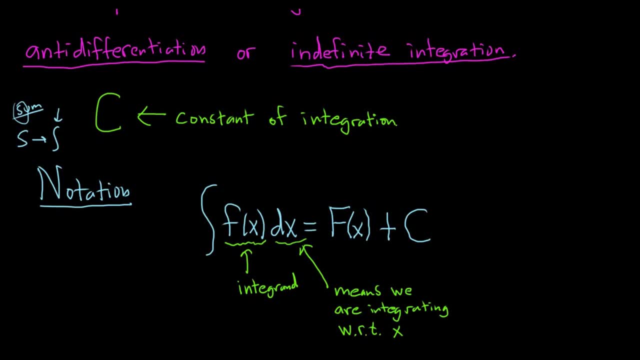 we have like integrals, where we have like dx, dy and even dz, So we integrate multiple times with respect to different variables. So it's important to have this notation Here: big F, this is an antiderivative. An antiderivative. 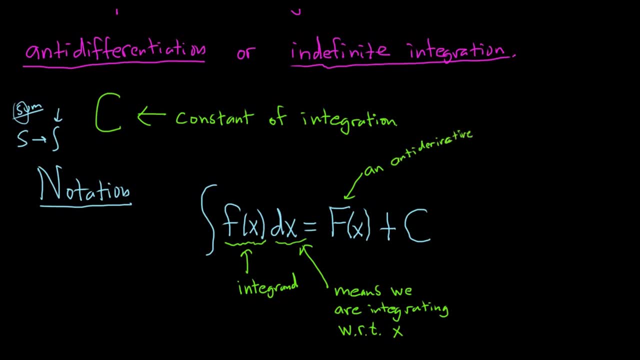 Derivative- I forgot how to spell Antiderivative- And big C is our constant of integration, so constant of integration. So when we add the C to the big F, we get the general antiderivative right. This whole thing here is the general antiderivative. 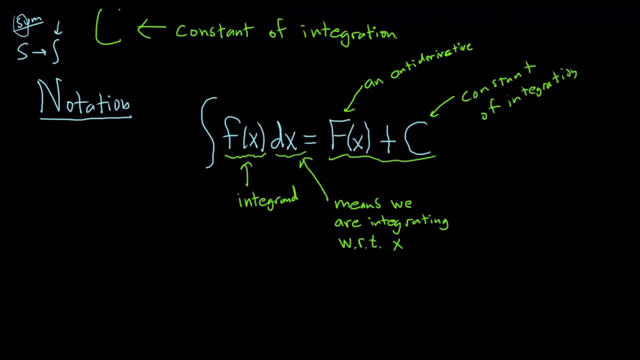 Notice something: If we differentiate both sides, so note: if we differentiate both sides, So if we differentiate both sides, What happens when you compute d, dx of the right-hand side is big f of s plus our constant c, So this is equal to well. we would take the derivative of big F. 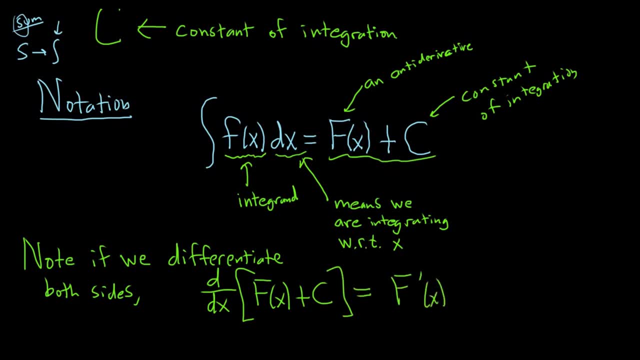 and the derivative of c is zero because c is a constant c of f. What we would do- we're taking the derivative of big F and the derivative of C is 0 because C is a constant c of f, So we're going to use big F on both sides. 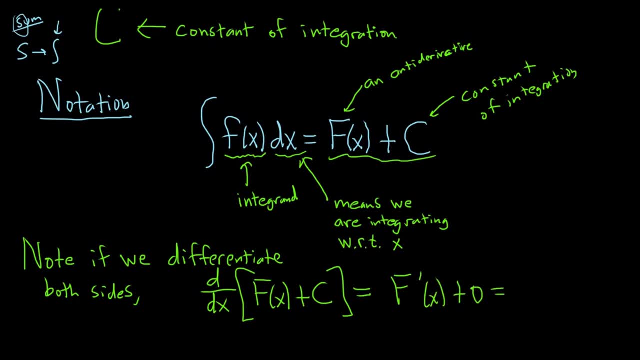 constant. Well, we know that big F is an antiderivative for little f, so this is just equal to little f, right? So it checks. You can always check your answer by taking the derivative. So you can check your answers this way. That's it. I think I'll stop this video here In the 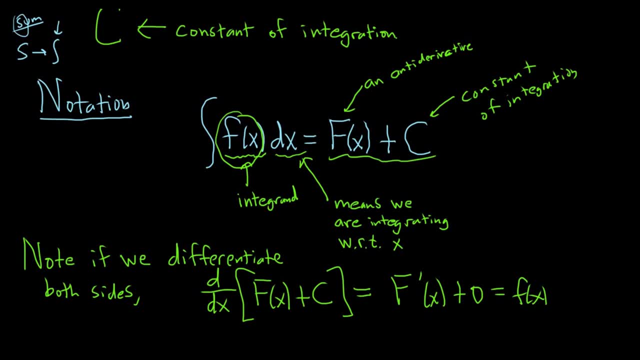 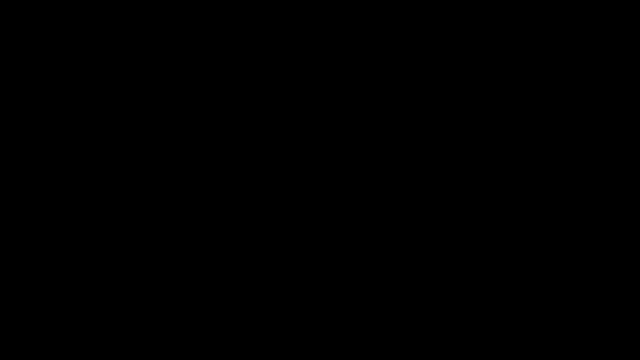 next example we'll talk about some basic integration rules. That's it, Hi everyone. In this video we're going to discuss some of the basic integration rules, So the first rule we're going to look at is a formula for the integral of zero, with respect, 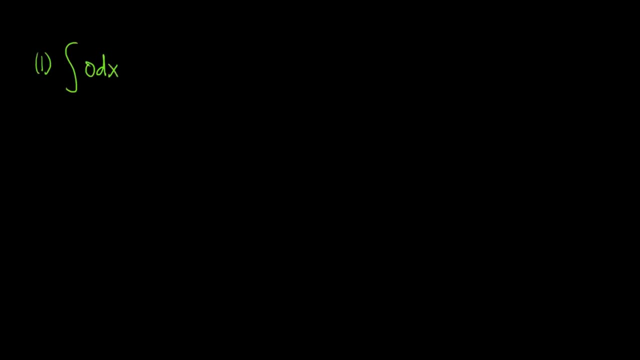 to x. So when we're trying to integrate zero with respect to x, we have to ask ourselves: what is a function whose derivative is zero right, Because we're going backwards? Well, that function would just be the constant function. Again, the reason this is is because, if you 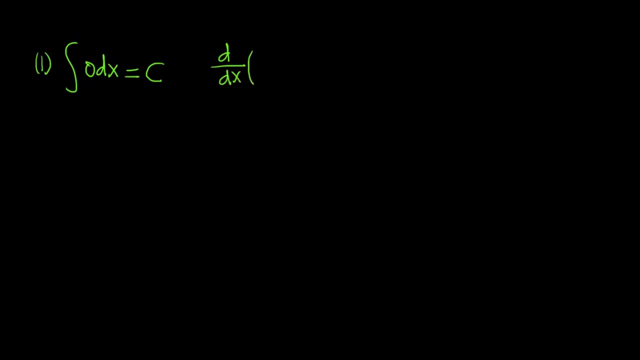 take the derivative with respect to x of a constant function: you get zero. So if you integrate zero with respect to x, you get zero. So if you integrate zero with respect to x, you get zero. So if you integrate zero with respect to x, you get zero. So if you 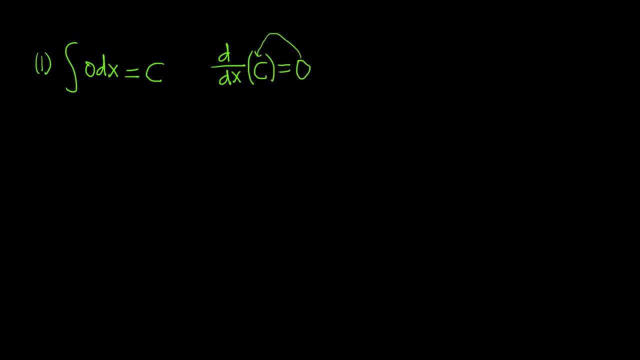 integrate zero, you should get back the constant function, right? We're anti-differentiating or integrating, So we're going backwards. The second formula is a formula for the integral of a constant, which we'll call k with respect to x. So you have to ask yourself again what. 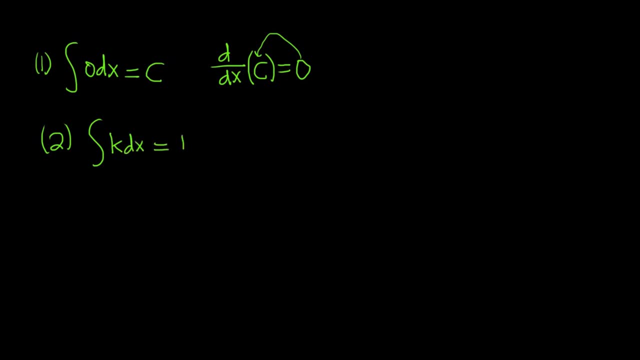 is a function whose derivative is k. Well, kx. And then we add our constant of integration, c. You could check: if you take the derivative of kx plus c, You just get k right. The derivative of kx is k and the derivative of c is zero Here. 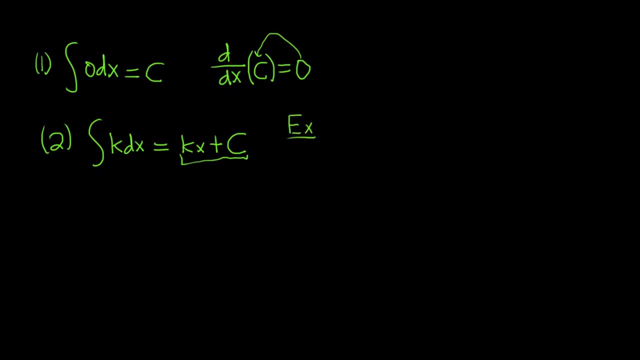 is an example. So you see how this works. Let's say we have two and we want to integrate this. Well again, what's a function whose derivative is two? Well, 2x. and then we just add a constant. I just memorize it. Whenever there's a constant, you just put an x. next. 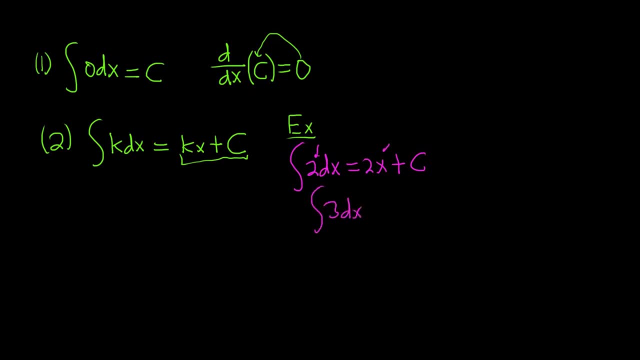 to it. For example, say we had 3dx, then you would just write that as 3x plus c. So the next rule we're going to look at is a very important one. It's called the power rule, and it basically says: if you integrate x to a power, with respect to x, this is equal. 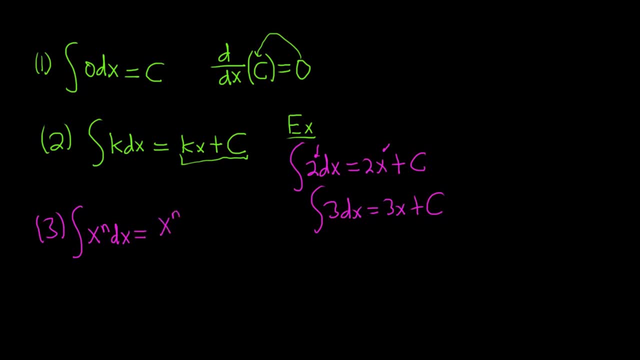 to x, And so what you do is you add one in the exponent and then you just divide by that number and then you add c, And this formula is only valid if n is not equal to negative 1.. You'll notice, if n is equal to negative 1,. 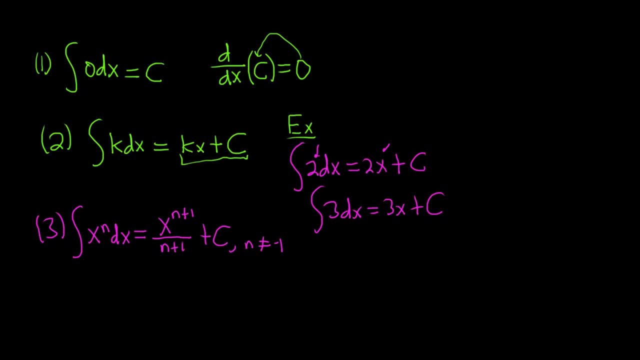 you end up dividing by zero. If you're curious- and this is a bit premature- if you have negative 1, what happens is you get the natural log of the absolute value of x plus c. But this is later Later on. we will look at this. For now we just focus on the case where n. 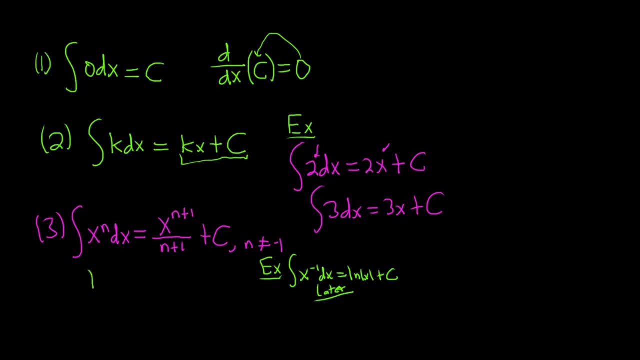 is not equal to negative 1. Let's look at an example right away. So say, we have to integrate x squared. So in this case we just simply add one to the exponent, So it'll be x to the 3. Then 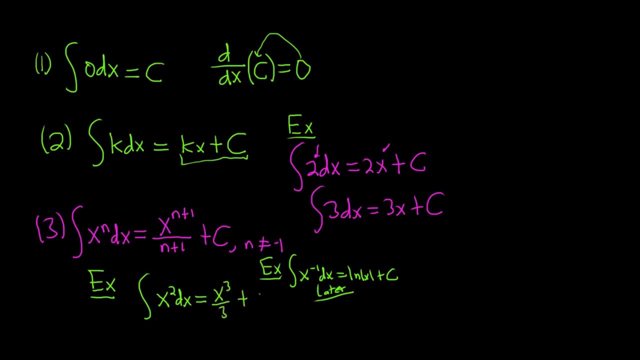 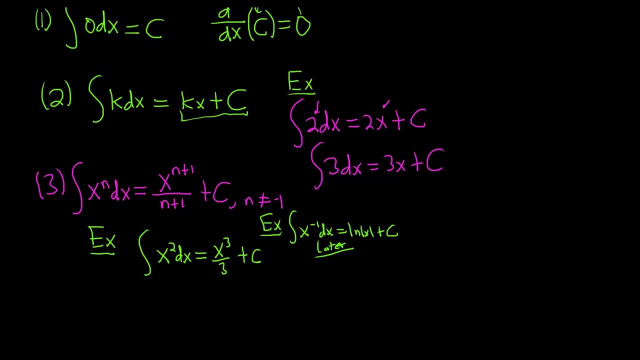 we just divide by that number again, So 3 plus c, And you can convince yourself that this works by checking your answer. If we take the derivative of this piece, we would get 3x squared right, bringing the 3 down over 3 plus 0. So let's go ahead and do that. 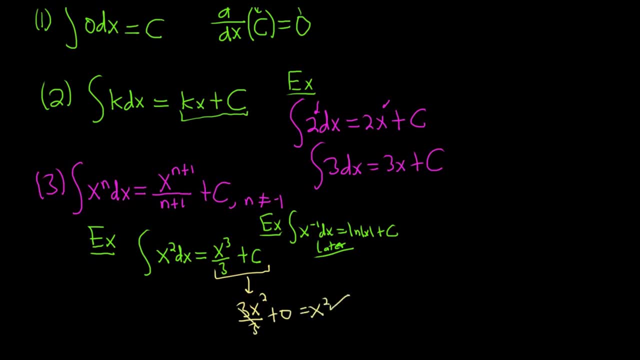 It goes away. So you just get x squared. Yep Checks Looks good. x squared. Say we had x to the 4th dx. Same thing In this case. we just add one. So 4 plus 1 is 5.. Then you 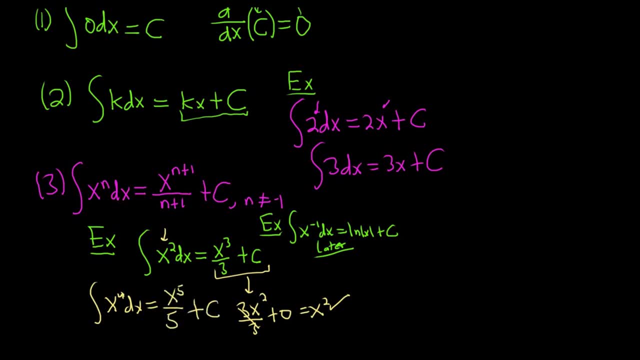 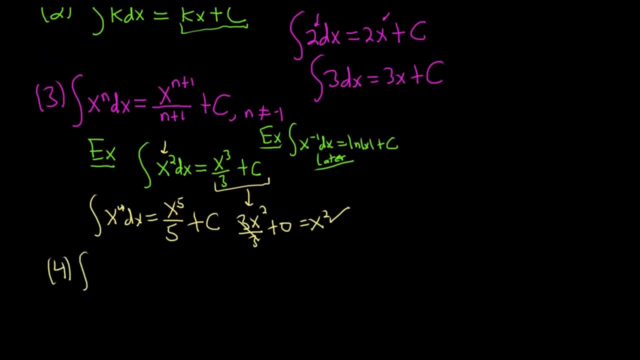 just divide by 5. And then you add your constant of integration c. The next rule says that if you have a constant times a function, you can pull the constant out. So say you have k f of x dx And that's equal to k integral f of x dx. So you're allowed to pull constants out. 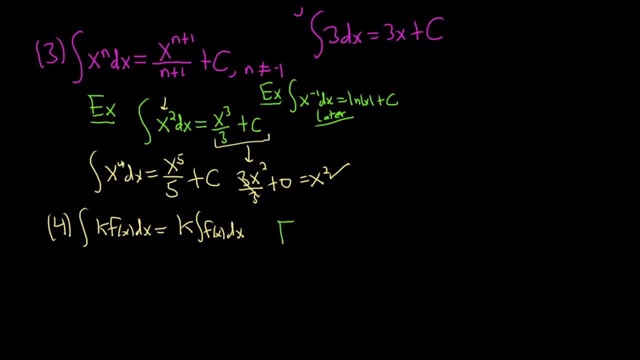 Let's do an example of this, And we'll do two examples. We'll do the same example two different ways, just to illustrate a very, very, very key point. Let's just think about something simple. I don't know How about x, cubed dx, And let's put a 4 here? Okay? So if we integrate, 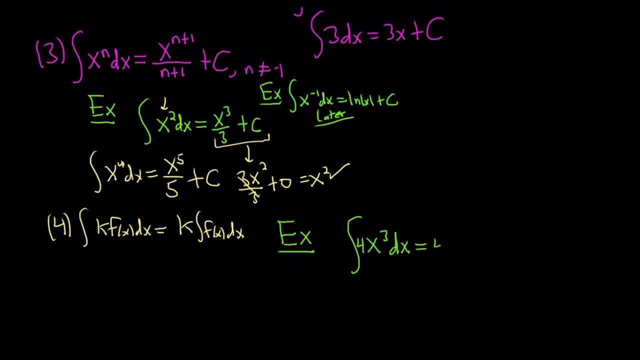 this okay. one way to do it is to pull out the constant, So we get 4.. And then we get x cubed dx, So this is equal to. so first I'm going to show you the way that people don't do it. 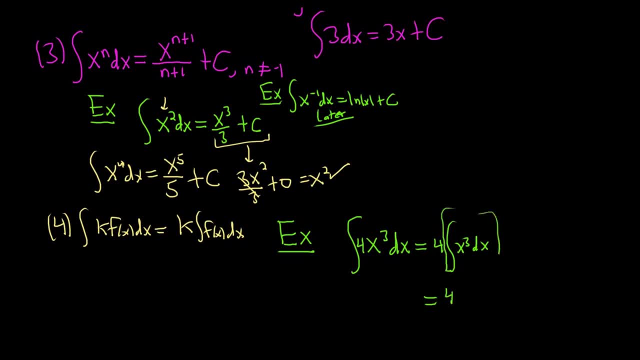 So this is 4.. And it's 4 times all of this, right, So it's 4.. And then you integrate x, cubed, So it's x to the 4 over 4, plus a constant of integration c. Right, You have parentheses. 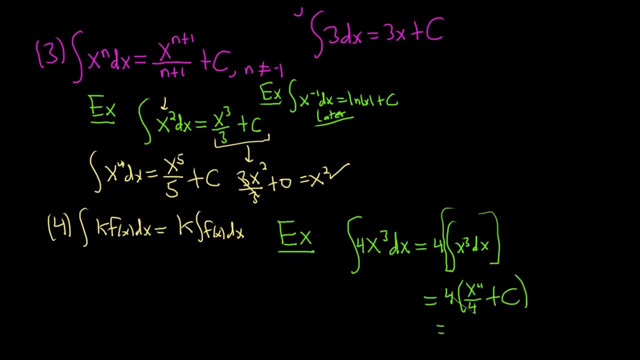 here You distribute the 4. So they can't be equal. So you have 4 times x cubed dx, So they cancel here. And then you get x to the 4th And then 4 times c is 4c, So c could. 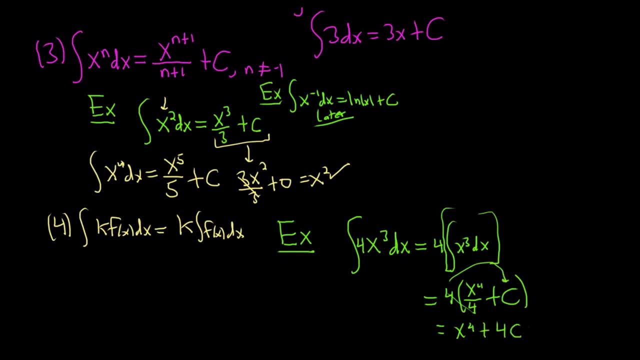 be any number. It's called an arbitrary constant. We don't know what it is. So when you multiply it by 4, it could still be any number. You don't know what it is. So what you do is you call it something else. Let's call it c1.. So that's what people don't do. So the way 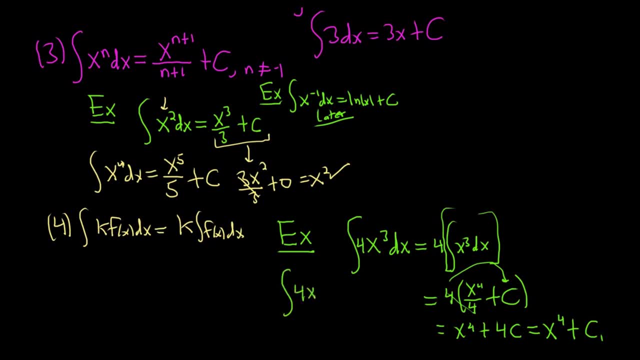 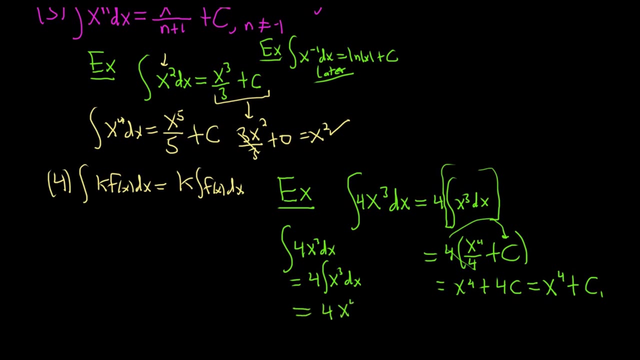 people actually do it, or one way to do it is: you pull out the 4. And then you multiply it by 4. And then you have your integral symbol dx, And you just don't worry about the parentheses, right, You just integrate the x to the 4.. So you write 4 x to the 4. 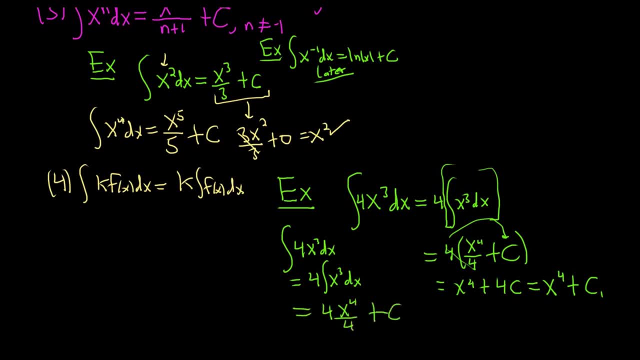 over 4.. And then you just add the c at the end, right, Because you know it's not going to matter anyways, Because when it gets multiplied by 4, it's still arbitrary. So boom, So that's how people typically do it. Another way to do it is not even pull out the 4.. So here's. 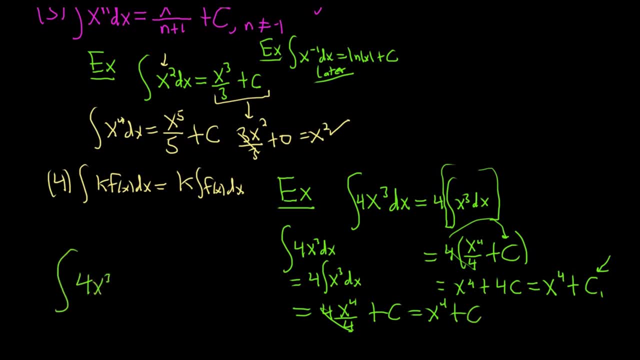 another way to do it. I'll just do it again one more time: Total overkill. This is how I do it. If I don't feel like pulling off the number, I just leave it there. It kind of just hangs out. 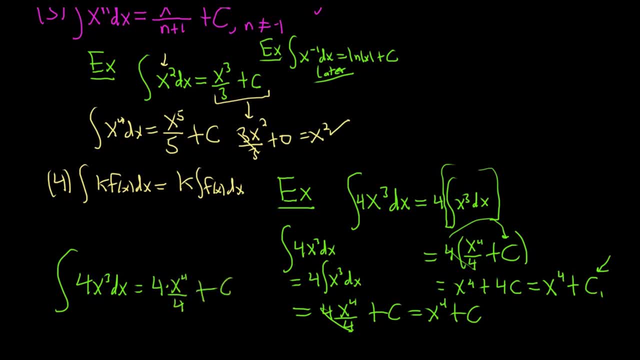 And then you just integrate this and then you just add the c, right? That's the easiest way to do it. So you just get x to the fourth plus c. That's the way I would recommend doing it when you're integrating. 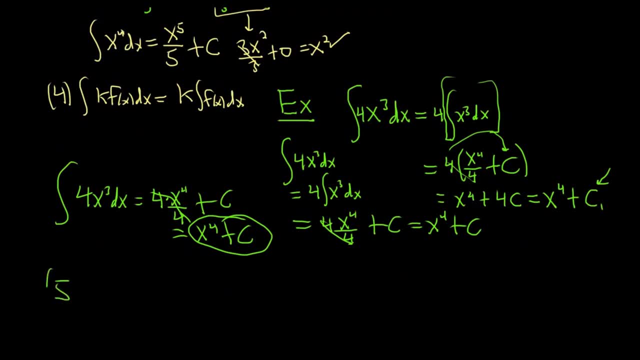 And the last formula that we have that we'll discuss in this video, tells us a formula for the sum or difference of two functions. right, So the integral of f of x plus or minus g of x. This just basically says you can integrate each one. 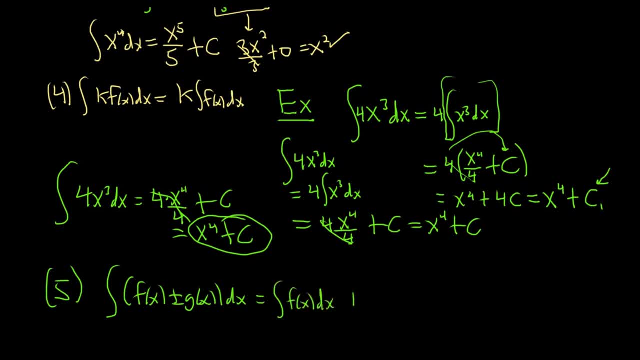 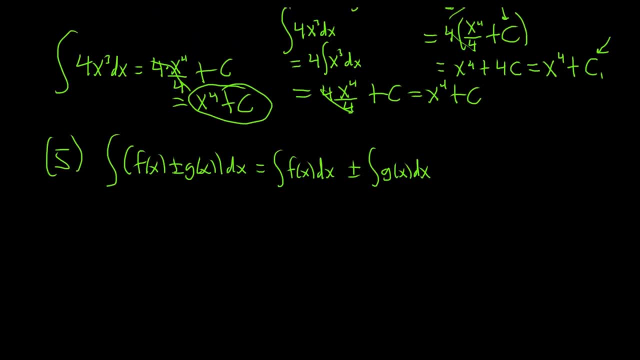 So this is the integral of f of x, plus or minus the integral of g of x, And this just basically says that you can integrate stuff term by term. Let's look at a simple example. So say, we're trying to integrate 2x plus 3 dx. 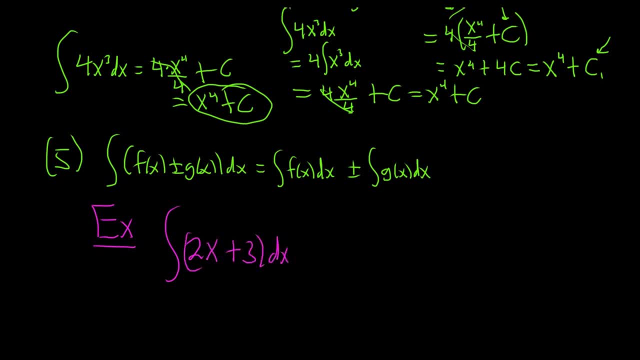 This just means you integrate each piece. You don't have to write the integral symbol twice. You can just again just integrate each piece. So there's a 1 here. So this one's going to be 2x squared over 2,. 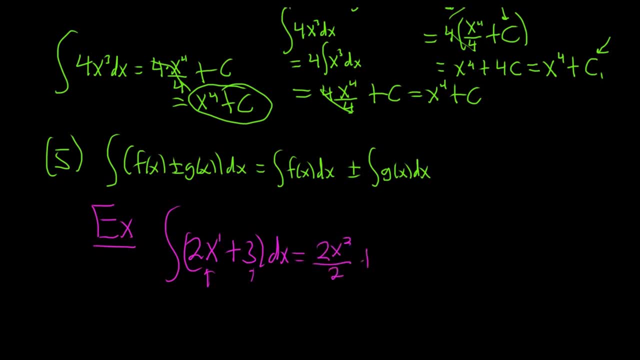 because you add 1, right, 1 plus 1 is 2, and you divide And then 3,. using the other formula gives us 3x And then we have our plus c. So this will be equal to x squared. 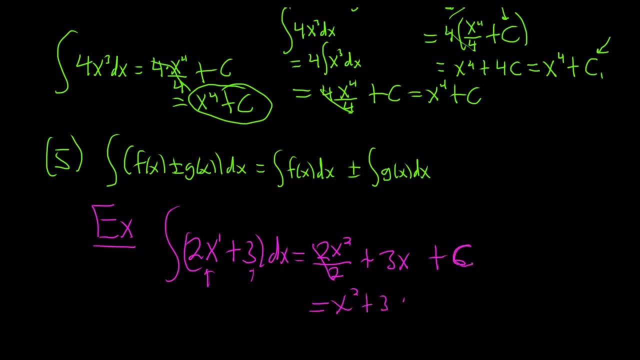 Whoops, that's a c, not a 6. x squared plus 3x plus c, And that would be the answer. Okay, so in the next video there will be more examples. That's it We're being asked to integrate. 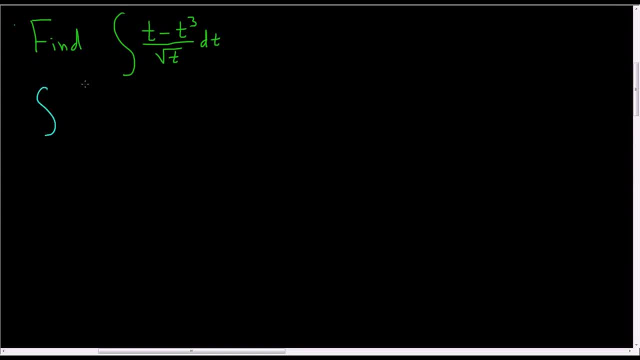 So the first thing to do here is break everything up. This will be t over the square root of t, So it's really t over. let's write it as t to the 1 half, so that we can simplify, And then minus t cubed over the square root of t. 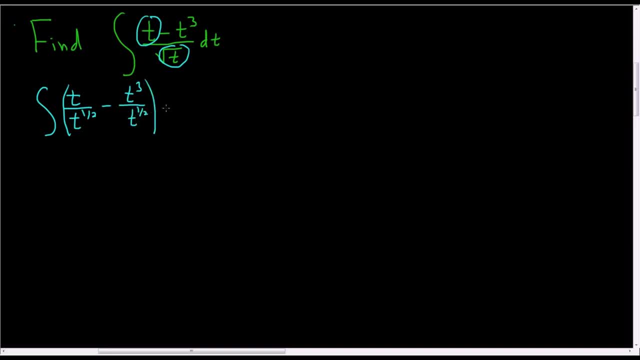 which we'll write as t to the 1 half. And all of this. we have parentheses and we have a dt. Let's keep going. So here there's a 1.. So 1 minus 1.. 1 minus 1 half is 1.. 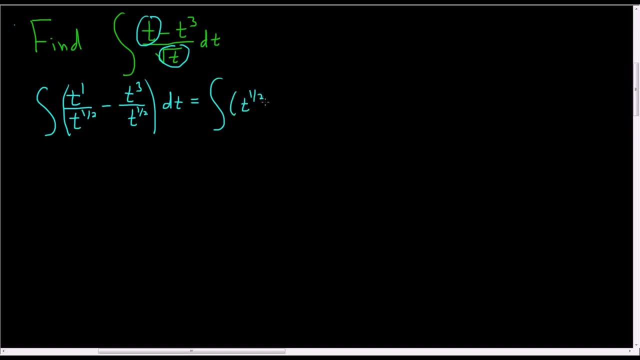 So we get t to the 1 half minus. here we have 3.. So you want to think of 3 as 6 halves. So 6 halves minus 1 half that will be 5 halves. So this is t to the 5 halves dt. 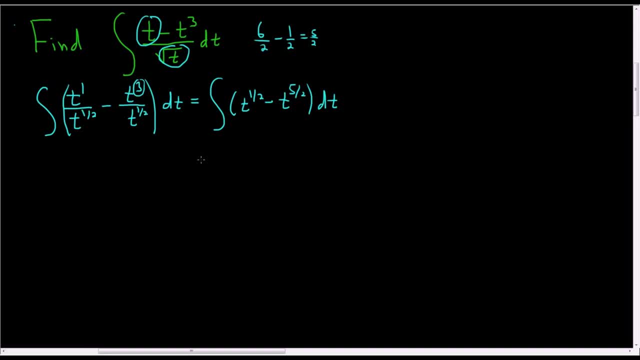 And now we're ready to integrate. We just have t to a power in both cases. So this will be t: When you add 1 to the 1 half, you get 3 halves, And then we have t to the 1 half. 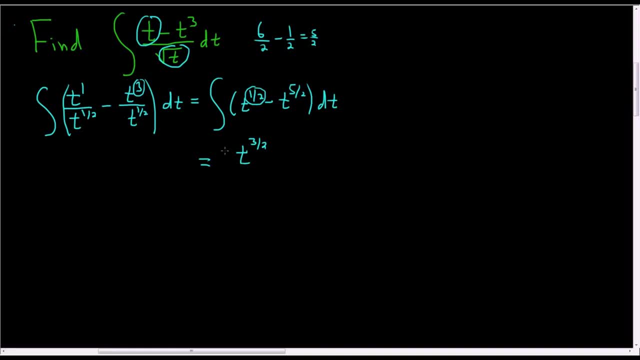 And we're supposed to divide by 3 halves. Now, instead of dividing by 3 halves, you can multiply by the reciprocal, So 2 thirds. Likewise, here we have minus t. Now 1 plus 5 halves is 7 halves. 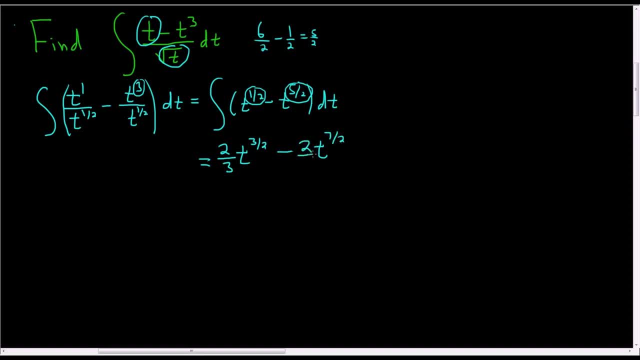 So, instead of dividing by 7 halves, let's multiply by the reciprocal, which is 2 over 7.. And then plus our constant, which we'll call c, And that's it. Find the antiderivative of 3x times t. 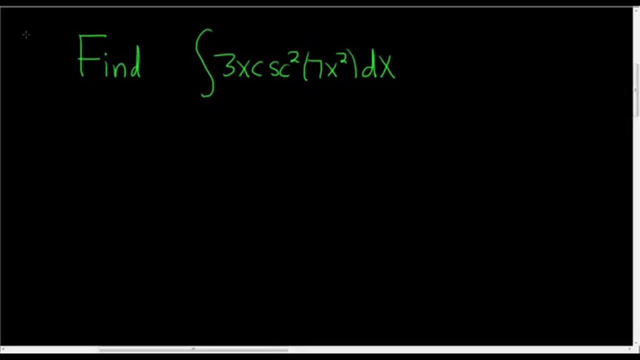 Find the antiderivative of 3x times the cosecant squared of 7x squared solution. So it looks like a? u substitution might be a good first approach. If we set u equal to 7x squared, then du is going to be 14x dx. 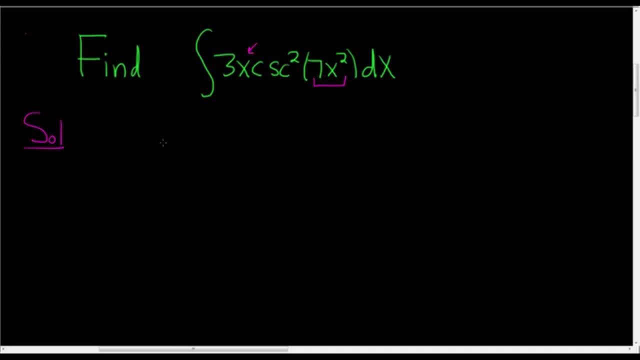 And we do have an x here. So then we can manipulate that to finish our substitution. So let's go ahead and try. So u is equal to 7x squared, And then so du will simply be 14x squared. So we have 14x dx. 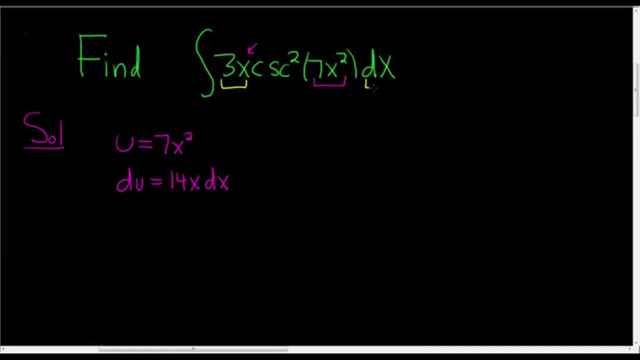 Now we have 3x dx, And here we have 14x dx, So we want to have a 3 here. So what we'll do is we'll multiply both sides by 3 over 14.. And then what happens is we're left with 3 over 14 du. 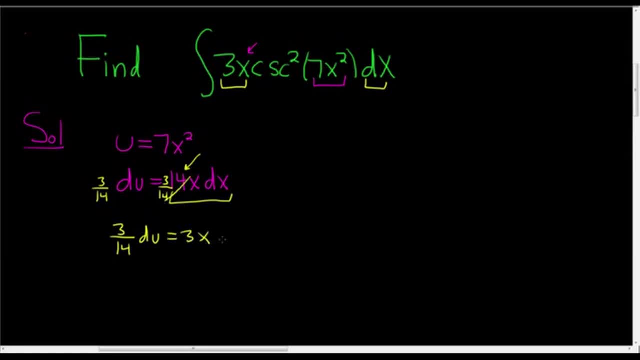 And then the 14 cancels here. So we're left with 3x, dx, And now it looks like we're ready To make our substitution. So we have the indefinite integral Now, the 3x and the dx. that's right here. 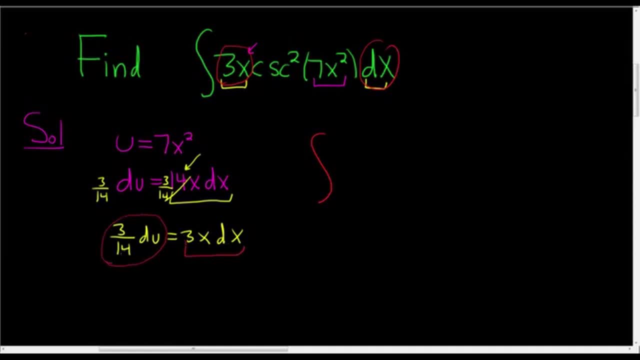 And that's going to be 3 over 14 times du. So we can write the 3 over 14 outside and put the du over here. And what's left over? Cosecant squared. So cosecant squared of u, Because all this stuff inside here, that's simply u. 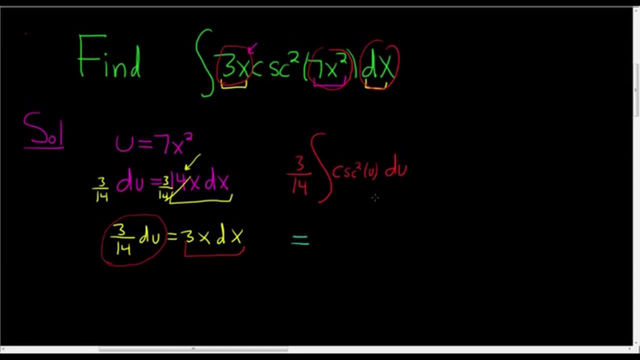 OK, To finish, we just have to think: what's a function whose derivative is cosecant squared? Well, the derivative of cotangent is negative, cosecant squared, So we need a negative cotangent. So I'm going to go ahead and put the negative here. 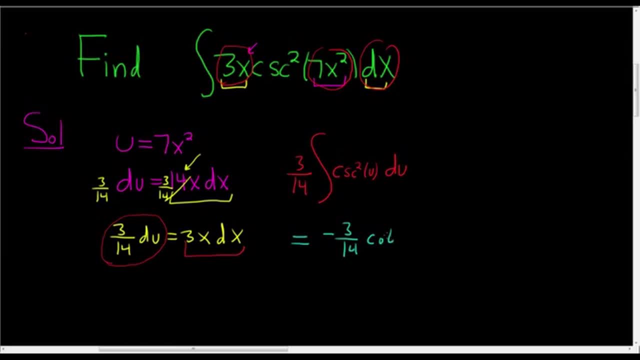 So negative 3 over 14 cotangent. And then u plus our arbitrary constant c, And then u was 7x squared. so this is negative 3 over 14 cotangent of u And u, we said, was 7x squared. So this is negative. 3 over 14. cotangent u and u we said was 7x squared. Subtract u and put 3 over 14.. You know we've been doing those a lot on the alphabet So we're really good at supposed to leaving u after u. 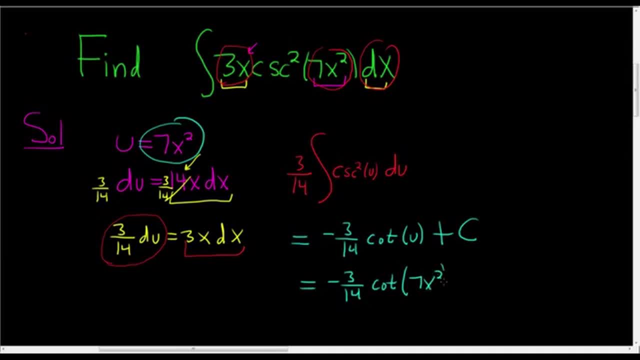 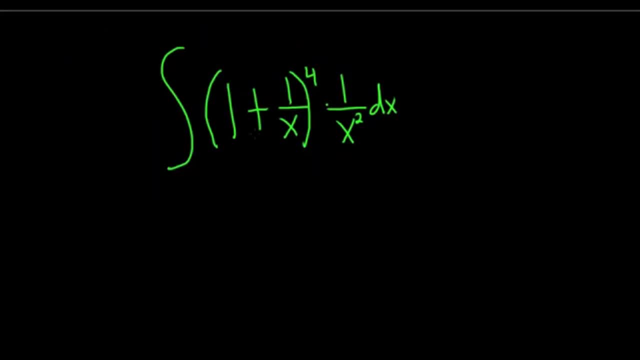 7x squared. So 7x squared and then plus our constant c and that's the final answer. In this problem we have an indefinite integral, So 1 plus 1 over x, all to the fourth power times 1 over x squared. So solution: So multiplying this out seems like a lot of work. 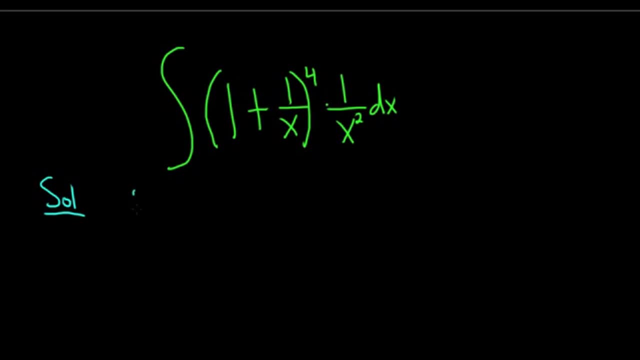 and so you have something here that's being raised to a power. So it's usually a good idea to make a u substitution, and typically your u is whatever is being raised to a power. So we'll start by letting u be equal to 1 plus 1 over x. Then we have to compute du. 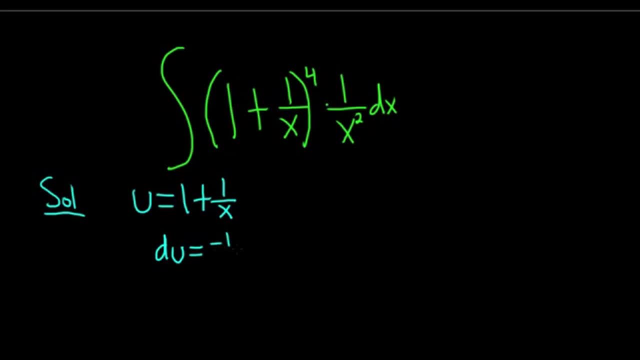 So the derivative of 1 is 0 and the derivative of 1 over x is negative- 1 over x squared- and then we have the dx. If you don't know how to compute that derivative, what you can do is you can write it like this: by bringing the x upstairs, because there's a 1 here. 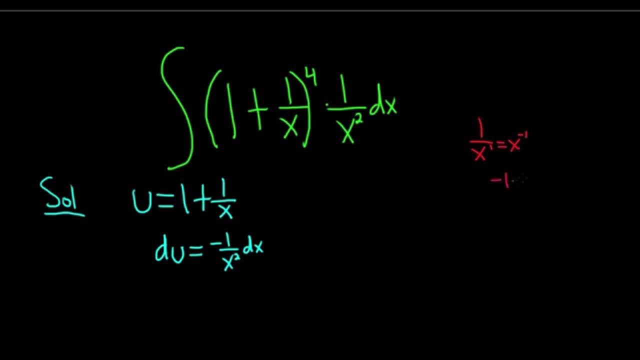 Then, when you differentiate this, you put the negative 1 in the front. You get times x and then you subtract 1 so you get minus 2.. Then you can bring it back downstairs so you get negative 1 over x squared. So everything checks Okay. once you get here, you have to make this look like whatever you have in your 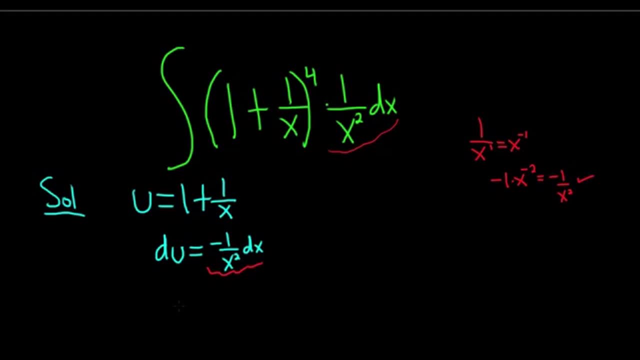 integrand So here we have an extra negative 1 so we can multiply it over to the other side. So negative du is equal to 1 over x squared dx- Good stuff. So now we're ready to make our substitution. So 1 over x squared dx, that's this piece right here. that's going to be negative du. 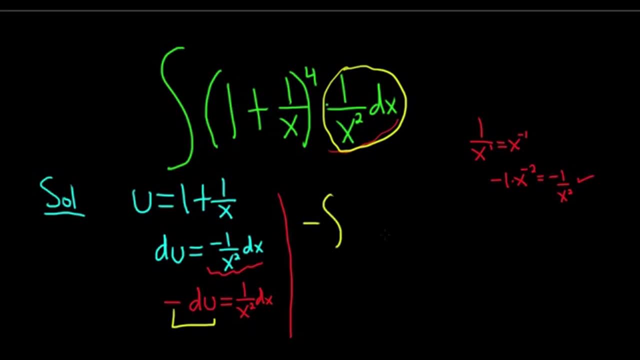 So what you can do is you can put the negative outside. So we have negative du And all that's left is this piece right here now. So this piece here is just your u. So we have u to the fourth. Alright, then we can integrate using the power rule. 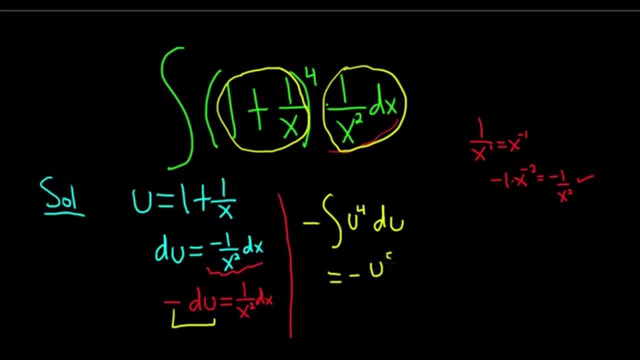 So this is negative. You just add 1. so it's u to the 5 divided by 5, plus a constant. So add 1 and divide by the number And the last thing to do is substitute u back in. So we said u was 1 plus 1 over x. 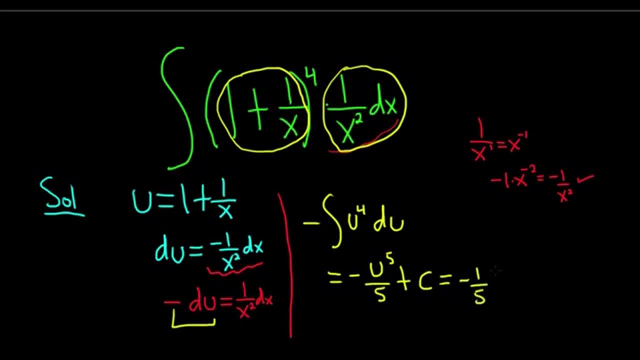 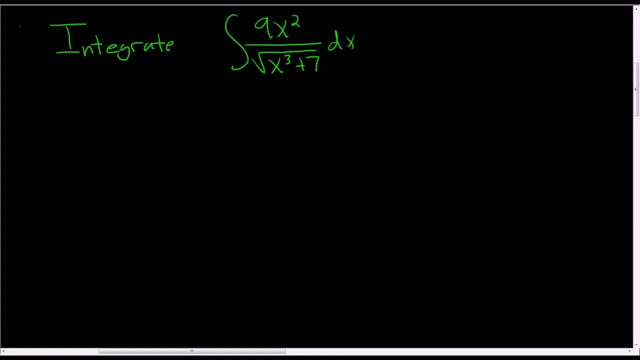 You can pull the 5 out and write it as negative 1 fifth. Then you have 1 plus 1 over x to the fifth, Then you have plus c And that would be the final answer. That's it, Alright, so we have to deal with this integral solution. 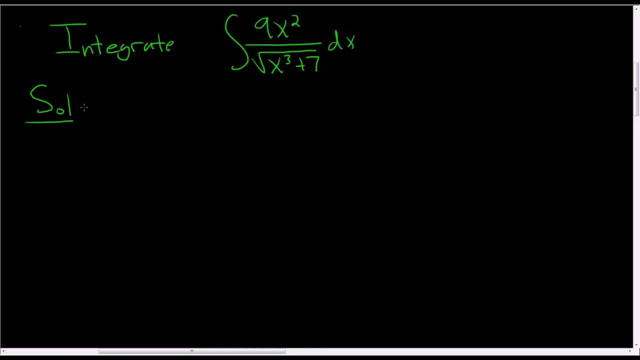 Now it seems like the here. let me try. let me try blue. Yeah, it's better. Blue, Okay, It seems like the best way to go with this problem is to do a? u substitution. Why? Because if you let u be this here, then du kind of appears in the numerator. 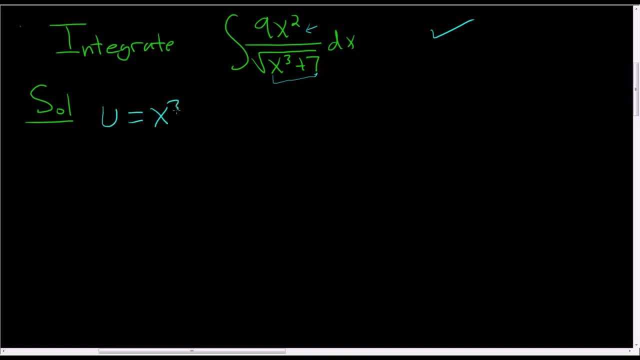 So let's try it. So set u equal to x cubed plus 7.. And so du is 3x squared, dx. Alright, we have a 9x squared, so we'll just multiply both sides by 3.. So 3du 3 times 3 is 9.. 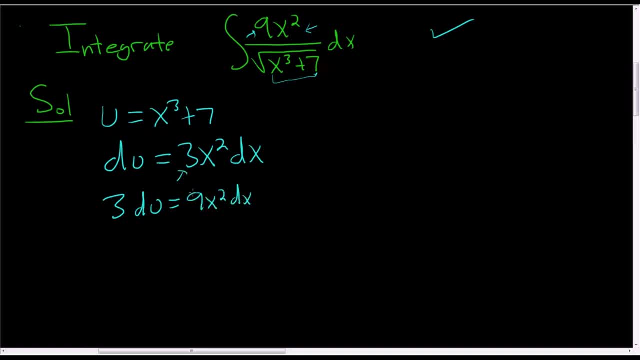 So you get 9x squared dx. Alright, now we're ready to go. We're ready to make our substitution. So 9x squared dx is right here And it's also down here. That's equal to 3du, So we'll have 3du. 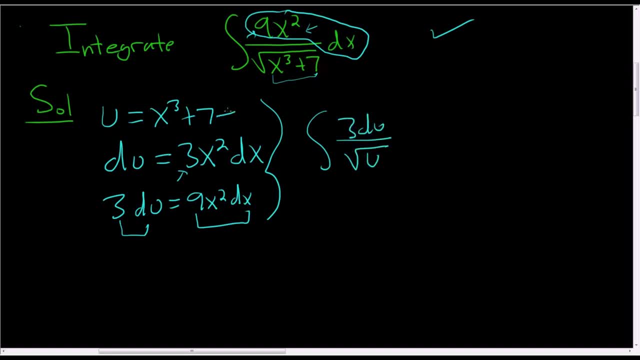 over the square root of u. Right, Because u is x cubed plus 7. And it's right here. Okay, To integrate this, we have to write this as u to a power. So the square root of u is u to the 1 half. 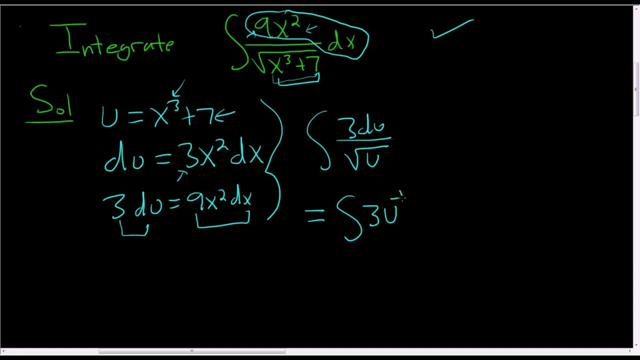 And when we bring it upstairs it becomes: u to the negative 1 half du, So this is equal to 3: u to the negative. 1 half plus 1 is 1 half, And then you divide by 1 half Plus a constant. 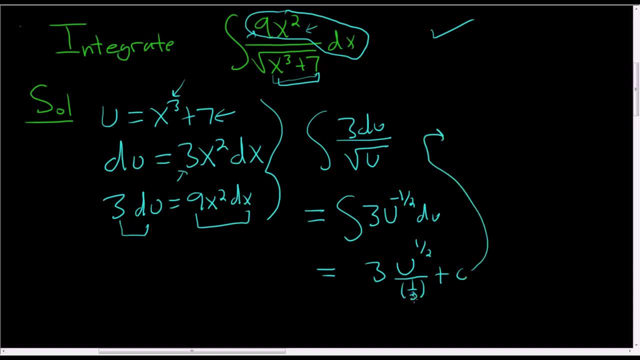 This ends up being Well. when you divide by 1 half, you really multiply by 2 over 1.. So it's 6.. 2 times 3 is 6.. Square root Right. Rewriting the? u to the 1 half. 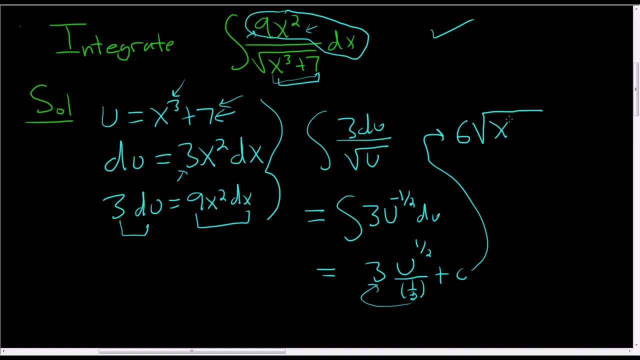 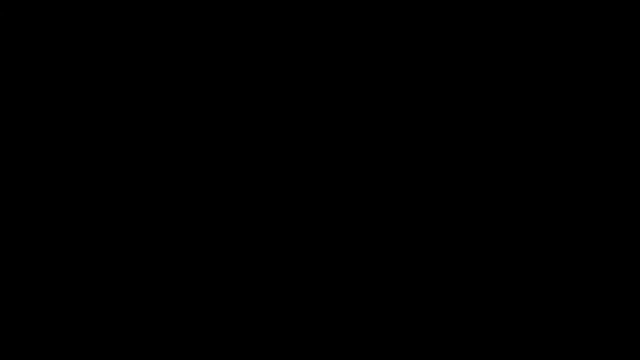 And u was x cubed plus 7. x cubed plus 7. Plus our arbitrary constant. In this video we're going to briefly recall summation notation And then talk about some of the formulas used to compute area under curves. So first recall the following notation: 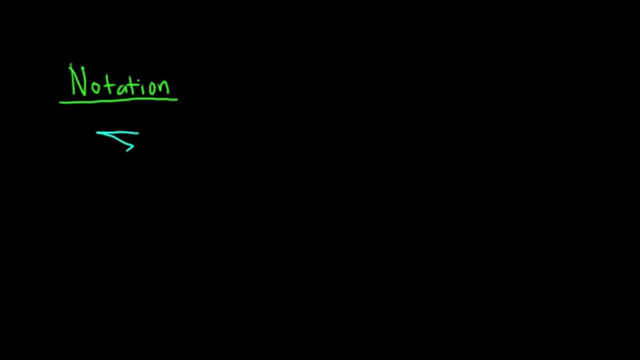 So there is a Greek letter. It looks like this, So something like this, And it's called sigma, And so sometimes we put a little i here, And this is equal to 1. And then we go to n, And here we have a sub i. 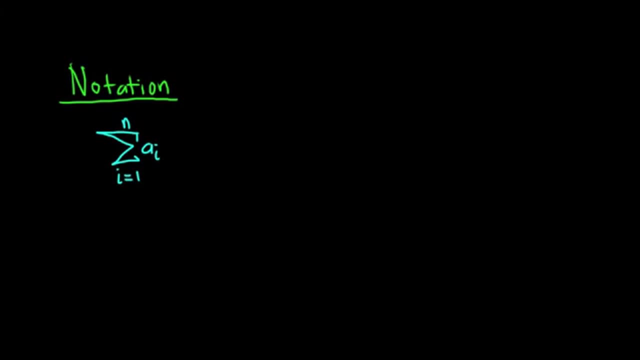 And so how this works is: you start at the number here at the bottom, So you plug in 1.. So you plug in 1.. And this symbol, when you see it, it means you add So plus. Then you plug in 2.. 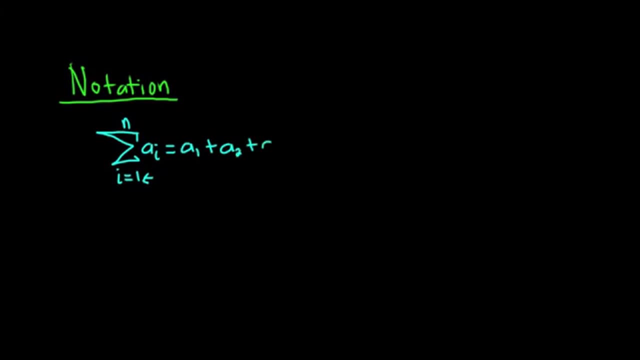 And then again you add So plus, And then you plug in 3.. And then you add Etc, And you keep adding, And the very last number you plug in is the top number. So n, So a sub n. 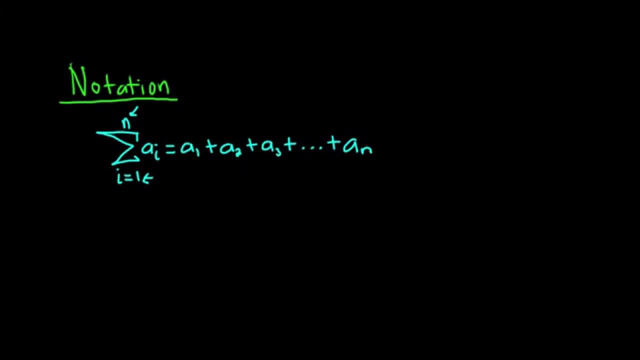 So this is called summation notation. Several of these things have names, So i here is called the index of summation. Index of summation. Typically people like to use i, j and k for the index. A sub, i, A sub i is called the i-th term. 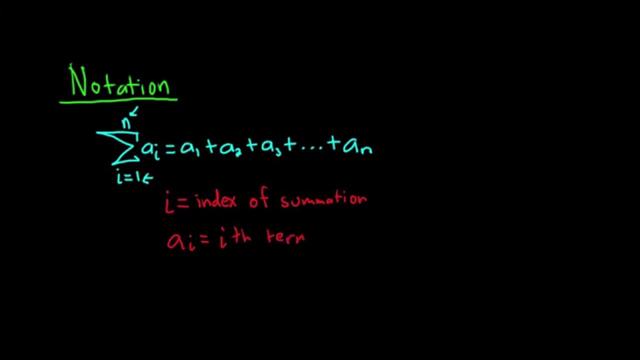 i-th term. So a sub 1 would be the first term, A sub 2 would be the second term, A sub 3 would be the third term. A sub n would be the n-th term. The numbers 1 and n. these are called the bounds. 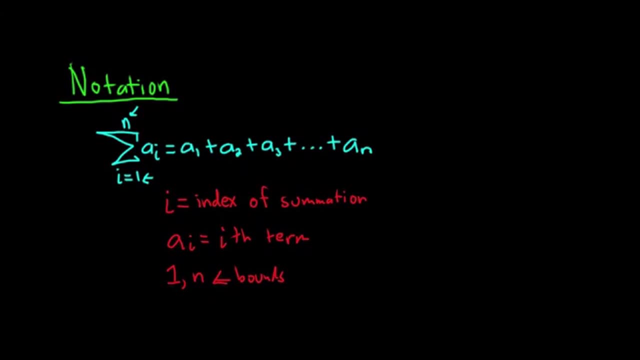 So bounds, Bounds of the summation are just the bounds: 1 is the lower bound and n is the upper bound. So there are some formulas. Before we look at the formulas, let me just do a simple example over here of how the summation notation works. 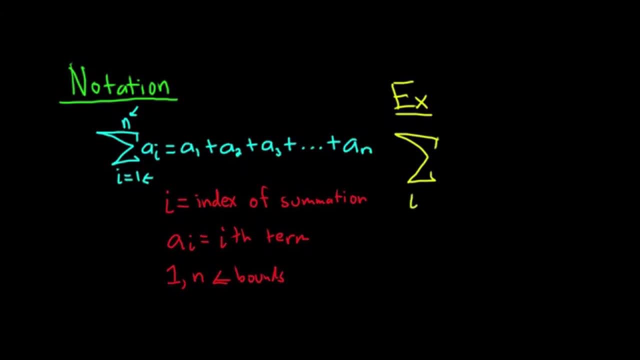 So say we had the sum- as i runs from 1 to 3.- Of 2i. So in this case the first number you would plug in is 1.. So you'd plug in the 1 for the i, so you'd get 2 times 1.. 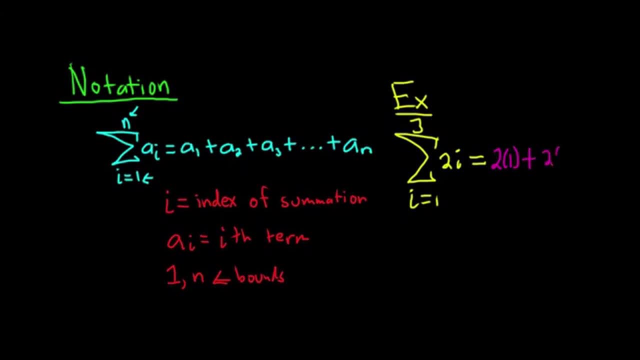 And the symbol means you add, And then you plug in 2, so 2 times 2.. And the symbol means you add, so then you plug in 3, so you get 2 times 3. And you stop at 3.. 3 is the upper bound. 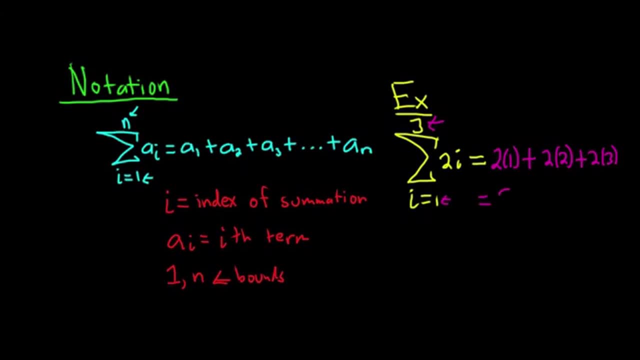 And 1 is the lower bound. So this would be: 2 times 1 is 2.. 2 times 2 is 4.. 2 times 3 is 6.. So you get 2 plus 4, which is 6.. 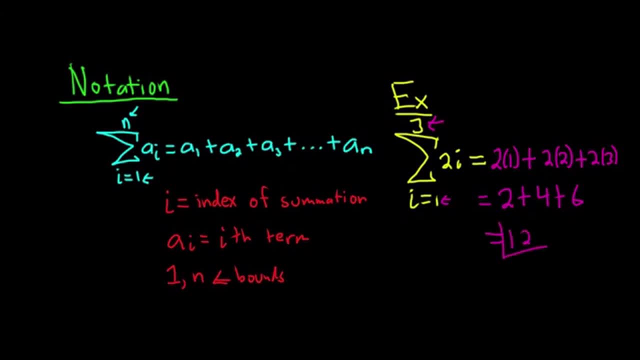 6 plus 6 is equal to 12.. So this summation is equal to 12.. Now, in our area problems, what's going to happen is we're not going to have a number here. usually We're going to have a variable like n. 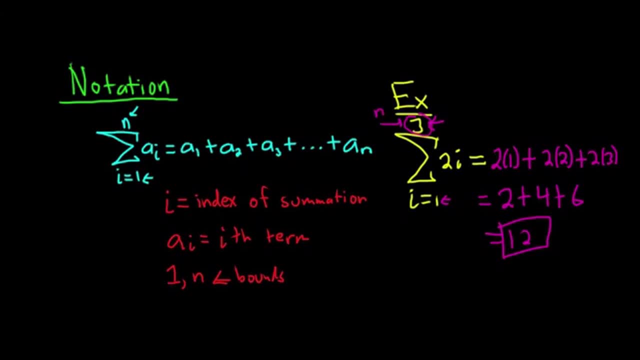 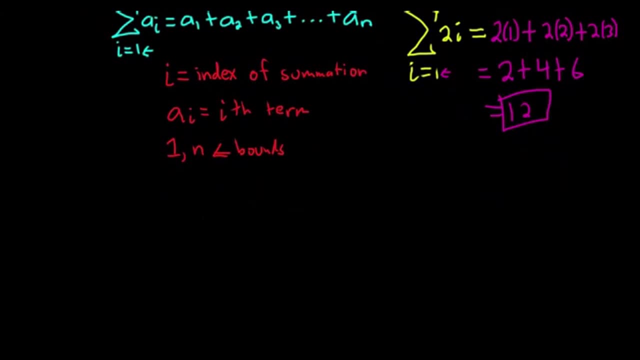 And so we'll need to somehow resolve these sums. We'll need to get rid of the summation notation in order to take a limit. So the following formulas are very, very useful and are totally worth memorizing for That purpose. So formulas, formulas. 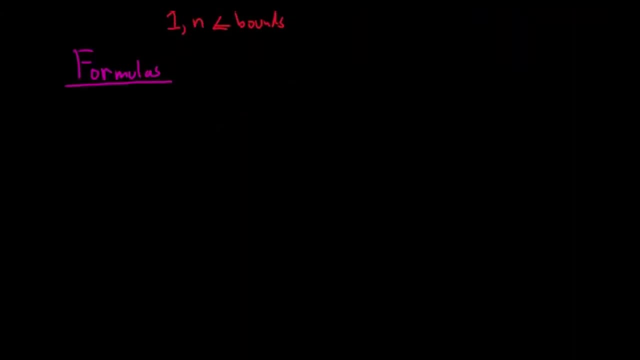 So the first formula that we'll have is if you have a constant being added over and over again. So the finite sum, as i, runs from 1 to n of c. So when you plug in 1 here, you get nothing, You just get c, so it's c. 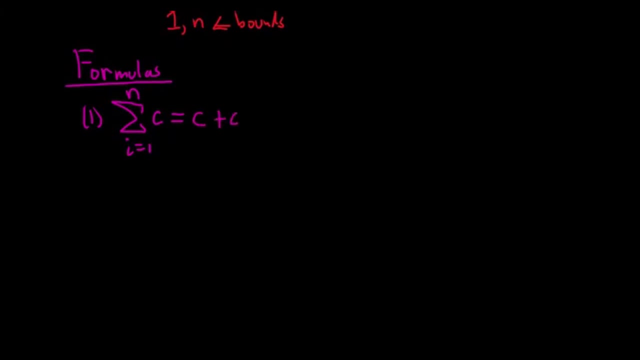 And then you add again. so you just get c again, And then you add, and then you just get c, And you just get c every time you plug in the number. The last number you plug in is n and you get c. 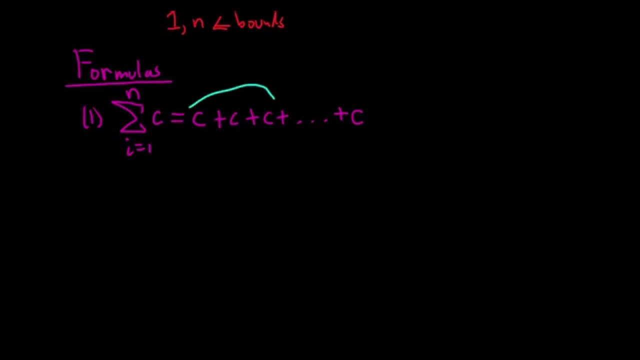 So you have n copies of c. There's n of them. There's n copies of c, So you just get n times c. If that doesn't make sense, think of a simpler example. Say you had 2 plus 2 plus 2.. 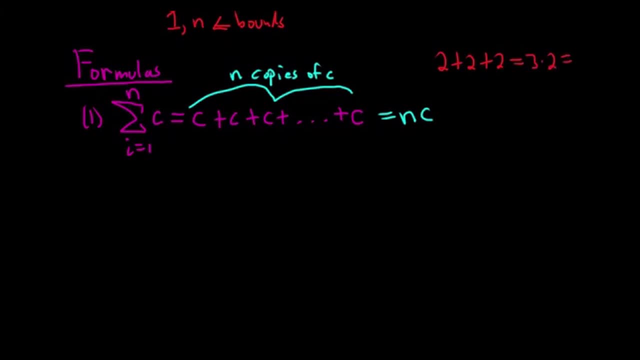 You have 3 copies of 2.. 3 times 2, so it's 6.. If you have 2 plus 2 plus 2 plus 2, you have 4 copies of 2, so it's 4 times 2, so you get 8.. 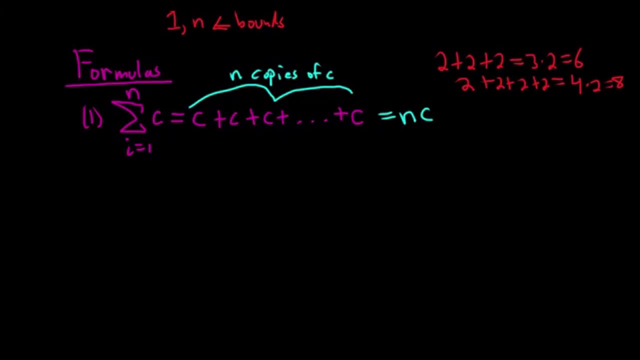 Et cetera. So here we have n copies of c, so it's nc 2.. Another useful formula is when you have the sum, as i runs, from 1 to n- of i, And this is equal to n, n plus 1, all over 2.. 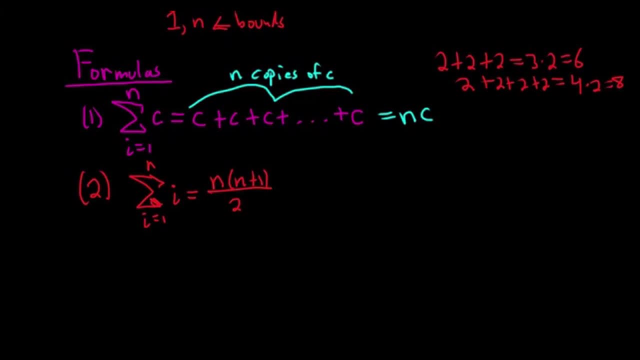 Very, very, very useful formula, Very, very useful. 3.. You have the sum, as i runs from 1 to n, of i squared. This one's a little bit harder to remember: It's n n plus 1.. 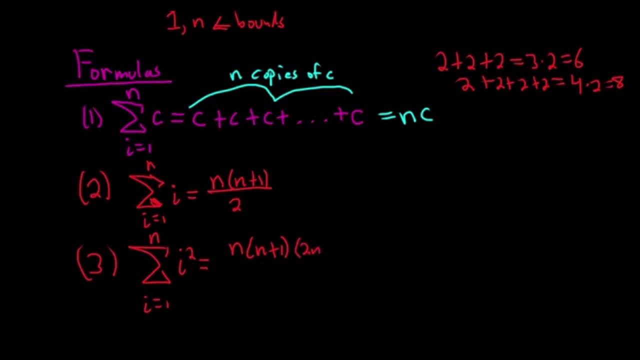 That part's easy And the weird part is that it has a 2n plus 1, and it's all divided by 6.. This one takes the most effort to memorize And the very last one. there's a little trick to memorize it. 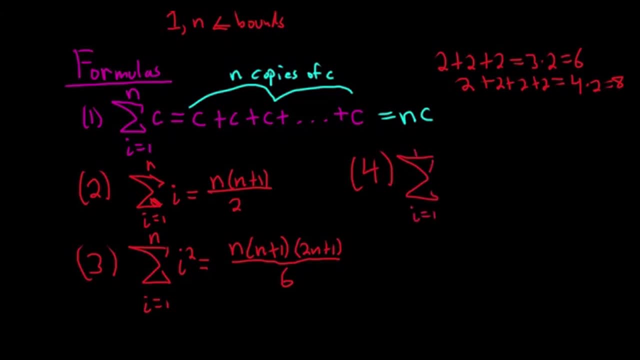 It's the sum- as i runs from 1 to n- of i cubed, And the way I memorize it is: you just square this one, So you square the n. You square the n plus 1.. And then you square the 2, so you get 4.. 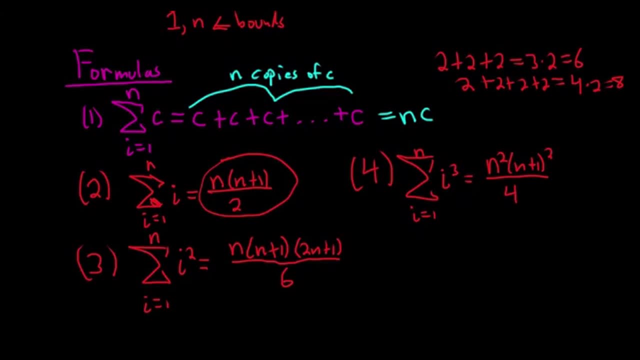 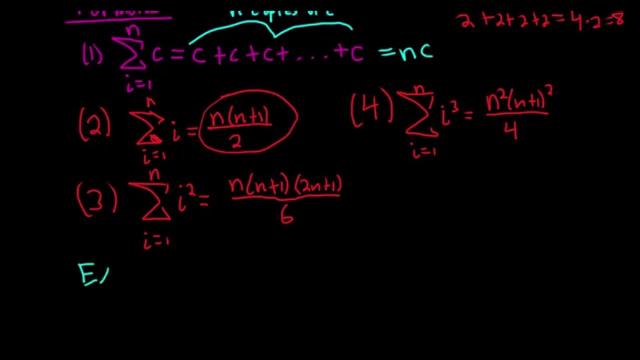 So these are the formulas that we'll need for area. Let's go ahead and do a simple example. I'll give you an example of using these formulas. So ex means example. Let's compute the sum, as i runs from 1 to I don't know 5.. 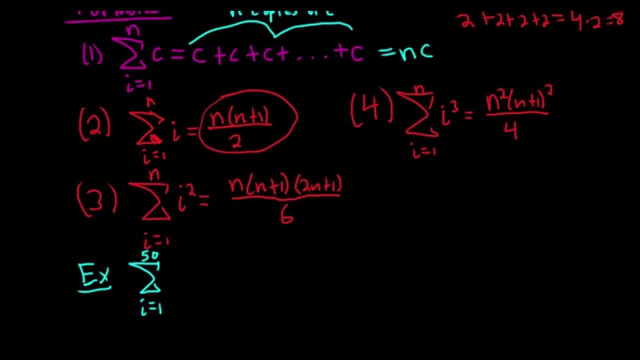 No to 50.. To 50.. Let's be bold And let's do 2i plus i squared, 2i plus i squared, So to do this sum. what we typically do is we break it up Right. 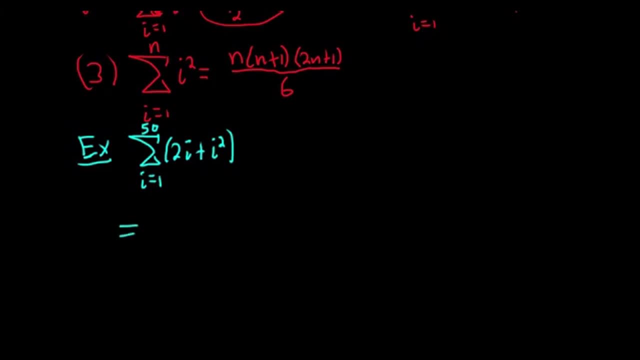 We break it up. So basically you can pull out anything that doesn't have an i, So you can write this as 2, finite sum: i runs from 1 to 50 of i. Okay, that's this piece here, Right. 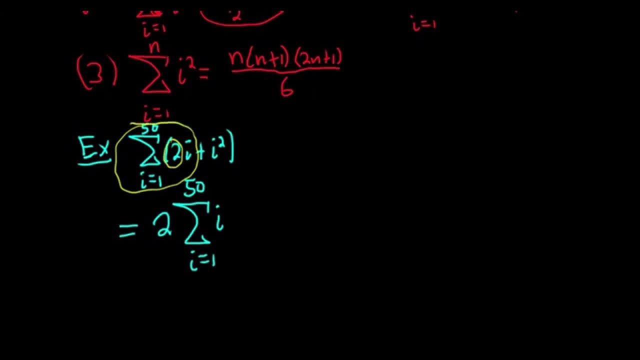 That's this piece here. So basically we took this piece and we pulled out the 2. Plus, and then we have i squared And i runs from 1 to 50. So we have 2i plus i squared. We have the same thing down here, except we pulled out the 2.. 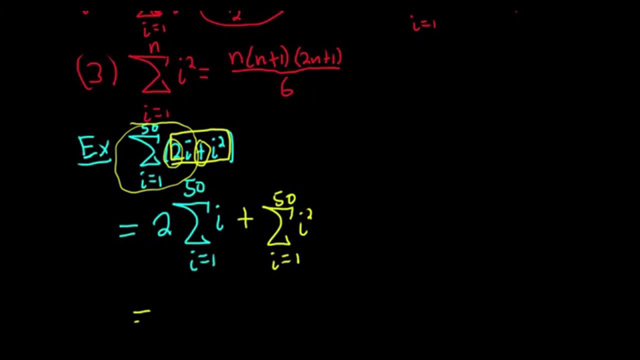 And we broke them up because it was a plus sign, And so now we just use the formulas, So it's 2.. So this first piece here, this piece right here, that's the formula. I'll write it again over here because you can't see it. 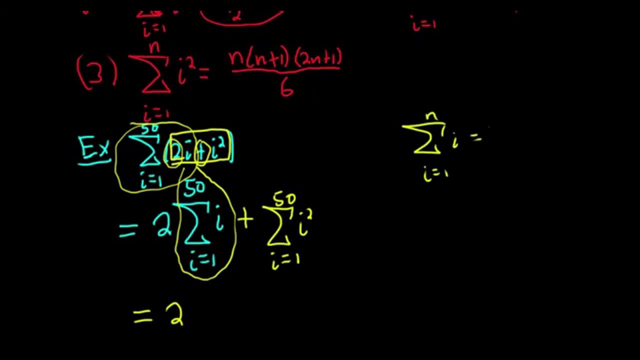 It's i equals 1 to n, And then it's n m plus 1 over 2.. So in this case our n is 50. Which is 50, 50 plus 1 all over 2.. Plus, and the other formula is still up here. 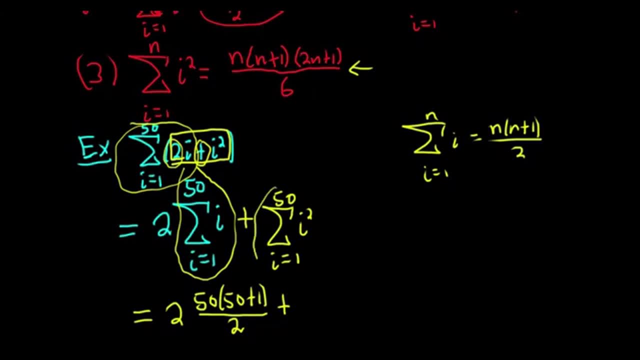 This is the other one, for i squared. So again this whole thing becomes this piece here, And then you just plug in your n and it's 50.. So it's 50, 50 plus 1.. And then 2 times 50 plus 1, all over 6.. 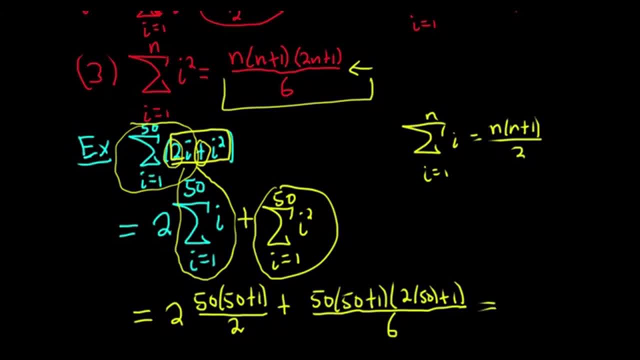 And this is the part where you have to go to the calculator. So I'm going to go ahead and type this in To make it easy for me. I'm going to cancel these 2s. That should make it a little bit easier. 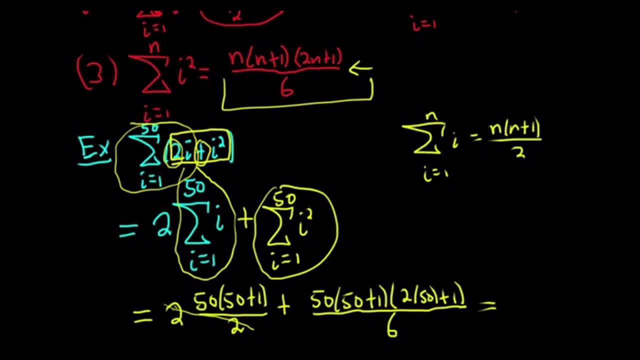 So it's 50 times 51.. That's the first piece. So the first piece is equal to 2550.. So 2550 plus- I'm going to type in this piece into my calculator. So that's going to be 50 times 51 times. 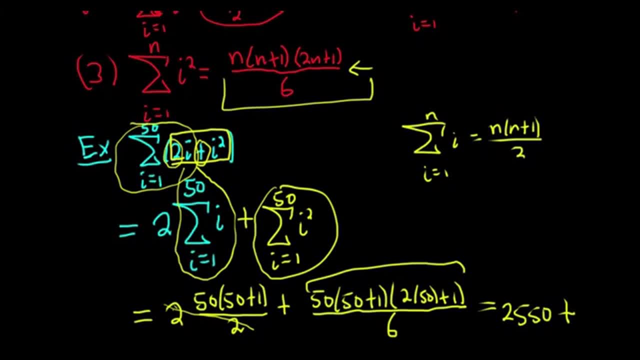 and the second piece here is 101.. Right, And this piece here is 51. So I'm going to type that in 50 times 51 times 101.. And that's all divided by 6.. So I got 42925.. 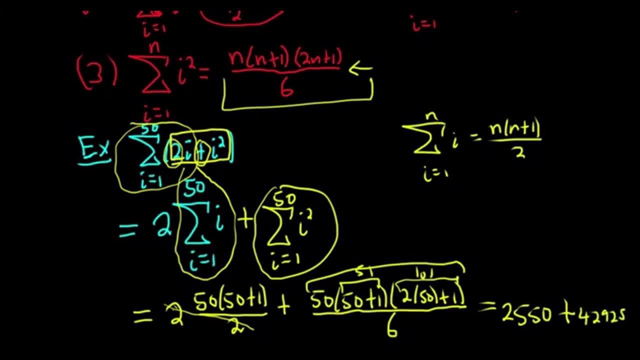 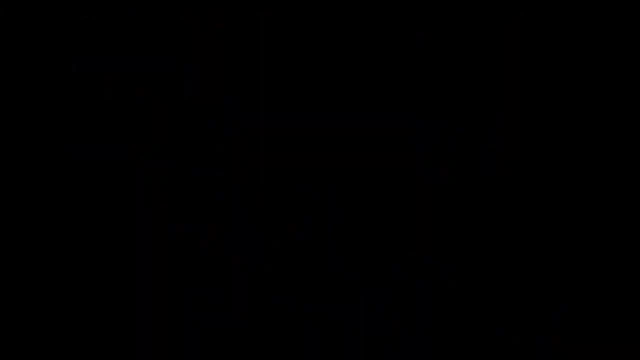 Wow big numbers. So 42925.. Then you add these numbers up, So plus 2550.. So you get 45475.. So 45475.. And that's the final answer. That's it, Hi, everyone. In this video we're going to define Riemann sums, definite integrals. 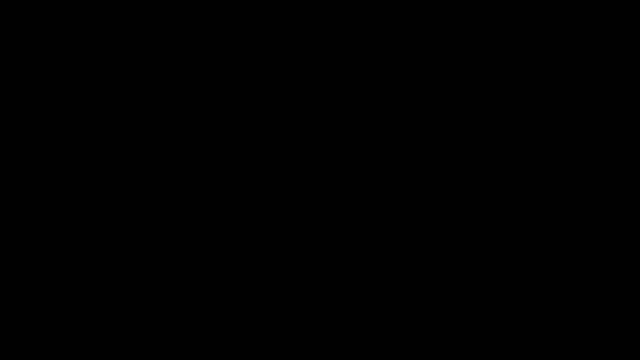 and then I'll give you the formula to find the area under a curve. Before we do that, let me just tell you what a Riemann sum is, intuitively. So let me draw a picture here. So this is the y-axis and this is the x-axis. 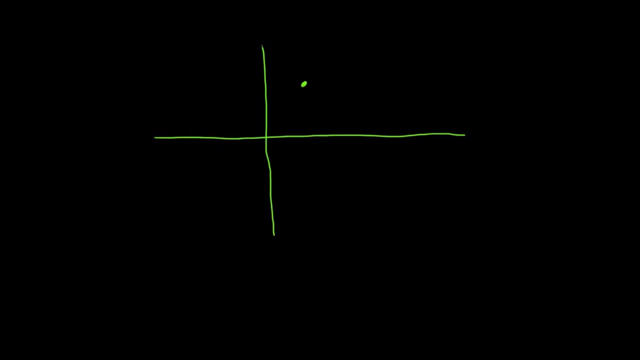 And say: we have a function f. It goes from here to here And this is a and this is b. So we have some function And now I'm going to draw a bunch of random rectangles. So I'm going to draw a rectangle here. 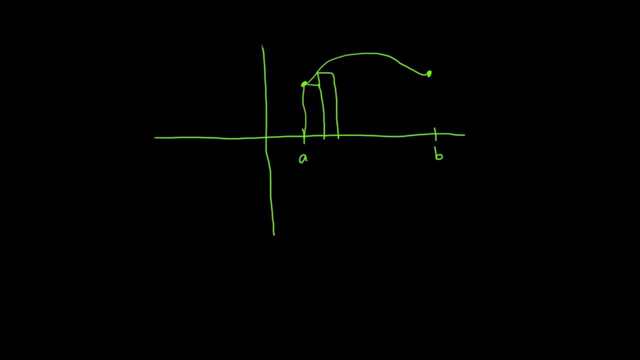 I'll draw a rectangle here. Okay, I'll draw a rectangle here. Okay, I'll draw a rectangle here. It's a big rectangle. I'll go ahead and draw a little skinny rectangle here, And I'll draw one here, And I'll draw one here. 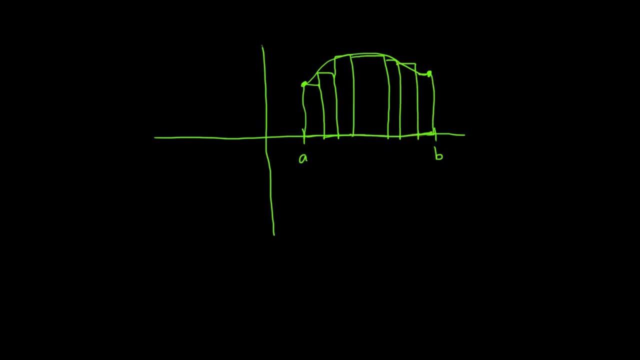 So I have a graph and I just drew a bunch of random rectangles. okay, If you add up the areas of all of these rectangles, you get a Riemann sum. So a Riemann sum. basically, all you do is you take a graph. 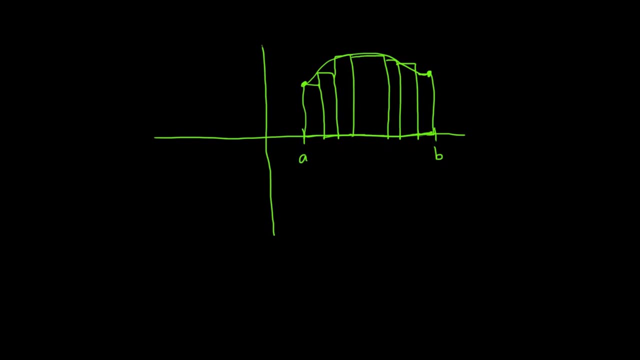 you draw a bunch of rectangles and you add up their areas. That's a Riemann sum. The catch is it can be any random rectangles, right, So you can't specify what they are. So let's go through the formal construction of the definite integral. 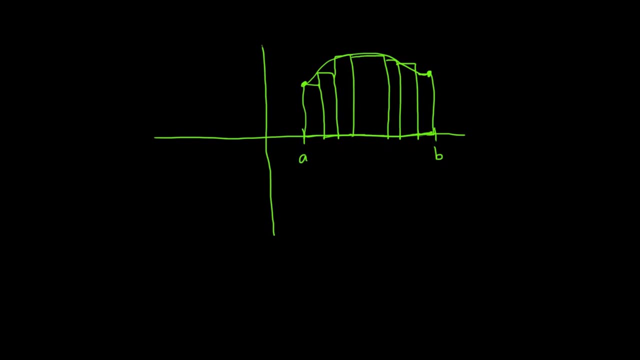 so you see how intense it is. It's really really cool. So we'll start by having a function, f, and it's defined on a- b. So f is defined on a- b. Okay, so that's our a and our b, just like in our picture above. 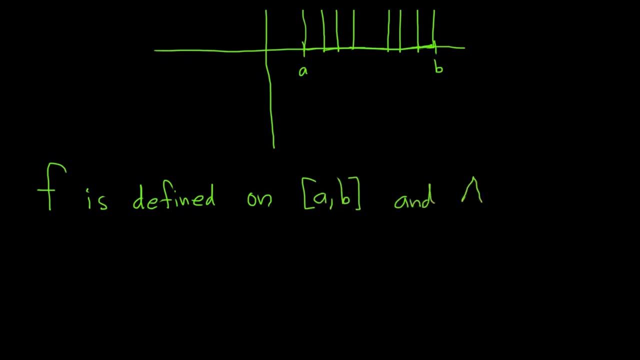 And capital delta. I believe this is the capital Greek letter delta. There's another delta. I think that's lowercase, Not positive, but I'm pretty sure This is a partition, Partition, Partition of a, b Given by. So a partition is just a bunch of numbers that break up an interval, right? 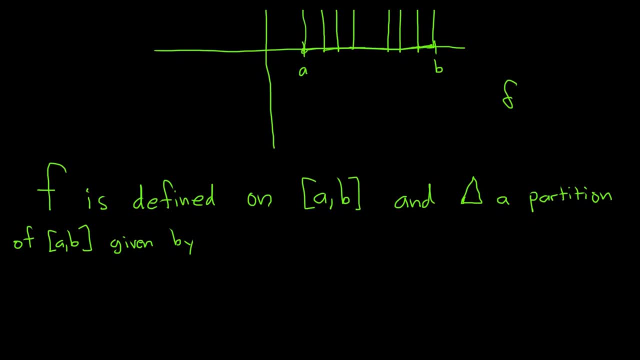 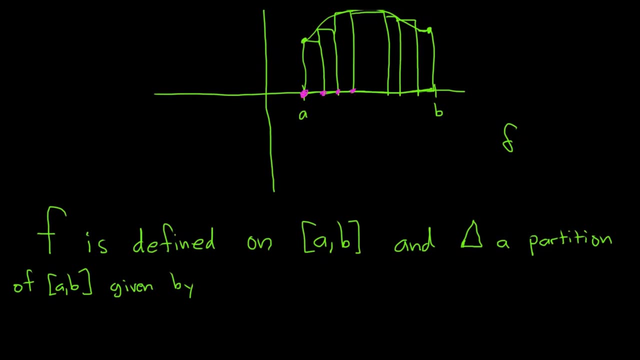 So our partition in the picture above- let me scroll up so you can see it- In the picture above, our partition is these dots here which I'm about to draw. That's our partition, those random numbers there that we picked to break up the interval. 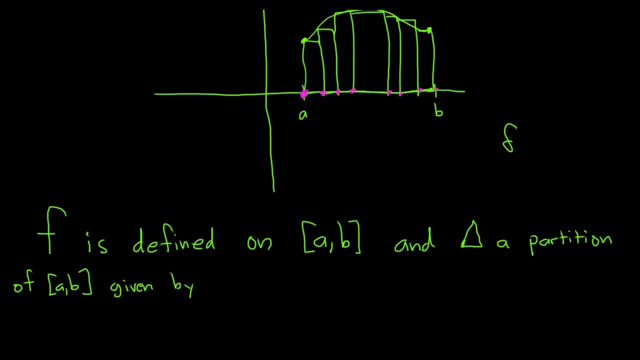 Okay, that's our partition. So here we're going to give them names. So the first number notice here it's a in this picture. So I'll say it's a and we'll call that x sub 0. That's less than the next one, which is x sub 1.. 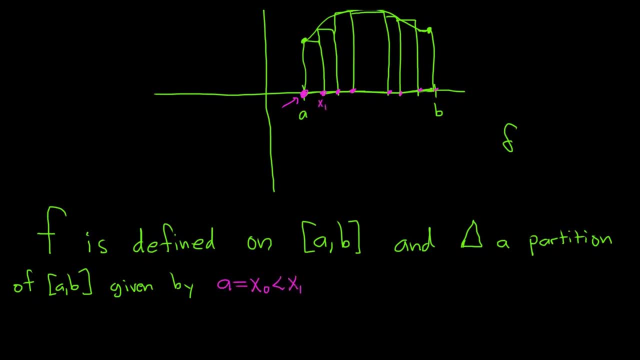 So maybe this is x sub 1 in our picture, Less than dot dot dot, Less than x sub n, And we'll call that b. So I'm going to go back to our picture and just call this x sub n and x sub 0, just for added clarity. 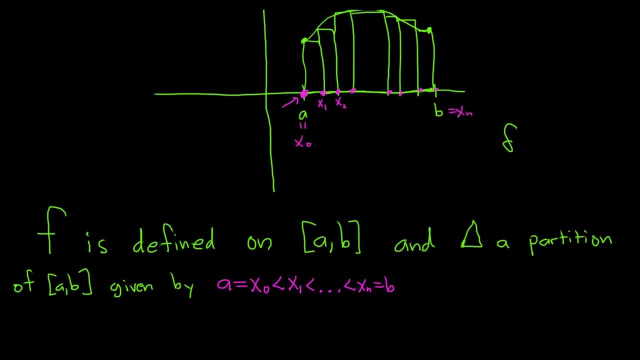 And this would be x sub 2,, et cetera. So we're taking an interval and we're just breaking it up randomly. So taking an interval and randomly breaking it up, We don't know what these numbers are. Where delta x sub i is the width of the i-th subinterval. 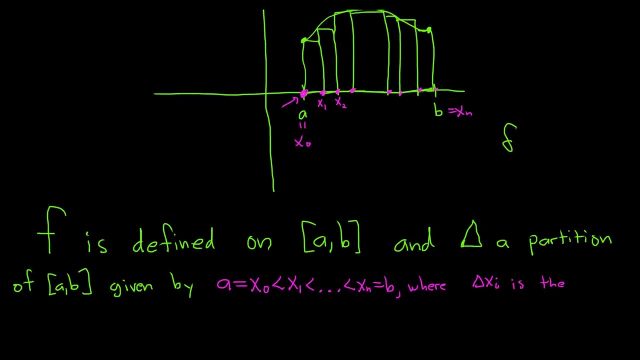 is the width of the i-th subinterval. So in our picture this here is delta x, sub i. They're all different in our picture, Or some of them might be close to the same, But they don't necessarily have to be the same. 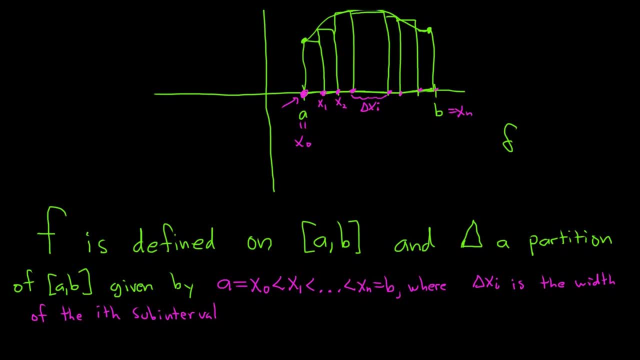 So in our picture it's the width of the rectangle. We haven't formed the rectangle yet down here in our description, But we will. we will Now, if c sub i is any. I'm going to underline this. this is key. 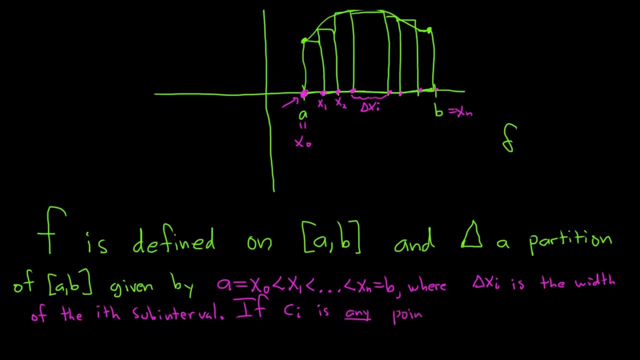 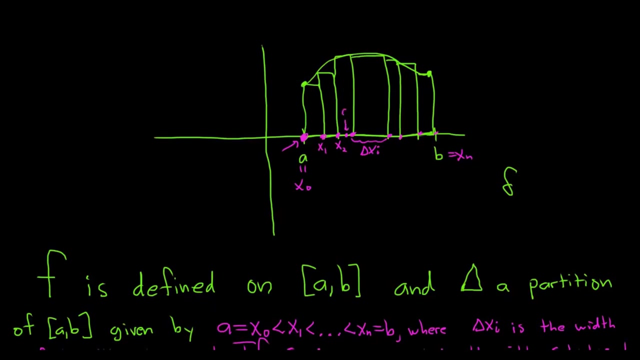 is any point. so any number in the i-th subinterval. So you just basically pick a random number in the subinterval, So like, for example, let me scroll up so you can see a little bit better. So like here, maybe Here, this is my c c sub i. 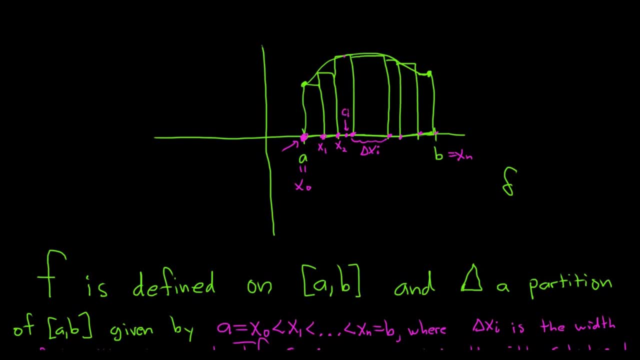 Right, That's my c sub i, right there. And that what happens is we're going to plug that into the function to get the y-value here, f of c sub i. You see, So when you plug in c sub i into the function, 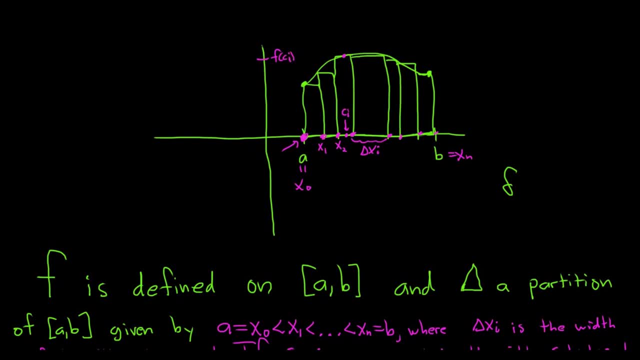 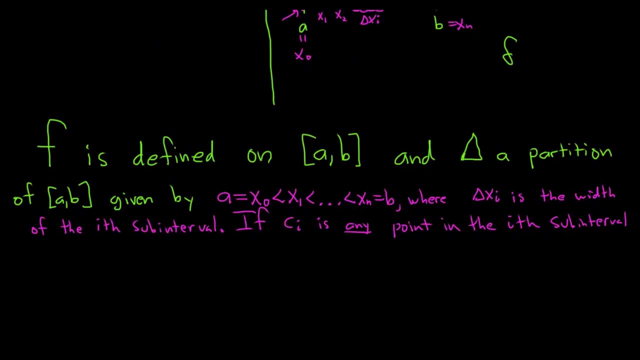 that will give us f of c sub i And that will give us the height of the rectangle which you'll see shortly. So if c sub i is any point in the i-th subinterval, then the sum, so the sum. here we have a sum. 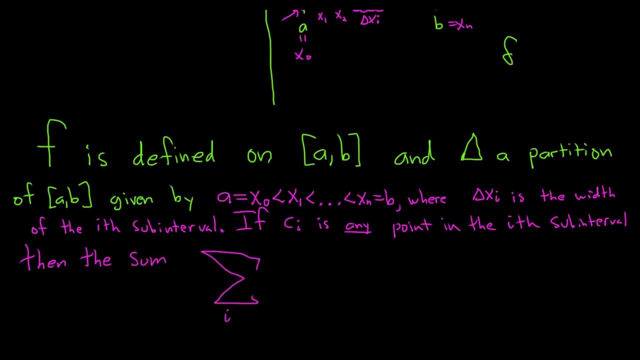 The sum goes from: i equals 1 to n And it's the sum of the areas of the rectangle. So it's the height which we said was f of c sub i times the width of the rectangle, which is delta x sub i. 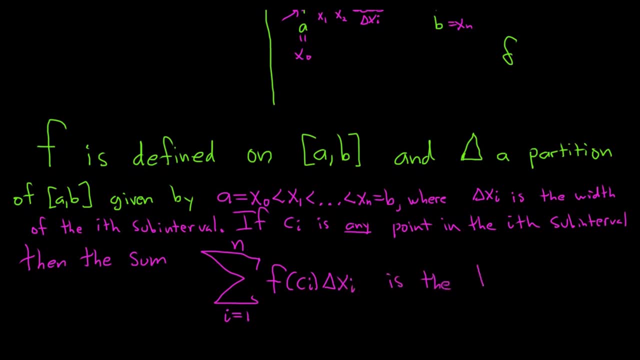 So this is the Riemann sum Of f for the partition delta. So again, we take a bunch of random rectangles and we add up their areas and we call that a Riemann sum. All of this is just a formal way of saying all that. 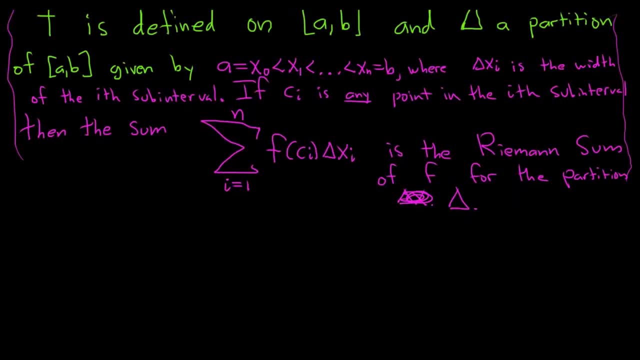 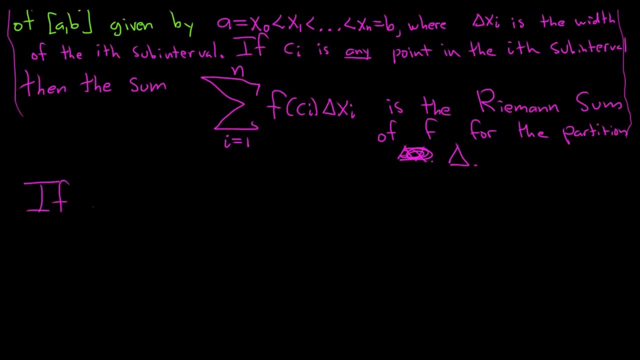 So what is an integral? So here's where it gets really crazy. Okay, So if or what is the definite integral? That's what we're defining. So if each just a random comment, if each subinterval is of equal width, 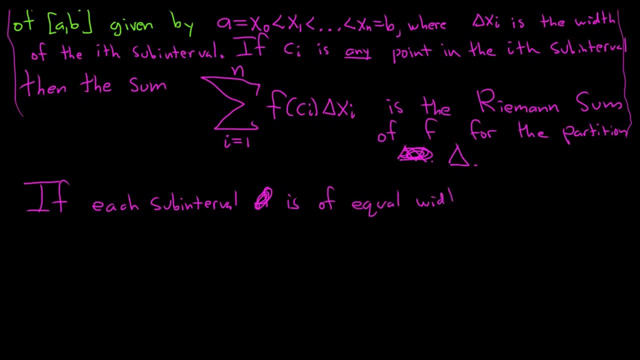 so if they're all the same width, the partition is called regular, So the partition- we can't assume that but it's important to know it. So the partition is called regular And in this case we don't need delta x sub i. 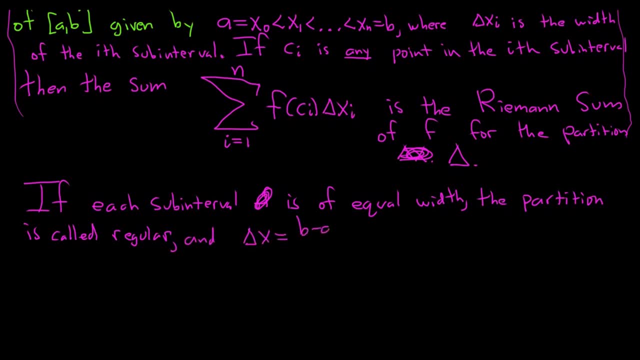 we just have delta x, and that's b minus a over n. So in actual calculus problems, when you do these problems you use this formula, which I'll write down again in a little while. You assume it's regular right. 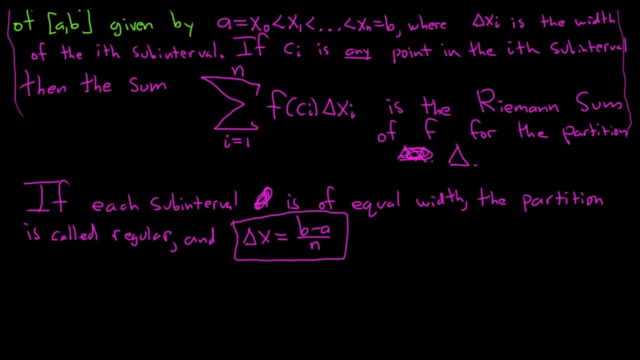 Because you assume that you can find the answer, so you can use any partition you want. So that's what that would be. So now we're going to define something. We're going to let this symbol here, so like these double bars around the partition. 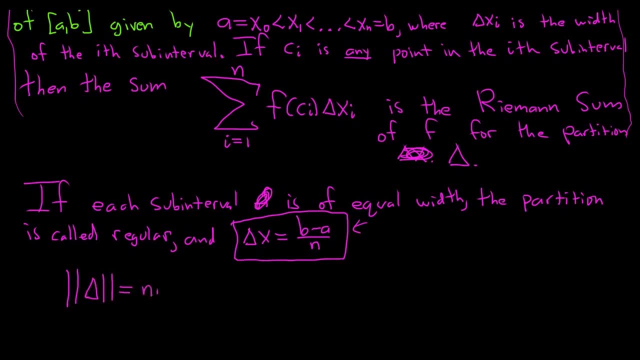 we're going to say: this is the norm of delta. And what is this? This is the width of the largest subinterval. Okay, of the largest subinterval. It's the width of the biggest one. Okay, the width of the largest subinterval. 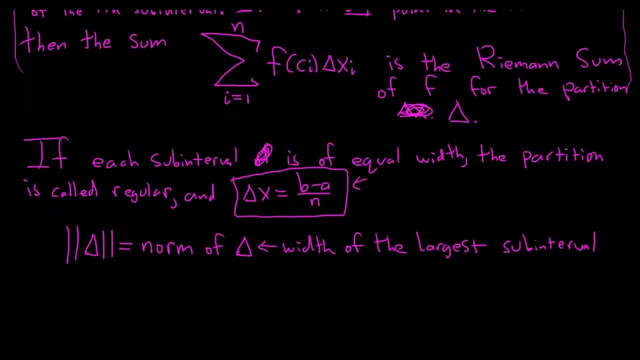 Notice. if the partition is regular, they're all the same. So if the partition is regular, in the regular case you would get that the norm is equal to delta x, which is equal to b minus a over n. That's kind of cool to notice. 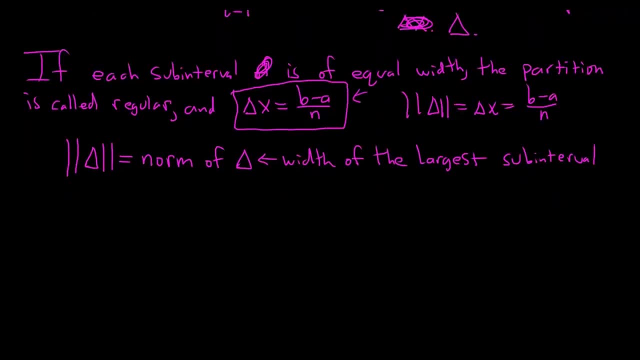 and we'll come back to that. All right, so here's the key. So if we take the limit as the width of the largest subinterval goes to zero of the finite sum of the areas of these random rectangles, and if this limit exists, 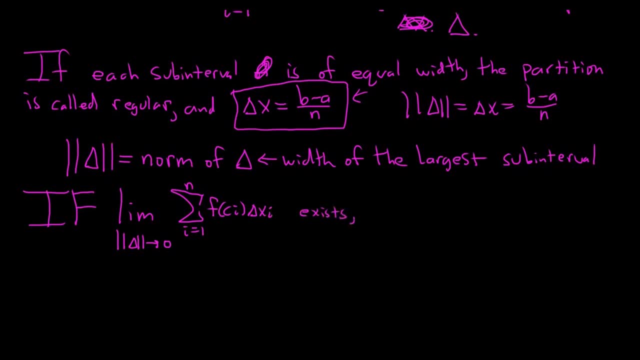 so if this limit exists, we say the function is integrable. We say f is integrable on a- b. Okay, we say it's integrable on a- b And the limit, right since it exists, is: I'll write it again: 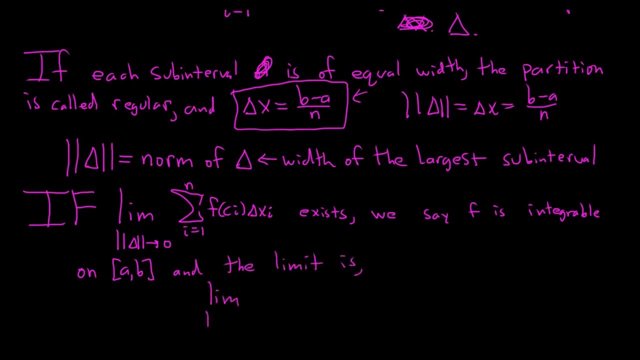 we have the limit, And I'll explain why. intuitively, this is the case as well in a second. The limit, as the norm, goes to zero, of the finite sum, as i runs from one to n of f of c sub i times delta x sub i. 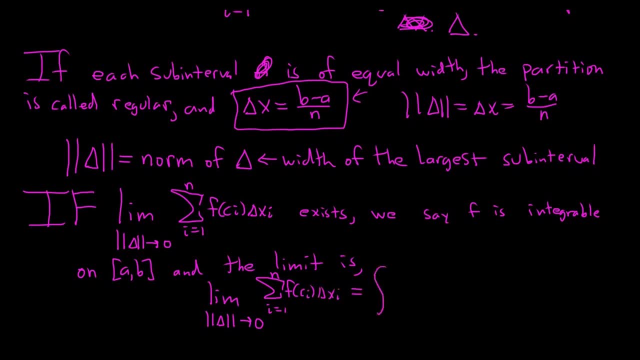 We're going to say it's equal to what's called the definite integral of our function. So the definite integral of f of x with respect to x, from a to b, That's what it's called. It's called the definite integral of f from a to b. 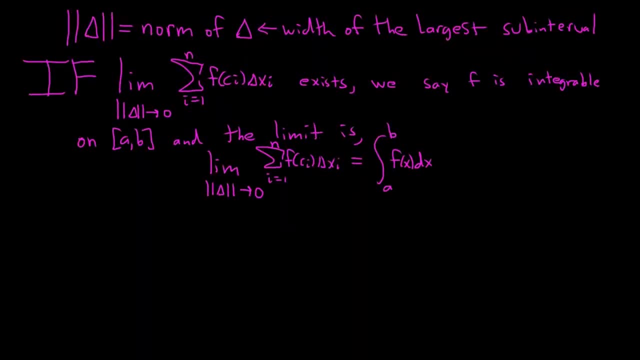 Okay, And in the case if f is non-negative, so if it's greater than or equal to zero on a, b, then the area under the curve will be this: Okay, that will be the area under the curve, Before I give you the formula for the area. 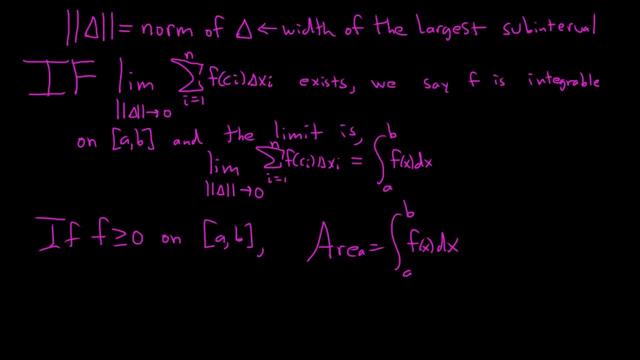 let me just explain why this should make sense, because it probably doesn't yet or might not. So if you have a bunch of rectangles right and you're trying to find the area, you're either going to get an under approximation or an over approximation. 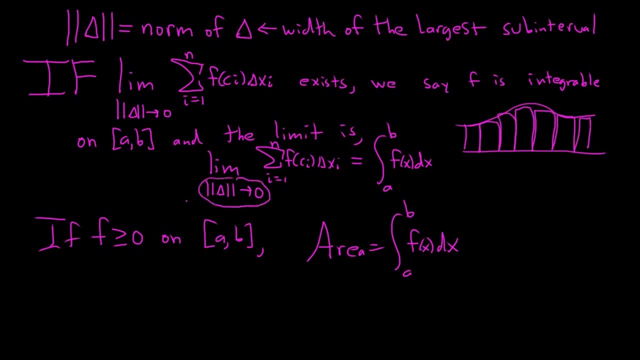 So if you let the width of the biggest rectangle go to zero, what's going to happen is you're going to get smaller and smaller rectangles. Right, You'll get more rectangles, So eventually you have infinitely many rectangles and they cover the area, and so you get the area. 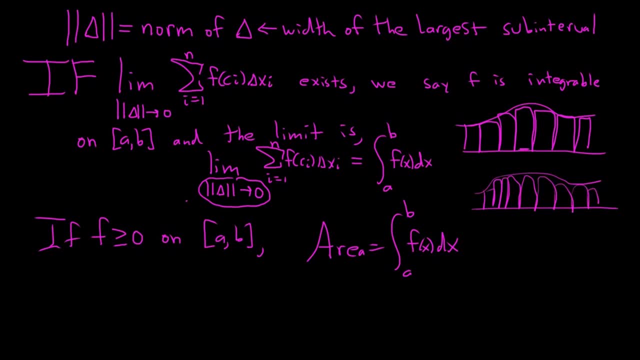 So because if the biggest rectangle in width goes to zero, all the other ones must go to zero too. So you get like tons of really super skinny rectangles and you get all of the area. Notice in the case where it's regular. so if all of the subintervals have equal width, 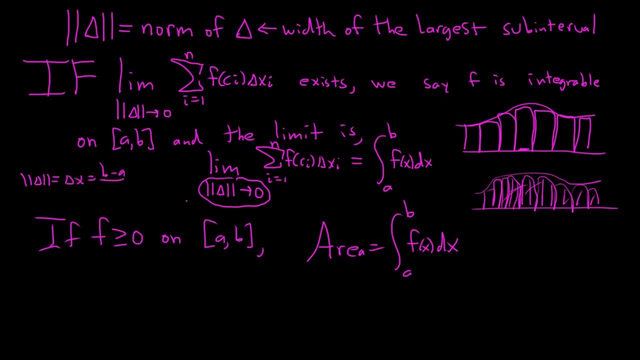 we just got delta x, which was b minus a over n. So if this goes to zero, then n goes to infinity. So if you like, you can replace this with n going to infinity in your mind, and that way you can actually compute it. 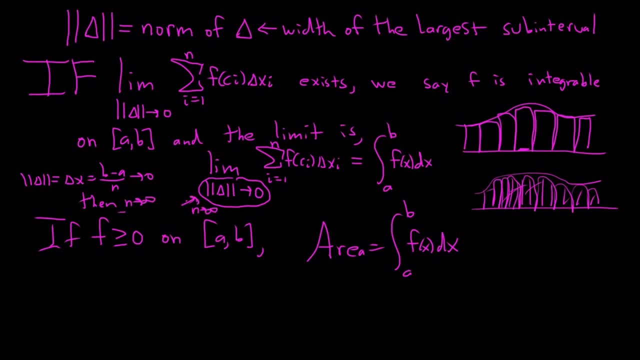 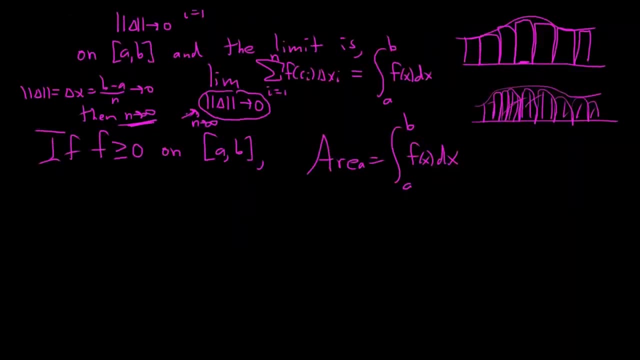 In fact, in the problems that's what we do right. We let n go to infinity, and the reason we do is because we assume a regular partition. So the formula that we tend to use in problems is the following: So the area under the graph from a to b, 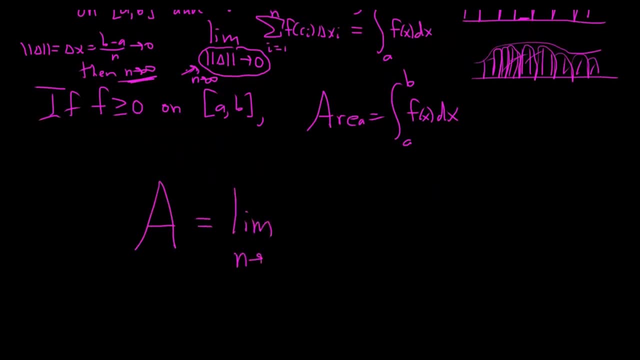 we say it's the limit, as n goes to infinity, Of the finite sum. as i runs from one to n of f of c, sub i times delta x. okay, And so delta x here is b minus a over n. And notice, this agrees with our definition up here, right. 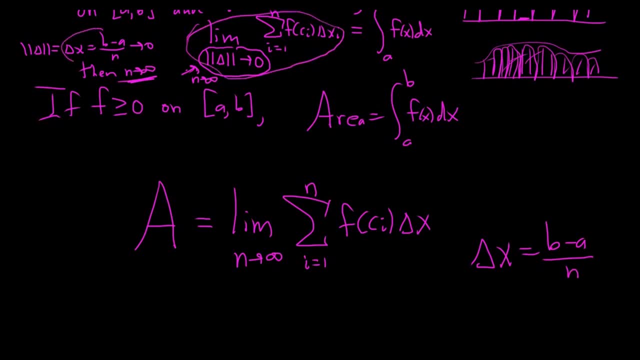 If the length of the largest subinterval goes to zero and delta x is equal to this, that means n must get really, really big. So n goes to infinity. That lets us actually do the computation mathematically. And c sub i. well, before it was any number in the interval. 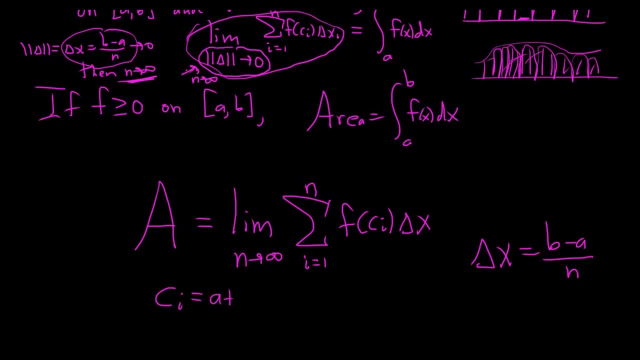 so we force it to be a plus i delta x, So we can actually compute it. This is the right endpoint. So this is the formula we use to find area. So definitely not going to do an example in this video, because they take like 10 minutes. 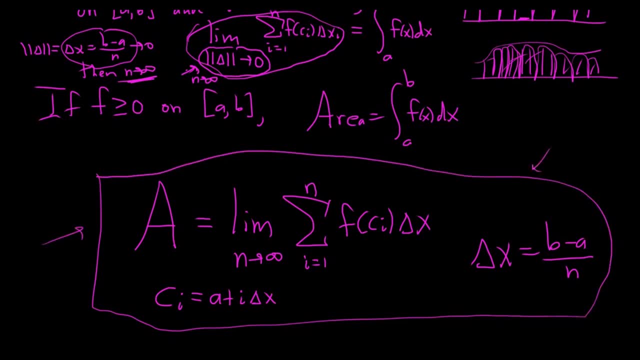 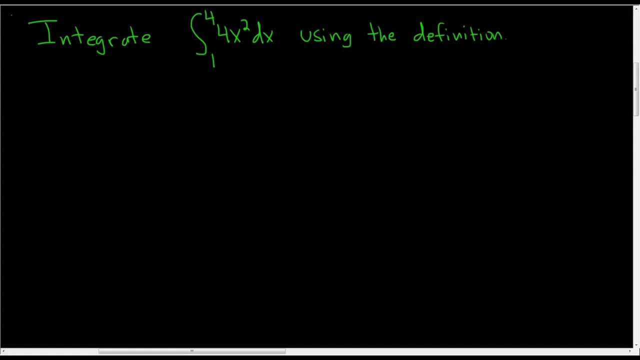 They're really long. You have to work through all of this, But I hope this video was helpful. and yeah, that's it. We're being asked to integrate using the definition so solution. So the goal is to use the formula. 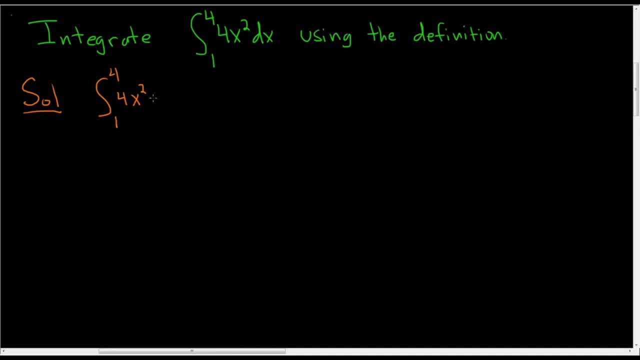 So if we have the definite integral of 4x squared from 1 to 4, this is actually equal to the limit, as n approaches infinity, of the sum, as i runs from 1 to n, of f, of c sub i times delta x. 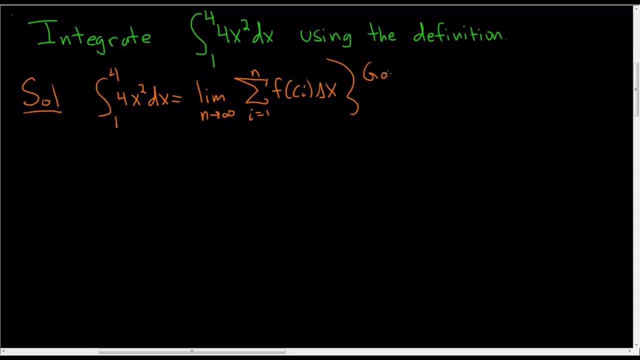 So the goal is to come up with that, So I like to do it in steps rather than do it all at once. So first identify a and b. So a is equal to 1, and b is equal to 4.. a is always the one on the bottom. 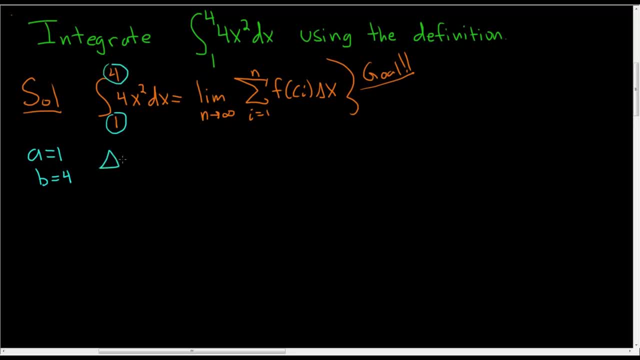 and b is always the one up here- And then compute delta x. So delta x is b minus a. divided by n, b is 4, so you get 4 minus 1 over n and that's 3 over n. So delta x is 3 over n. 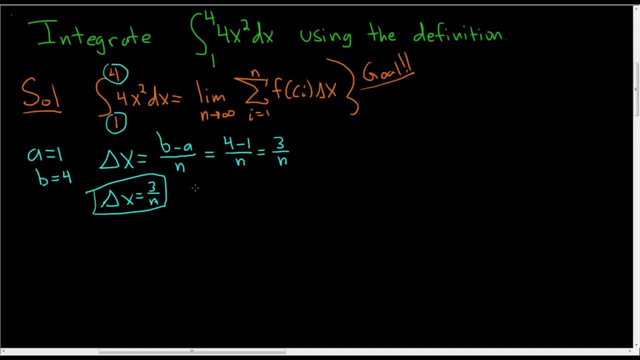 So that part is done. Then I like to write down c sub i. This is the right endpoint, So it's a plus i delta x. a in this problem is 1 plus i times delta x, which is 3 over n. 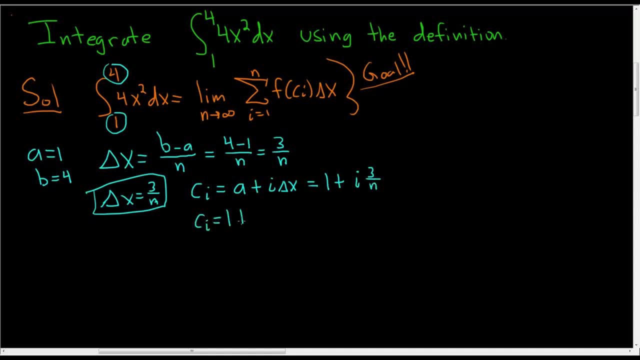 Let me write it again over here: So c sub i is equal to 1 plus 3i over n. So there is our c sub i. But we not only need c sub i, we need f of c sub i. So let's work that out. 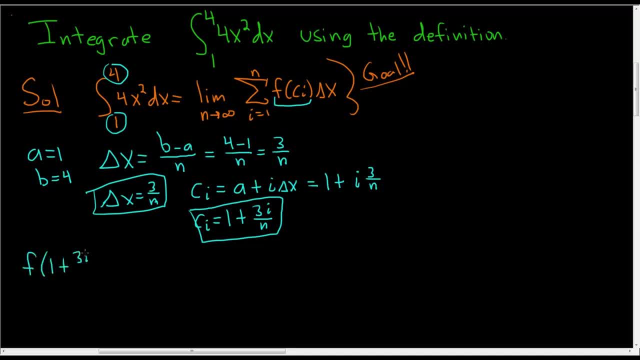 So f of 1 plus 3i over n, You might say: well, what's f? f is your integrand So in this problem, f of x is equal to 4x squared, So this will be equal to 4,. 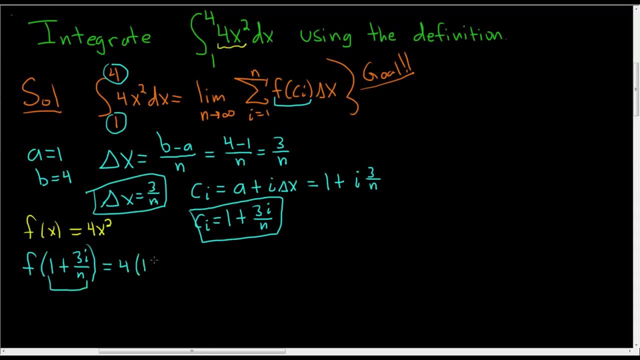 and then this whole thing. here this is our x, So 1 plus 3i over n, and this whole thing here is squared. So this is 4.. Now to square this, let's take the shortcut. So you square the first one. 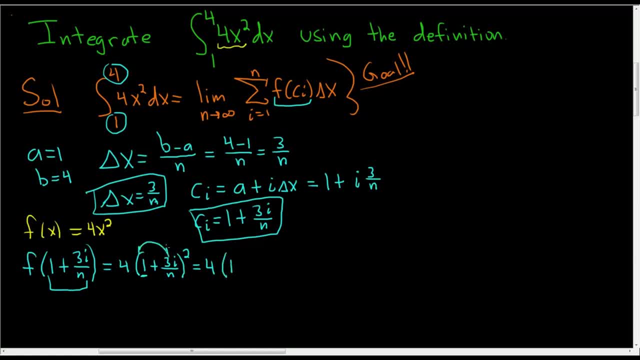 so you get 1, and then you multiply these two and you double it, So 3i over n times 2.. So 6i divided by n plus, and then you square this last term here, So it's going to be 9i squared over n squared. 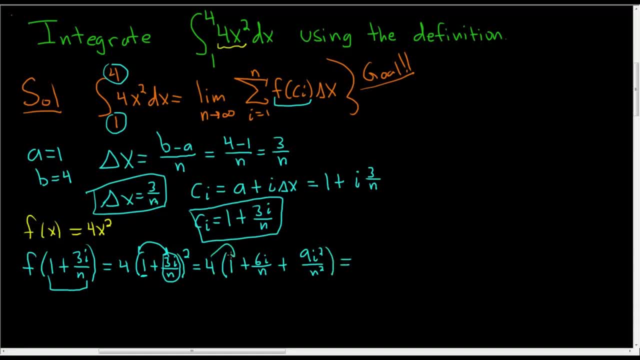 Let's go ahead and multiply the 4 through, So 4 times 1 is 4 plus, and then 4 times this thing. here is 24i over n, and then it looks like the last one is going to be 36i squared over n squared. 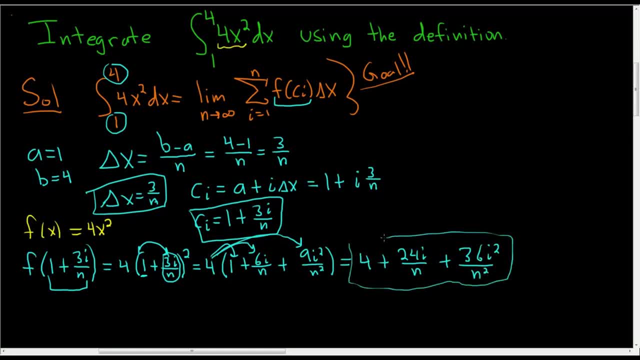 So this here: this is our f of c sub i. So first step is you come up with a and b. That's super easy. Write down delta x. We did that. Write down c sub i. We did that. Take c sub i. 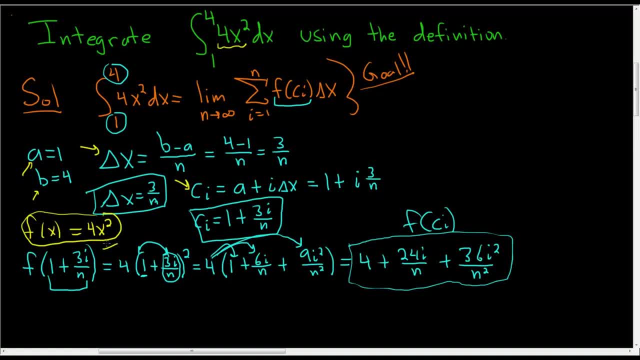 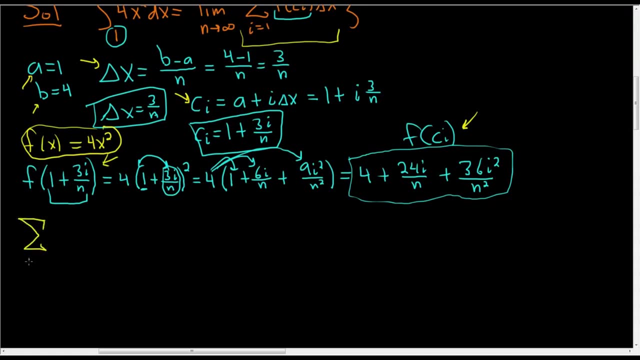 plug it into your function. We did that here and we got it here. Now we just have to take the sum and simplify it. After we take the sum, we'll take the limit and we are done. So the sum as i runs from 1 to n. 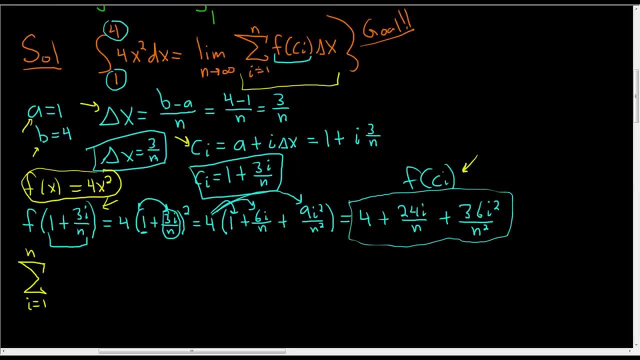 let me scroll up so you can see it. first We have to write down f of c sub i. So that's this. Let's go ahead and write it down. So this is 4 plus 24i over n plus 36i squared over n squared. 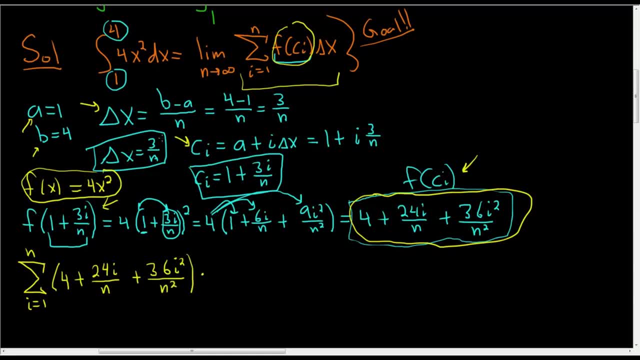 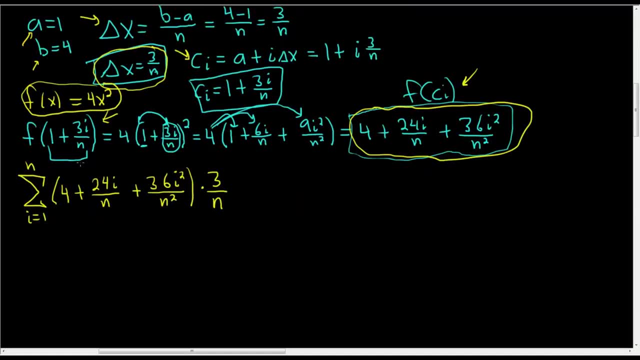 and this is being multiplied by delta x. Well, delta x is here. Delta x is 3 over n. All right, In this next step, I'm going to go really, really slow, because I skip all of the work. I go straight to a form. 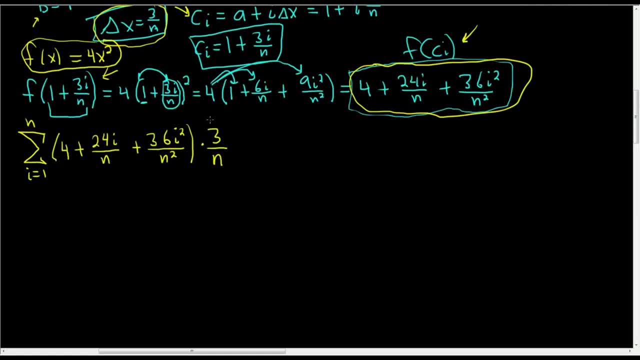 that we can just, you know, do it. So I'm going to take this 3 over n, I'm going to multiply it by 4.. That's 12 over n. That doesn't have any i's, so you can write it outside. 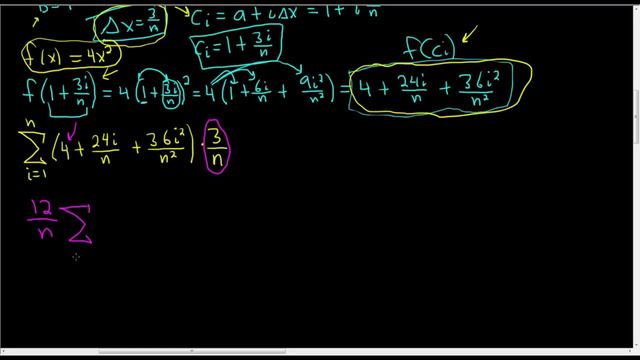 So 12 over n, and then i runs from 1 to n. So if it doesn't have an i, you can write it outside of the summation sign Plus 3 times 24.. That's 72.. So we get 72 divided by. 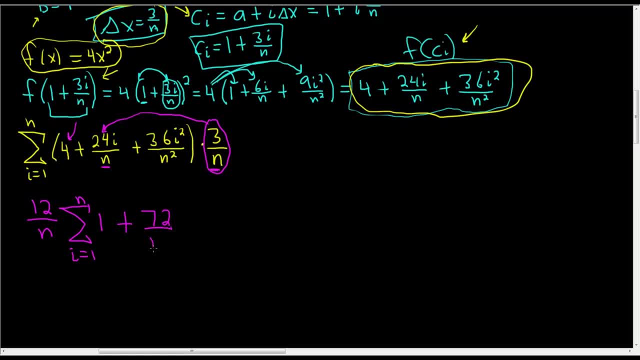 and then n times n is n squared, Then we have the sum, as i runs from 1 to n- of i plus 3 times 36.. So if you can't do that in your head, just go to the side or pick up a calculator. 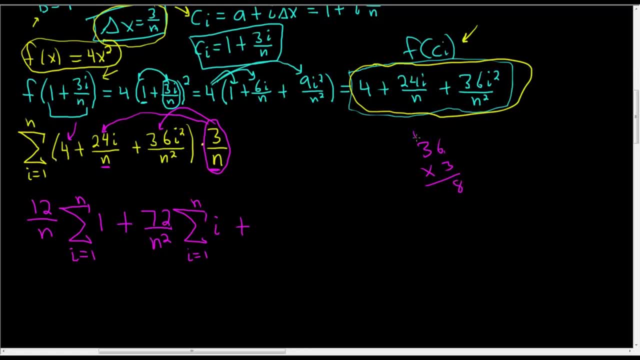 3 times 6 is 18.. You carry the 1.. 3 times 3 is 9.. 108.. Old school, So 108 over. and then n times n squared is n cubed, And then we have the sum. 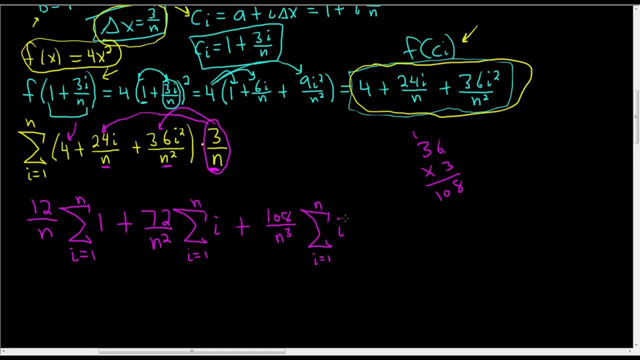 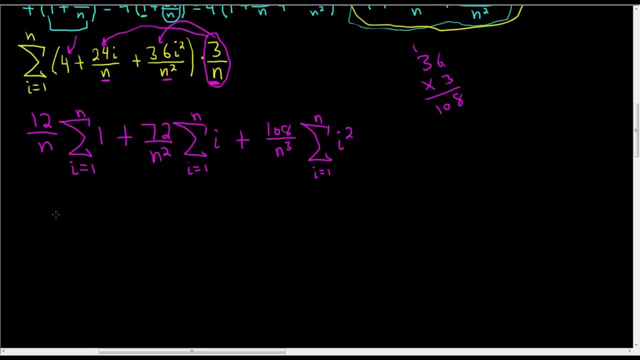 as i runs from 1 to n of i squared. So if it doesn't have an i, you can write it outside. All right, let's go ahead and use the formulas. So this first one is 12 over n, and then we just have n. 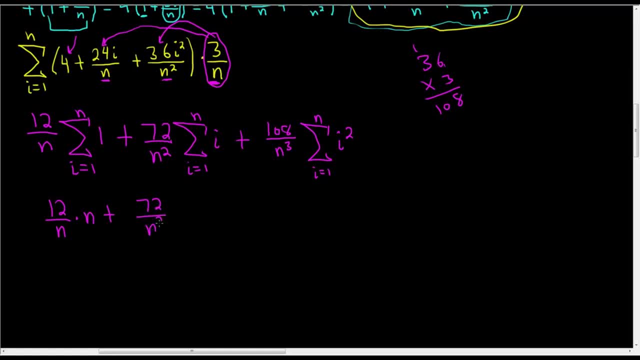 Plus 72 over n squared. All right, you have a 1, so it's just 1 times n, which is n Here. the formula for this is n n plus 1 divided by 2.. Plus 108 over n cubed. 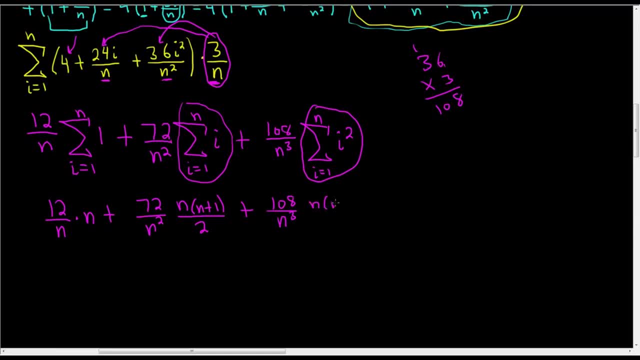 And here the formula for this is n? n plus 1, 2n plus 1, all over 6.. So I guess you do have to memorize these. I actually have them memorized. So here you have a number 1.. 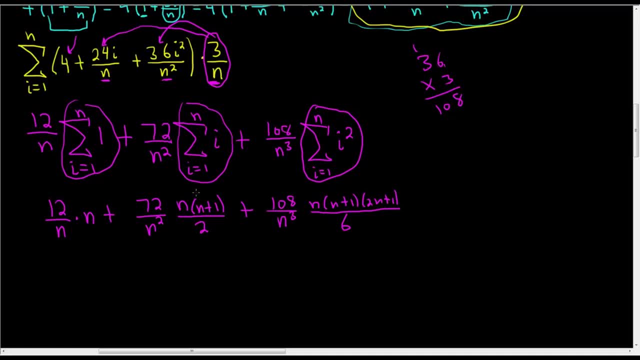 So it's just 1 times n Here, it's this formula here, And then this: here is this here. Let's go ahead and take the limit. You can simplify it first, I won't. So this is the limit as n approaches infinity. 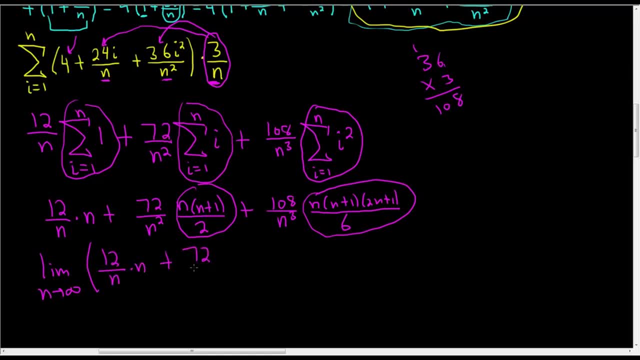 of 12 over n times n plus 72 over n squared. Just writing it down again. I'm not doing anything here, I'm just writing it down really fast. So n n plus 1, 2n, Just copy-paste. 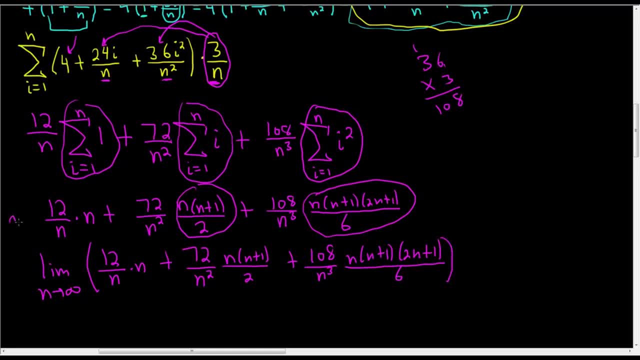 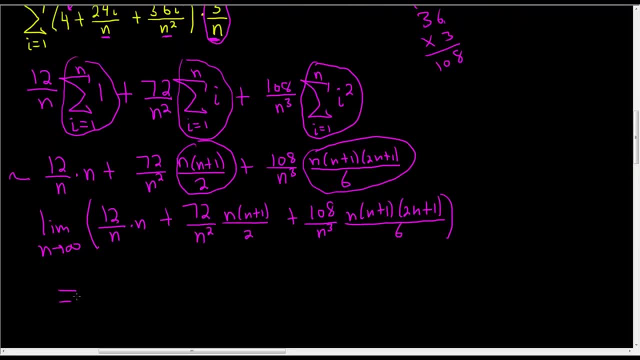 I probably could have cheated And I could have written the limit sign over here, But so all I did was write the limit sign around everything that we had, And now let's take the limit carefully. So this is these: cancel, so you get 12.. 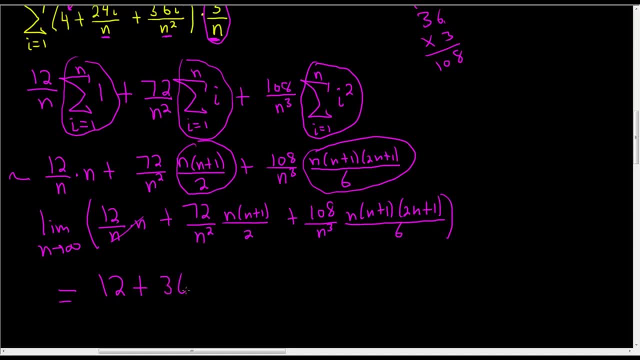 Here you get 72 over 2.. So you get 36.. Right, the degrees are the same n times n is n squared. You have n squared over n squared, So it's just the ratio 72 over 2, 36.. 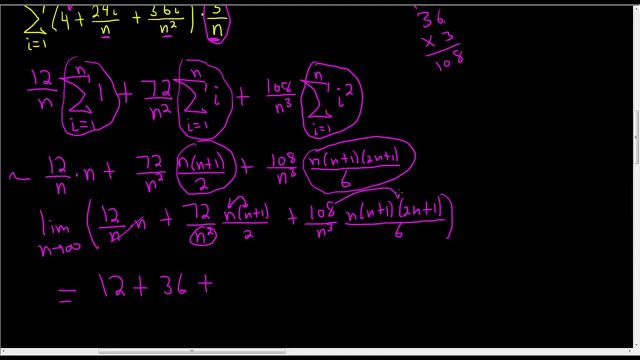 Plus, here you have to be careful. It's 108 times 2 divided by 6. So 108 times 2 divided by 6. So again, these cancel, so you get 12.. That's okay. We have n squared over n squared. 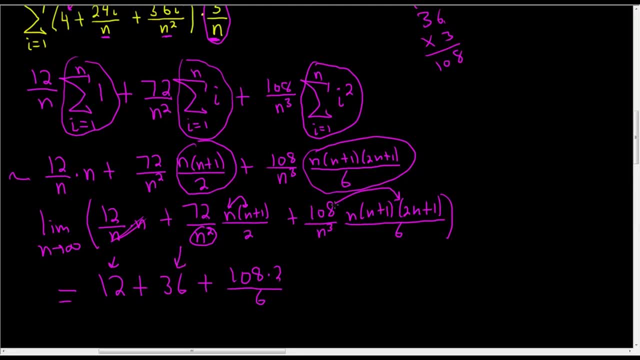 So you just get 72 over 2, which is 36.. And here you multiply 108 times 2, all over 6.. And notice it's n cubed over n cubed. So we can do that. This is equal to 84.. 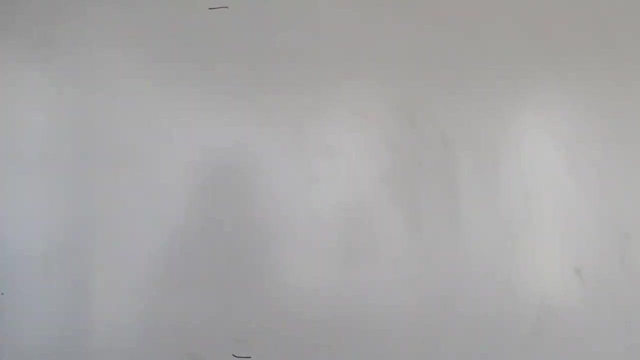 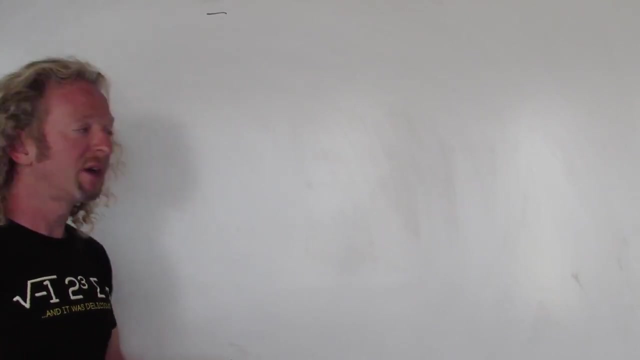 And that's the final answer. Hey, YouTube. In this video we're going to look at one of the most important theorems in Calculus 1.. It's called the Fundamental Theorem of Calculus. We're going to go through the theorem. 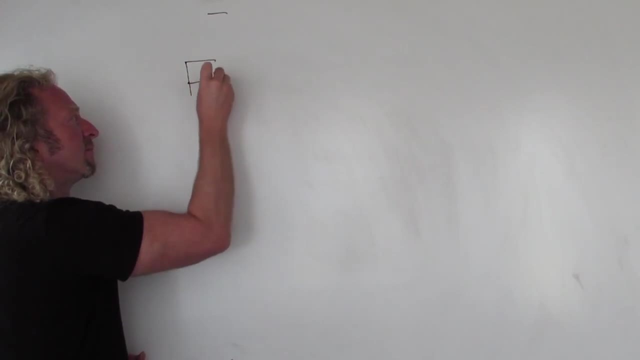 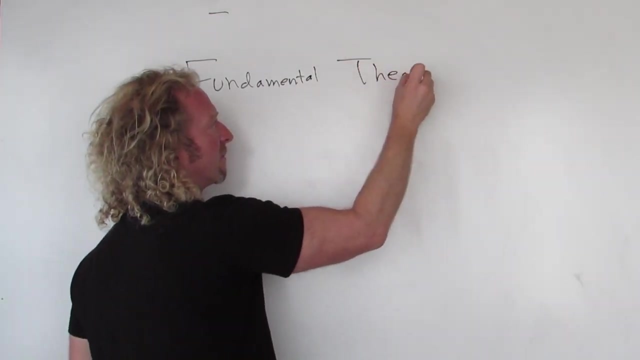 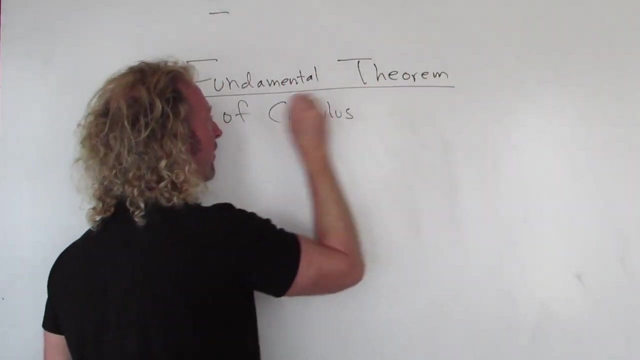 and then do an example of how to use it. Fundamental Theorem of Calculus. Theorem Of Calculus. Fundamental Theorem of Calculus. You can abbreviate it with three letters: F T C, F T C. 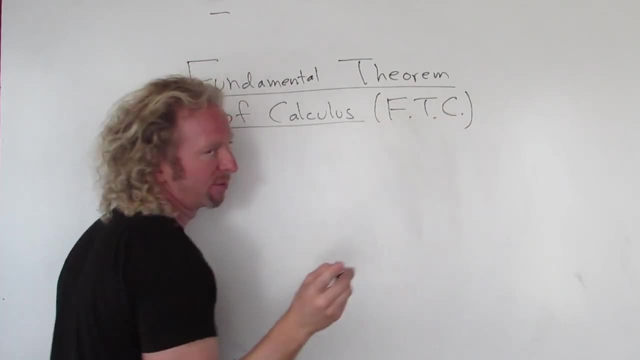 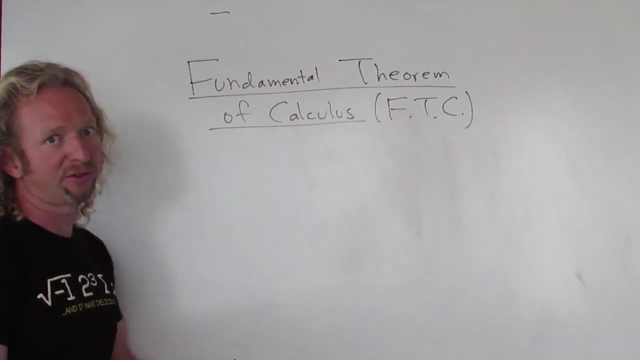 Sometimes people call this the first Fundamental Theorem of Calculus, And the reason is there's actually a second one. There's also an extended version. There's a video for it in the playlist. if you're looking at the playlist, my Calc 1 playlist. 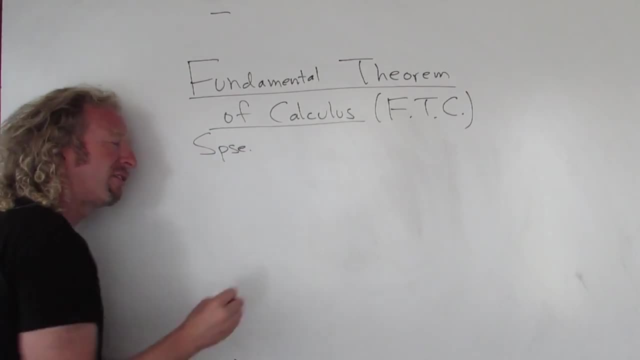 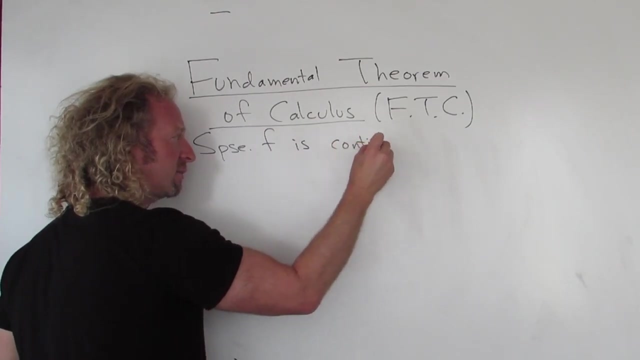 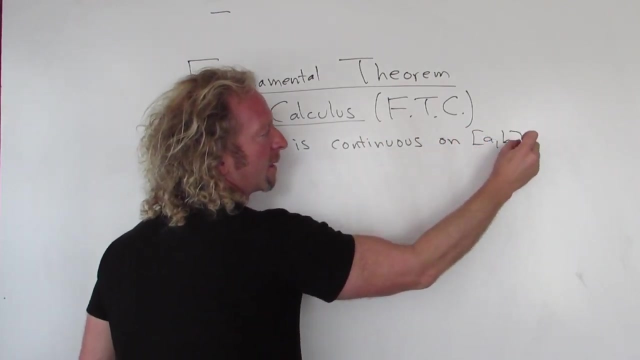 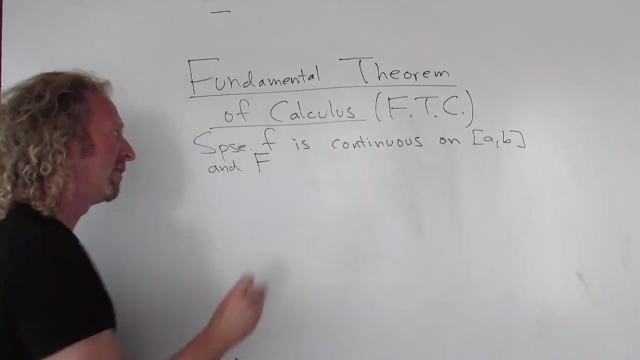 So let's take the theorem. It says: suppose you have a function that's continuous on a closed interval. So suppose F is continuous on a closed interval. Let's say a, b And big F is an antiderivative of little f. 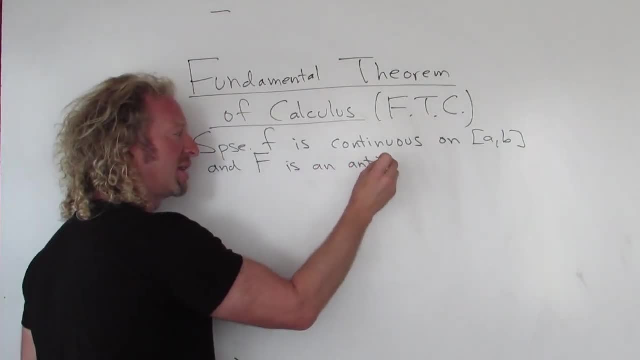 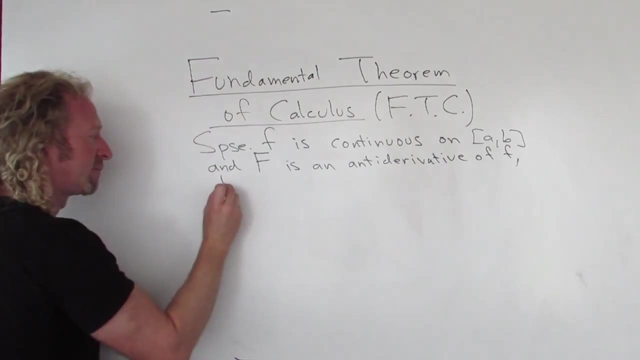 So is an anti. I'll explain what that is. derivative of little f, Then let's pause here for a moment. So we have a continuous function on a closed interval, which seems to be a very common requirement for all of the theorems. 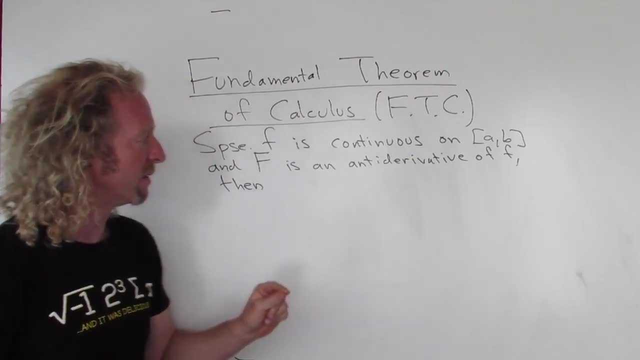 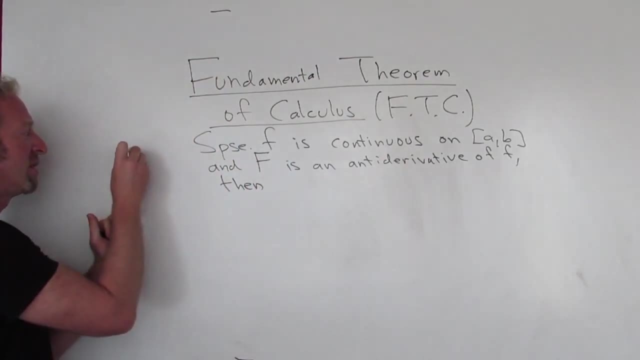 in calculus And big F is an antiderivative. So what does that mean? That means if you take the derivative of big F, you get little f. So for example- I'll write it here- Say: big F is x squared. 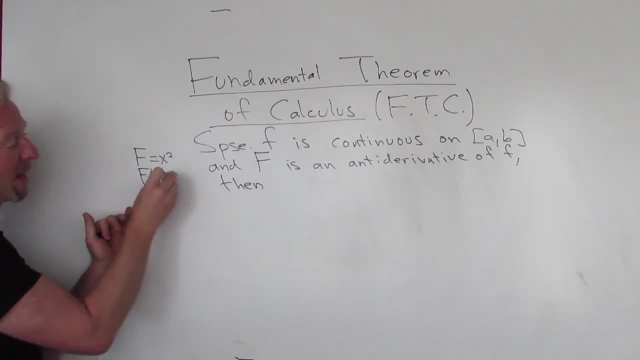 So if you take the derivative of big F, you would get 2x via the power rule. This would be little f. So if you take the derivative of big F, you get little f. In other words, if you integrate little f. 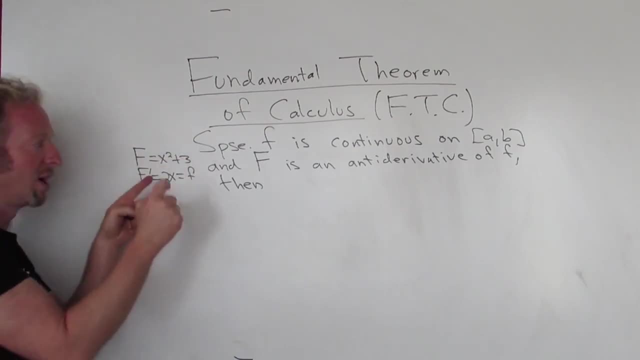 you get big F. Now you could add a number here and nothing would change, right, Because the derivative of a number is zero. You could add c here, then big F would be the general antiderivative. That's what it's called. 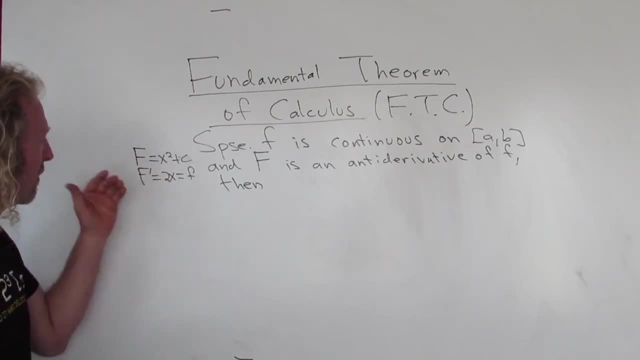 It's called the general antiderivative. So basically, if you differentiate big F, you get little f, Or if you integrate little f, you get big F. Same thing, All right. So suppose F is continuous and big F is an antiderivative. 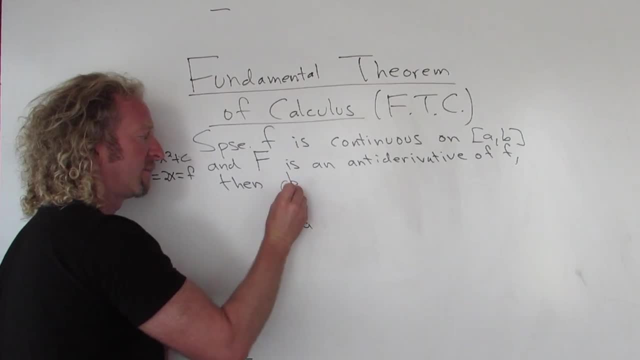 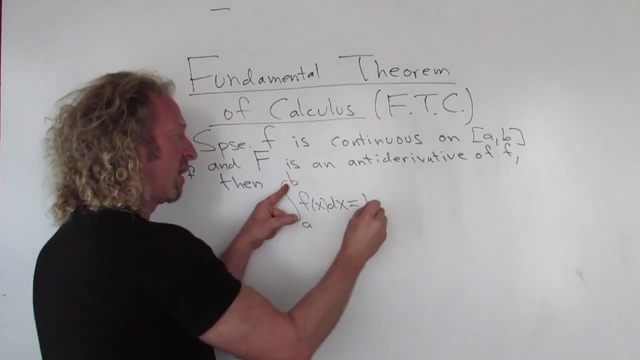 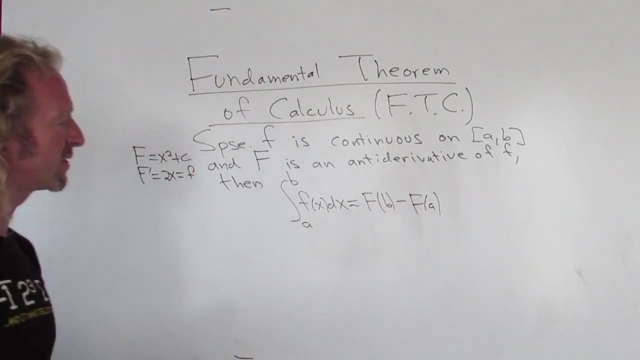 of little f, Then the definite integral from a to b of little f with respect to x is equal to big F of b minus big F of a. So this formula lets us avoid the long way of computing definite integrals. Remember. 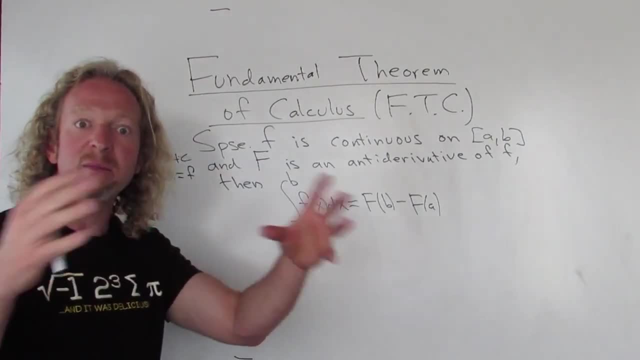 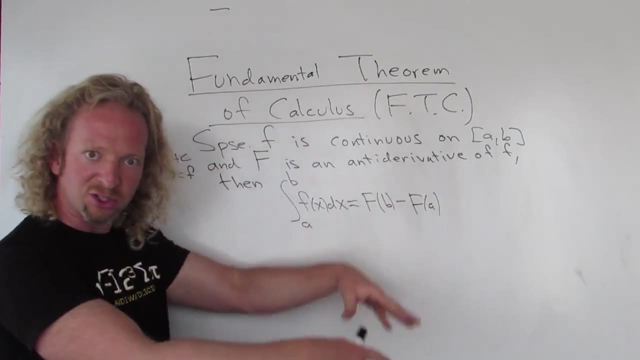 the long way is the limit process, the limit definition. when you have delta x and delta y, You take a limit of a sum and you have to use all those formulas. It's a huge, huge, long problem. Those days are gone. 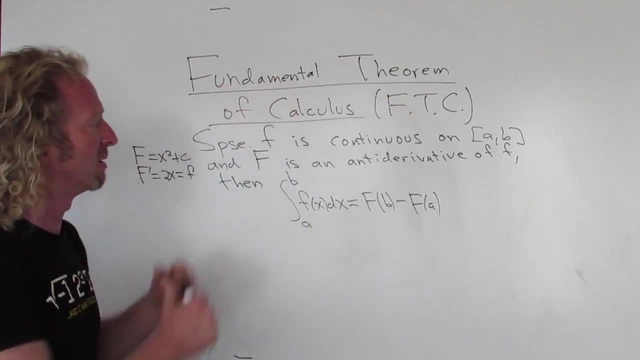 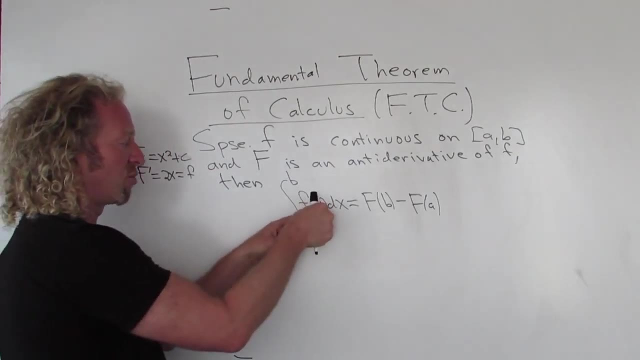 All right. So this is the easy way to do definite integrals. That's what this theorem is about. Okay, That's what it's used for. It connects differentiation and integration. right, because you can think of this as the derivative. 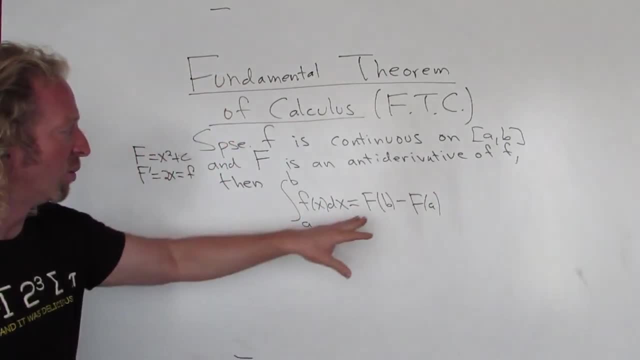 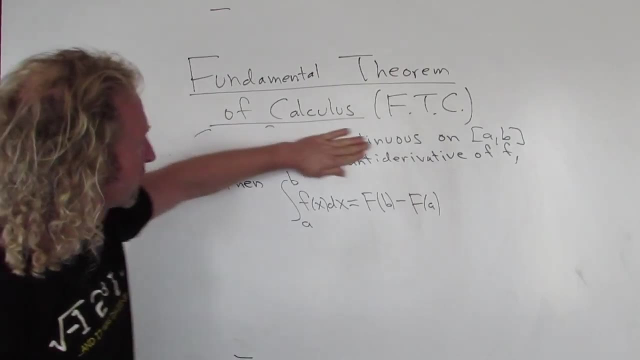 of big F. So when you integrate the derivative, you get this other creature here which involves the antiderivative. Okay, And I'll show you how to use it. So let's do it. So let's see, Let's say we have. 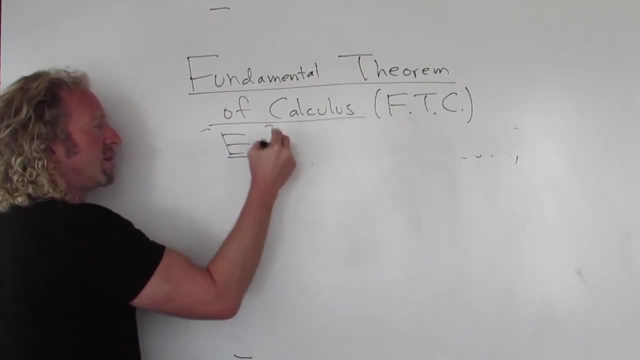 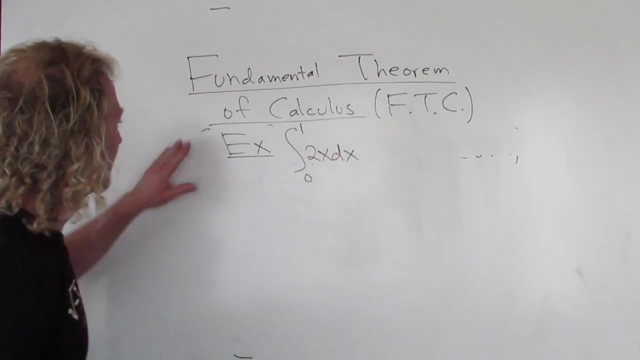 let me, let me, let me write, get some more room. Say, we have the definite integral from: let's keep it really simple: 0 to 1, 2x dx. Okay, 2x dx. So if you want to use, 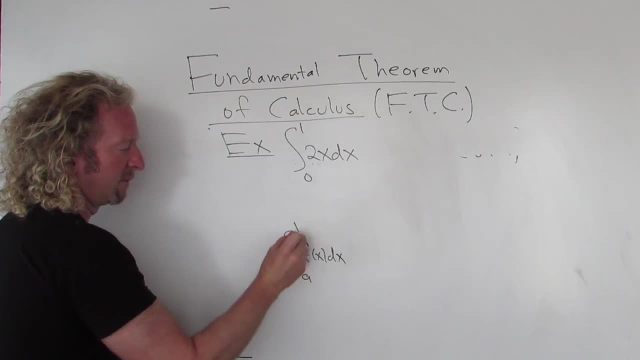 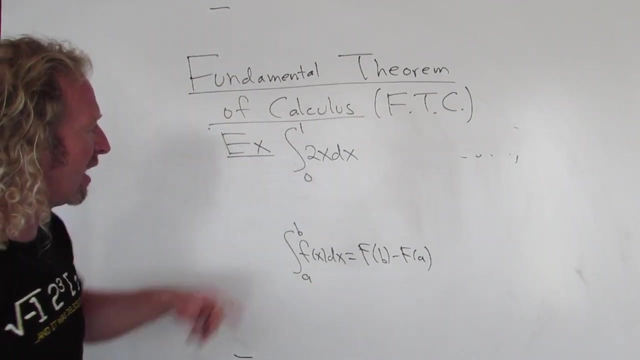 the formula which I'll write down here. so the formula says that the definite integral from A to B is equal to big F of B minus little f. So you can identify your little f, And this is not how people do it. 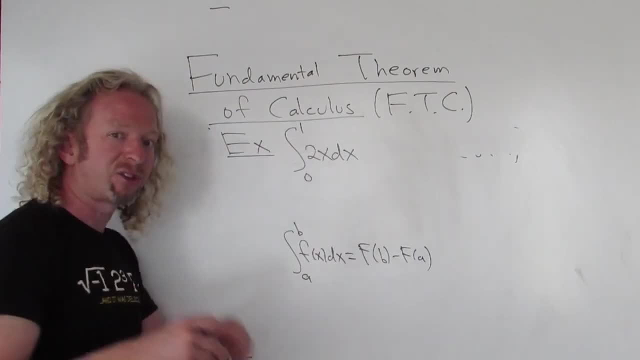 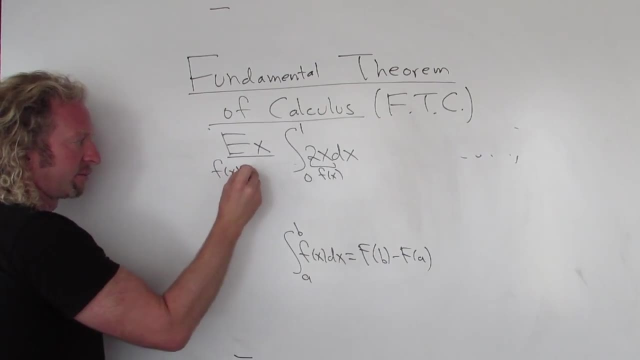 by the way, I'm just going to go through it first and show you how to use the formula carefully, and then I'll show you how people do it. So I'm going to call this little f, So little f of x. 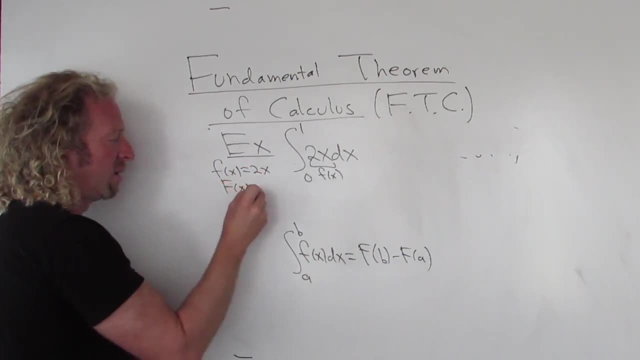 is equal to 2x, So we have an antiderivative of little f, So you would just integrate it. When you integrate this, you get 2, and then you add 1, right, So big F of x. 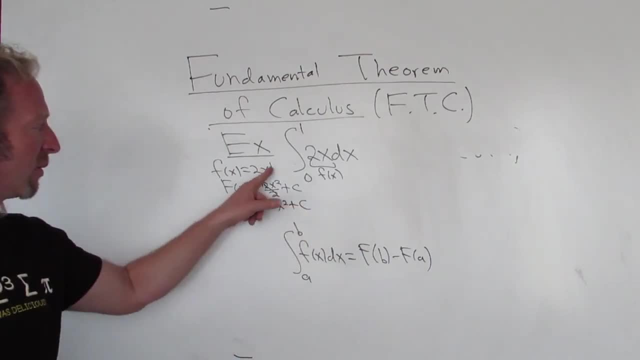 would be x squared plus c, right? Just use the power rule to integrate, end up canceling, and that would be the most general antiderivative. That's called the general antiderivative of this function. Alright, so now we just plug in. 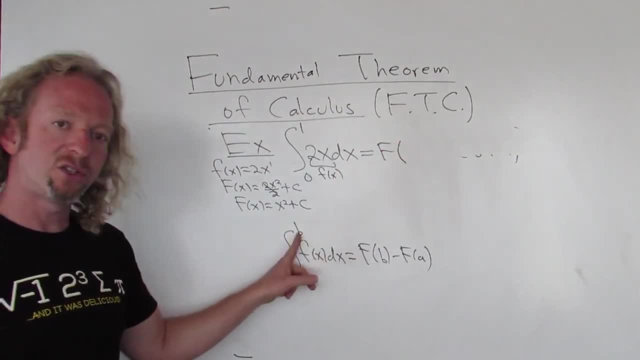 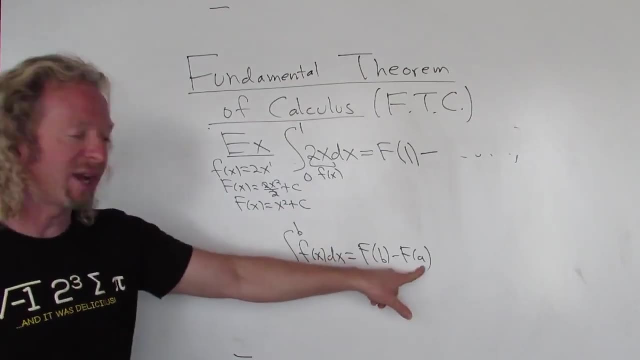 the numbers. This would be big F of, and then B is your first number, right? So that goes here. So B minus and then big F of 0.. So that's your A, So minus big F of 0.. 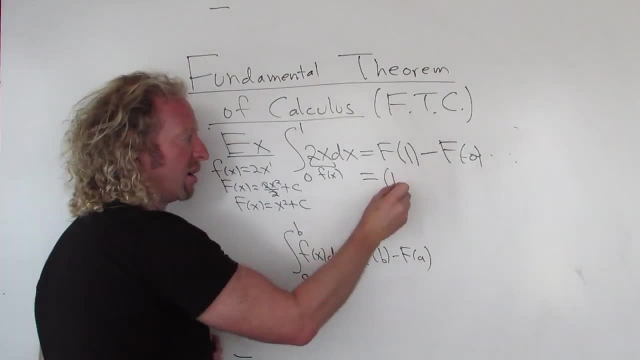 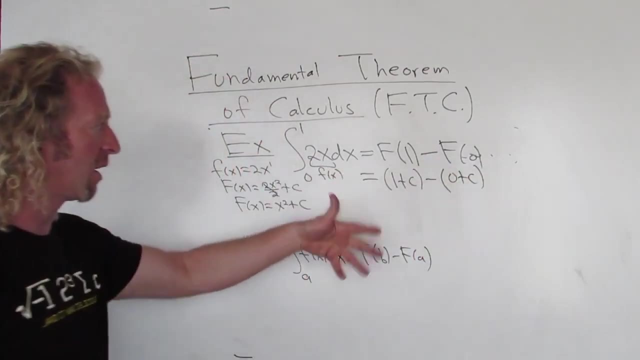 You plug in the numbers right, So you would get 1 squared plus c or just 1 plus c. So 1 plus c minus and then 0 plus c, right, 0 plus c. It's instructive to do this. 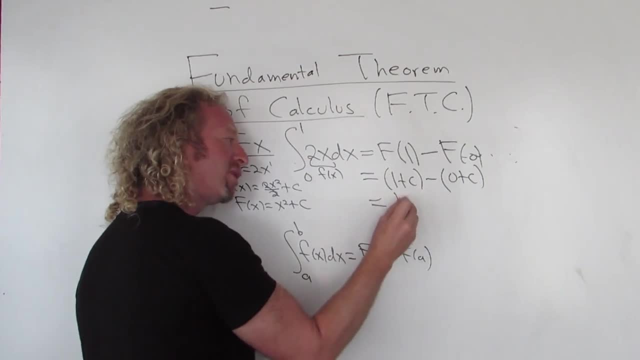 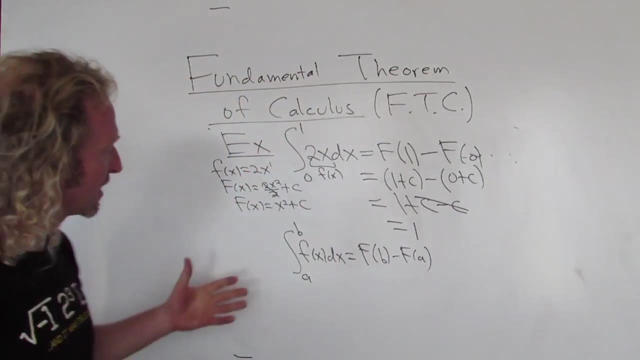 This is not how normal people do. this I'll show you in a minute, but it's good, It's worthwhile. So here we get 1 plus c, minus c and the c's cancel right. So the answer is 1,. 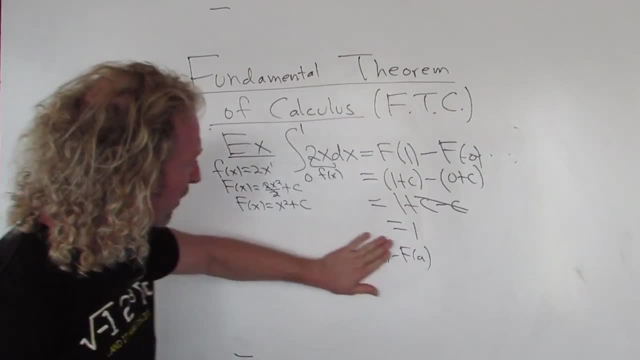 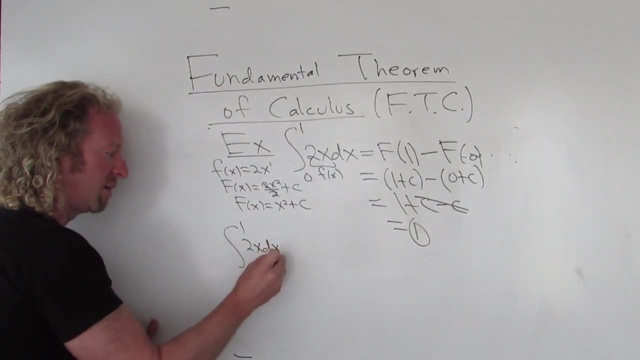 right. The answer you get here is 1.. So how would you do it if you didn't want to stick to the formula, if you just wanted to do it The shorthand way? the way people do it is typically well. 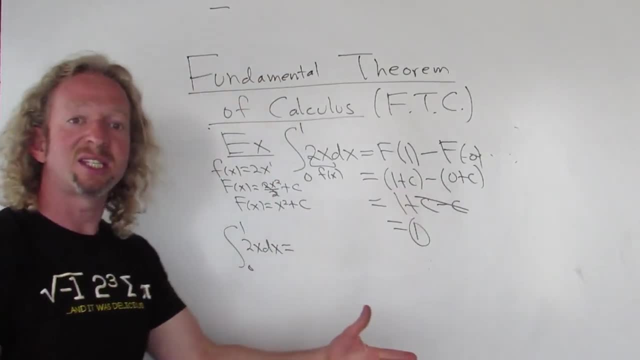 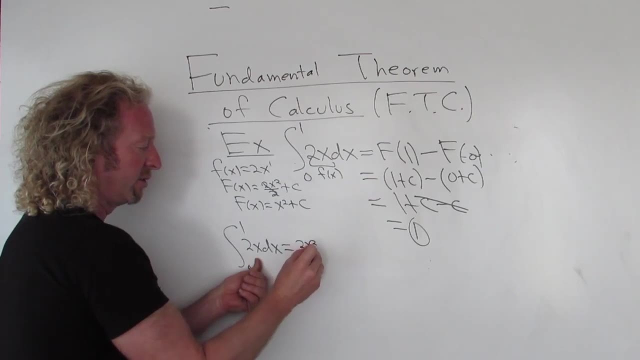 first of all, they don't write the c. As you notice, the c's cancel, so it's not necessary to write the c. So what you would do is you would just integrate this and you would ignore the c. So 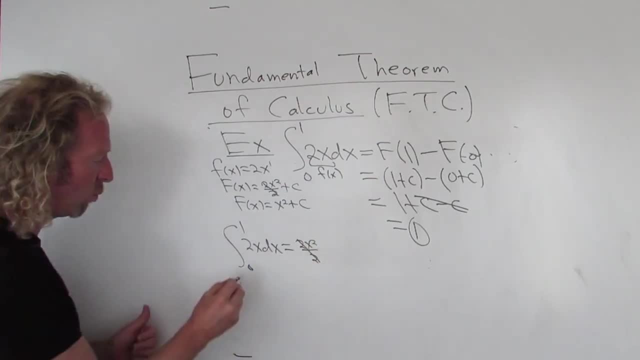 you would get 2x squared over 2. So the 2's cancel, So you would just get x squared. And then there's a couple ways to do it. You can use this number here and this number here. 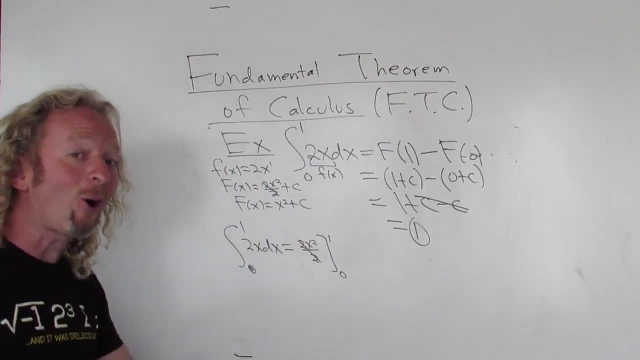 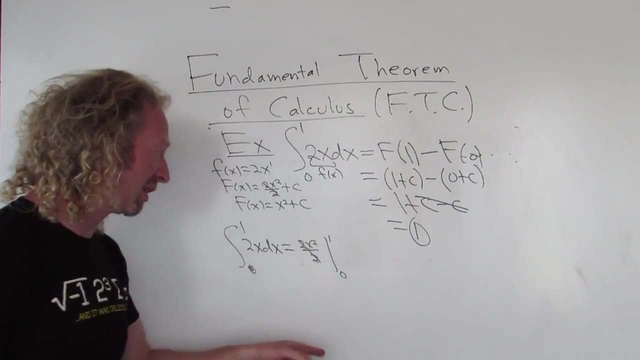 Or you could use one bracket, Or, if you're really lazy, you can just use a line. So those are the three ways I've seen. So double bracket, single bracket or just a line, And then you just plug in the 1.. 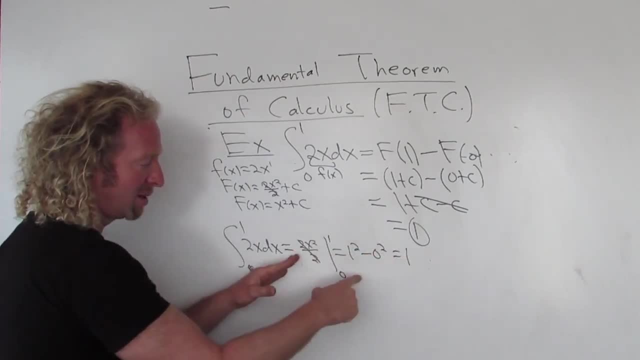 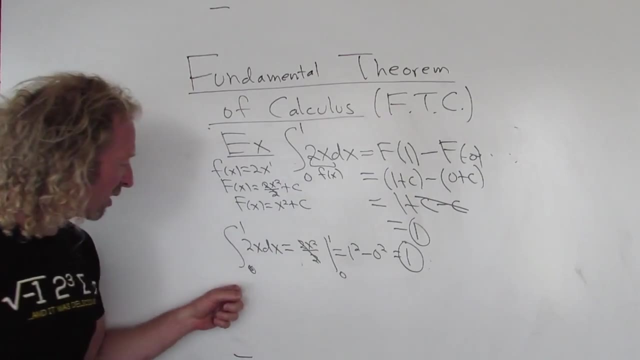 So you get 1 squared, You subtract and you plug in the 0. And so you get 1.. So you integrate, don't write the c. plug in the number. subtract, plug in the number and that's the answer. 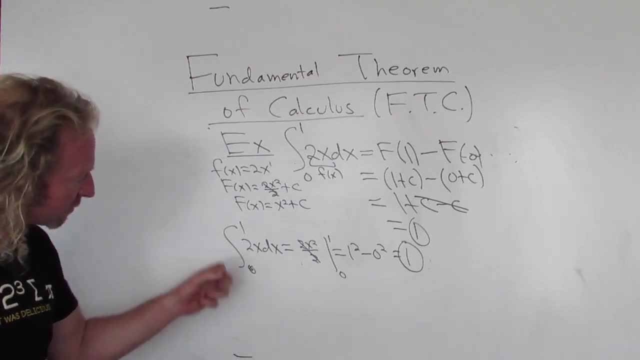 So you have limits of integration. That's called the lower limit, That's called the upper limit. Don't write the plus c. If it's a definite integral, don't worry about the plus c. What does this number mean? Ah, 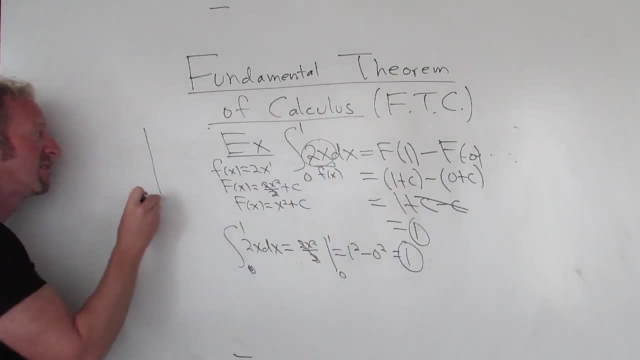 Well, in this case, since this function is non-negative, right, it's up here. So, whoops, whoops, whoops, let's do that again. So this is the line 2x and we're going from 0 to 1.. 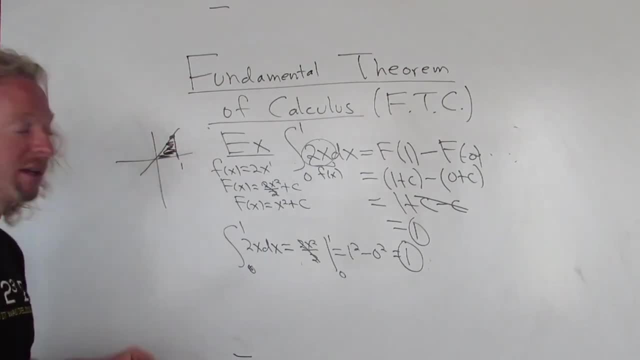 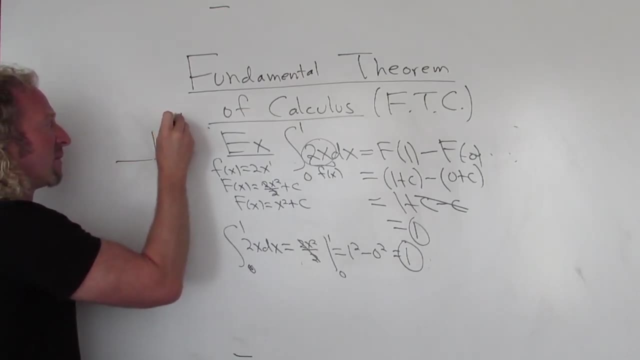 Right. So we're finding the area of this triangle right. So we found the area of the triangle using calculus. let's be bold. This line here is 2x, So the y value, when x is 1, is 2.. 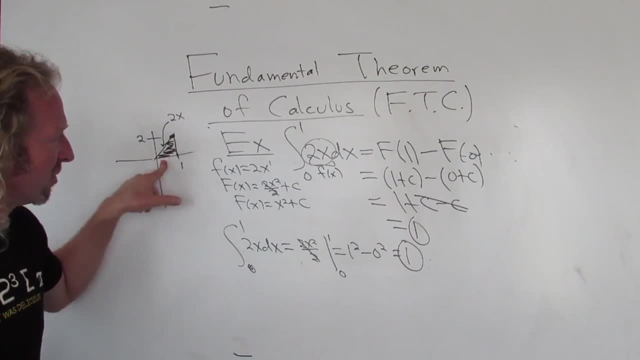 We should be able to find the area of this triangle using geometry right. Remember the area of a triangle. just for fun, it takes a second 1 half base height. Why not right? The base here is 1.. 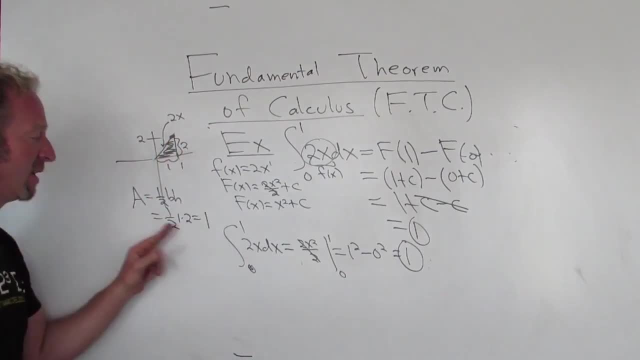 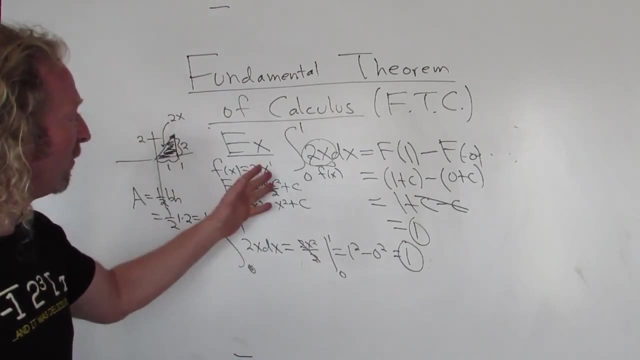 The height here is 2.. Boom, We get 1.. So via geometry we get 1, and via calculus we'll get 1.. So pretty cool. Anyways, hopefully, what you get from this video is whenever you have a definite integral. 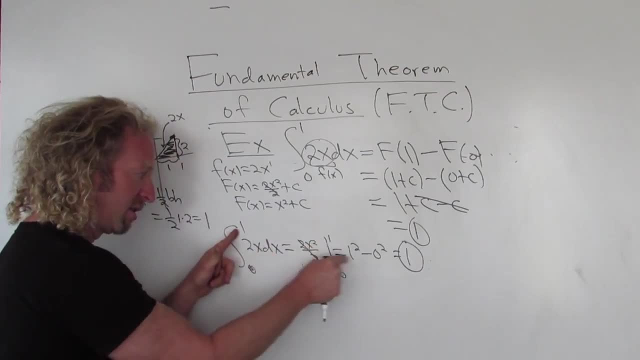 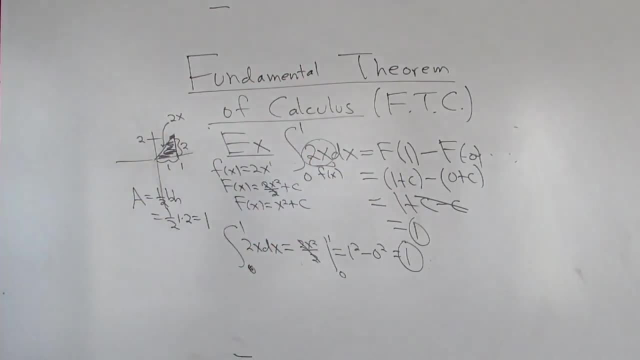 don't worry about writing the plus c and then just plug in this number, first subtract and plug in the bottom number. I hope this video helped. Thanks for watching and see you next time. So we have a definite integral. 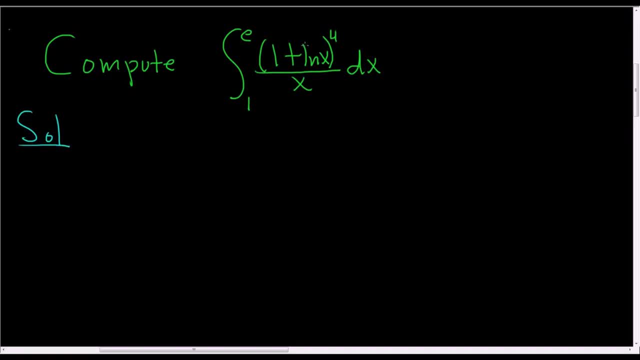 Let's go ahead and work it out. Solution: So we need to make some type of u substitution, and the obvious choice, I guess, is this piece here, Because if we let u be equal to 1 plus the natural log of x, 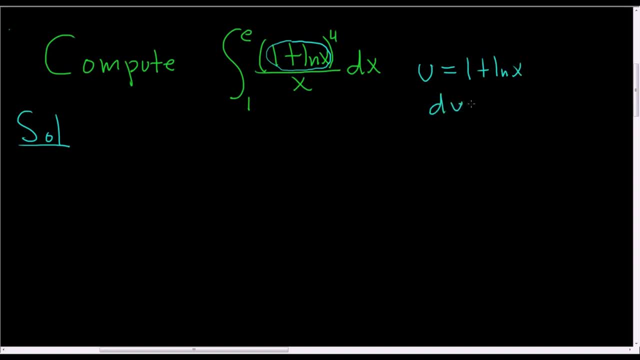 then du is well, the derivative of 1 is 0, and the derivative of ln x is 1 over x, dx. So you need to have some foresight when you're picking your u. You need to pick a u. that's going to lead to a du. 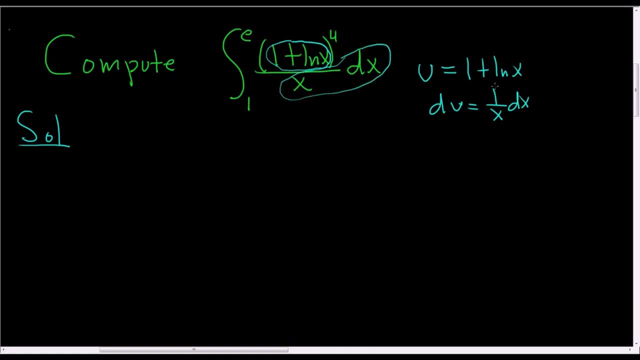 that somehow appears in the integrand and it does right. 1 over x, dx is right here. Before we rewrite our integral, we need to change the limits of integration, because these limits are in terms of x, and now we're changing everything to u's. 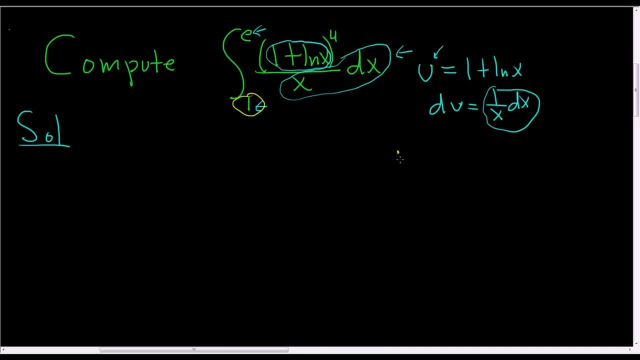 So let's carefully do that. So we'll start with the 1.. So when x is equal to 1, let's work out the u. So u is equal to 1 plus the natural log of 1,. 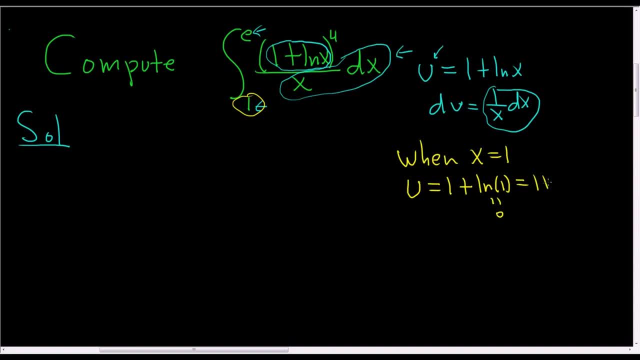 and the natural log of 1 is 0. So this is 1 plus 0, which is 1.. And then now we'll do the upper limit of integration. So when x is equal to e, we end up with u equals 1 plus the natural log of e. 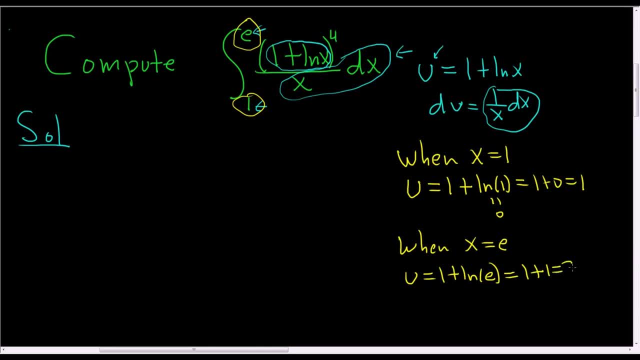 and that's going to be 1 plus 1, which is 2.. Alright, now we're good to go. We have the definite integral. Let's see: When x is 1, u is 1.. When x is e: 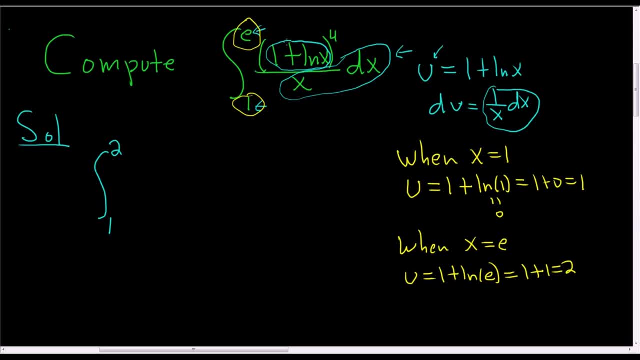 u is 2.. Got to be really careful. And this piece, here is u to the fourth, and then we just have du, Wow, that cleaned up, nice right. This is u and it's being raised to the fourth power. 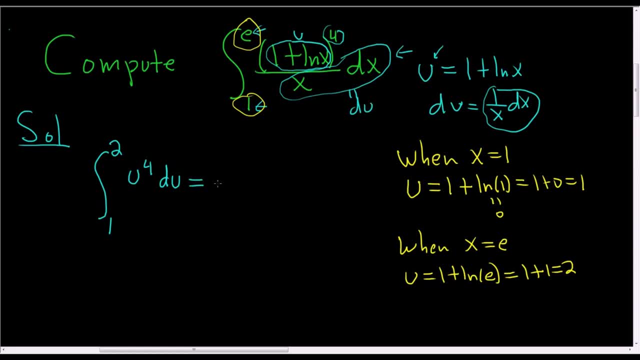 and then this piece here is just du To integrate this. we'll just use the power rule. So this is u to the fifth over 5, and we're going from 1 to 2, and first we plug in the 2,. 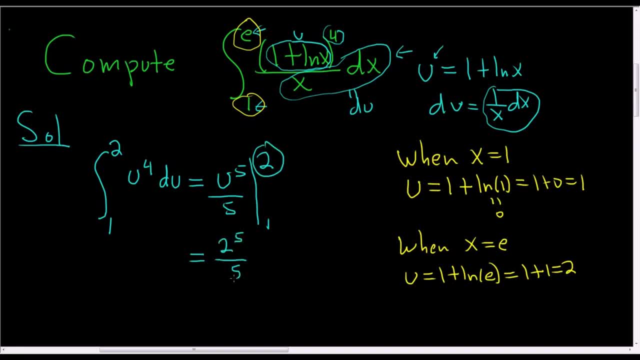 so we get 2 to the fifth over 5.. We subtract and we plug in the 1,, so 1 to the fifth over 5.. 2 to the fifth is 32, so 32 over 5.. 1 to the fifth is 1,. 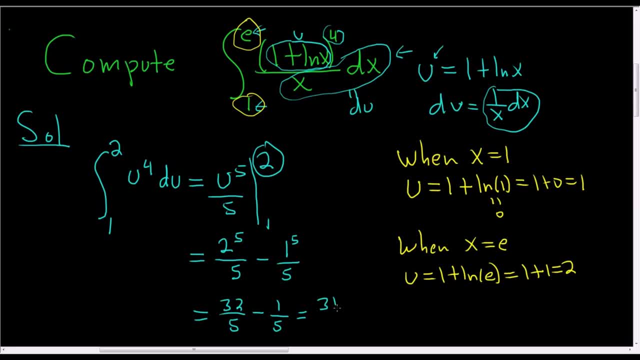 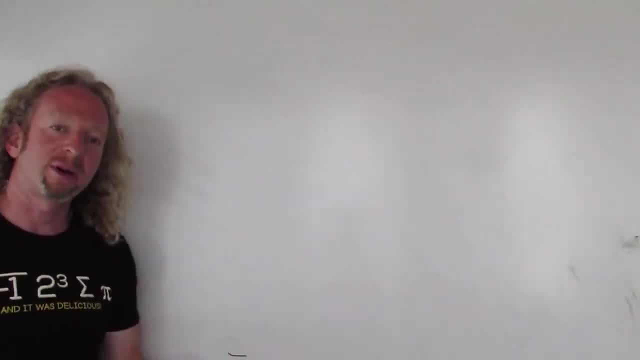 so 1 over 5. And 32 minus 1 is 31. And that is the final answer. Hey, YouTube, In this video we're going to talk about a really important theorem from calculus. It's called the mean value theorem for integrals. 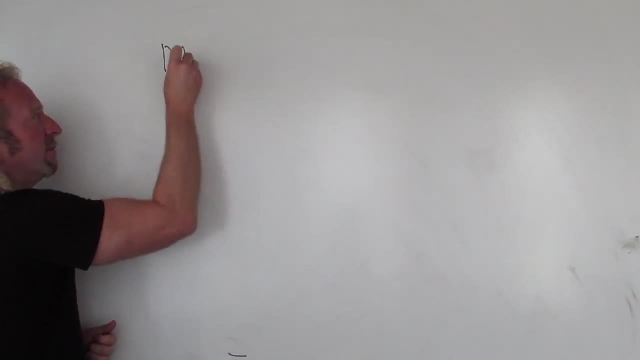 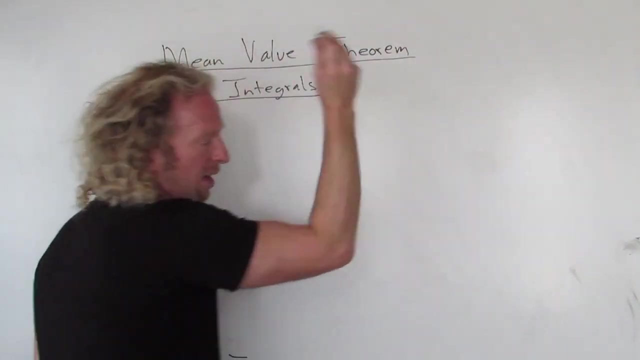 Let's go through it very carefully. So mean value theorem for integrals. We're also going to talk about something called the average value of a function over an interval. That's kind of almost like a consequence of this in our discussion. So 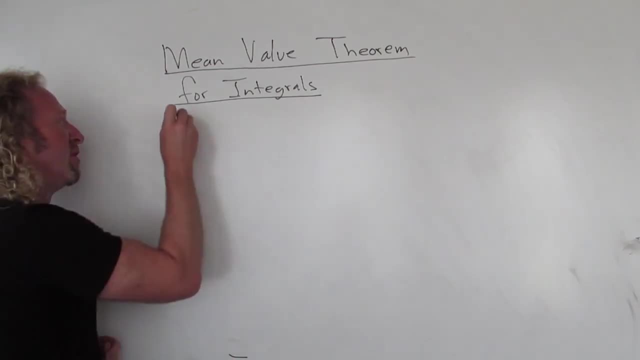 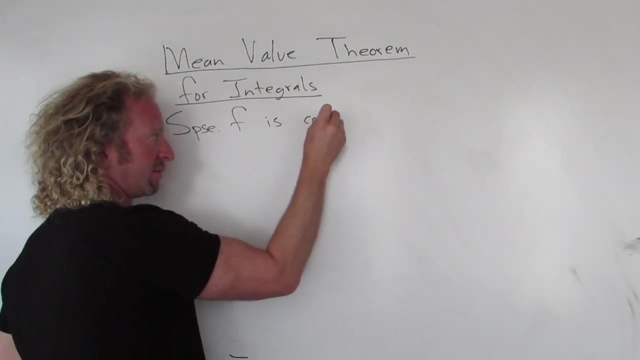 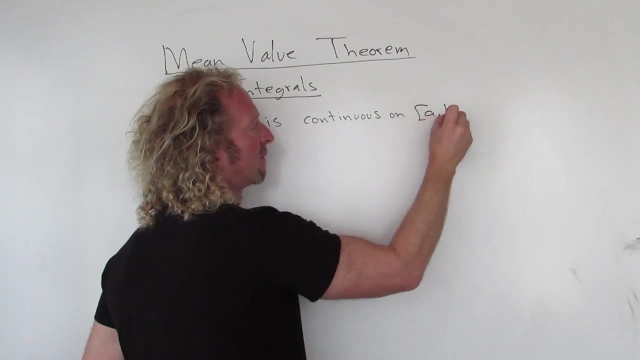 first we'll state the theorem and then we'll go through the picture. So suppose you have a continuous function. So suppose f is continuous on the closed interval. so on a b, So on a b, Okay. 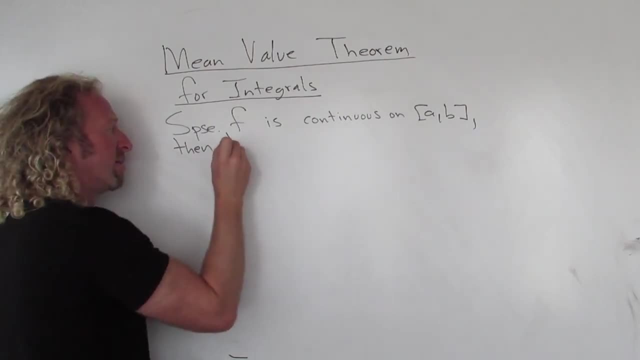 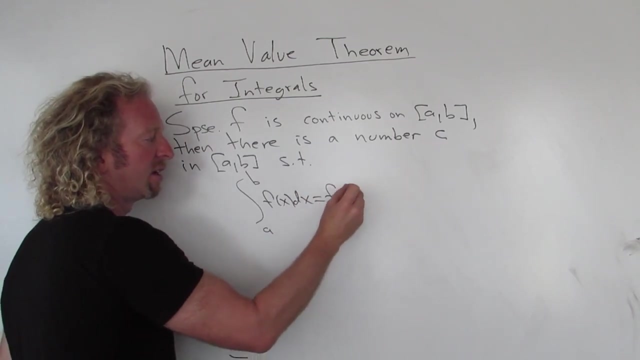 Then you can find the number. So then there is a number, There is a number c and the closed interval a, b, such that the definite integral from a to b of f of x with respect to x is equal to f of c times b minus a. 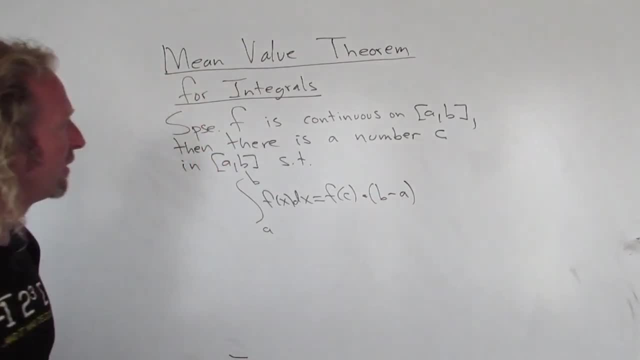 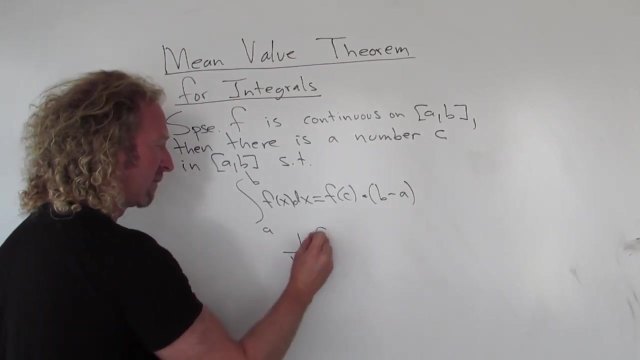 Okay, b minus a. So that's the statement of the mean value theorem for integrals. Okay, If your function is integrable, in other words, if you can integrate it. there is another result that shows that the quantity 1 over b minus a. 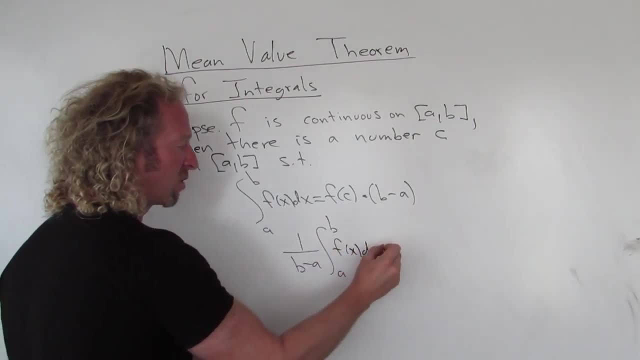 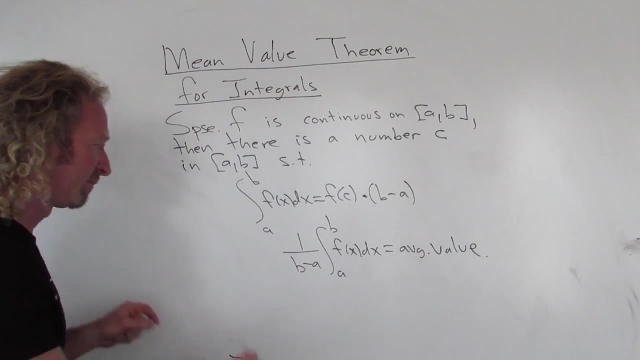 a to b, f of x to the x is called the average value. So if you assume everything is good and it's continuous, you can think of this as f of c. So if it's continuous, this is called the average value. 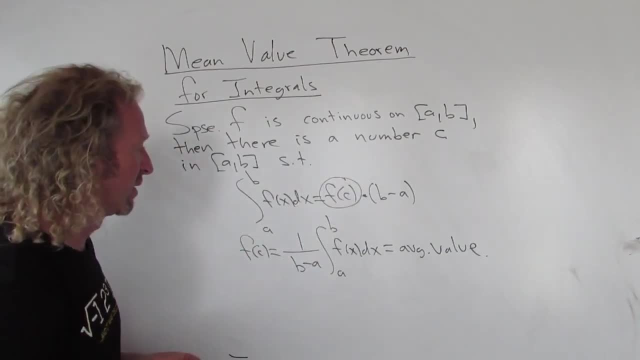 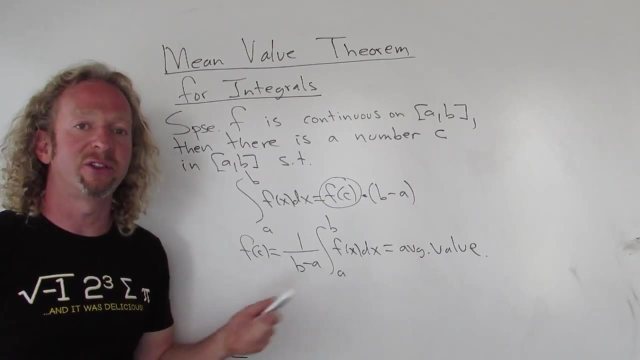 So f of c is called the average value of the function. So the mean value theorem for integrals is deeply connected with the average value of the function. f of c is the average value of the function. Let's draw a picture so you see what all of this is. 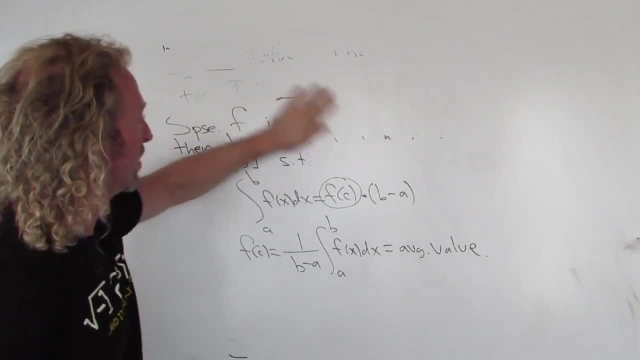 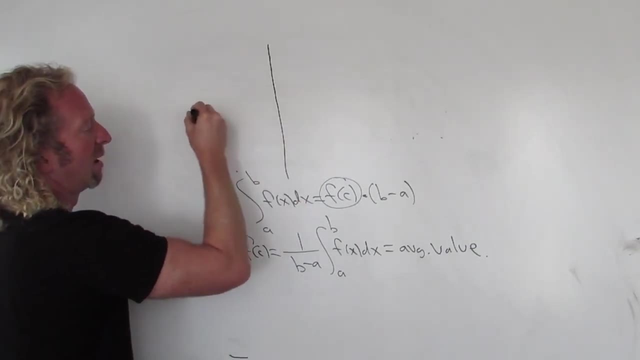 It's really, really interesting. So I'm going to erase this because we don't need it anymore And I'll draw the picture up here. So this will be our y-axis, This will be our x-axis, So. 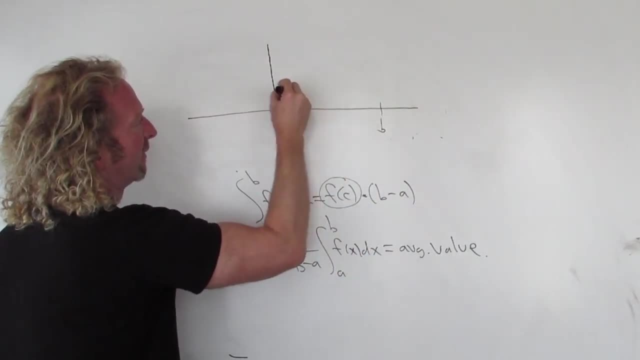 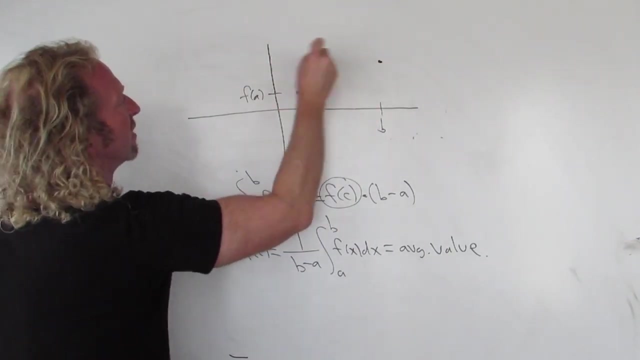 here's a and here's b. Okay, I'm going to be careful. here, This is f of a, All right, And then maybe here, this is f of b. So this is f of b, Good stuff. 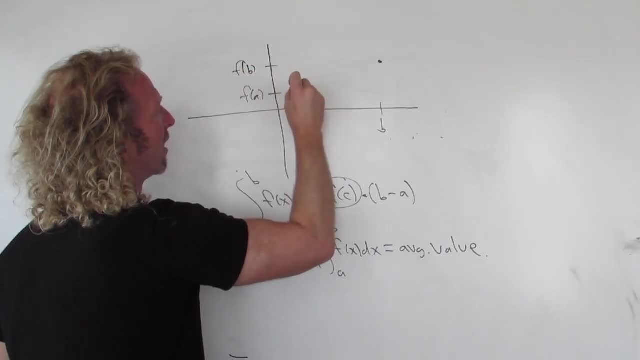 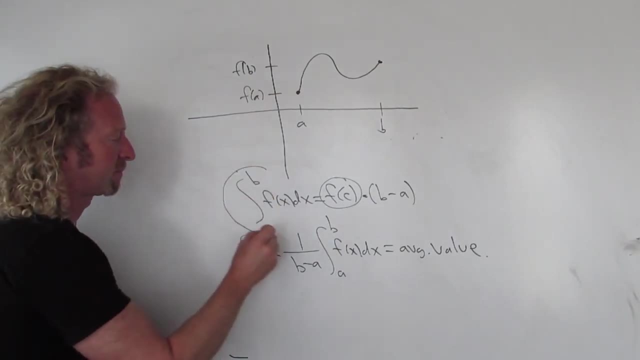 And then maybe draw it like this: There we go, All right, There's our function, And so first let's examine this. This is the area under the curve Right. So this area here is the area under the curve. 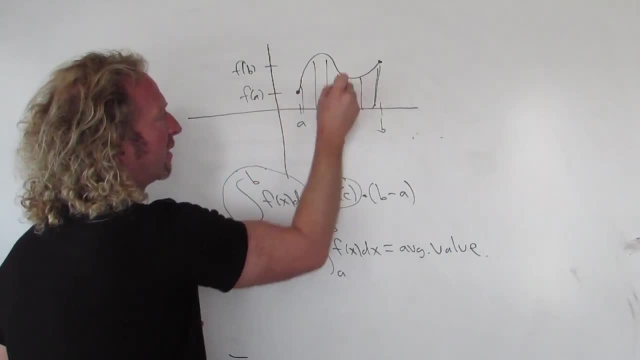 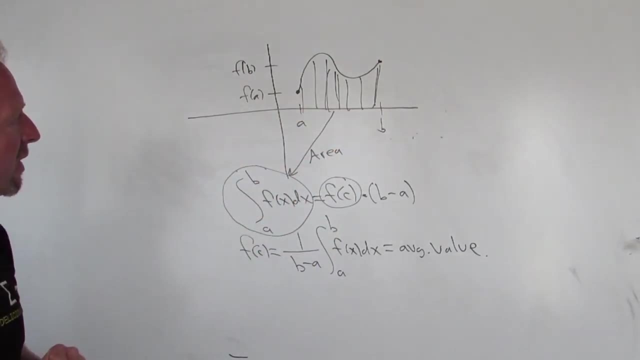 So this area here is the area under the curve. So this is the area, All, right, That's the area under the curve, Right? So the area under the curve. okay, the area under the curve is equal to this expression. 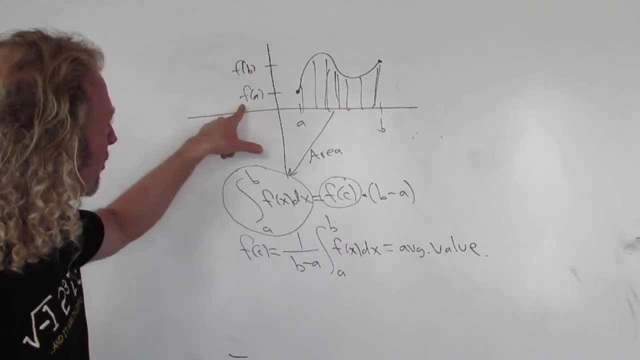 So what is this expression? Well, the mean value theorem says there is a number c. So I'm going to pick the number to be here so that the picture makes more sense. I'll do it here. So if this is c, 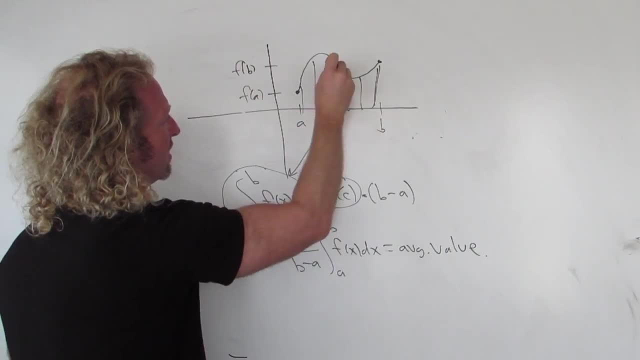 this is f of c. Okay, So I'm just picking the number And what you can do is you can draw a box whose height is equal to the area under the curve. All right, So if this is c, this is f of c. 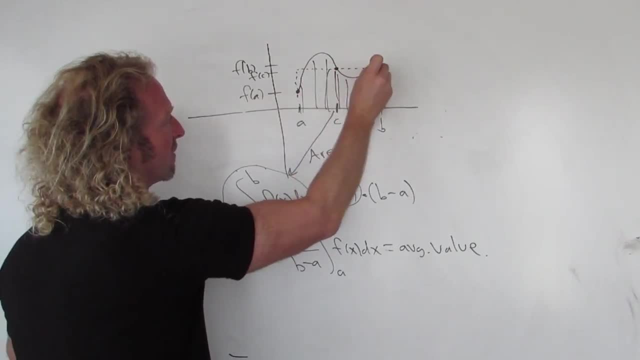 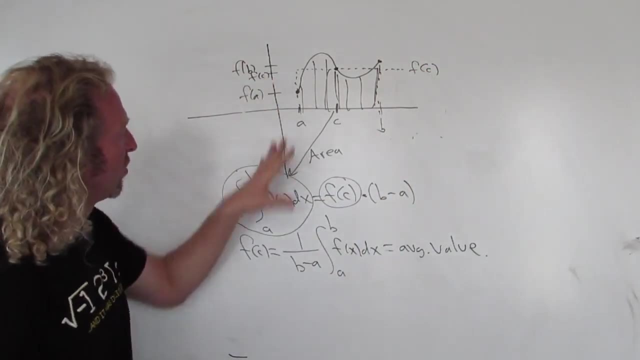 Okay, So if this is c, this is f of c. Okay, So this is f of c. So f of c is the height of this box, And so what the mean value theorem is saying is that the area under the curve is equal to the area. 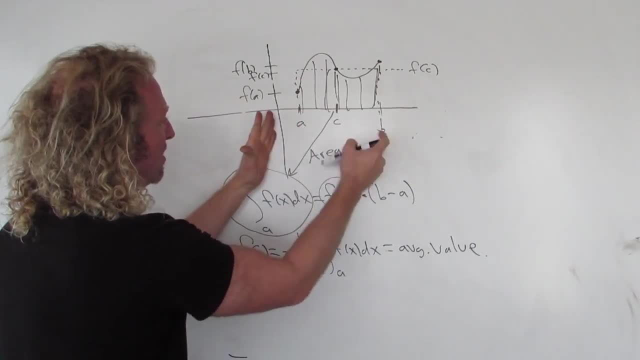 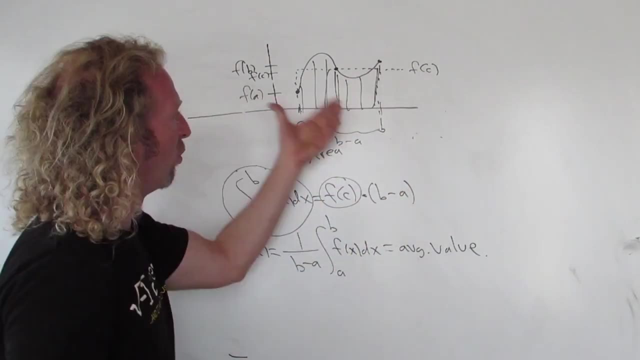 of the box Right. Think about it: If this is a and this is b, then this distance here is b minus a. So remember, the area of a box is the width times the height. Right, The height of the box is f of c. 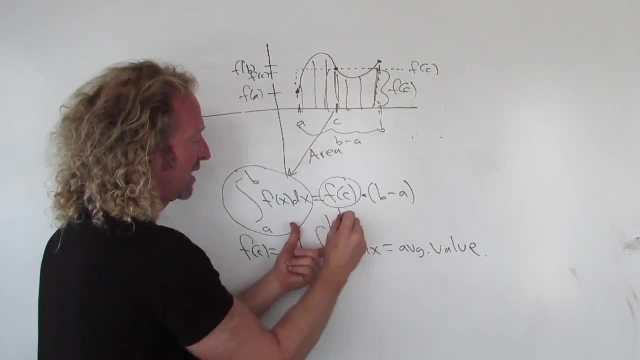 The width is b minus a. Okay, So this is the height times the width. So the mean value theorem for integrals says: if you have a continuous function it's continuous. right, there is a number c in the interval, such that the area under the curve is equal to. 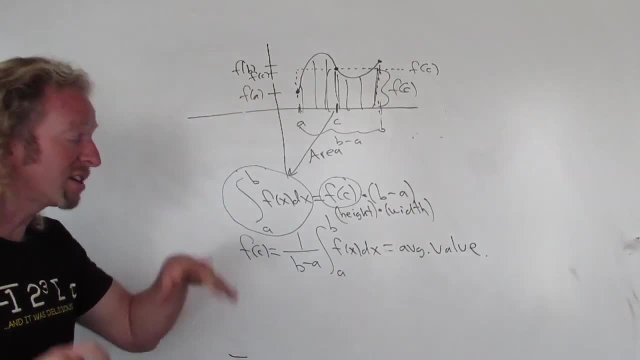 the area of the box whose height is f of c And what is the height of the box? The height of the box is the average value of the function. Deep stuff, Pretty simple, Okay. So let's see So. 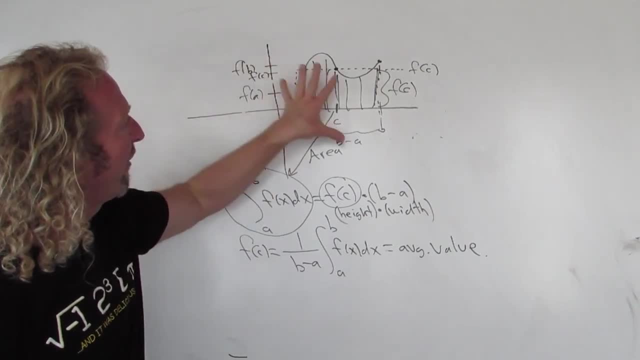 if this is c, this is f of c. Okay. So if this is b minus a, this is f of c. Okay. So what the mean value theorem for integrals says is: if you have a continuous function, it's continuous. 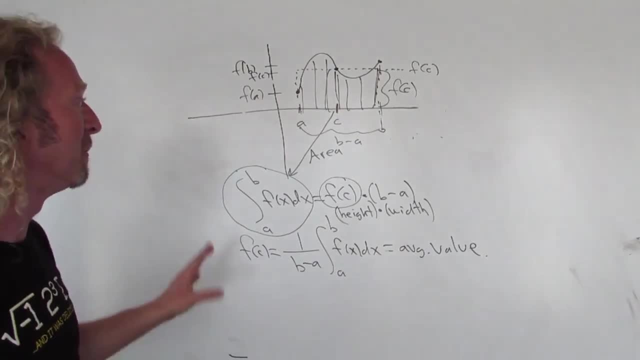 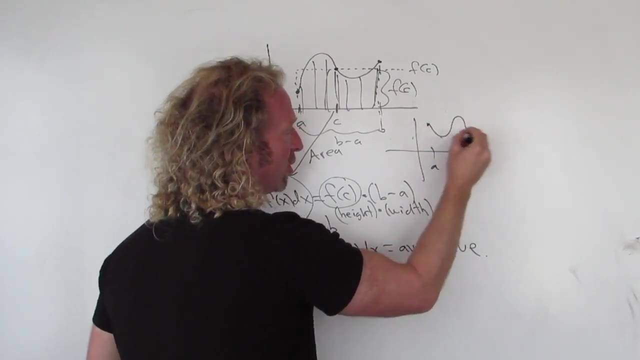 Right. So what is the height of the function? Deep stuff, Pretty wicked. So again. so if you have a and you have b and you draw a picture like this, you should be able to find a box that gives you the same area. 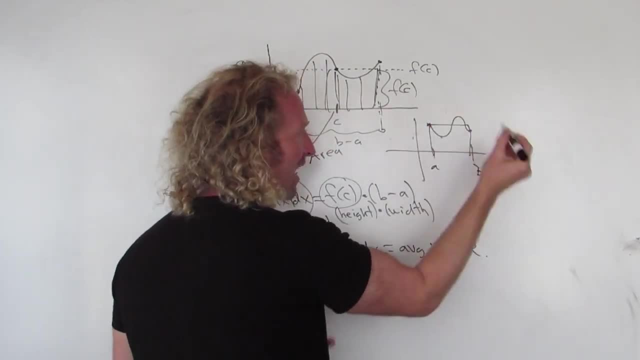 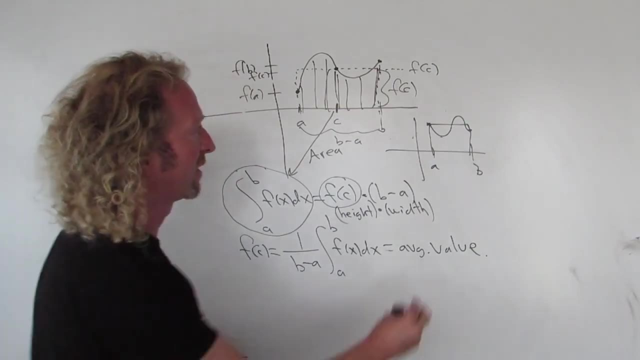 somewhere. So maybe, maybe this is that box Right And the height of that box is called the average value of a function Right. So the height of that box is called the average value of the function In this case. 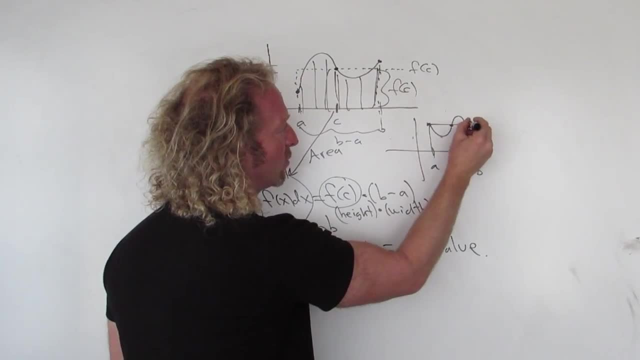 this here would be the value of c Right, And this would be your f of c. f of c is the height of the function- Okay- of the box. it's the average value of the function right. The width of the box is b minus a. 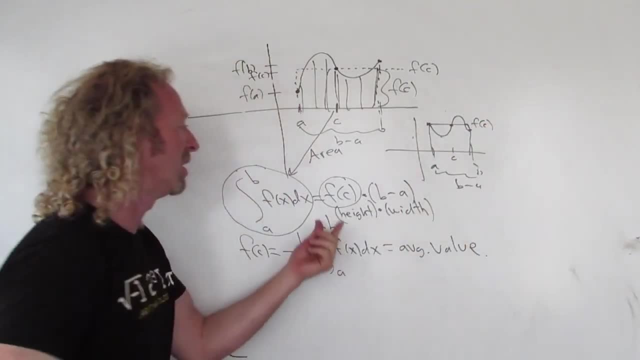 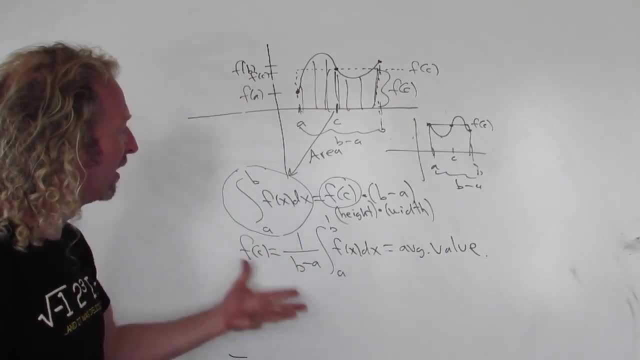 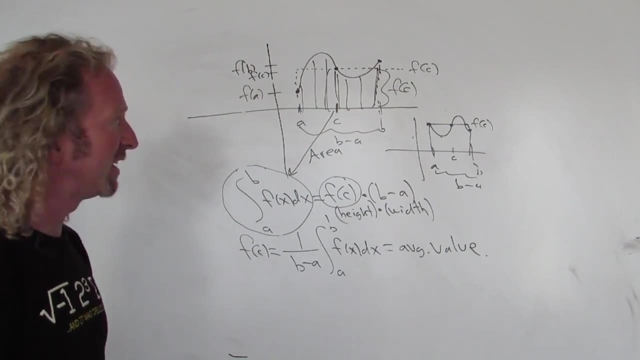 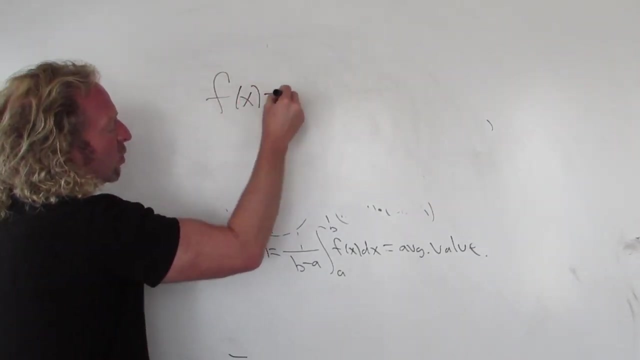 and do a simple example of finding c. maybe Let's try to find c and let's try to find the average value. So I'll see if I can make one up. Let's see: f of x equals. let's see, I guess we 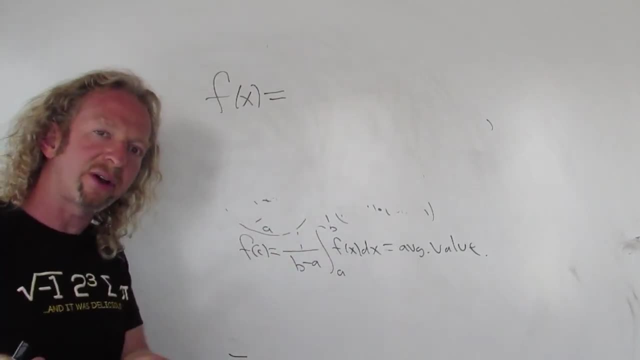 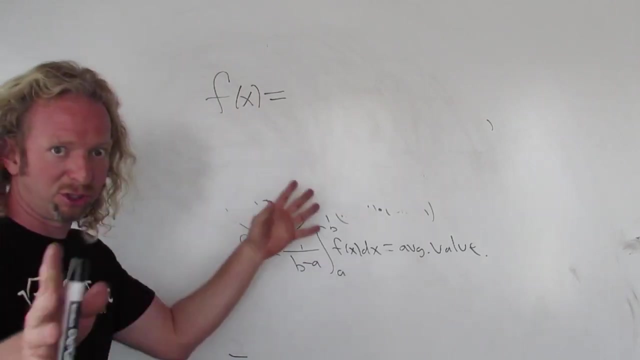 should be able to do this regardless. As long as we have a continuous function right, this should work right. So the criteria is: we have a continuous function on the closed interval. So if I make one up, we should be able to do it. Here we go. I'm going to try to make up the easiest possible one. 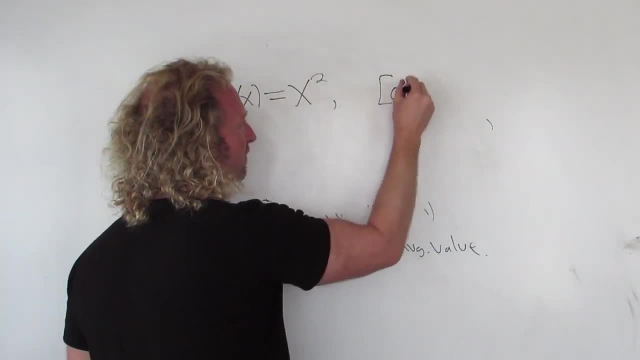 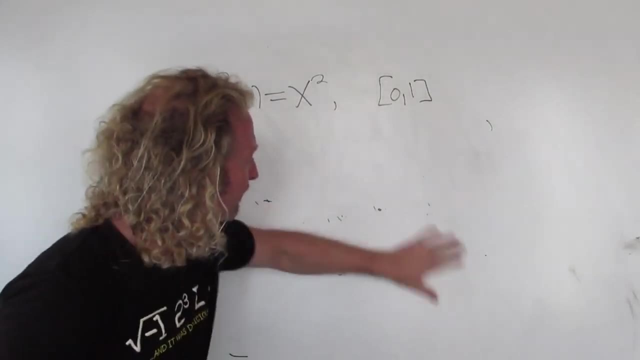 f of x equals x squared. Let's just look at 0,, 1,. okay, Let's see, Let's find the average value and then let's find the value of c. So the formula, the way I like to memorize the formula for these problems is as follows: 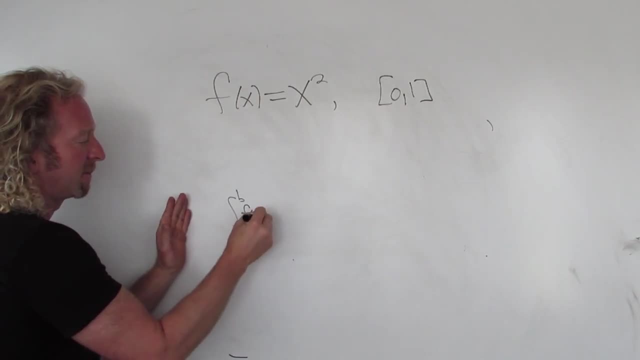 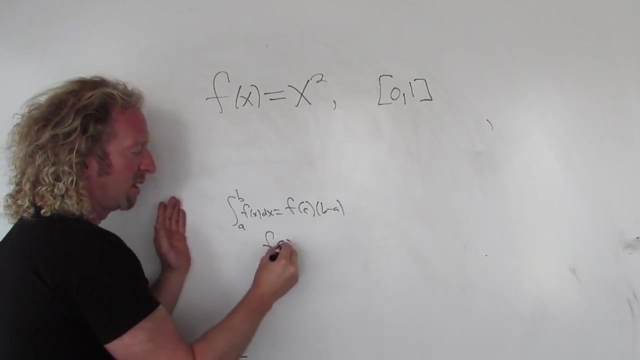 The theorem says you have the definite integral from a to b and that's equal to f of c, b minus a. So if you divide by b minus a, you get f of c equals 1 over b minus a times the definite integral. 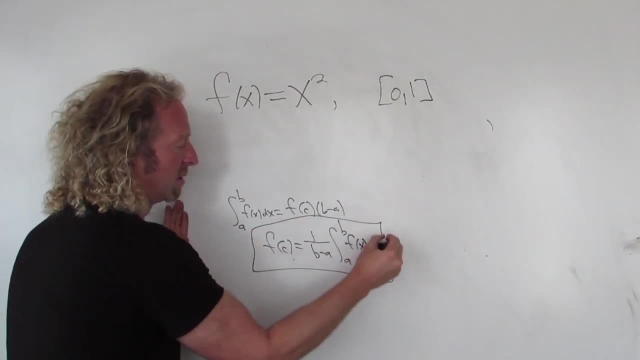 So this is the formula I always use for the problems. It's just easier, right, So I'm going to use this one. f of c is the average value. So if you had to find c, you just work this out and then. 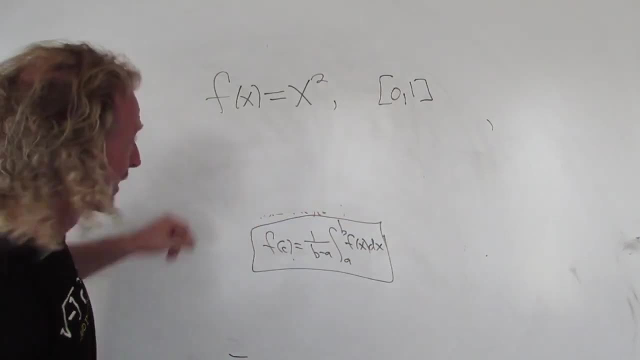 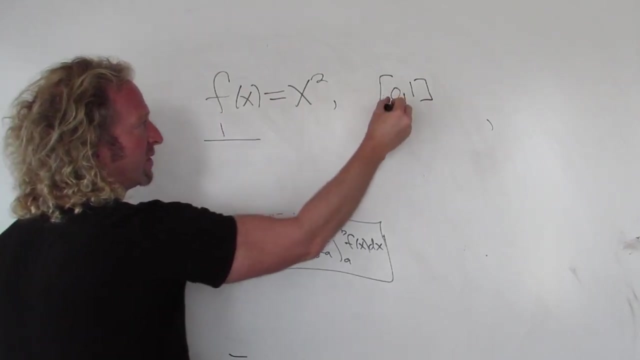 you set it equal to f of c. It's pretty simple. I hope Let's find out. So let's work out this piece first. That will be the average value, So it'll be 1 over. so this is a and. 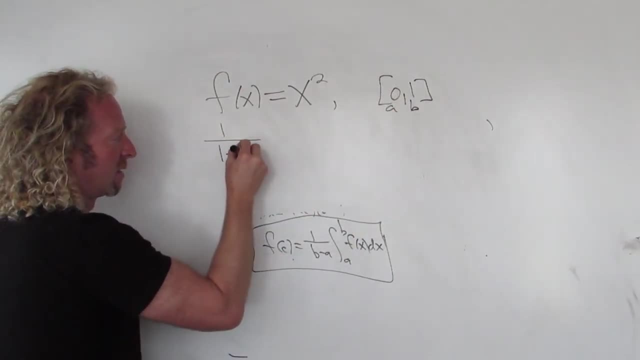 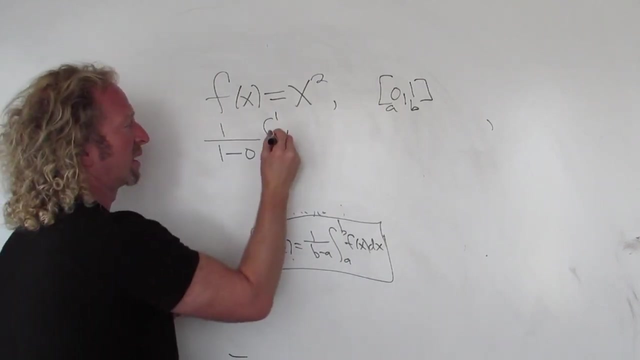 this is b, So it'll be 1 minus 0, and then we're going from 0 to 1, right? So of course I'm good. And then f of x is x squared, so x squared dx, That's just 1.. 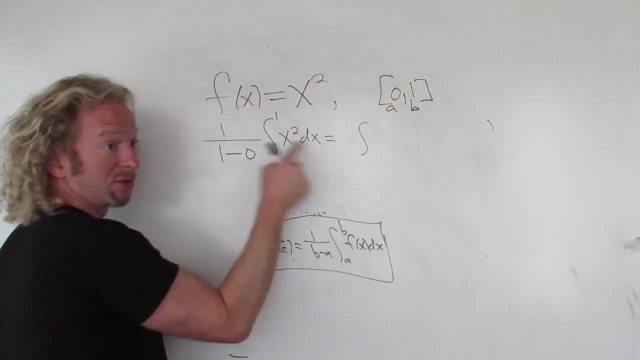 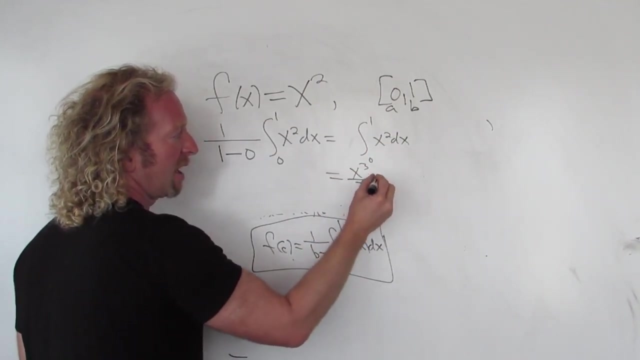 And then, so it's just 1.. So it's just 1.. I won't write it. And then 0 to 1, x squared dx. When you integrate x squared, you get x cubed over 3.. And we're going from 0 to. 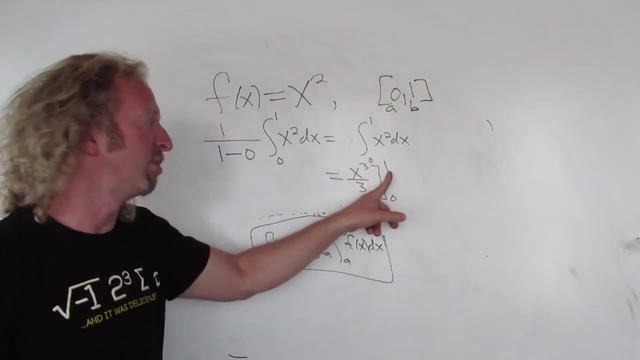 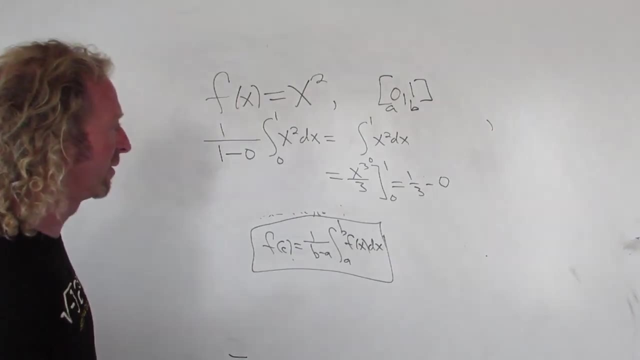 1.. Then the final model theorem of calculus says you plug in the 1s subtract and plug in the 0. So you get 1 third minus 0, right, Because 0 over 3 is 0. So you just get 1 third. 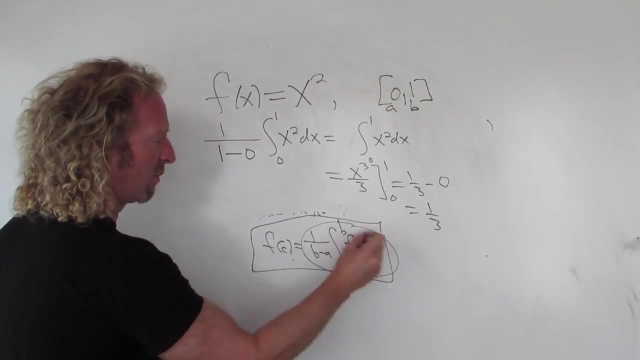 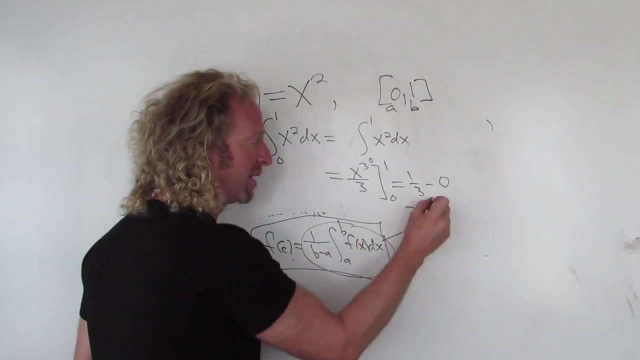 So 1 third. So we work this out and we got 1 third right. So now we just take f of c. Oh, and what is this? This is the average value. This is the height of the box, right? This is the average value. This is the average value of. 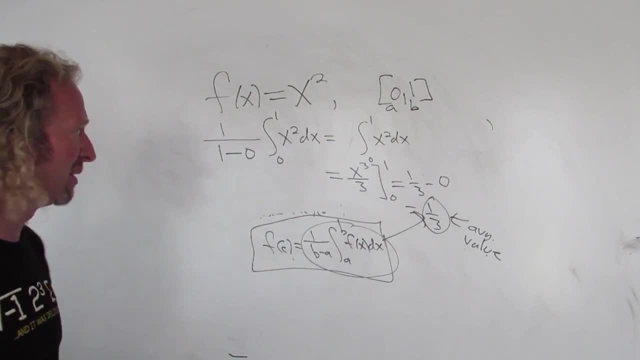 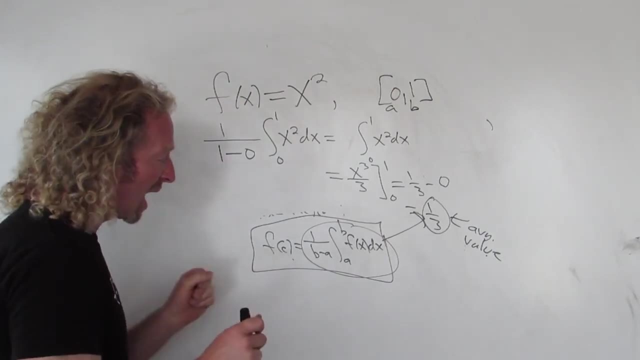 the function over the interval 0 to 1, right It's the height of the box. right That gives you the same area as the definite interval from 0 to 1.. OK, So now we're going to find f of c. So how do you do that? We're going to find c. 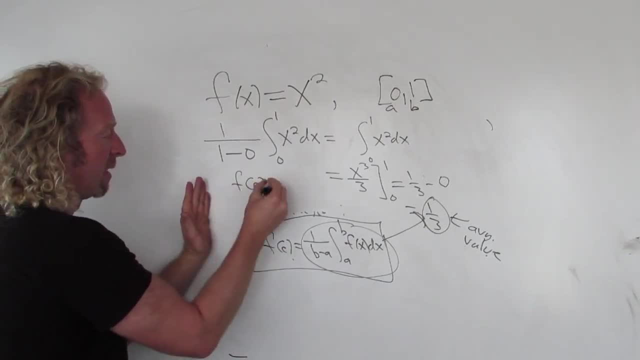 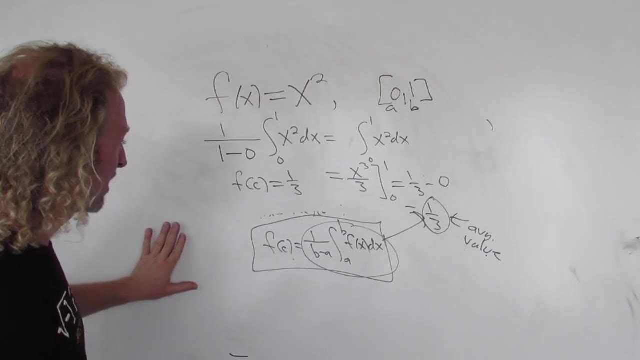 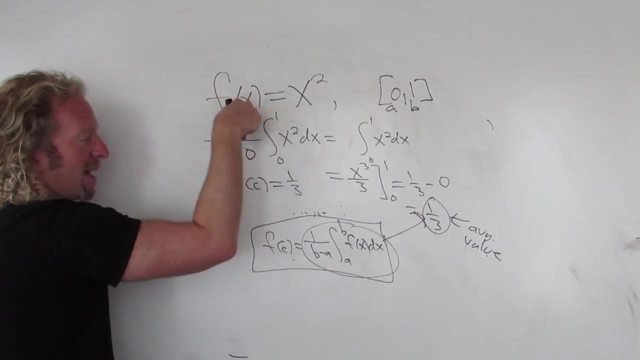 rather Sorry. We're going to find c, So we'll set f of c equal to the quantity which we worked out, equal to the average value. OK, And then we just replace c with what it is, So f of what it is. So f of c is the same as f of x, except x is c. So this is c squared. 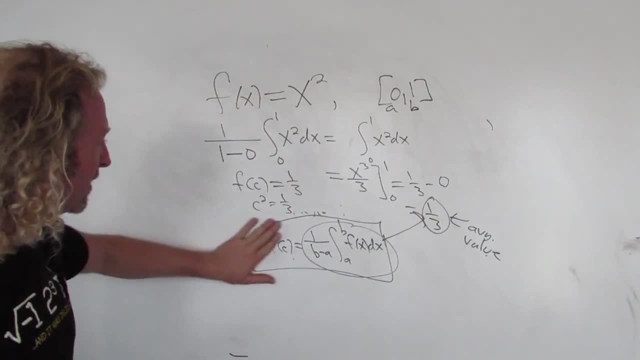 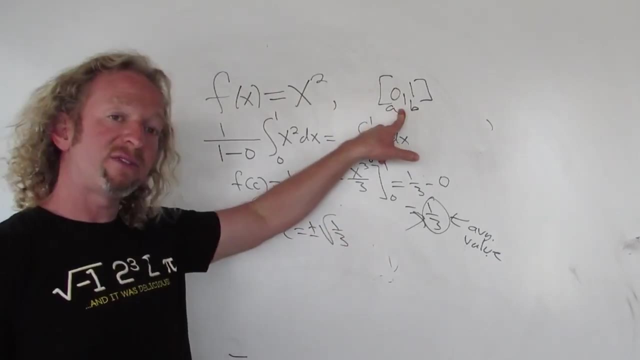 equals 1 third. All right, c squared equals 1 third. And then, to finish, we just take the square root, So you get: c equals plus or minus the square root of 1 third. Ah, but we had to throw one of these away, right, Because our c has to be in the interval. So we want. 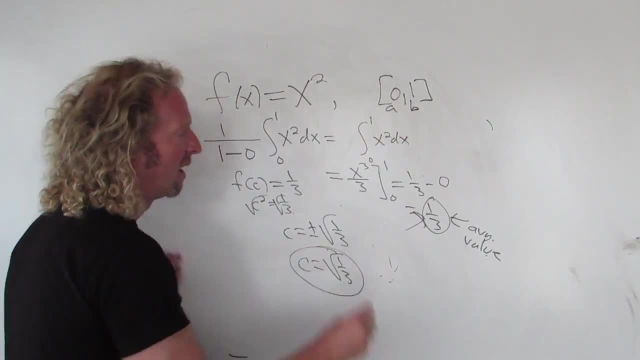 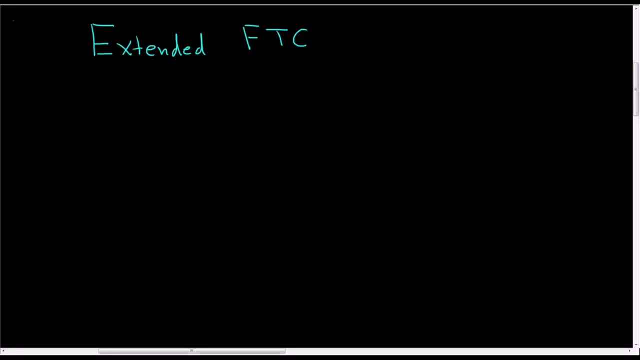 the positive one. So that would be the value of c. I hope this video made sense and I hope it's helped you understand what the mean value theorem is. So let's talk about the extended fundamental theorem of calculus. I'm actually not sure. 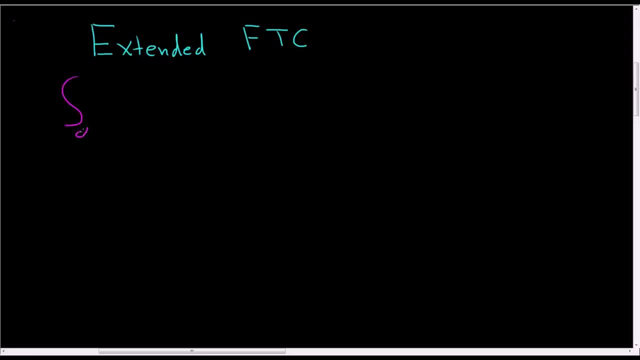 if it's called that. but that's what we'll call it. So if you have the definite integral from alpha of x to beta of x, of f of t with respect to t and you take the derivative of this beast with respect to x, this is actually equal to f of beta of x times beta prime of x minus. 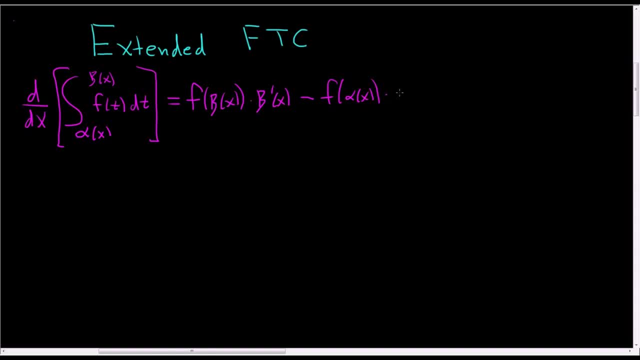 f of alpha of x times alpha prime of x. Let's go ahead and give like a quick proof sketch, So I'll put proof in quotes, So kind of terse. So let's write down the integral from alpha of x to beta of x. This is equal to big F of beta of x minus big. 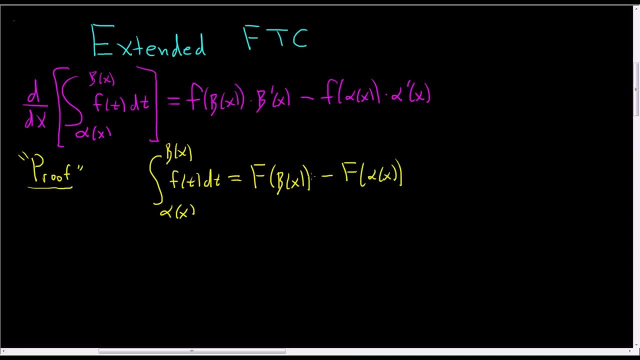 f of alpha of x, where big F is an antiderivative of little f. And now, if we take the derivative of both sides, with respect to x to delta of x, this is equal to x to beta of x. So this is the integral. So if you take the derivative of alpha of x, this is equal to f of beta. 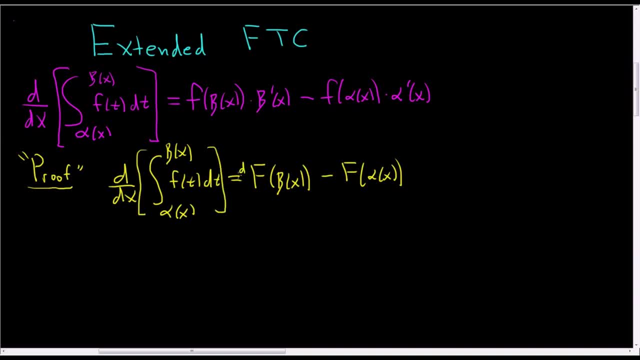 of x. So if you take the derivative of both sides with respect to x and you take the see- if I can squeeze it in here- ddx of this stuff, let's see this is big F prime evaluated at beta of X times the derivative of the inside chain rule. so 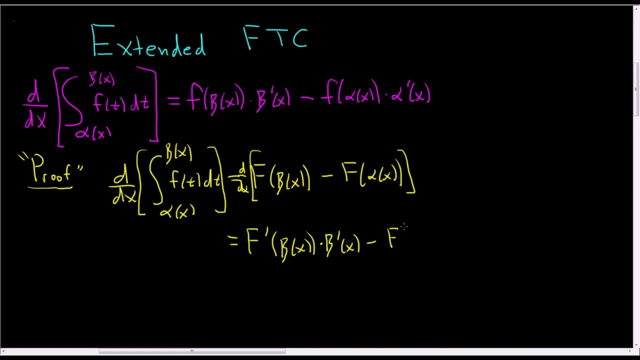 beta prime of X minus big F, prime of alpha of X times the derivative of the inside, so alpha prime of X. but we said that big F was an antiderivative for little F, so big F prime is little F. so we get little F of beta of X times beta. 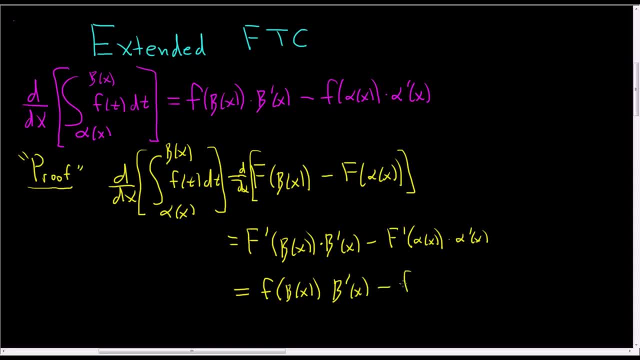 prime of X minus little F of alpha of X times alpha prime of X, and I guess that's the proof. sketch kind of terse. let's do a couple quick examples to show you what we're going to do here. so we're going to do alpha prime of X minus. 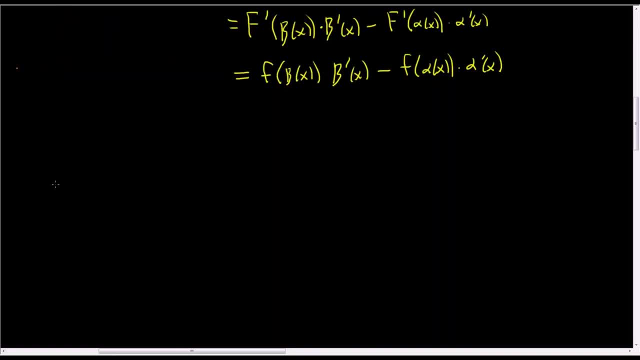 the inside. so just think about this for 5 seconds and let's just do a couple quick examples and let's see why this is so useful and so powerful. this is usually not found in calculus books. say, we had a function, let's call little G, and we can just make it up and do it. we had sine X here and then here we have X. 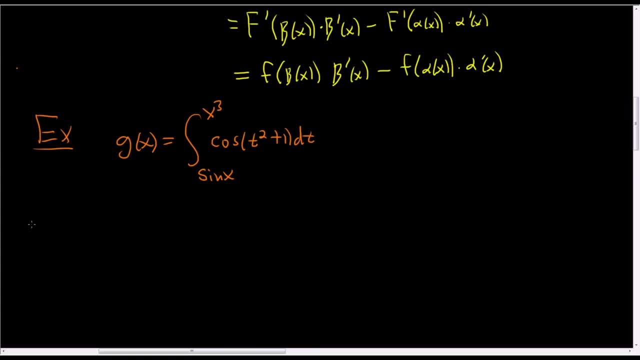 cubed, and here we have cosine of T squared plus 1 dt. let's find the derivative of little G, so little G, prime of X. well, how do you do this? well, first, So you get cosine of x cubed, squared, so you get x. to the 6th right, because you have 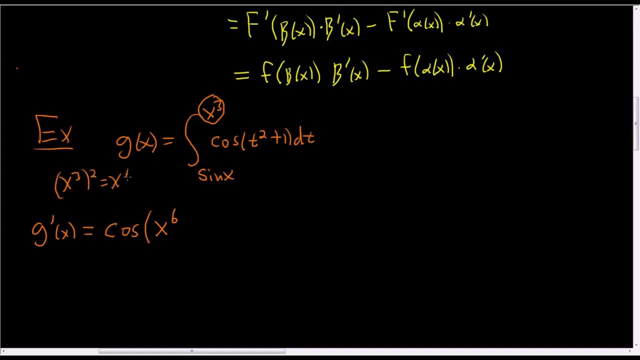 x cubed and it's being squared, so you get x to the 6th plus 1, then you multiply by the derivative of x cubed, so 3x squared subtract. now you plug in the sine function for the t, so cosine of sine squared x plus 1, and then you multiply by the derivative. 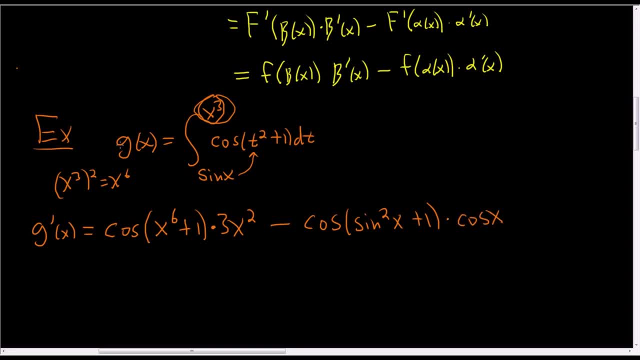 of sine, which is cosine. so again, first you plug in this one and then you multiply by the derivative of that one, so it's there. then you put a minus sine and then you plug in the sine. we did that- and you multiply by the derivative of sine, which is cosine. 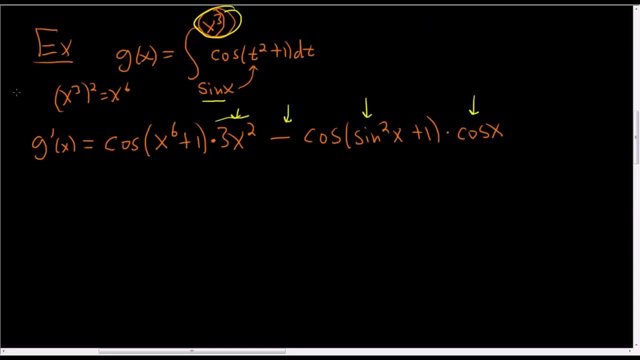 so really, really straightforward. let's do another one. So example: let's see little g of x will be the definite integral from. let's see x squared to ln x. and let's look at arctan t dt. 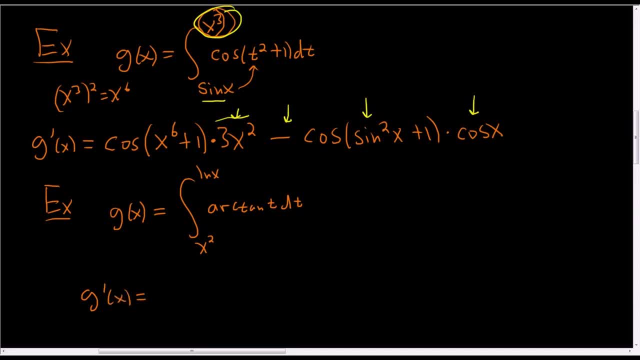 So when we take this derivative we first plug in the natural log for the t, so we get arctan and t is n, ln, x. then you multiply by the derivative of the natural log of x, which is 1 over x. 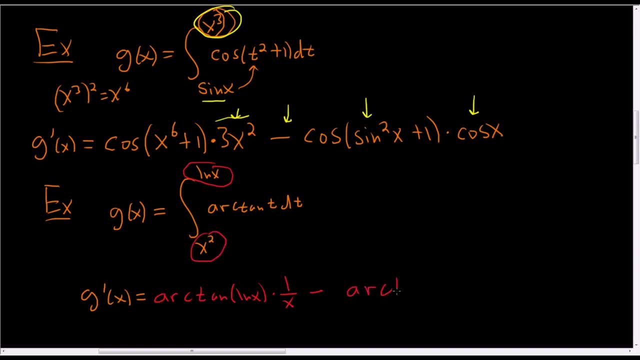 subtract and now you plug in this one. so arctan x squared, and then you multiply by the derivative of x squared, which is 2x. So you plug this one in multiply by the derivative of this subtract. plug this one in multiply. 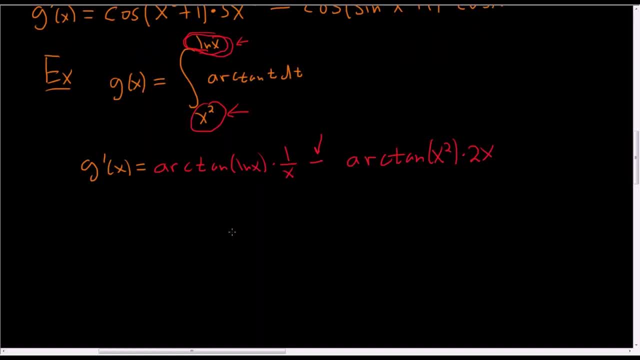 by the derivative of this. and you're done. Let's do another one, One more, one more. Let's see if we can make it ridiculous. Let's see: little g of x equals the definite integral of. well, maybe not ridiculous how? 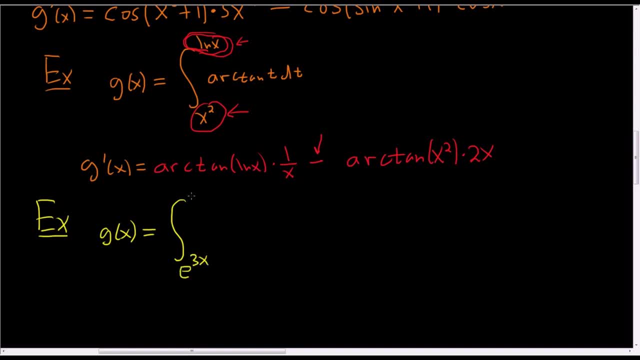 about e to the 3x? And then here let's put, ooh, let's put a cosine function, cosine of x. and what can we put here? How about, hmm, how about just sine of the secant of t squared plus 4?? 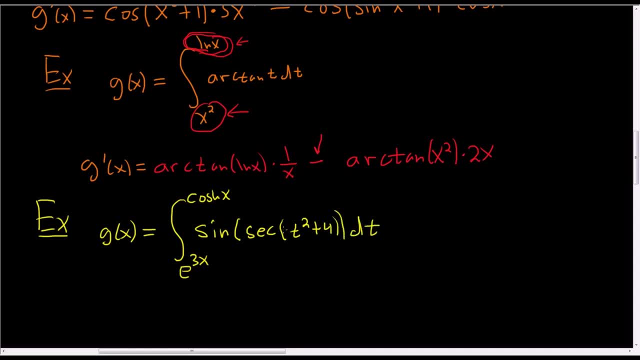 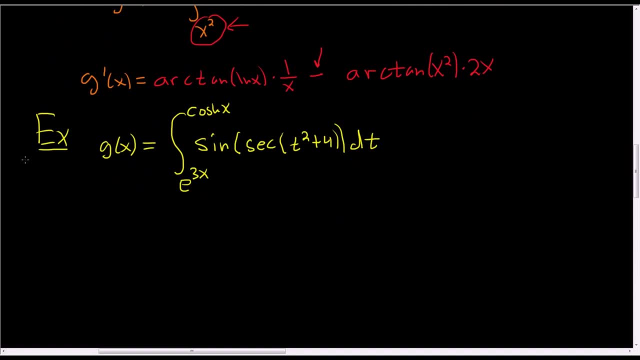 Yeah, let's make it look really scary. dt. This looks absolutely ridiculous, right, it looks really really hard. but with our extended fundamental theorem of calculus we are invincible, at least in terms of these problems. So g, prime of x, let's see. first we plug in the cosine function. 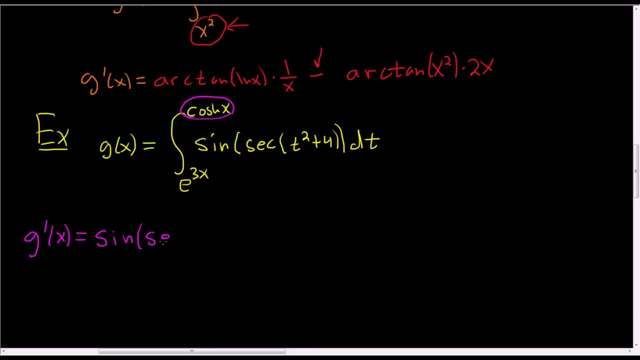 So we get sine of the secant of t squared plus 4.. So cosine squared x. Okay, so all we did was plug in the cosine for the t, and then we multiply by the derivative of cosine, which is sinh, We subtract, and now we plug in e to the 3x. 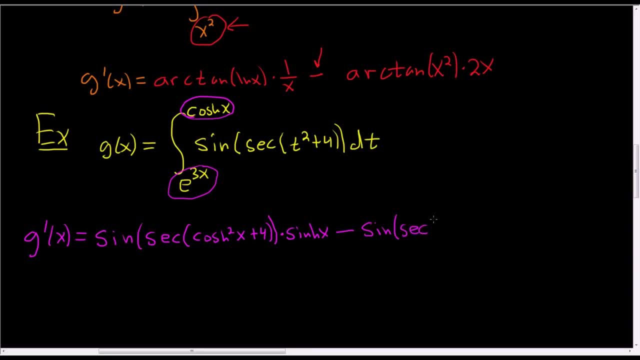 So sine of the secant, let's see e to the 3x and it's being squared, So e to the 6x plus 4.. Okay Times, the derivative of e to the 3x, that's e to the 3x times 3, right chain rule derivative. 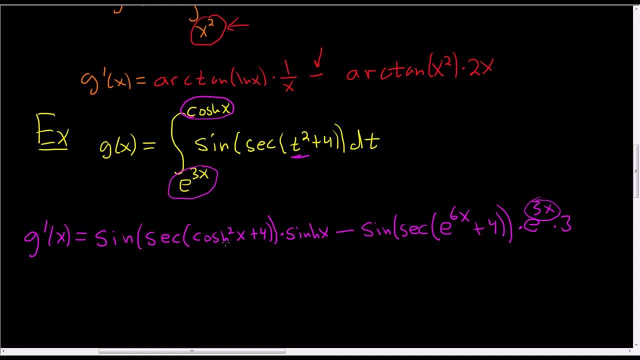 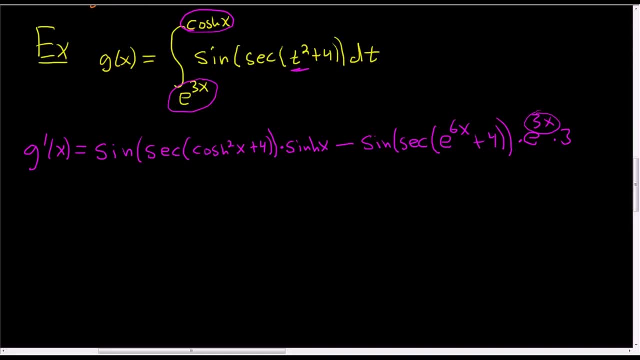 of the inside. I hope you've noticed I haven't really been simplifying any of my answers. I'm just going through these and showing you how to use the formula. Let's do another one, why not? These are kind of fun actually. 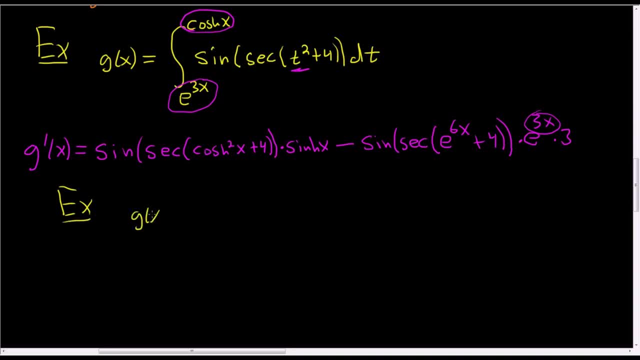 Let's see, let's look at little g of x equals the definite integral of tangent. Okay, So g, prime of x, and here we'll put, let's see x, and let's put an arcsine here, arcsine tdt. 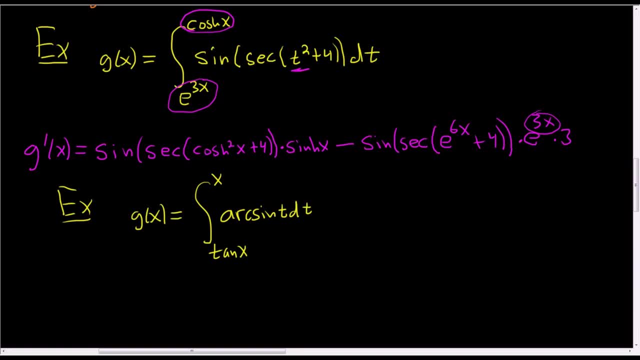 All right, let's do it use a different color. So g prime of x. well, first you plug in the x, so you get arcsine of x, and then you multiply by the derivative of x, which is 1.. 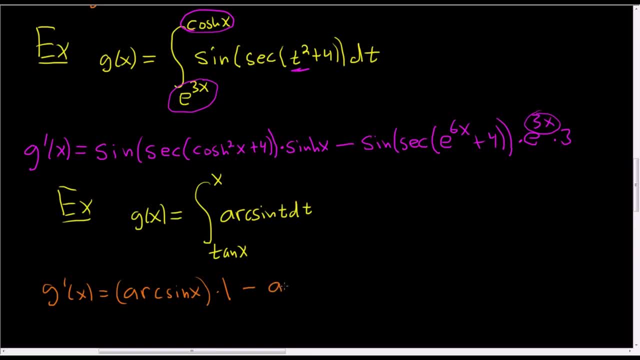 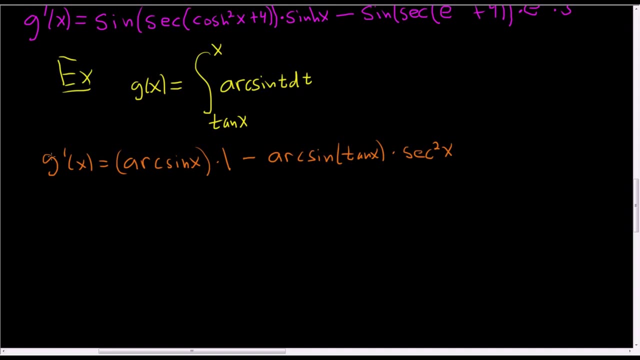 Okay, Subtract, So you plug in the tangent, so arcsine of tangent, and then you multiply by the derivative of tangent, which is secant squared x. I probably should have done an easier example at the beginning. Let me do an example that you would find like in a calculus 1 class. 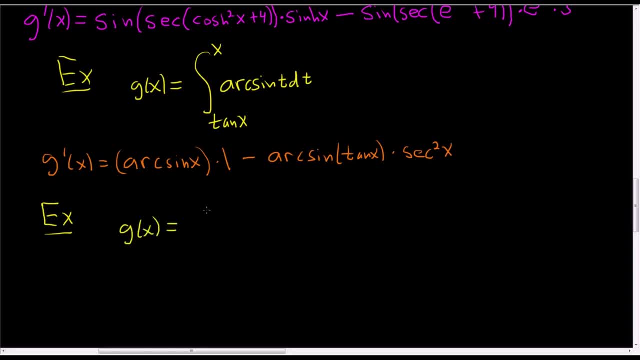 These are really easy. So let's see little g of x is the definite integral from 0 to x of I don't know. let's make it super easy sine tdt You could actually just integrate this and then take the derivative. but in calculus 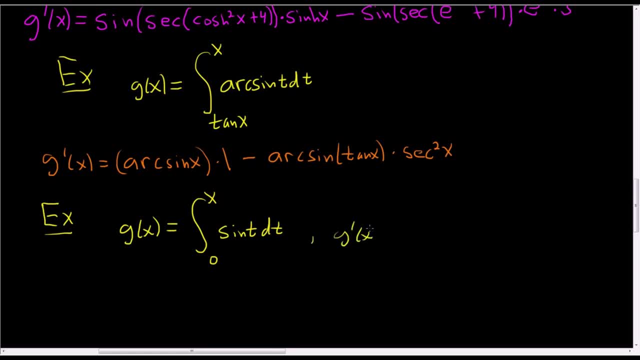 classes. they just say: do this. They say, okay, Take the derivative and just plug in the x. That's how you do it. Take the derivative, you plug in the x. Let's do it our way. So g: prime of x: well, first you plug in the x, so you get sine of x times the derivative. 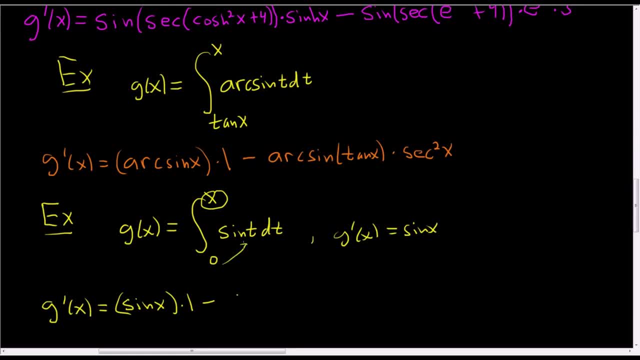 of x, which is 1, minus. now you plug in the 0,, so you get sine of 0, times the derivative of 0, which is 0. So this whole thing here is just going to be 0, so you just end up with sine of x. 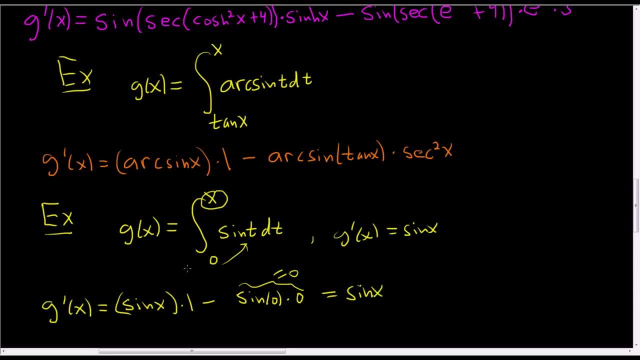 So our way is longer. Take the really easy examples. But if you have a function here on the bottom, then things change and then our way probably becomes the better way. I hope this helps someone out there. It's a pretty cool formula. 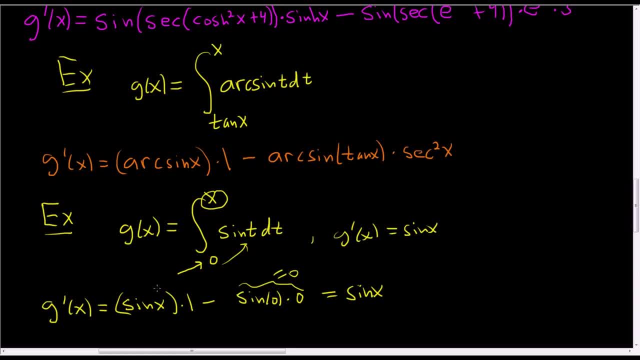 I saw it in a book many years ago- no idea what book- and I proved it right away. I'm like, oh, let me make sure it's okay and make sure I can prove it. And really really nice formula. Simpson's rule is used to approximate definite integrals. 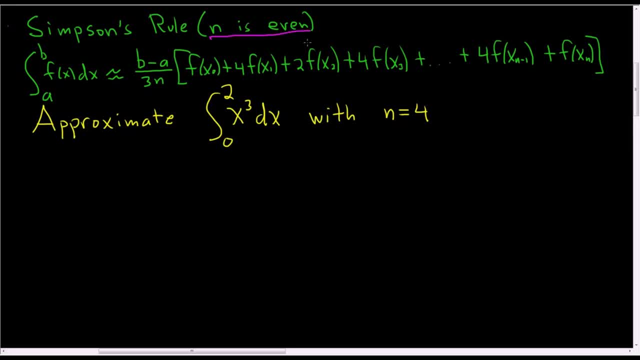 It only works when, When n is even, So the n you use has to be an even number, And it basically says that the definite integral from a to b is approximately equal to this stuff over here on the right-hand side, this huge mess. 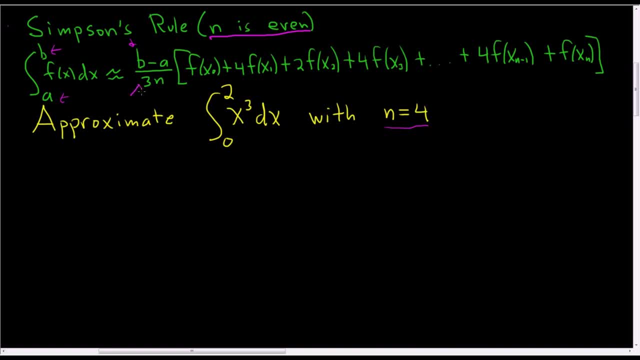 There's a really easy way to memorize this: Just memorize the 3n and memorize the b minus a And look at the coefficients. It's 1, 4,, 2, 4, etc. for 1.. 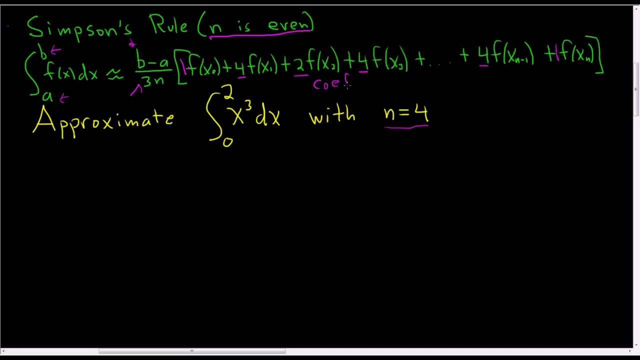 So the coefficients 1,, 2,, 3, etc. 2, 3, etc are 1,, 4,, 2, 4,, 2,, 4, 1, right, It always ends in 1.. 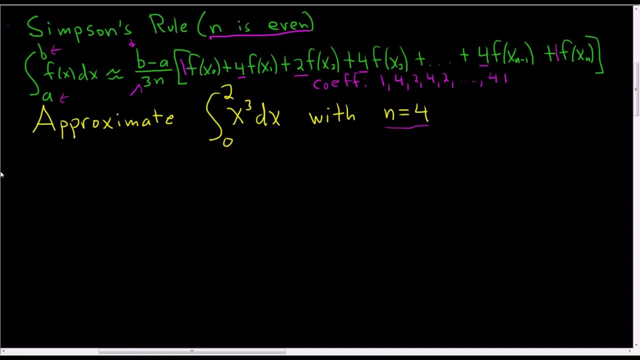 It always ends in 4, 1 as well. Okay, so we're asked to approximate this definite integral with: n equals 4.. So let's do it So. whenever I use Simpson's rule, I always work this out first. So delta x is equal to b minus a over n. 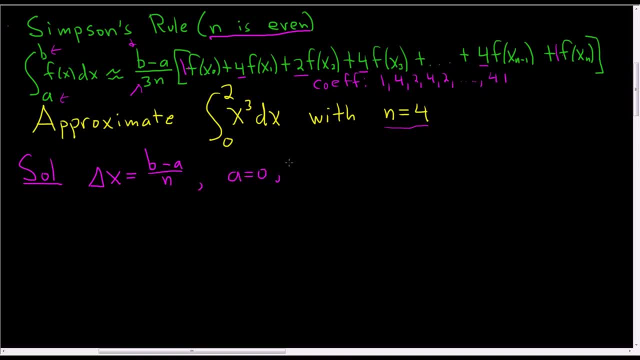 In this case, a is equal to 0, and b is equal to 2, and n is equal to 4.. So delta x: well, b is 2,, a is 0, and then n is 4.. So you get 2 over 4,, which is 1 half. 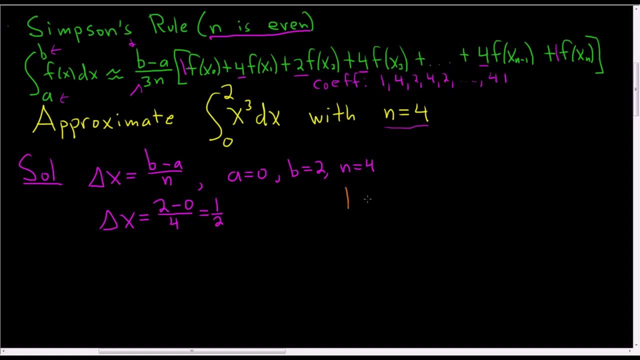 Then I draw a picture. Let's do that. Let's draw a little picture And we're integrating from 0 to 2.. So what I do is I just keep adding and subtracting. So I'm adding delta x. So 0 plus 1 half is 1 half. 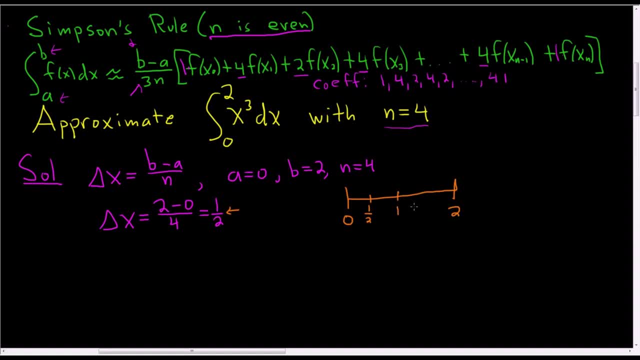 If you add 1 half again, you get 1.. And if you add 1 half again, you get 3 halves, And if you add 1 half again, you get 2.. So these guys are our little x's. 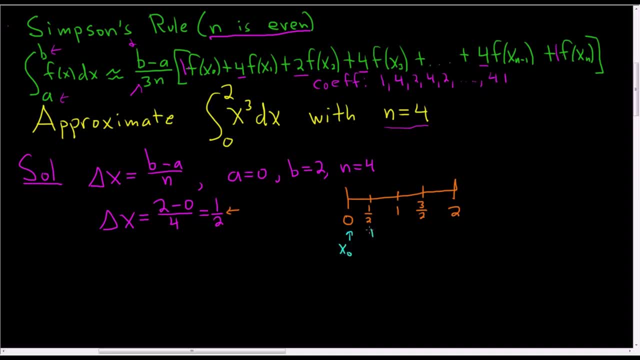 So this one here is x sub 0.. This one here is x sub 1.. This one is x sub 2.. This one here is x sub 3.. And this last one is x sub 4.. So again, you start by writing down delta x. 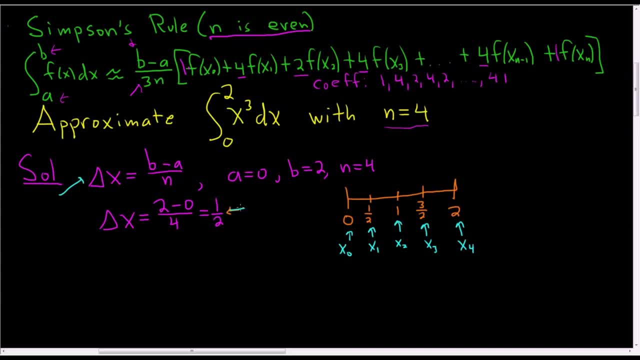 Plug in b, a and n, work it out, Draw a little picture like we did here, And just keep adding delta x. So we start at 0. So you add 1 half to 0. And you get all the little x's. 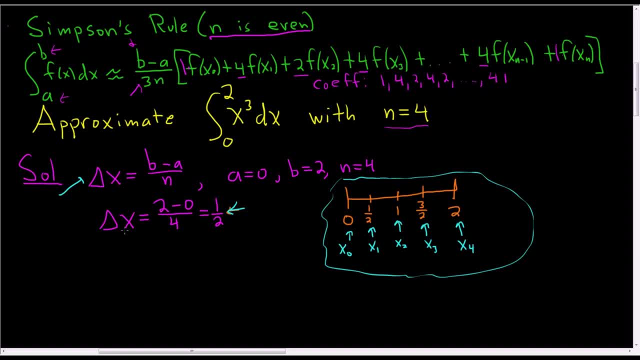 The last thing to do is use the formula. Okay, so let's attempt to do that. Let me use a different color. Actually, I'll stick with blue. I like the blue, So, alright, let's do it. So the definition of delta x. 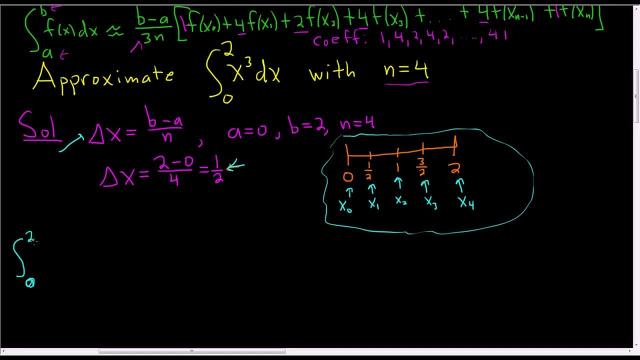 definite integral from 0 to 2 of x cubed dx, Our a is 0.. It's approximately equal to- let's see b minus a divided by 3n. So b for us is 2.. So 2 minus 0.. 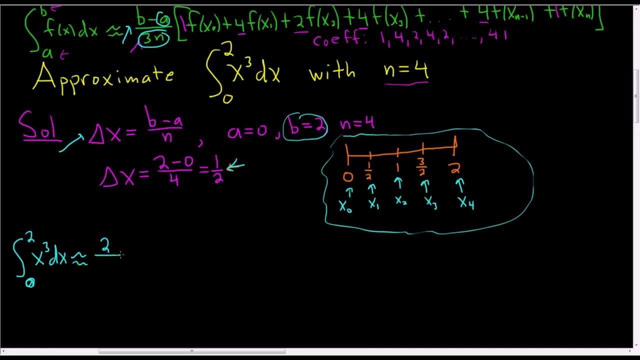 So 2 over, and then 3n. Well, n is 4.. So 3 times 4 is 12.. Yep, it sure is. So 2 over 12.. Then we have the bracket. Now we have to write down f of x sub 0.. 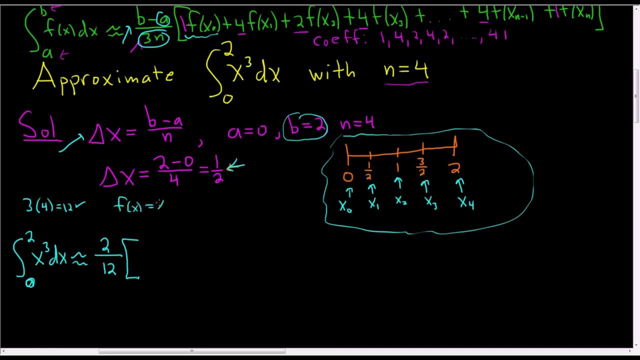 Well, in this problem, f of x is x cubed, That's the integrand. So f of 0, I'll actually write it f of 0. And then plus 4 times f of x1.. Well, x1 is 1 half. 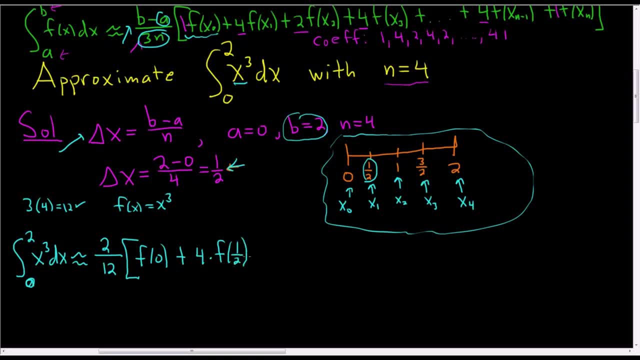 So it's f of 1 half. Just be really careful when you do this, Plus 2 times f of 1.. That's the next little x guy right: x of 2 plus 4 times f of 3 halves. 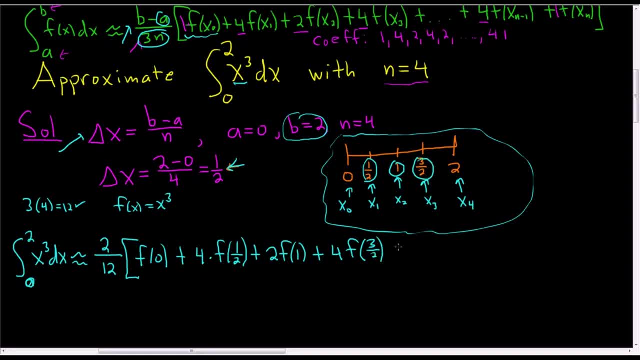 That's the next little x guy we have, And then the last one is 1 times f of 2.. And this is all in brackets. Let's keep going. This is 1. sixth f of 0 is 0 cubed. 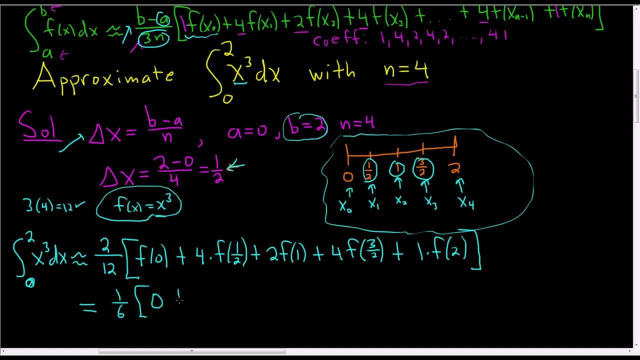 We're plugging it in here into f of x. So we just get 0 plus 4 times 1 half cubed plus 2 times 1 cubed plus 4 times 3 halves cubed. We just cube all the x's. 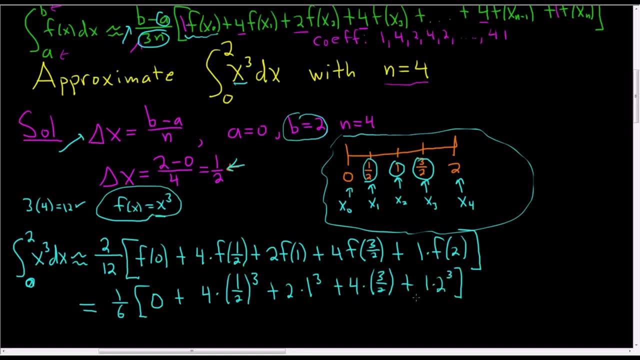 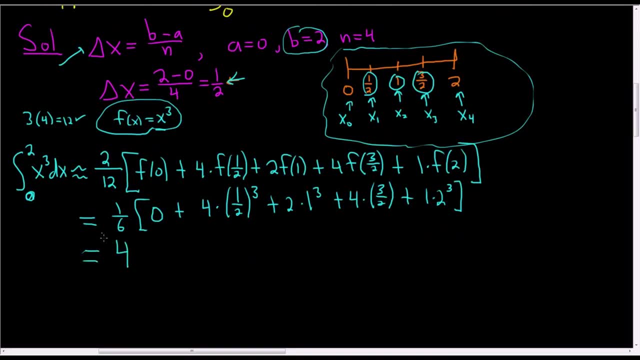 Plus 1 times 2 cubed. What a mess. And if you work this out, it magically gives you 4.. So that's the answer using Simpson's Rule. Note, if you actually work this out, if you actually integrated this from 0 to 2. 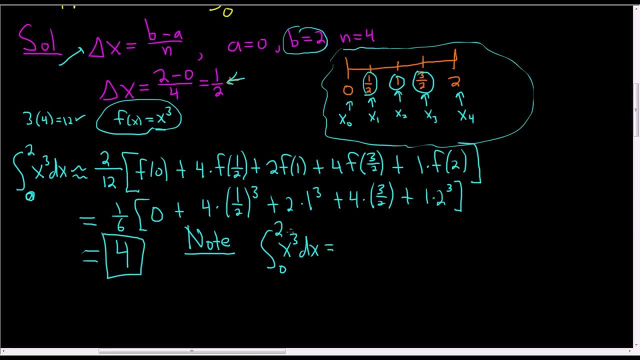 with respect to x. how would you do that? Well, you would add 1. So you would get x to the 4th over 4.. Then you draw your little line. You put the 0 here, You put the 2 here. 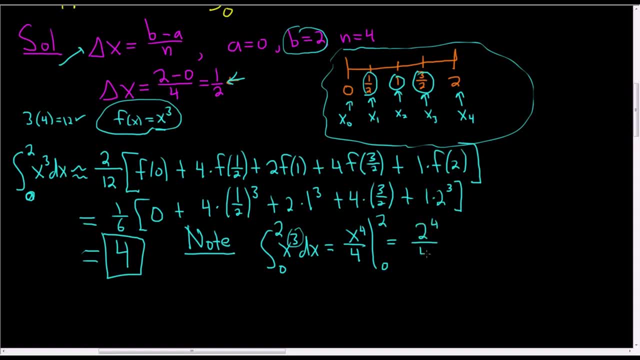 Then you plug in the 2 first, So you get 2 to the 4th over 4. Minus, And then you plug in the 0. So you end up with 16 over 4, which is 4.. 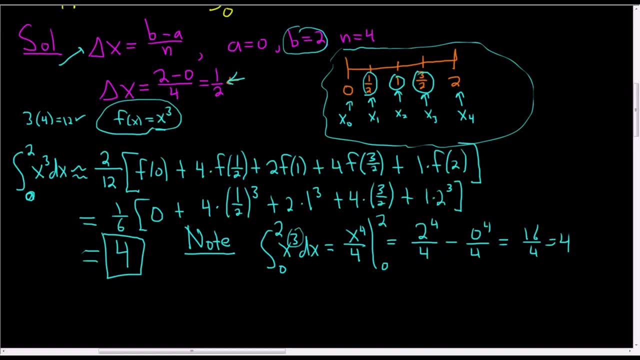 So in this case, in this case, Simpson's Rule is just perfect. It worked out exactly right. That does not always happen. It's supposed to be an approximation method. I hope this helps someone out there who's trying to work through Simpson's Rule. 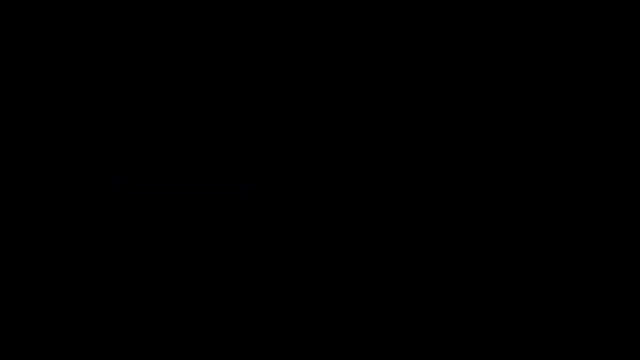 In this video we're going to define the natural log of x using some calculus. So our definition is the following: So we write ln x and we define it to be equal to the definite integral from 1 to x of 1 over t. 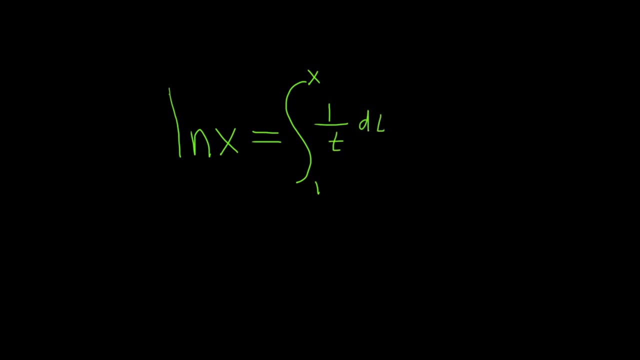 with respect to t dt. This definition will be valid for positive values of x, So for x greater than 0.. We're going to say that this is the natural logarithmic function, So the most important rule that we're going to get from this definition: 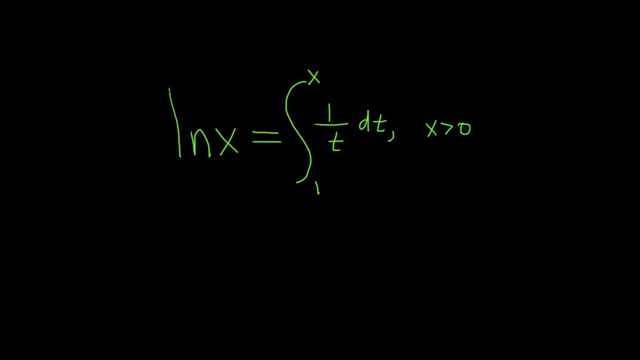 is the derivative of ln x. So recall the second fundamental theorem of calculus, So the second FTC. The second FTC says: if you take the derivative, with respect to x, of the definite integral from, let's say, 1 to x, of f, of t, dt. 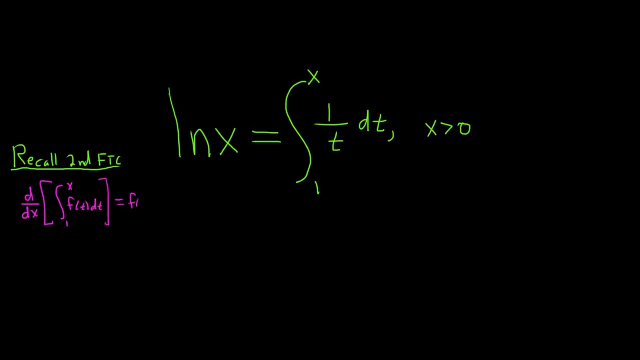 that this is equal to f of x. It's a really simple proof. I don't want to reprove it, but maybe I will just to sketch it and highlight it. If you think about the first FTC, you can rewrite the integral as big: F of x. 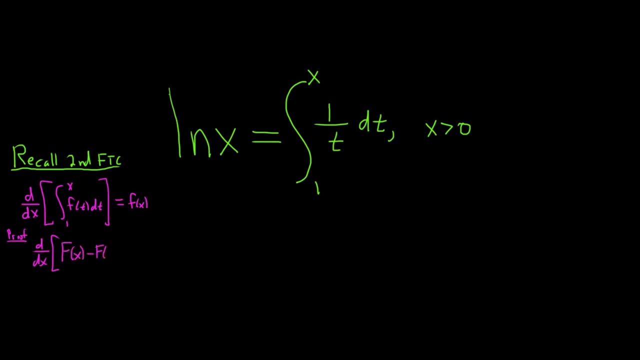 where big F is an antiderivative Minus big F of 1, where big F is an antiderivative of little f, Then taking the derivative gives you big F prime and then f of 1 is a constant, so minus 0.. 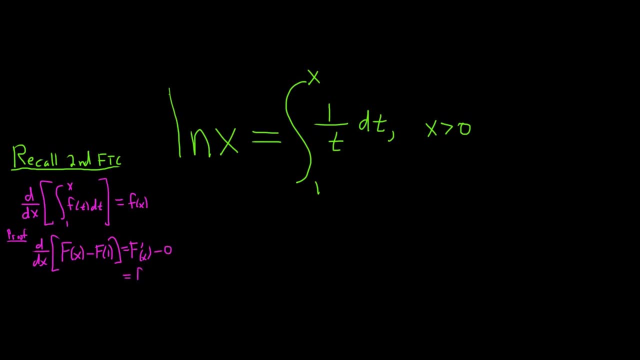 Well, big F is an antiderivative of little f, so its derivative is little f by definition, and that's the proof, a rough proof, of the second FTC. So in this problem here, that was a lot of knowledge, lots of information In this problem here. 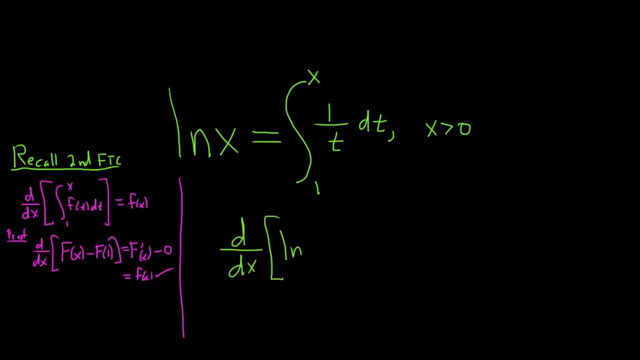 we're taking the derivative of ln x Right, And so we're taking the derivative of this integral here on the right hand side, And so we just take notice, you just take the x and you put it where the t is Right, So you just get f of x. 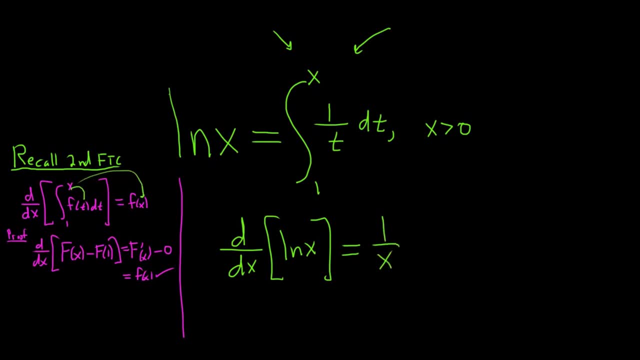 So here you just get 1 over x, And that's the formula that this video is about. Right, The derivative of ln x is 1 over x. Let's go ahead and do an example or two of using it. Okay, So let's find some derivatives. 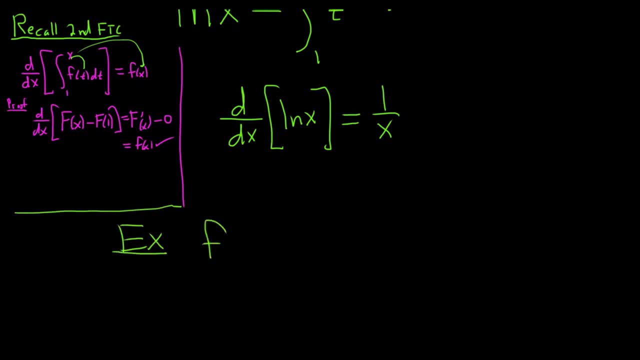 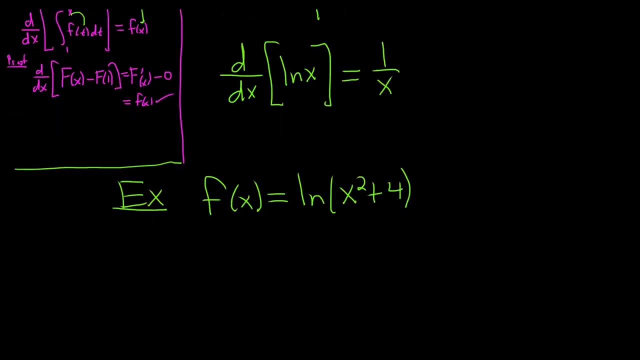 So let's say we have- I don't know- f of x equals ln x squared plus 4.. Just a simple example, And we're going to compute the derivative of this. So if it was just ln x, it would be 1 over x. 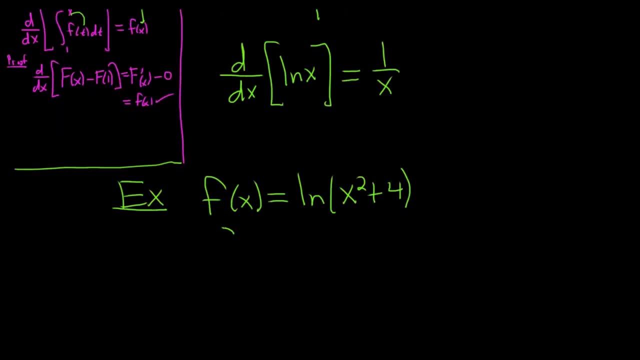 But here it's ln of x squared plus 4.. So what we do is we use the chain rule. So f prime of x, So it's 1 over whatever you see here. So it'll be 1 over x squared plus 4. 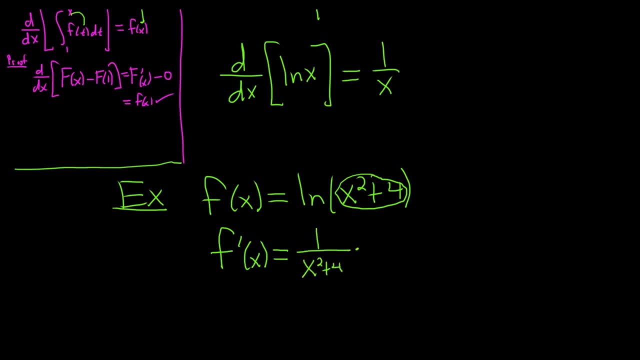 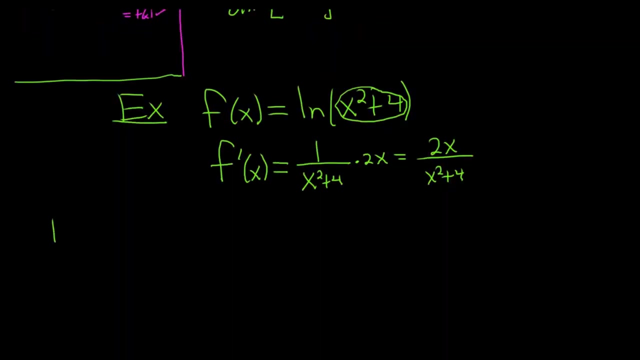 times the derivative of the inside. So times times the 2x, And that's it, Right, You would just get 2x over x squared plus 4.. And that's it, Let's do. let's do one more, One more, so you recall some stuff. 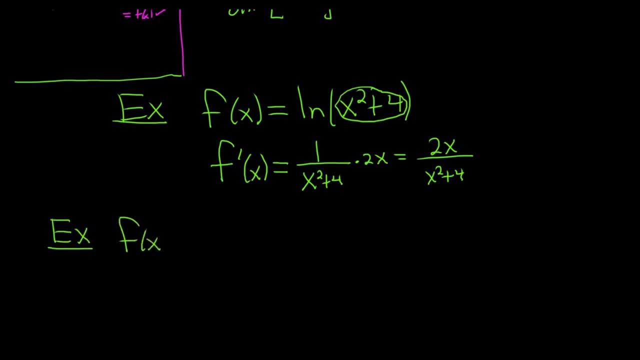 Let's say we have f of x equals ln, parentheses, x times x plus 4 times x, squared minus 7.. Okay, And so in this case, if you take the derivative, it's 1 over all of that stuff, times the derivative of all of that stuff. 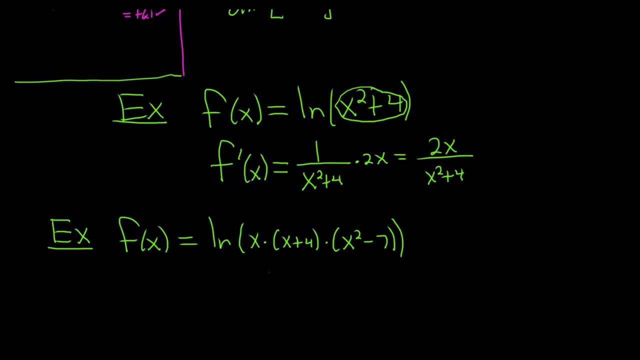 That could be a bit of a problem. Right, That's a lot of product rules. So what you do is use the property of logs. I don't know if you remember this, but if you have ln of a times b, the multiplication turns into addition. 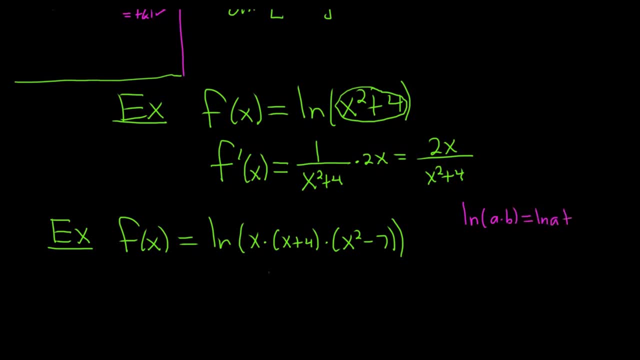 I love how it rhymes. ln of a times b is ln of a plus ln of b. Right, That's called the product rule for logs. You also had the quotient rule. ln of a over b was ln a minus ln b. 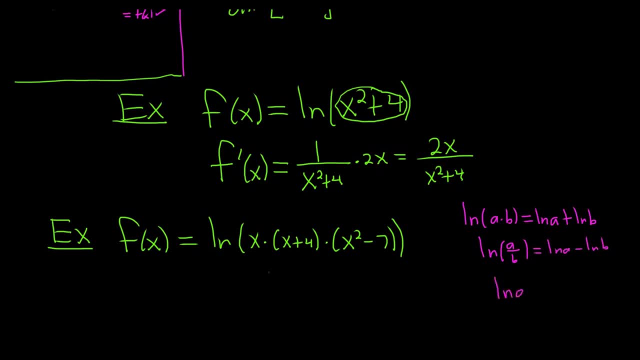 And then you also had the power rule ln of a to a power. You could put the powers in the front. So these were the, the properties of logs from algebra Right, And they come up a lot in these derivatives. So typically when you have a derivative, 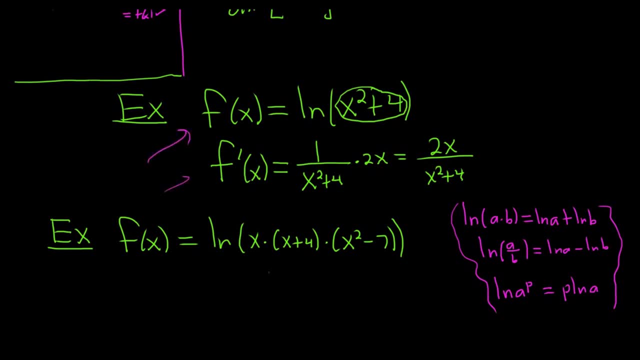 if you can just do it and it's not too messy, like in this example, here we did it, But here, here we have to do some work. So let's rewrite this using the product rule for logs. So this is our first piece. This is our second piece. 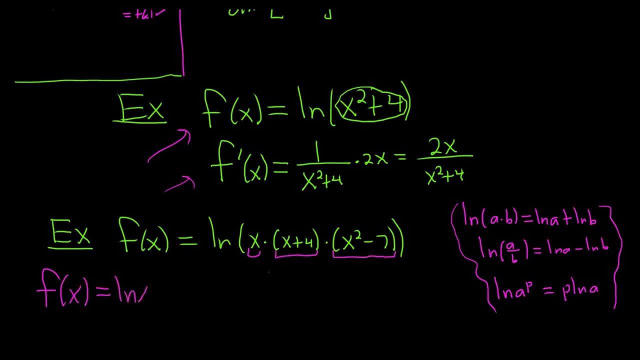 This is our third piece, So it'll just be the natural log of each piece. So ln x plus ln x plus 4 plus ln x squared minus 7.. What a beautiful problem. Really really nice stuff. And now we're ready to go. 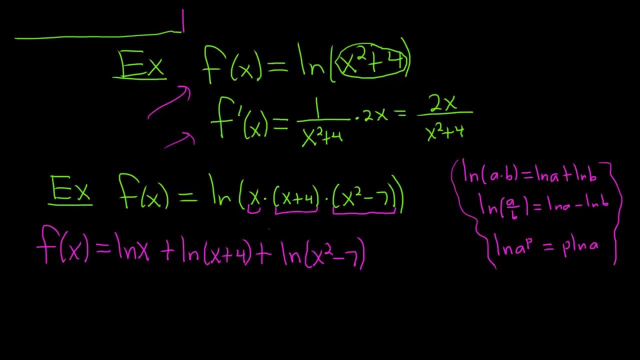 Right, We just differentiate. So we just take the derivative of each piece using that one formula. Right, The derivative of ln x is 1 over x. So for the first piece, that's exactly what we have. Right, The derivative of the natural log of x. 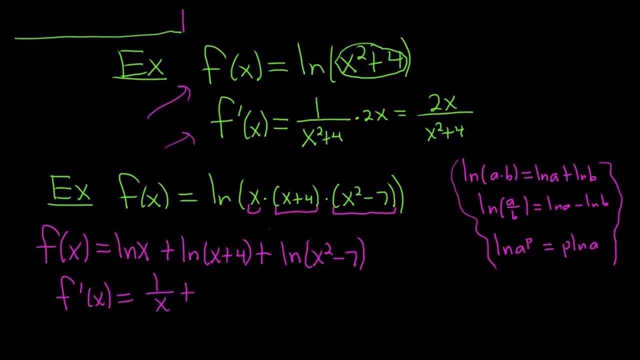 is 1 over x, Plus the second piece, it's the chain rule Right, So it's 1 over x plus 4 times the derivative of the inside function, which is simply 1. Plus 1 over x, squared minus 7.. 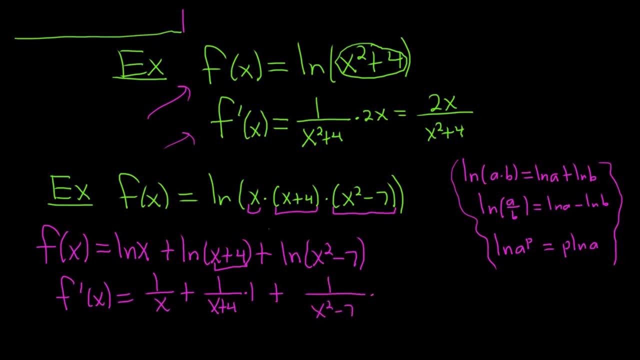 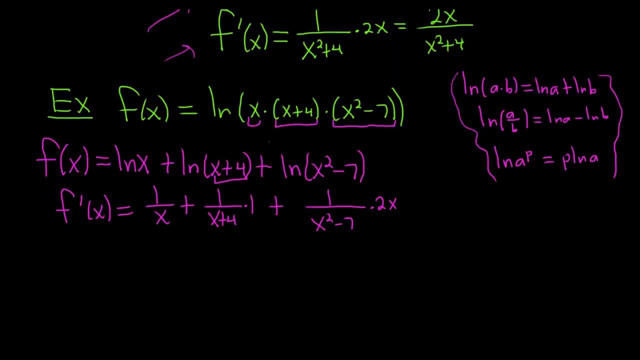 Times the derivative of the inside function, which is simply 2x. Right, The derivative of 7 is 0.. The last thing I suppose we could do is rewrite this in a nicer way. So f prime of x is equal to 1 over x. 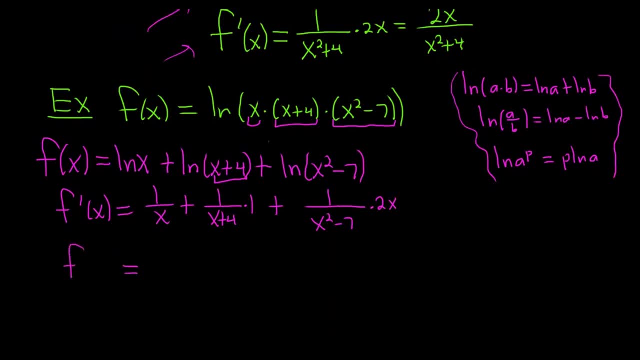 plus 1 over x plus 4.. And then we have the 2x. we can put it up top, So 2x over x squared minus 7.. And then we have the 2x: we can put it up top, So 2x. 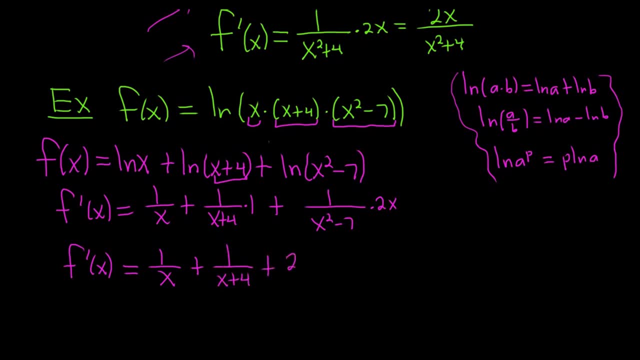 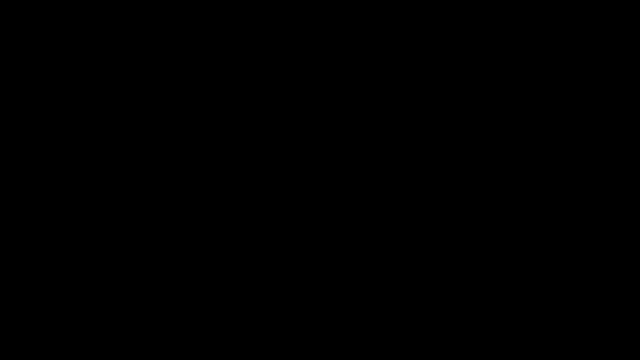 over x, squared minus 7.. And then we have 1 over x plus 1 over x plus 4.. And that is the final answer. I hope this video has been helpful in some way. In this video we're going to introduce some common integration formulas. 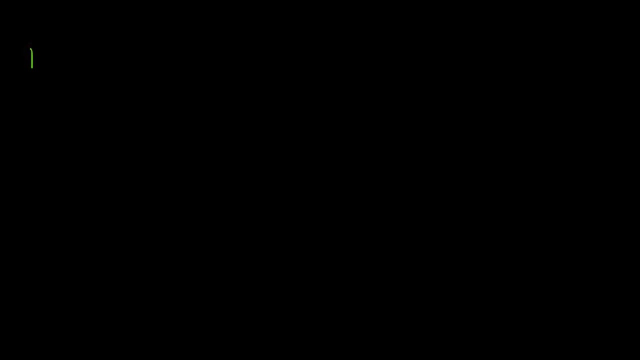 and do some examples. So the first formula is the formula for the integral of 1 over x with respect to x. So this is going to be equal to the natural log of the absolute value of x plus our constant c. Obviously, here x is not 0.. 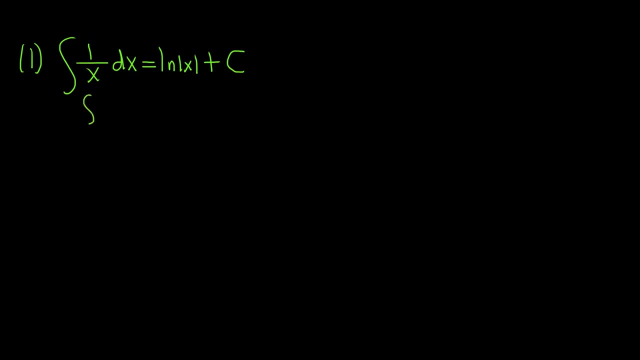 By the way, another way to write this would be the integral of x to the negative 1, dx. So recall that when you had the power rule, you would just add 1 and divide. But the power rule excluded the case where n was negative, 1, right. 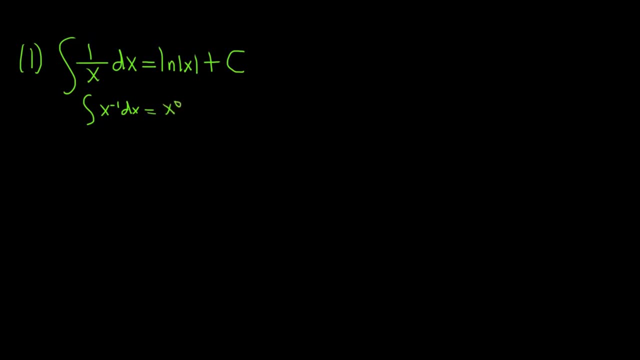 If you try to add 1 here, you get x to the 0 over 0 and that is just a fail, So that doesn't work. So this is a very useful formula. Let's do a simple example of it over here, so you see how it works. 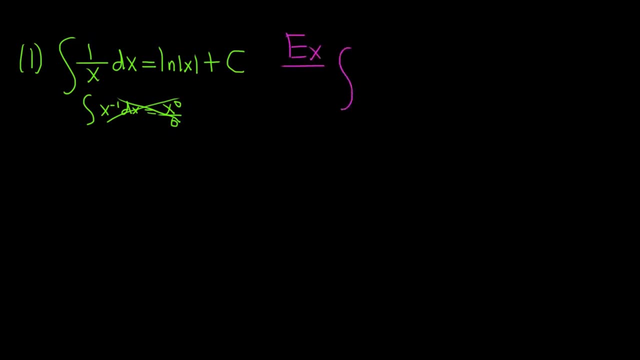 Let's say we have the indefinite integral of 1 over 2 minus x, dx. So in this case it almost looks like 1 over x. So what you would do is you would make a u substitution, You would let u be equal to. 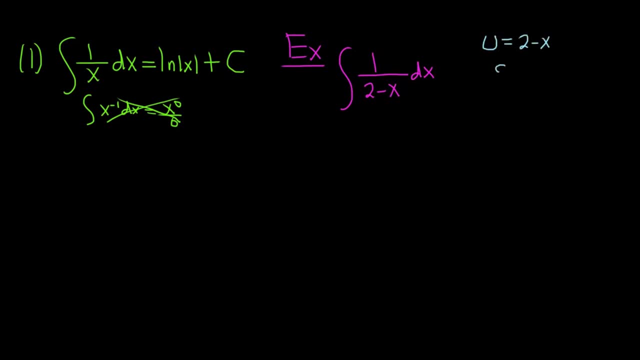 2 minus x and then du, that's equal to negative dx. taking the derivative. And recall that when you make u substitutions, you try to make this look like what's in your integrand So we don't have a negative sign in our integrand so we multiply. 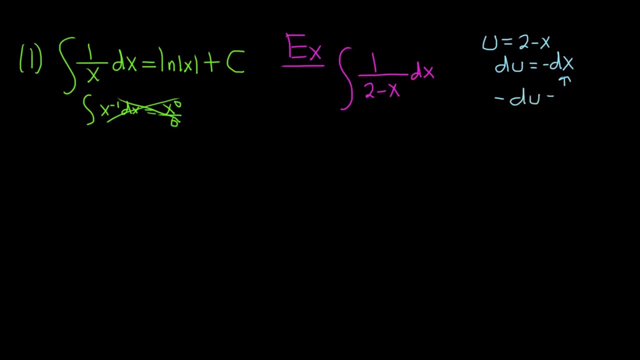 or divide both sides by negative 1.. And that brings us here. So now we can make our substitution: Our dx is negative, du, This is negative, pulling the negative out, du, and then we're left with 1 over u, And so now we can apply the formula. 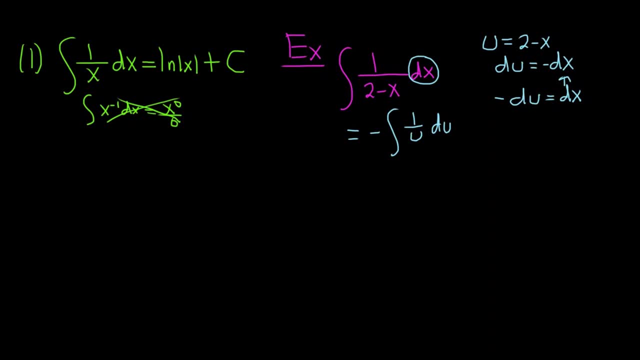 The formula says that the integral of 1 over u du is ln absolute value of u. so this is minus ln absolute value of u plus our constant c, And then you just replace u with what it is negative: ln absolute value, 2 minus x. 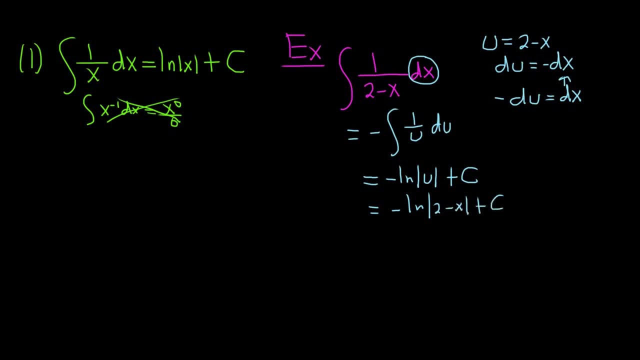 plus c. So that's an important formula. and this was just a quick, simple example. The other important formulas we're going to look at are the following: So the integral of tangent x with respect to x dx, this is going to be negative. ln. absolute value of cosine x. 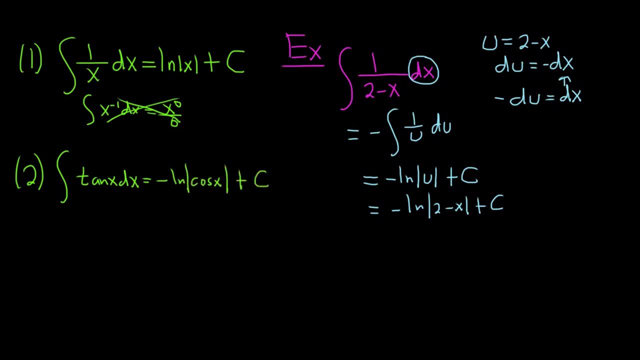 plus c, And you could work this one out using a similar technique. You could write tangent as sine over cosine and then use the formula from 1 to do it. So this is going to be negative ln. absolute value of sine x plus c. 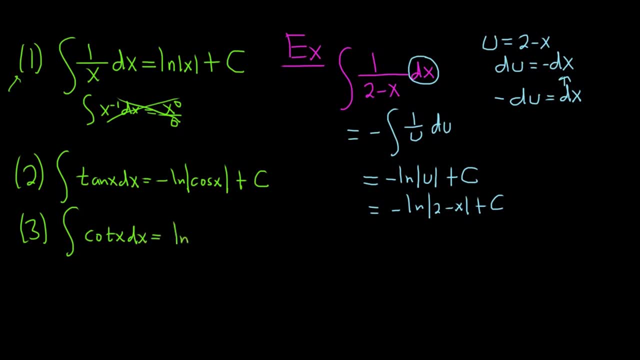 And again, if you wanted to show the work for this one, you could memorize it or show the work. I usually think about it. For example, cotangent is sine over cosine. I know no, sorry, cotangent is cosine over sine. I know that you can make. 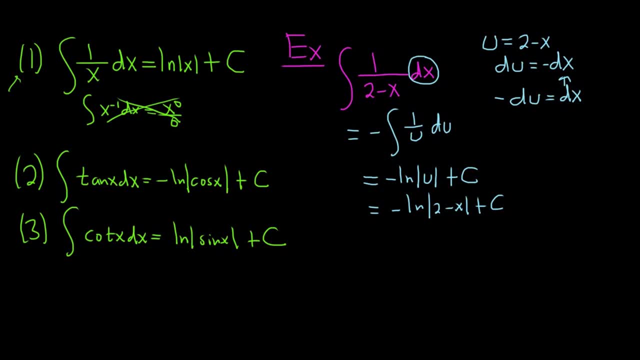 the bottom equal to u and then. so you're going to get a natural log with the sine. Here tangent is sine over cosine. the bottom is cosine. so you know you're going to get a natural log and a cosine. The negative comes because the derivative of cosine is negative sine. 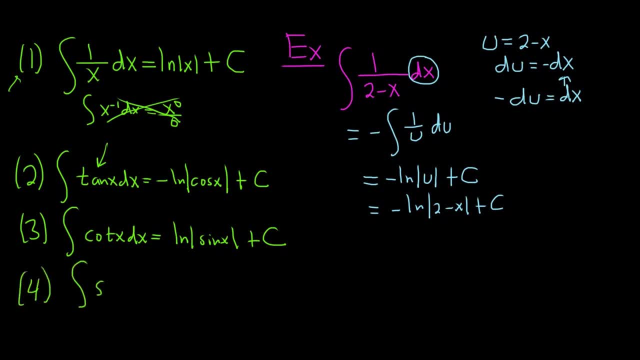 So 4. The integral of secant. this one is not so obvious, so this one takes some work. This is equal to the natural log of the absolute value of secant plus tangent x, Then plus c. So this is one that people often forget. 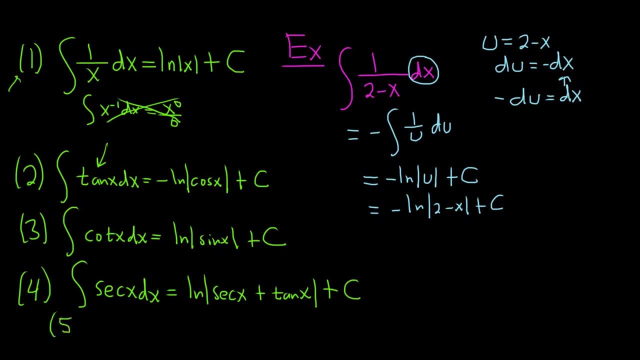 It's worth working out this problem. I have a video on this one, so you should check it out. It's a really cool problem. And last but not least, the integral of cosecant x dx. this is negative ln absolute value, cosecant x plus cotangent x. 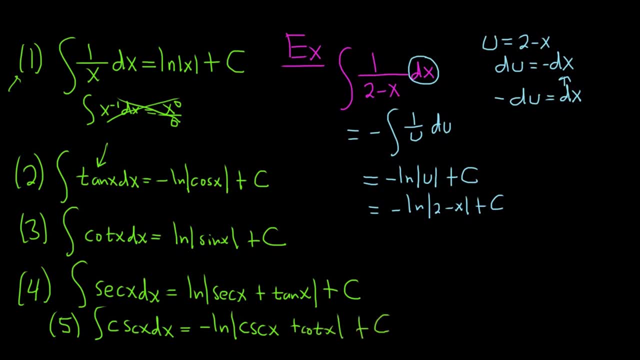 plus c. This one is very similar to secant. If you watched the video on secant, in theory you should be able to do this one And again. the ones for tangent and cotangent. let me at least briefly describe cotangent over here. 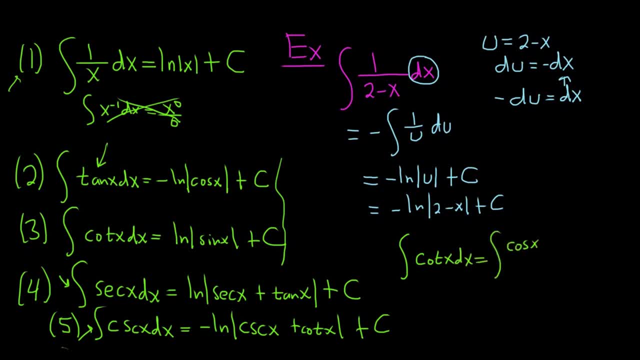 So if you have cotangent of x- dx, you would write that as cosine x over sine x. I guess I might as well finish it for you, It's not so bad. And then you let u be sine x, And then so du is simply. 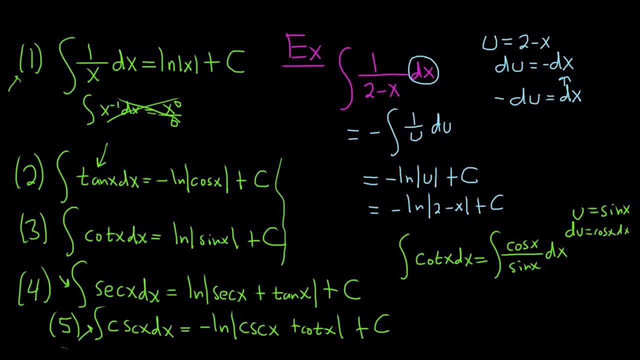 cosine x, dx. So that's your numerator. Your numerator is du, So this is just du, and then on the bottom, you get u. So it's really simple. By the way, this is the same thing as 1 over u, du, du over u is the same as. 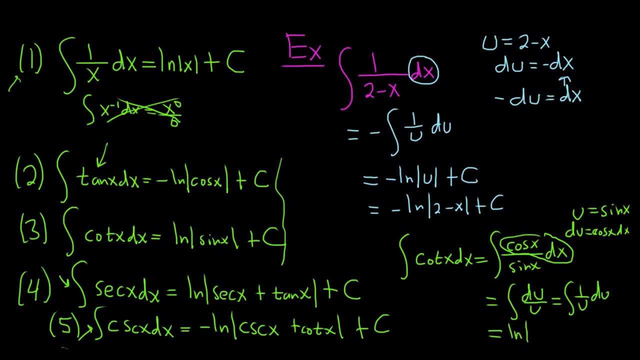 1 over u times du, And this gives you ln absolute value of u, but u is sine x. And then we have our plus c: ln absolute value of u, but u is sine x. So typically what I do when I see these tangent and cotangent- 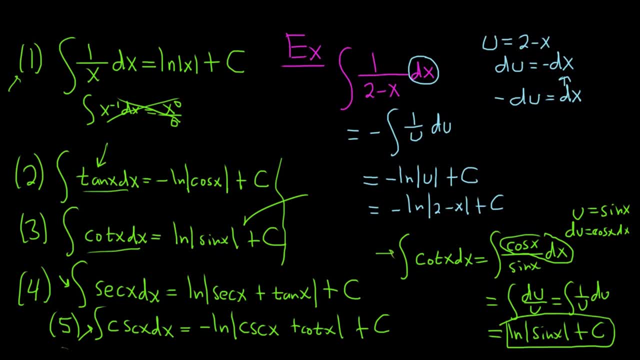 is. I think about this in my head, I just think about what's on the bottom and I go through the process and then I'm able to write it down As far as secant and cosecant. well, once you work out cosecant on your own, check out the video. 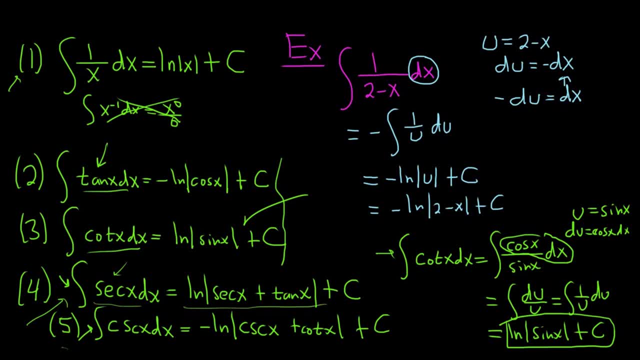 you'll never forget it. It's such a cool trick, So I hope this video has been helpful. The purpose of this video was simply to introduce some formulas and hopefully help you with some memorization techniques for memorizing these, So that's it. 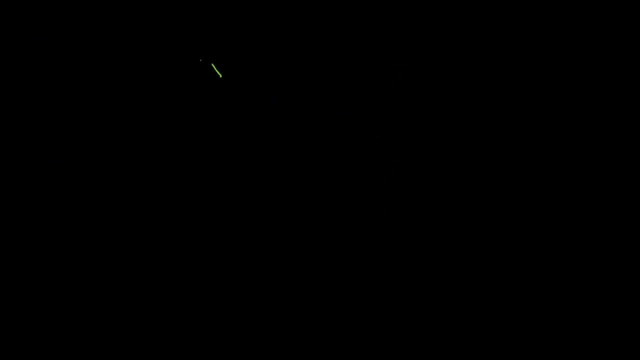 The next function that is extremely important in mathematics is called the exponential function. So f of x equals e to the x. This is called the natural exponential function. So natural exponential function, And I'll explain why it's called the natural exponential function So we can define it in this video. 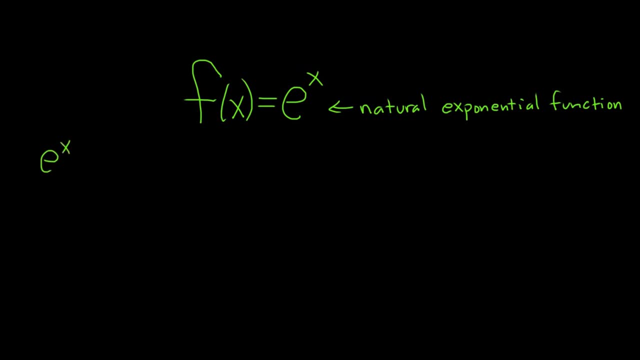 as the inverse of ln, x. So e to the x is the inverse function, is the inverse of the natural log of x. They're inverse functions So if you were to graph them, they would be symmetric across the line. y equals x. Let me do it for you over here, so you see it. 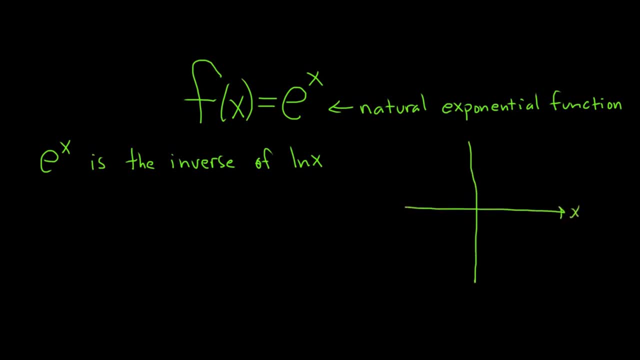 It's a beautiful picture. There's y, There's x, And then the line y equals x is right here, And then ln x will be. this light blue graph, This is the natural log of x- right here, Passes through one. 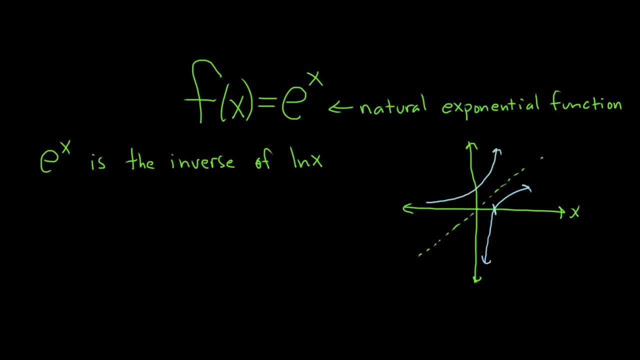 And then. so e to the x would be right. here It also passes through one. So this is e to the x And this is the natural log of x, And they're inverse functions, They undo each other, And so there is a formula. 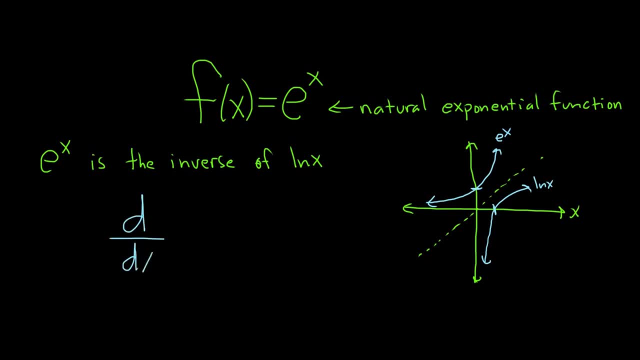 If you take the derivative with respect to x, of e to the x, you simply get e to the x. This is not true for other exponential functions like 2 to the x or 3 to the x, Hence the name natural. What does this equation mean? 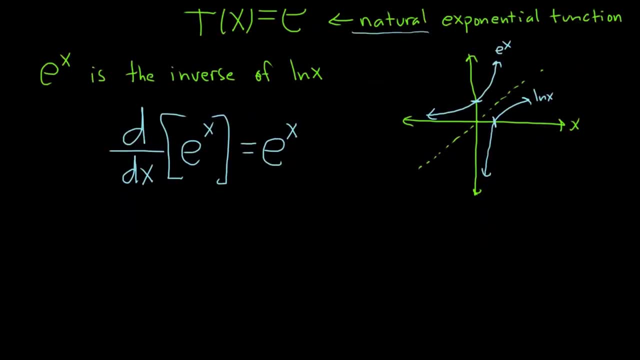 It actually means something really quite interesting. Let's draw a picture, so you see, So here is the y axis And here is the x axis, And so let me go ahead and draw the horizontal asymptote e to the x has one of those. 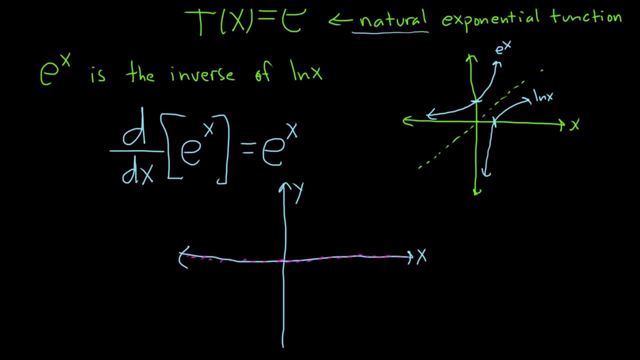 Right here at 0.. And use a different color for e. So here is the graph of e to the x Looks something like that. So we're saying the derivative of e to the x is e to the x, If you take any point on the graph. 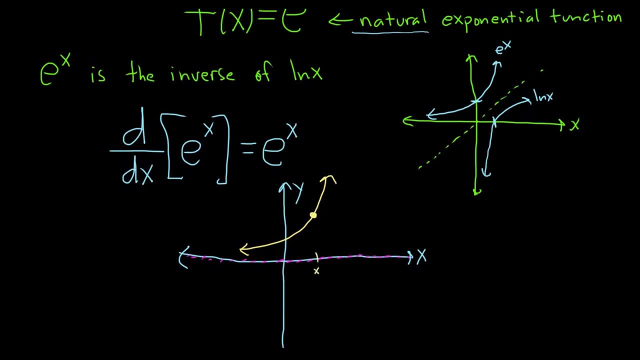 take a point here: This value here is x, And so this y value here is e to the x. So the height here is equal to e to the x. It's the y value Now if you look at the slope of the tangent line. 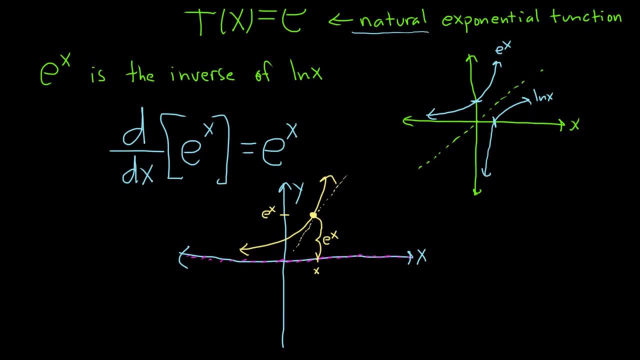 at that number. Recall that the slope of the tangent line is the derivative, So the slope of this line, so the rate of change at x, is the derivative of e to the x. But we know the derivative is the function, So the slope is equal to the e to the x. 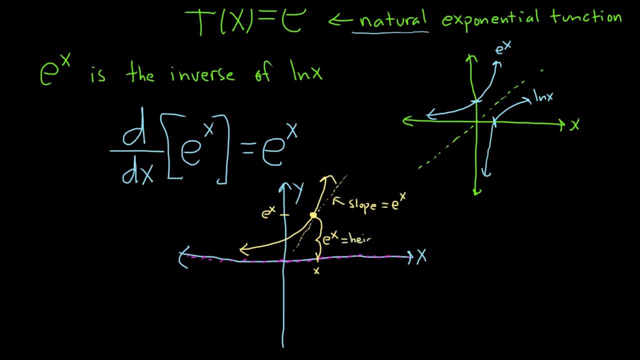 But that's also the height of the function. So e to the x is the only non-zero function in the entire world where its slope is equal to its height. It is the only function where its instantaneous rate of change is equal to the height of the graph. Hence it is the 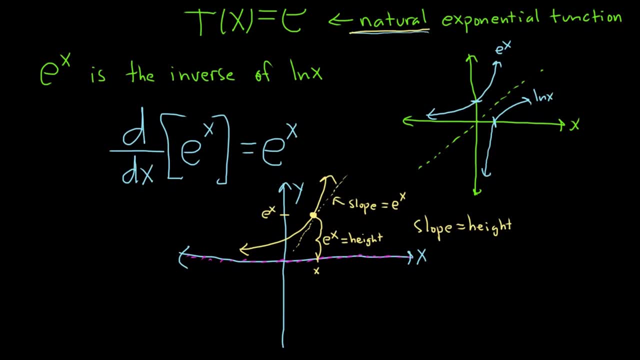 natural exponential function. It is the natural choice for the base. That's why we call this the natural logarithm. This is the natural logarithm Because it's the inverse of the natural exponential function. Let's finish this video with a quick proof of the 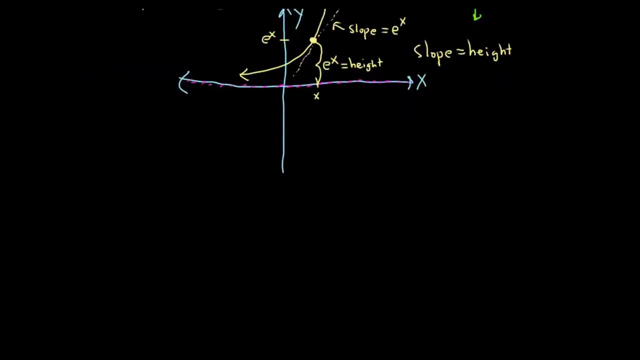 derivative of e to the x. just so you see Again, probably one of the most, if not the most important function in all of mathematics. Let's prove that the derivative of e to the x is equal to e to the x. What an amazing. 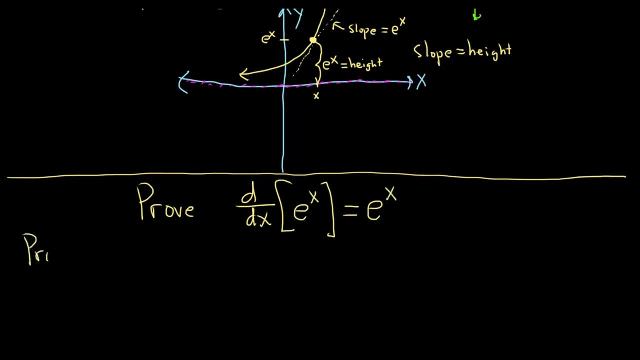 function Proof. Let's try to do it, See if I can still wing it. We'll start by calling y equal to e to the x. We have to find dy dx. We have defined e to the x as the inverse of the natural. 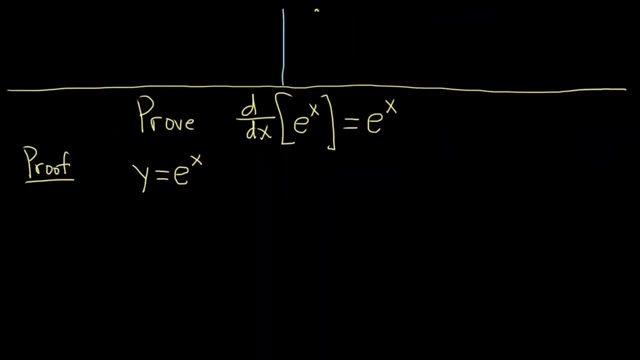 log of x. What we'll do is we'll take the natural log of both sides to somehow involve that, Taking the log, on the left hand side we get ln y and on the right hand side we get ln e to the x. So you, 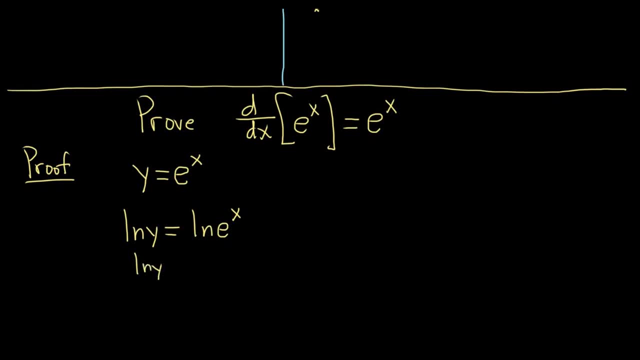 see, here we have ln, y And then here. well, e to the x and the natural log of x are inverse functions, so they undo each other. So if you take the natural log of e to the x, they cancel and you just get back x. 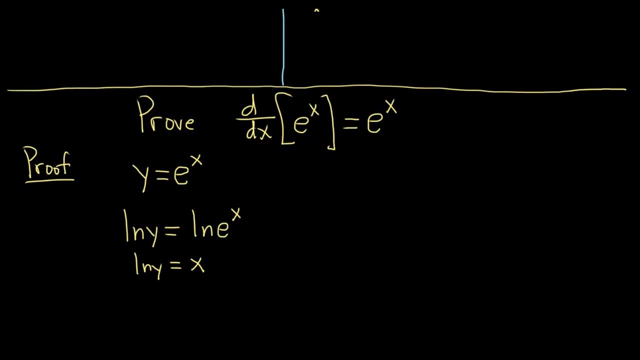 Now we'll take the derivative of both sides with respect to x, So differentiating the left hand side. so let me write that over here. We're going to differentiate, differentiate, differentiate, differentiate. we end up with 1 over y. That's the derivative of ln- y. 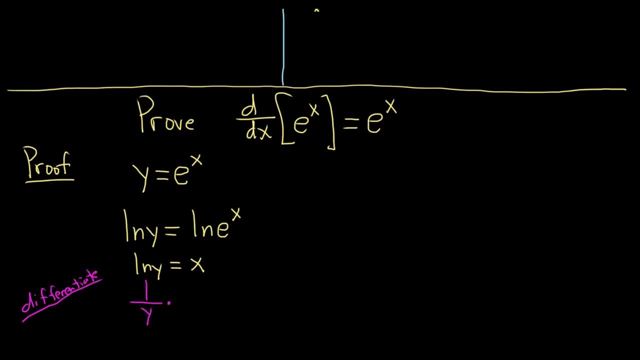 times the derivative of the inside function right Chain rule. So dy, dx, Right, we're using implicit differentiation. y is a function of x. When you take the derivative of ln- y, you write 1 over y, then you multiply by the derivative. 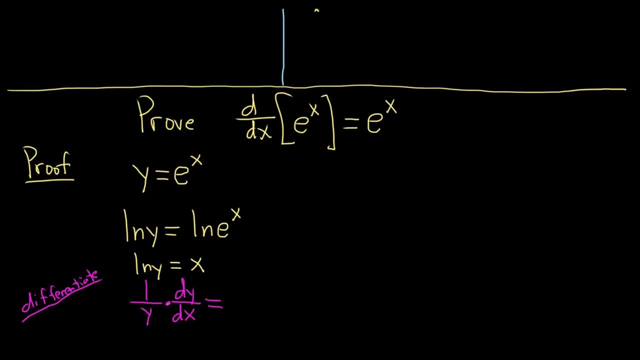 of the inside, On the right hand side, the derivative of x is 1.. Now all we'll do is multiply by y, so we end up with dy dx equal to y, So we have dy dx. Oh, look at that, we're done Equal. 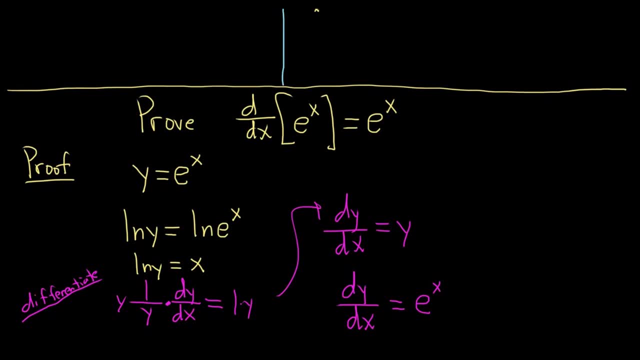 to e to the x right, Because y is equal to e to the x right. But what is y? y is e to the x. You can write it again as follows: You can write it as d, and then this is your. 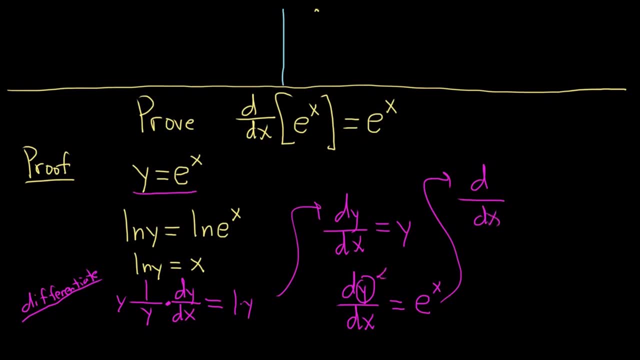 y, So dx, and then your y is e to the x. Right, that's your y, and that's equal to e to the x, and the proof is complete. So I hope this video has been enlightening or helpful in some way, and so the derivative. 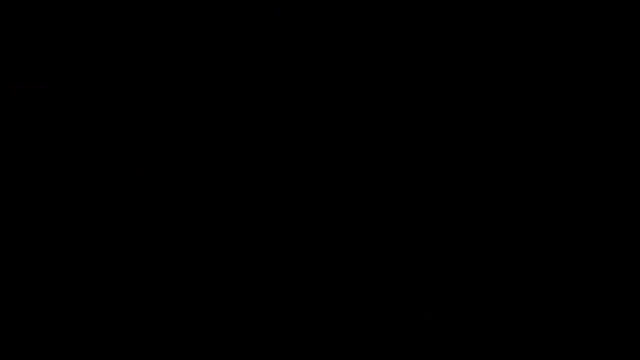 of e to the x is e to the x. Hi everyone, in this video we're going to look at some important formulas. So the first formula we're going to look at is the formula for the derivative, with respect to x, of an exponential function. 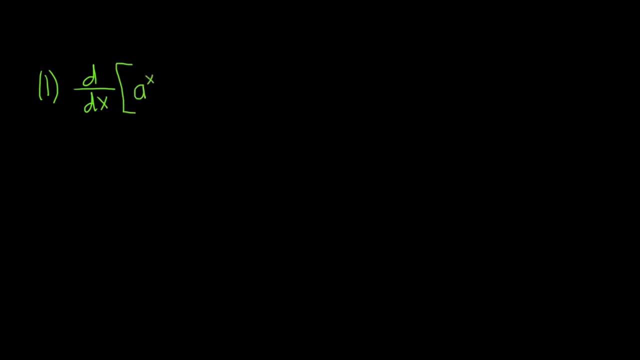 So a to the x. So a here is a base, So a here is positive and it's not equal to 1.. The formula says that this is equal to a to the x times the natural log of a. So pretty easy to memorize this formula. 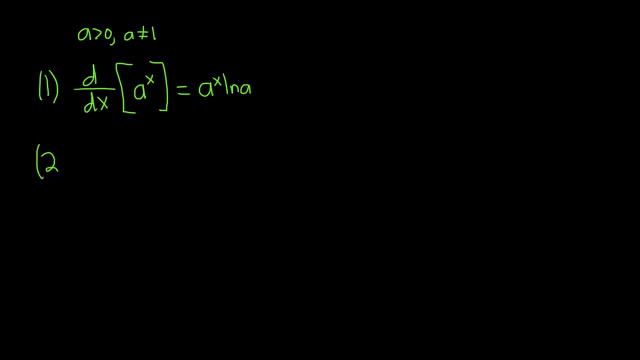 We'll prove it in a second. The second formula tells us: if we take the derivative with respect to x of the logarithm base a of x, this is equal to 1 over x times 1 over ln. a Kind of a strange formula, and we'll also prove it. 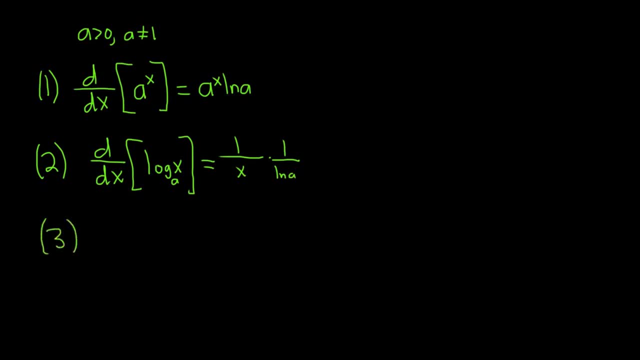 in just a few seconds. And the third formula says that if we integrate a to the x with respect to x, well, this one's pretty easy to memorize. So when you differentiate, you multiply by the natural log of a. So when you integrate, you just divide by it. 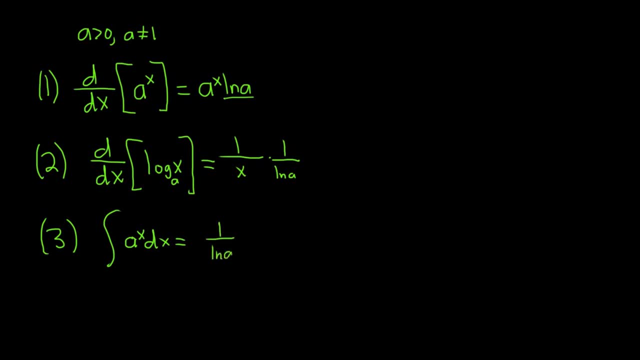 So it's 1 over ln a, and then you have a to the x plus c Or just a to the x over ln a. if you prefer to write it that way, You could write it like this: a to the x over ln a. 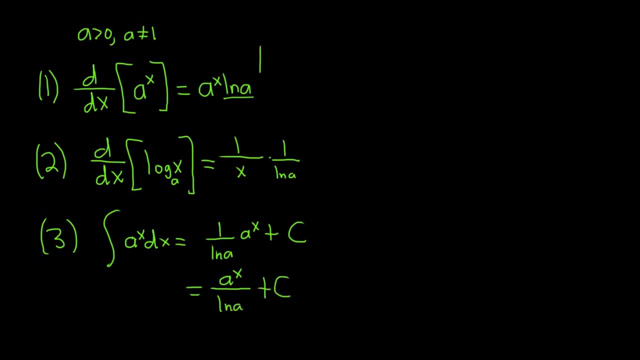 plus c. Okay, so let's go ahead and prove all of these. So let's prove one. The last one was just a few words. The last one pretty much follows from the first one, But we'll talk about that in a minute. Let's do the first one. 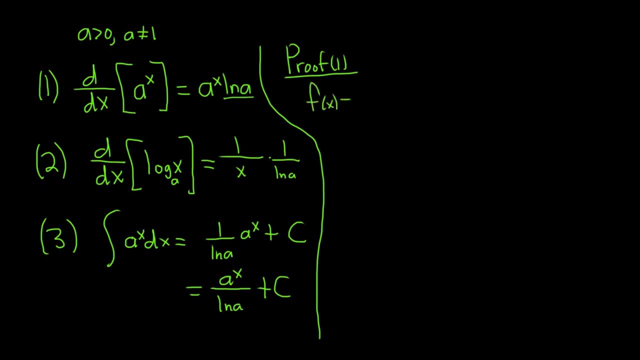 So I'm going to call this a to the x and then- I don't know if you remember this, but if you have e to the ln x, that's equal to x. So I'm going to write this as e to the ln, a to the x. 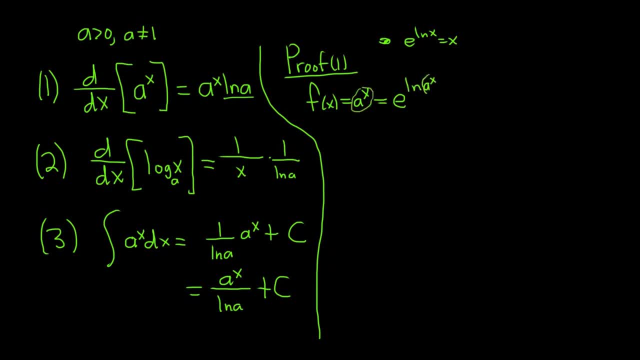 Right, That's your x, That's your x. Same thing, right, The e and the ln cancel. Then you can put the x in the front. So it's e to the x, ln, a. It's the power rule for logs. 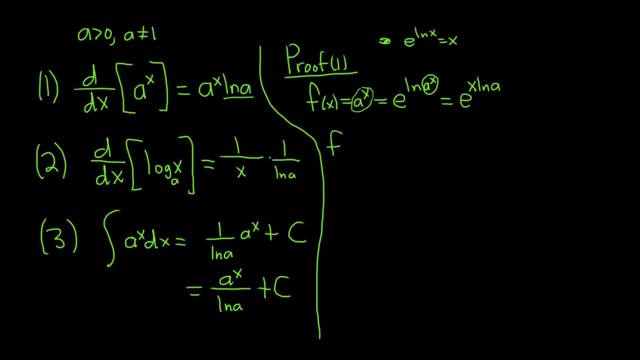 And now we're ready to differentiate this bad boy. So f, prime of x. well, the derivative of e to the x is e to the x. So here it's just e to the x, ln a times the derivative of the inside. So we have to think about. 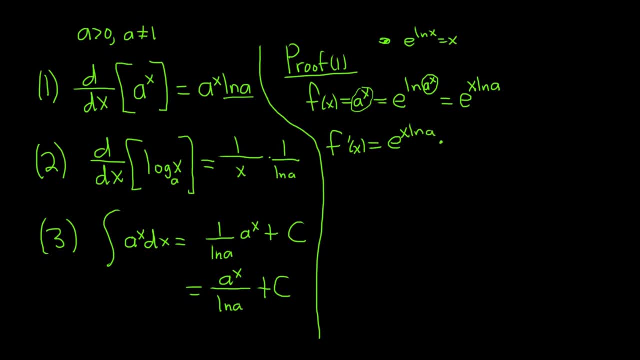 what the derivative of x ln a is. Well, ln a is a number, So the derivative of x- ln a is just ln a. The derivative of x is one and the ln a is a constant. So it hangs out. Now, what we can do is we can bring the x. 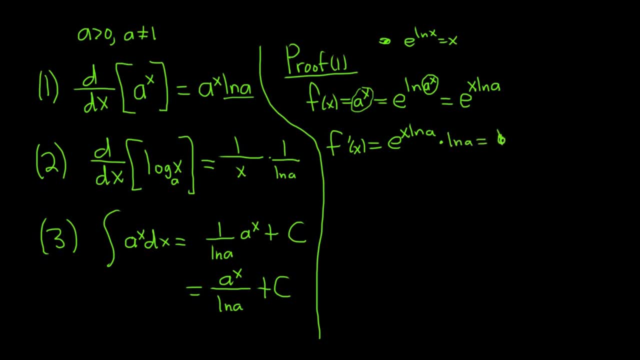 back upstairs. I'm going to put the ln a. well, I'll leave it there. So I'll put the x back upstairs like this, And we have the ln a here And these cancel, And so you end up with a to the x. 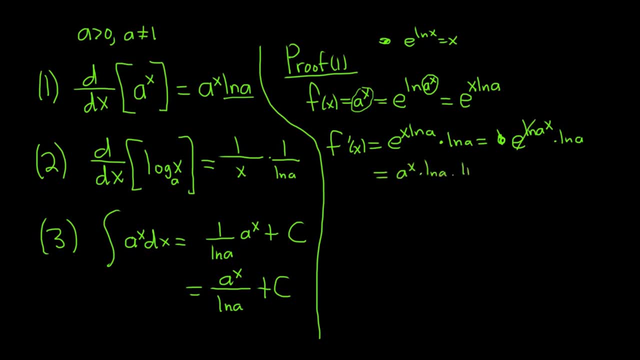 times ln, a. And that completes the proof of one. Let's do the proof of two. So proof two. So the proof two again. we'll start by calling the function a name. We'll call it f of x, And it's equal to the logarithm base. 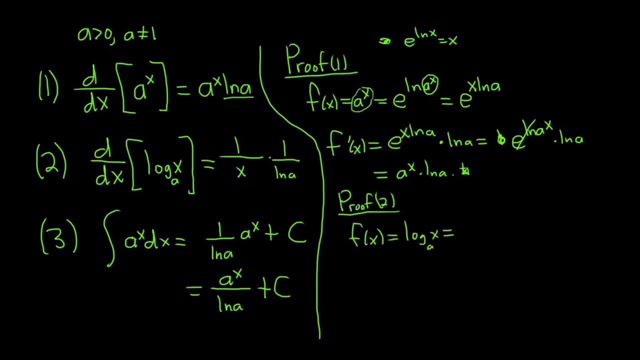 a of x, And now we're going to use the super powerful change of base formula. It says we can write this as the natural log of x over the natural log of a, And again, for convenience, perhaps we can write it like this. This will make it a little more clear. 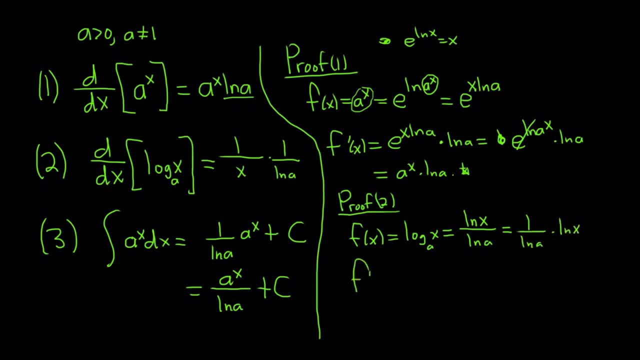 And now we take the derivative. Well, this one over ln a is a constant, so it hangs out. And the derivative of ln x is one over x, And that completes the proof. That's exactly what we have over here. So the first two proofs. 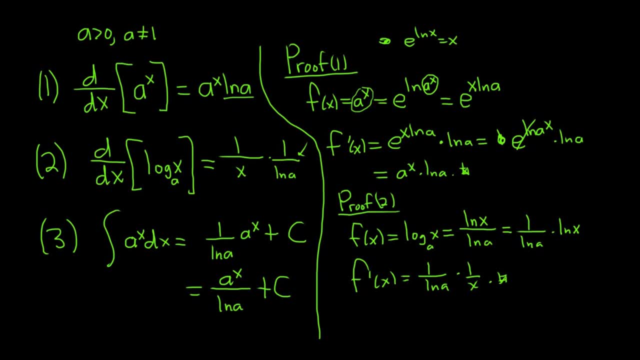 aren't so bad. The third one again, is kind of a consequence. Let's look at it. Let me see if I can squeeze it in over here. So we're saying that the integral of a to the x is this. So basically, if you multiply- 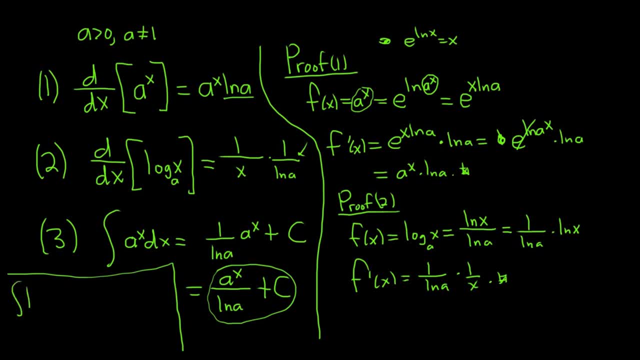 both sides of this. by ln a, you would get ln a. We're not going to prove it, but maybe just talk about it. You would get this And you ask yourself: what's a function? whose derivative is this? Well, a to the x. 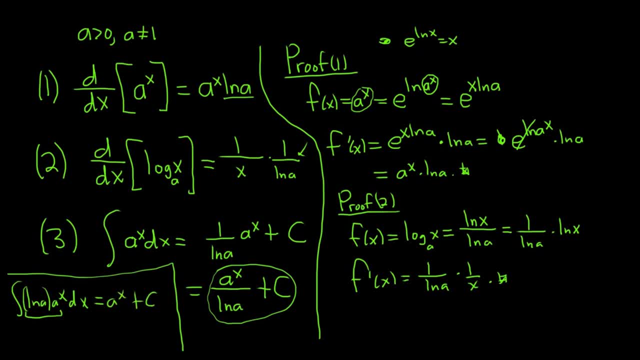 Because the derivative of a to the x is a to the x, ln, a. So you start with this and then you divide both sides by the natural log of a and you get this So really easy to memorize. when you differentiate, you multiply, when you integrate, you divide. 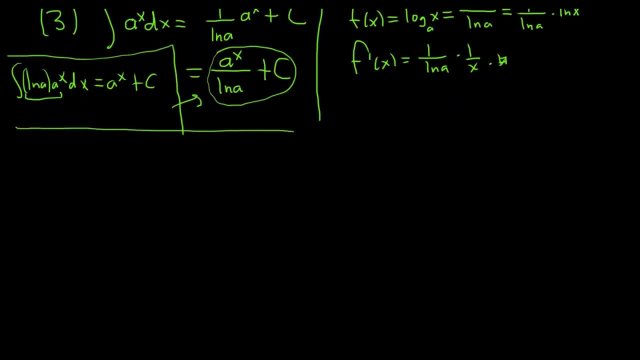 Let's do just three simple, simple, simple, easy examples of this. Let's find some stuff. Let's find d dx of 2 to the x, Really basic, So let's see. So this will be 2 to the x and then ln 2.. 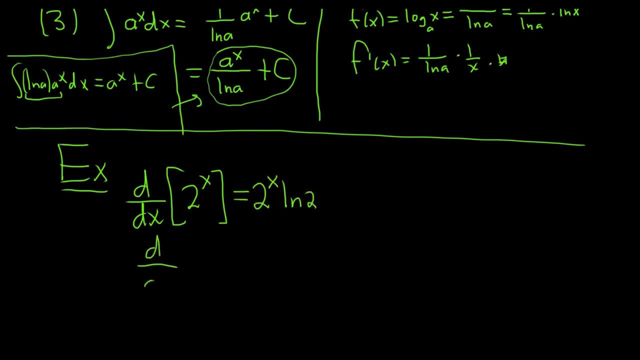 Boom, we're done. Let's find one we already know. Let's find e to the x. We know, e to the x is just e to the x. Let's pretend we're just using this formula: We get e to the x, ln e. 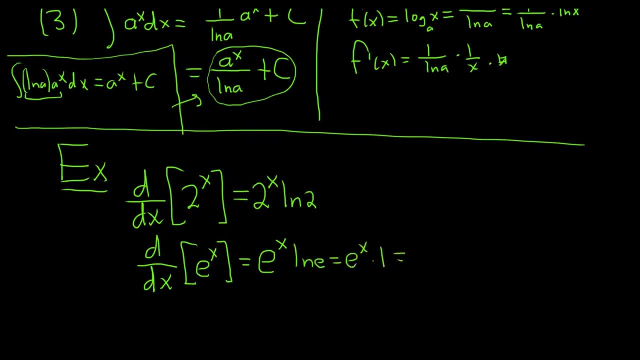 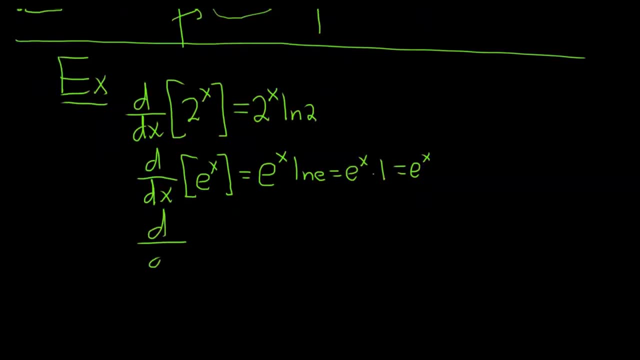 ln, e is 1, so we get e to the x times 1, so we get e to the x. So it certainly agrees with what we already know. Let's try another one: d, dx. how about log base 2 of x? So using the formula, 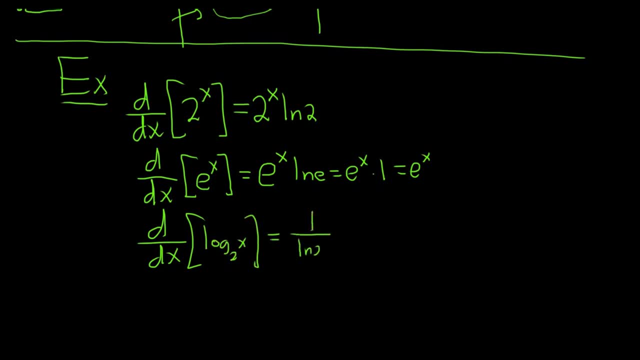 this is 1 over ln 2 times 1 over x, And you can put the 1 over ln 2 in the front or you can put it in the back, It's up to you. So when you differentiate, you multiply, and then when you integrate. 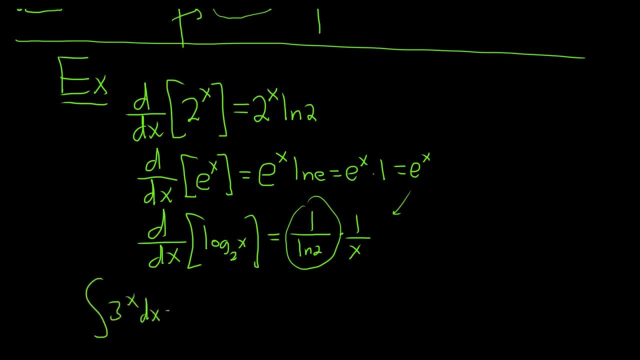 which we'll do now. you divide, So it's 1 over ln 3, 3 to the x plus c. So when you integrate exponentials, you divide by the ln of the base. When you differentiate, you multiply by ln of the base. 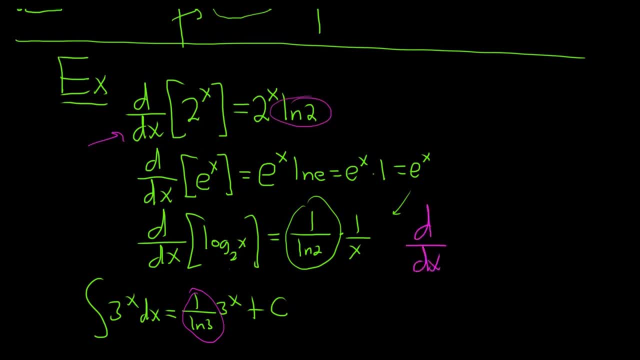 So one more just to make the point. Say we had d dx of 4 to the x. we're differentiating, so we multiply by the natural log of the base. But say again one more time: say we had to integrate, then you would divide by the natural log. 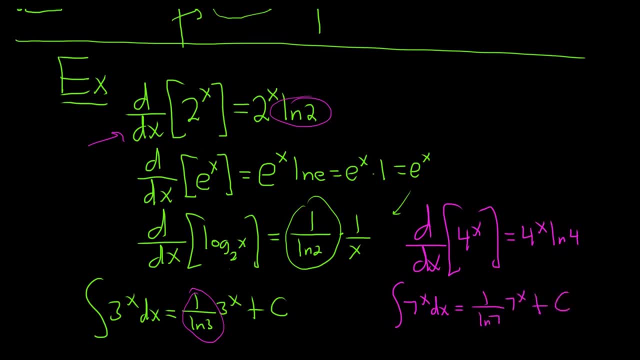 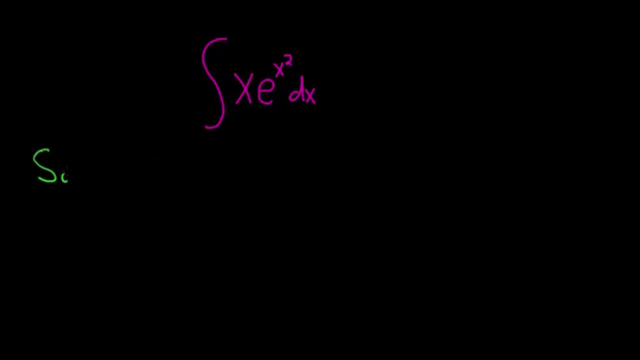 of the base. Just wanted to do a couple quick, easy examples to help get you started before you see harder problems. So I hope this video has been helpful. That's it. We have the integral of x times e to the x squared. Let's go ahead and try to work it out. 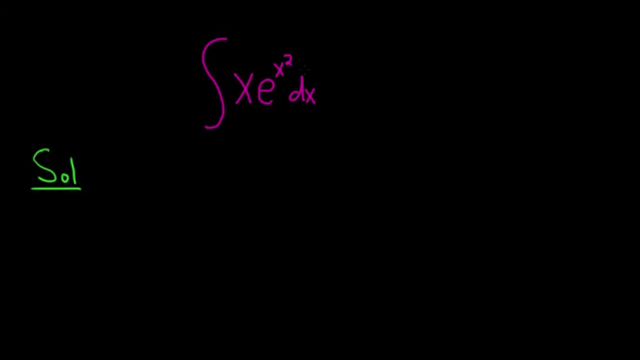 So when you see a problem like this, the e to the x squared sticks out. so if you let u be x squared, something nice happens. When you compute the derivative of both sides, you get du, and then here you get 2x, dx. So it. 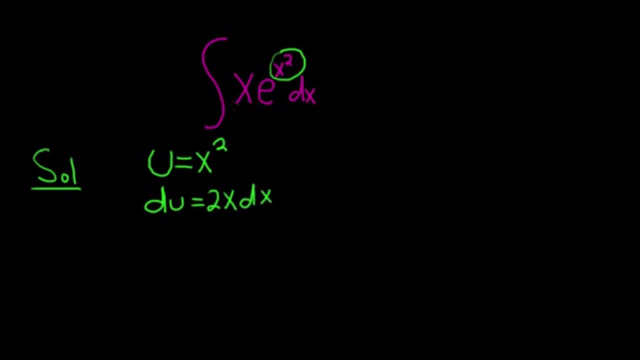 almost looks like what you have in your problem, in your integrand Right. here you have x dx, here you have 2x dx, So you have to make it match. So what you do is you divide both sides by 2.. So when you do that, you end up with: 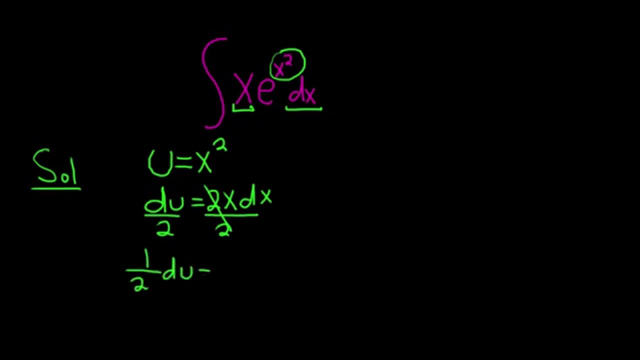 one half du equals x dx, And then now you can go ahead and make the substitution, So x dx is our one half du. So let's go ahead and make that replacement. So we have one half integral, and then here we have du. 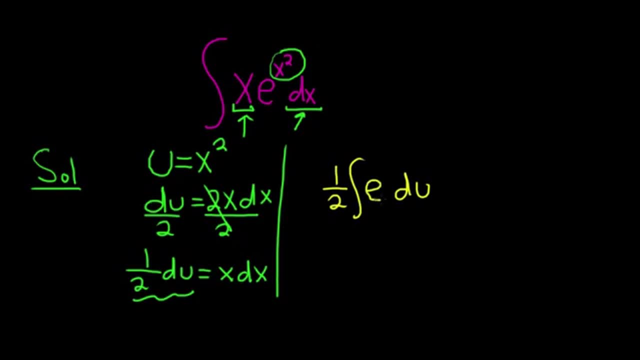 And then we have e to the x squared. We said x squared was u, so it's just e to the u. Now we can integrate. Everyone knows that the integral of e to the u is u to the u, So it's e to the u. 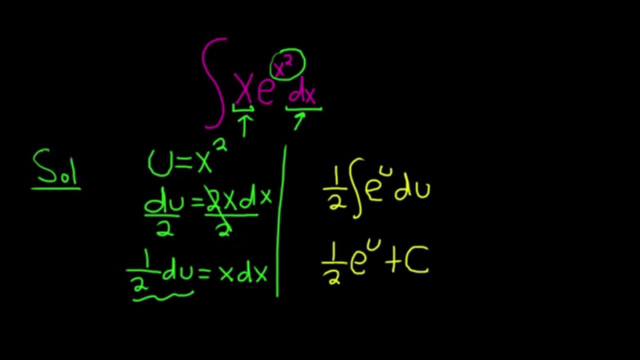 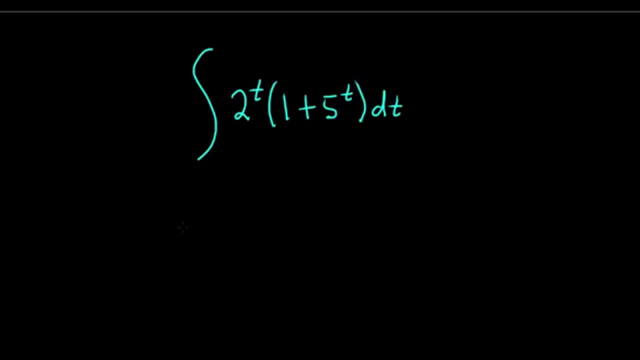 plus c, And the very last thing to do is replace u with x squared. So this is one half e to the x squared, and then plus our constant c. That's it, And I hope this video has been helpful. Integrate 2 to the t. 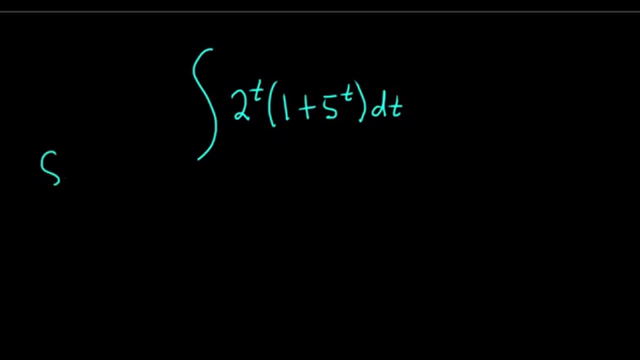 times 1 plus 5.. That's the 5 to the t solution. So we have a product here and there is no product rule for integration. So maybe we can try just multiplying the 2 to the t through, So 2 to the t times 1. 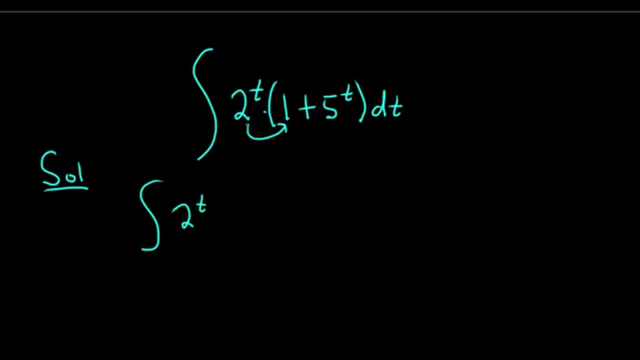 is 2 to the t And 2 to the t times 5 to the t is just 2 to the t times 5 to the t dt. So we can integrate 2 to the t. There's a formula, If you have a. 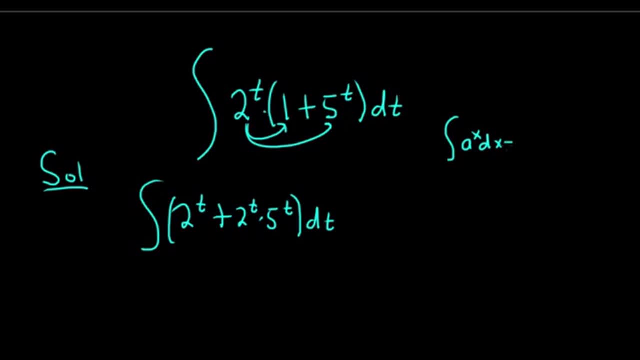 to the x dx. the formula is that this is equal to a to the x divided by the natural log of a plus c. That's the formula to integrate a to the x. However, the 2 to the t times 5 to the t is a problem. 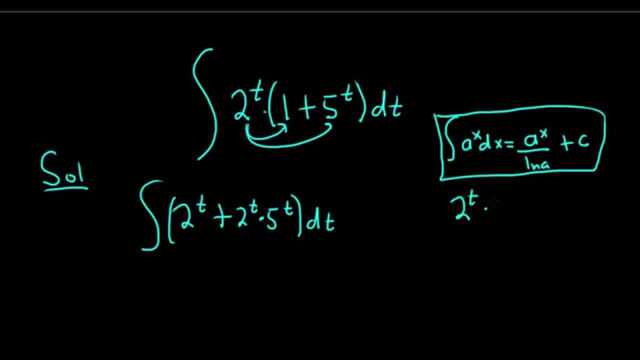 So here's the thing I think we can do. We can rewrite this using properties of exponents: 2 to the t times 5 to the t is really 2 times 5 to the t. It's a property of exponents. 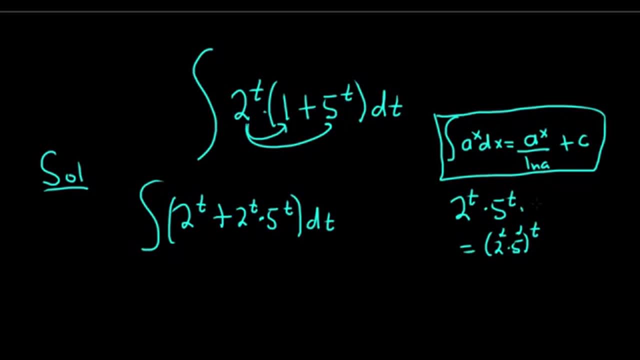 If you go backwards, you just raise each piece to the t-th power and you get this: 2 times 5 is 10.. So this is just 10 to the t. So, rewriting what we have, We have the integral of parentheses 2 to the t. 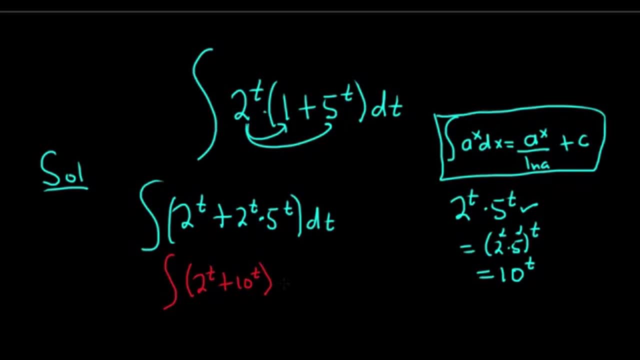 plus 10 to the t, and then we have the dt, And now we just integrate each piece using our formula. So the first one gives us 2 to the t divided by the natural log of the base, so ln 2 plus. and the second one is 10 to the t. 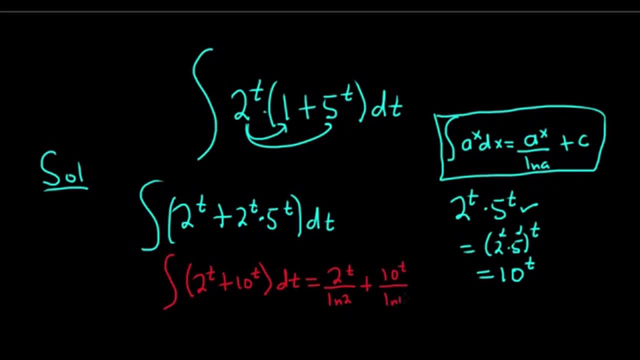 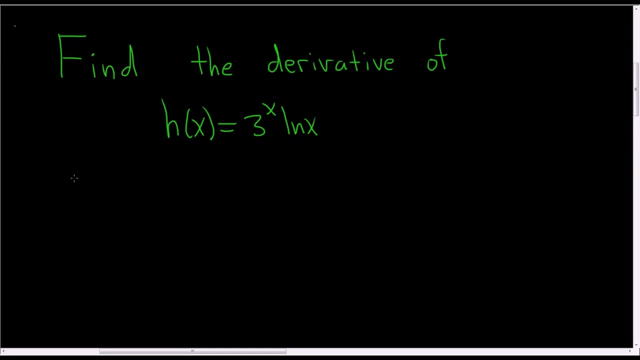 again divided by the natural log of the base, so ln 10 plus our arbitrary constant of integration, capital C. I hope that made sense. That's it. In this problem we have to find a derivative and we will use the product rule. The product rule says that if you have 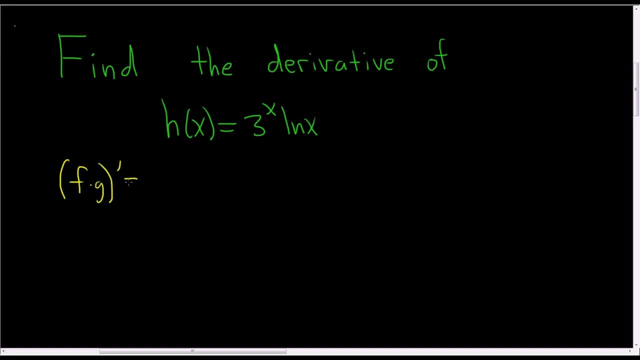 f times g and you take the derivative. well, the way I do it is, I think of f as the first factor and g as the second factor, And so it's the derivative of the first times, the second plus the first times, the derivative of the second. 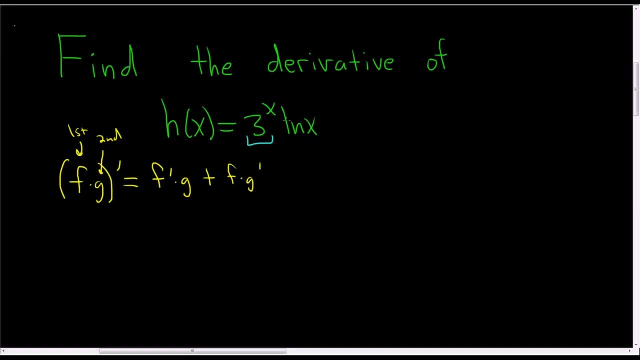 So in this problem, this is our first piece and this is our second piece. So, h prime of x. well, the derivative of the x is 3 to the x natural log 3, so that is our f prime. that's this one times the second factor. 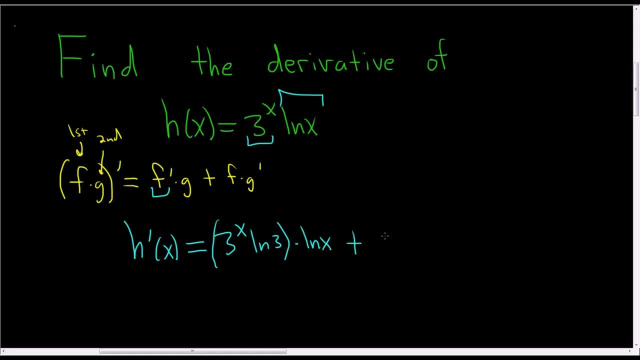 so the natural log of x plus the first factor, so 3 to the x times the derivative of the second factor. the derivative of the natural log of x is just 1 over x, And that's pretty much it. there's not much we can do here. 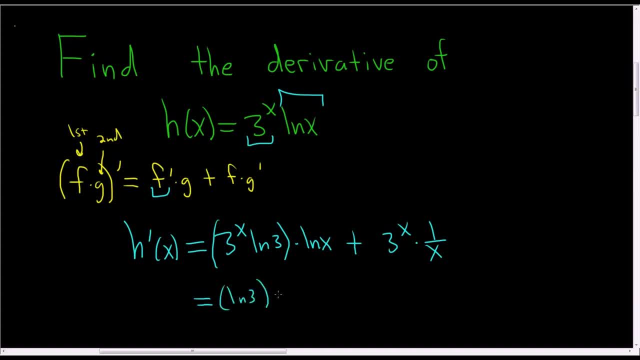 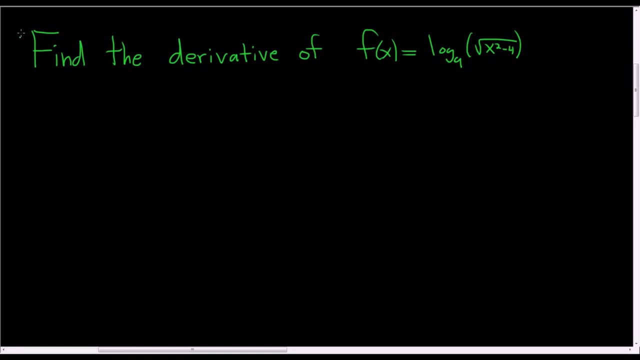 maybe we can write it as ln 3: 3 to the x, ln x plus maybe 3 to the x divided by x, and that's it. I hope this helps Find the derivative of the log base 9 of the square root of x squared minus 4. solution. 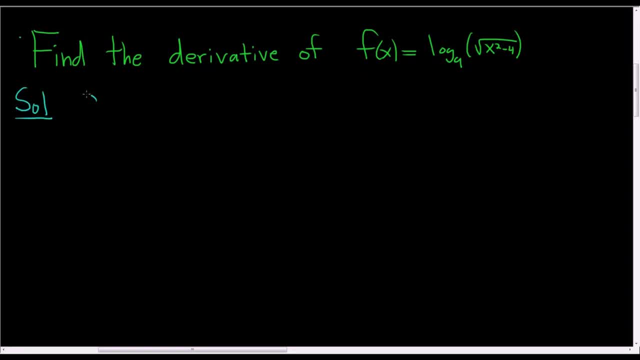 Before we can take the derivative, or rather, it's a good idea to rewrite this before we take the derivative. you can just take the derivative, but it's probably better to rewrite this to the square root function in another way. we can write this as x squared minus 4. 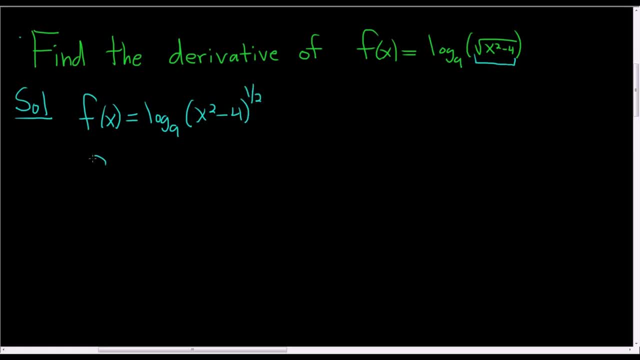 to the 1 half and then now we can bring the 1 half down. so this is still f of x and bringing the 1 half down using the power rule. we end up with this, and the reason we did that is because, if you just take the derivative, 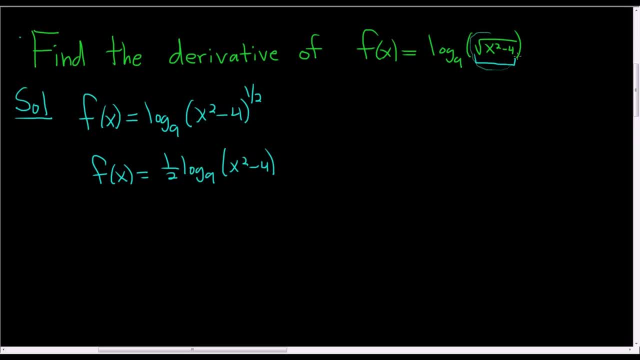 right away. you have to use the chain rule. then we have to take the derivative of the square root, and that's not very fun. so first we write it in exponent form and then we bring the 1 half down. so a lot of times in these problems with logs, 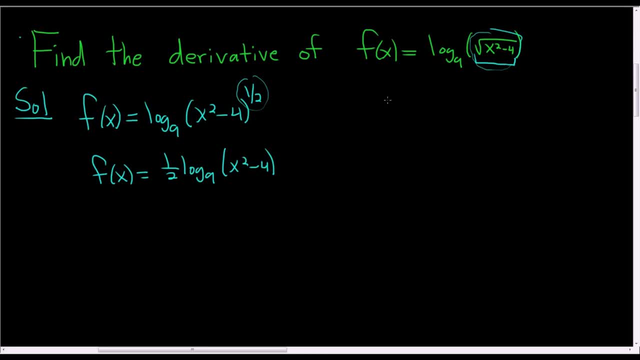 you want to rewrite them first, then take the derivative. so first recall that the derivative of the log base 9 of x, this is 1 over x, 1 over ln 9. so in this case it's very similar, except we have x squared minus 4. 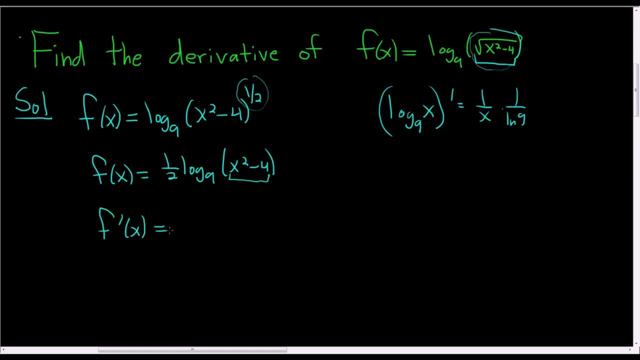 so we will have to use the chain rule. so f prime of x, this is 1 half 1 over x squared minus 4. so whatever is there, you write it, and then 1 over ln 9, and now we use the chain rule. now we multiply by the derivative of x squared minus 4.